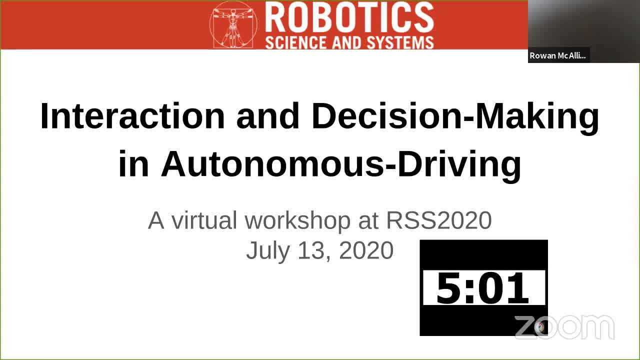 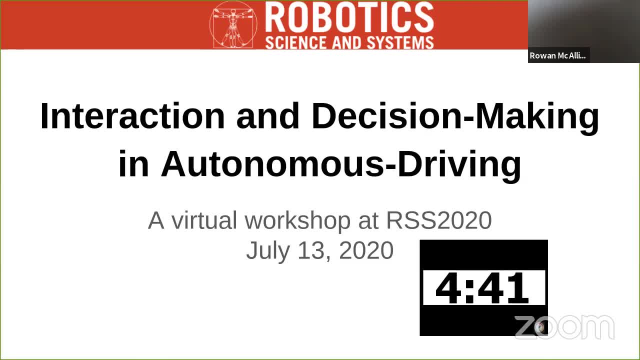 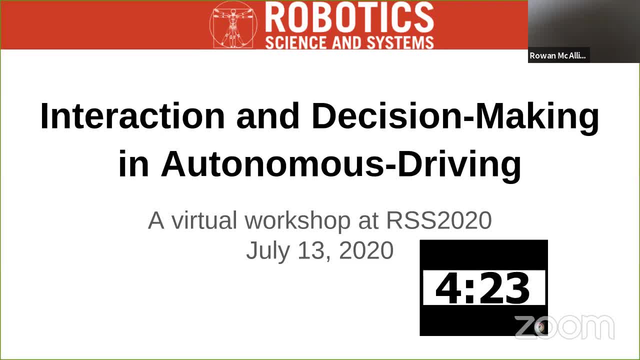 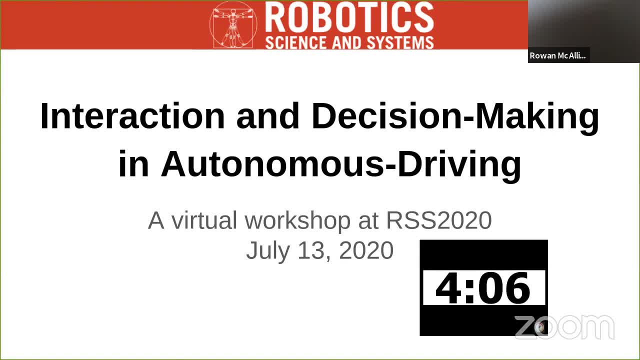 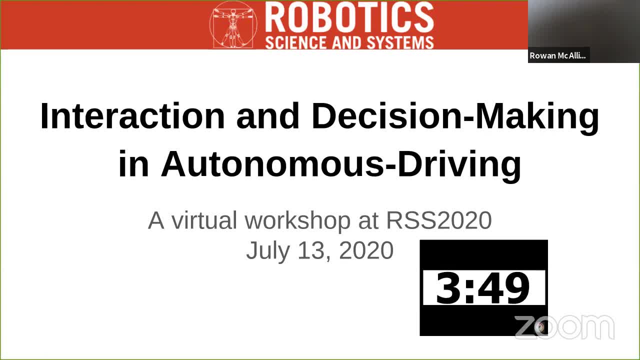 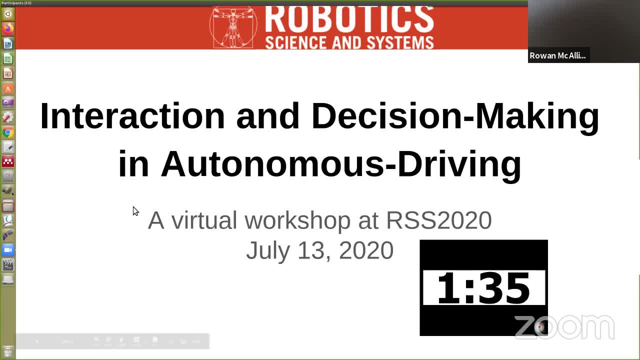 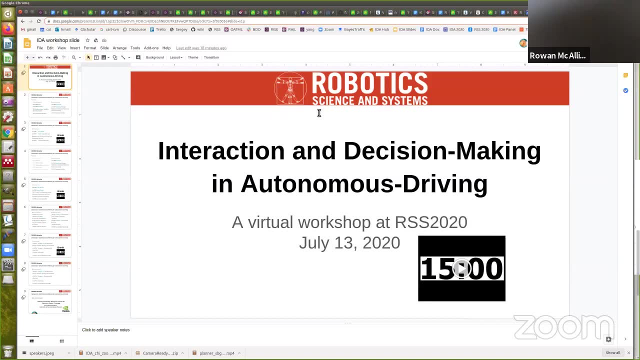 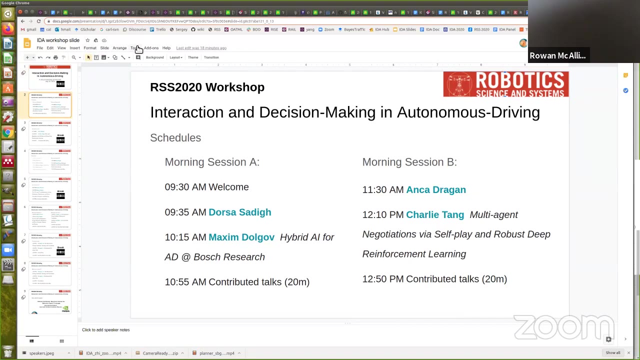 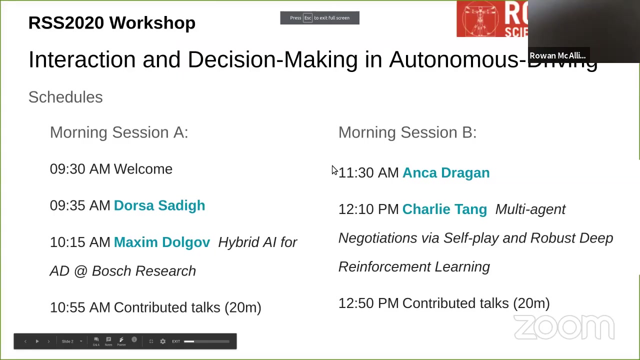 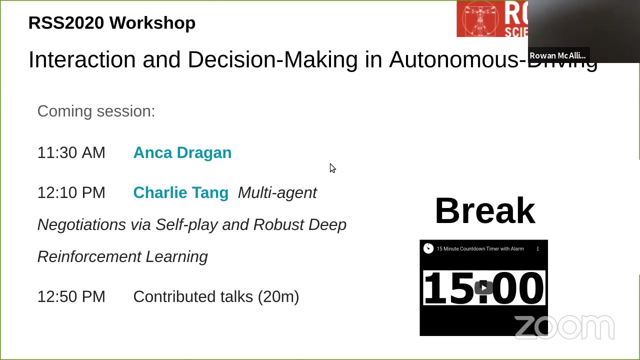 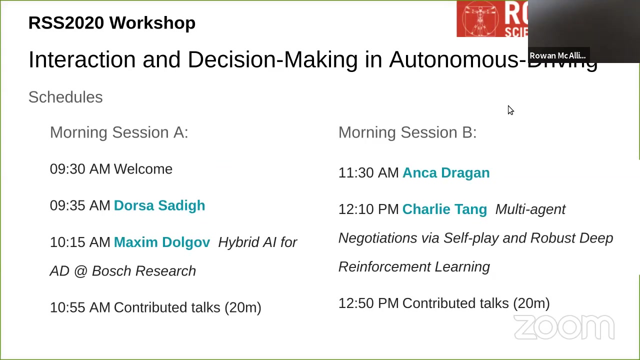 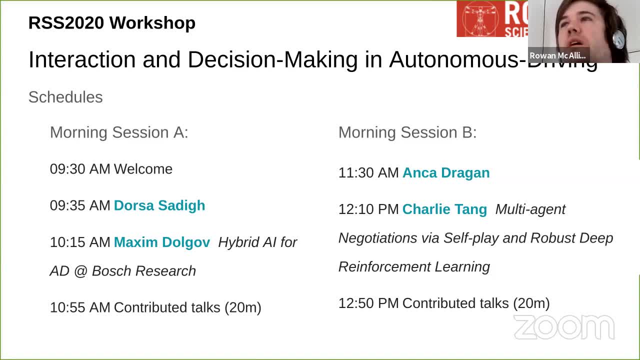 so if you have any questions during the day, you can ask any of us and we'll do our best to respond. We also have some sponsorship today for a best paper, So NVIDIA Corporation was happy enough to sponsor us. So there's a best paper prize, a Titan RTX. 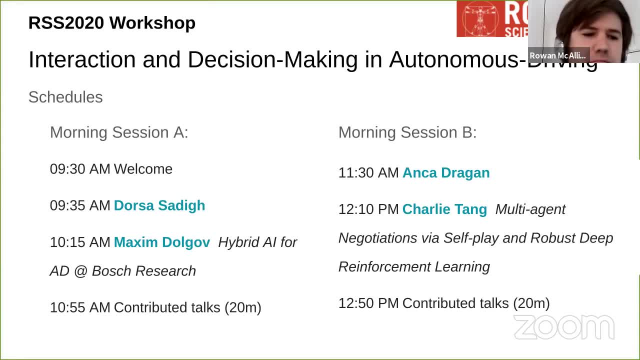 which we'll announce at the end of the day. The way in which it'll work today is speakers will present for about 30 minutes and then there'll be about 10 minutes of questions. If you have any questions during their talk, just enter them into the Zoom chat. 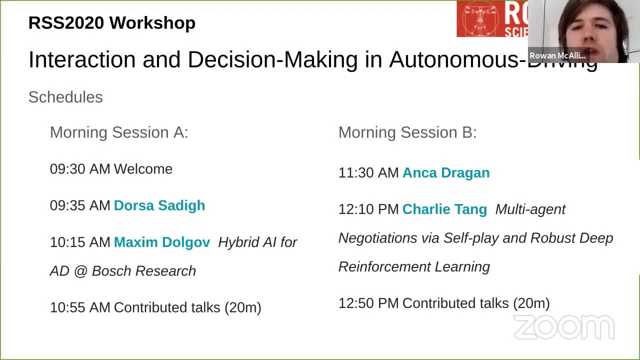 and then we will then go through that Zoom chat after the speaker presents their material and selects questions from there. So feel free to write away in the Zoom chat questions, as the speaker maybe says something that you want to ask a question about. Okay, so I think we're almost ready to start. I also want to draw your attention to the 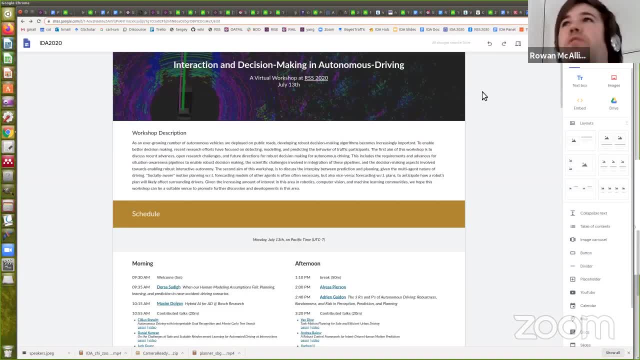 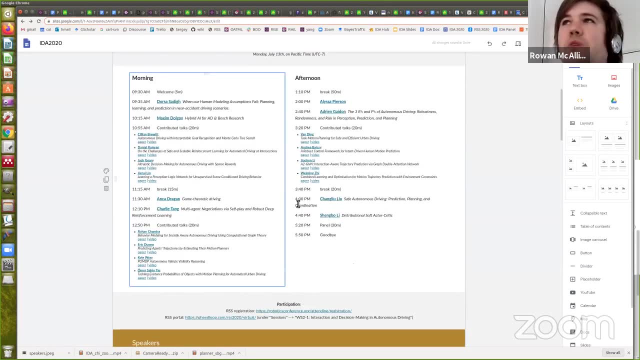 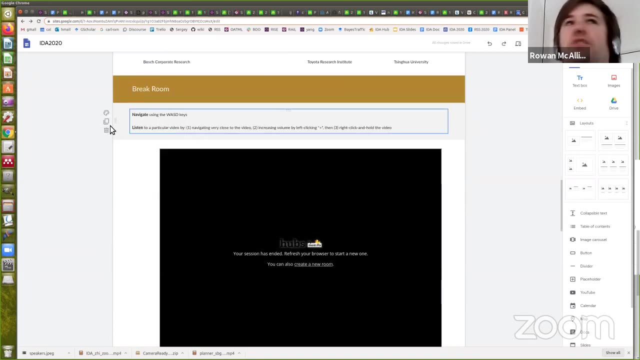 website, So we've got the schedule. Something we were going to try during the breaks was a little bit of an experiment, but if you scroll down here, there's a break room, And so here what you'll be able to see is a virtual environment with everyone's videos, And it can be a little bit noisy. 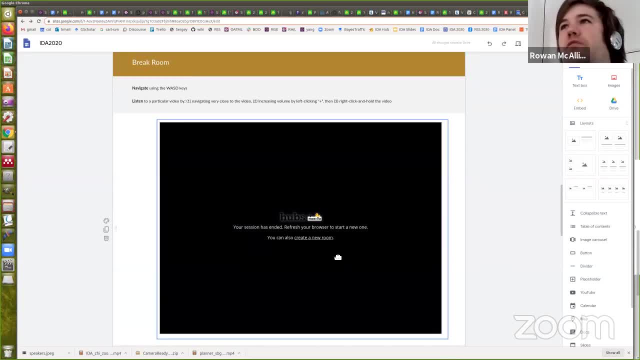 but if you follow the instructions you'll be able to see that. it's a virtual environment with everyone's videos and it can be a little bit noisy, but if you follow the instructions, you'll be able to follow the instructions. at the top You should be able to hear videos that you're interested in. 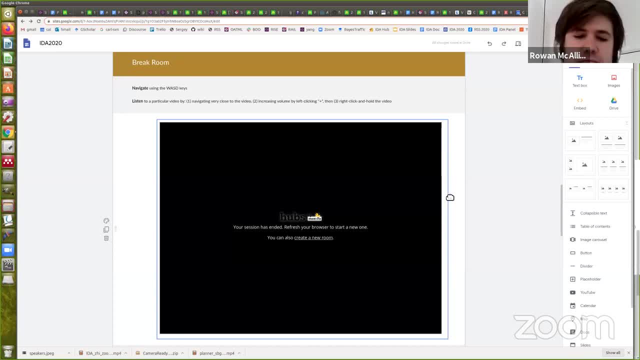 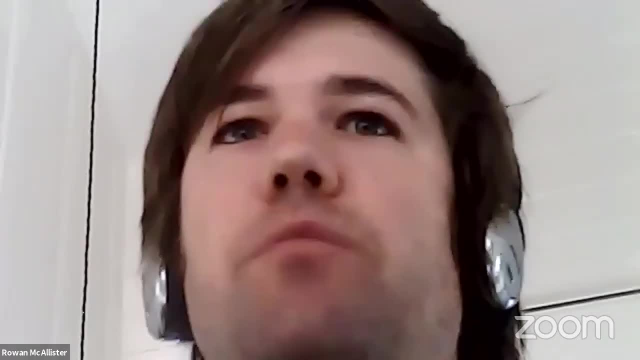 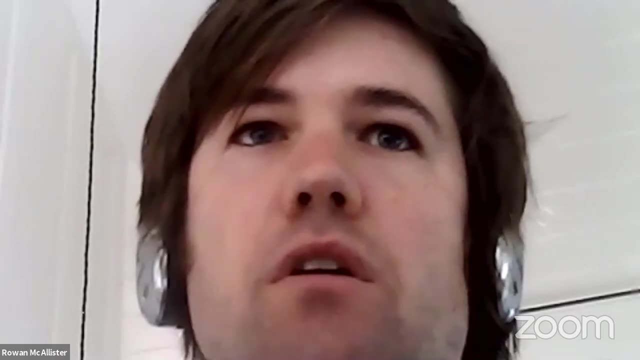 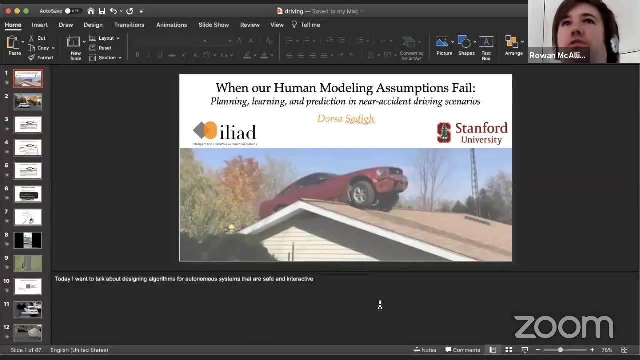 and be able to interact with other people. Okay, I think I am going to stop share screening, So our first speaker, Dorsa, will be able to share screen. Dorsa, whenever you're ready, you are able to share screen. 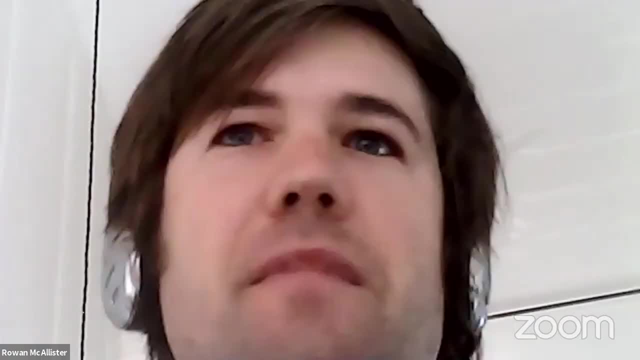 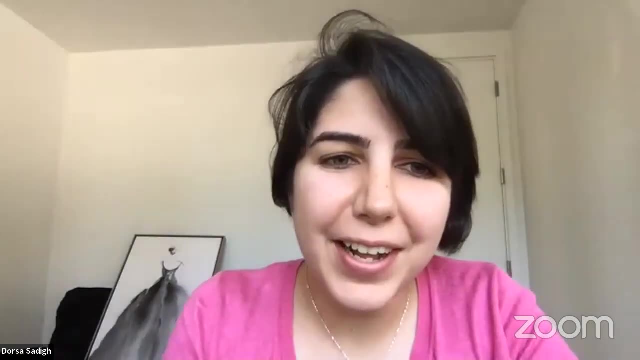 No, Hello, Oh, I am unmuted now. Okay, I couldn't unmute myself, sorry, All right, so perfect. Let me just share a screen then. Great, yeah, we can hear you. great, Thank you, perfect. Can you guys see my screen? kid. 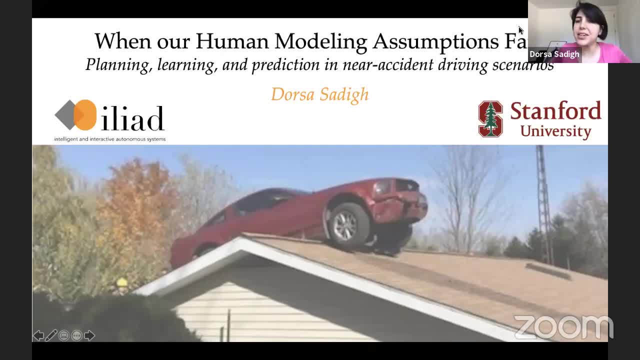 Yes, yeah, it looks great. Okay, so let me start. All right, Hi everyone, Thanks for inviting me. I'm really excited to be here. This sounds like a really fun workshop. So today, what I'd like to do is I'd like to: 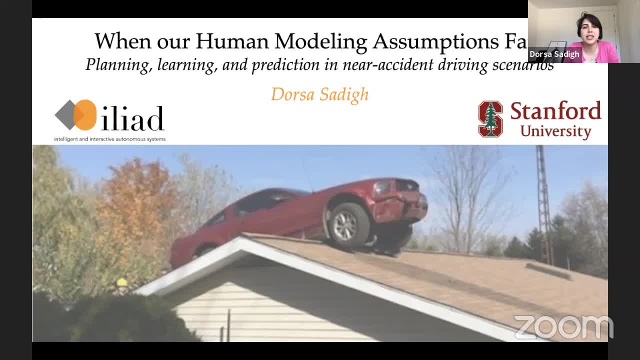 talk a little bit about planning, learning and prediction in near accident driving scenarios. So I really want to focus on these settings where some of our assumptions about human modeling or assumptions in the environment actually fails- specifically near the end of the risk spectrum or near accident settings- and how we should go about planning, learning and predictions. 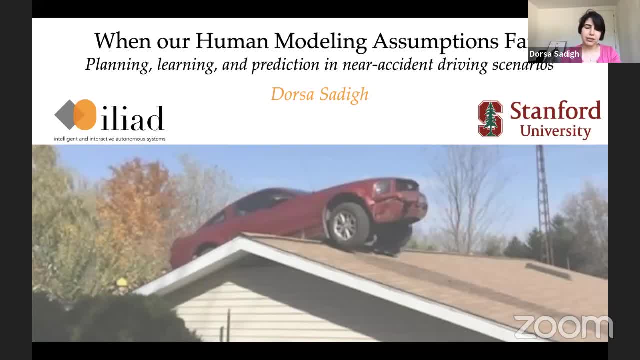 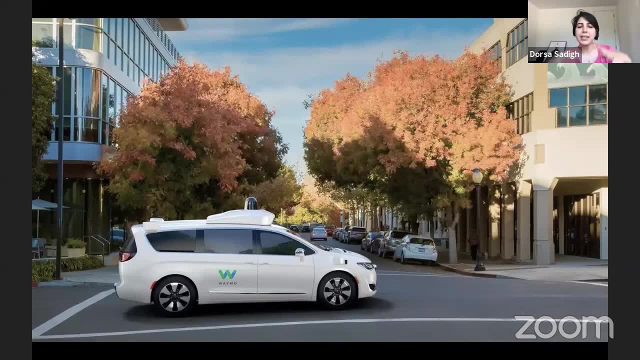 in those settings. So let me just jump into it. So I'm going to focus this talk mainly on autonomous driving And if you think about the field of autonomous driving over the past decade, we have seen a lot of advances in driving. Even a few years back, we didn't see any cars autonomous. 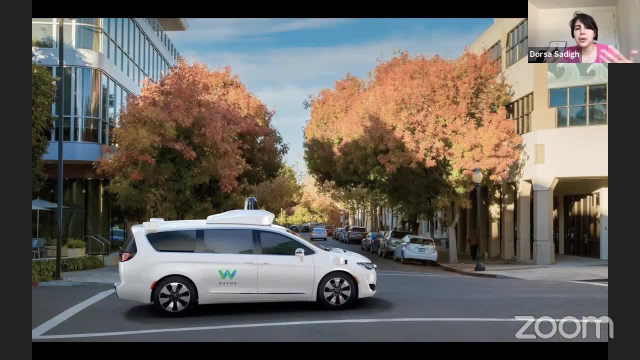 cars on normal city roads. right, They would mostly work on highway driving and things of those forms, So it's really exciting to see that these vehicles are finally out there interacting with real people, And this was actually something that I was pretty excited about during my 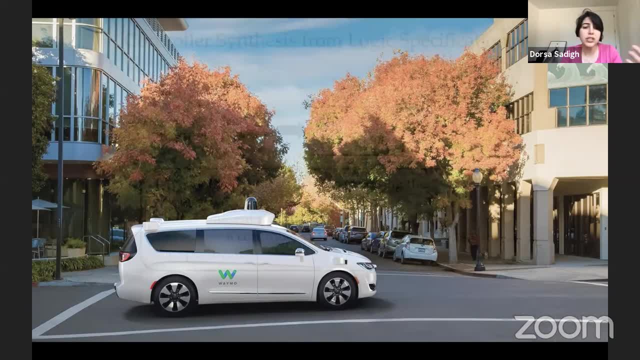 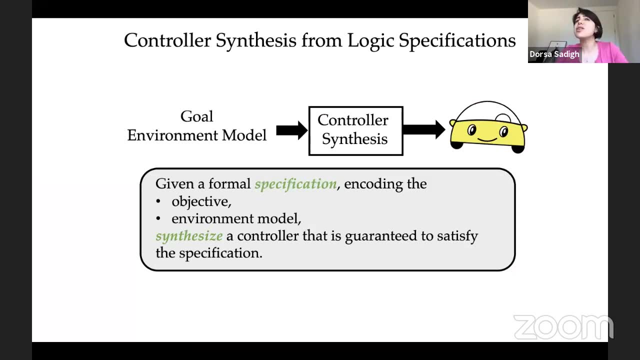 PhD too. So the way I started working in this domain was from a perspective of control and formal methods. So what I really cared about back in the day was autonomous driving was just becoming a thing at the time, And this was actually the time that people were saying: 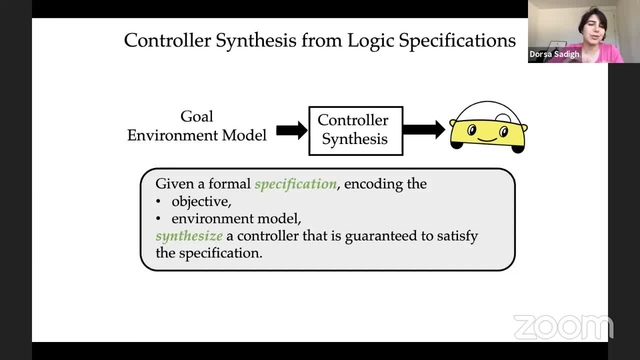 we're going to have autonomous cars by 2020, because 2020 was so far ahead that it was okay to say that. But at the time I was thinking: well, if you're going to have autonomous cars by 2020,. 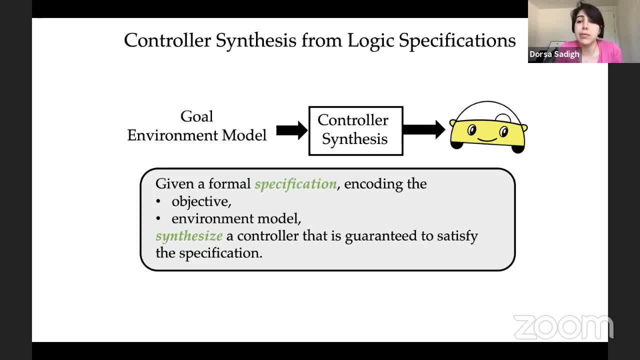 then there should be a way of giving guarantees about these autonomous cars, because we can't put them on the road if we don't have any guarantees, or if we can't, how are we going to insure them? How do insurance companies work if they don't have any sort of guarantees of how well 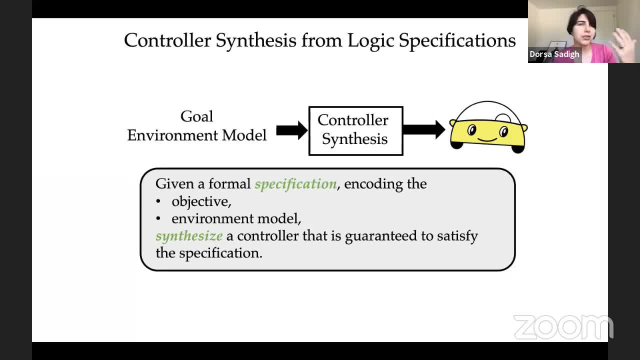 these autonomous cars work. So this is like old Dorsa thinking that. And the way I started formalizing this problem, I was thinking: well, I'm going to have a car that's going to be autonomous cars, and I'm going to have a car that's going to be autonomous, And I'm going to have a car that's. 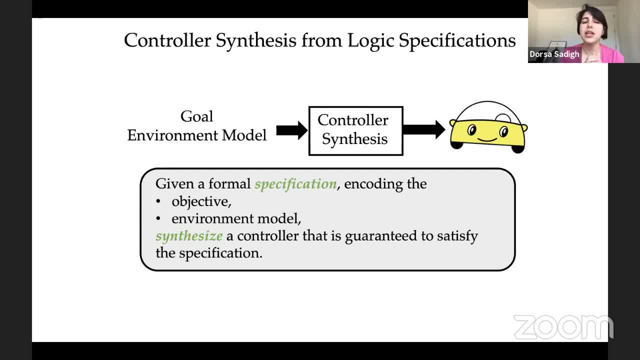 going to be autonomous. And then I started thinking about the idea of a control and reactive synthesis problem, thinking about starting with an objective, thinking about, like I need to write out a formal specification, writing out what the objective is and what the 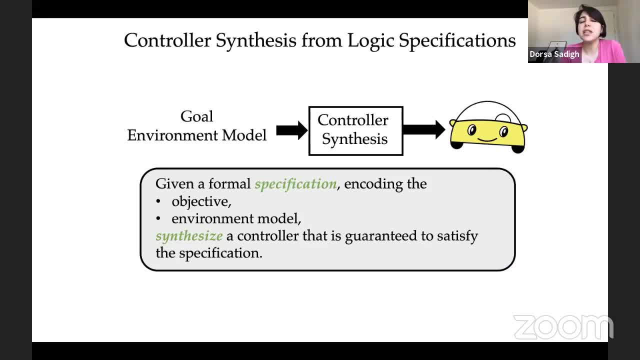 environment model is. And then, once I have that formal specification, then the question is: can I go ahead and directly synthesize a controller that is guaranteed to satisfy this specification? Can I come up with a provably correct controller for my autonomous car? 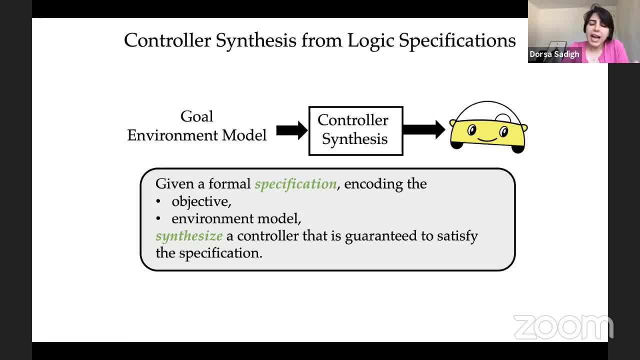 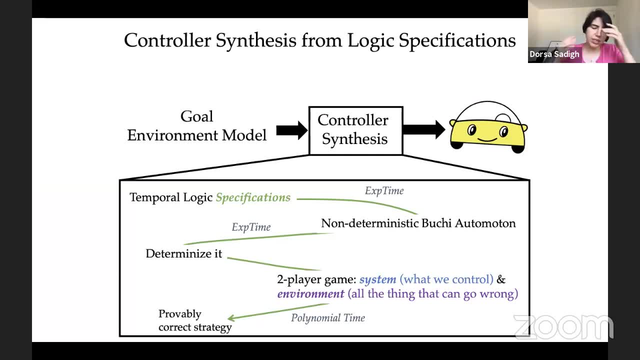 And I know that sounds really strong and rigid, but when you actually try to attempt this. and then we took different approaches towards it. So one common way of going about it- and we did some work in this domain- was starting with a temporal logic specification, then translating that to a Buki automaton and terminizing it. 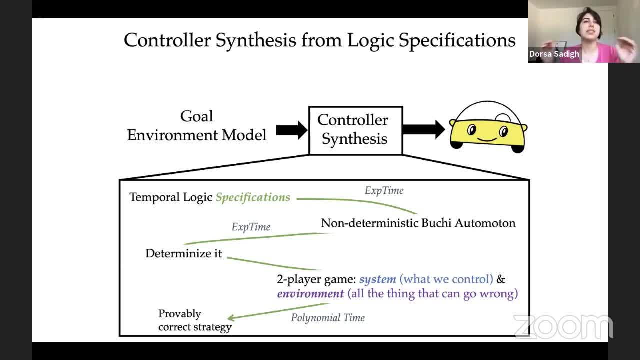 And at the end of the day you have a game. You have a game between your system, which is your autonomous car, and the environment and everything else that's going on in the environment, And you solve that game And at the end you have a strategy and you have a proof with it. 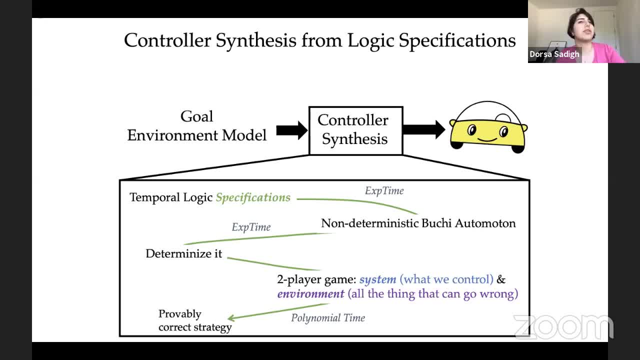 That's definitely correct And there's policy that is definitely correct for your autonomous car, So definitely sounds very rigid. Lots of assumptions that go in this box that I'm pushing under the rug in order to give any sort of guarantees, And one of those assumptions that 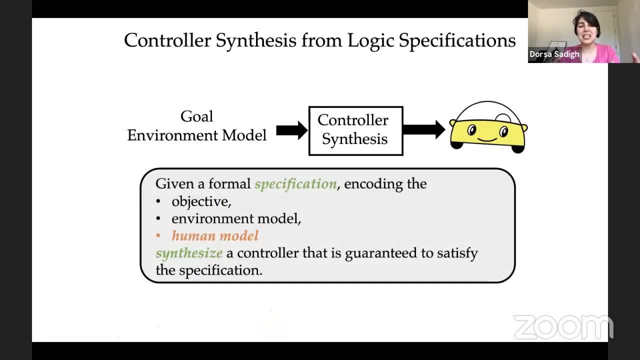 was bugging me so much was basically this idea of there is a human model out there. So the way we approached this was we said: well, we have an objective, We have an environment model. We've got to have some sort of model of how. 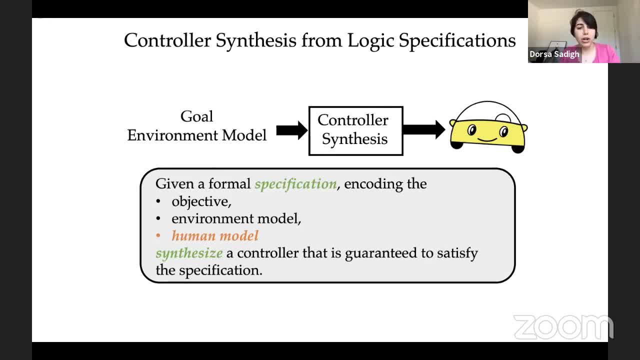 other cars around us drive, And with that model I can give a guarantee. So I explicitly remember this. We talked to some car companies And they were like: well, you can assume that if your car is driving 60 miles per hour, it's going to stay with 60 miles. 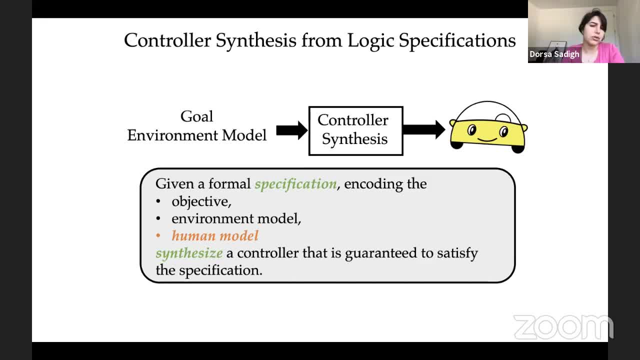 per hour. So keep that velocity. That is the model we're going to use for how cars around us are actually going to work. And once you put that model in, then you can give all sorts of guarantees. Then you can say: well, my car is safe because this other car is still going 60. 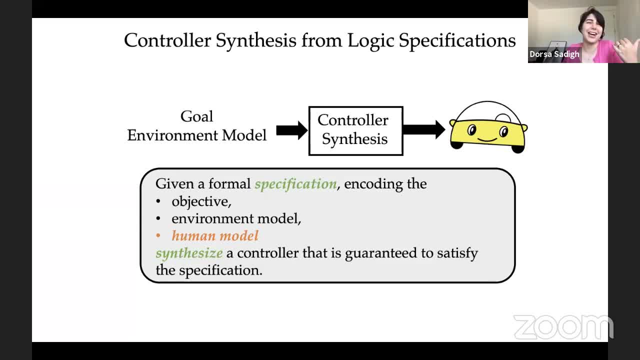 miles per hour And doesn't really pay attention to the fact that there's an autonomous car driving right next to it, which seemed a little bit silly to me. So I was like, well, if I want to be safer, maybe I should have a different type of human model. 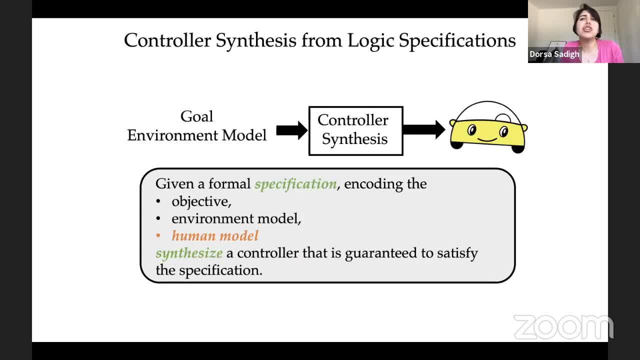 So one other way, one other extreme, is: assume that humans are adversarial and they're trying to get you. And if you assume human-driven cars around you are adversarial, then you don't really have any guarantees. Most of the time, this approach doesn't really come up with any strategy. 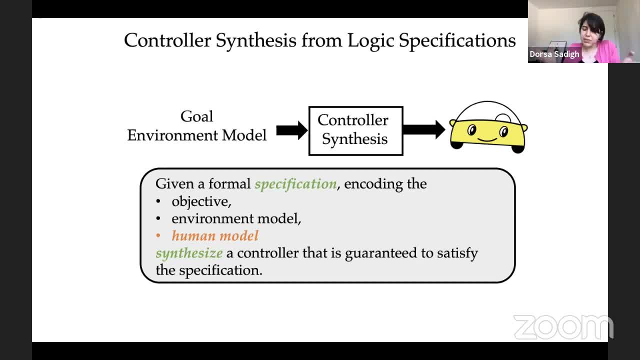 that is safe, because that wouldn't exist, And both of these seem like extremes to me And it kind of felt like human modeling and then thinking about how cars around us act around us and respond to us is the core of the problem here And we're kind of ignoring it And we're kind of 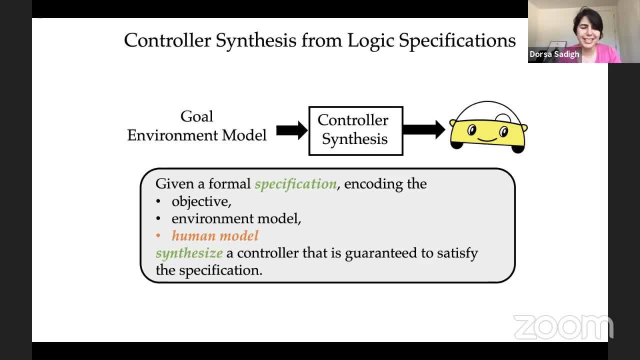 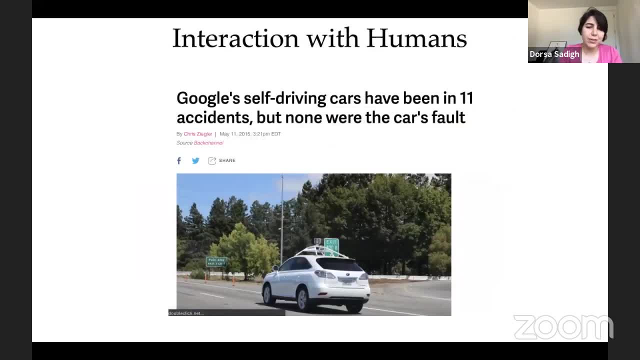 assuming someone comes and gives us that human model and everything will be great. I wasn't alone in this, actually. I think a lot of other people were thinking the same thing. This was around 2015, where Google started putting out their cars. This was around 2015, where Google started putting out. 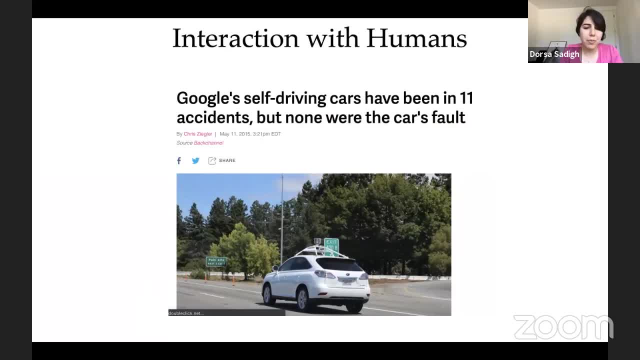 their cars. This was around 2015,, where Google started putting out their cars. This was around 2015,. out in the streets And in only a few months they had 11 accidents. And all of these accidents the Google car was being rear-ended. So of course it wasn't their problem, But if you think about it, 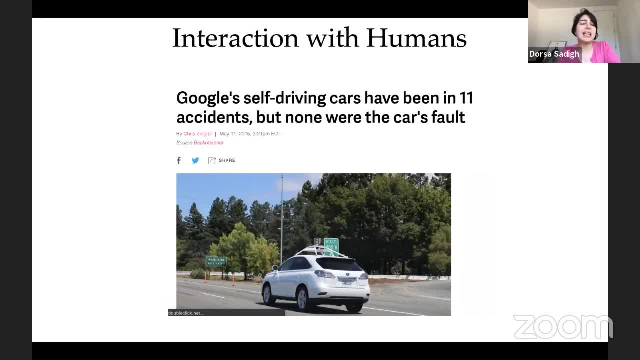 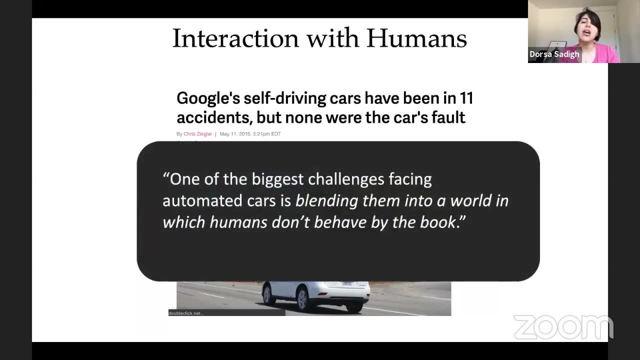 well, one reason that one can argue that these accidents happened was that you're putting this vehicle in a road where you think all the other cars around you are acting like robots and you're just driving like a robot would do, And humans don't really do that. Humans don't necessarily. 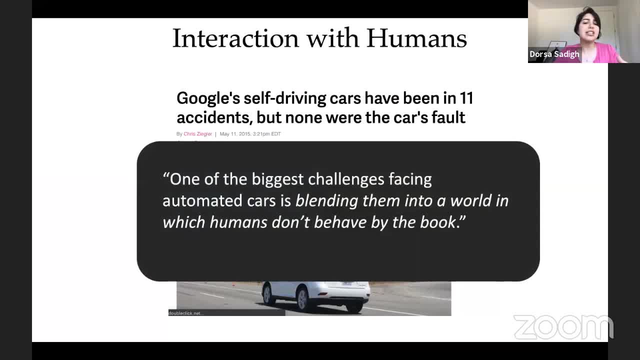 behave by the book or don't want to behave by the book. They don't necessarily behave by the book or don't follow all the rules, And they can easily coordinate and collaborate with each other. And then the Google car at the time was not really thinking about that. 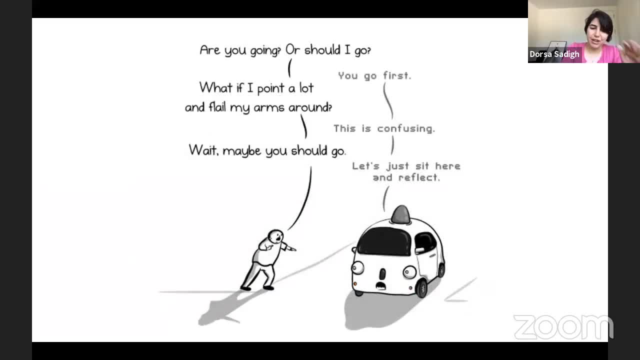 So this was actually a cartoon back in the day that I really liked And I felt like it explains the problem so well, And unfortunately this cartoon is still true. I was driving right by my apartment, like two blocks from my place, yesterday, And there was a rainbow car And I had 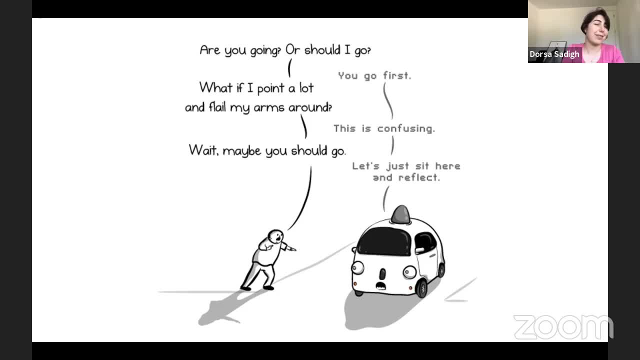 this exact interaction with it And at some point I was like I'm going to give up, You're not going to be going, I guess I'm crossing. So this is still a big problem Interacting with people. I think in some sense at the beginning of the field of autonomous driving, we undermined it. 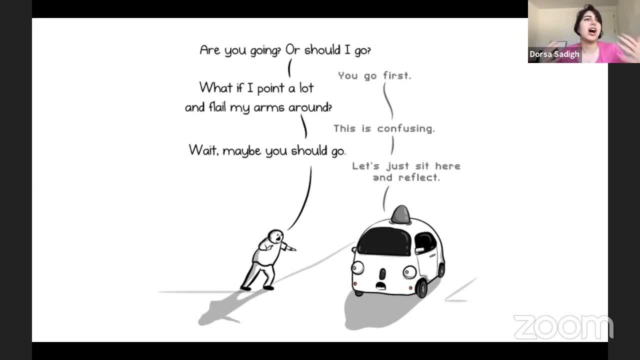 because we assumed that, well, I just want to build this awesome car that's really good at prediction and perception and is really good at detecting obstacles and things of that form, And we kind of ignored the fact that, hey, this car needs to interact with real people. 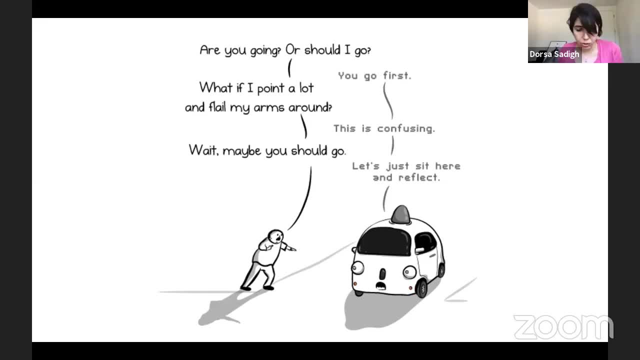 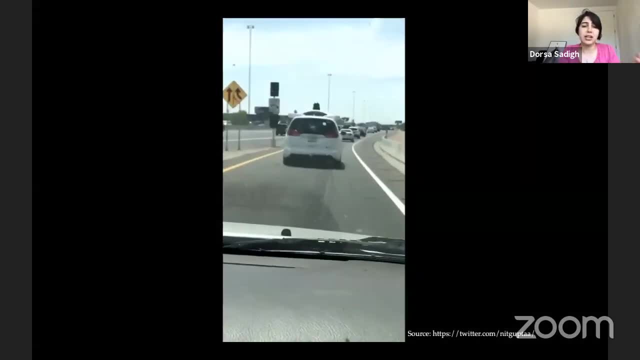 and you can't really eliminate humans, human drivers or pedestrians around you, And you actually need to interact with them. And if we were to change this and we, well, we've with them. this is actually a video of um, a rainbow car. that kind of deals with the same problem. 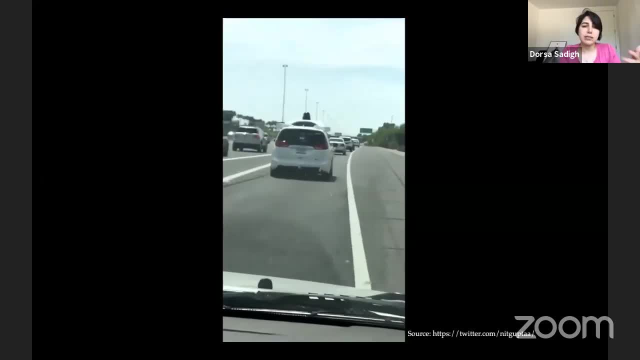 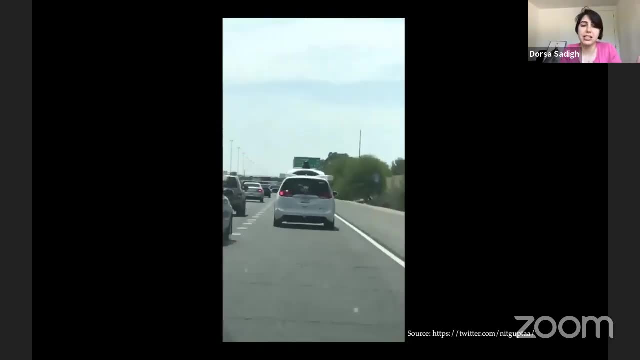 um, this video is a little bit old by now, but here this rainbow car is actually trying to be interactive. it is, it is signaling, so it is trying to be interactive. it wants to change lanes. it's in an exit lane, but in terms of its motions it's not doing any sort of interactive behavior. so how? 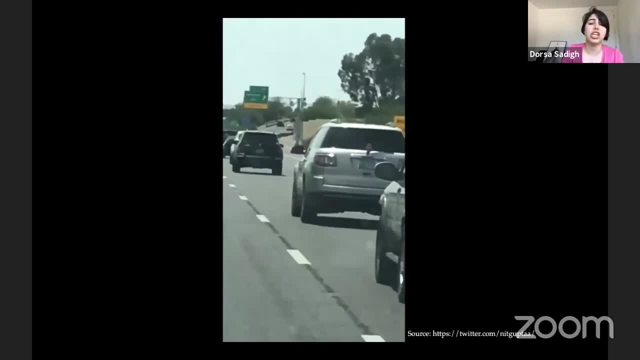 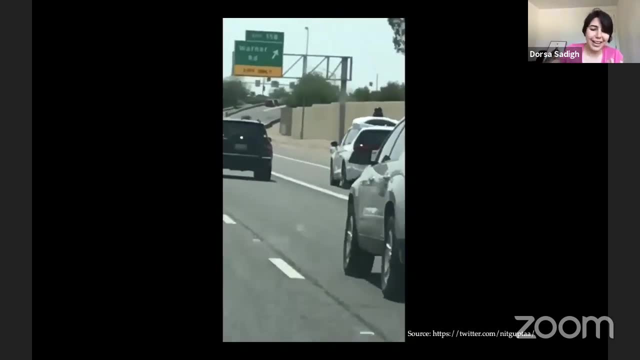 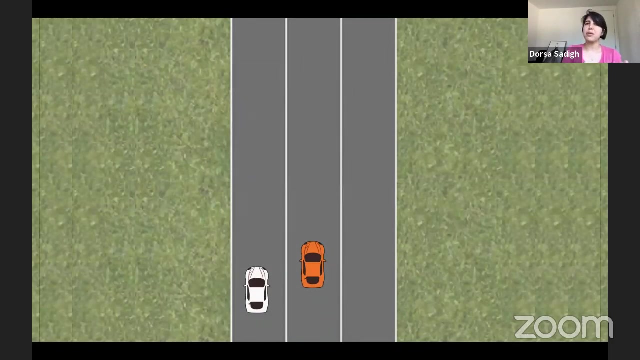 would these cars know that, like when this car actually wants to change lanes and because of that, like the rainbow car, needs to exit and come back around and then try again, which is not so great. so what we decided to do is we decided to actually model these human-driven cars around us. 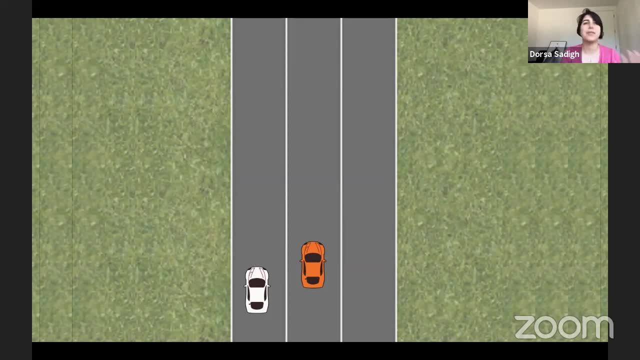 a little bit more carefully and i think that perspective is a good perspective. so so we thought about having, let's say, an autonomous car- the orange car- on the road- and a human-driven car, where there there's a human inside it and this human also has some sort of objective, some sort 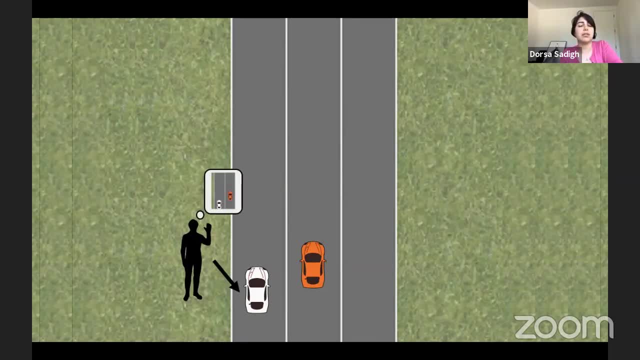 of goals, and then we shouldn't treat this human-driven car just simply as a moving obstacle and we should actually worry about like this interaction and how we go about this interaction. so so we modeled this interaction in a game, theoretic fashion. what we did was this: 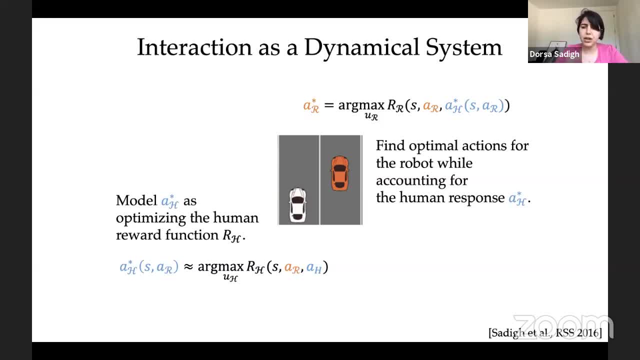 is work at rss in 2016. it was a joint work with anka, shankar and sanjay. actually, anka might be talking about this a little bit later today because i saw her title. the title of her talk it's about game theoretic- uh, autonomous driving- and actually this was like one of the first works. 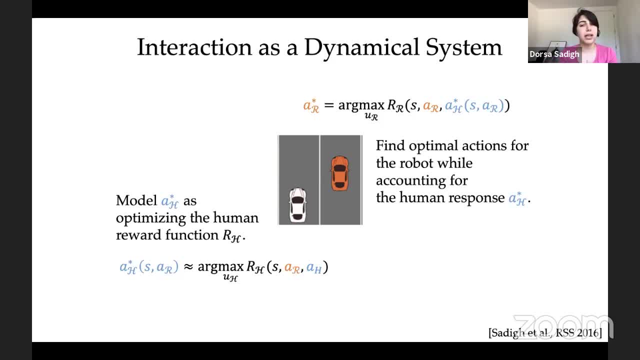 that was trying to approach the problem from this game theoretic perspective, where we modeled the interaction as an underactuated dynamical system, where we say: well, i have an autonomous car, that's the orange car and the way i'm going to go about planning for the autonomous. 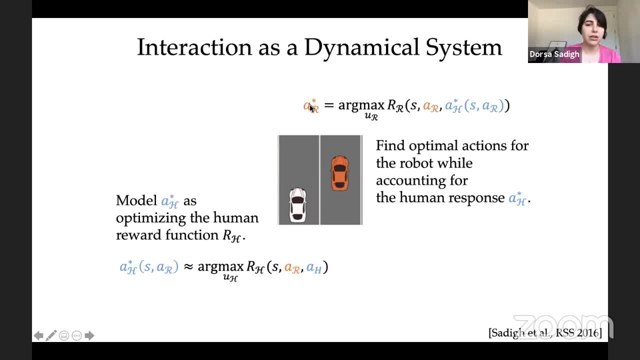 car is. i'm going to come up with a policy ar star which is the maximizer of some sort of objective for the autonomous car. very good question to ask is: what is that objective? how do you come up with that objective? we thought it is simple. it's actually not simple to think about what that 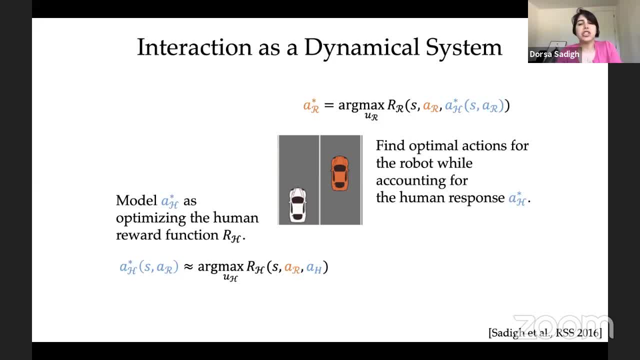 objective should be normally a function of state and actions, but it should also depend on the actions of the human, because the robot, the autonomous car, can actually influence people. and a very good question to ask again is: what does the human do, or how does the human act and respond? in this setting, where you 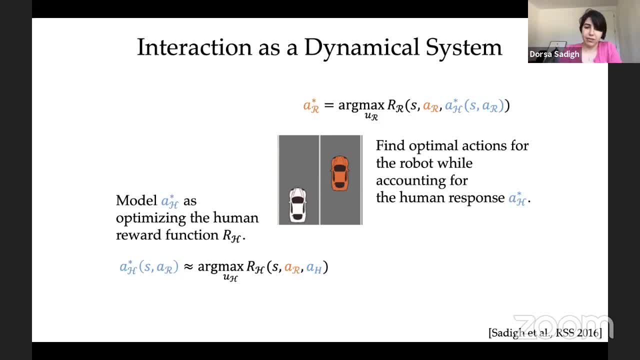 have this interactive setting like like, how would it, how would it drive in such settings? and the way we approach this was, we assumed, humans are approximately optimizing their own reward function, rh, and we learned that reward function function through inverse reinforcement learning, and there's a lot of work in imitation learning. 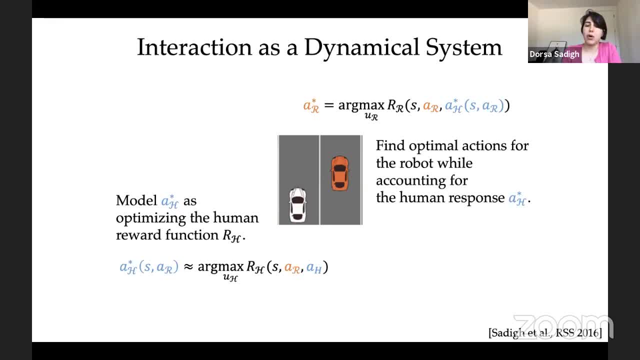 and generally trying to figure out what that reward function or what that policy looks like. so a big assumption here. i'll come back to this assumption later in the talk. but in general, once you have this, this human policy, and once you have this robot policy, then you can think about this. 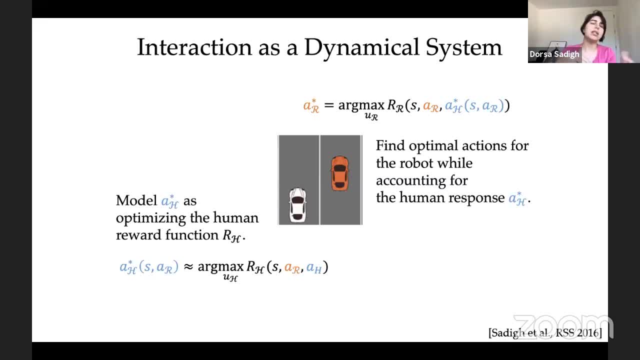 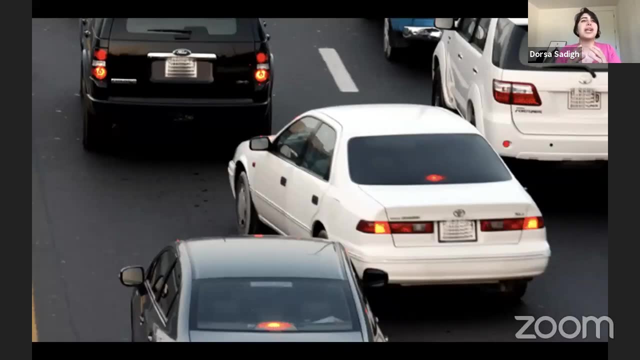 interactive game theoretic approach of the robot influencing the human and the human responding back, and we made a lot of approximations to make that work, including solving this problem as a stack of right game, and eventually we got really interactive behaviors. so the exciting part was we ended up getting an autonomous car being able to nudge in in front of other cars. 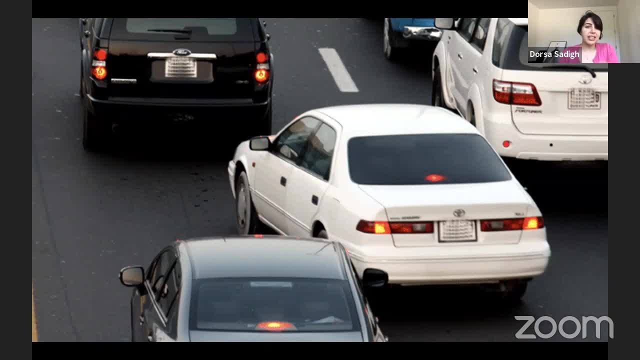 and actually make them slow down to change lanes, and this is a very interactive behavior. this is how humans change lanes, so like when you're changing lanes, you're not going to wait for every single car to pass and then wait for them. at some point you cut in front of people like kind of. 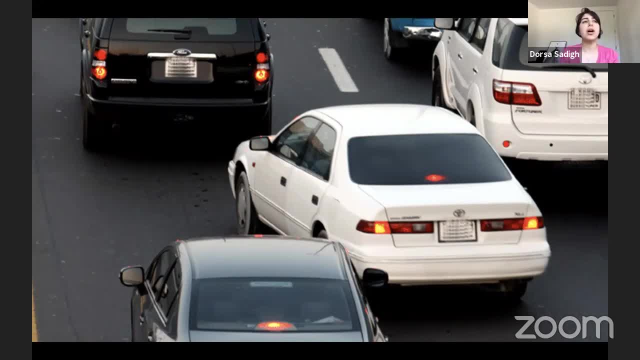 like what this white car is doing here, and based on this game theoretic modeling, we ended up getting very interactive behavior, which is really exciting, like we end up getting very interactive behavior emerging out of the optimization. so that is great, but i would lie to you if i say this: interactive. 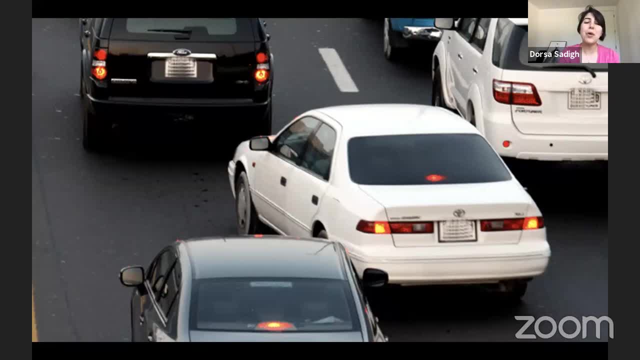 behavior is the safest thing you can do in the world. right the moment you start taking this assertive action, nudging in front of other, this other person, you're putting yourself in danger. you're- you're actually like reducing your safety because you're becoming closer and closer to these. 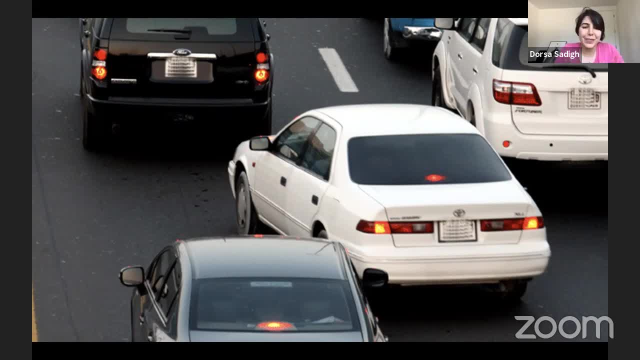 other cars around you, and that's a big trade-off that exists here between safety and everything else, efficiency and comfort and everything else- and- and- and i think that trade-off matters a lot when we are in near accident scenarios and also when you're not in your accident scenarios, because we have to take 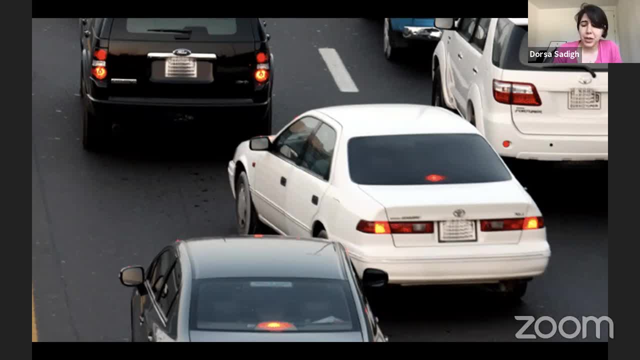 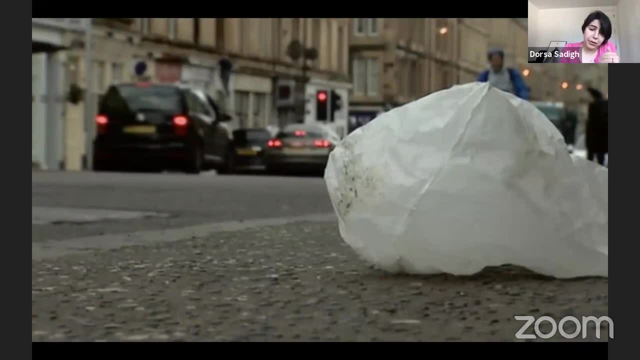 those trade-offs. uh, if you want to be more efficient, if you want to be more comfortable, if you want to drive like you want to actually use these autonomous cars, so let me, let me just give one more example and then i'll jump into what i'd like to really talk. 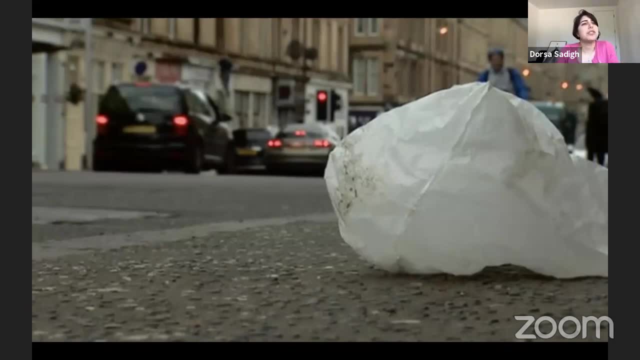 about um. so the one thing that i wanted to talk about is the problem that this like type of type of trade-off shows up in is is not necessarily when you're interacting with people, but even when you're interacting with objects and your environment. so so this is a plastic bag problem. um, this is a. 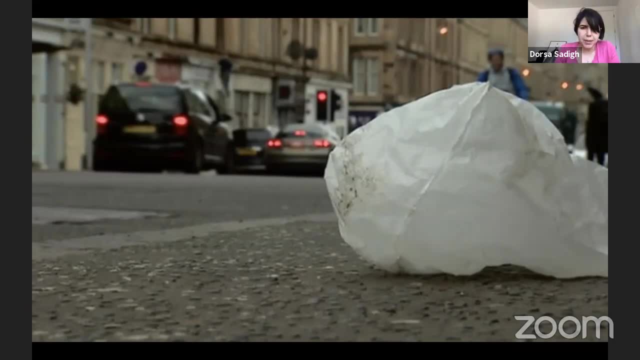 problem that actually, one of my friends who was uh leading one of the driving autonomous driving groups uh mentioned this to me a couple years back and basically he was saying: well, this is a problem that i deal with every day. i can't even get this car like driving in a way that i'm, i'm, i'm. 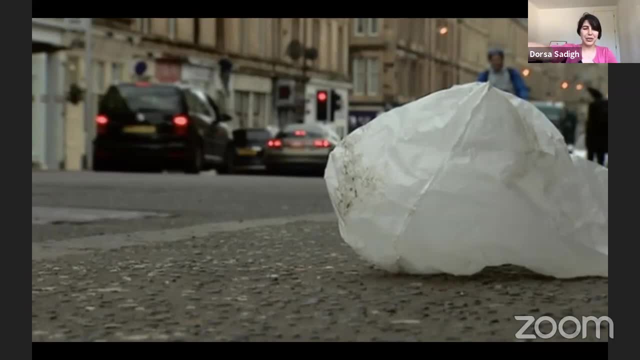 going to be happy about it. imagine that you have a plastic bag on a road. if you have a plastic bag on a road, what are you going to do with it? so, so, so. one thing that you can do is you can say: well, that is an obstacle. i want to be the safest car in the planet. and if i want to be the safest, 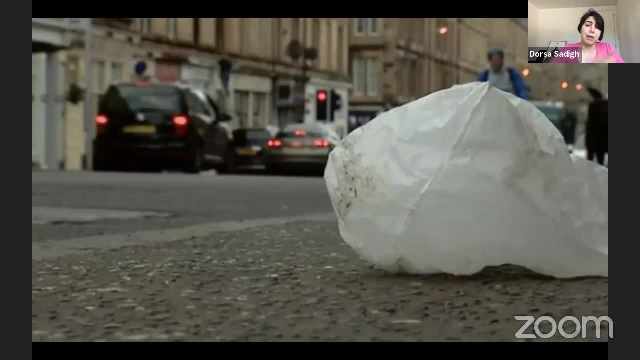 car on the planet. there is a chance that that plastic bag is maybe a person holding a plastic bag that and is covered by that plastic bag, and because of that, i am going to just slow down every single time i see a plastic bag. and well, if you do that, the person who is sitting in the 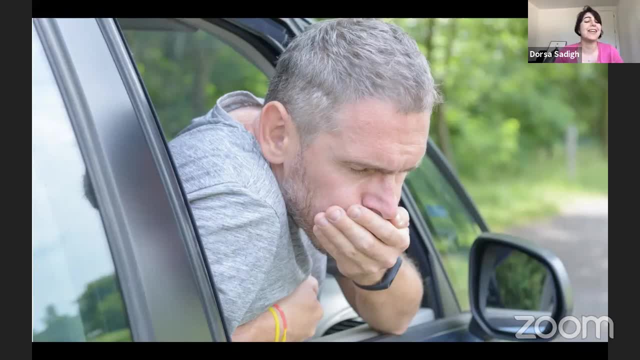 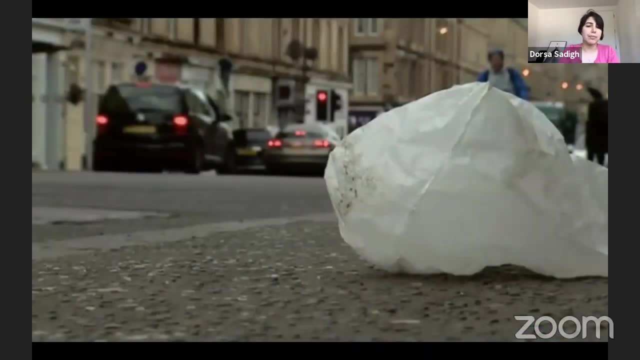 car is actually going to feel nauseous, right like. this is not going to be very comfortable and this is not going to work out. the other option is to say, well, that's probably a plastic bag. i'm going to ignore that plastic bag because it is a plastic bag, right, and the moment you do that. 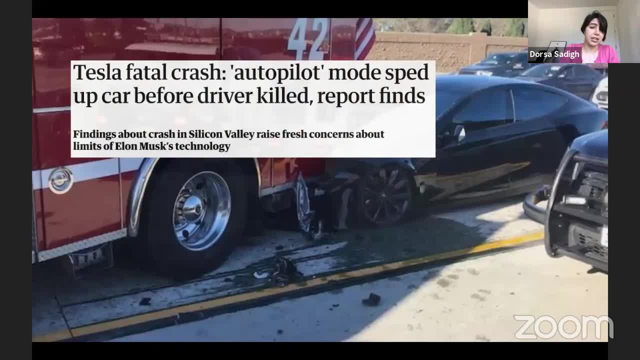 there could be scenarios. there could be near the end of the risk spectrum, scenarios where your car didn't detect it correctly. maybe it wasn't a plastic bag, it was a person holding a plastic bag and and because of that you might end up in fatal crashes, as we've already seen a couple of them. 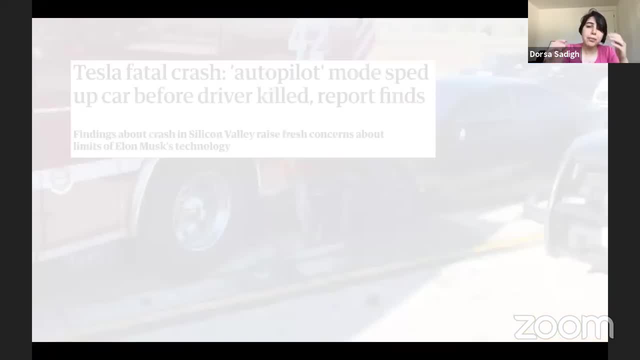 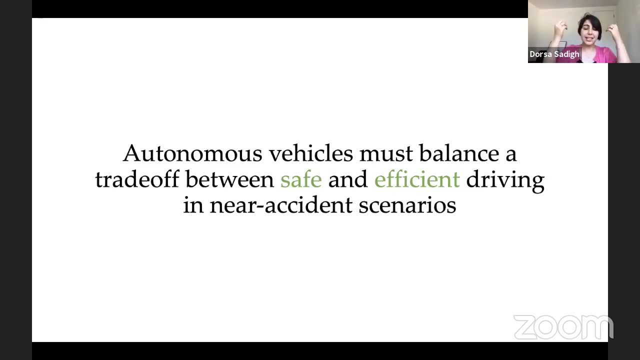 over the years. so so that is the problem. the problem is, we got to have autonomous cars that are able to balance this trade-off between safety and efficiency. and specifically, again, that becomes really important when we are in near accident scenarios and- and it's crucial to handle well when you're in your 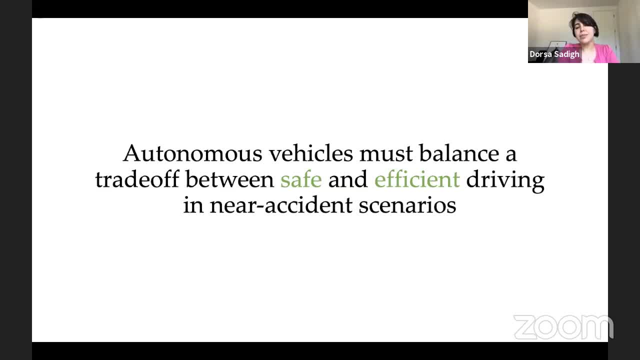 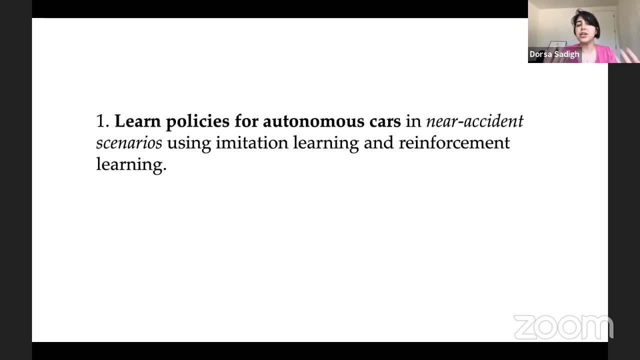 accident scenarios. so i'm not claiming we've solved like all the problems here. what i'd like to do is i'd like to talk about two starting works. that tries to specifically address near accident scenarios. so my plan for this talk is to start off by talking about some of our work where we are trying to learn policies for 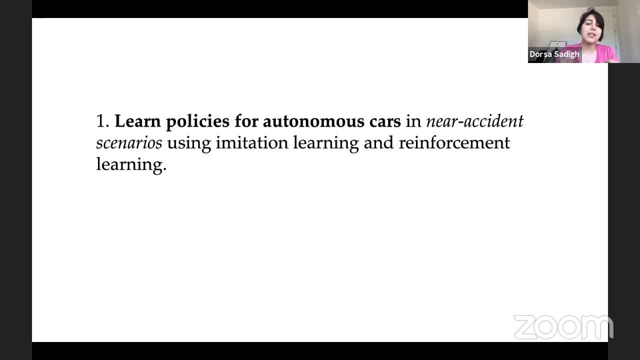 autonomous cars in near accident scenarios, specifically using a data-driven approach, using imitation learning and reinforcement learning together to figure out how this autonomous car should drive when we are near accident settings, and then after that, for the second part of the talk. what i'd like to do is i'd like to focus on not necessarily what the 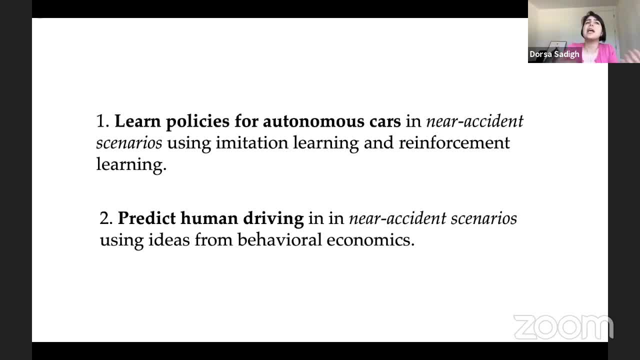 autonomous car should do, but the autonomous car predicting how the other drivers around it are acting when we are in near accident scenarios. and then for that i'd like to take a more model-based type of approach and use ideas from behavioral economics to think about risk a little bit more. 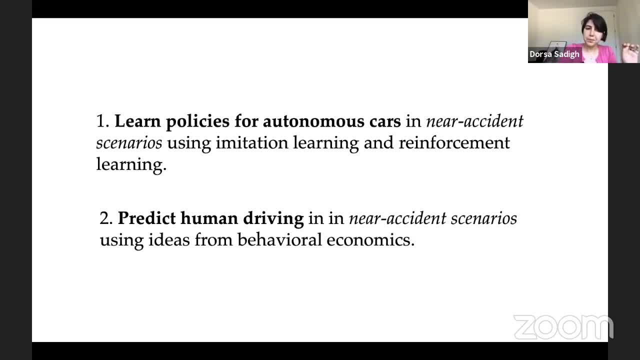 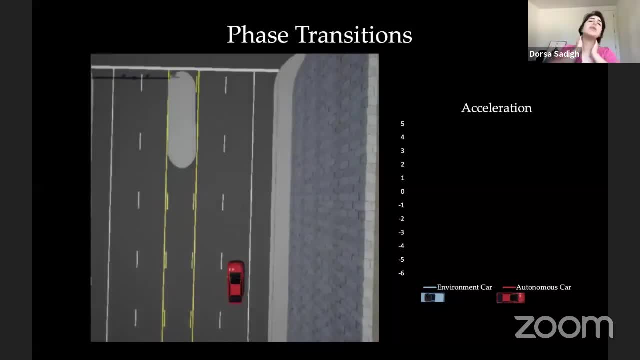 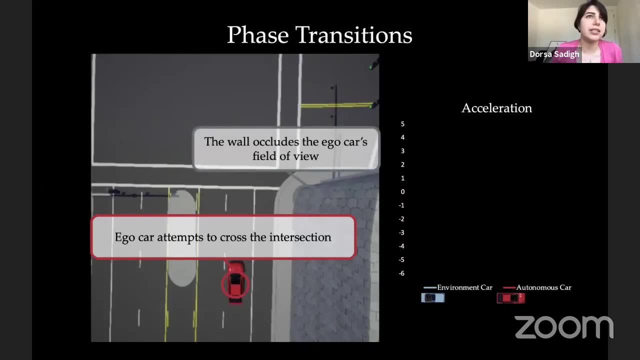 carefully. all right, so that's my plan. let's jump into it, okay. so let me think about near accident scenarios. one question to ask is: well, how are we defining them? what is special about near accident scenarios, and, i think, what one thing that particularly happens in in many near accident. 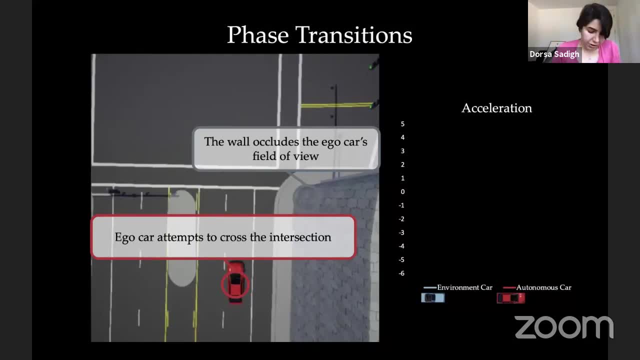 scenarios is the idea of phase transition. so so the idea of phase transition here is: i have an autonomous car- that's my red car- coming down this road and it looks at the environment and the environment actually smoothly changes, uh, over time and and there is there's no big jumps or weird. 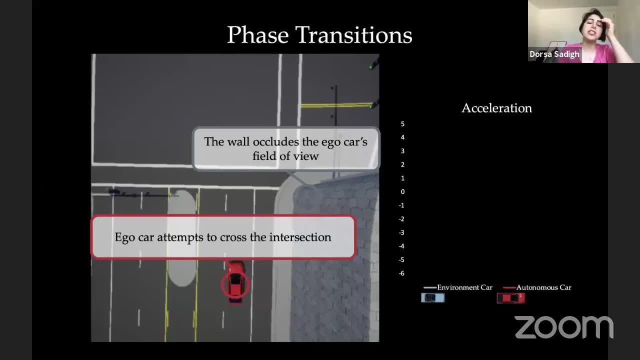 behaviors in the environment. the environment actually like much, much smoothly changes, but the autonomous car needs to have a jump in its actions. for example, if the autonomous car, the red car, is coming down the road and the environment is occluded, it gets to an intersection. let's say that this doesn't have any lights, so it's a two-way. 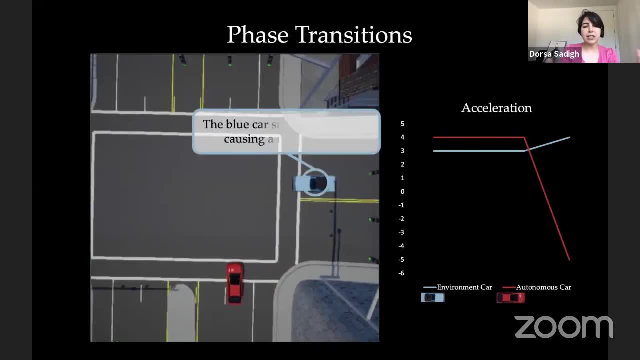 intersection and and it might actually at some point after the occlusion, it sees the, the blue car, the environment car, and once it sees that then the autonomous car to be safe, it should slow down. so it should like break really hard. so this breaking this, this really hard breaking, is almost a phase. 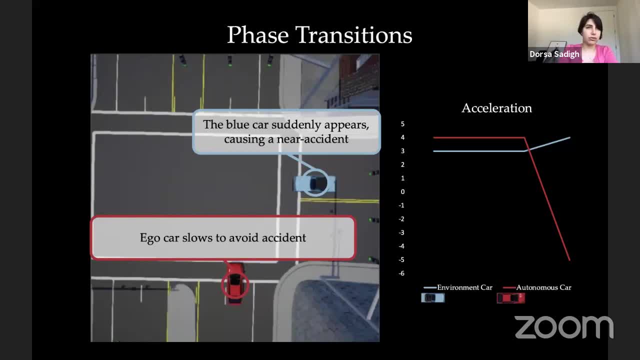 transition in the policy of of the autonomous car. it was driving normally and it's got a break- and then go down to a different, a very different policy based on smooth changes in the environment. so so that is really the difficult thing that we need to handle and we need to handle well in near accident scenarios. so if you think about these, 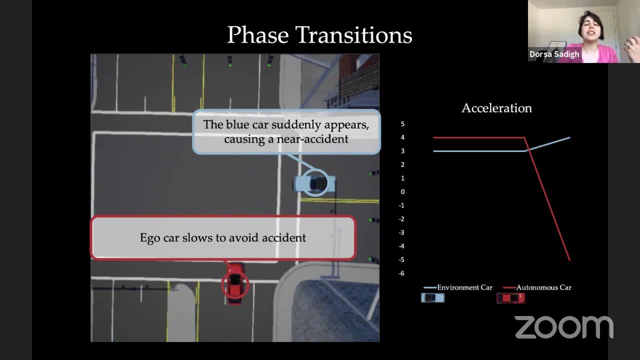 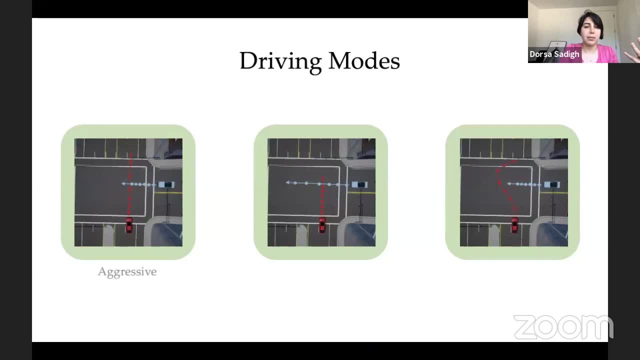 phase transitions. these phase transitions actually naturally create a set of a set of modes in the environment, a set of different modes of driving in the environment, and, as much as i hate to discretizing the world, this actually makes sense in this setting. so so, in this setting um this, 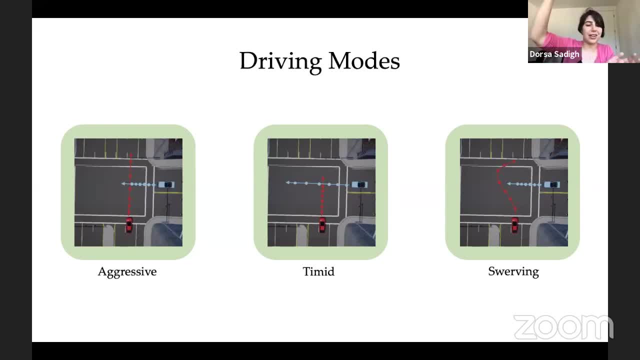 vehicle could continue to driving as it was driving and stay in this aggressive mode, could actually have like this braking mode behavior, kind of slowing down, or could maybe swerve and go around this vehicle. so there are different policies and almost different homotopy classes that exist here. 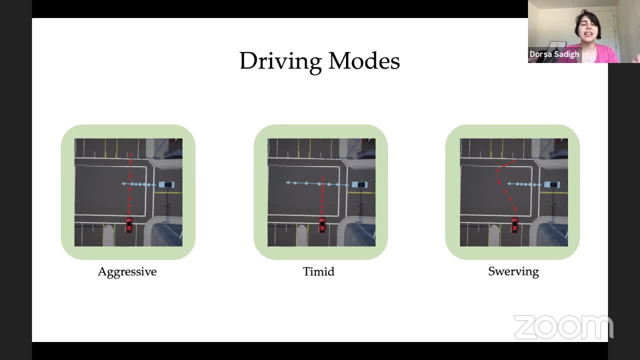 and this autonomous car could take any of these different policies, and those different policies create a natural set of modes here in invent when it comes to thinking about describing behavior. so what we think is: when you're in your accident scenarios, we need to handle phase transitions and 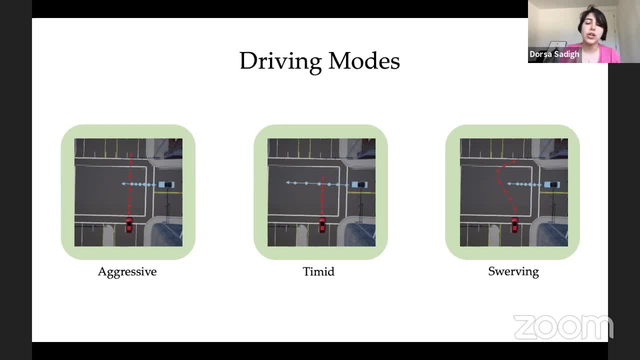 what that means is we need to handle how you're switching from one mode to another mode and and that problem is much easier than and then dealing with, let's say, let's say, trying to imitate, like how humans generally drive in these settings. so the way we approach that is as we think about this. 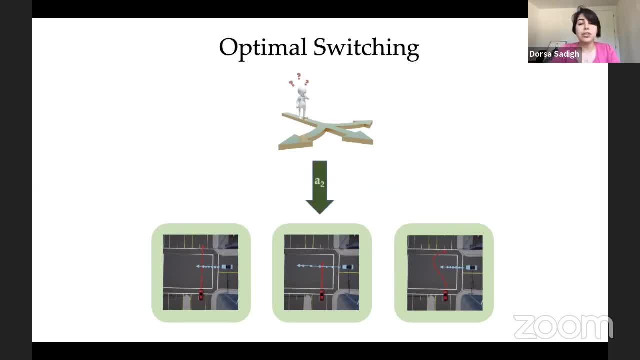 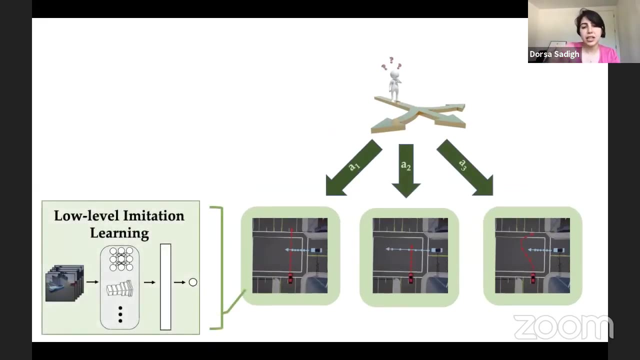 problem of phase transition as optimal switching between these discrete modes that exist in how people actually handle these types of settings. so, at the end of the day, what we, what we try to do, is we take a hierarchical approach here where we say each one of these modes are a specific type. 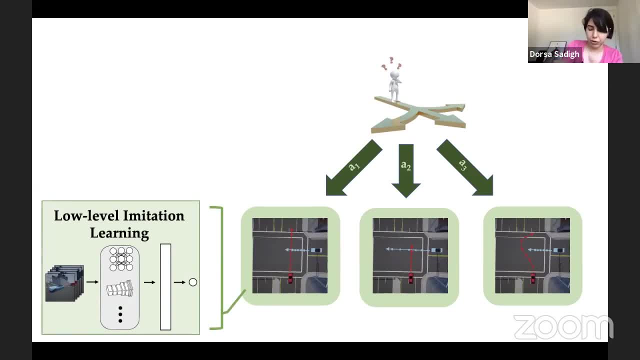 of driving behavior and i have very limited data in general for my new accident driving behavior. so i have limited data for each one of these modes but because i'm learning a specific behavior in each one of these modes, like training, a policy for each of these settings is actually not that. 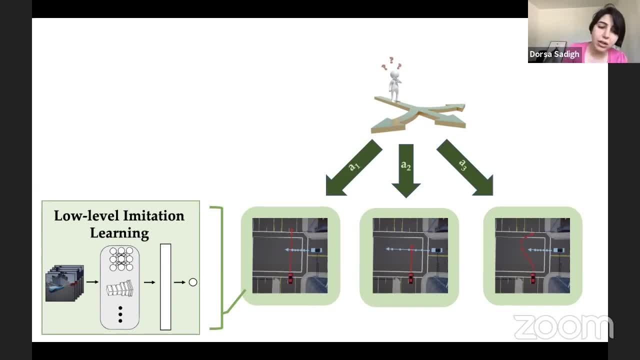 difficult i can. i can run a low-level imitation learning policy for each one of these mode behaviors, for aggressive driving, or sure we're slowing down? and then, specifically, we do that using conditional imitation learning, where we collect visual data of how cars drive in each one of these settings and then we have a policy. 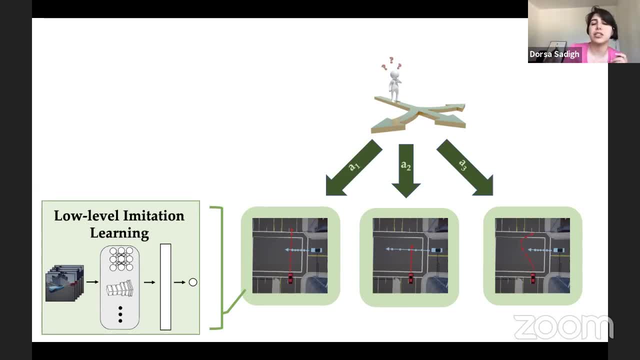 a low-level policy for how the car should behave in each setting, and then, at the top level, we have a reinforcement learning agent, and all the reinforcement learning agent needs to do is to figure out how it needs to switch between these low-level imitation learning policies. so the high-level reinforcement learning 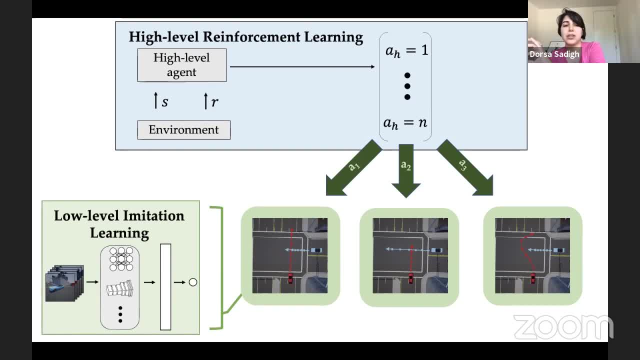 policy decides on these low-level imitation learning policies and this kind of hierarchical approach tries to handle this problem of phase transition in an efficient and scalable way. because if you were to apply just reinforcement learning to the full problem, it wouldn't scale. if you were to apply just imitation learning to the full problem, that wouldn't scale. 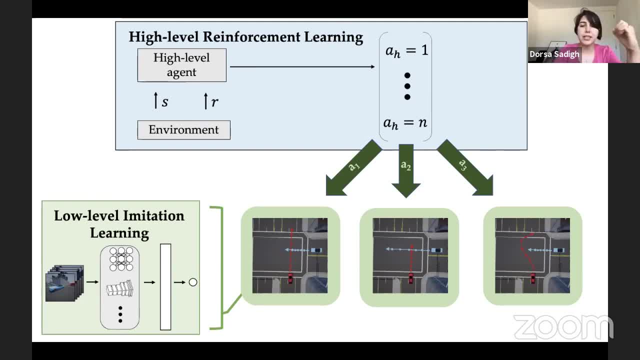 and have its own, all its own issues. so so so this kind of like breaks down the problem in a natural way to to handle how, how the autonomous car should actually drive when it comes to these types of phase transitions. okay, so so the proposed approach combines reinforcement learning and imitation learning. 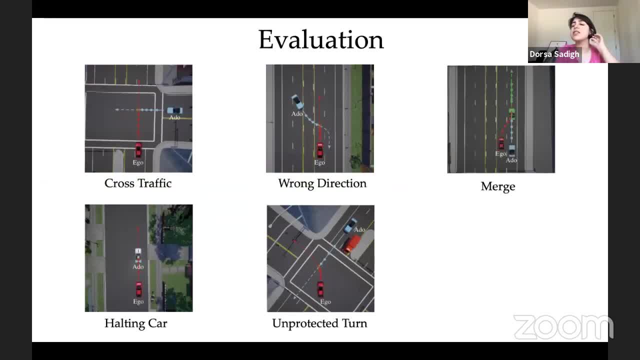 together and, if you're interested in details of this, this is actually an RSS paper and then we're going to talk about it on Tuesday. so I want to just briefly show one example of how this works in practice, but for more details, definitely like attend a discussion session, so we tried this out. 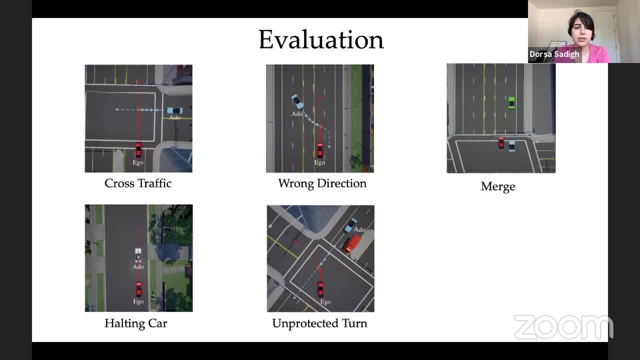 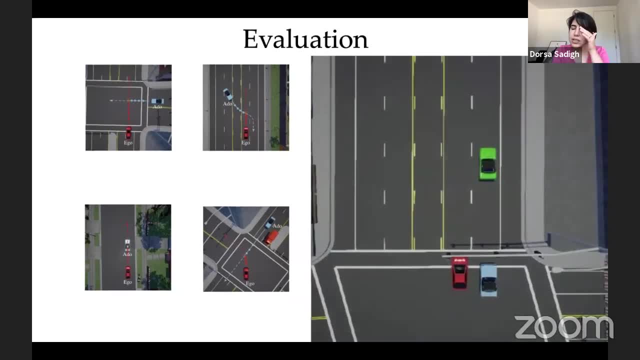 and in a few different near accident scenarios in Carla, and I just want to show you, maybe the merge scenario, just one of these scenarios. so so, this is the scenario where we have a, this is a setting where I have an eco vehicle, the autonomous car, the red car. and what? the red car? 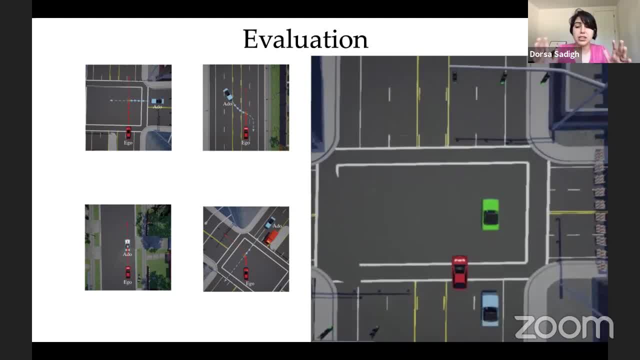 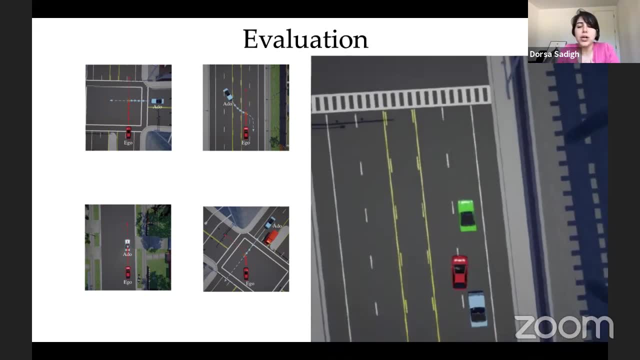 wants to do is it wants to change lanes, go to the right lane because there's an exit coming up and it really needs to change lanes really soon and and it can either emerge behind the blue car or it can try to like, merge in front of the blue car and, depending on the setting, 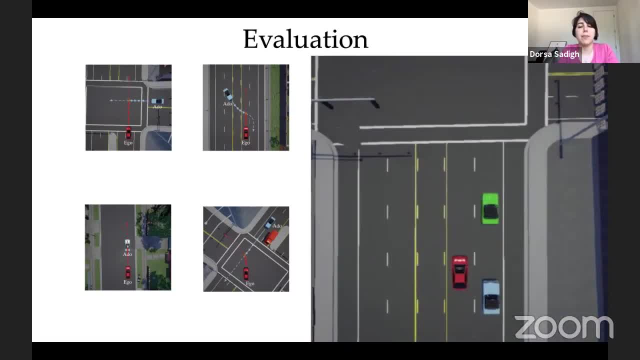 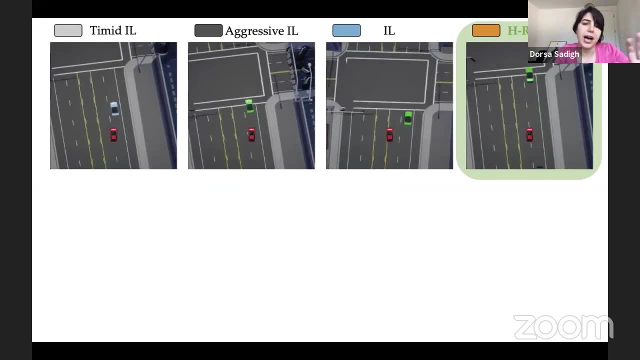 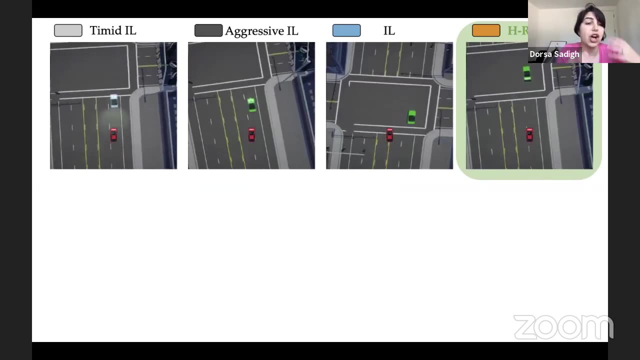 uh, it needs to kind of balance out what would be the thing that makes sense to do in this setting. so, um, I'm just going to show you some videos of how this compares with some of the other approaches. so if from the left, if, if you look at an imitation learning agent that is trained on just the timid data, the car is going, 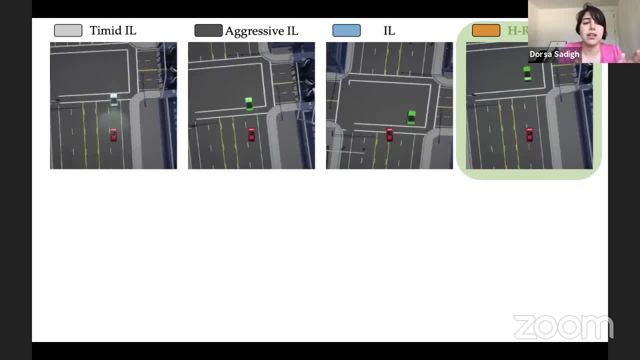 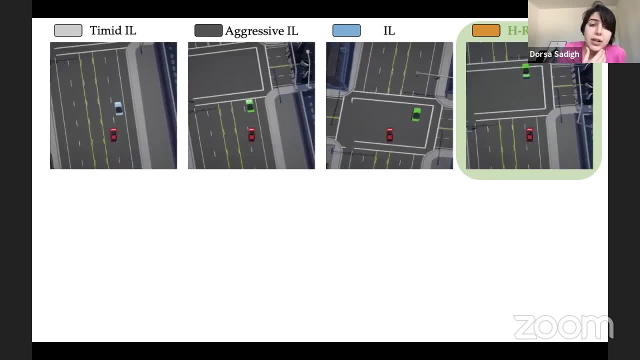 to merge behind the blue car all the time. uh, so that's kind of like what the timid behavior would do and that's what that data looks like. if you train an imitation learning agent on aggressive driving behavior, the car is always going to cut ahead, and this is getting close to an intersection. 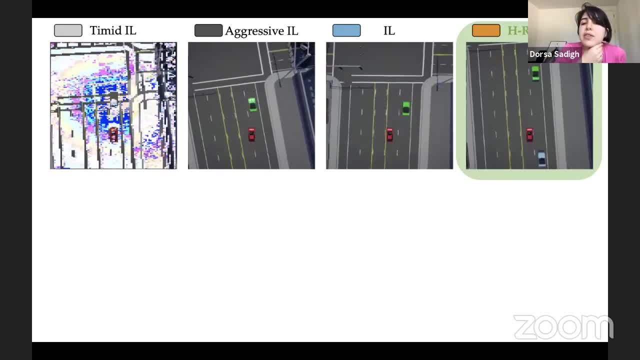 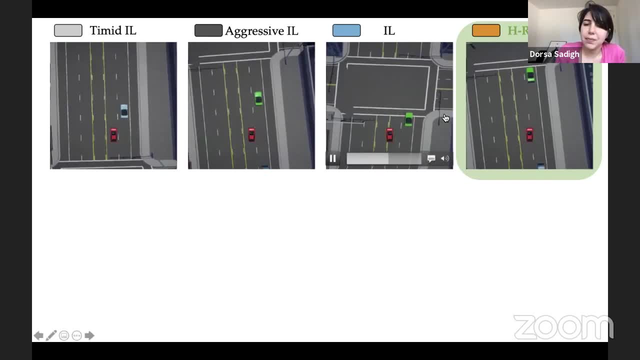 too. so you might say, well, uh, that could be an aggressive behavior if you're training it on the right lane, or if you're training it on the left lane, or if you're training it on the right lane, and then you're going to get like um, weird, like uh, shift type, uh behaviors where the car merges. 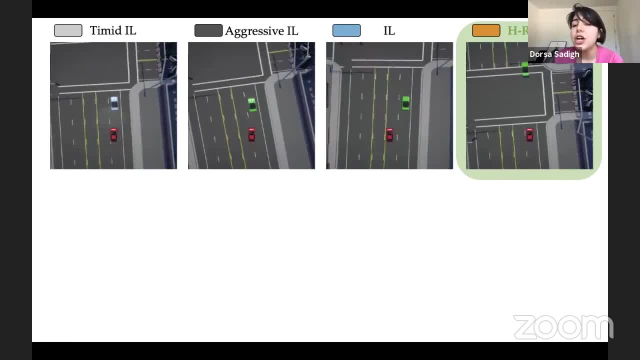 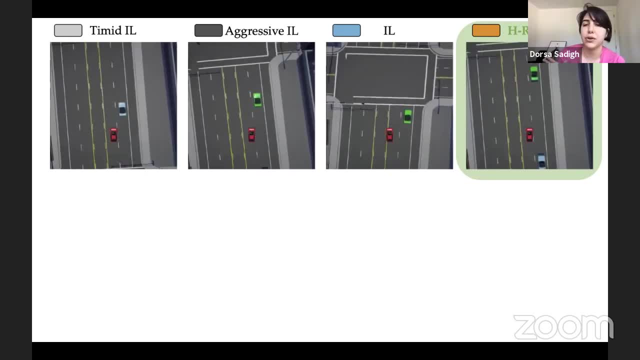 to to um, a different, completely different lane and finally, taking this hierarchical approach, uh, we would end up getting a behavior where the car does sometimes cut in front of the blue car, depending on what scenario you are in. so this is just a sample video of different runs of um of 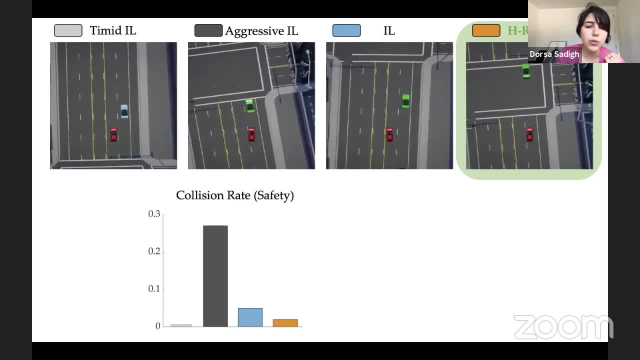 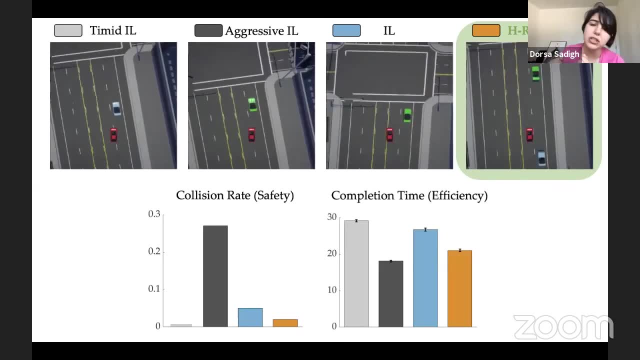 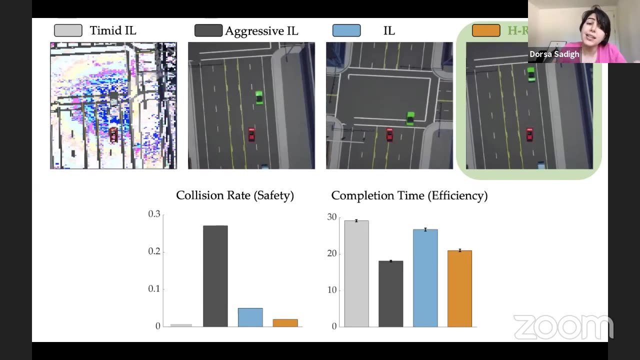 this problem. but looking at it more quantitatively, over multiple runs, um compare, compare safety and efficiency between this h rail approaches, hierarchical approach, combining reinforcement learning and imitation learning with some of these other baselines, and it turns out that in terms of safety, this approach actually does fairly well. of course it is not. 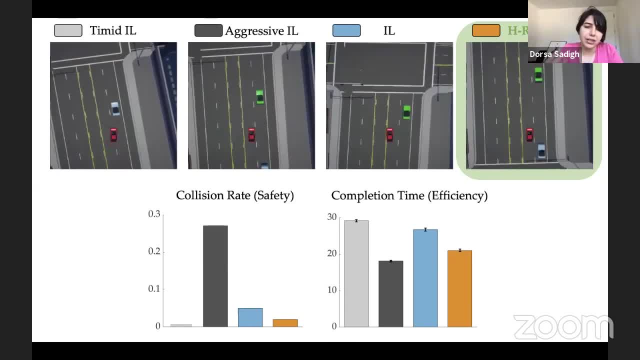 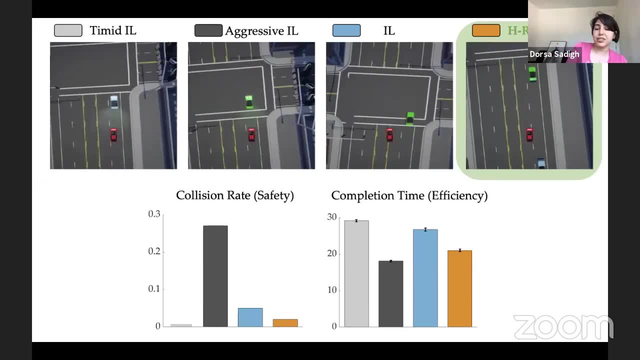 going to be as good as the tenet approach, but it is like fairly well, like in terms of balancing safety and efficiency, and again, in terms of efficiency it is, it is pretty efficient. of course, it's not going to be as efficient as the aggressive approach, which is just this line here, um, but 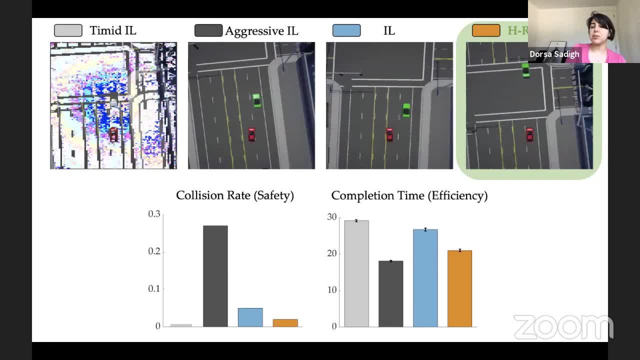 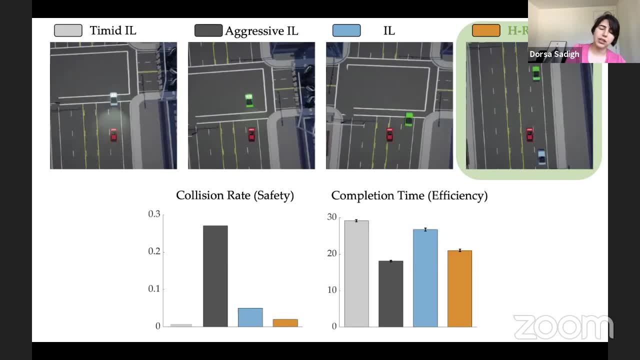 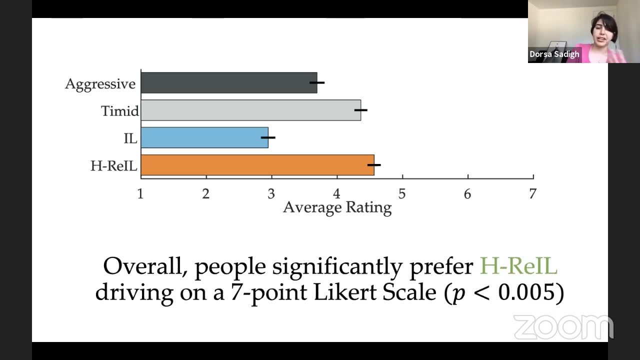 like the point is, by combining imitation learning and reinforcement learning here, we can better balance between safety and efficiency in a way that handles these phase transitions more gracefully. We also ran a user study where we showed these different driving behaviors to our users and then we asked them which one they would actually prefer, and they all strongly preferred. 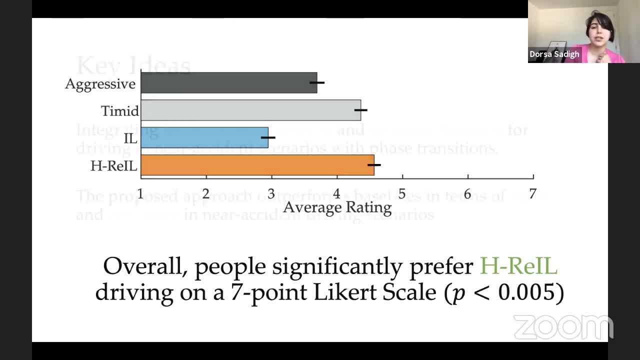 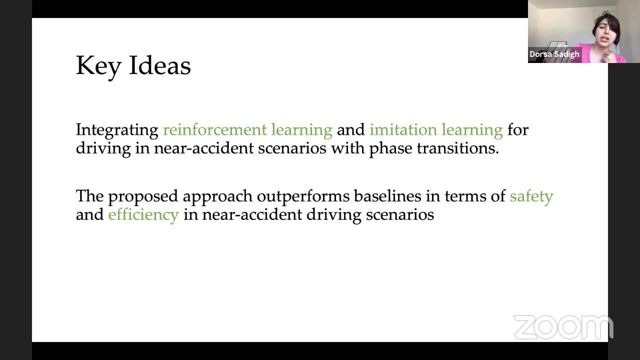 the hierarchical approach compared to some of these other baselines, which was kind of nice. So the key idea of this section of the talk was this idea of integrating RL and imitation learning in a way that we can think about balancing safety and efficiency in near accident. 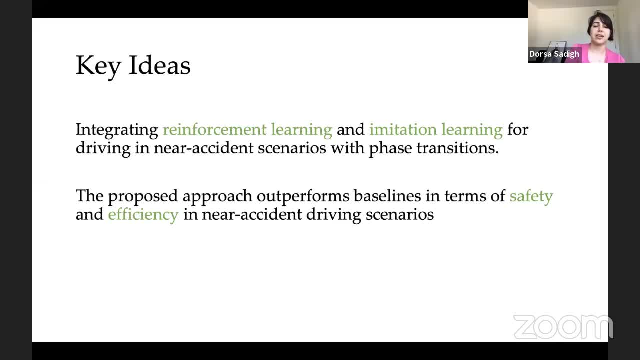 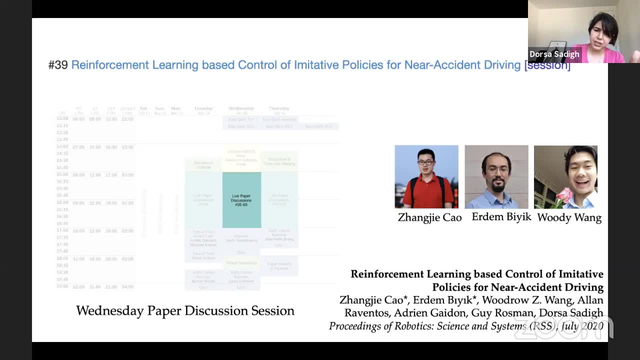 scenarios a little bit more carefully, because I think that actually matters when we are in near accident settings. and again, as I mentioned, this is joint work with TRI, actually with Adrian, who's giving a talk later today. Students who are leading the project are Zhangjia Erdem. 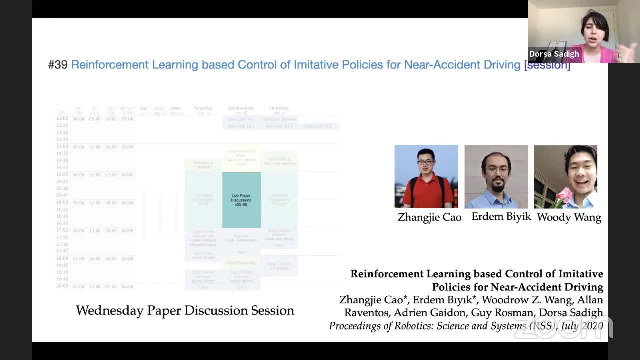 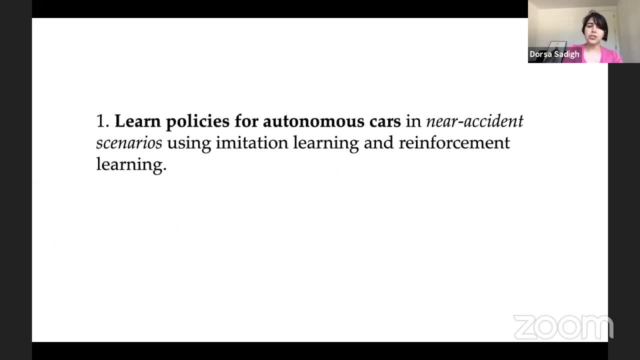 and Woody, so this is a paper on Wednesday, so feel free to join that discussion session if you're interested in more details of this project. All right, so okay, so that was about learning policies for autonomous cars in these settings, but what I'd like to switch to now is this idea of still being in your accident scenarios, but 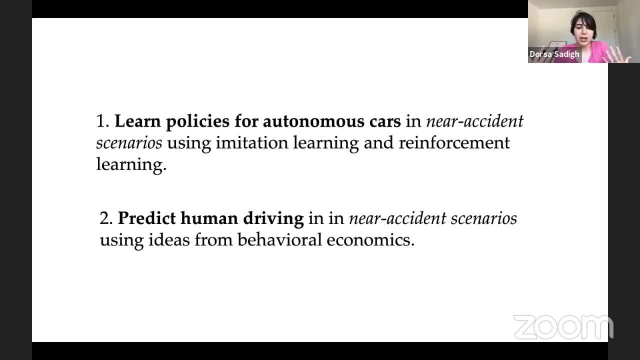 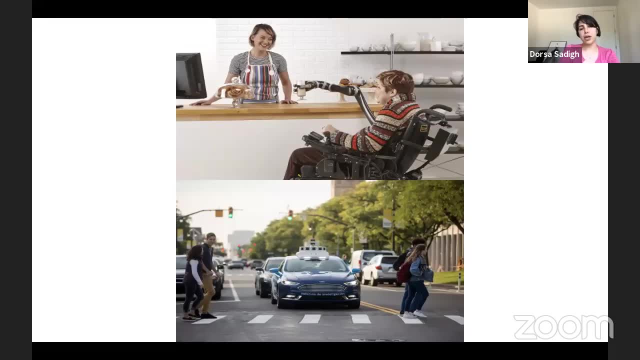 thinking about how we can predict human driving behavior and taking a more model-based approach, as opposed to the previous work, where you basically combine RL and IL together. All right, so I think we are now at the end of the session, so if you have any questions, feel free to reach out to me at. 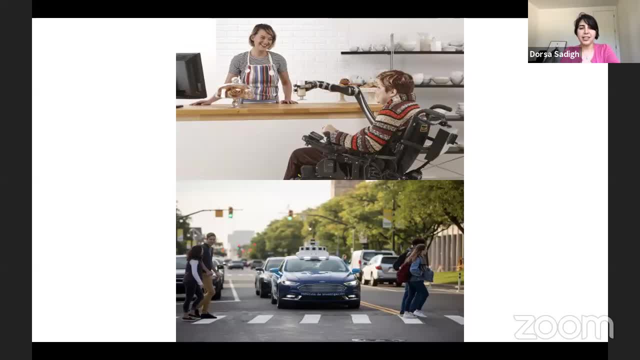 the end of the session. Thank you, Thank you. We all agree that if you want to have a robot interacting with a person, that robot needs to predict how humans around interacting. or if you have an autonomous car interacting with humans, pedestrians or human-driven cars, that autonomous car needs to have models of these agents around it. 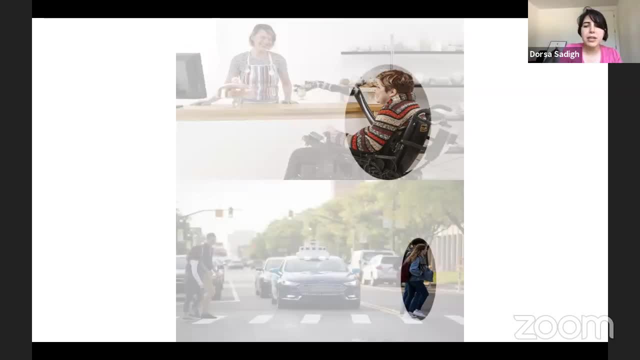 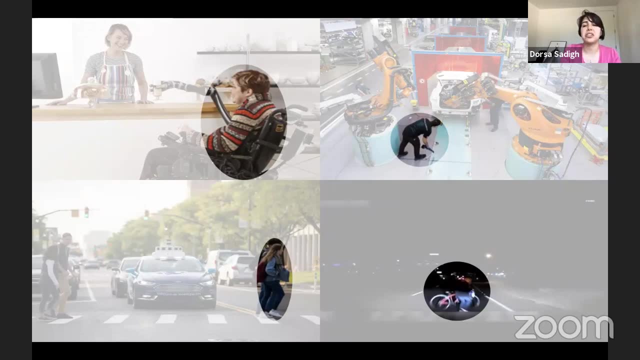 and the question that I think is interesting to ask is what happens if you go to slightly more safety critical situations? What happens if I have now a person interacting with these robots in a dangerous like factory floor? or what happens if you're thinking about an autonomous car? 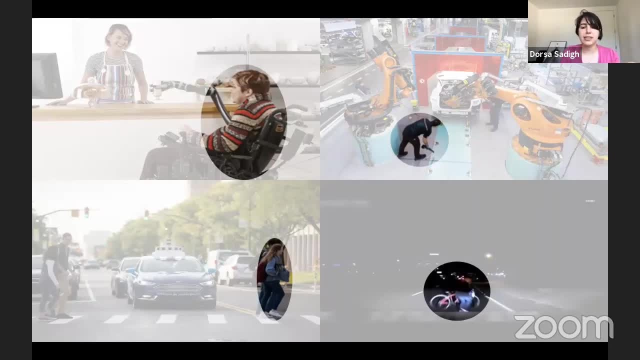 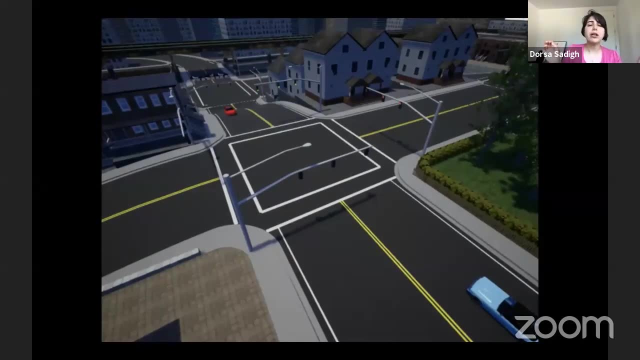 And you're interacting with people in your accident driving settings. So let me motivate this a little bit more by by an example, by running example that you can go over. So imagine that we have an autonomous car. again, it's a red car coming down the road. 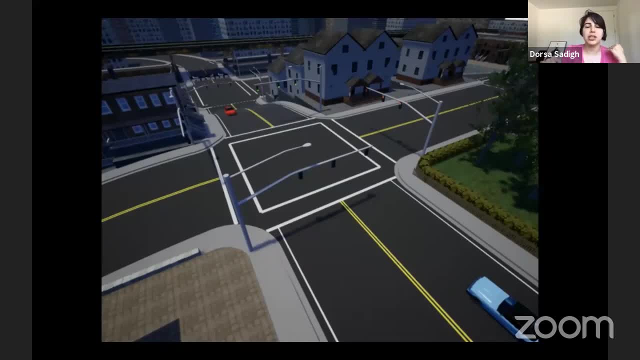 and what the red car wants to do is it wants to make an unprotected left turn. So it wants to make a left turn at the intersection and it's coming down the road and there's also this blue car that is coming down from the other side and at some point the light turns yellow. So when the light 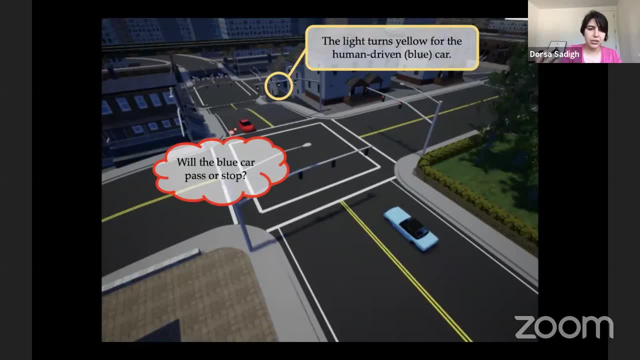 turns blue. it's in the middle section of the road, so we have a red car that we can go to And at some point the lights turn yellow. So when the light turns yellow, we have a red car- yellow. a good question that this autonomous car could ask from itself is: is the blue car? 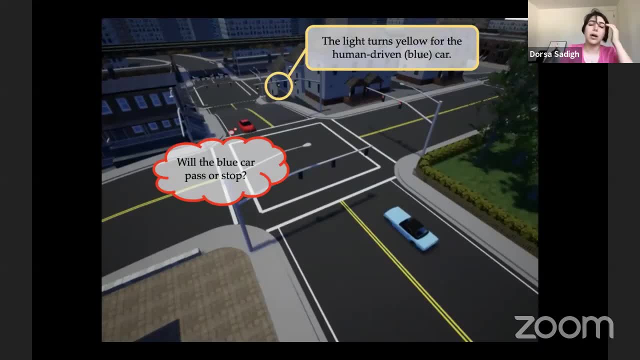 going to stop or not? Will the blue car stop or not? So the autonomous car could think about what would be the optimal action here, Based on the reward values. you can think about and compute what would be the optimal behavior of the blue car And actually the optimal behavior of the. 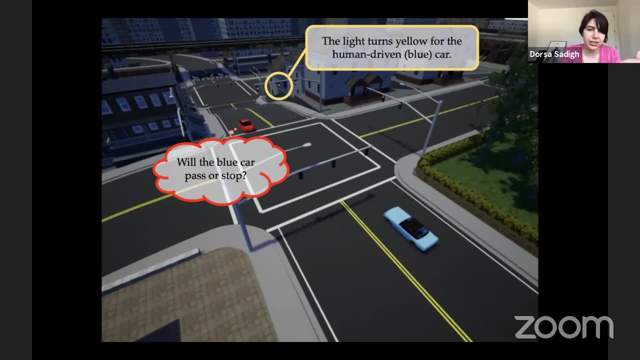 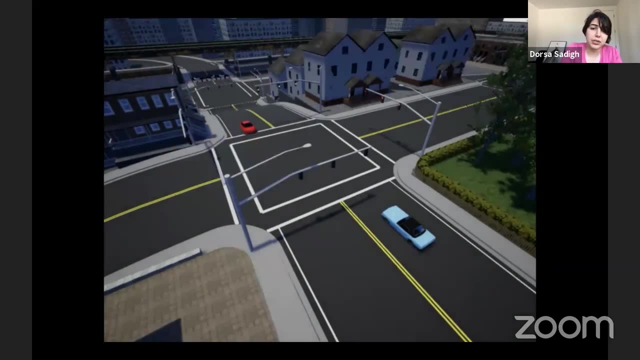 blue car in this setting is to stop because the light is yellow, it's going to turn red, it's got to stop And because of that the red vehicle should decide and proceed and try to make its left turn. But I think we all have seen cars passing yellow lights or red lights. 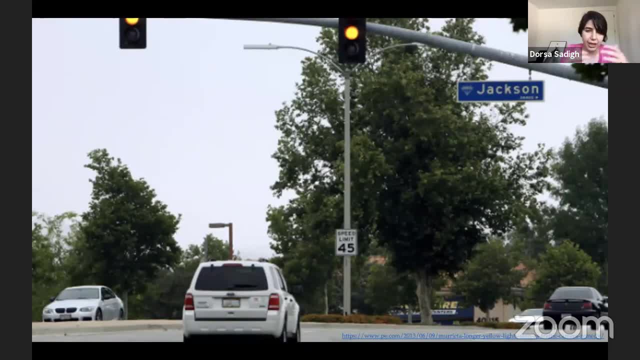 even though it might not be the optimal behavior based on a reasonable reward function. I agree one can change the reward function. so passing the yellow light would be the more reasonable reward function. But I think we all have seen cars passing yellow lights or red lights. 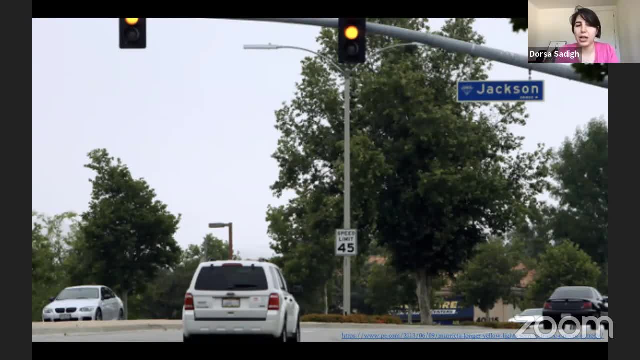 which is the more rewarding thing, But even if it is not the more rewarding thing, I think we have a lot of times seen people taking suboptimal actions and not necessarily maximizing reward functions, And that's exactly, I think, what robots in general need to handle. Robots should. 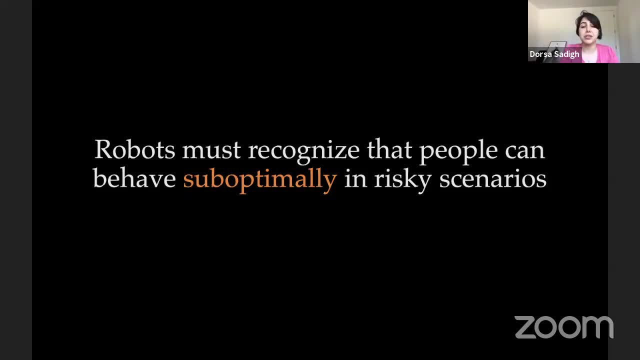 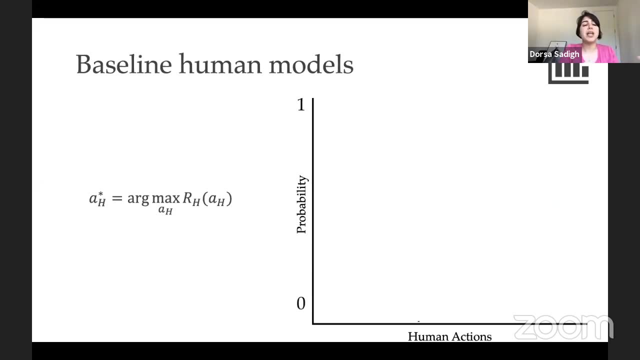 recognize the fact that people can behave suboptimally in risky scenarios. So so far, like the human model that I've been relying on, is this human model where we assume that there's a policy for the human, that's a maximizer of a reward function. This is the model that I 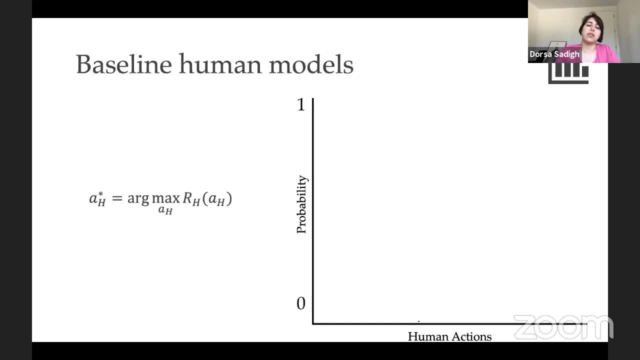 used earlier in the earlier work, where the car- like- not just in front of other vehicles- changes lanes right. So this is a model that I assume my humans are actually like acting- acting with- And this assumes there is an optimal action and the human is rational and will take the optimal. 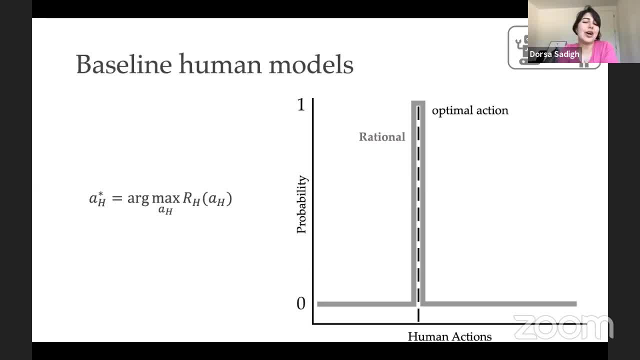 action. The problem with that is humans are not always rational, optimal agents that are optimizing reward functions, And I think in recent years people are realizing that that is not necessarily true and humans are not going to always act optimally. So so 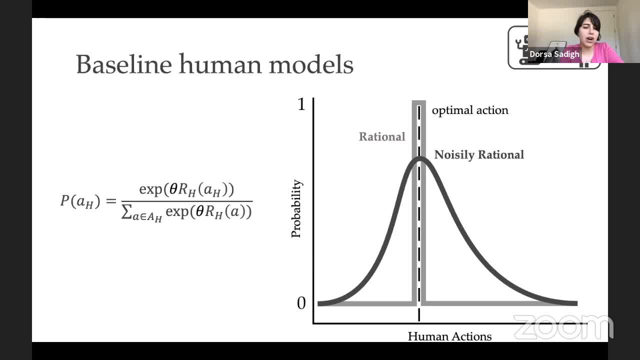 kind of like. a slightly better model than this rational, optimal agent model is this other model called the noisily rational model, where we assume actions of humans are probabilistic, So at least they're not deterministic, They're not deterministically picking something Their. 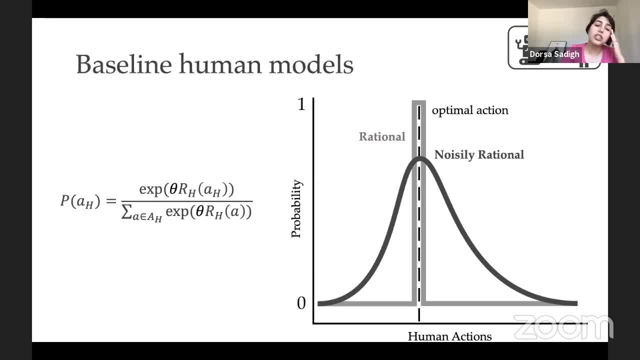 actions are probabilistic and probability of these actions is proportional to exponential of some theta parameter times. some reward function, And this theta parameter is a temperature parameter. It's commonly referred to as a rationality coefficient And, depending on what this parameter is, if you put that equal to infinity, you get your optimal action. If you put that equal, 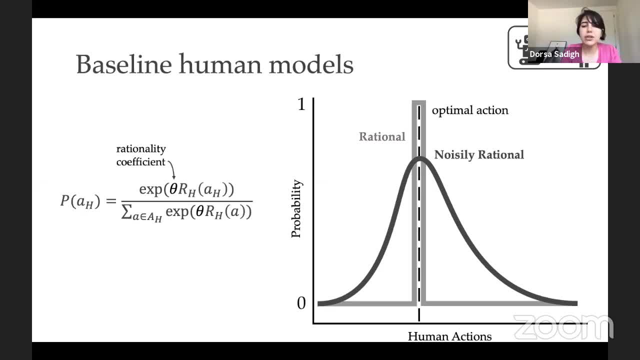 to zero, you get random actions And, depending on what you pick, then you get some sort of some sort of curve here that represents how humans act. Okay, So this is a better model, but there is a problem with this model, And the problem is this noisily irrational model, The 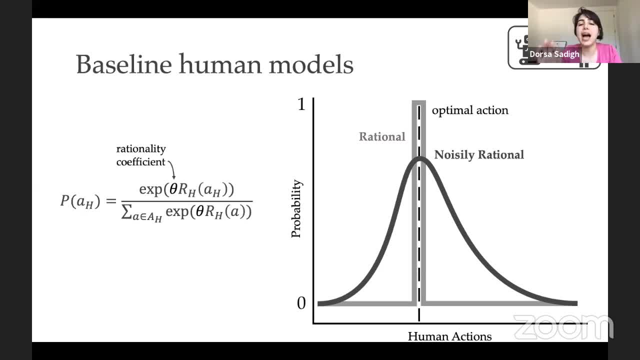 human still assumes that the most likely action of the human is the optimal action. So so it doesn't really capture the fact that, Hey, there could be scenarios where the most likely thing that people do is not necessarily an optimal action. Maybe the most likely thing they would do 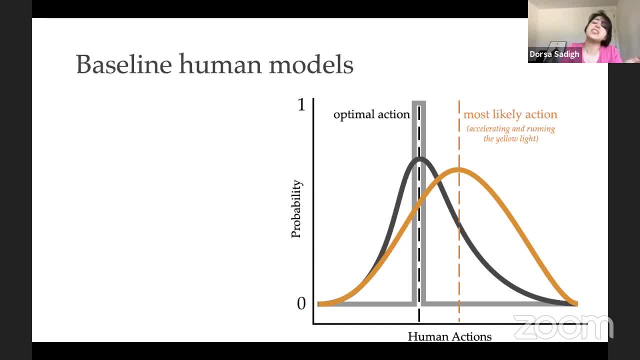 is to accelerate and run a yellow light, And that is not necessarily the optimal action. So, ideally, if you would want to be able to capture something like the orange curve using using some model that is able to capture something like the orange curve, and then think about 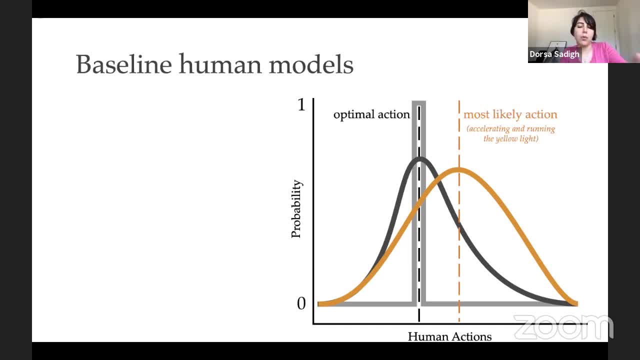 settings where we are able to handle a most likely action of human being, something suboptimal. Okay, And you want to do that in a systematic way, right, Like I understand, if you change the reward function and sit down and try to do reward design, you could come up with this: 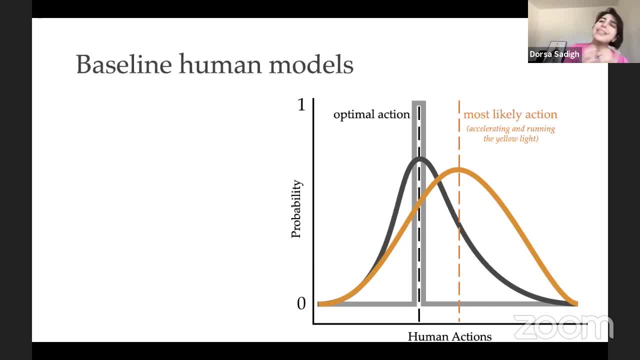 curve and make this one the optimal thing. But the thing is, reward design is really difficult And I don't want to spend time on reward design. Instead, I would like to write the reward function- that seems the most natural thing to do- and then do some set of transformations on the reward. 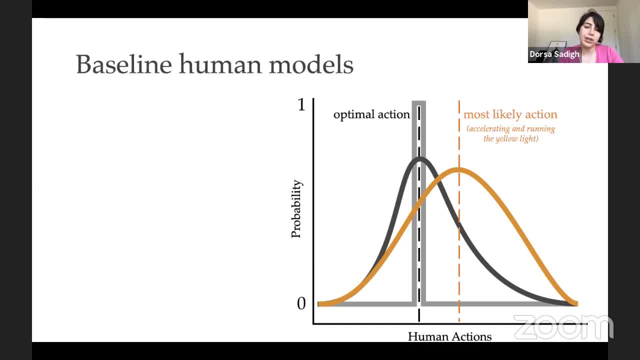 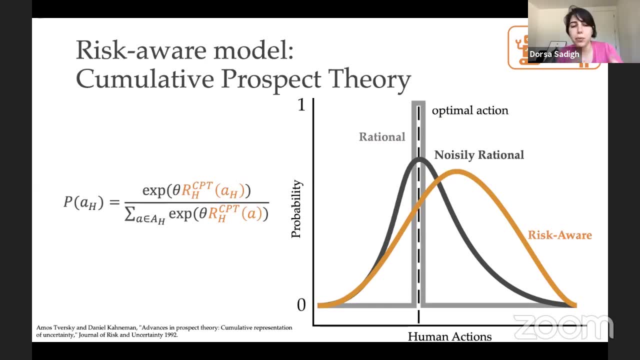 function to be able to capture these risky, risky behaviors. So the way we go about this is we use the same model as before. We say, well, probability of actions of humans is proportional to exponential of some theta parameter times, some reward. But this reward is going to be a transformed 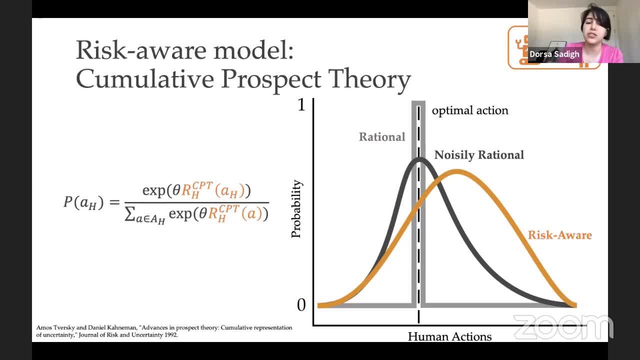 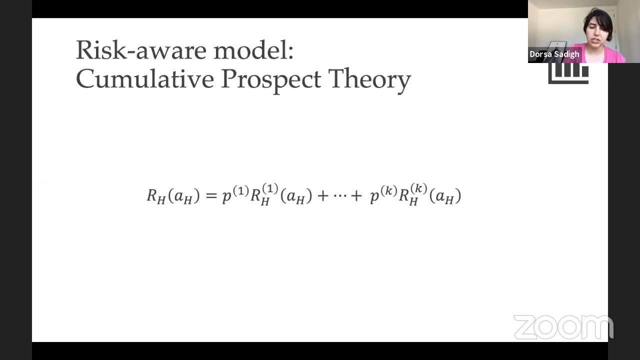 reward of our original reward function. We make a set of nonlinear transformations on top of the original reward And these nonlinear transformations is based on ideas from prospect theory and behavioral economics where one can actually capture risk. So just to quickly go over, like what these transformations look like. imagine: well, I have my reward. 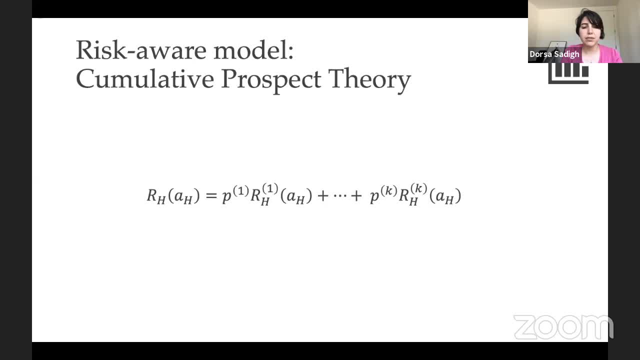 function. It's a sum of products, of probabilities of events, times, rewards of events, maybe passing a red light or not passing a red light, And then, if you think about each one of these probabilities and rewards, one can make nonlinear transformations on top of them. So, looking at the reward, 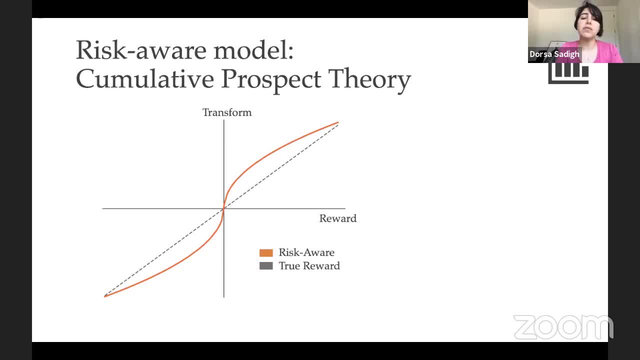 if this is the true reward, what prospect theory tells us is, when it comes to risky scenarios, we actually need to make this particular nonlinear transformation using a set of hyperparameters, And this transformation is exactly what tells us, like the fact that people are having a hard time differentiating between high reward scenarios. 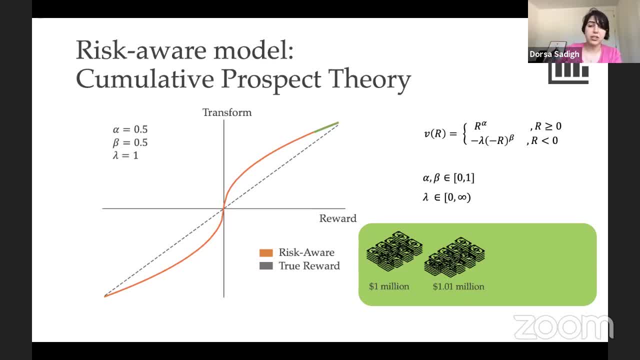 for example, differentiating between $1 million and $1 million and 10K, right, 10K doesn't have that much value in that setting, But if you're trying to differentiate between $1 and 10K, 10K actually has a lot of value. So this is actually the exact same idea And, using this, 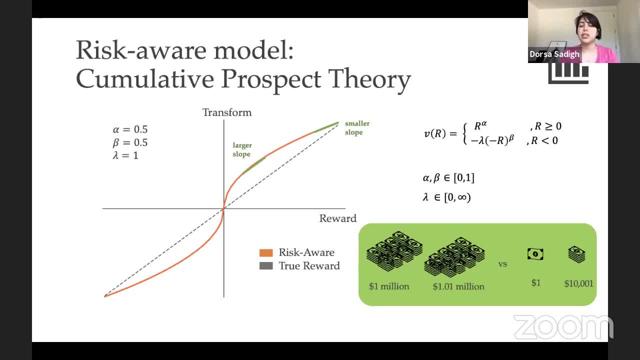 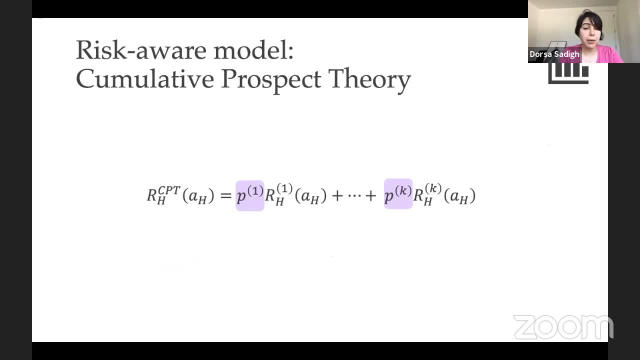 nonlinear transformation we can basically capture this type of biases that humans have And another set of biases that shows up is in the probability. So one can make a set of nonlinear transformations also in the probability. And specifically the nonlinear transformation we are making here is by overweighing low probability events and underweighing high probability events. 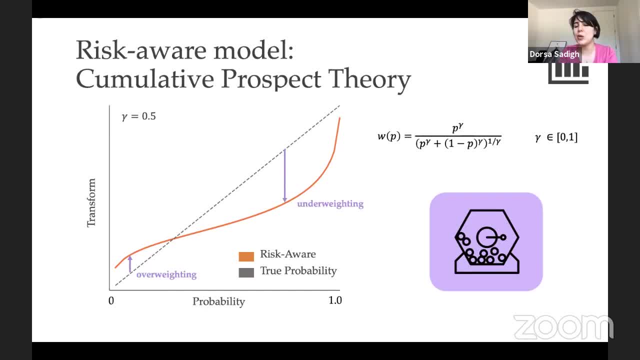 This is again the same exact transformation that one would do when you're thinking about settings where you buy a lottery ticket or when you buy insurance. This is like very low probability events. People tend to overweigh them And that is why the true probability is kind of like a nonlinear version of what you'd think. 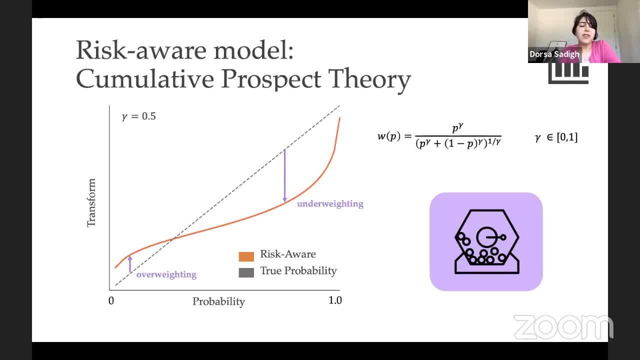 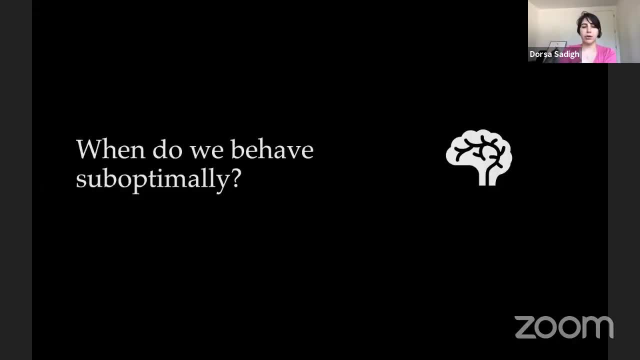 would be the true probability. And in here are a set of hyperparameters, and these hyperparameters could actually be tuned based on the data collected from humans. All right, so let me just show you some results on this. So we decided to try this out in the 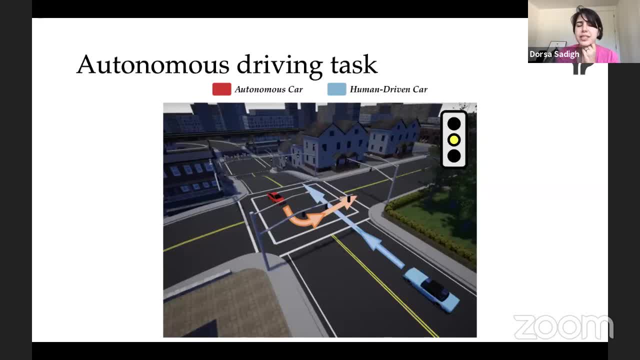 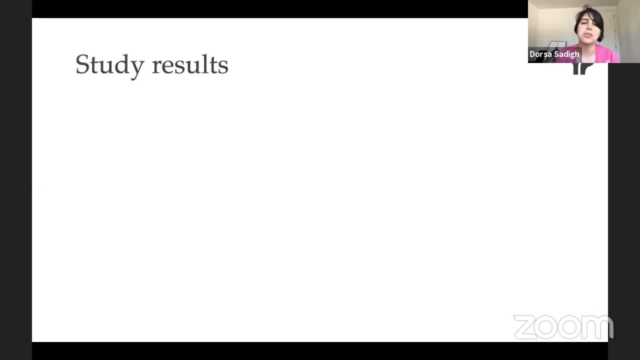 near-accident driving scenario And what we wanted to do first was to just run a user study to see, like, how people make decisions here, like how to actually people make decisions when it comes to these near-accident scenarios, And we vary the set of factors and the main factor that 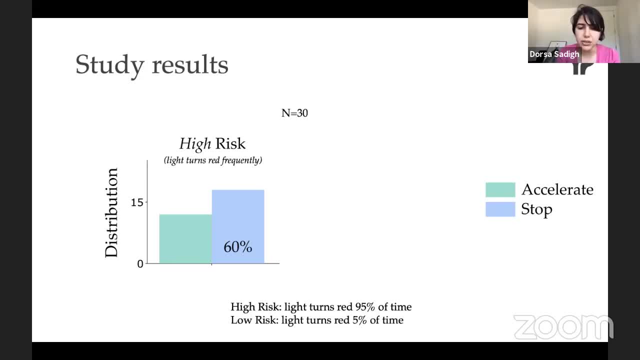 actually made a difference here was risk. So we have high-risk scenarios where the light turns red 95% of the times, and we have low-risk scenarios when the light turns red only like 5% of the times. And in high-risk scenarios, people 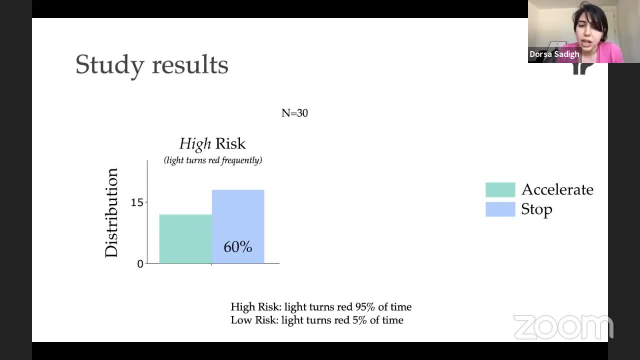 are more likely to stop. They actually take the optimal action, But it turns out that when you're in low-risk scenarios, that is, when the majority of people are preparing the suboptimal action, They tend to stop, but the optimal action is to accelerate. 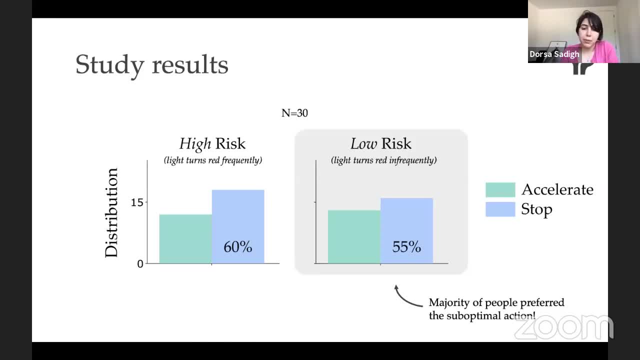 So that's interesting. That tells us that in low-risk scenarios, people are not making the optimal action, And what we do here is we try to basically learn the set of hyperparameters based on the data and compare a risk-aware model with the noisily rational model. 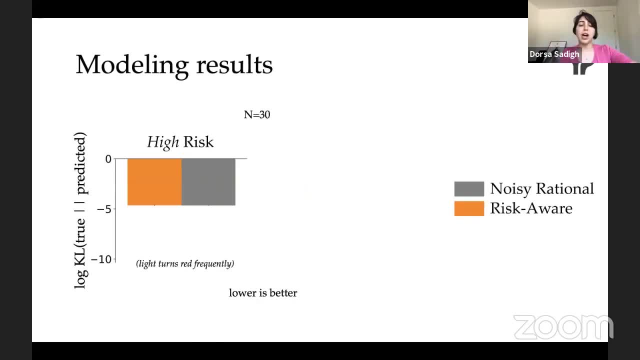 So, going back to the same exact scenario, if you're in the high-risk setting, in the high-risk setting actually there isn't any difference between the risk-aware model and what the noisily rational model would do. But if you're actually in the low-risk scenario, 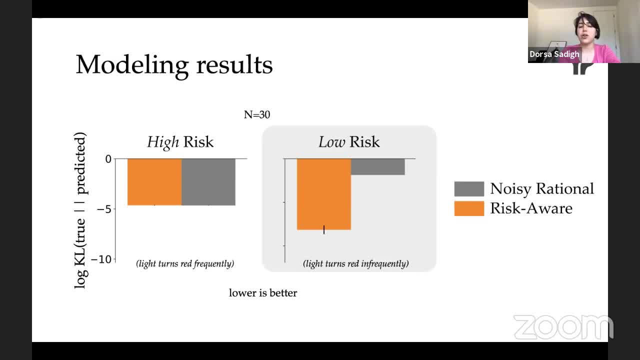 when people are making these suboptimal decisions. the risk-aware model is better at capturing the fact that how people would actually drive in these settings. Just to extend this: this is not just about driving. One can go beyond driving when it comes to thinking. 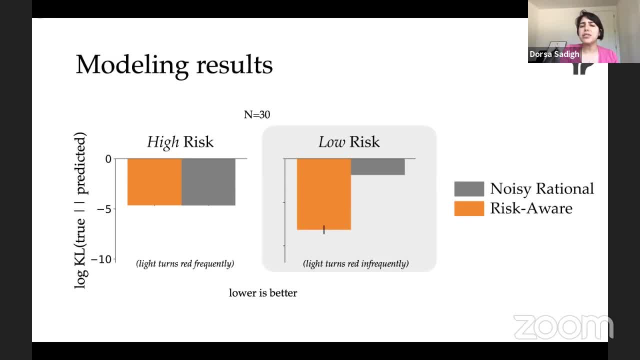 about these types of behaviors And we decided to run an experiment where we have a robot that plans based on these models. So if I have a robot that plans based on these models, that wants to plan based on these models, the question is, how would the robot collaborate? 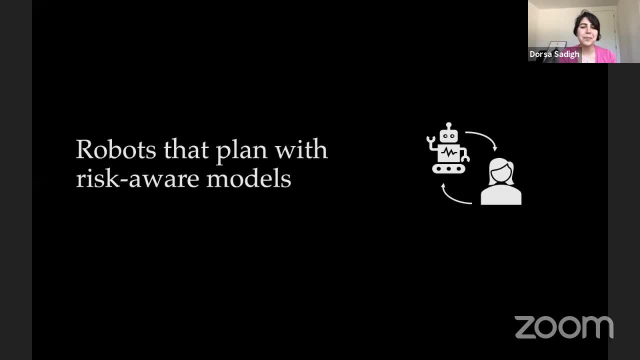 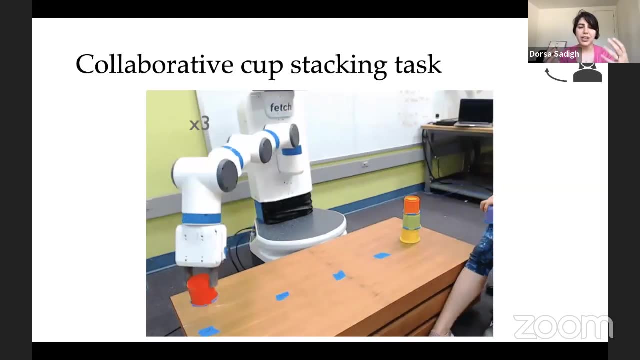 and coordinate with humans, based on the risk-aware models. So we decided to run an experiment where we have this collaborative cup stacking task, where we have a human and a robot taking turns and putting cups on top of each other And they have two options. 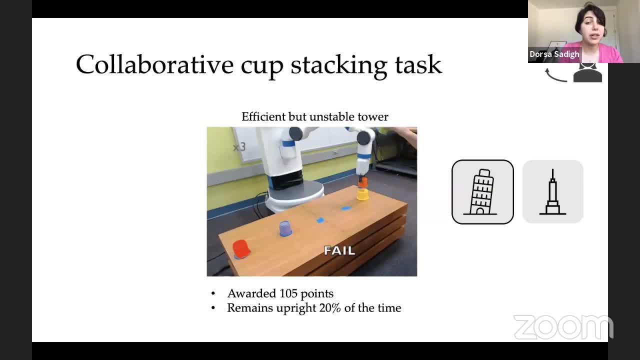 One option is to build an efficient tower but an unstable tower, something like the Tower of Pisa, where you're putting the cups on top of each other very efficiently but the tower only stays upright like 20% of the times. But if it stays upright you get a lot of points. 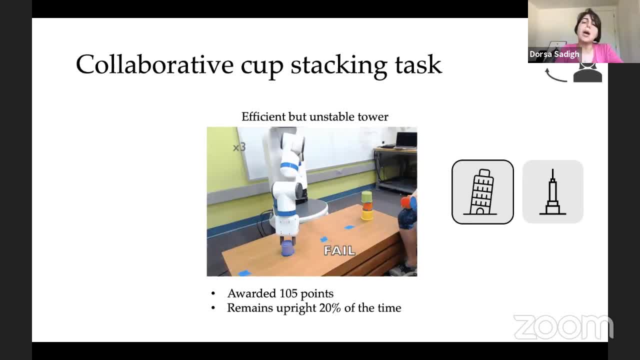 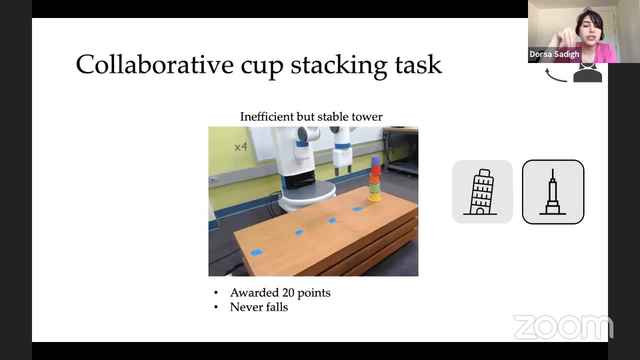 You get 105 points. The other option is to go for an inefficient tower. but it's stable. So you decide to put the cups on top of each other in the decreasing order of size, so you make sure that it stays stable. but it's very inefficient to do it. 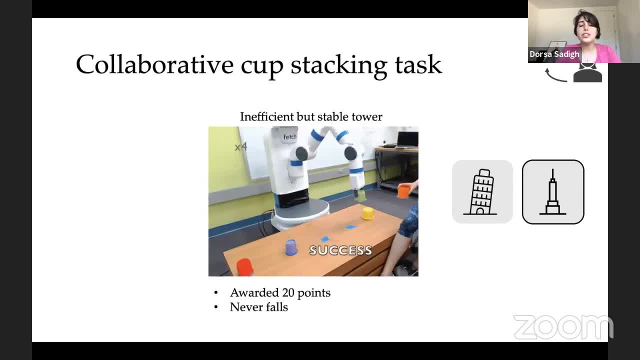 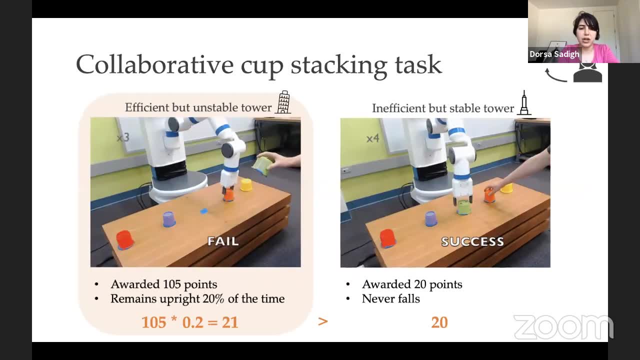 because you have to think about it. So this tower never falls, but you only get like 20 points because you're guaranteed to make the tower work. So we actually have humans and robots coordinating with each other on this task. And if you think about the reward values, 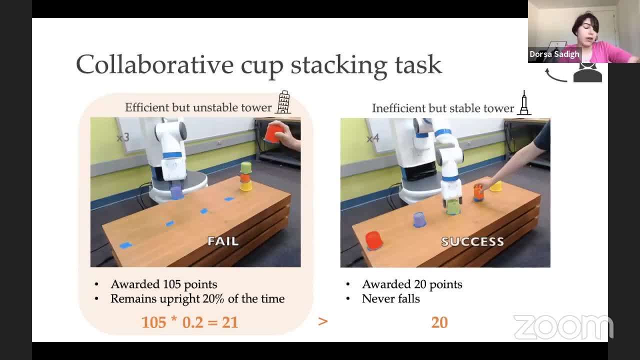 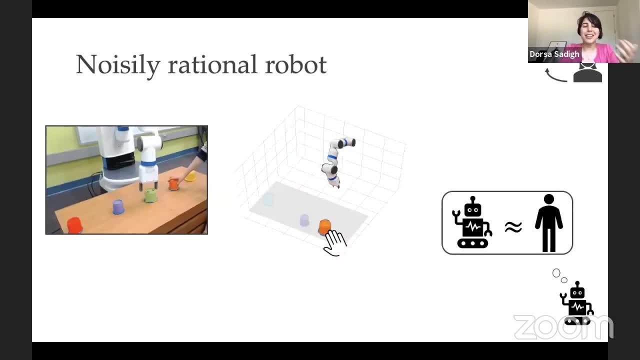 the optimal thing is actually to take risks and go for the Tower of Pisa, try to build that unstable tower. But it turns out that when you have humans interacting with these robots, humans are overly concerned about the tower falling, So this is like a risky scenario for them. 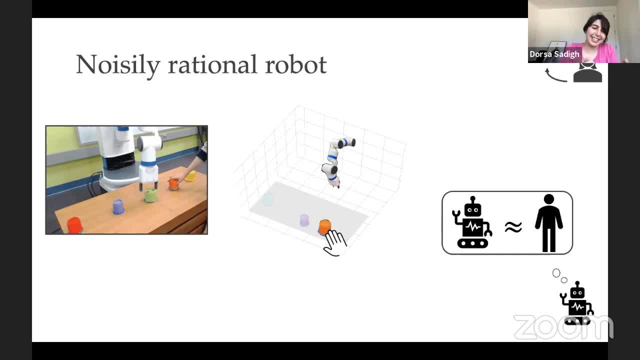 And they actually don't want to build the Tower of Pisa. Like humans, like in these settings, actually prefer to take the more conservative action, be more risk averse, And what ends up happening is that a robot with a noisily rational model, the human, doesn't detect that. 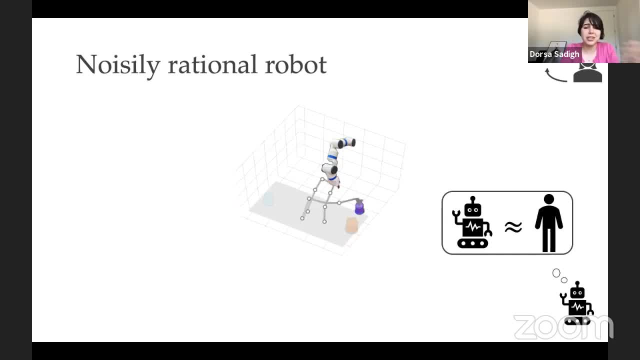 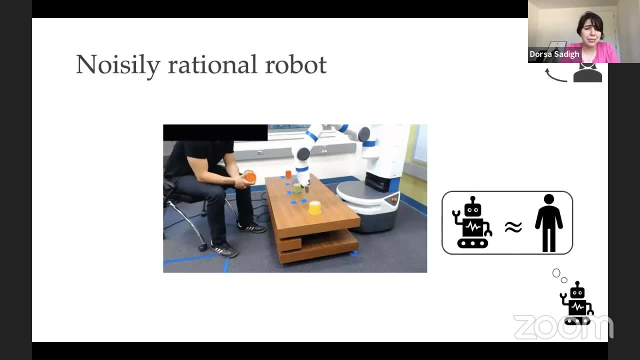 And because it doesn't detect that it needs to replan and go and pick up something else and come back around Here. it's actually seeing it in action. Like Roberto goes and picks up the orange cup, Robot also goes and picks up the orange cup. 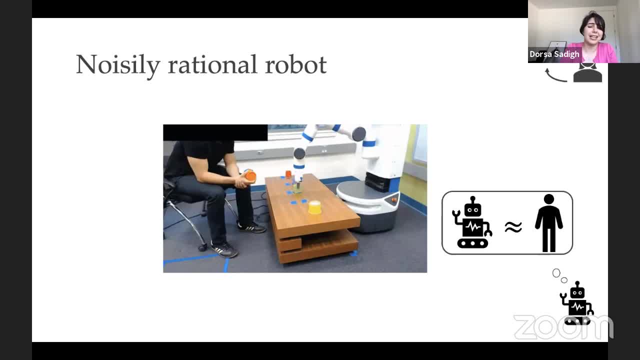 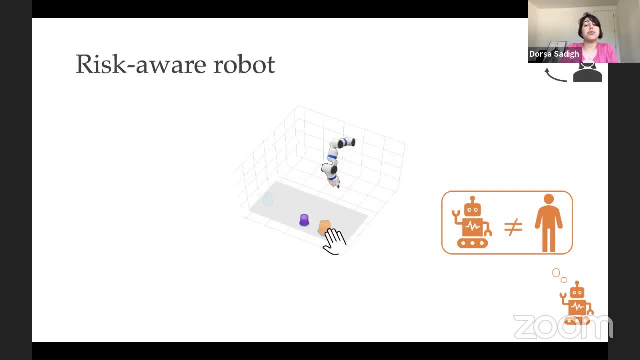 but it comes empty handed and it needs to replan and try out again. But if we actually have this robot using a model, a risk aware model of the person, then the robot would realize that the human is going to be overly concerned. 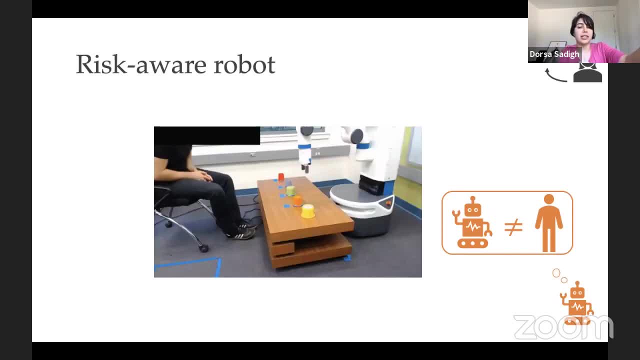 So it just takes a complimentary action from the beginning and they end up collaborating and coordinating with each other much better. So I know this example was not about driving, but a similar thing is actually true in driving, Like if you have again an autonomous car. that 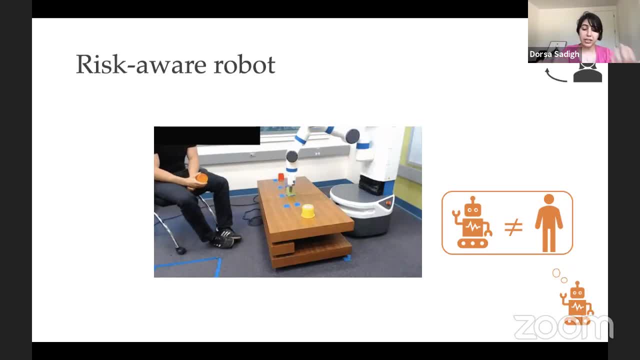 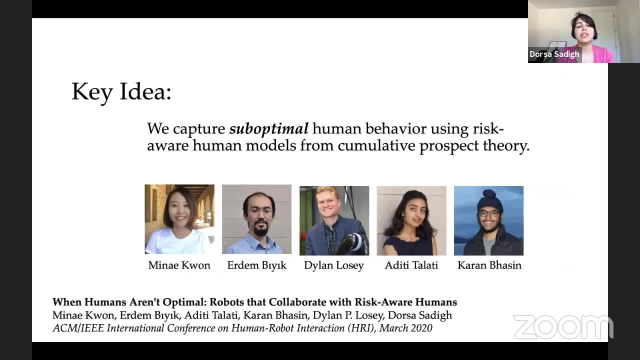 can capture the fact that humans are going to act suboptimally, then that autonomous car can better coordinate and collaborate with that human and predict what that human is going to do in a near accident driving scenario. So just to summarize the key idea here: 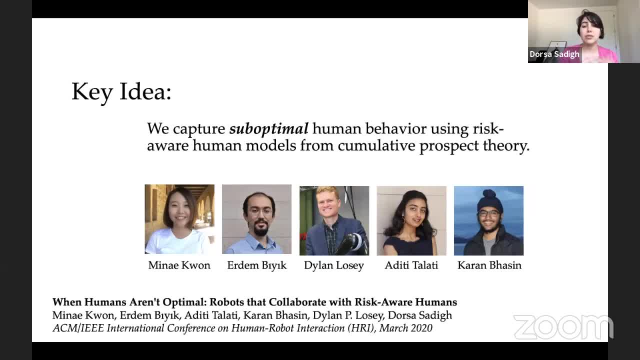 is, you're capturing these suboptimalities using a notion of risk and using a notion of basically modifying the reward function, using nonlinear transformations based on ideas from prospect theory and behavioral economics, And this was actually a work that we presented at HRI. 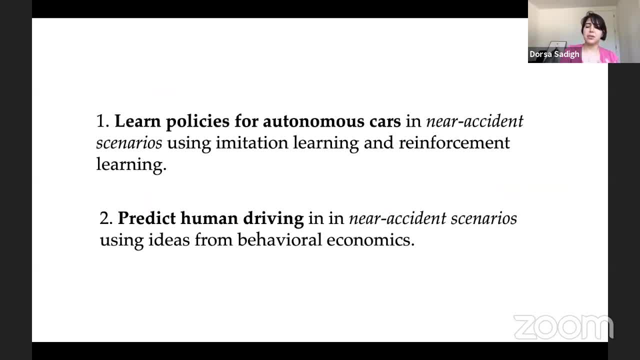 this year. And then just to quickly summarize, I think handling near accident scenarios is really important and we need to start paying attention to that a little bit more, Because that is where some of our assumptions actually fall short. And today, what I basically talked- 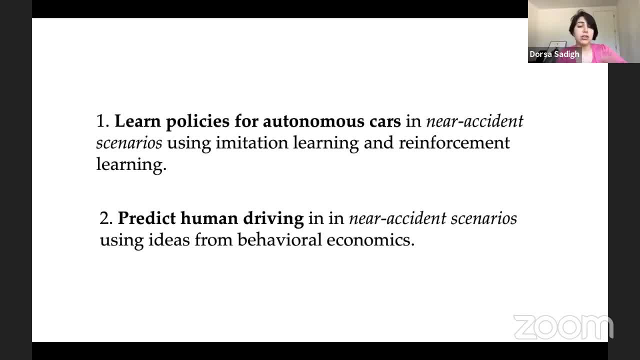 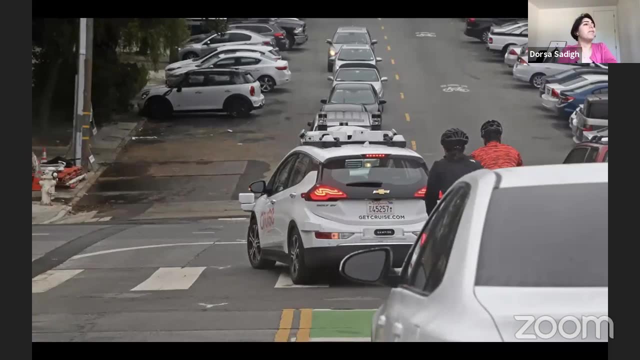 about is how we can use a learning-based approach and data-driven approach to think about how cars should drive in these settings and then how we can take a more model-based approach to better predict risk and how human-driven cars around us actually drive. And going forward, I do think this idea of modeling humans 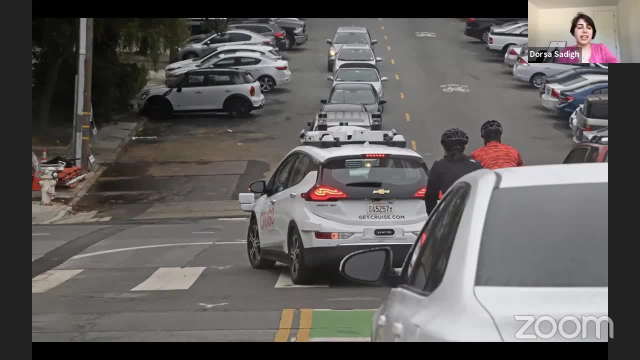 and thinking about interaction a little bit more carefully matters a lot, And one step ahead, I think, is thinking about adaptations. thinking about my behavior when I'm driving right next to this autonomous car for the 10th time is going to change. 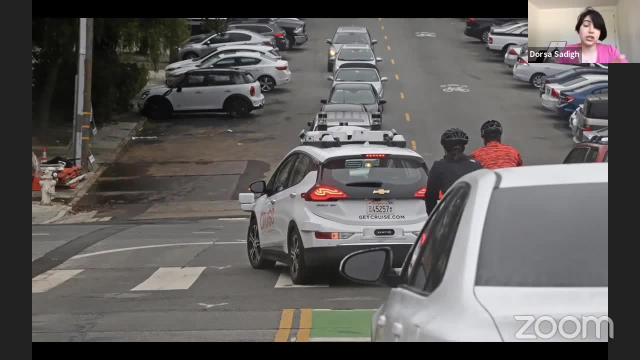 And I'm not going to, for example, like if I see this car driving I might just go around it, if I bike around it, Because in the previous settings when I've interacted with this car, this car was stuck, So because of that I would decide to go around and maybe 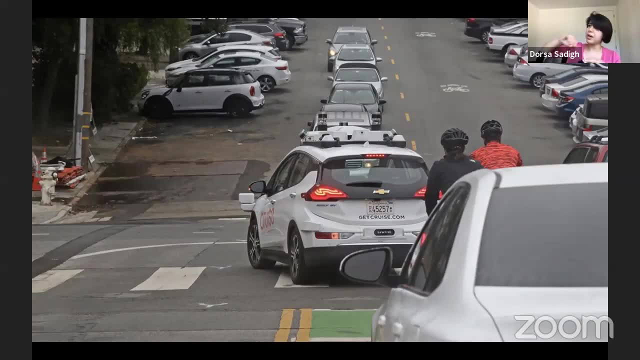 do something else. So this idea of adaptation, like everything I've said so far, is about building human models, rewards, functions, policies that are fixed, But humans adapt, and then we actually need to start thinking about how humans adapt in these interactive scenarios. 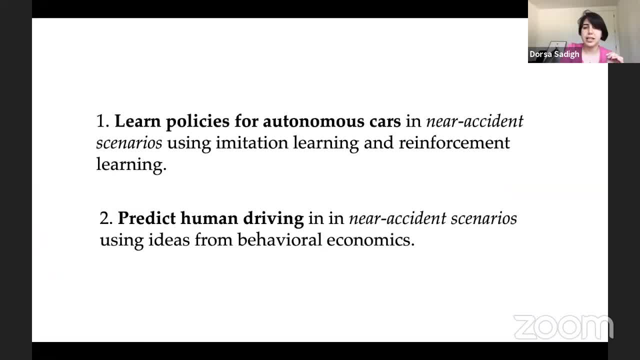 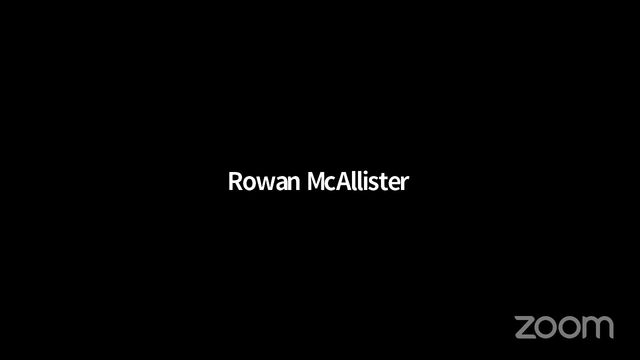 Thank you, And with that I'd like to thank you guys and I can take any questions. Great, Well, yeah, thank you. Thank you so much. Thank you so much, Delosda. So OK, so as a reminder if you have any questions. 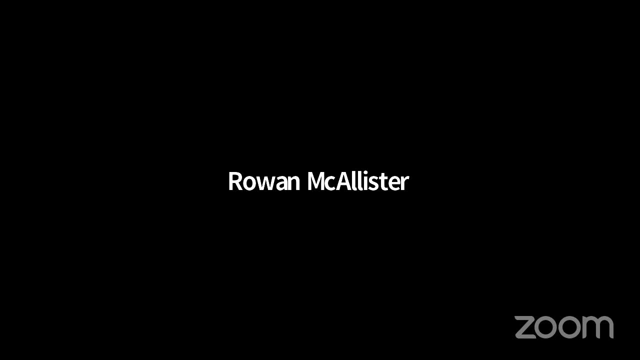 if you open up the chat, it should be at the bottom or maybe the top, depending on how feed loop is working. OK, we've got one question from Salah here, Delosda. The question is: I was wondering how computational complexity is. 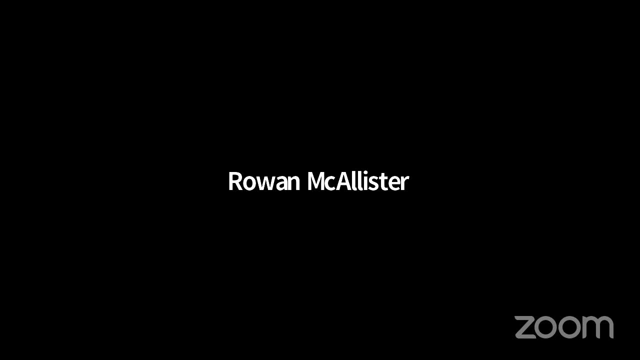 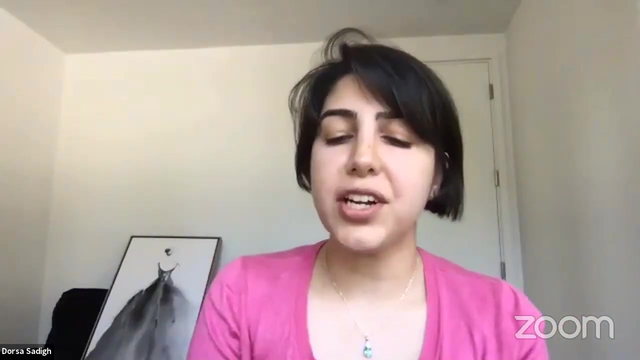 impacted. when you consider a distribution over human actions, rather than assuming drivers are rational, Is there need for alternative assumptions to make the problem tractable? I think that's a very great question. So I think what Salah is referring to is when you think about that interaction. 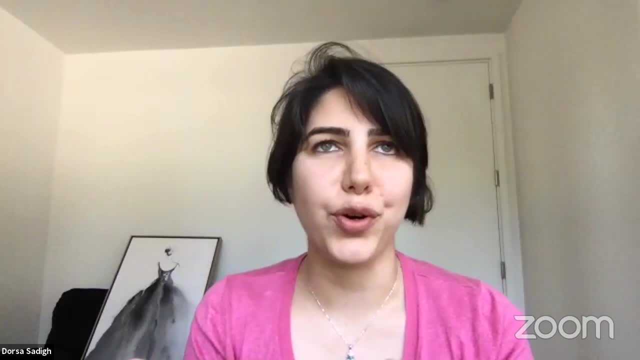 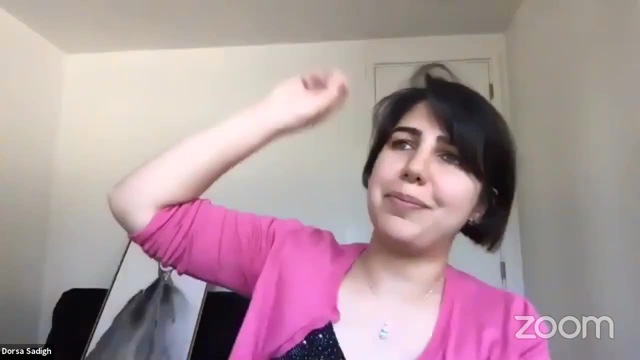 that I mentioned earlier. I assumed the human is optimizing a report function. One can have a better model than that, right, Like you might say. well, there is a distribution. The human is following the distribution. It is not necessarily picking the top of that distribution. 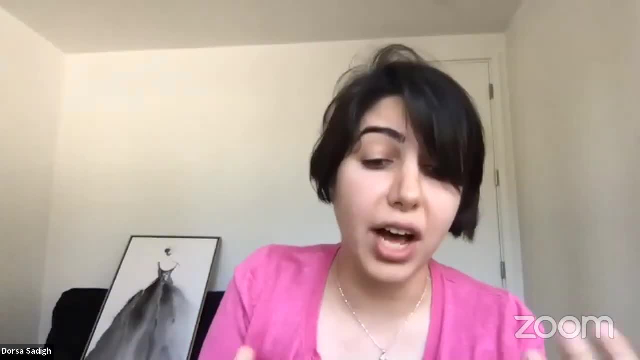 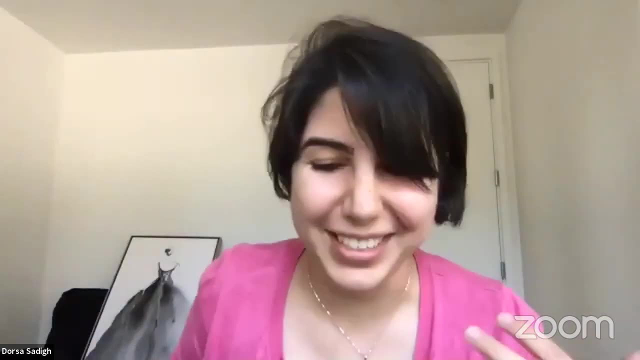 The human could take anything from that distribution, And that introduces a lot of computational issues. And actually that is the exact reason that in the earlier work you just assumed humans are deterministic. right, Like we assumed humans are rational and that they're deterministic. 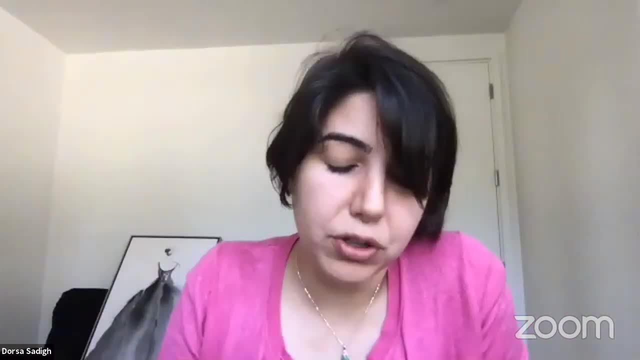 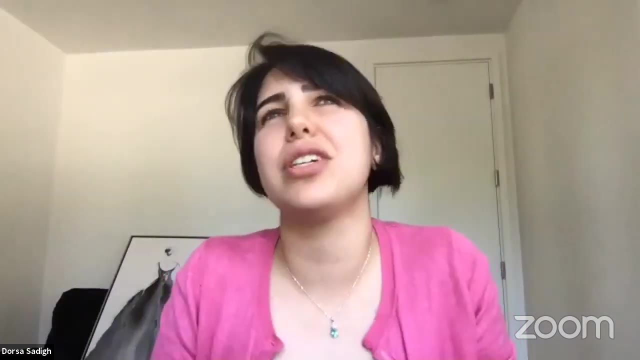 And they are not. And one can take a sampling-based approach, for example, to address some of these computational issues, But that doesn't really solve the problem. That's still going to be computationally really difficult. So the prospect theory approach is actually very efficient. 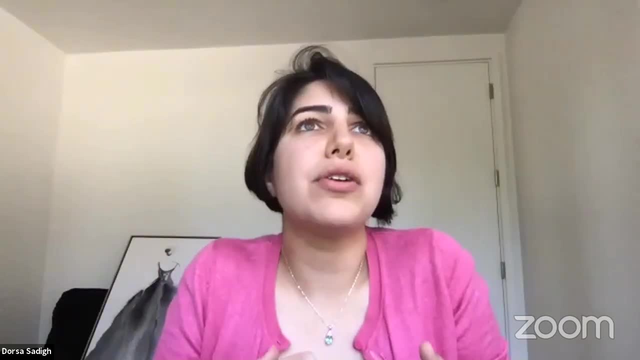 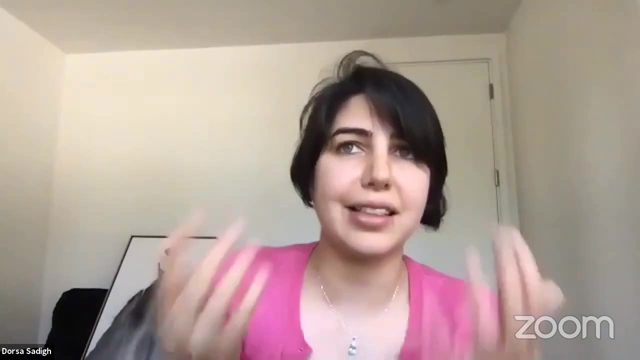 And it tries to kind of address that. So the prospect theory approach just does a transformation on the reward function. Instead of worrying about the distribution, you still pick the top of that, That part of the distribution That's a particular reward function. 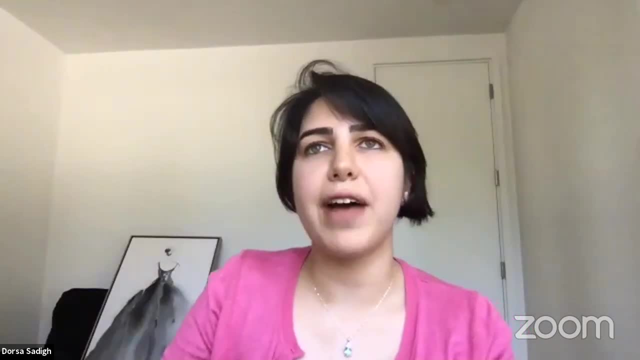 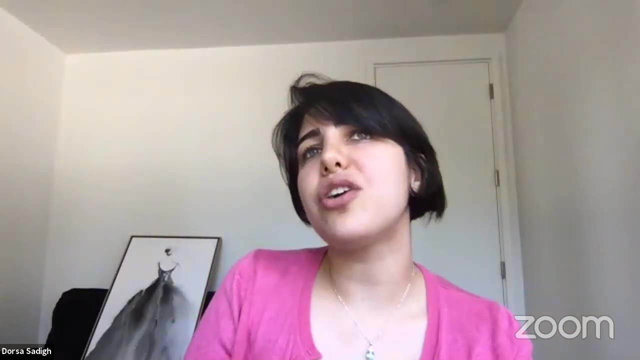 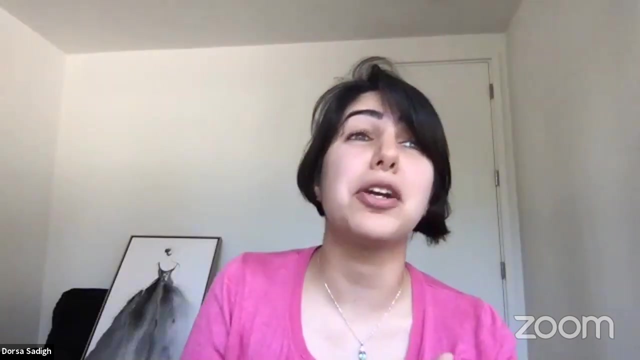 But making that non-linear transformation handles the fact that in risky scenarios people might act differently. I'm not suggesting that answers everything. I think in general we need to come up with way better computational approaches of handling these behaviors. I think representation learning does play a big role here. 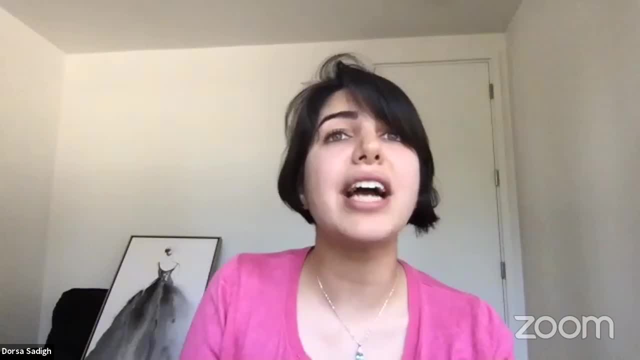 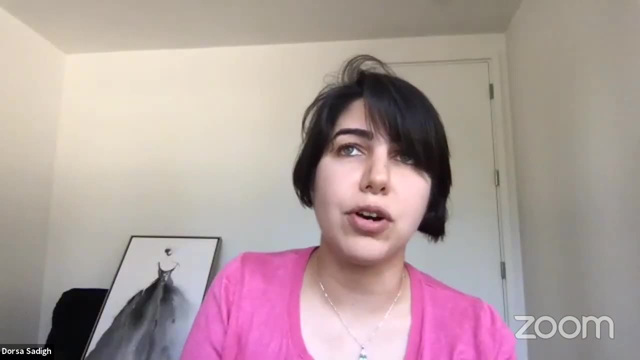 when we think about interactions- And I think that's actually how people interact with each other, Like when people interact with each other a lot of times they build representations, much lower dimensional representations, with each other, And that is the thing they keep track of. instead of full-on distributions of your partner's policies, And I think that could be a way forward to make things more computational. OK, great, Yeah, thanks. I also had a question. Oh, and we've got a response from saying. that makes sense. 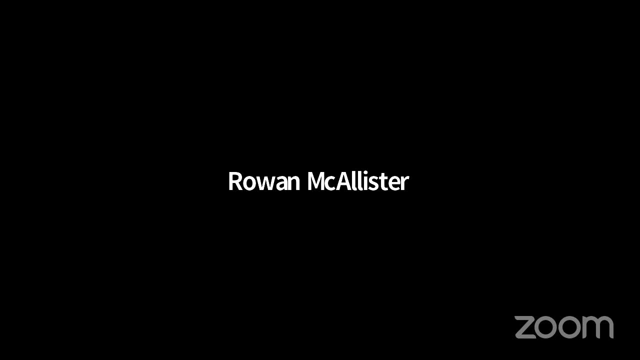 Oh, and I might ask- I might skip my question because someone else is asking for one. So Eric says, when a robot collaborates, should the robot make a decision and hope that the human would adapt to the action of the robot, Or should the robot always adapt and yield to the human's action? 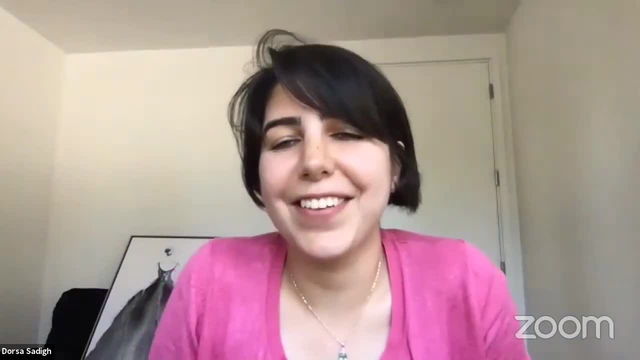 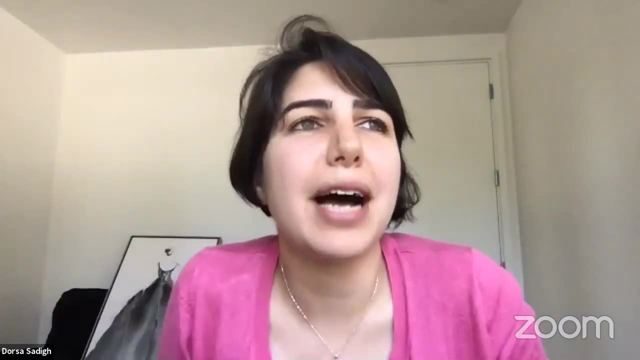 I think that's a very good question And that's something that we still don't know the answer to it. And it's a difficult question because I think a lot of people have started talking about co-adaptation and the fact that hey, 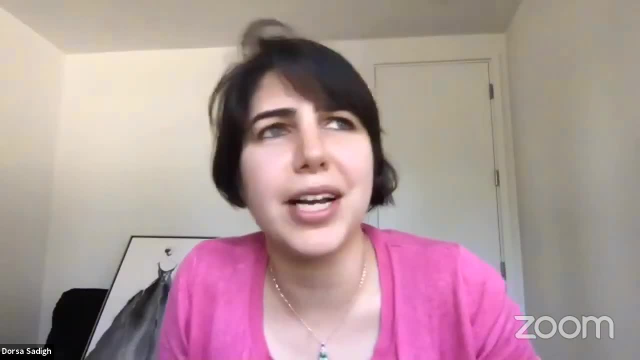 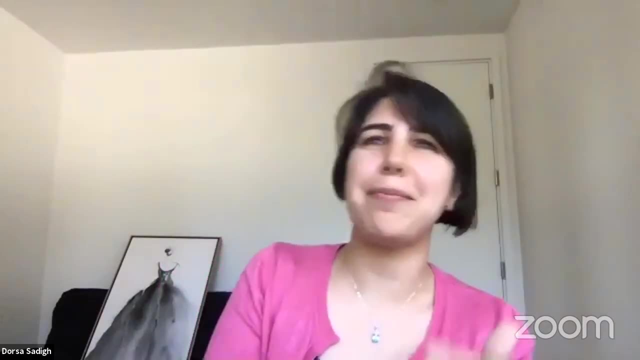 robots need to adapt to humans too, because otherwise humans adapt and they start taking advantage of you. But the scales of behavior, I think. but the scales of these actually matter too. Like, if I'm adapting and you're adapting, then you never get a chance of getting used to each other. 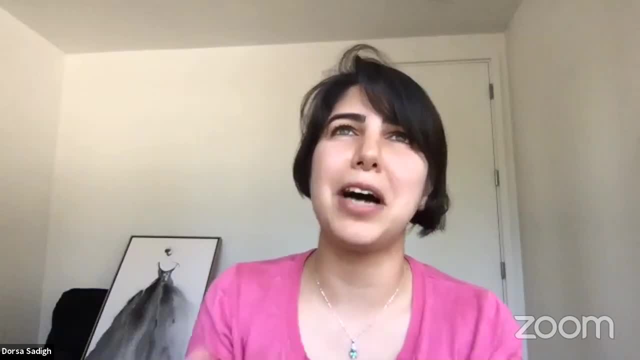 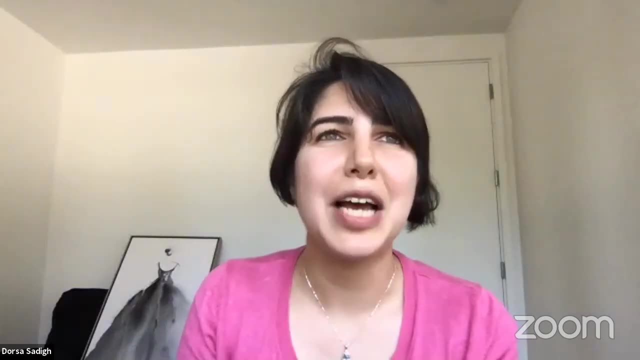 I do think they both need to adapt, Like in the case of autonomous driving. when I see autonomous cars around me, my behavior changes and I adapt to them, And the autonomous car can wait for that. But that would actually not be good for it. 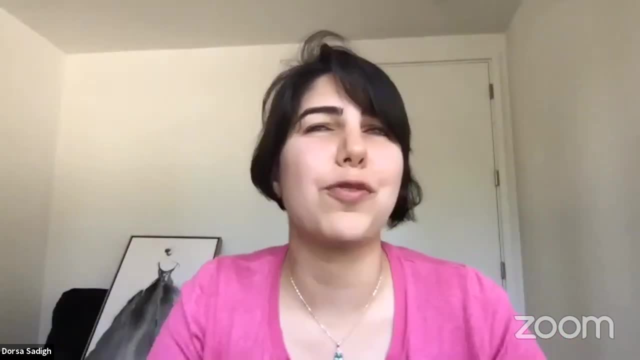 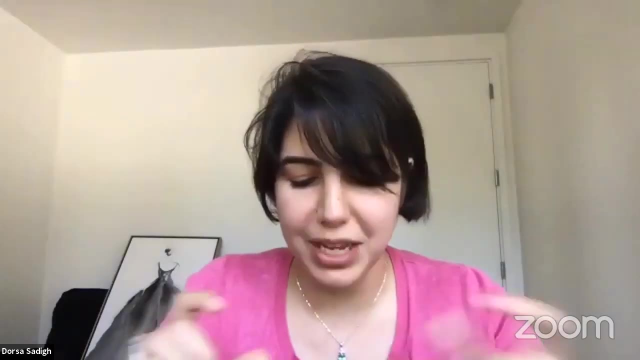 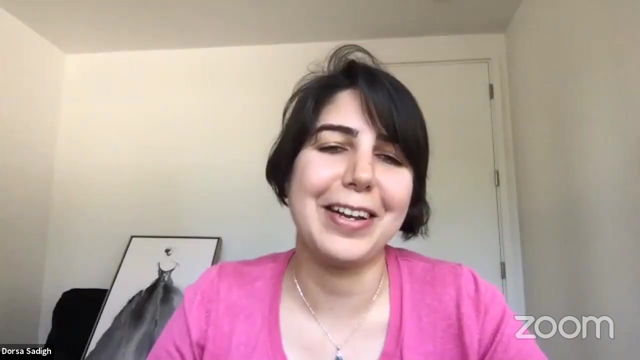 So over time it might realize that it should also adapt to its reward function. But the time scales and frequencies of these actually matter a lot For both of these agents being learning agents. So my answer is they both should adapt. How to do that is still a very open question. 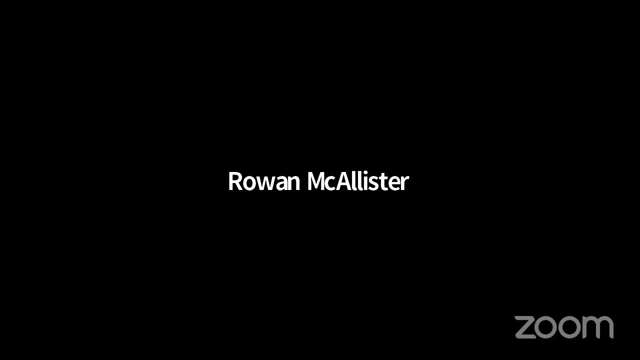 OK, great Thanks, And we've got time for one more question And so has asked. also thanks for the great talk. As you said, we have seen many, many new algorithms and technologies for planning and control of autonomous cars. 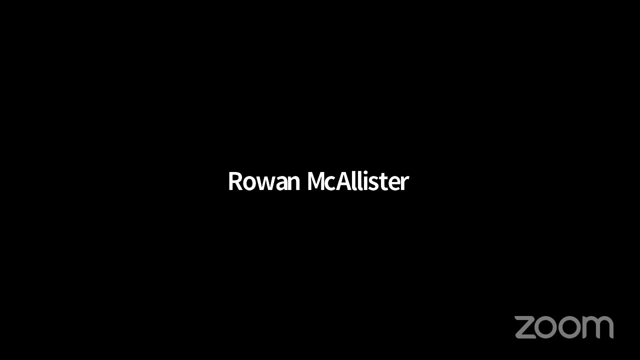 And safety rules somehow play the role of constraints on those algorithms. I'm wondering: do the safety rules and standards for commercial autonomous cars match with those new technologies? How conservative are they in the current state? Yeah, that's also a very good question. 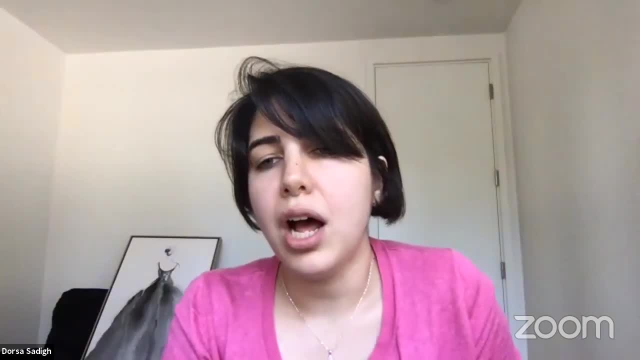 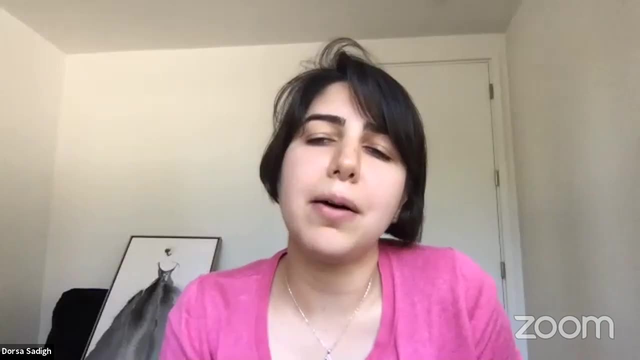 I think how you're addressing safety is an important question And at the moment I'm not that heavily working on some of these issues at the moment. I used to work on them, But based on conversations I've had with people, it seems like safety rules are not too. 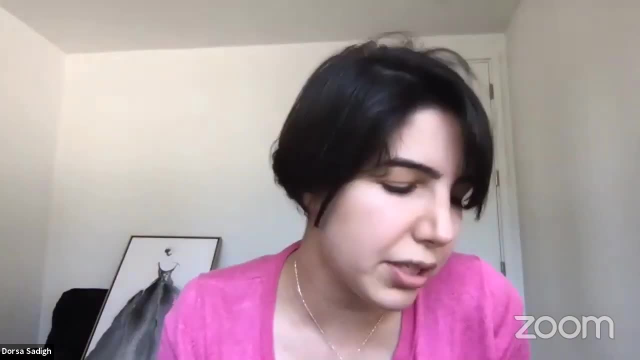 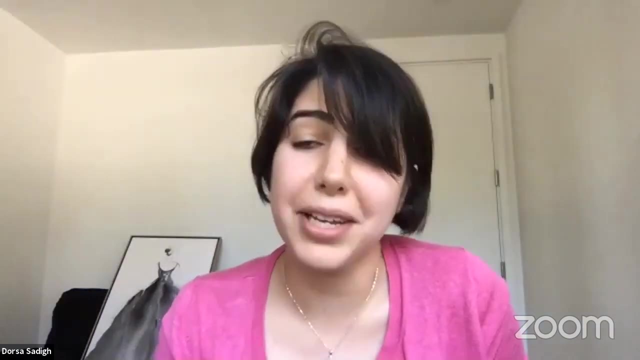 too big of a constraint at the moment. Actually, car companies- people I know in the car companies they are putting constraints, more constraints on themselves than the actual rules that are out there. There is a big mismatch between those rules and what the technology actually can and cannot do. 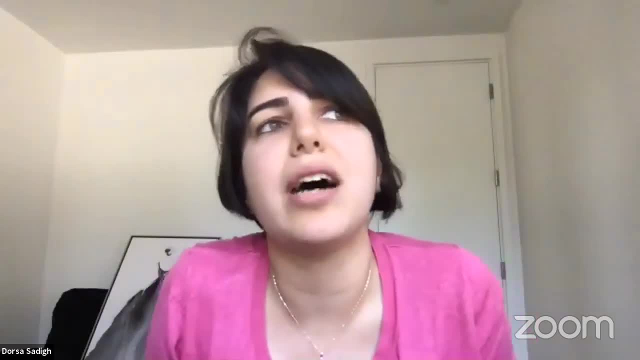 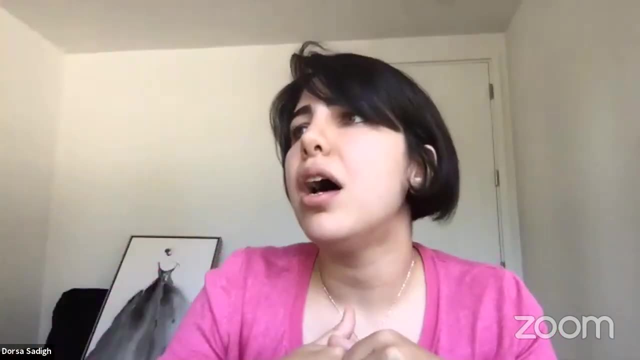 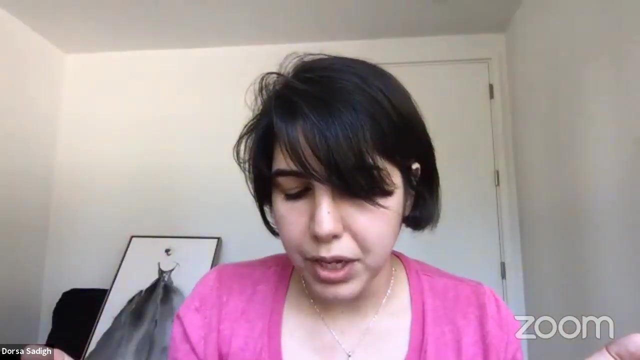 And I do think car companies, thankfully, are quite careful about being safe and satisfying way more constraints than what Nitsa, for example, tells them. I do think that mismatch needs to be solved and they need to like get closer to each other. 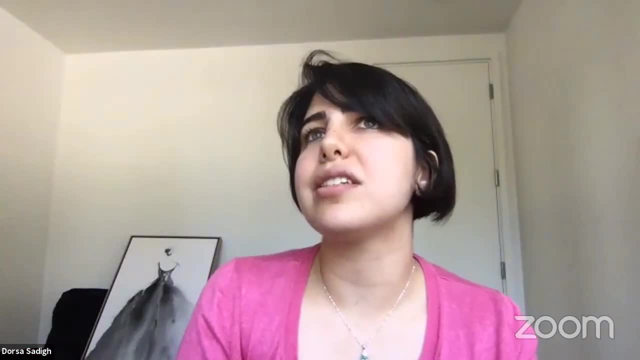 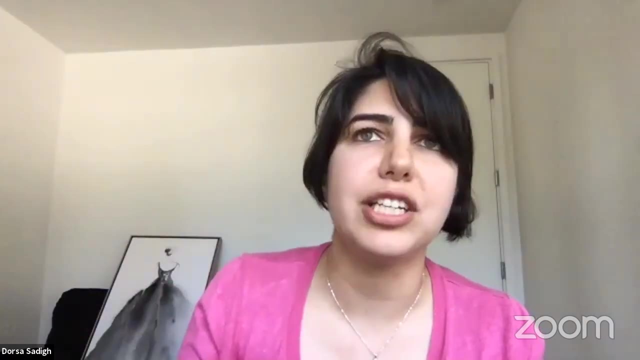 Yeah, yeah. so that's one answer. And then the other answer is like: maybe our behavior, the way we are treating safety, might change over time too, And it might not be as rigid as it used to be. Maybe we are not able to give guarantees. 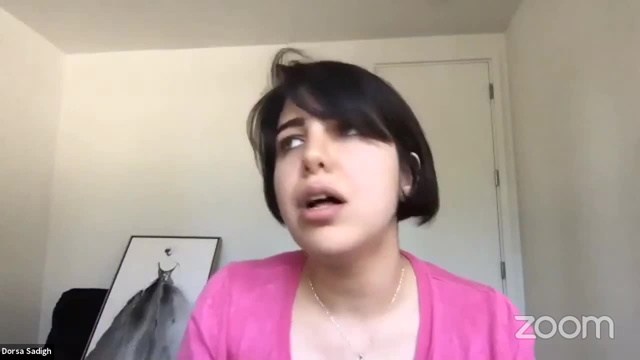 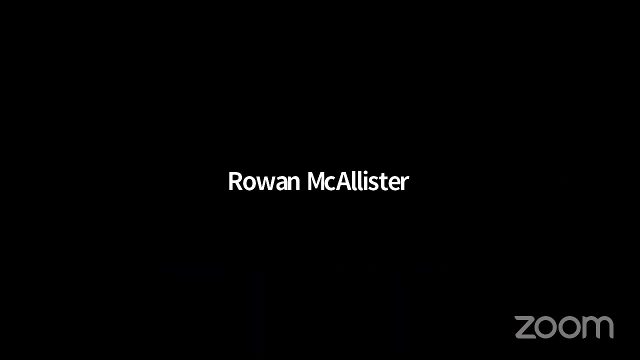 but maybe we are able to like self-diagnose and repair if things fail. So I think that could be a different view of safety that we start looking into more closely. Great, well, yeah. thanks very much, Delisa, for that really interesting talk. 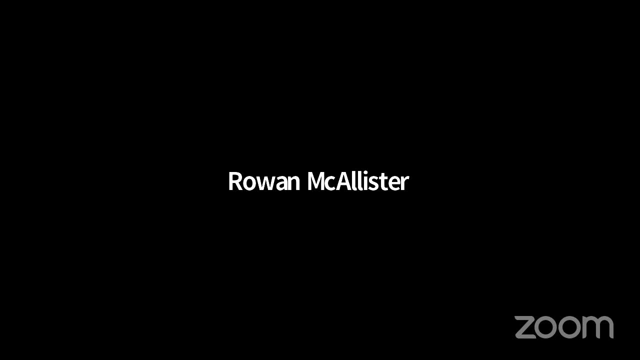 If anyone has any further questions. maybe, Delisa, if you want to hang around for a few extra minutes, there may be some extra questions for you in the chat. Yeah, so thanks very much, Delisa, And so we'll now move on to our second speaker. 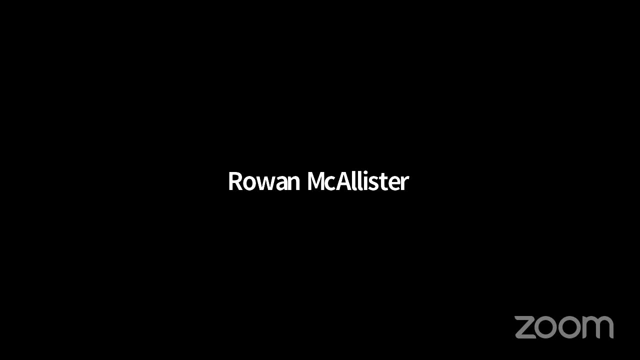 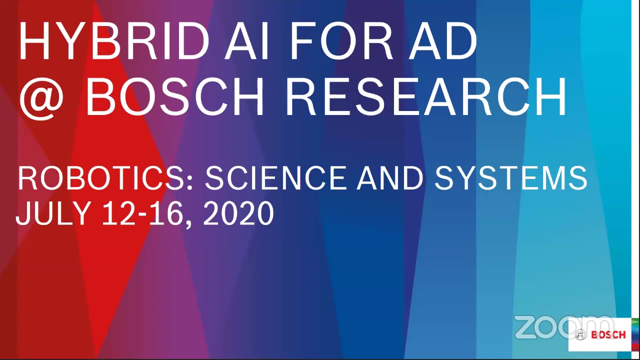 So our second speaker is Maxime Daldorff, who did his PhD at the Kohl's Institute of Technology, where he worked on stochastic control and control of microchips, And he's been working on the development of microchip systems. 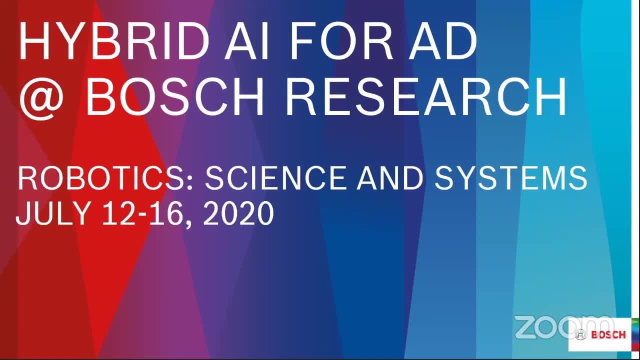 So since 2017, he has been with Bosch Corporate Research and works on behavior and motion planning for automated driving. His research interests are in imitation and reinforcement learning, especially in combining classical, model-based and modern data-driven approaches. So, Maxime, oh yeah, looks like you're sharing the screen. 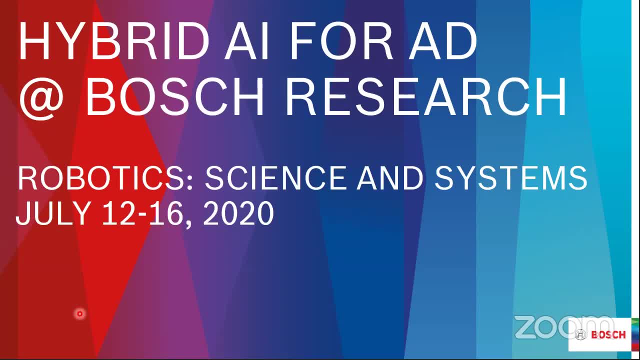 Great, And I want to thank you for your time, Delisa, And thank you for sharing your thoughts as well, and thank you for your comments, And I'll stop sharing my screen, So if anybody has any questions, please feel free to reach out to me. 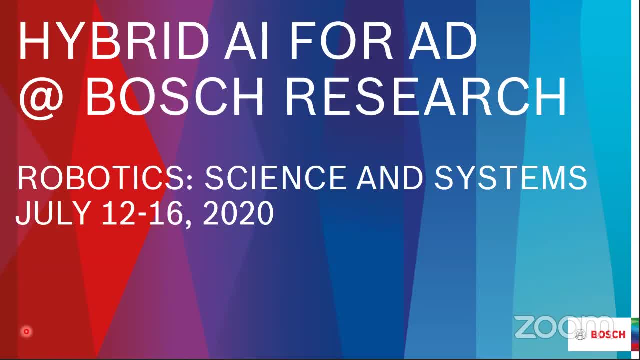 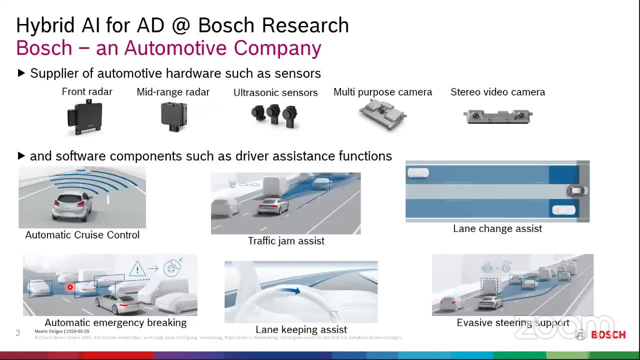 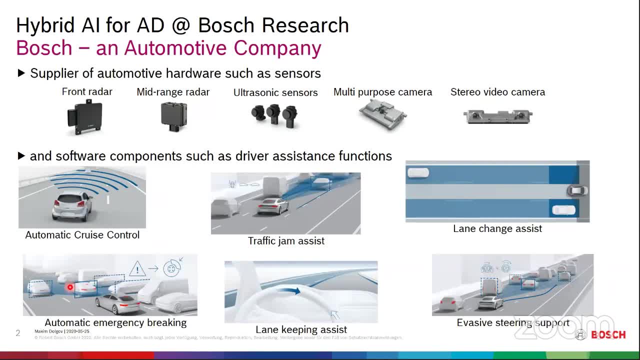 Thanks everyone. Maxime, you may be muted. still, We can't hear anything. in case you want to, okay, i thought i thought i was muted by you and you unlocked me. okay, now it's fine. now, now we can hear you, but you have to start again, okay. so yeah, thank you, um. 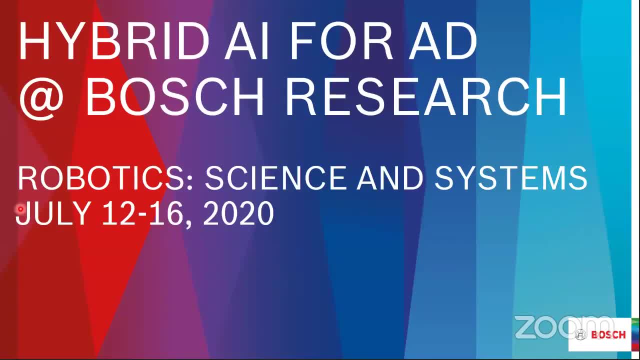 thanks for inviting me, uh, to a great workshop. it's a great opportunity to share with you what i'm working on and, um well, my talk would will be about, um, combining classical and data-driven approaches at bosch research. so, um well, when i tell people that i work at bosch, they usually 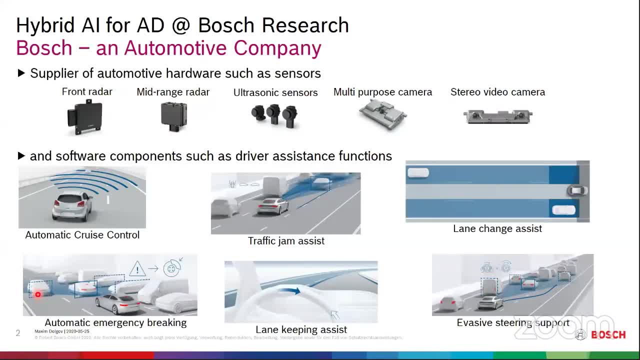 have coffee machines in mind and drills or washing machines. and what many do not know, that bosch is one of the major automotive suppliers in germany and we have a wide range of automotive components, ranging from brakes, injection systems to different sensors, for example radars, ultrasonic. 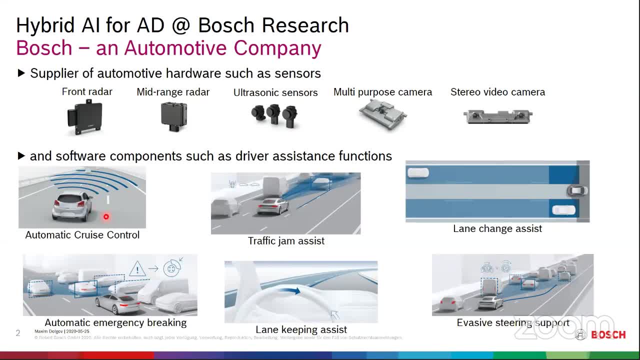 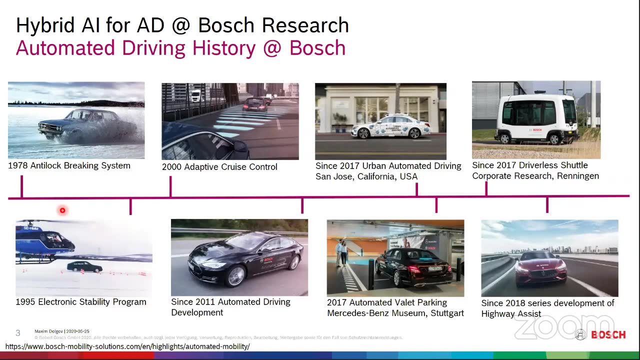 sensors, different camera configurations, and we also develop software for automotive automated driving and driver assistance and offer these functionalities to our customers also. what many do not know is that bosch has a long history of working on driver assistance. for example, the antilock braking system was invented at bosch and well, since 2011, we are. 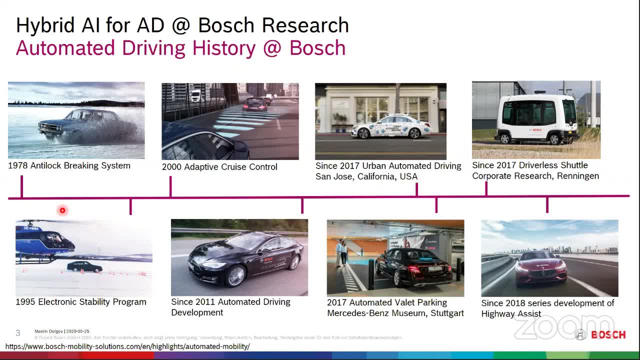 also working on automated driving, and the most recent projects are, for example, the urban automated driving project together with daimler, or the automated valid parking at in stuttgart- fully automated valid parking. then we also work on driverless shuttles for mixed scenarios where you don't have the structured road but rather a campus, for example, and since 2018, we also work on 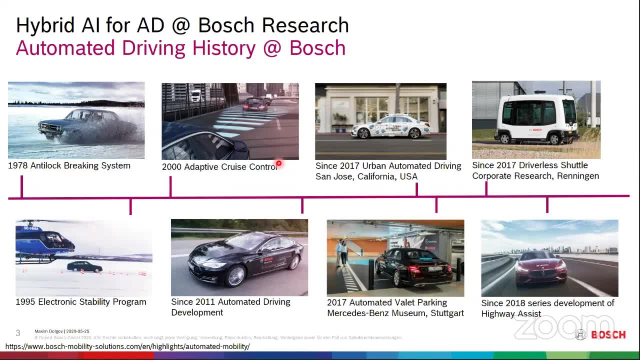 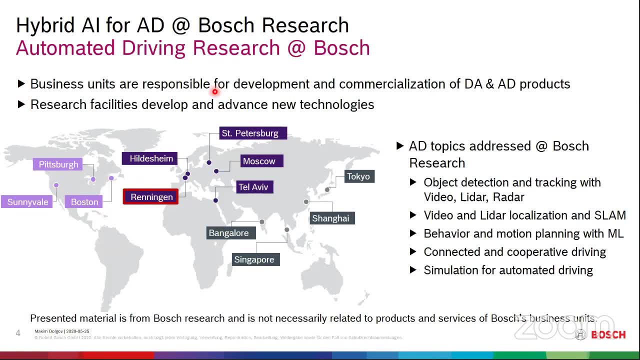 development of highway assist system. in my talk i will be presenting topics from bosch research and, due to this long history of being automotive supplier, we have a separation between development of products for our customers at the business unit and doing research in corporate research all over the world. so the research? 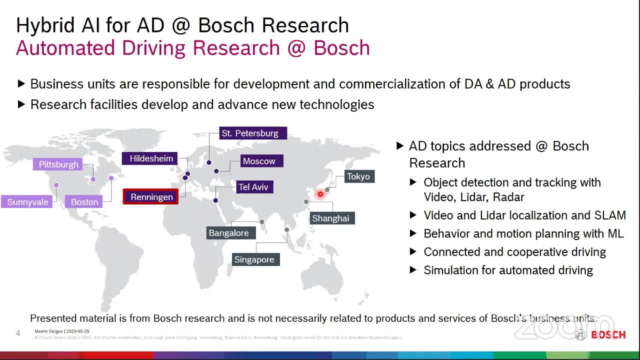 at bosch is not only limited to automated driving. we also work on topics ranging from sensors to metal alloys, ceramics, plastics and other things that we do, and we also work on the development of robotics, through quantum computing, machine learning to robots and automated driving and in the field. 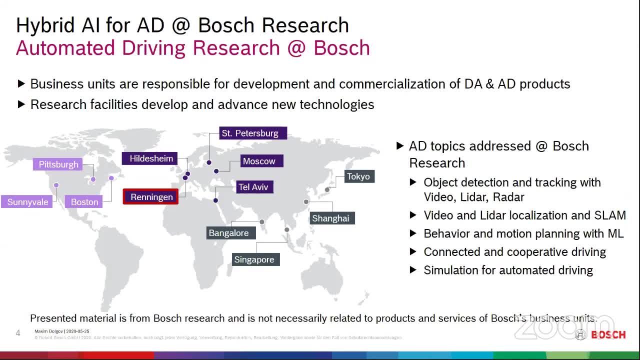 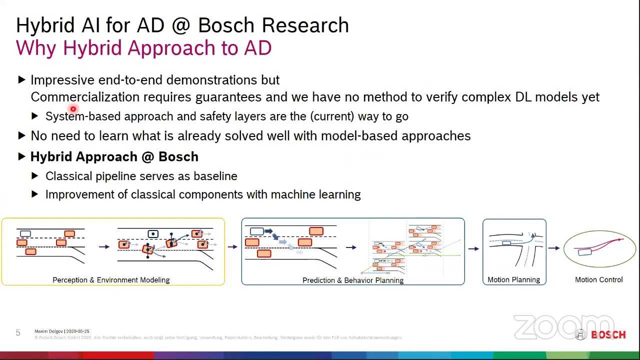 of automated driving. we work on perception and tracking system with video, lidar radar, also on video and lidar localization, slam, behavior and motion planning, connected driving and also sensing behavior simulation for automated driving. okay, so now why hybrid approach for ad? we have seen many impressive demonstration of end-to-end driving and also many learning-based. 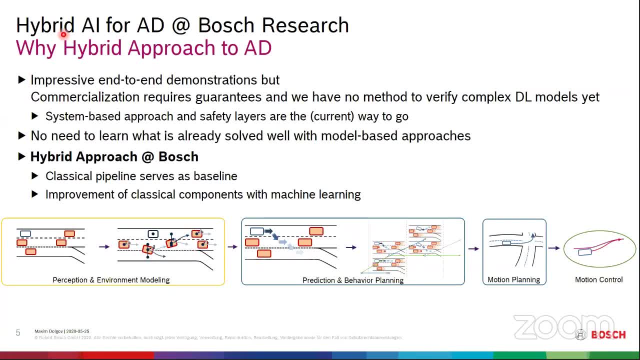 approaches, but if you want to commercialize such a system, you have to provide guarantees. so even if your end-to-end system is able to generalize over a wide range of scenarios- which is difficult by itself- you still need to have some sort of validation of the system. so we have a lot of 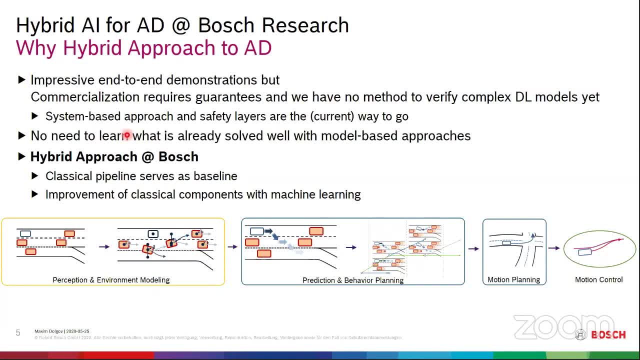 validation being provided for a system. and so, at bosch, and i myself personally think that this classical divide and conquer approach, where we can address one problem at a time, improve one component at a time and have this iteration loop of becoming better and better, is the way to go for. 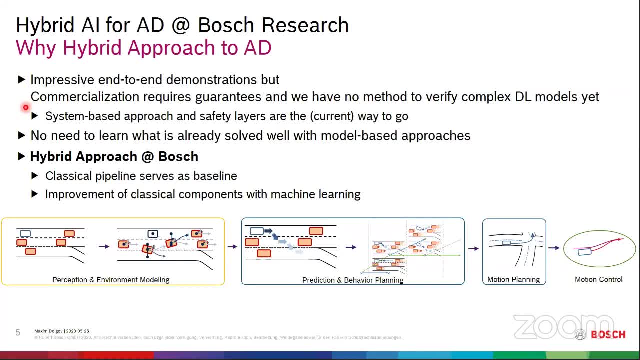 the first generations of automated driving. of course, you could argue why classical approach did not give us fully automated driving yet. so we're still in this phase where 2020 is here and we have no automated vehicles yet being rolled out for the public. so we have many. 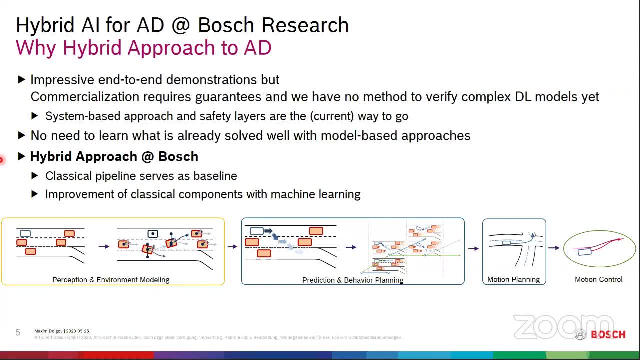 testings ongoing, but what is starting to get is we begin to have this classical pipelines being deployed and being improved, one at a time, with machine learning, and this is also what what we do at bosch research. so we have a classical baseline of a single processing pipeline with perception. 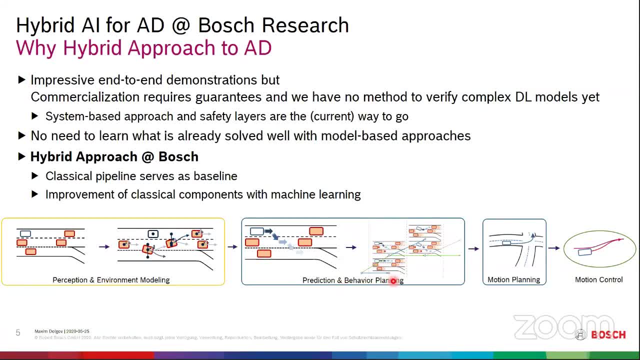 environmental modeling over behavior planning, prediction, motion planning and motion control, and we take one component at a time and try to improve it with data-driven methods in order to get it to the state where we can roll it out in public. and today i'm going to talk about having deep learning detectors that estimate uncertainties for classical 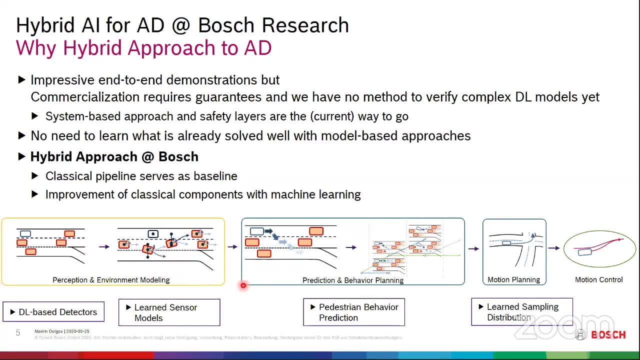 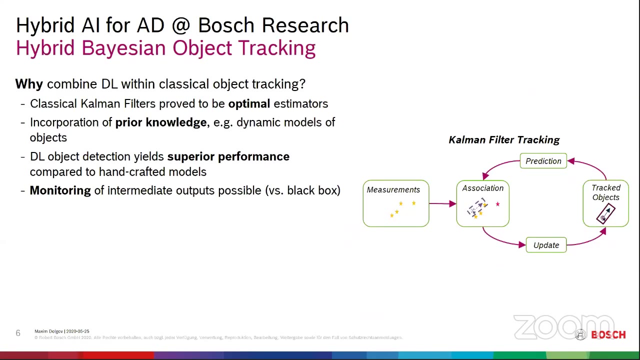 environmental modeling, learn sensor models, how we improve prediction by having pedestrian prediction being learned, and also learning sampling distribution for motion planning. okay. so why would you want to combine a classical tracking pipeline with a learned methods? well, common filters have been widely used in perception system. they offer a mathematically sound way to incorporate prior knowledge into tracking, such as: 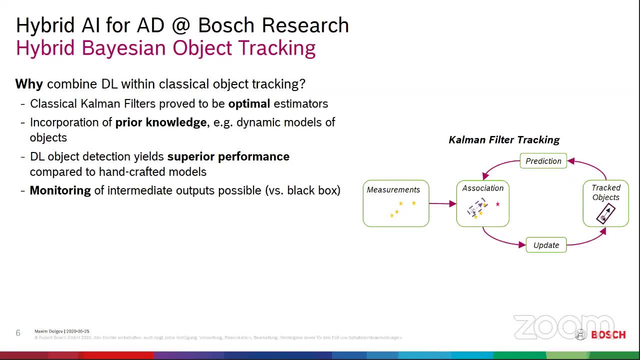 motion models of tracked objects. for example, you have different behavior for a truck and then a bicycle. also, you can incorporate the knowledge about the strength and the weakening of your sensors. so, for example, LIDAR provides you good position estimates and radar, on the other hand, can measure relative velocities and what you want to do in this classical perception. 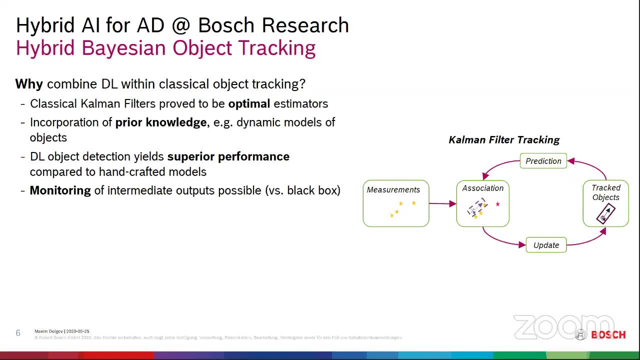 pipeline that works very well in the scenarios. improve it, just individual components of it. so, for example, if you stick with with detection, what you want to have is you want to incorporate your learn detection and to this end you need some sort of of uncertainty being provided with the 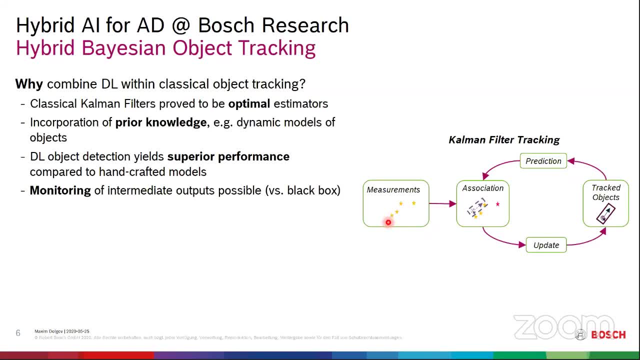 detection. the standard engineering approach would be to have this yeah, to assume an a certainty and then do filtering with it. or, if you have ground truth detection data, maybe you could tweak the uncertainty. but instead of, yeah, such an engineering approach, instead of tweaking to specific scenarios, what you want to have is having an estimate. 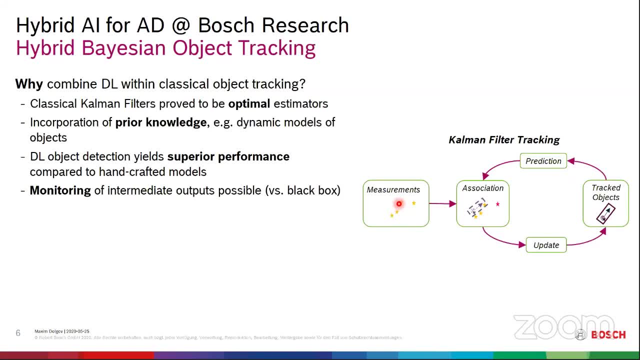 of uncertainty being provided together with your, with your detection, and this is something that we, for example, do with LIDAR detection. you can see here our approach developed by Dee Fang and our group is a PhD who is together with University of Ulm and he does detection of 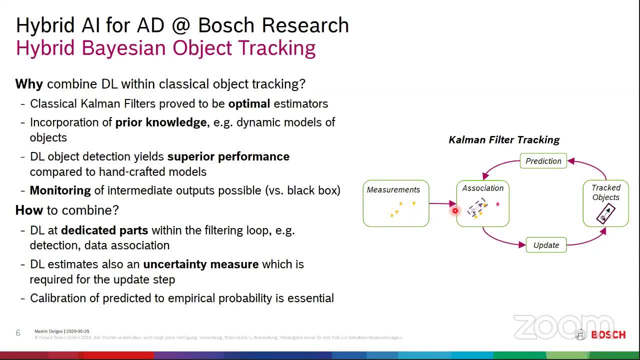 of objects in LIDAR point clouds. here are some examples from from a kitty data set. here you have the RGB image just for visualization and detection of objects in such a point clouds and what you can see is Dee developed a model that estimates uncertainty. it's depicted in a log scale. you have low uncertainty here, larger uncertainty here and if you look at 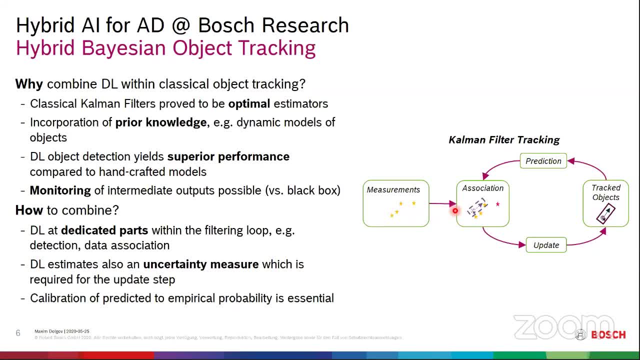 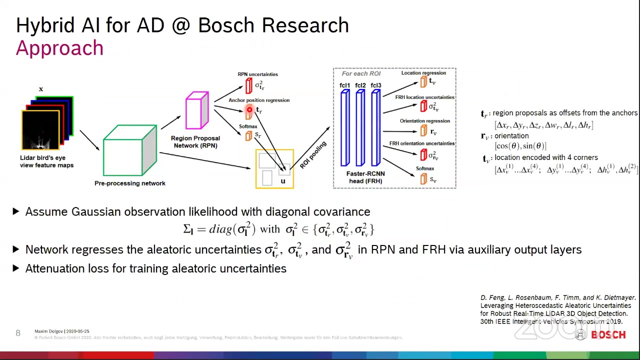 this bounding box is estimated by our models. you can see that the uncertainty gets larger when the vehicles are far away, or if you have inclusion so that you don't see the entire bounding box from the side, or if you have fewer reflections on the objects. okay, the approach that Dee used is rather standard in literature. we take our LIDAR birdseye. 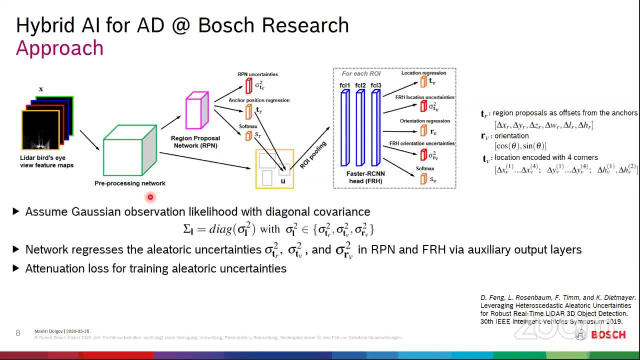 feature maps, feed them through a VGG16 pre-processing network, do region proposal ROE pooling and feed it through a file R-CNN had And in addition to standard output, where you only have denker, position regression and softmax of your bounding boxes and later. 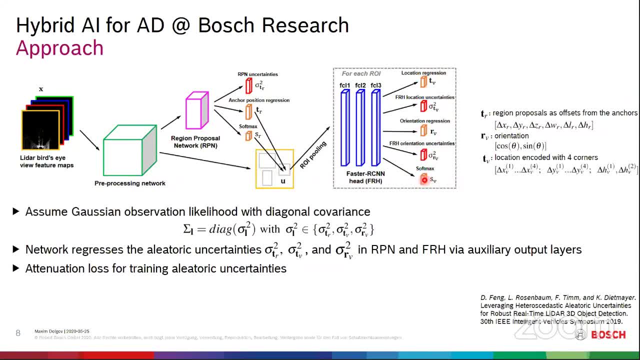 location regression, orientation regression- the softmax of your detection. he added outputs to consider uncertainties: your region proposal uncertainty, your localization uncertainty and the orientation uncertainty. In his work he assumed standard Gaussian uncertainty and was able to learn the result that I showed. 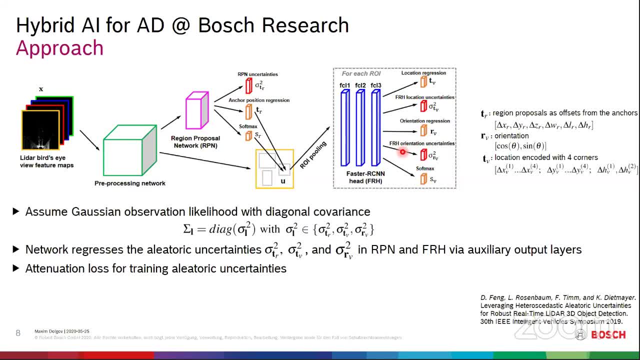 you And of course you could also assume non-standard uncertainties and having your model also predict the strengths and the weaknesses of your sensors. So again having different uncertainties, uncertainties in different directions of your sensor, So for example, the detection of the velocity, if you do it in tracking. 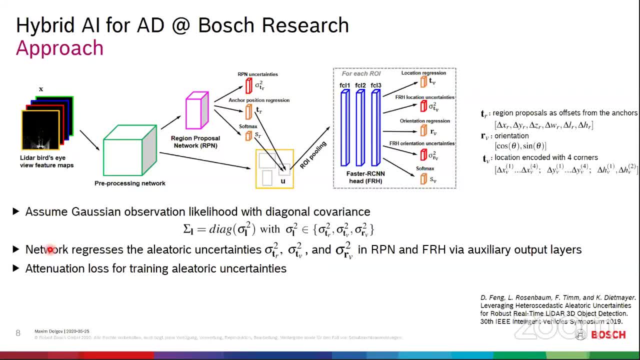 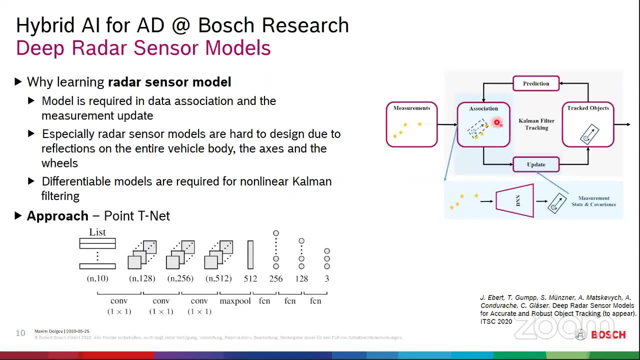 could have much larger uncertainty than the position. Okay, if we go further in our pipeline. what you also could improve in environmental modeling with machine learning based methods is having sensor models being learned from data. Well, usually what you have. so this is the work done by on deep 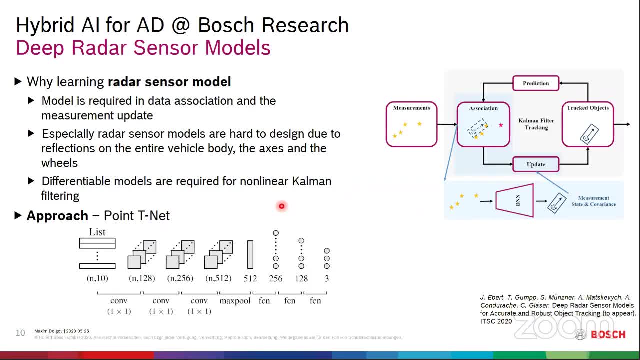 radar sensor models and it will going to be presented this year in the ITSC. the radar sensor models are quite challenging. So if you have a camera or a lidar or you have measurements from the surface of the radar, just know that that this radar here is not going to work successfully, So it's going to need 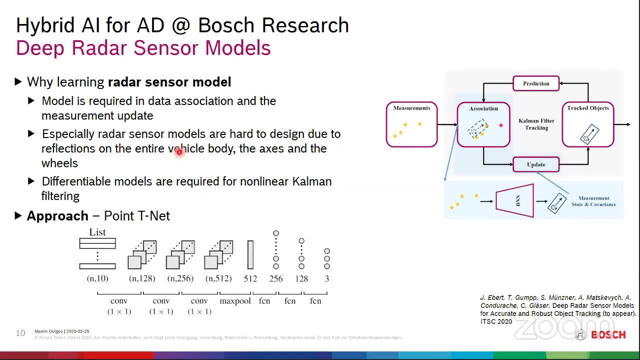 of the object. This is something that you as a human can grasp and you can tweak your covariances, But the radar is much harder for humans to grasp. You have reflections not only from the surface, but from the axis and from the wheels. 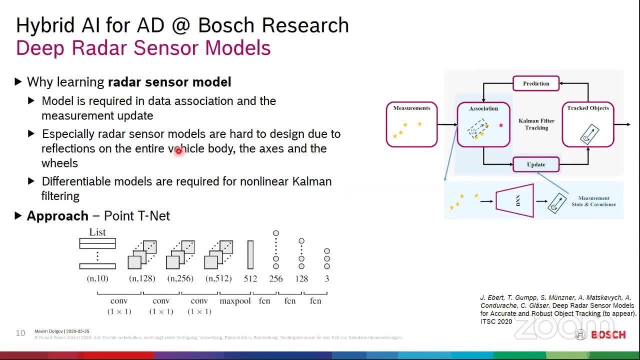 of the vehicle, And also you have the Doppler effect, multiple reflections and so on, And this is something that engineers try to come by with Gaussian mixture models, for example. But still, if you use some sort of engineered model, you have to address it with prior knowledge. 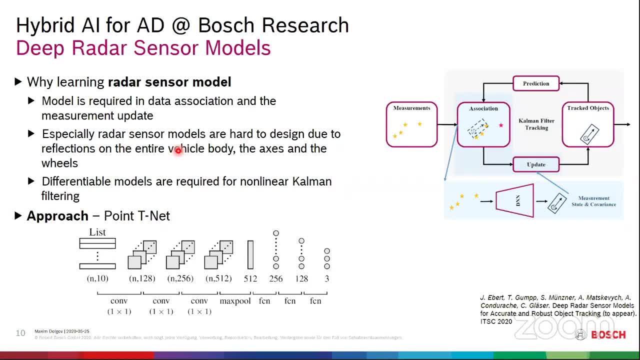 So you have to put into modeling your experience, where the reflections can occur, how many components of Gaussian mixture you need to add. And in this work we learned a deep model inspired by the point net from LiDAR perception, And the advantage was: 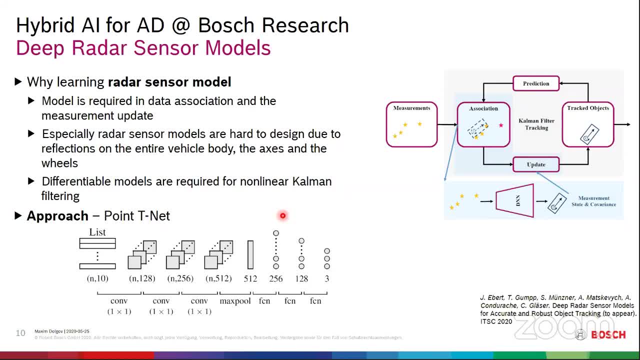 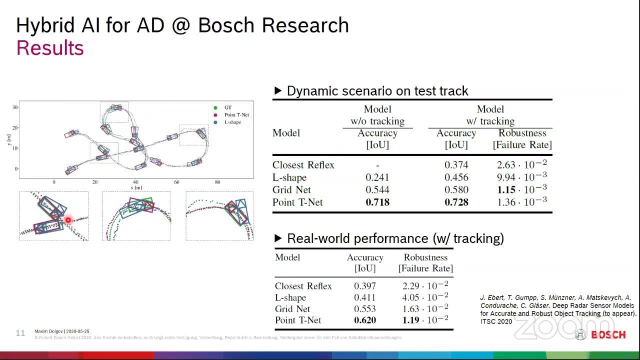 not only that we got better results, but also we have a differentiable model that can be seamlessly integrated with a Kalman filter After evaluation in this challenging environment on a test track that your standard radar-based automatic cruise control in your car would not be able to cope with simply because it is tuned. 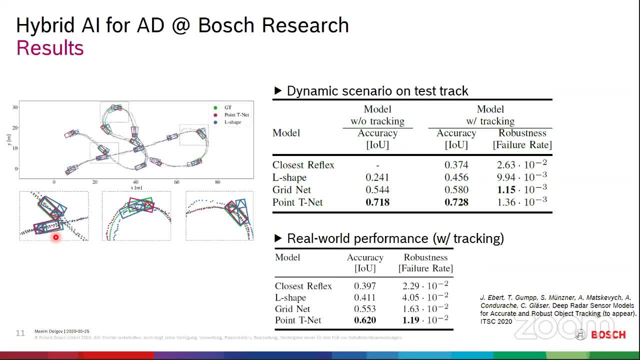 to curvatures That usually occur in the road and parallel traffic and so on. We could get superior results with a pretty simple setup, And this is something which also showed beneficial in our real-world evaluation. So, again the thing: you have a classical baseline and 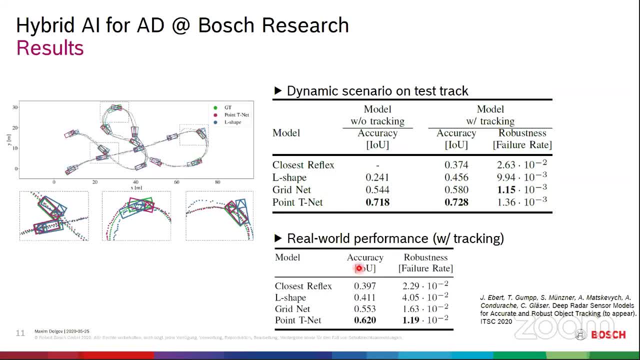 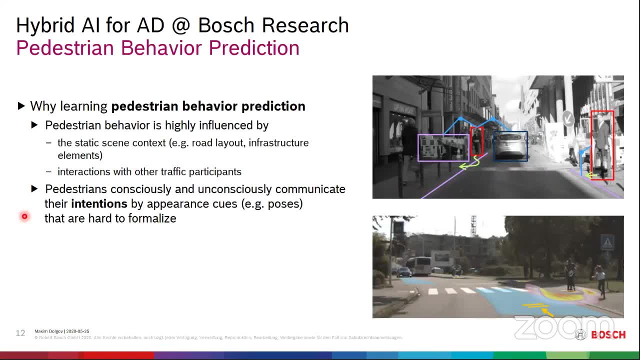 you improve one component at a time, And this is something that we can improve. So next, when we get further in our signal processing pipeline, we have a problem of prediction, And we heard already from Dossal that humans behave different with robots and you want to somehow to capture this. 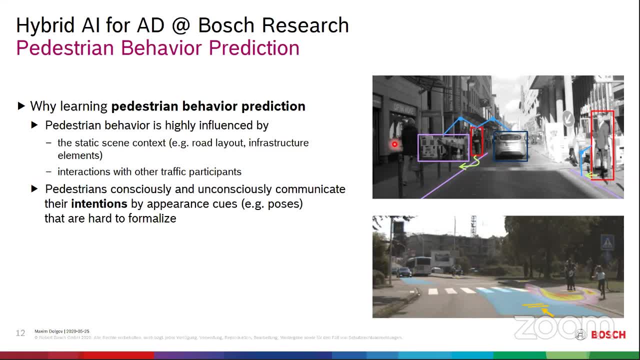 behavior of humans, And doing so with classical approaches is pretty hard. Pedestrian behavior is influenced by many contexts, by the context in the scene. So, for example, if a pedestrian sees something on the other side of the road, he would cross it. 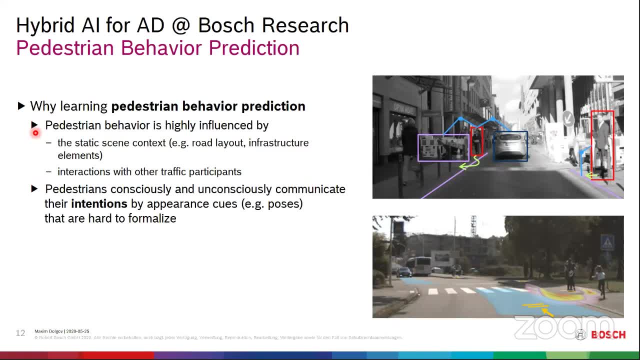 So you have to infer intent. Also, you have interactions between pedestrians themselves, Like this child here which runs on the sidewalk either on this side or this side of the standing. human And pedestrian also implicitly communicate with each other, which you can hardly capture with classical models. 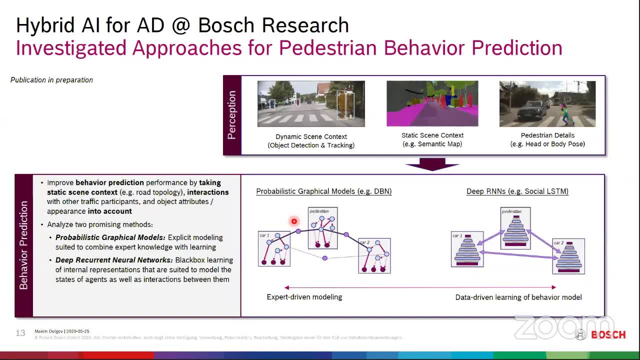 Thus, in our improvement of pedestrian prediction, we looked into different models, where you go from expert-driven modeling with probabilistic graphical models to more data-driven approaches with RNNs. This is work in progress, so just a small teaser here. What we used in this work was dynamic scene context. 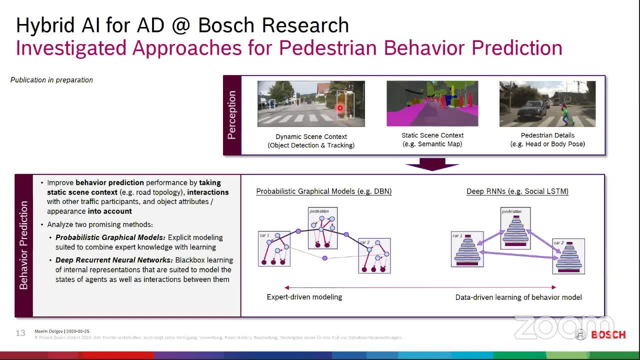 so the detections of our pedestrians, detections of the cars, semantic information and also post-estimation from pedestrians And from our results we got that probabilistic models allow you to capture to be pretty robust. But when it comes to performance, data-driven approaches, 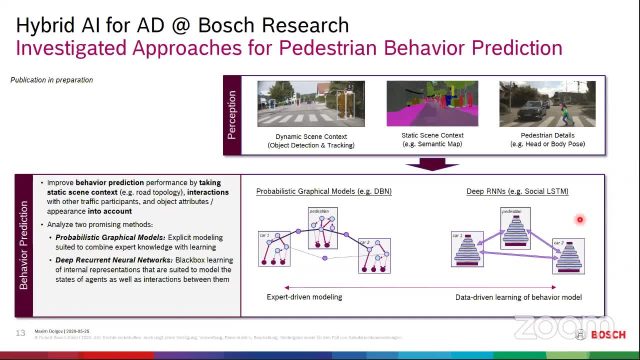 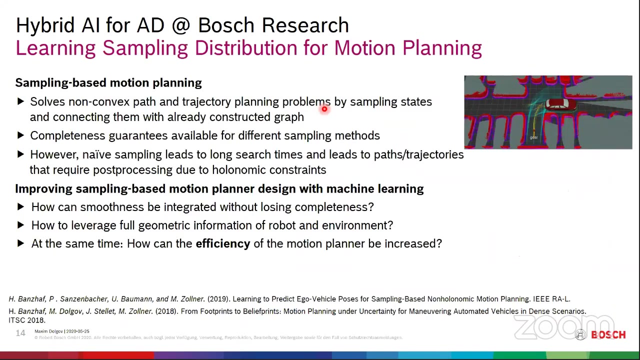 are way better, at the cost, of course, of maybe failing in some scenarios where you want to be good. So maybe the way to go is having both of them in your model and switch depending on the context- Something different that we also address further. 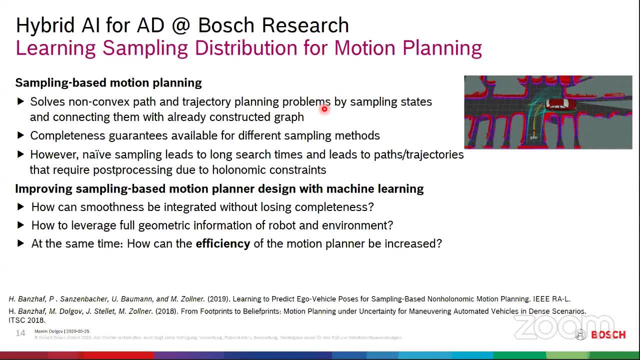 in our signal processing pipeline where it comes to motion planning is learning sampling distribution for motion planning. Okay, so here we consider a maneuvering example that we use using sampling-based motion planning, simply because you can address non-convex problems like taking the other way of a blocked road. 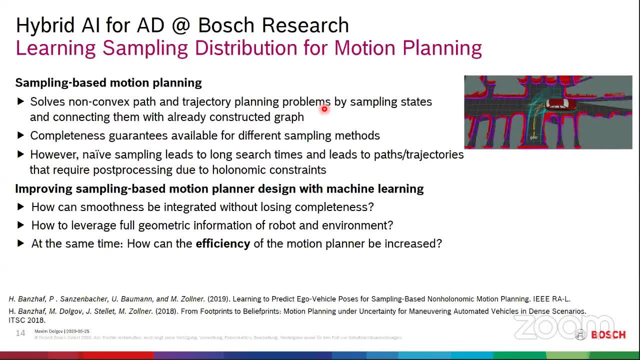 And this is something that is difficult to solve with optimization-based approaches, And you also have nice theoretic results like completeness, depending on your sampling methods. So there are strong guarantees that for different sampling strategies you may have, almost surely- you're almost surely- being able to find a solution. 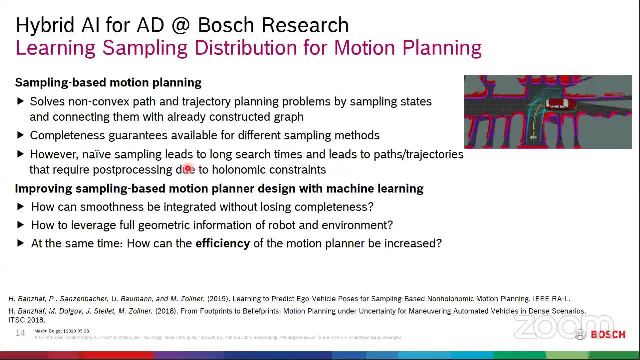 But when you take a naive sampling approach, you have to do post-processing In order to get smooth trajectories for the controller, or the naive sampling approach may take too long And this is something that may pose a problem when you try to roll out the system. 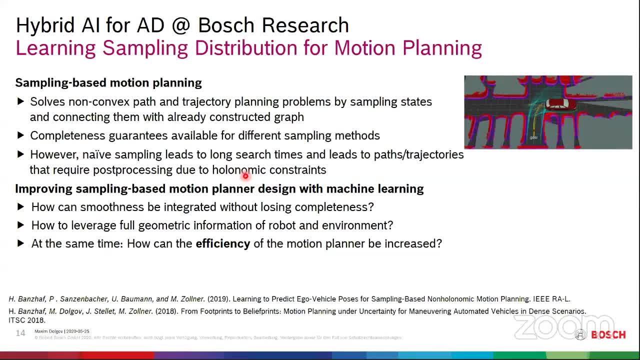 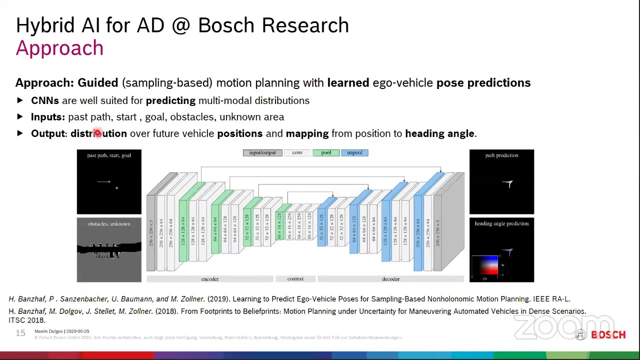 And exactly here we can help with machine learning approaches where you improve the sampling of new poses which you then can add to your search graph And search with classical approach. Kim, this is work done by Holger Banzhaff, who also works at my group. 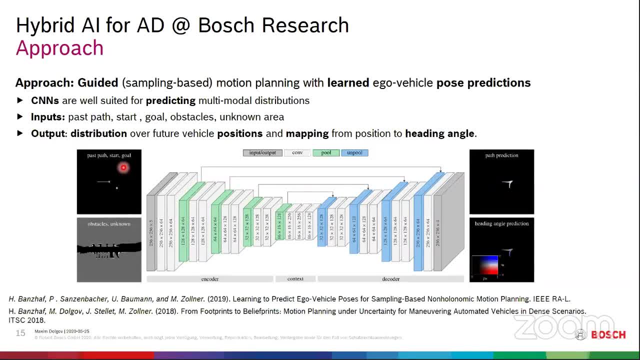 And what Holger did was to train a CNN to output a distribution of future positions of the robot and also the angle. So by the robot I mean a vehicle here with a CNN that gets as an input the past trajectory of the vehicle, the goal and the obstacles. 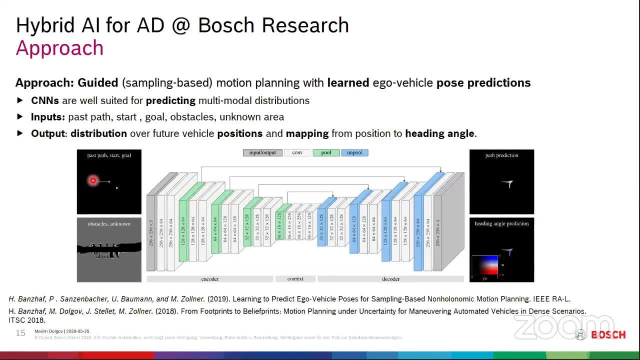 and the unknown environment as a grid map. Maybe let's take a look at this video here. On the left side we have a bidirectional RT star with orientation-aware state exploration And on the right side we see our models And if you look closely, 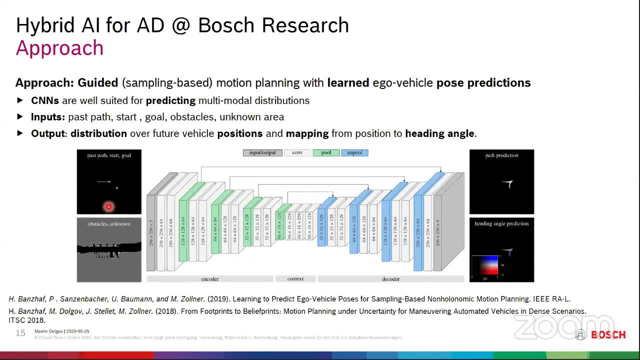 so the trained model is able to find a solution much faster here in this scenario than the classical model. If you look also at the path, you can see that the maneuver is more human-like than the maneuver which is found by the classical algorithm. These are: 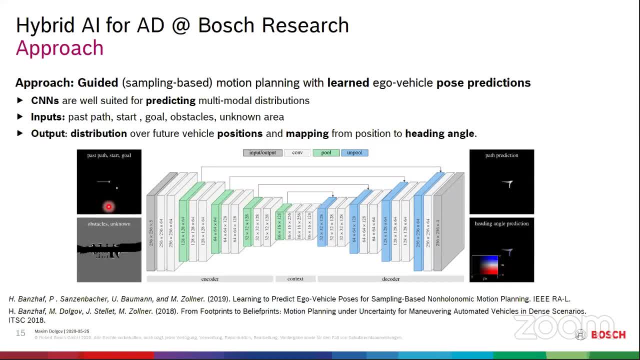 the samplings. here the grid map, the environment and the path that is driven by the vehicle is depicted in green. So here you see different sampling distributions output by the CNN in our experiments And you can see that the model is much faster. 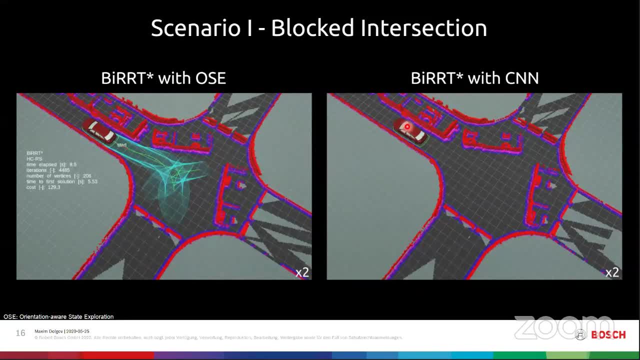 than the classical model. Okay, another scenario here. This scenario is actually pretty good for a classical approach without machine learning, But nevertheless we did not train on this scenario and still the learned approach was able to output a nice trajectory. So what I want to advocate with the talk: 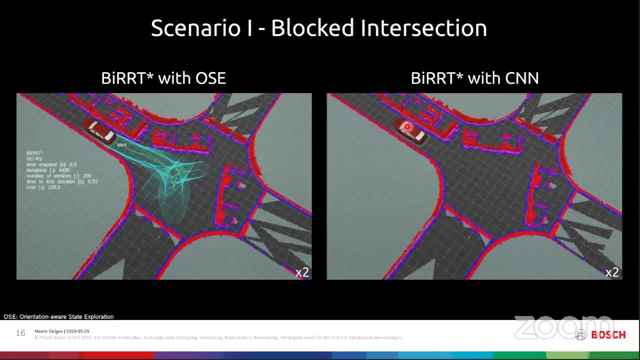 is that there are components in the system that are reasonable to learn and then components that are not reasonable to learn, And in this case, RT star is already a good conventional method that you do not have to relearn. You can already benefit from just improving it. 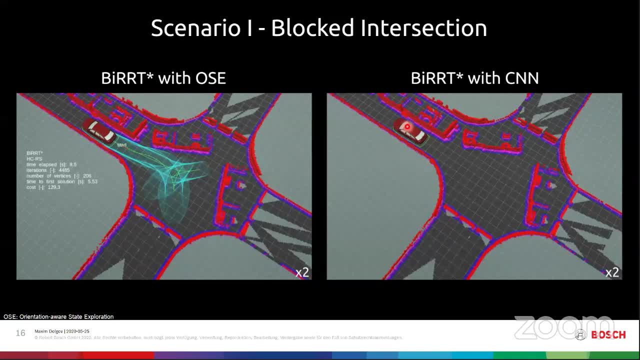 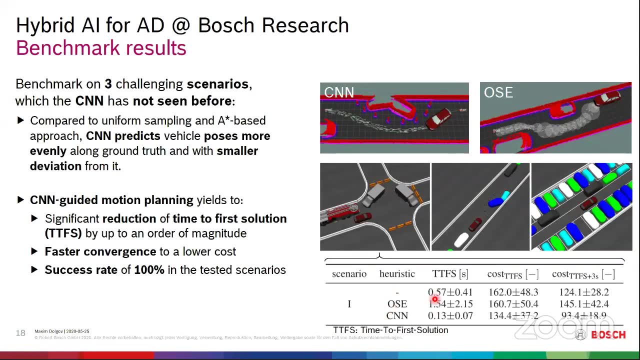 with machine learning, with little data, with guarantees of your classical system, And this is also something that we got in our results. So the CNN guided motion planning was able to reduce the computation time significantly. We had faster convergence at a lower cost. So if you assign a cost function to a motion planning, 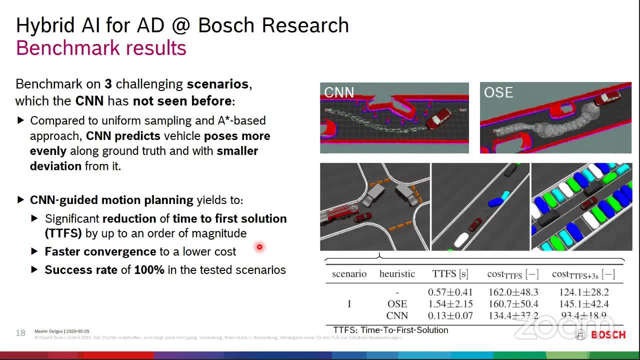 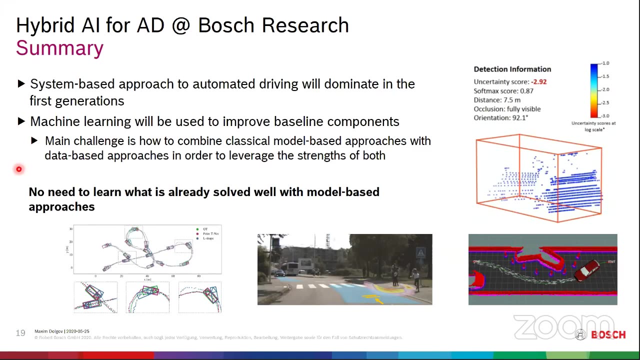 and compare the classical results with the CNN supported results, you get lower costs And also, we didn't lose anything on success rate, even in scenarios that we did not see. So let me summarize this. So what I want to advocate- and this is also my personal opinion- 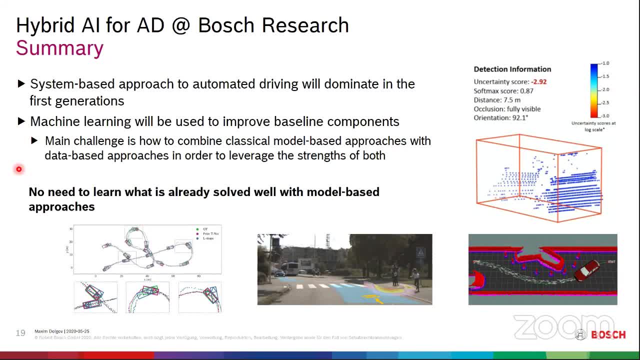 is that system-based approach to automated driving will dominate in the first generations. We need to avoid to learn things that are already done well with model-based approaches And what we do. what we have to do when it comes to automated driving is we have to produce robots. 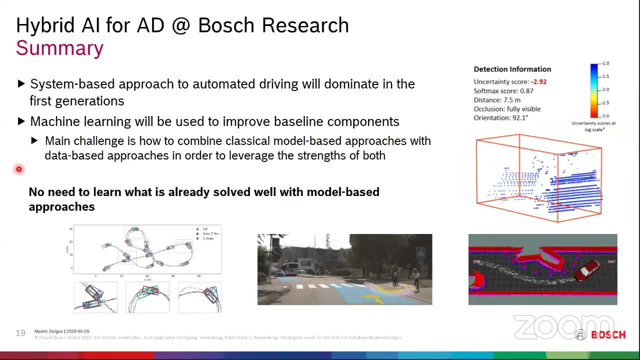 where you can understand what is going on. Maybe we will not get this human-like behavior as advertised or as expected by people, But we need to be performant enough, we need to be predictable and we need to be safe, And I think we can also expect from humans. 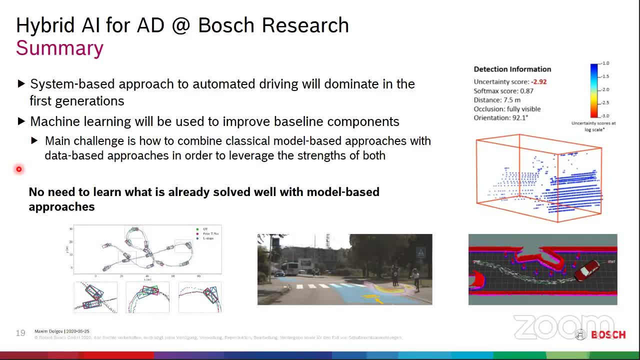 that they will adapt to the robots on the road. And maybe it has to be this iterative approach where we do not roll out robots that are capable to deliver human-like driving, but instead we start small, have specific scenarios where we have automated driving. 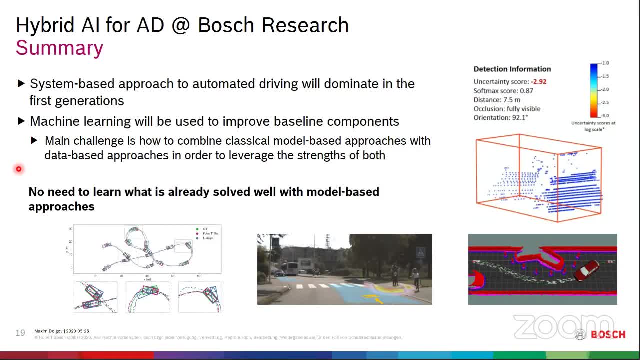 for example, in the highway, maybe on rural roads or suburbs, and then people will start to get used to robots, will learn from it, will adapt their behavior and we will have a much easier challenge to solve. Okay, thank you. 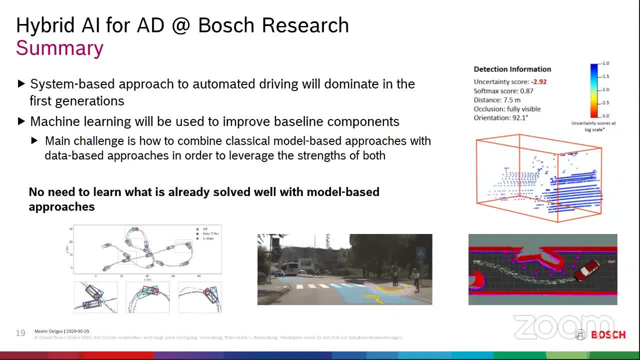 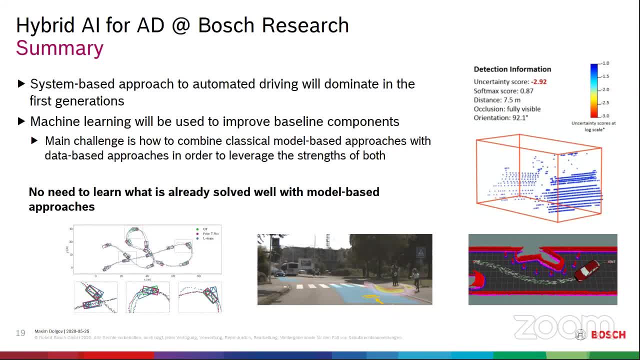 into the group chat and we can all see it and I will read it out so everyone can hear. So yeah, actually, maybe I can go first. So, Maxim, you talked about these architectures that you use for LiDAR and also radar. 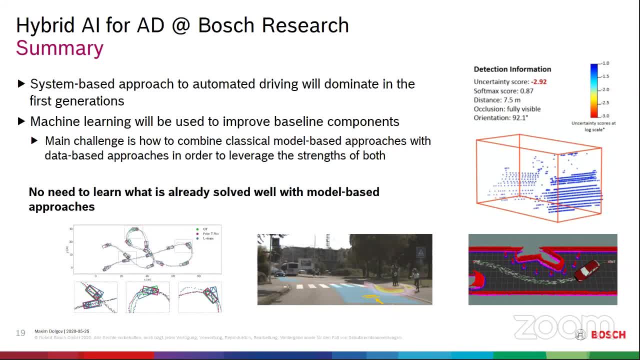 Have you ever kind of combined them both, like in case a vehicle has both of them? I mean, are you able to integrate both of these sensors operating at the same time in a way that could potentially give benefits more than either one of them alone? 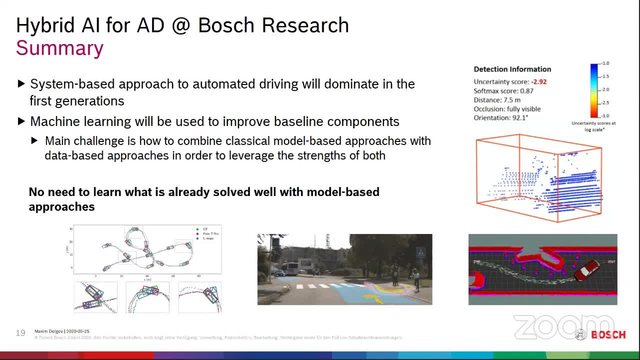 Yeah well, we have currently a project going on that combines them and bring them to the road. The colleagues already integrated LiDAR and video and radar would be the next step. And also, we not only have just this classical pipeline, we're working on learning the tracking itself as well. 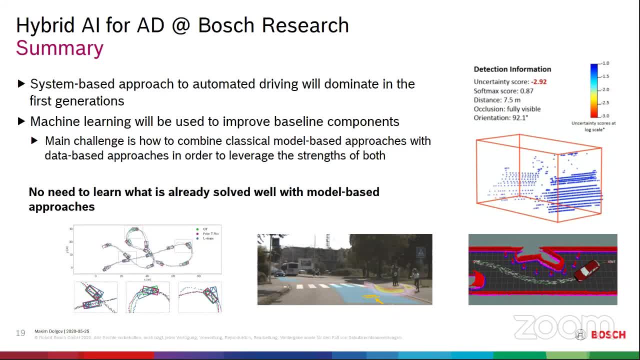 And this is something where you get robust results and you're also able to do ablation studies. You can switch one of the sensor modalities off and see how well the others still work. being in a learned environment, you will use your classical models as a fallback. 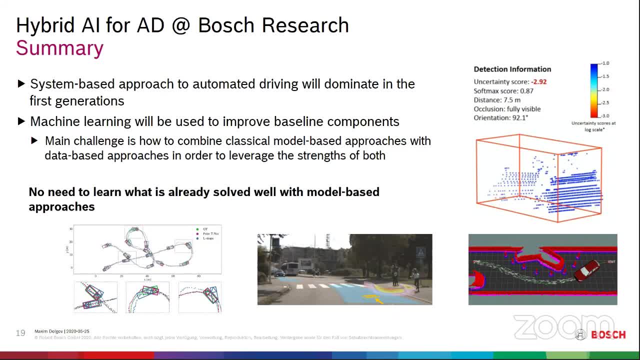 This is something that you can only do if you have individual components, if you have a framework where you can exchange one component at a time. Okay, great, Yeah, thanks. Okay, we've got a new question coming over the chat from Salah. 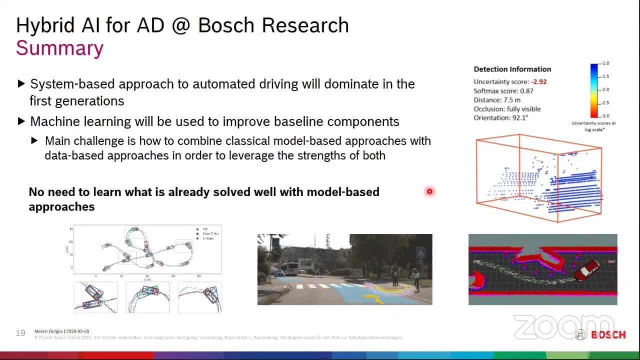 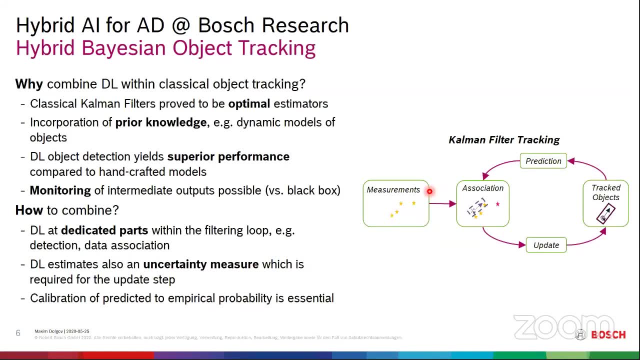 So Salah says: thanks, Maxim. Could you clarify how the Kalman filter was integrated with data, The data-driven DNN approach? Yeah, Okay, so usually what you get from your deep model is a detection of an object, maybe some sort of regression of the state. 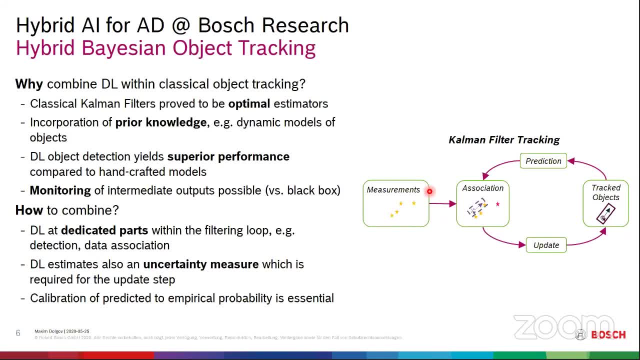 And then the question is how to integrate this detection into a Kalman filter. You need a model of your target. You need to do measurement association. So if you have multiple tracks and you want to know from which of the tracks the detection comes from, 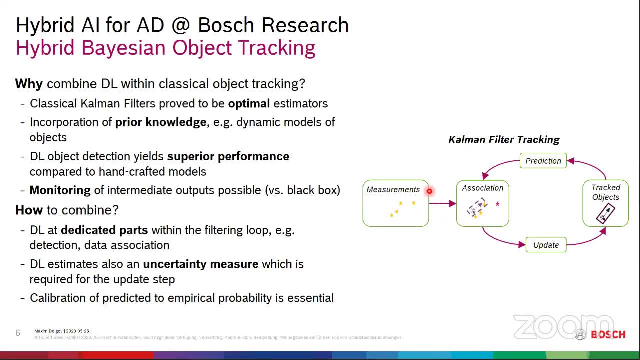 you need to do some sort of data association And the Kalman filter uses this update loop where you iterate between update and a prediction And in classical approaches you have some sort of a sensor model that gives you the update metrics, the measurement metrics. 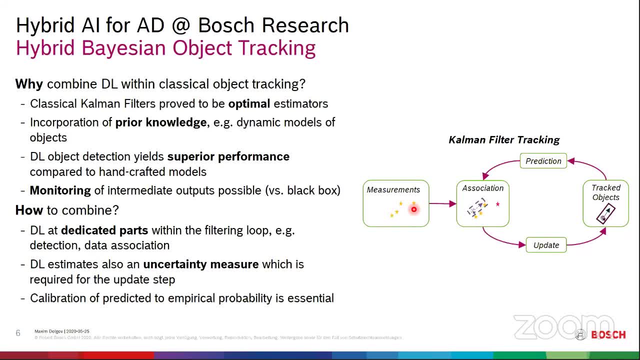 And you also have a model of your noise, depending on the object that helps you evaluate who you trust more: the measurement or the prediction model- And in this approach with LiDAR, we focused on having this uncertainty being provided by the model as well. 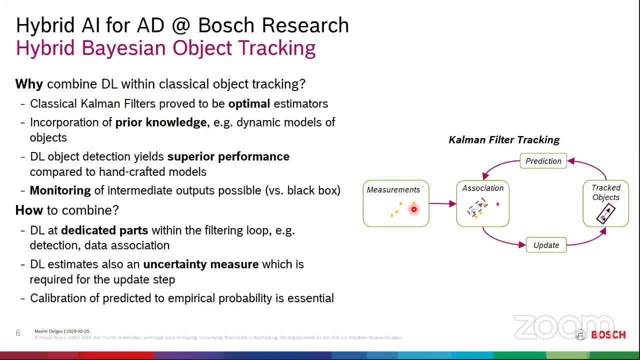 So you would still have a measurement model that is engineered And for LiDAR detection it's just the position of a bounding box in the simplest case and the size of the object. But then you want to be able to assess. do you trust the LiDAR detection more? 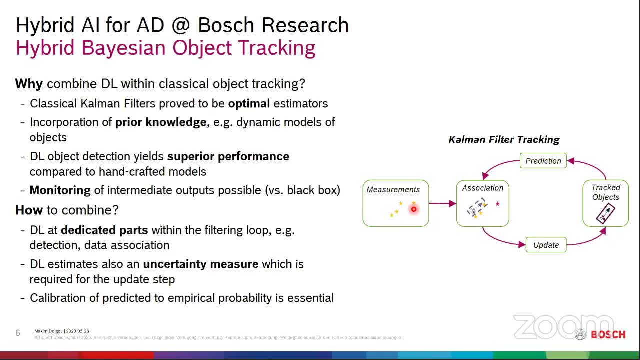 or do you trust your prediction more? And here is where the uncertainty measure helps. So if you look at this slide, you have quite good estimates. in a reasonable range from your vehicle, You would trust the LiDAR detection And as soon as it comes to cases, 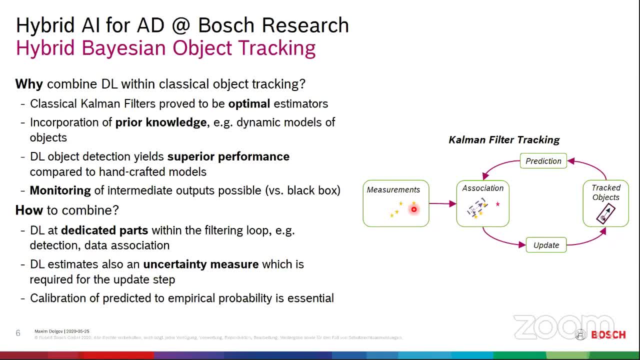 where you have occlusions or the vehicle is too far away, you would start to trust your model more, But it's okay, because these vehicles are usually far away and do not pose this. you know threat right now And they are not that critical for your planning. 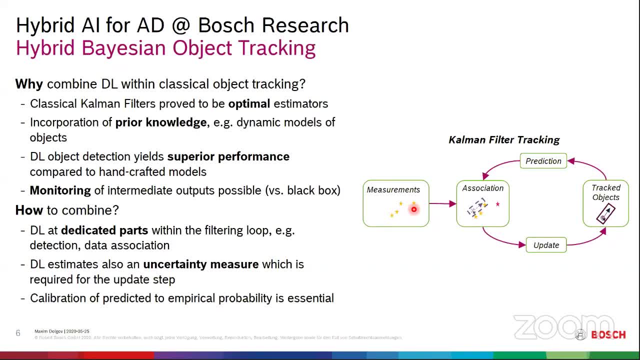 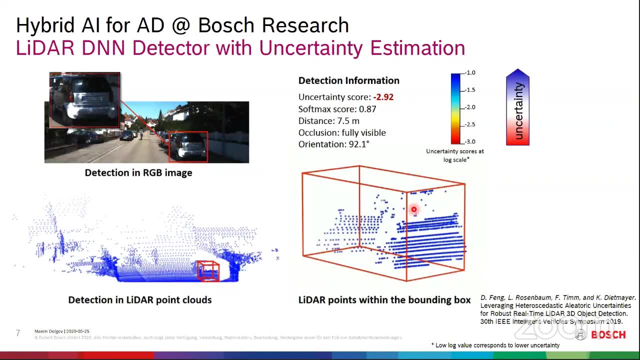 So, for example, in this detection here you would assume a model and just yeah, have still an improvement of your detection, of your tracking, but relying more on the model that you have and not the measurement itself. Yeah, Okay, great. 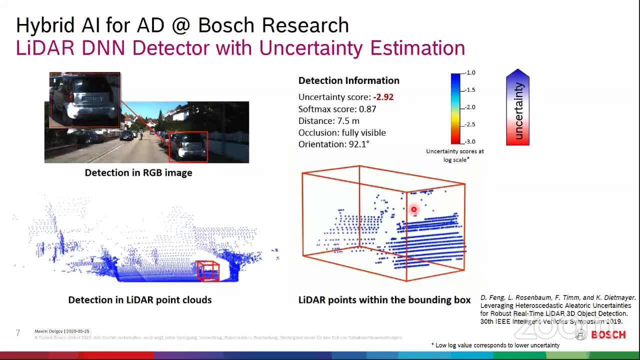 Thank you, We've got another question. So how is the tracking performance in the presence of occlusions Mm-hmm Okay? so yeah, it depends on what model do you assume If you have, for example, a constant velocity model? 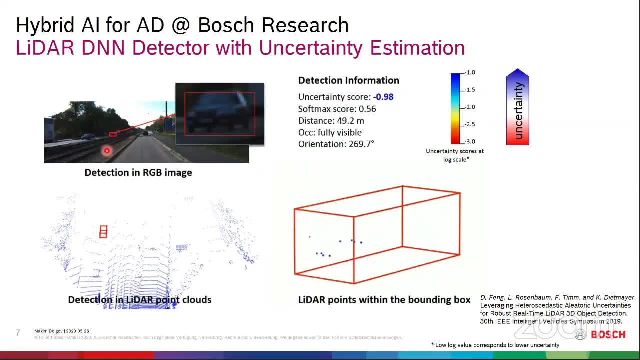 and the behavior of the vehicle matches your model assumptions, you have pretty good tracking And if your behavior, the behavior of the object, doesn't match the model, you get worse tracking. But usually it doesn't matter if you have objects that are too far away. 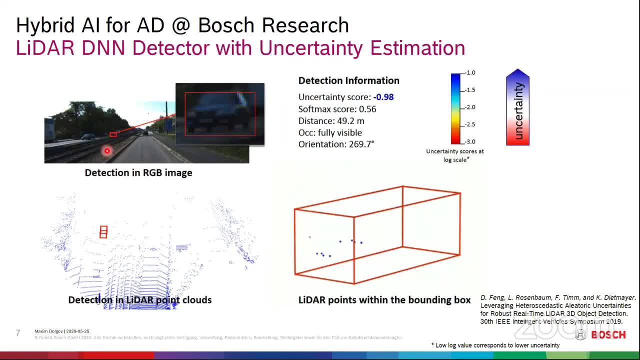 And near your vehicle where tracking is critical. you usually have additional sensors that can help, For example, the radar sensor that may not only be able to see the vehicle in front of you, but can see- yeah, some sort through it due to reflections from the ground. 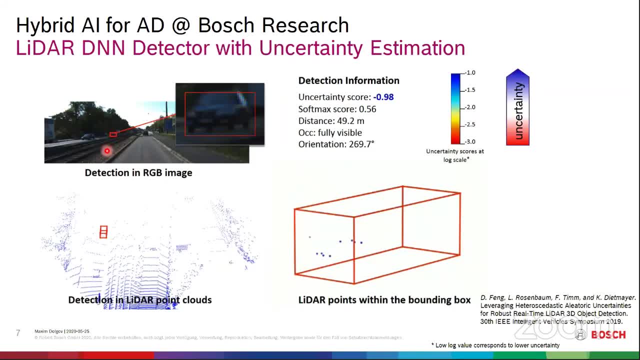 And well, this work here was especially targeted towards having this- the model, the detection and certainty- being output. We didn't analyze its influence on the tracking performance, But in our current integration project that we also will publish soon, we have scenarios where traffic is pretty good. 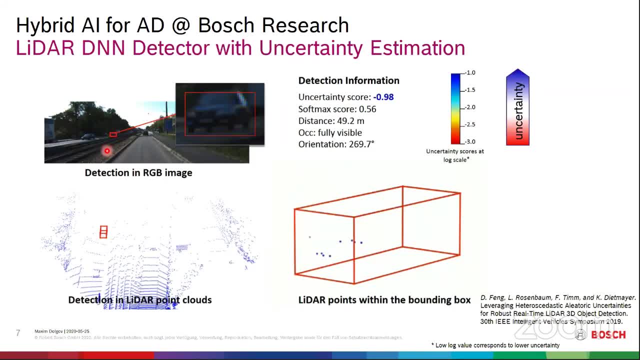 Okay, so I cannot provide specific numbers, but the model itself is critical, And you can see it with humans as well. So humans have really good models when it comes to occlusions to objects, And this is something where we can get to by. 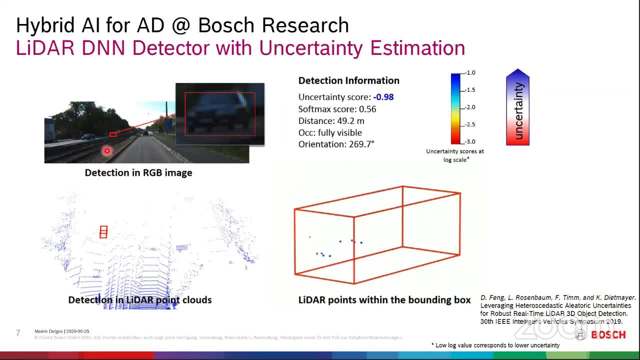 yeah, also learning prediction models for the Kalman filters. Okay, great, Yeah, thanks, Thanks again. All right, If there's any more questions, feel free to type them into the text box. the chat in the next minute or two. 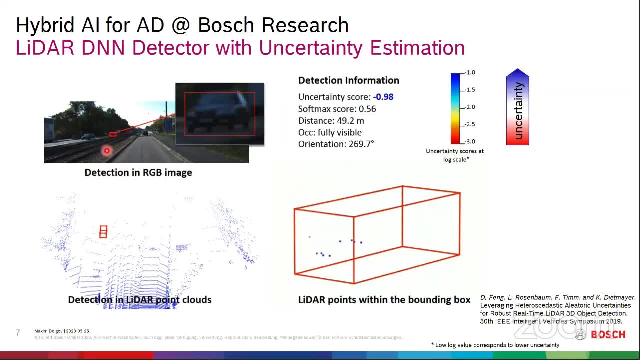 We're running a few minutes ahead of schedule, So we've still got a bit of time. So if you have any other questions, please feel free to put them in the chat box And then we'll move on to the next slide And then, in a few minutes, 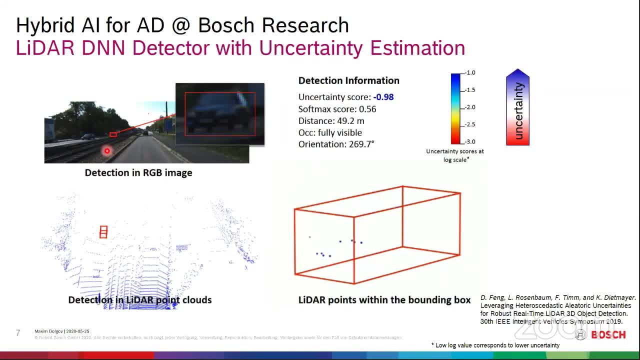 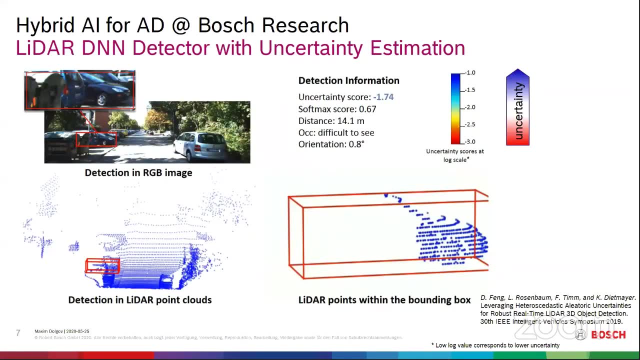 we'll move on to the contributed talks section. So we have four contributed talks And then we'll move on to the next slide, And then we'll move on to the next slide. So we have four contributed talks coming up. So the way this works is. 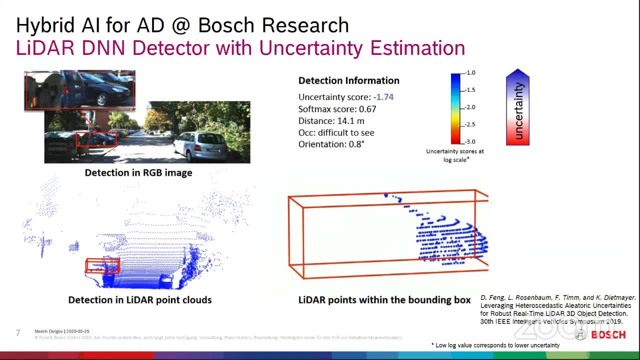 everyone has provided a three minute video which I will play from my machine here And then the author will be present here to answer any of your questions live, which is again just through the chat functionality, So that you can just type anything you want into this. 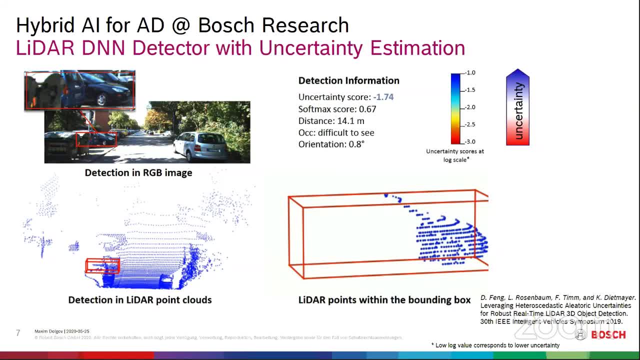 And then we'll move on to the next slide. So if you have any other questions, please feel free to put them in the chat box. So we'll move on to the next slide, And then we'll move on to the next slide. 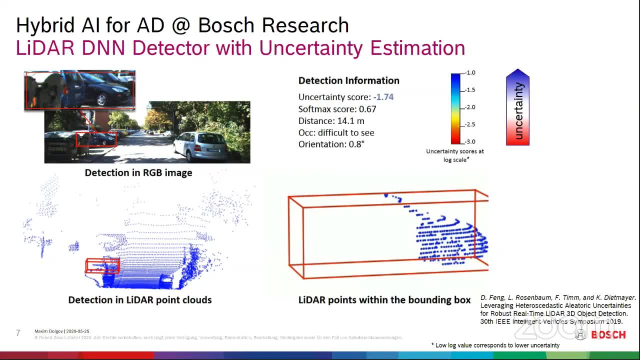 So the way this works is: everyone has provided a three minute video which I will play from my machine here, And then the author will be present here, And then the author will be presenting his or her question live on the chat box. So we'll move on to the next slide. 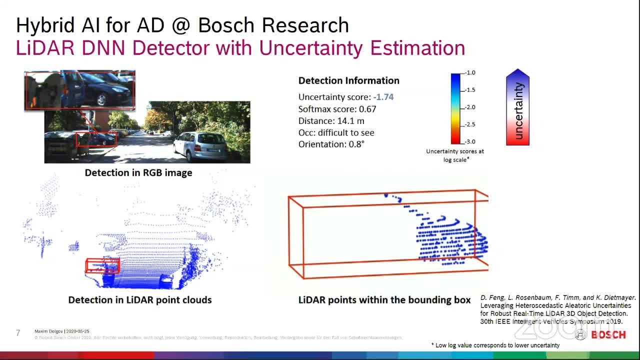 as opposed to trying to improve them with a data-driven approach. Okay, thanks for asking. Well, if you design a robot that you want to commercialize, you would probably have a very performance layer, which is for good scenarios, and have multiple safety layers. 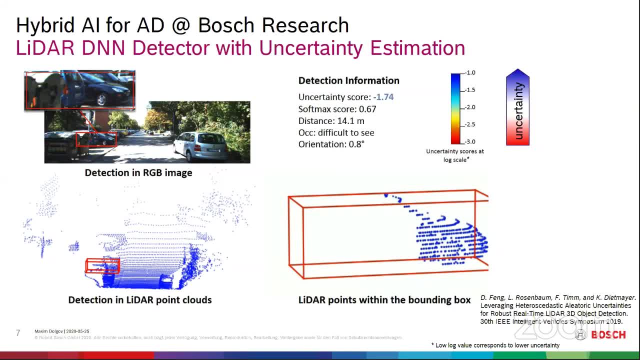 And I would prefer to have some of these safety layers being based on classical approaches, with maybe triggering conditions that are set to very close ranges, where you have little time to react, where maybe a pretty hard braking is acceptable And Well trying, of course. 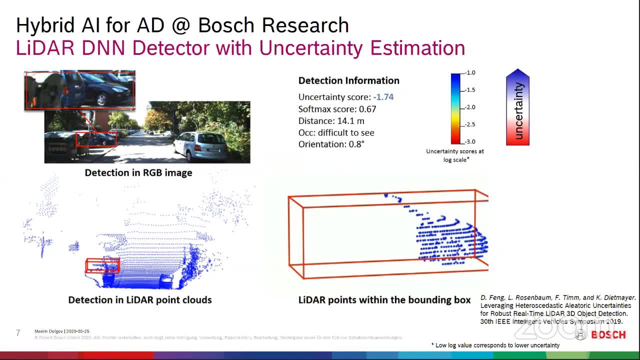 to avoid the situation with classical approaches, with approaches that are data-driven but still have classical approaches in the loop. Okay, great, And there is a question from Igor. What do you think the role of radar is in autonomous driving? How can it be better integrated? 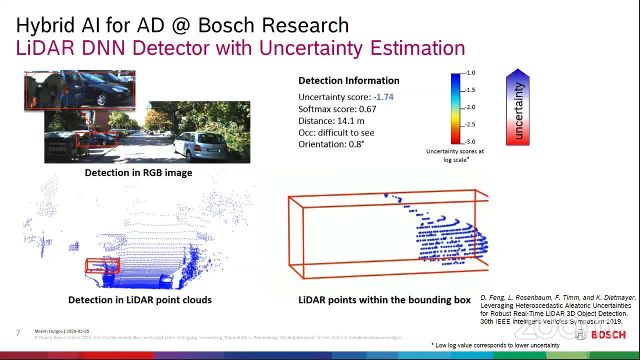 with existing perception approaches? Yeah, okay, Thank you for asking. So many classical driver assistance systems like automated cruise control are based usually on radar And we have seen that current approaches in literature and also what you, what you also get to see- are heavily based on LiDAR or video. 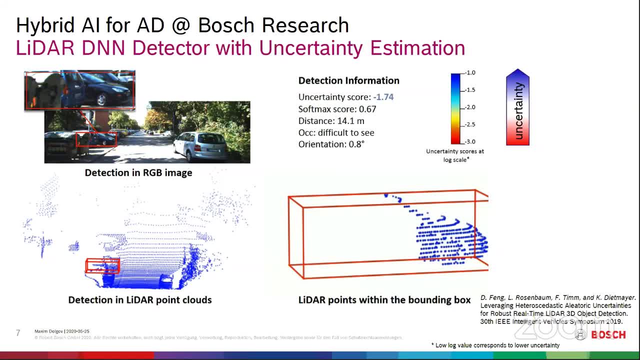 But I think radar adds a functionality that complements the weaknesses of the other two sensor modalities. So with a radar you can see in the dark where what is, or in the fog. that is pretty difficult to use with video, Or you have that. 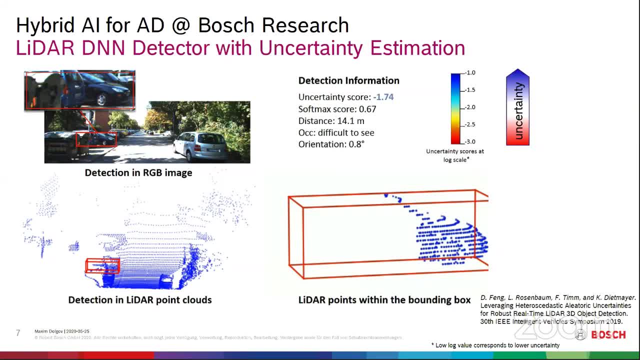 you have the advantage over standard reflection-based LiDAR, not the wave-modulated LiDAR, where you have velocity of the object being measured as well. And in order to be able to better integrate with classical approaches, I think you have to improve the radar as well. 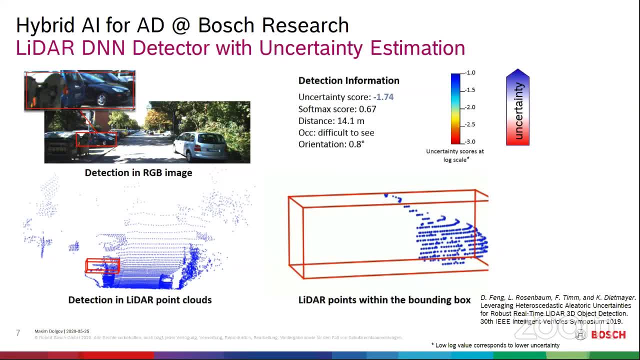 So when people think about radar, they have usually a single reflection in mind. And when people think about radar, they have usually a single reflection in mind. And we are in radar development already at the point where we can do, where we have multiple detections per object. 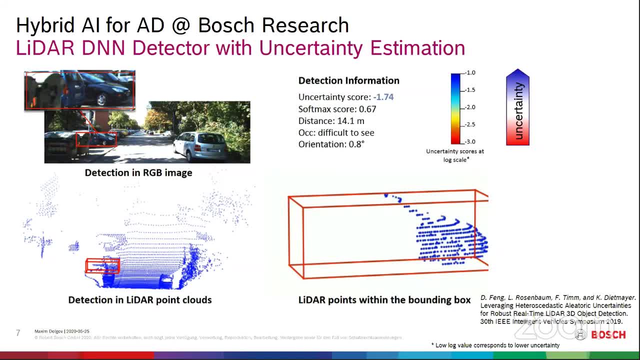 And this is something that is still hard to model. So standard approaches do a mean of this reflection, So take the one that is closest. And what we use for what we need for a better integration are radar models, Where we explicitly can do extended object tracking with radar. 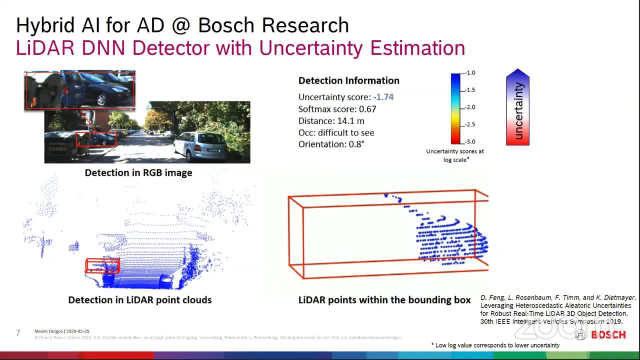 And as soon as we have these models, as soon as we have such an extended object tracking based on radar available, radar will be maybe on par with LiDAR and video as an additional sensor modality that you can heavily rely on in automated driving. 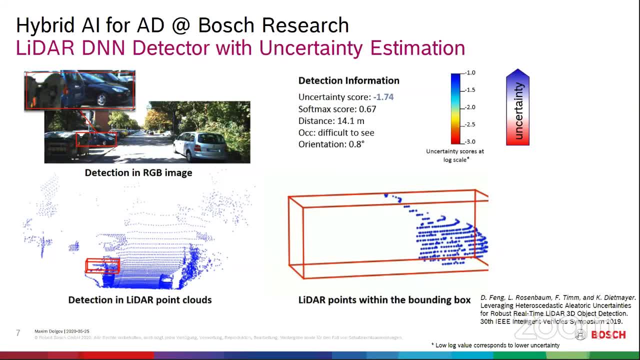 Great, Okay, Thank you. Okay, that's time, And so, yeah, thanks very much, Maxime, for joining us and giving us such an interesting talk. Thank you for the invitation. Okay, so, Maxime, if you should be able to stop sharing your screen. 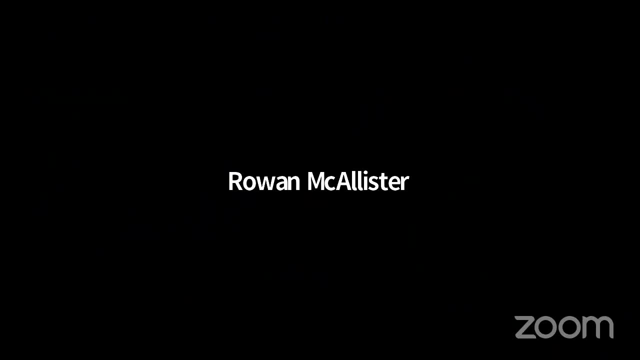 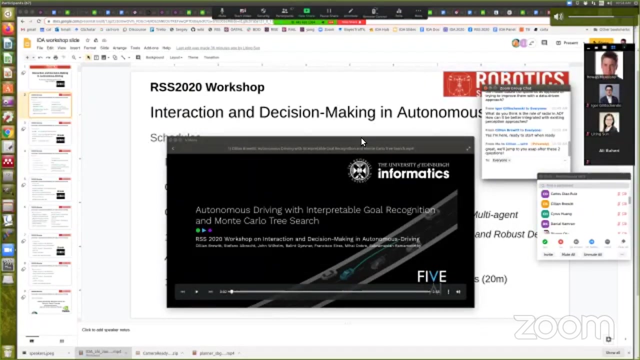 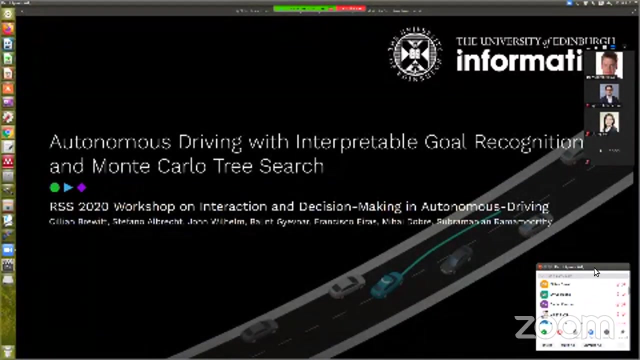 and then I will be able to start: Yeah, Great, thank you. Okay. so here we have a talk by Cillian Browett on autonomous driving with interpretable goal recognition and multi-colour tree surf. I'm going to present our 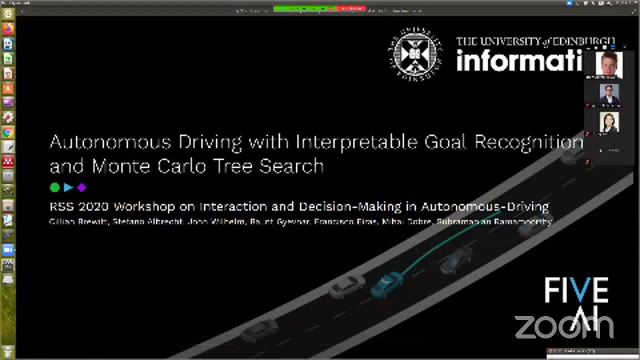 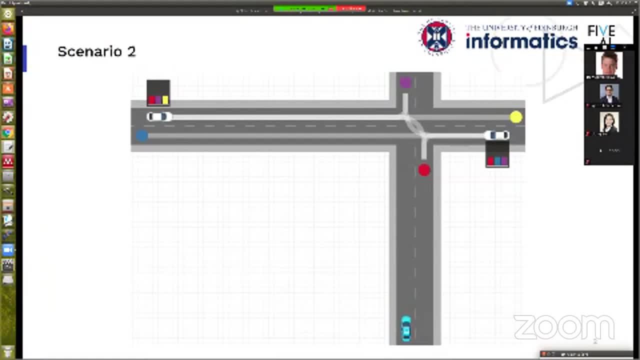 My name is Cillian Browett. My name is Cillian Browett and in this talk I'm going to present our interpretable planning and prediction method for autonomous vehicles. Prediction is an important but difficult problem. Accurate prediction can dramatically improve the performance. 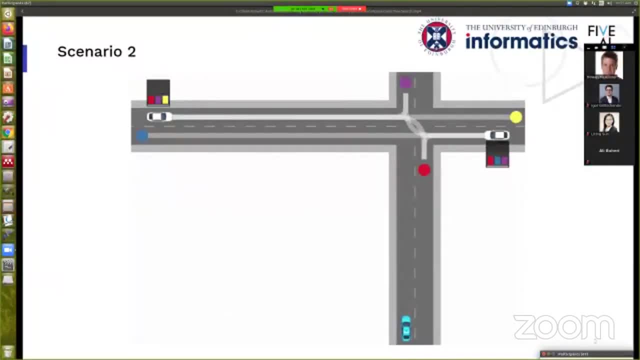 of autonomous vehicles, but the predictions must be fast to compute or based on limited amounts of information, and the actions of different road users can be highly coupled and interactive. Ideally, we want planning and prediction to be interpretable, and our system achieves this through rationality principles. 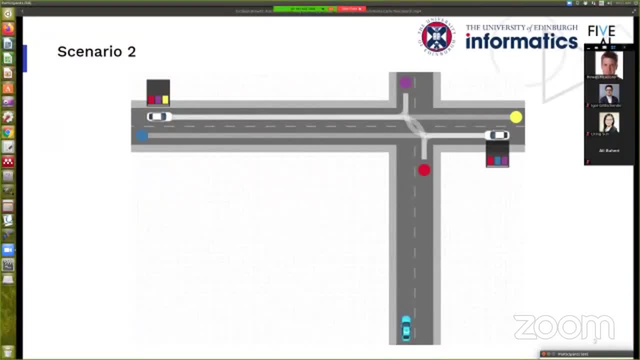 Take the example shown in this slide. Our car, the blue car, aims to enter the junction, but the vehicle is coming from the turn left. However, there is an oncoming vehicle coming from the right. By observing the vehicle coming from the left, 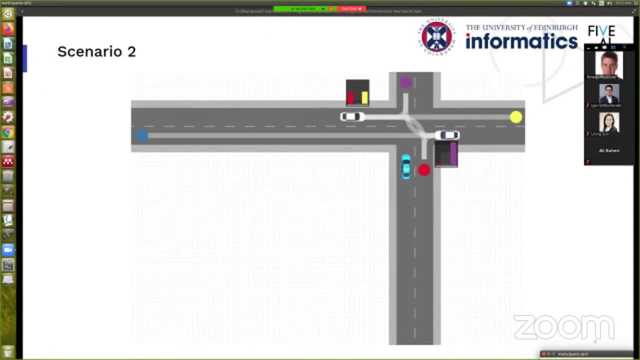 and the fact that the vehicle coming from the right has stopped to give way to this vehicle, we can infer that the vehicle on the right is trying to turn to the north. Given this knowledge, we can predict that the vehicle will not cross our path. 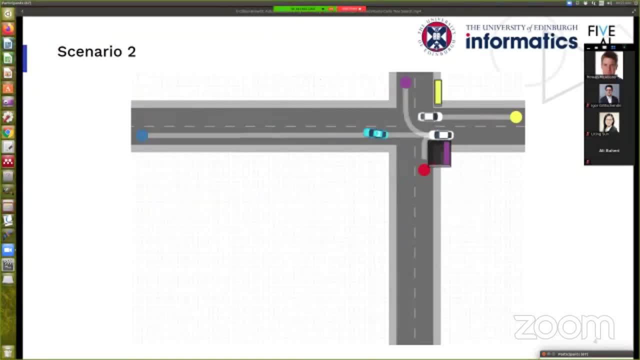 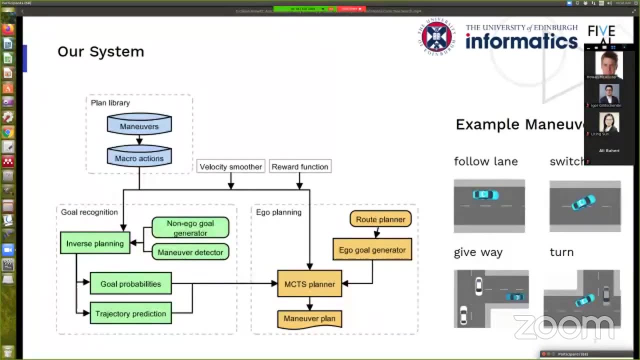 and we can safely enter the junction. Here is an overview of our system For both planning and prediction. we assume that agents use a predefined set of manoeuvres and macro-actions. In our prediction module we first use a classifier to infer a distribution. 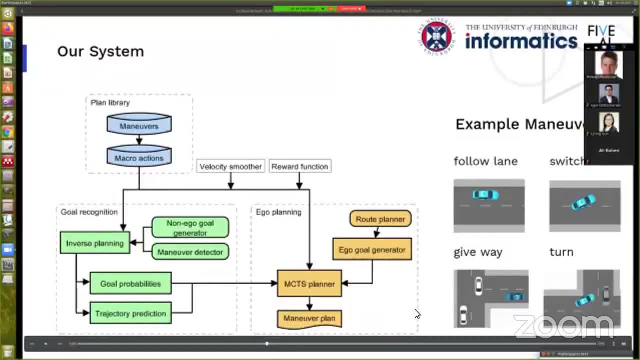 over possible current manoeuvres for each vehicle. We then use inverse planning to infer distributions over possible goals and for each goal we generate a set of possible trajectories. For the planning module. we use Monte Carlo TreeSearch to compute a plan for our vehicle. 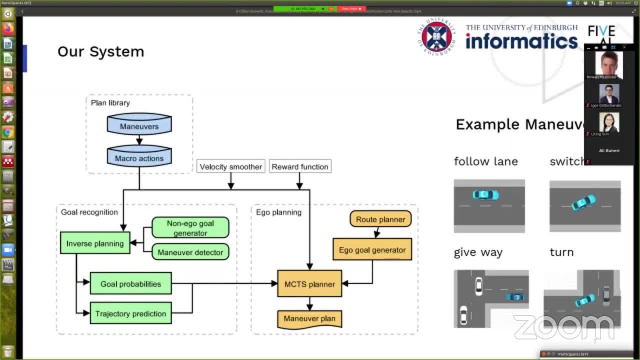 Monte Carlo. TreeSearch is an iterative statistical planning method and during each iteration, for each other vehicle, we sample a current manoeuvre, goal and trajectory from the distributions inferred by the prediction module. This shows another example of our system in action In this scenario. 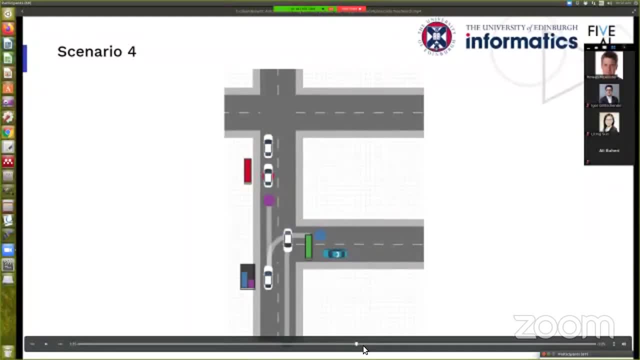 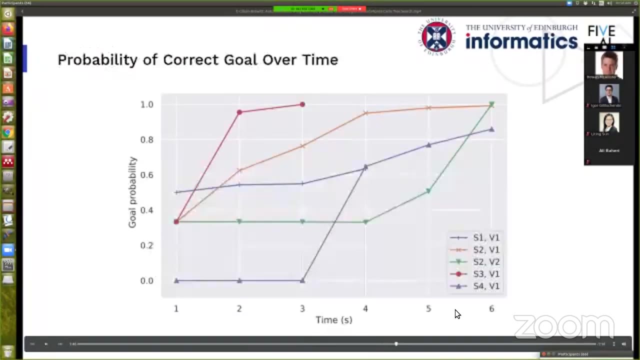 our goal is to merge into traffic. As we observe the vehicle coming from the south slowing down, the probability of it turning right rises As the vehicle stops. this reveals a stopping goal which rises in probability over time until we can safely merge. This plot shows the probability we assign to the correct goal. 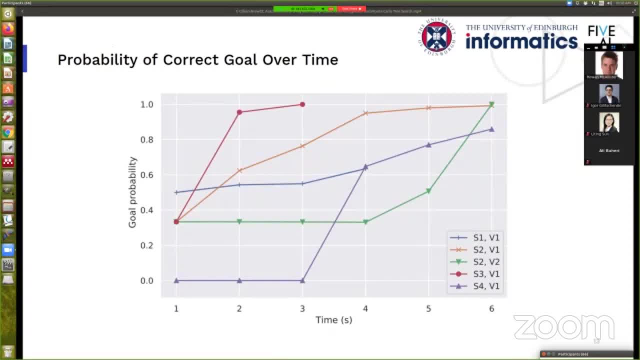 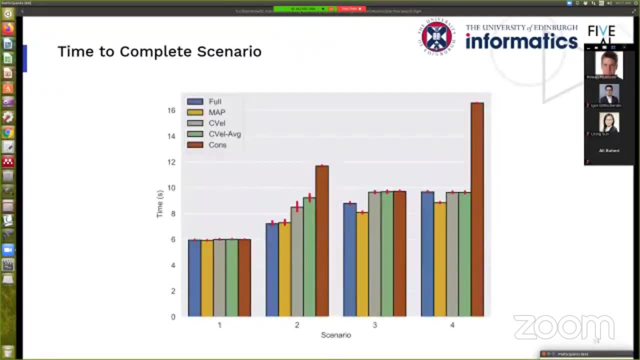 for some of the vehicles in our scenarios. As you can see, the probability rises over time as we gather more and more observations. We compared our method to several baselines which use simpler prediction methods. One of these methods made map predictions, where we only consider the most likely goal for each vehicle. 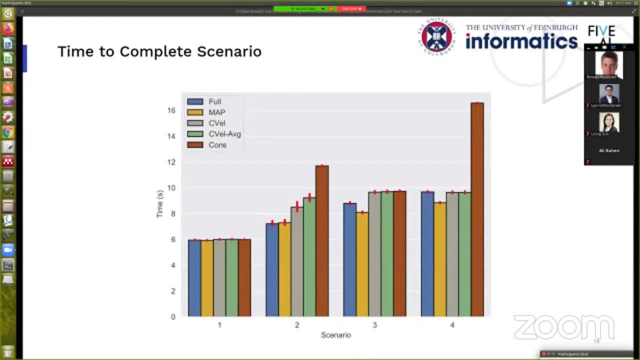 Another method simply predicted that other vehicles would continue following their current lane at their current velocity. Another gave similar predictions, but used the average velocity over the previous two seconds. We also used a conservative method where our vehicle always waits until oncoming vehicles have passed. 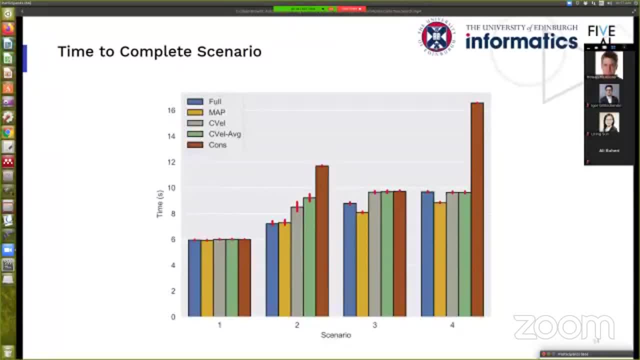 As you can see here, our method completes the scenario in the same time or faster than most of the baselines. One baseline that sometimes achieved a lower time than our full method was map predictions, where we only consider the most probable goal for each vehicle. 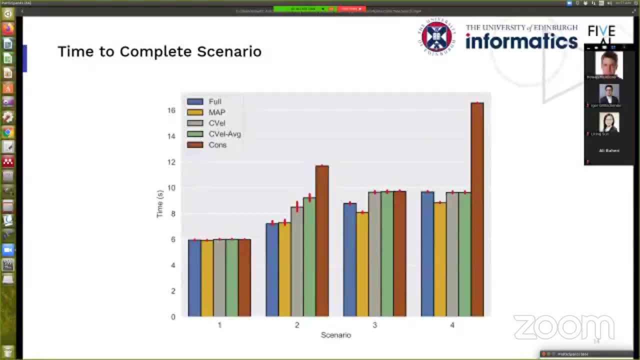 This extra certainty allows our vehicle to reach the goal more quickly on average, but can lead to dangerous behaviour, as it does not consider all possibilities. Even in the cases where our full methods achieve the same time as other baselines, it still has the advantage of being able to explain. 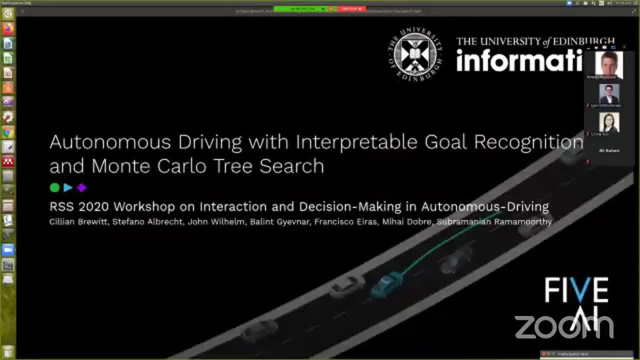 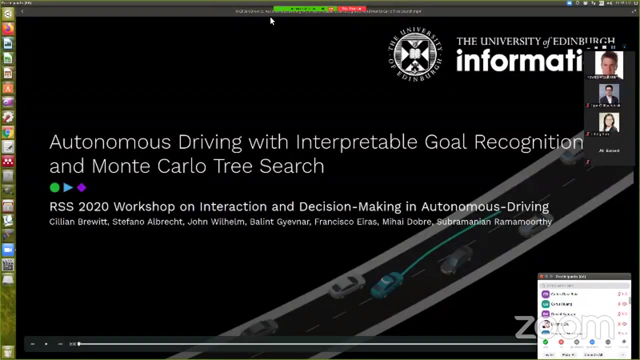 its predictions Great. Well, thank you, Celian. If there's any questions, please let us know. Well, to kick things off, I have a question, Celian. How does the time complexity work with these candidate goals? Is the runtime? does it scale linearly? 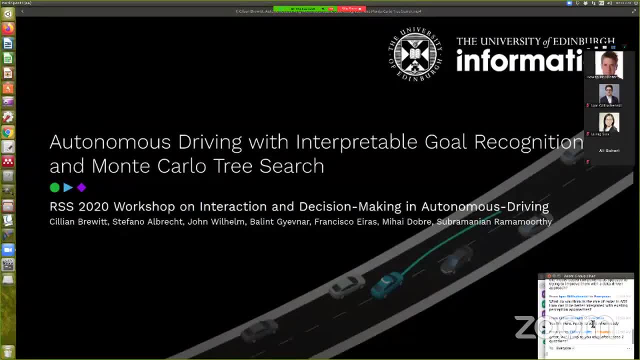 with respect to the number of goals and also the number of other vehicles. And if the situation is very complex, would there be a way to make it sub-linear? It is linear complexity in the number of vehicles and number of goals, But it is. 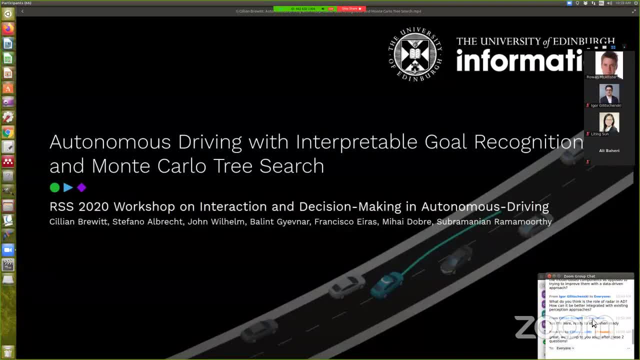 That complexity is parallelisable, So we can We independently make predictions for different vehicles. So if there are a lot of vehicles and a lot of possible goals, although it's linear, yeah, it's still parallelisable, So it could be feasible to compute. 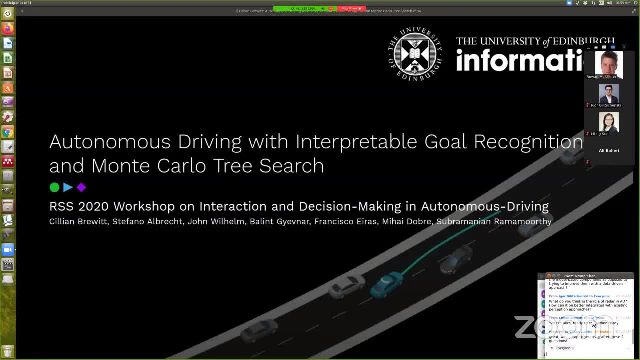 That makes sense. And actually another question I had is: so I thought the merge system was interesting, where you introduce a static goal to where the car is, so that we can consider that maybe that car has stopped and it's letting us in. 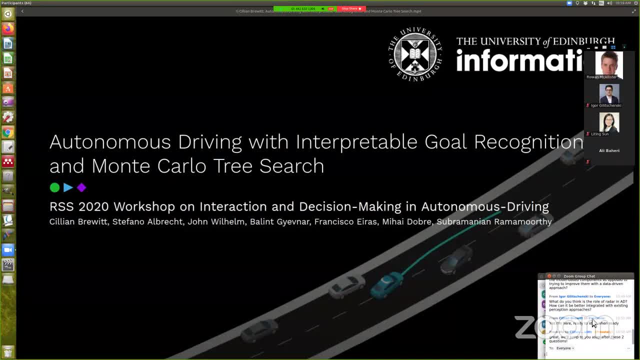 Do you think maybe there could be some interesting extensions to this work for non-ego goals, Like maybe, for example, dynamic goals, where that human driver will never come to a stop but they'll at least slow down for us to allow us to merge? 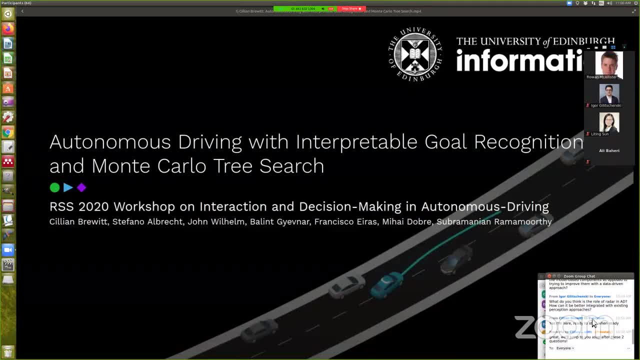 but they'll never actually stop. for example: Yeah, We could definitely extend it with more goals like that. In the scenario there it was just a stopping goal because it was merging a junction, But say, when we want to switch lane and merge into moving traffic. 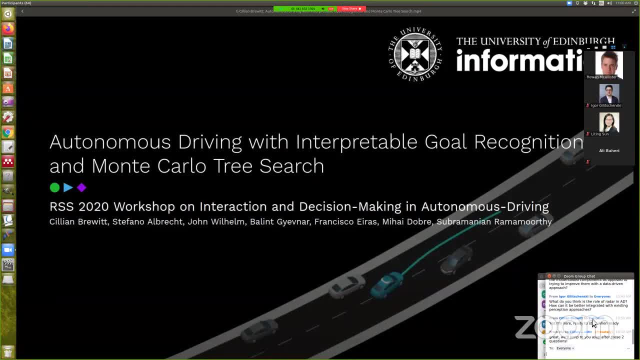 a car could have a goal where their goal is for you to be in front of them. So, in a way, our goal is their goal. Yeah, Okay, great, Okay, thanks. If anyone has any further questions for Cillian, please just type them into the chat. 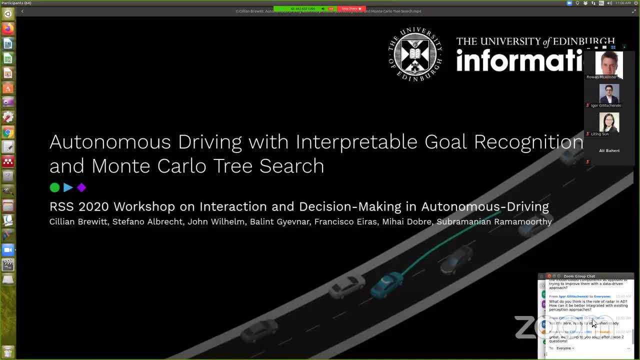 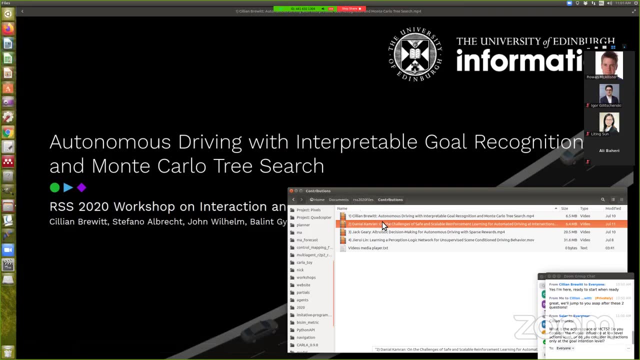 And Cillian, if you want to just keep an eye on that chat, maybe you can answer them from there. Okay, great. So next we're going to move on to Hello everyone. Next, we're going to move on. 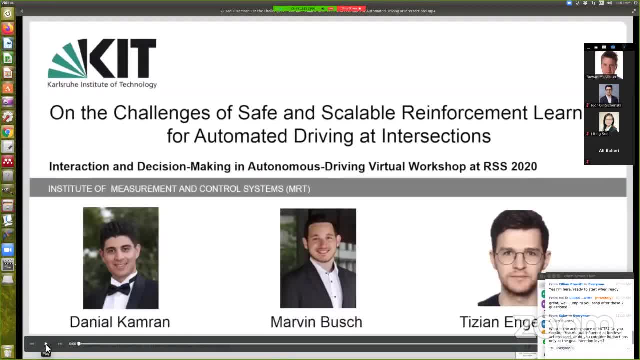 to a talk by Daniel Cameron. Hello everyone, Welcome to this presentation. In this video, we are going to present our paper on the challenges of safe and scalable reinforcement learning for automated driving at intersections. My name is Daniel Cameron and I wrote this paper in cooperation. 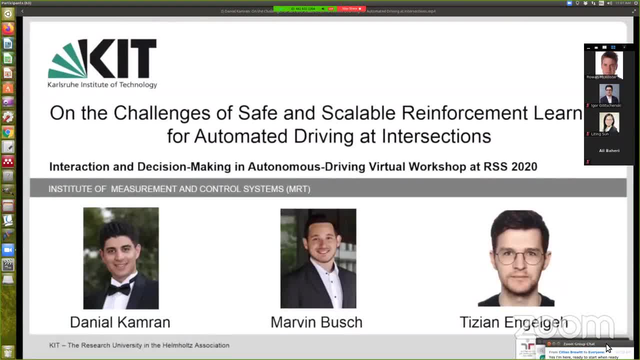 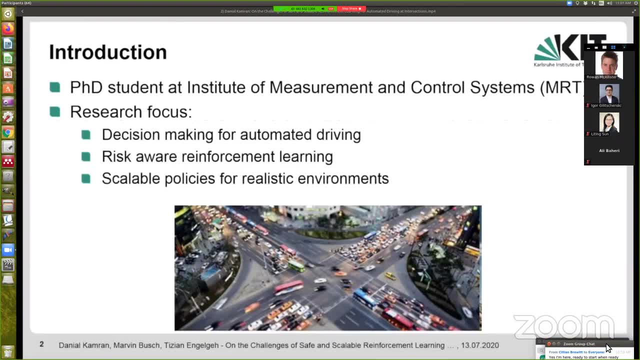 with Marvin Bosch and Tizian Elgenke. First I will have a short introduction of myself. I am a PhD student at Institute of Measurement and Control Systems at Kosfouhe Institute of Technology. My research interests are decision-making for automated driving. 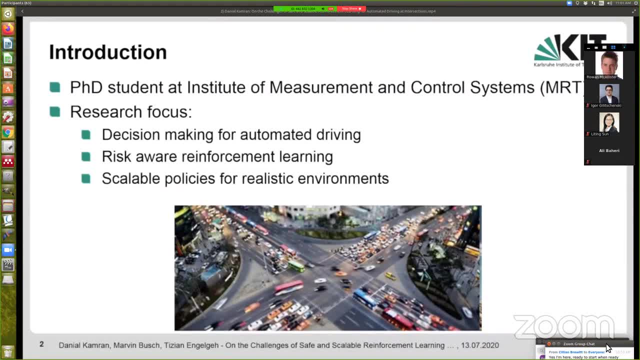 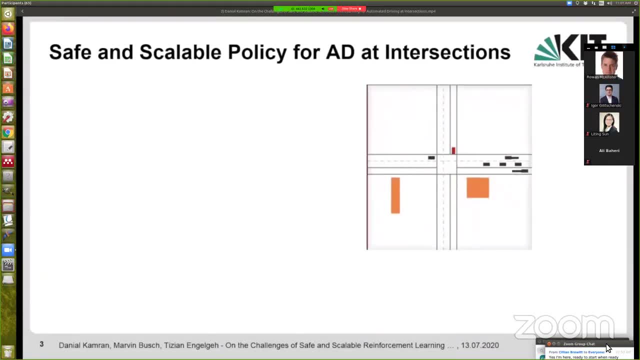 risk-able reinforcement, learning and scalable policies for realistic environments. There are some challenges to drive autonomously at occluded intersections. The number of vehicles and also the number of intersecting lanes can be different. Another important challenge is that some of these vehicles 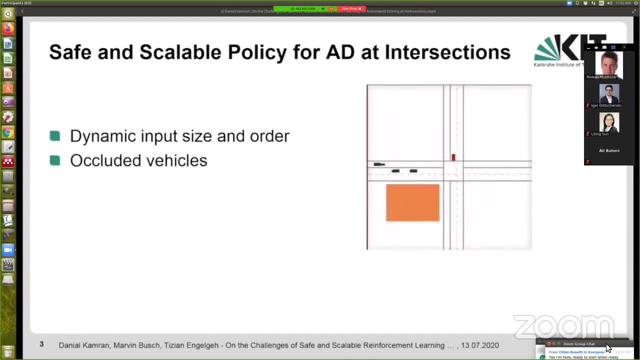 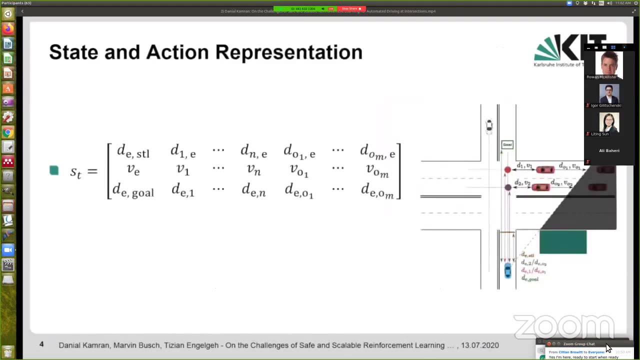 are hidden behind the obstacles, which needs the policy to know information about occluded areas. Our goal is to tackle these challenges by learning a safe and scalable policy with reinforcement learning for intersections. We represent the state by a matrix containing the ego-vehicle state. 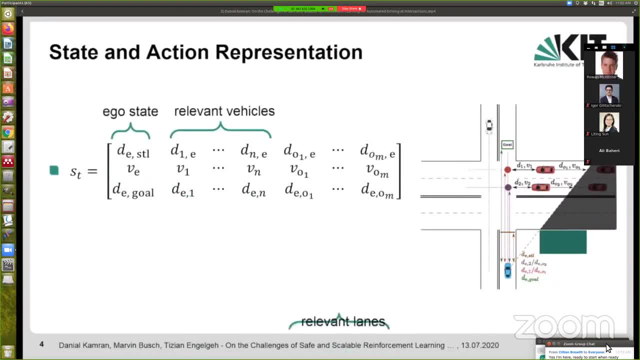 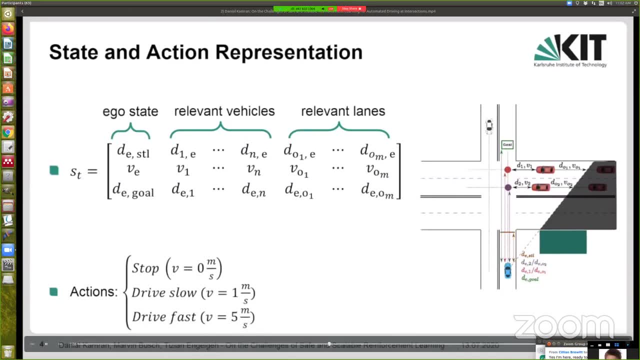 the relative distance and velocity of all vehicles and also maximum visibility distance and velocity for all intersecting lanes. In the output of our reinforcement learning agent, we have three actions to control the ego-vehicle behavior. These actions are: stop, drive slow. 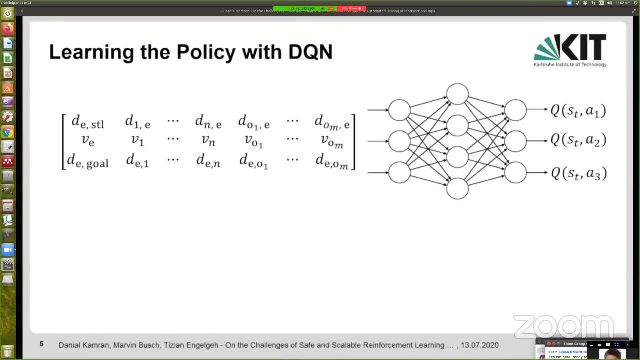 and drive fast. We use deep queue networks, known as deep queue-end, in order to learn the future return for each state and action. However, such implementation needs a big input size for dense traffic where there are many vehicles at the intersection. Also, the learned policy. 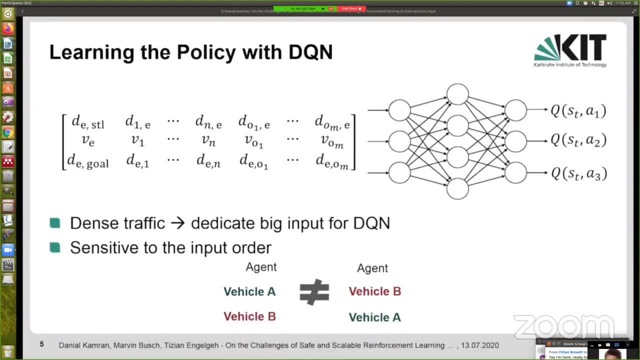 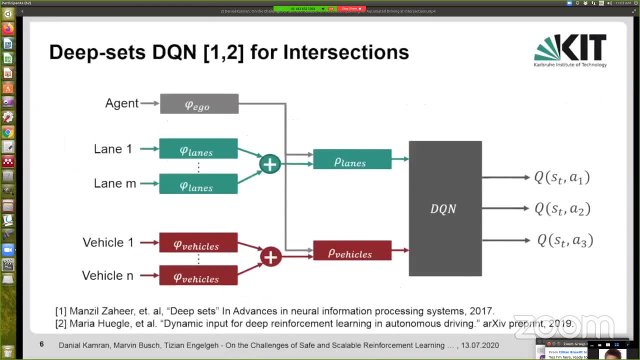 is very sensitive to the order of vehicles in the state representation and it may not be generic and scalable for different scenarios. Our proposal to solve this problem is to use deep sets architecture in order to process multiple input elements with same neural networks. We can then apply. 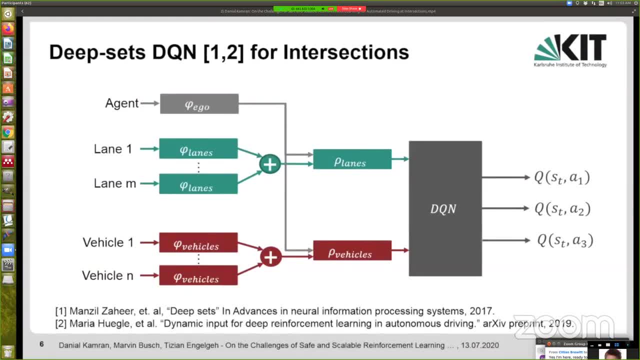 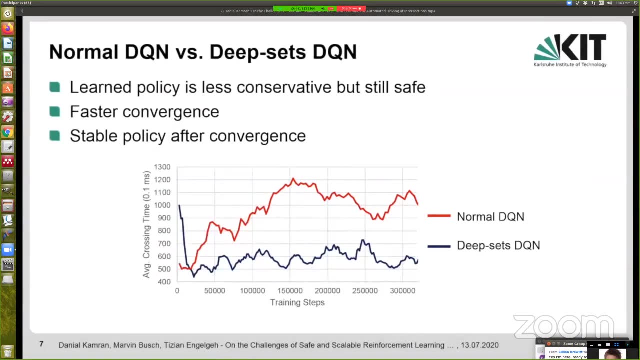 a permutation invariant operation on all processed data to have fixed input for our deep queue-end network. This operation also helps to be independent from the input order in our state representation, Comparing the deep sets deep queue-end and normal deep queue-end in our experiments. 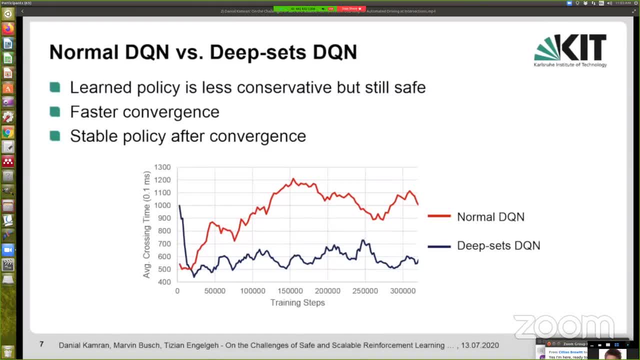 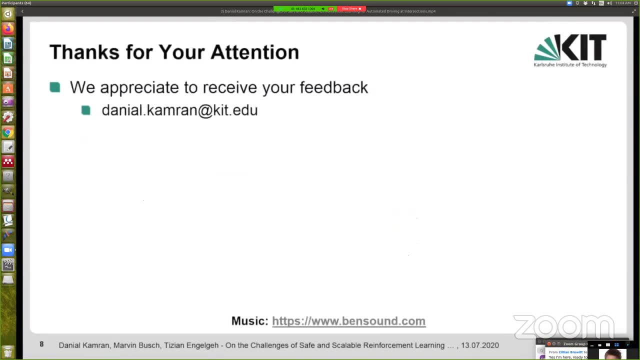 we observed that deep sets architecture could help to learn a less conservative but still safe policy. Also, the convergence time was shorter and the learned policy was more stable after convergence. Thank you very much for your attention. If you have any questions or feedback about my work. 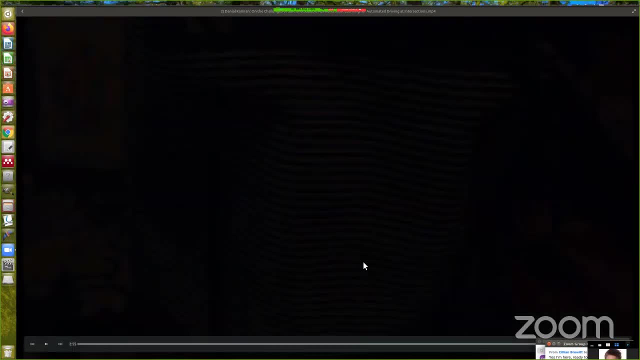 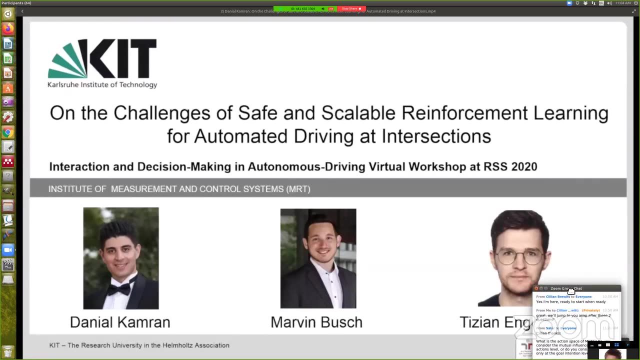 you can contact me through my email address. Great Yeah, thank you, Daniel. So again, if there's any questions, feel free to type them out in the chat. It looks like you have a question there, Celine, from the previous talk. 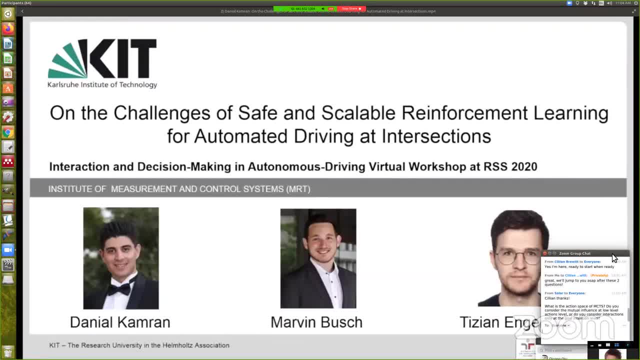 Maybe, to kick things off, I can ask a question, Daniel. So it seems like this deep set architecture helps with the exchangeability of vehicles. so, like invariance to vehicle order and things like that, Can it also help with a variable number of vehicles? 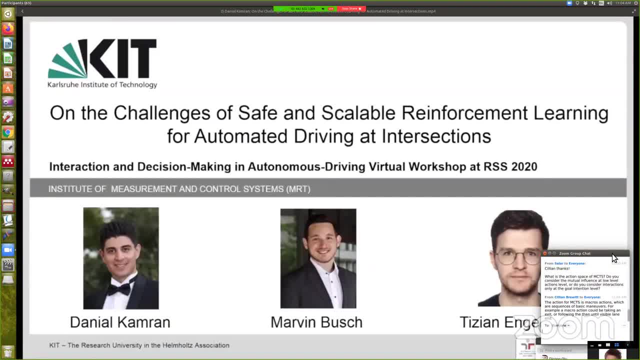 in case the number of them changes from one scenario to another, or the number of lane changes maybe? Yes, exactly, Actually, that's the main motivation that we want to use deep sets for such scenarios Because, as you said, for different traffic levels, 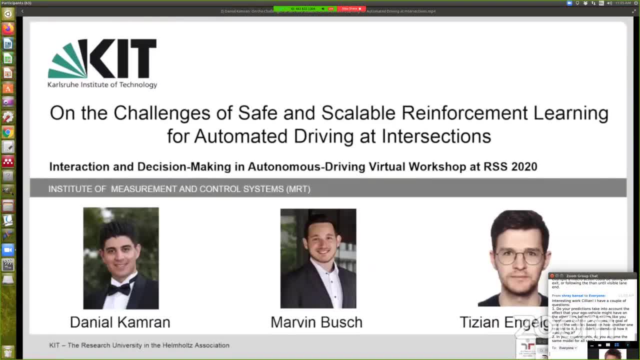 there may be different number of cars And also at different intersections there can be different intersecting lanes. So in order to have a generic and scalable policy, it really helps. Okay, great. And maybe another question is: so it looks like in these deep sets. 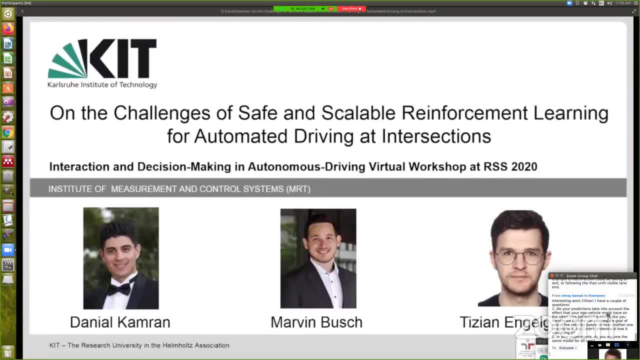 the lanes and the vehicles were pre-processed separately. Do we lose? Do we lose any maybe important information with respect to a vehicle being in a particular lane, say, the lane closest to us or the lane turning right? Yeah, that's true. 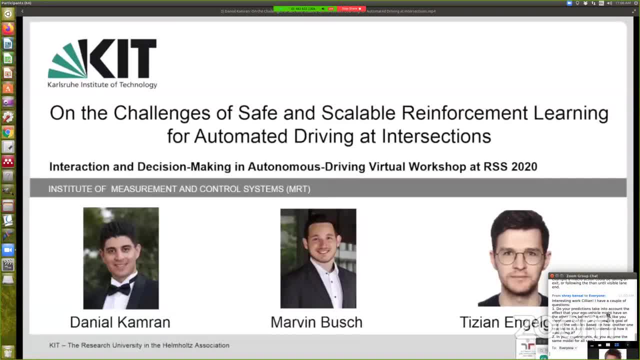 Actually, that's something that we can do for future work in order to provide a kind of attention from lanes when we want to process vehicles. But yeah, right now such kind of implementation it really works, And, on the other hand, because we just need to assume. 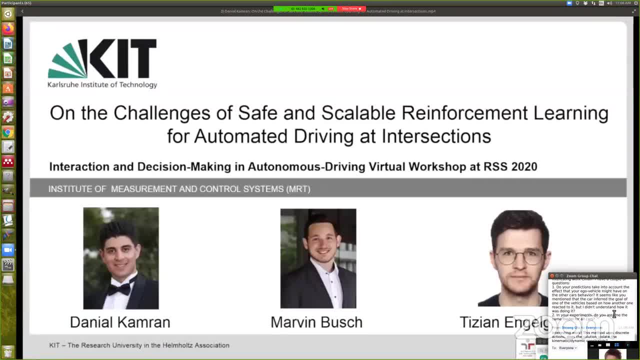 the worst case scenario for each lane. I mean just a scenario that there is one car driving very fast at occluded areas for that lane And the policy just need to know about that kind of worst case scenario. I mean just at this sense. 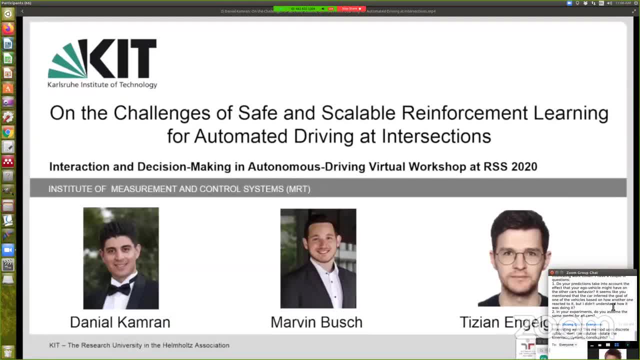 that can be occluded and the policy doesn't know about that car. So by that kind of information the policy should give us, get all of required information and, yeah, we should drive optimal. Okay, great, And we've just got a question. 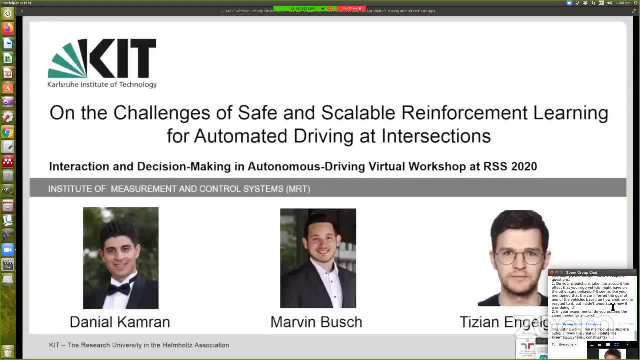 come in over the chat from Deacon saying interesting work. This method uses discrete actions. Does the solution violate the kinematics slash dynamics constraints? Well, the methodology that we have is to have some kind of high level actions or to learn some kind of high level actions. 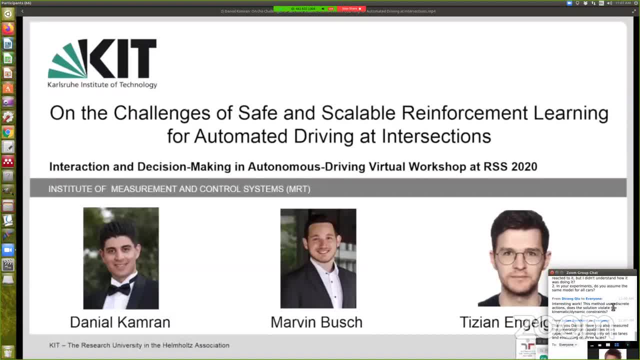 So that's right. We have to consider the transition changes that we may have for the vehicle because of- yeah, because of- changes in the control. Maybe we don't have a good controller, but we already consider that during training, So the decision time is not very small. 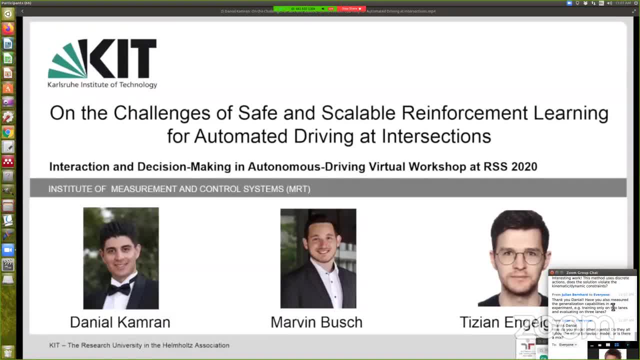 So the decision time is maybe, for example, half a second, And we hope that it helps to use that to solve this problem. Yeah, Okay, great Daniel. we've also got a bunch of questions coming in over the chat, but I might need to move on. 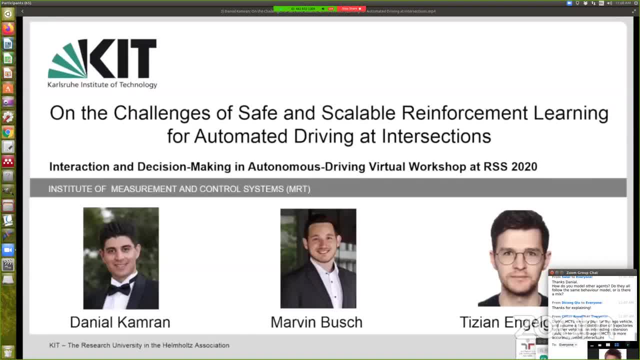 to the next speaker. So if you want to jump into the chat and answer those questions there and anyone, feel free to keep asking Daniel questions in the chat. Yeah, thank you. Okay. So next we're moving on to a talk by Jack. 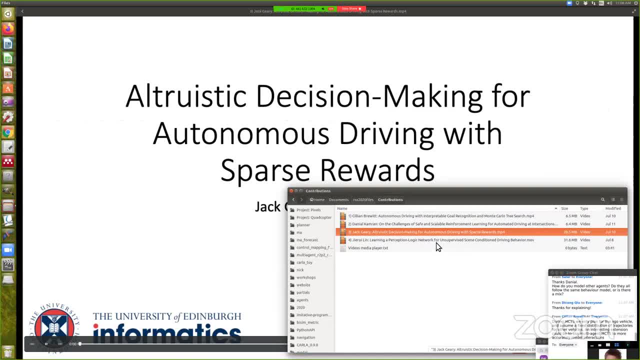 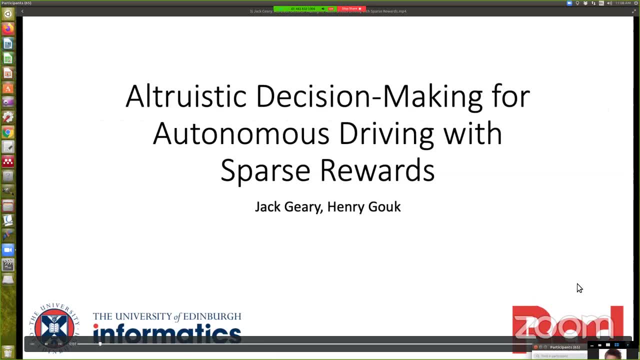 Nick, Hi everyone, Thank you for joining us. So we're going to talk about the potential for conflict in a Stackelberg game. So we're going to talk about the potential for conflict in a Stackelberg game. We present a method. 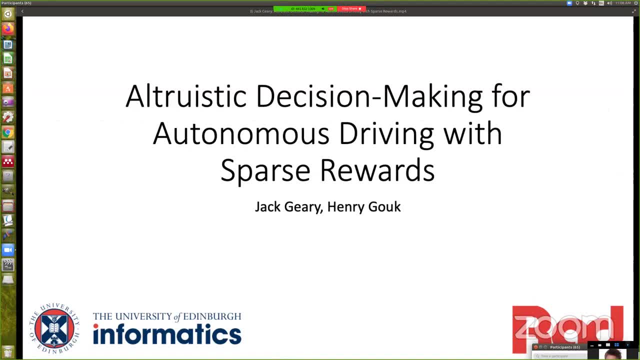 for measuring the potential for conflict in a Stackelberg game, We propose a novel reward definition that accounts for the altruistic tendencies of players and minimizes the potential for conflict. In the two-car interactive decision-making problem, each car must choose an action. 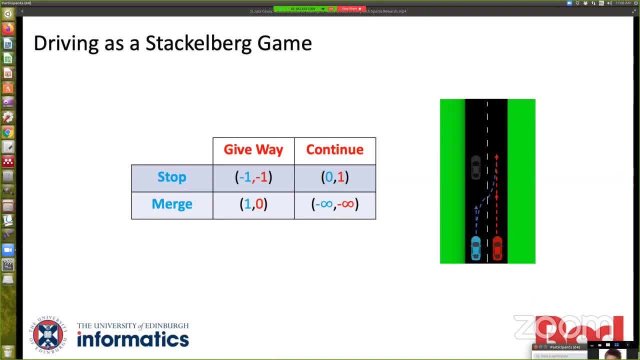 with the best outcome after accounting for the other car's behavior. This can be formalized as a Stackelberg game. In this setting, one car assumes the role of the leader and choose the action that matches the action that the other car does. 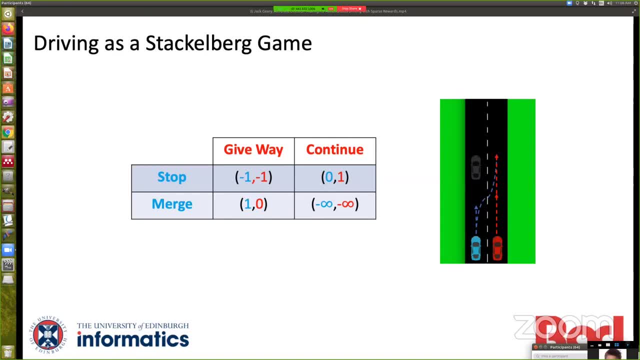 So the two-car strategy maximizes their reward. The other car, as the follower, selects their action optimally with respect to the leader's choice. In a Stackelberg game, it is presumed that the identity of the leader and follower are known. 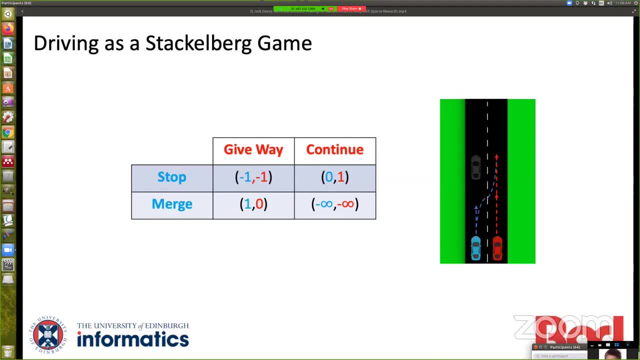 This can cause problems, as in many driving scenarios. this is not the case In the example shown. the blue car must change lanes in order to avoid a stationary obstacle. If the blue car assumes they are the leader, they will conclude that the red car 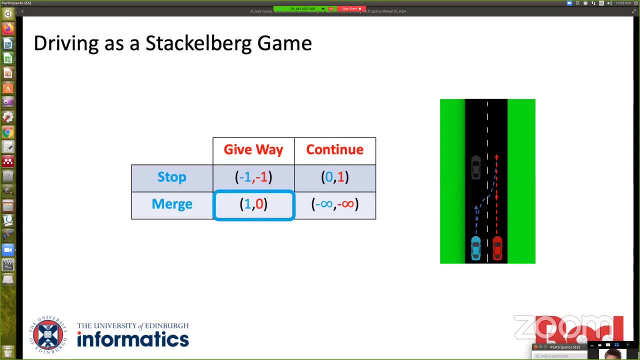 will give way to allow them to complete the merge. However, if the red car assumes the role of leader, they will expect the blue car to stay in their lane until they have passed. This ambiguity results in conflict, as the cars have differing beliefs about how the problem 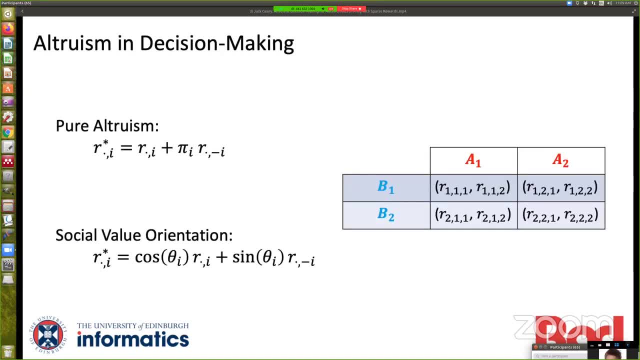 is being solved. This naive formulation neglects altruistic tendencies often demonstrated by human drivers. Methods previously proposed in the literature, such as pure altruism or social value orientation, account for this by defining each player's reward as a weighted sum of the naive rewards. 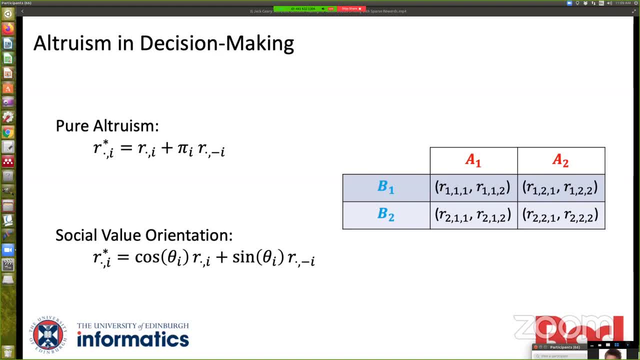 In our example, if either car is sufficiently altruistic, they will decide on the same solution to the decision-making problem, irrespective of who takes the role of leader or follower, thus resolving the conflict. We propose a metric for determining to what extent a stackable board game 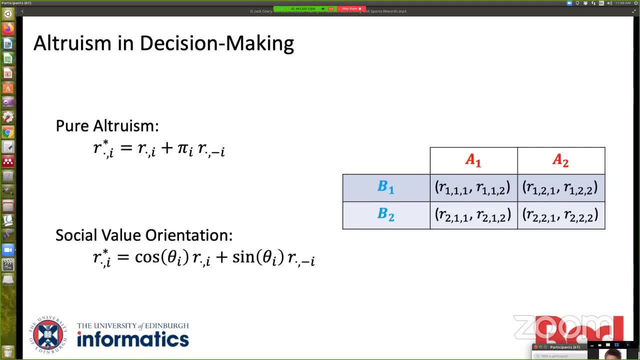 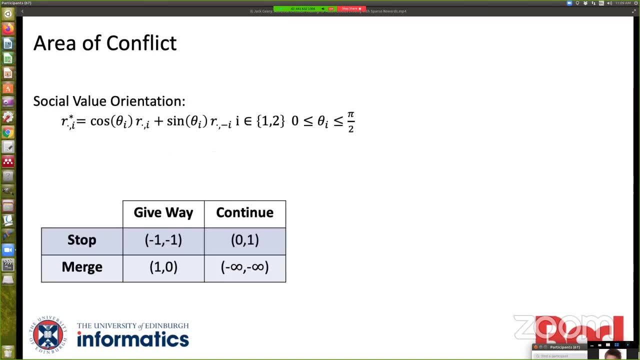 is susceptible to these conflicts for a given reward definition. This allows us to compare how effectively different reward definitions resolve conflict. for a given game matrix. We use the naive game matrix and the reward definition to identify regions in parameter space that result in conflict. The total size: 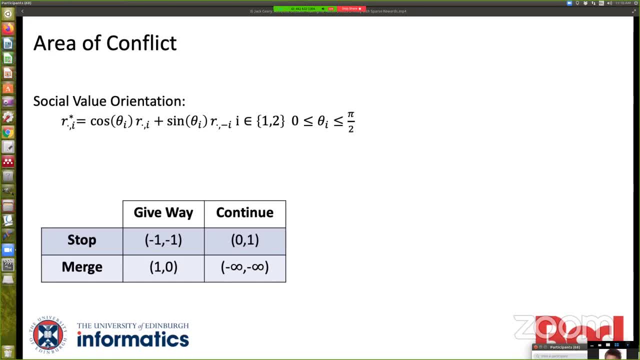 of these regions relative to the parameter space defines the incidence of conflict. We call this measure the area of conflict or the area of conflict. In our example, the constraints divide the parameter space for social value orientation into four equal regions, two of which are in conflict. 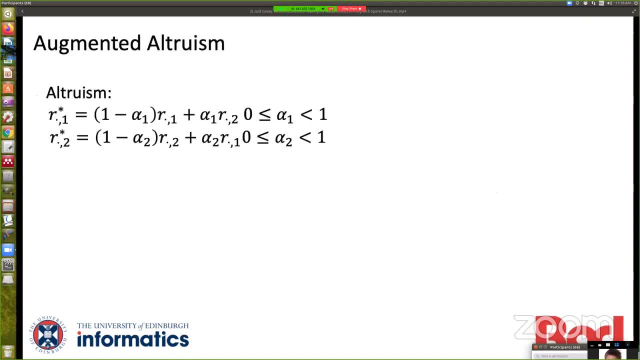 so the area of conflict is 0.5.. Iterated methods are often applied to simulate the reasoning used by humans when solving decision-making tasks. Using similar reasoning, we utilize a novel reward definition and formulate the rewards for each car for a particular action combination. 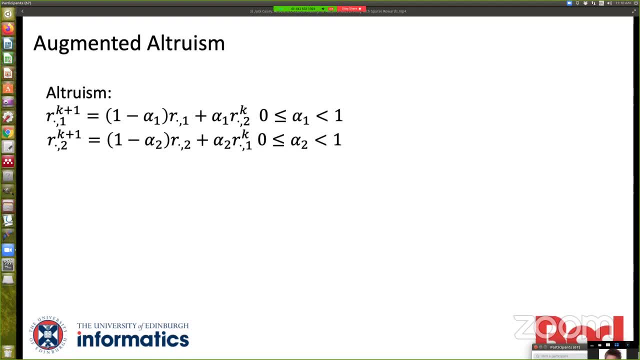 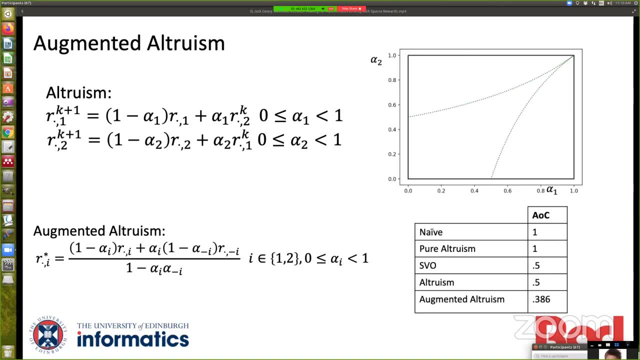 as a dynamical system. By identifying the steady state of this system, we find a reward definition that natively accounts for both players' altruism. when evaluating the reward, We observe that this reward definition has a minimal area of conflict. for the example scenario: 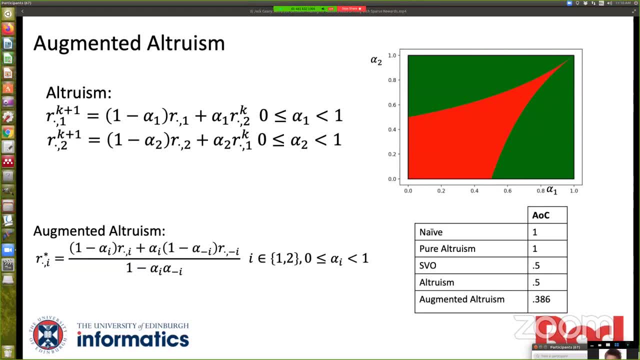 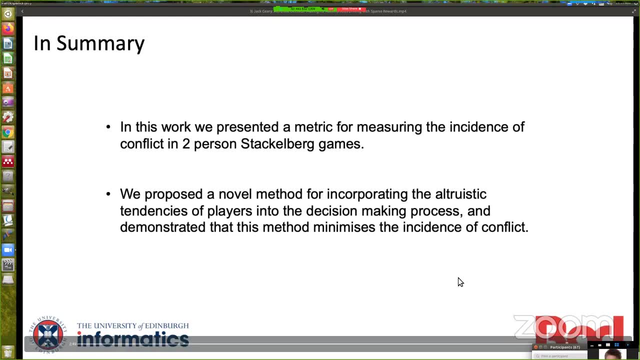 This reward definition consistently minimizes the area of conflict for a wide range of naive reward values. In summary, in this work we presented a metric for measuring the incidence of conflict in two-person Sacklebert games. We proposed a novel method for incorporating a method. 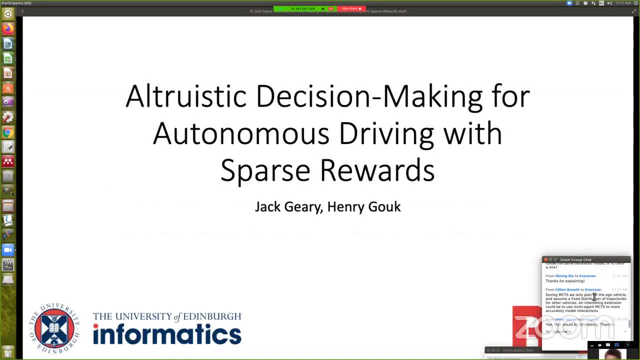 to demonstrate that this method minimizes the incidence of conflict. Okay, great. Thank you, Jack. Again, any questions, just type them into the chat chat box, Maybe to kick things off, Jack, does this assume that human drivers are altruistic? 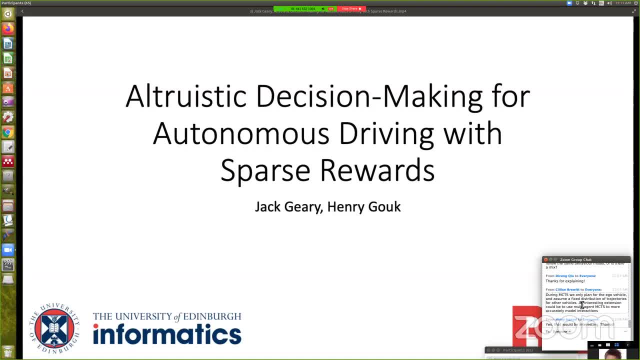 And if that assumption is sometimes broken, is there maybe anything to maybe infer how altruistic they are? So we don't. Altruism score of zero would correspond to purely egoistic behavior. So that would just be behavior that's motivated on their own. 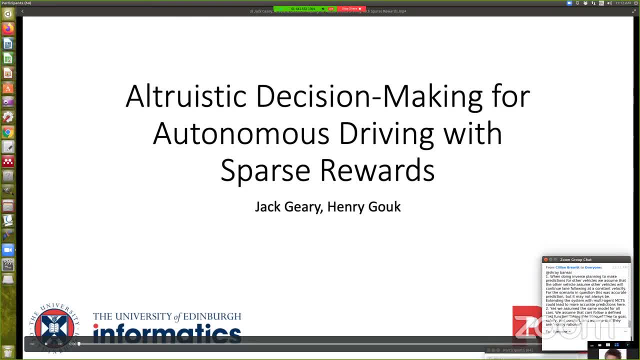 motivations. Future work we're planning is focusing on estimating the altruism values as we would find it for altruism and augmented altruism, But there is already work being done to understand what the actual value of the value, of the value of the value of. 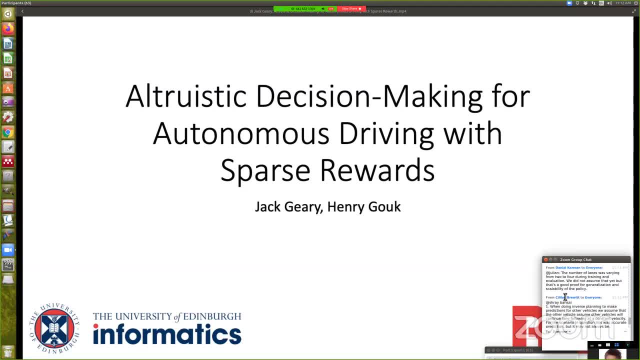 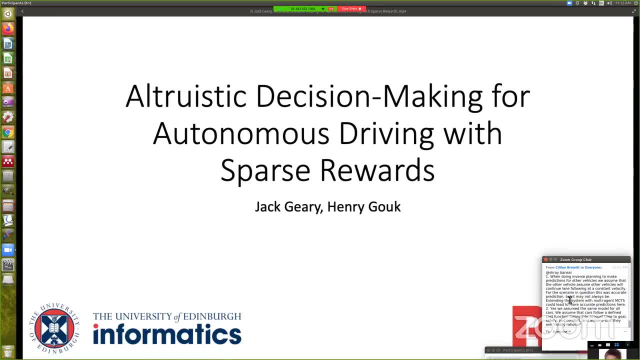 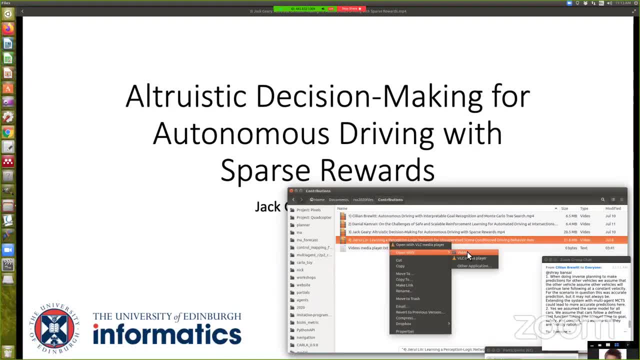 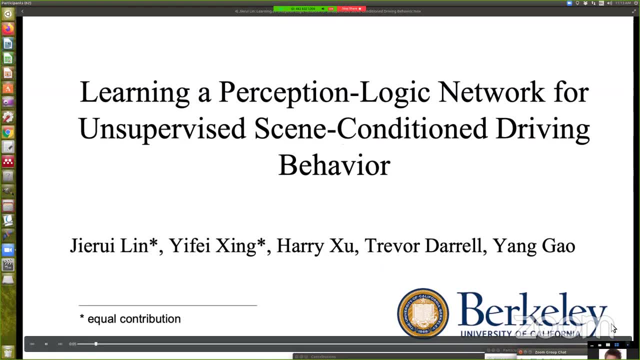 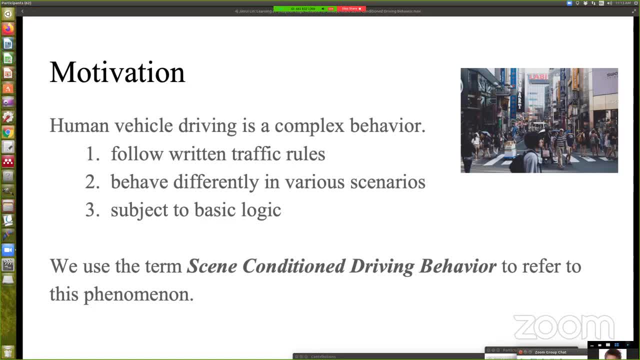 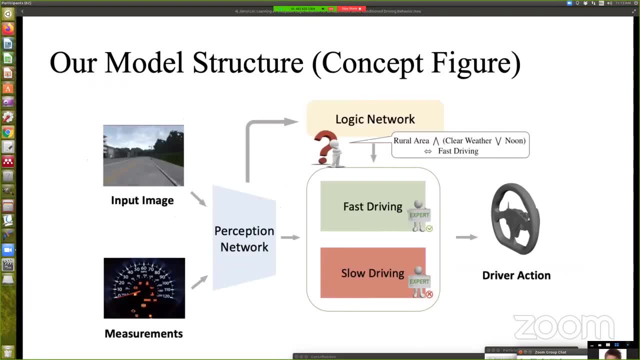 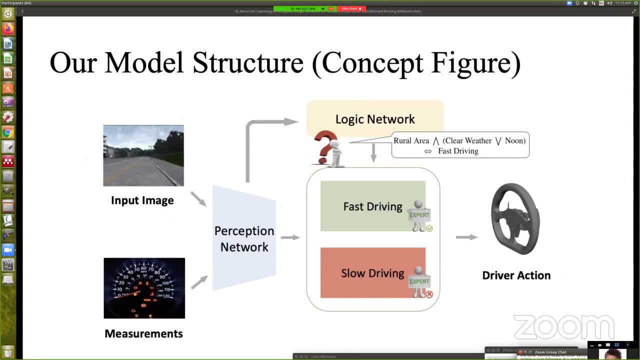 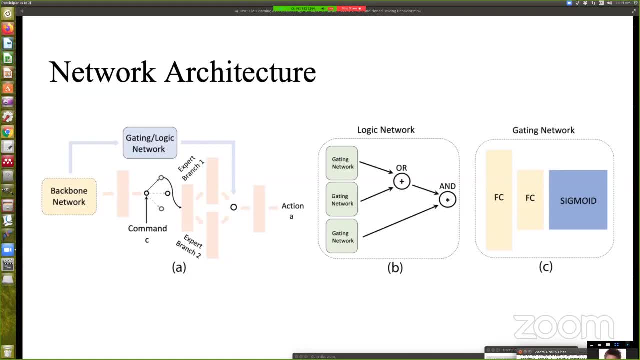 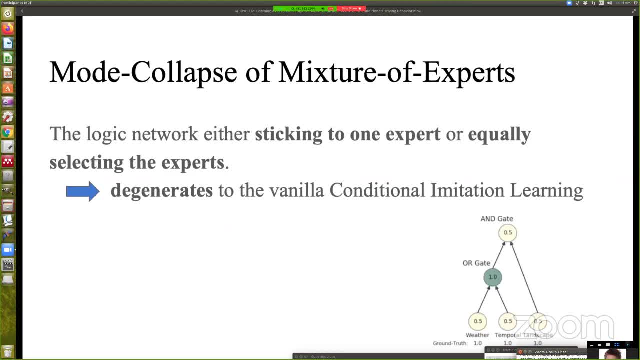 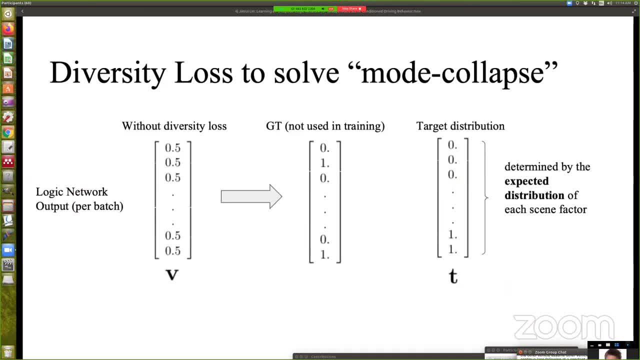 We propose a diversity loss to solve mode collapse. Without diversity loss, the output of our logic network looks like the vector drawn on the left. Although we don't have the ground truth labeled, during training we know the expected distribution of each scene factor and thus can generate a vector that matches the target distribution. 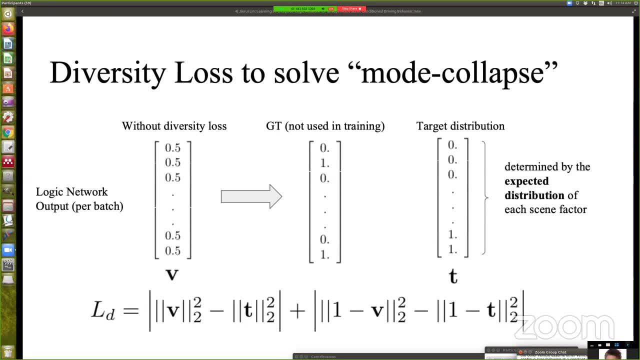 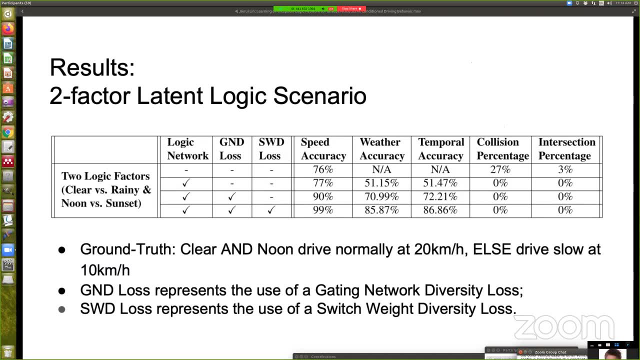 This leads to our diversity loss. that makes sure the output of our logic network is under the correct distribution. In our experiments we apply the diversity loss to every node of our logic network. We use the Carlos emulator, which is one of the closest proxies to real-world driving environments, to train and evaluate our model. 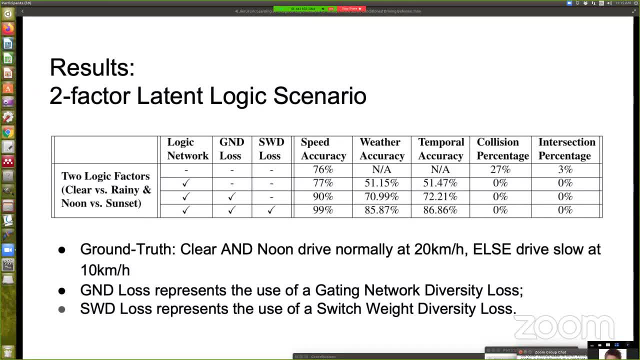 Here we show our results on a two-factor latent logic scenario where the ground truth logic is to drive at normal speed if, and only if, it is clear, and during noon time We can see that our agent, with both the logic network and all diversity losses, performs best in terms of the speed accuracy. 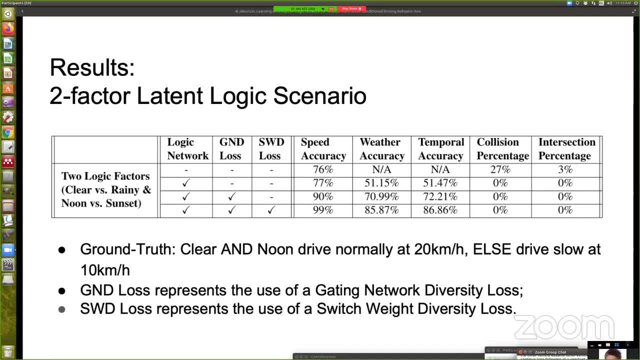 We also evaluate the scene factor prediction accuracy to check if our logic network learns the correct visual signal that determines the driving behavior. As shown in the table, the diversity loss plays an important role. We show the generalizability of our method by introducing landscape as one additional scene factor besides weather and temporal. 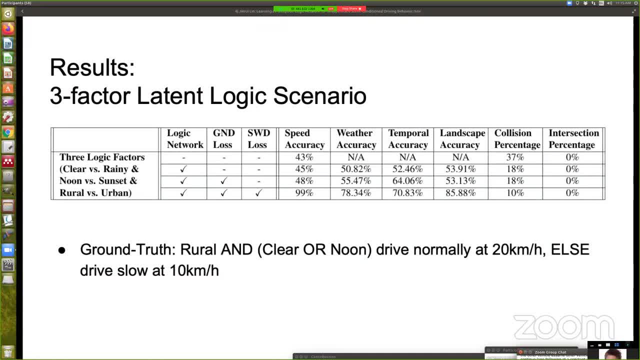 The logic role is to drive at normal speed if, and only if, it is in a rural area and it is clear weather or during noon time. From the numbers we can see that our agent performs perfectly under such a complex logic and the logic network learns the correct scene factors with little supervision. 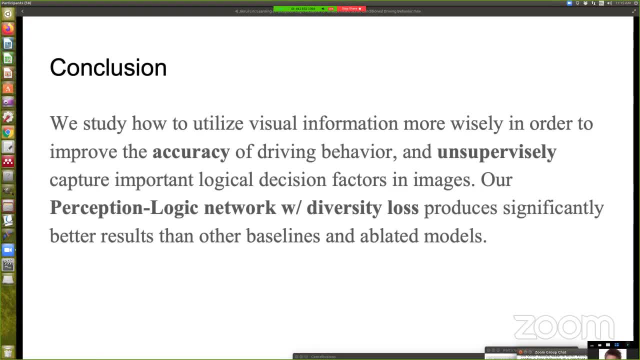 In conclusion, we study how to utilize visual information more wisely in order to improve the accuracy of driving behavior. An unsupervised vocabulary is important. It is also important to capture important logic decisions in images, Our perception logic network. with diversity loss produces significantly better results than other baselines and abelated models. 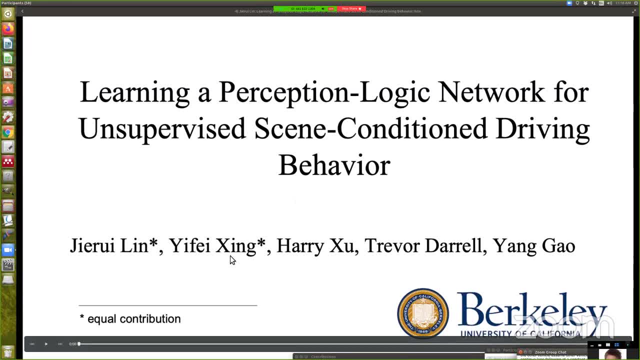 Great, Thank you so much. So any questions, again, feel free to just add them into the chat. So I guess, like, given these logic gates, given that they seem to have semantic meaning, do you think there's any extensions to this work in terms of the explainability of some of these decisions? do you think? 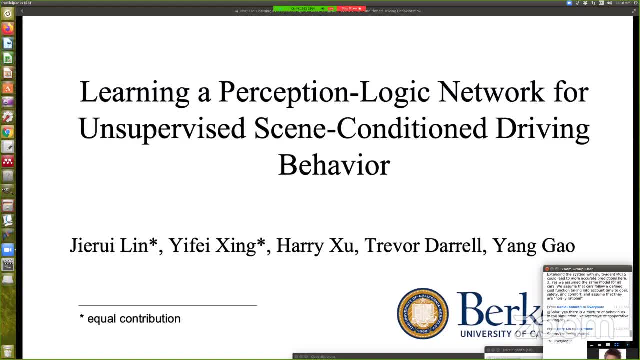 Oh, looks like, Sorry, Okay, yeah, Yeah, I think it's a good question, Like, so the logic variables, like may not have semantic meaning when like trained, like without explicit supervision. But I think, like our diversity loss and like the 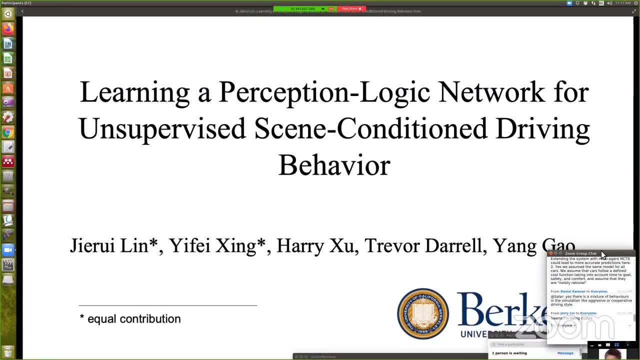 And our training data makes sure that, like, the output of the logic network matches the expectation of like how many of the data follow like each traffic group. So it makes sure, like it focuses on like the semantic meaning for states in our like training. 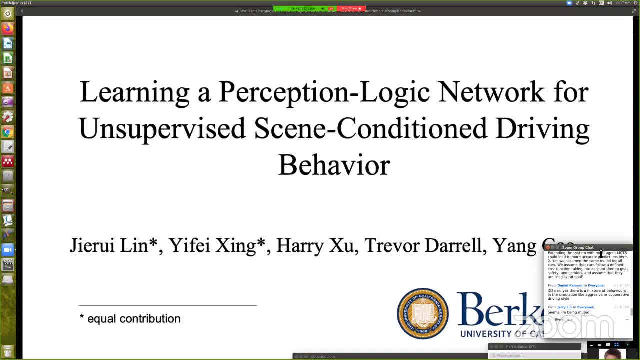 Yeah, Okay, great. So yeah, any more questions for Jerry. Just throw them into the chat And, Jerry, if you can hang around in the chat to look out for any questions, We're running a couple minutes over time now. 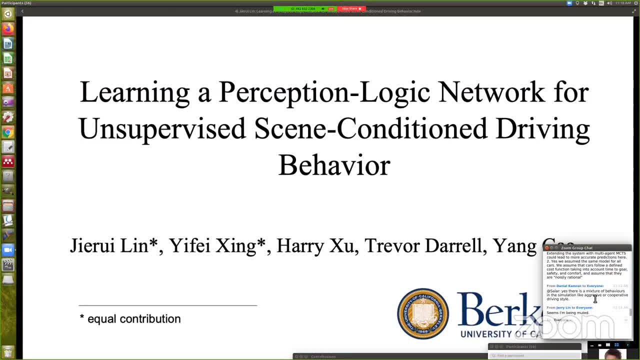 So I might close the questions And we're going for a break now. So this is an RSS-wide break. A lot of the other workshops are having a break right now as well. We're going to come back. I realize everyone's on different time zones. 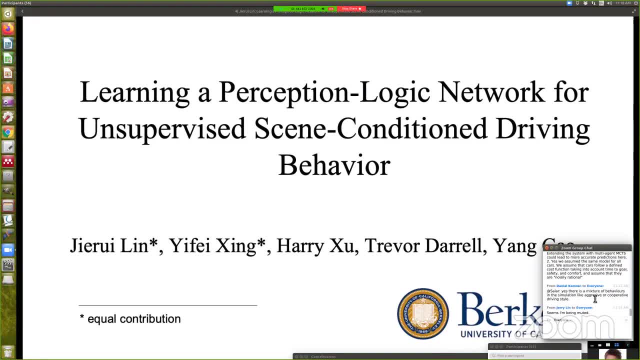 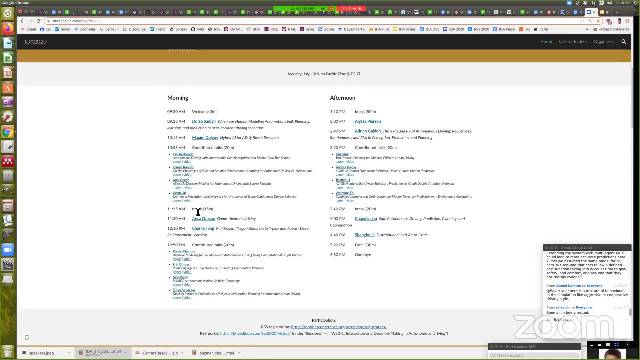 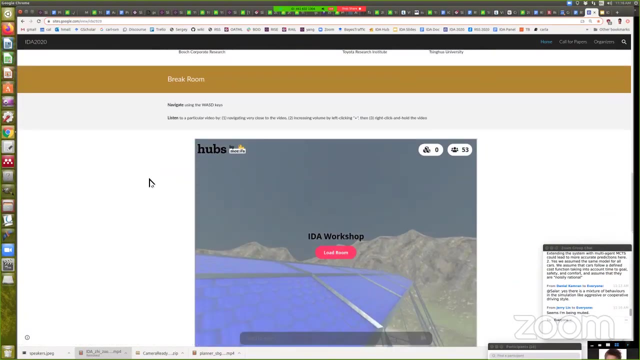 But we're going to come back at 30 minutes past the hour, So in 12 minutes, And I just wanted to show you that. So as a little bit of an experiment, So we're currently here in the schedule, We do have a break room, which is in: 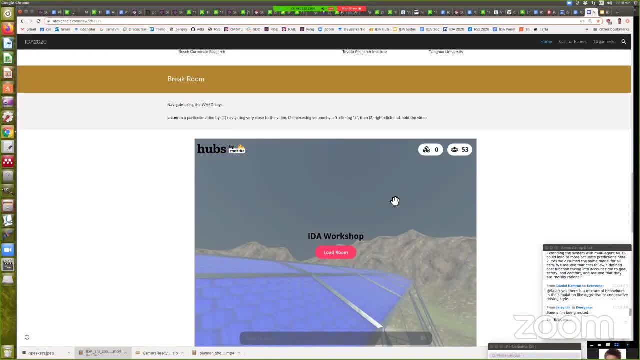 And so if you want, you can try entering that, And we've got all the videos there. If any of the authors of the videos want to go in, they might be able to explain them, But we're going to try and get the methods better there. 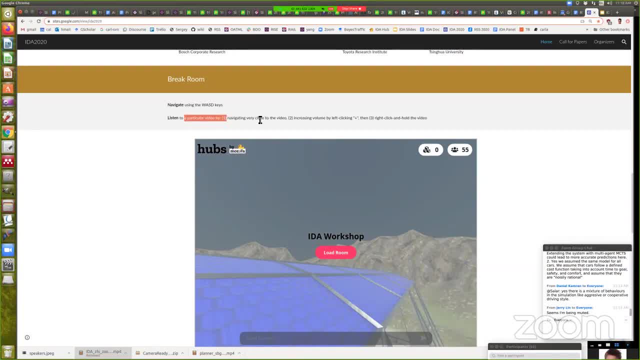 There is some instructions. It can be a bit noisy, But there is some instructions to basically go close to a video, increase the volume and then also right-click the video to hear that video better. So yeah, feel free to check it out any time during the day, including now. 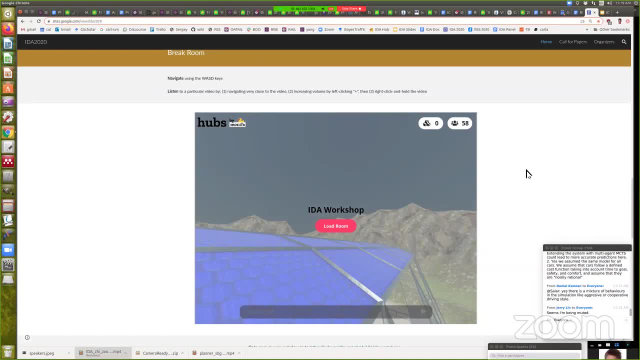 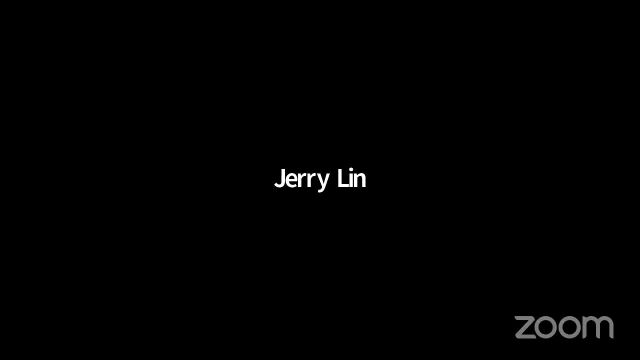 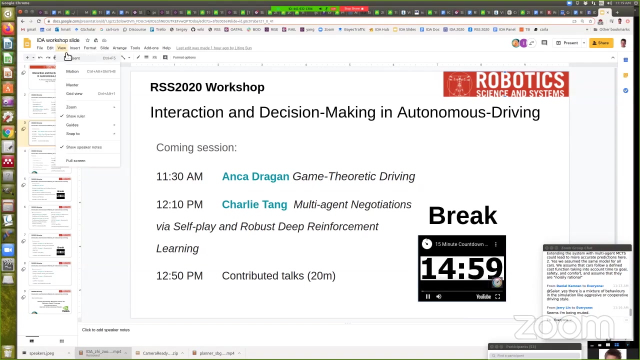 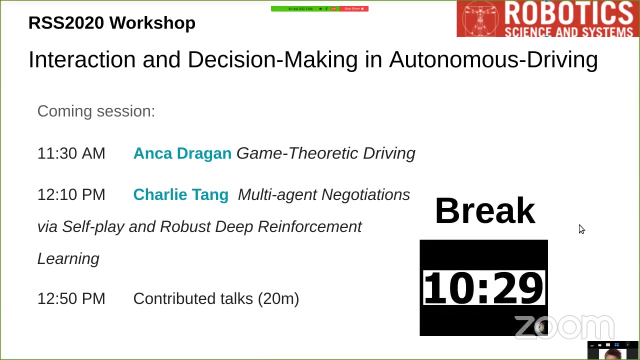 And we will meet back here in 11 minutes to hear from, To hear a talk from, Ankur. Thanks everyone, Bye-bye, Bye-bye, Bye-bye, Bye-bye, Bye-bye, Thank you, You, You. 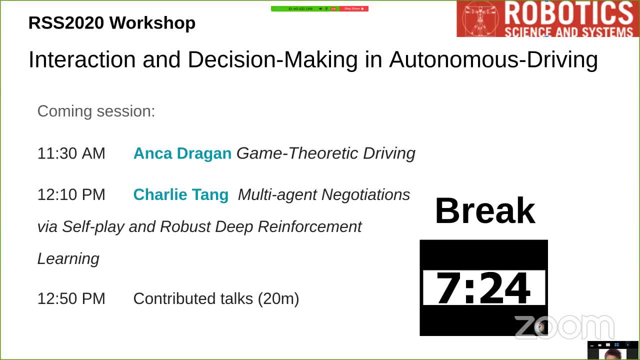 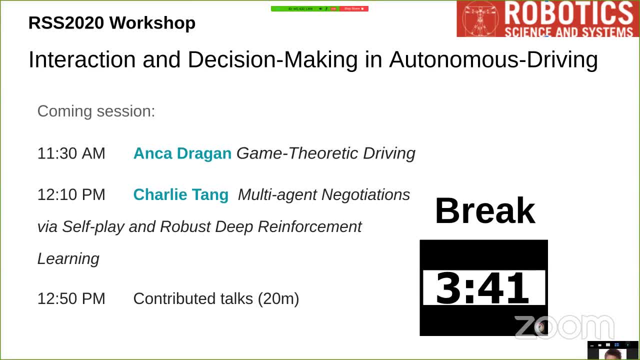 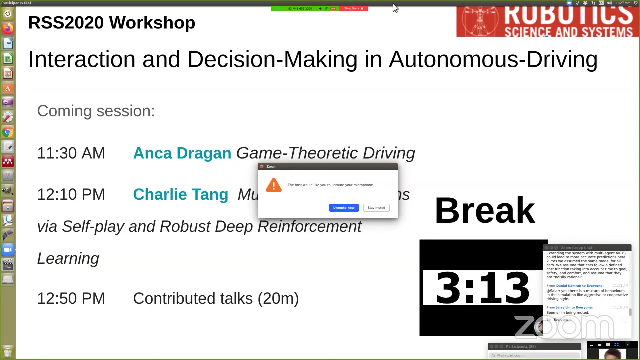 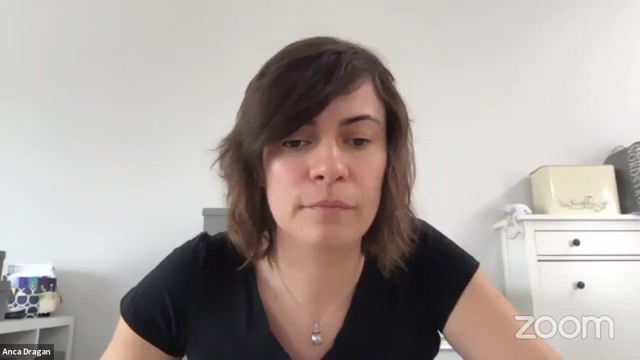 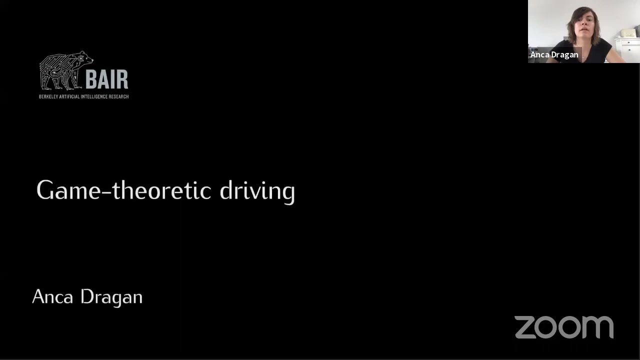 oh, let me ask him to unstop his. so okay, let me try now. how is this looks good? yeah, do you see my full slide title? oh, no, uh, uh, the whole slice. yeah, the whole slide, not the presenter view. no, presenter view, it's perfect. yeah, sounds great. i never know which screen is which. 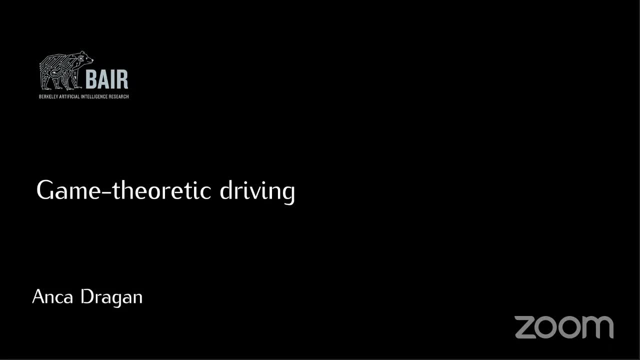 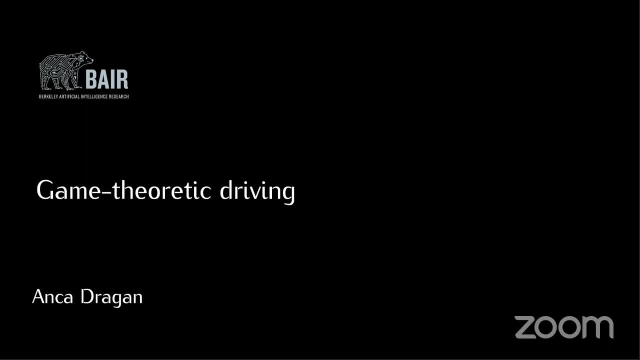 so, so, so, so, Okay, I think we can start. Okay, Welcome back everyone. So this is the RS 2020 workshop on interaction: decision-making in autonomous driving. So in this section again, we will have two invited talks and four contributed talks, And the next speaker. 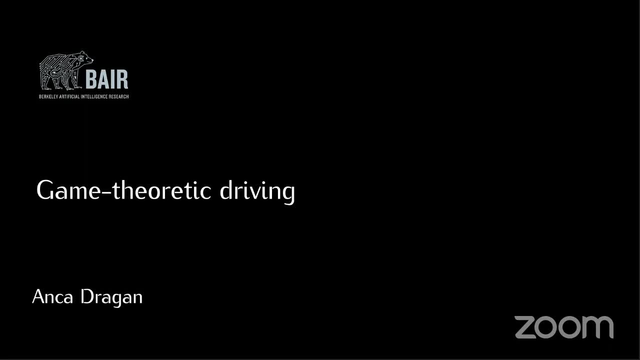 is Professor Anka. Dragan Anka is an assistant professor at UC Berkeley and she runs the Interact Lab. Her group focuses on designing algorithms to make robots to learn from humans and to better interact with humans. So let's welcome Anka. 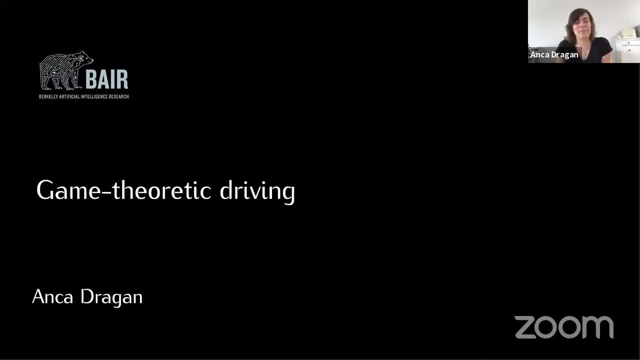 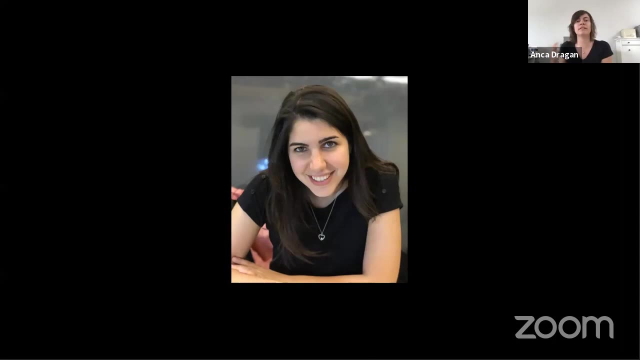 Thank you very much. Thanks for organizing this, And I'm so bummed that we can't all sit in a room together, but this will have to do So. I wanted to share a little bit today on game theoretic driving And I started doing research in this area. really, the intersection. 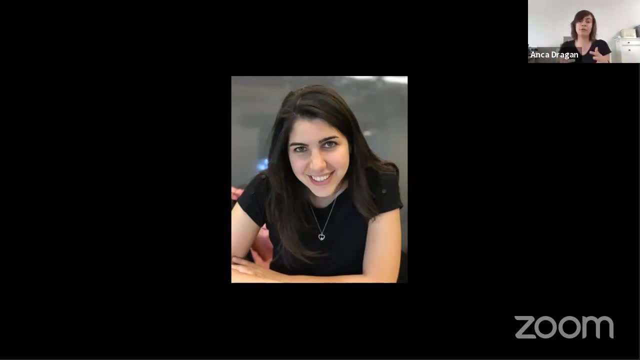 of interaction and decision-making for driving. I started doing this back in 2015 with Dorsa for her PhD, when we identified what seemed to be a gap in how academia- and, to the extent that we knew, industry as well at the time- was formulating the prediction or the forecasting. 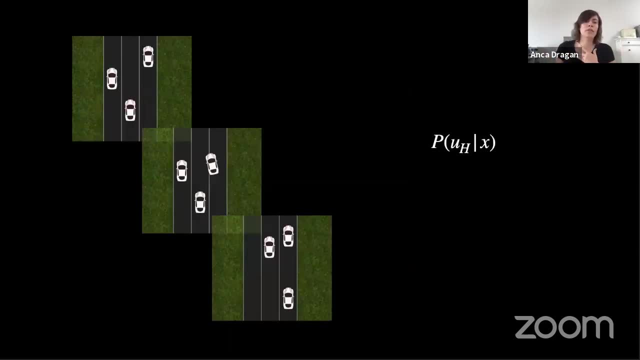 problem in driving. So what we figured is as what people were doing was. you collected some data And you can see here if you have a model of human driving and if it's a model that tells you what action a human would take in any state or what probability distribution over. 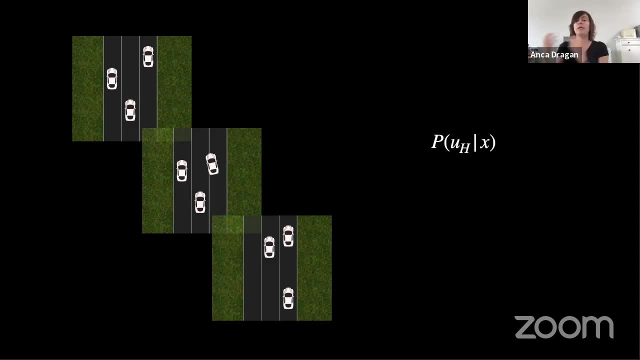 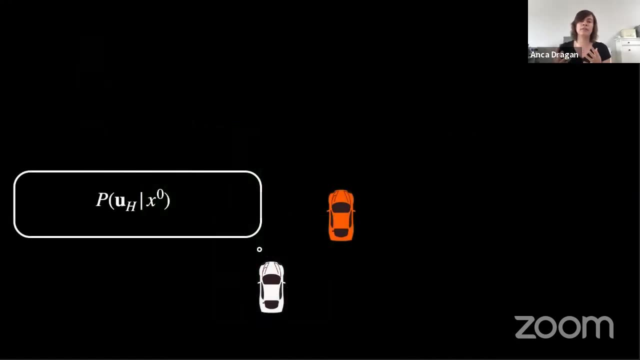 actions, And you know this would range from simple things like common filters, to planning based methods, to behavior cloning, to to what not. But then you know the autonomous car here. when in orange I'm going to use orange for the autonomous car in this talk, it would 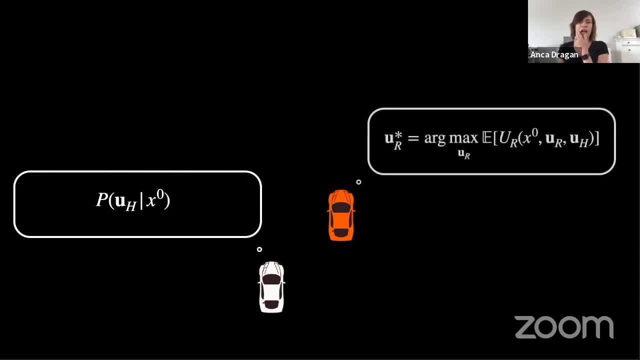 use that model to anticipate trajectories? Okay, and then it would plug that into its planner, which would then figure out how to maximize the robot's reward or minimize the robot's cost, if you're depending on whether you're optimistic or pessimistic. um, and that, of course, that cost included, depended on this prediction where you 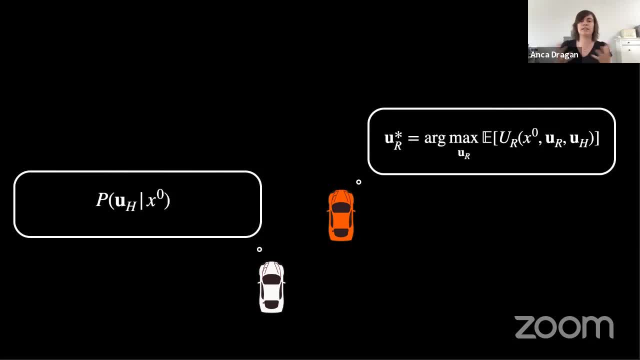 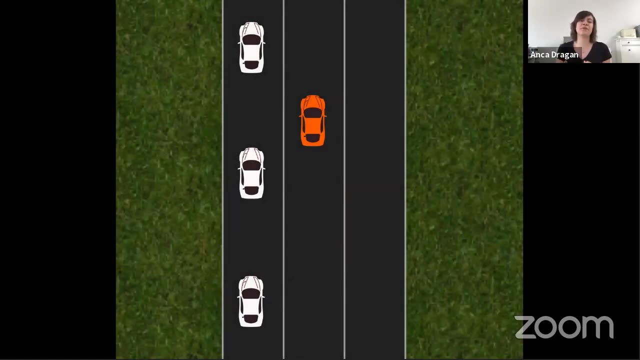 think the person was going to go um, because you wanted to, at the very least, stay away from the person um and so, um, this seemed like the framework that, uh, was kind of the standard, and this is odd, because just imagine any kind of situation where you have some traffic right, so say, 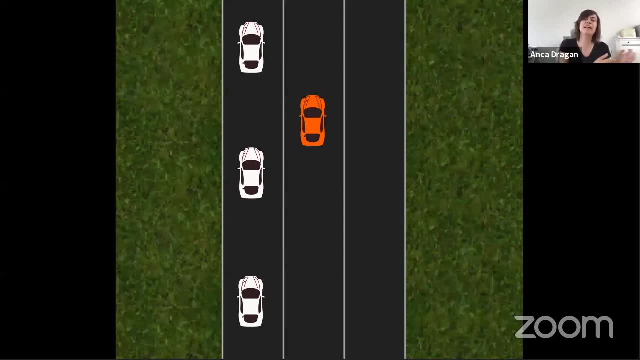 the car needs to go into the left lane to later take a turn. any prediction algorithm, in this case, would be able to predict where these folks in the left lane- uh, what they're going to do. they're going to keep going straight, so the car can't go in between them. 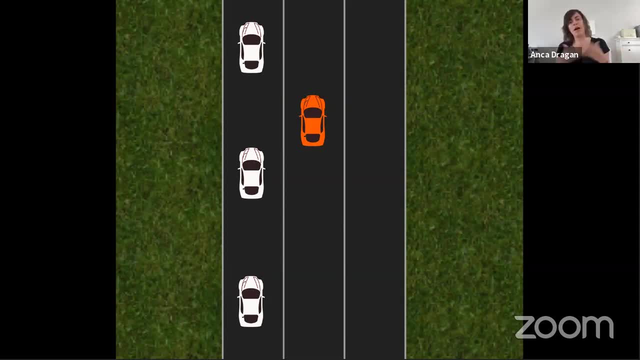 so now the car has two options and they both suck. so one option is to keep going and then miss the turn and reroute, or the other option is to slow down and wait for a big enough gap in traffic. um, but of course that makes a lot of people behind it angry. and the thing is, if one 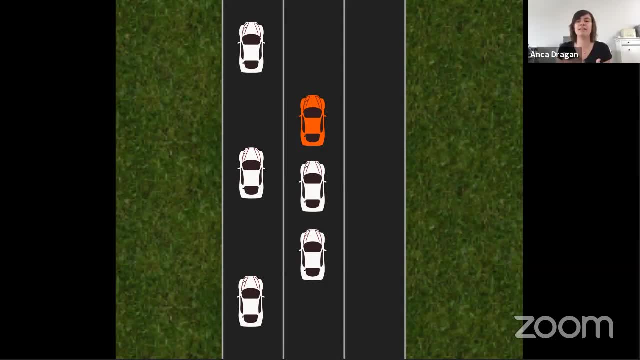 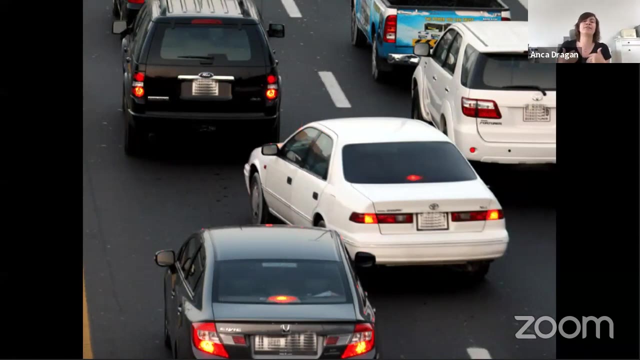 of us- any one of us, would actually be in this situation that the orange car is in. we would not accept being stuck and with one of these two options, we would invent a third option right, which is to nudge ourselves in there, because we know that the person behind will see this and we'll slow down and make. so that's how we got started on. 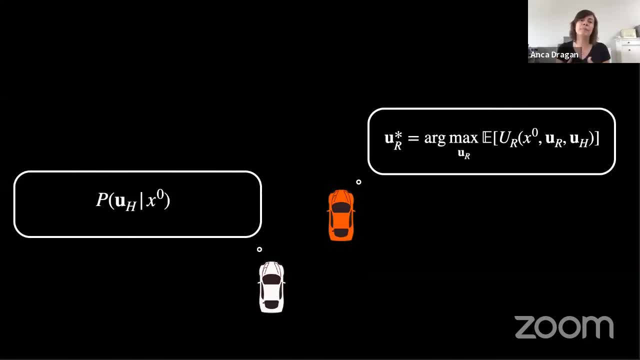 this notion of having prediction be in the planning loop. uh, we realized that when we're doing prediction we're kind of implicitly assuming that the human acts as if they're in isolation, not accounting for the robot. but in reality, of course, people very much take the robot into. 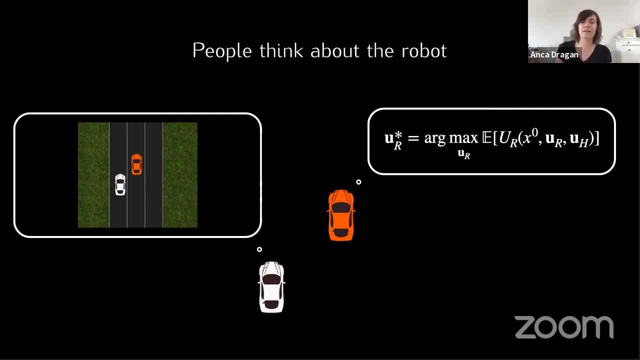 account. now i'm not saying that nobody had ever thought that cars, um, and what cars do influences what other people do, um, obviously, industry at least had to deal with this in some cases, because just imagine i having your autonomous car be in front of the person. if you stick purely to this framework and of prediction and then plan. 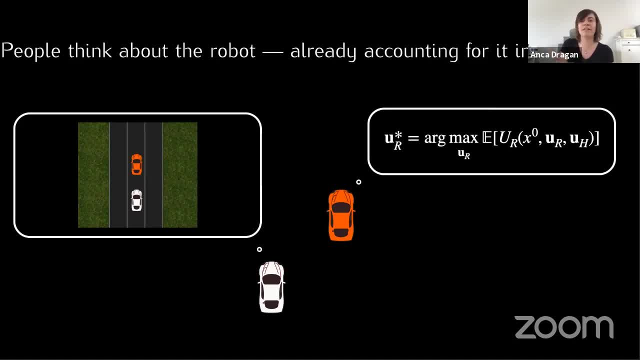 um, you won't figure out that you. it's okay to stop at a red light, because if you slow down and you don't think that it has any effect on the human behind you think that the human kept going and collide into you. so you freak out and say, well, i 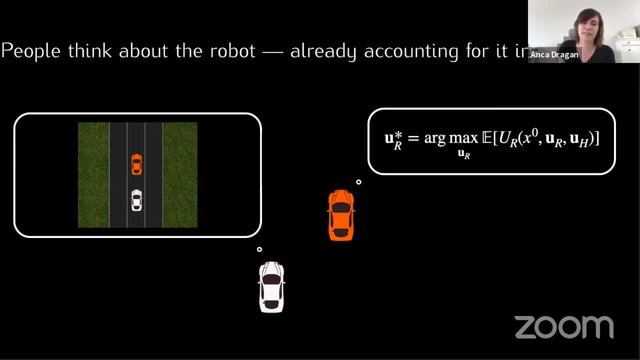 can't? you know? i have to run the red light because i can't actually avoid collisions otherwise, and so of course that that that's not how cars would work. but the thing is, it's part of the law to slow down and not hit the person in front of you, and so it's kind of easy to adjust predictions with that. 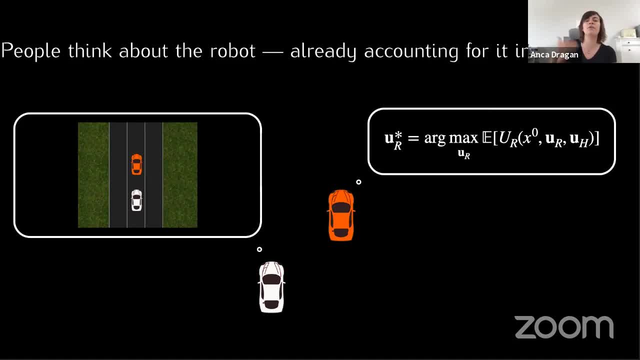 uh, without really capturing how the car, the human driver, is really responding to what the robot does, and there's no law that says: you know, people will slow down to let you merge in. They don't have to do that, So what gives? So you might think that you can solve this by having- and we did. 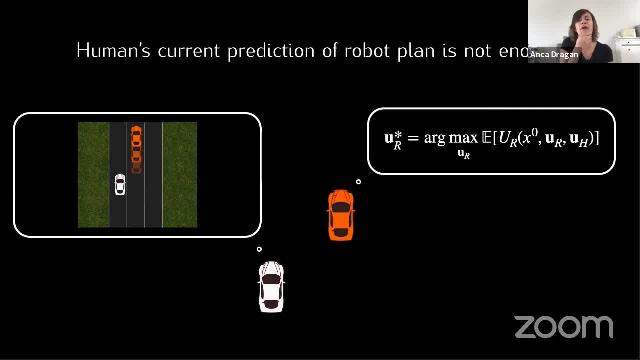 back in the day. let's just solve this by having the human prediction. Some might be based on what the human predicts the robot will do So the human prediction, the robot prediction, and then the human would sort of respond to what they think the robot will do their own prediction of the 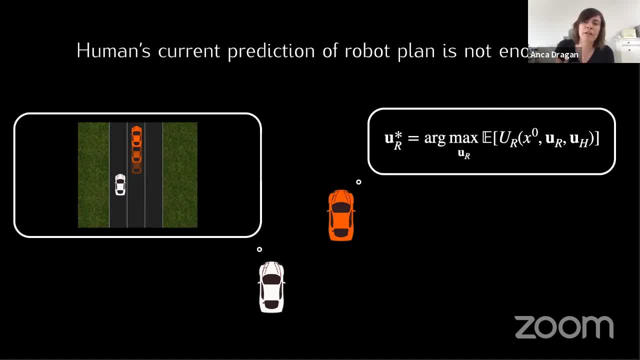 robot. But unfortunately that doesn't quite work right, Because here, if you haven't started changing a lane, the person has no reason to predict that you'll change a lane, which means that your prediction of them is still that they're going to just keep going forward, And so you'll. 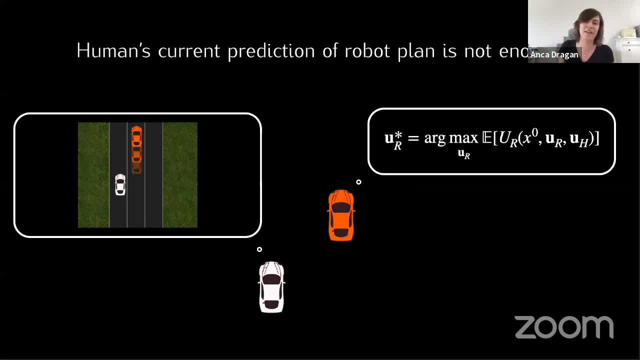 never start changing that lane to give the person a reason to slow down, and you'll be stuck in the same sort of thing again, And so the reality is that, of course, what we're trying to do is we're trying to make sure that the person is not stuck in the same. 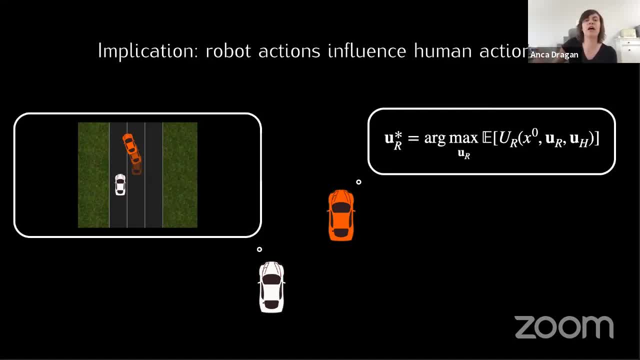 And so the reality is that, of course, what we're trying to do is we're trying to make sure that the robot plans on doing So. it's actual future actions, not what the human currently predicts that the robot will do. It's actual future actions affect what the person will eventually predict. 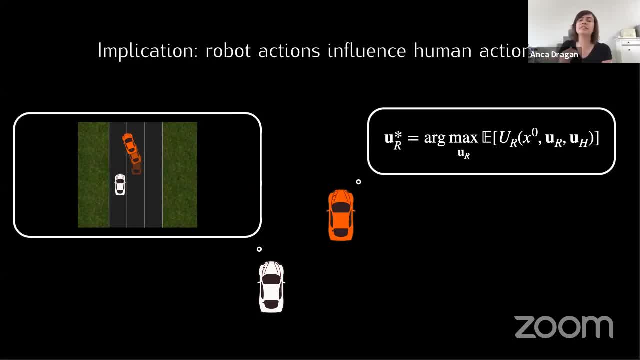 which then affects what the person will do, And, in other words, it's not just the current state and history so far that tells you what people will do. You actually need to account for the robot's future actions and how they will influence the future human actions, And so our first pass at 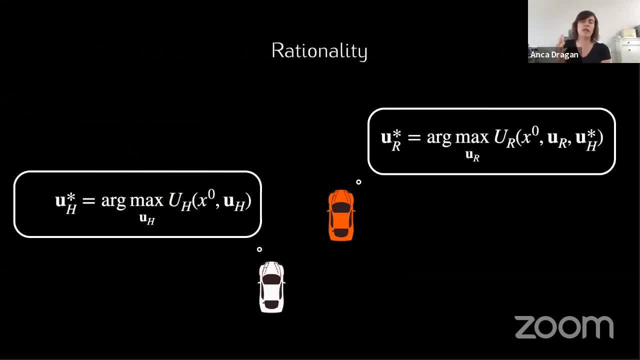 this started from the idea of what we're trying to do, And so we're trying to make sure that the robot's future actions affect what the person will do, And so our first pass at this started from this model that we were using in other settings as well, that treats people as planners. 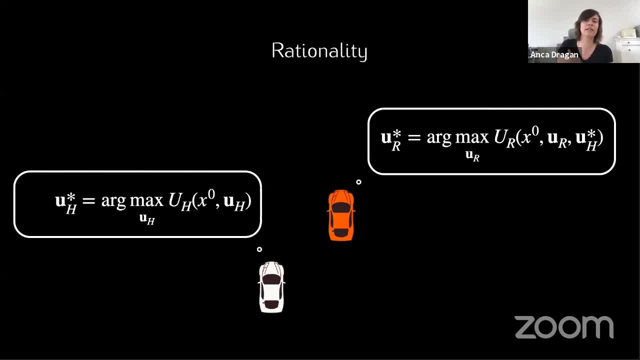 So the thought was that you could do some inverse reinforcement learning. You could learn a reward function that explains human driving And then online you could make predictions by essentially optimizing that reward function. So if you do that, let's say that recovery reward function is. 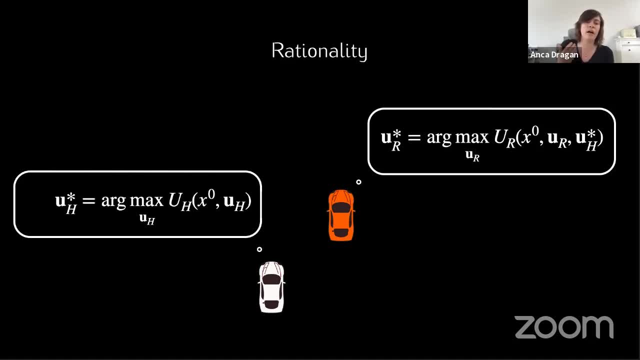 UH. You do that, you get your optimal trajectory for the human UH star and that's your predictive trajectory. Sometimes you might add some noise around this, You might do it for a different goal and have a multimodal distribution, But anyway, something like this, And so we started. 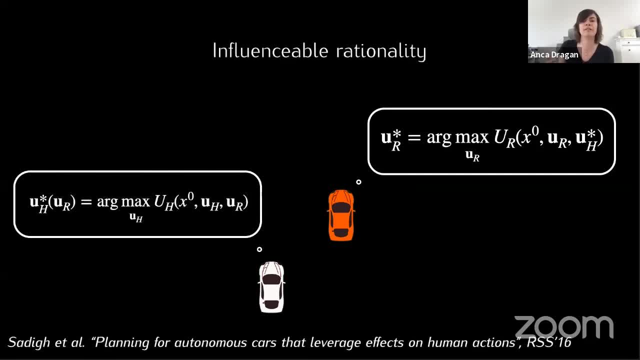 from such a model And we thought to capture the influence that the robot's future actions will have. we could do that by saying that the person's utility also depends on what the robot does, Because, for instance, the person also would like to avoid collisions with the robot, And so much. 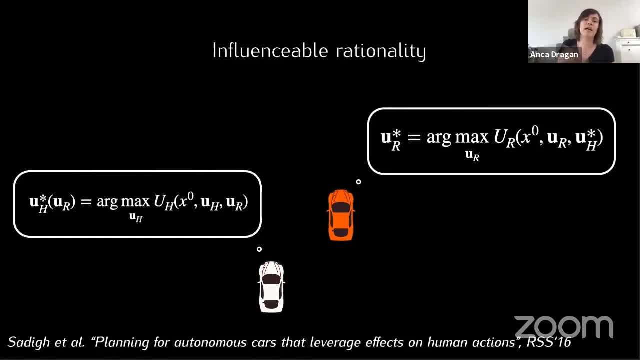 like the robot's utility depends on what the person's trajectory is, similarly the human's utility depends on the robot's trajectory. And so our model was: we essentially just conditioned the human prediction on the robot's trajectory, So we made it a function of the robot's trajectory. 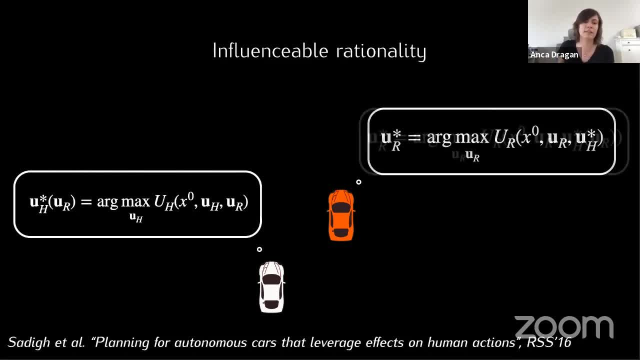 And now we computed the person's optimization in response to that. And now the robot would face this nested optimization problem, where it's planning for what to do such that when the person selfishly responds by optimizing their own utility, the combo of the robot's trajectory and the human's 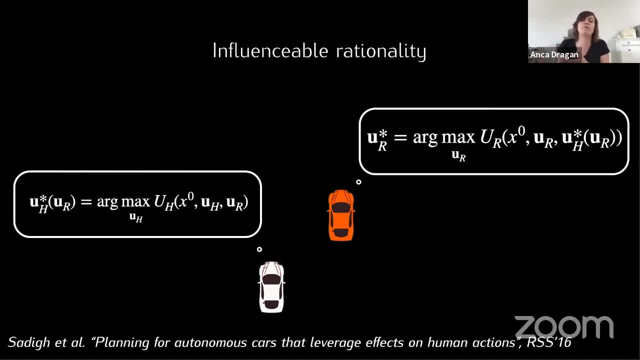 selfish response to that trajectory is a good combo for the robot's utility or for the robot's reward, And so we would solve this problem with projector optimization in kind of a receding horizon fashion. And it turns out you can do this because you can use implicit differentiation to 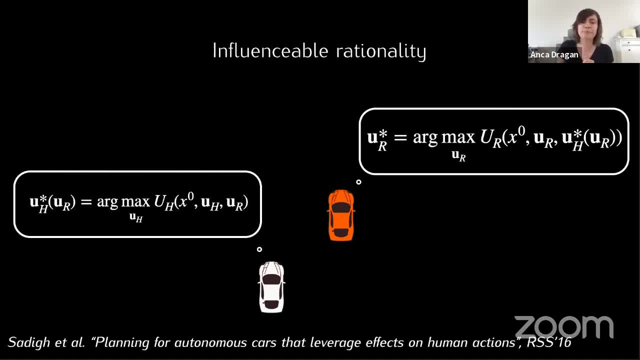 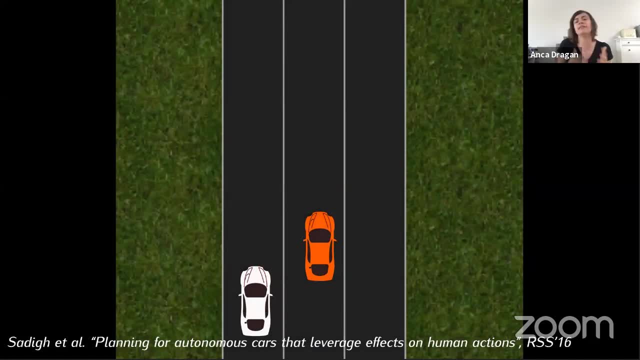 differentiate through the person's response, even though that's an mask. So that's what we did. Long story short. now the robot would consider. when the robot considers what to do, it has this gradient. So now the를 vastно, when the robot considers what to do, it kind of has this gradient right. That tells it how a 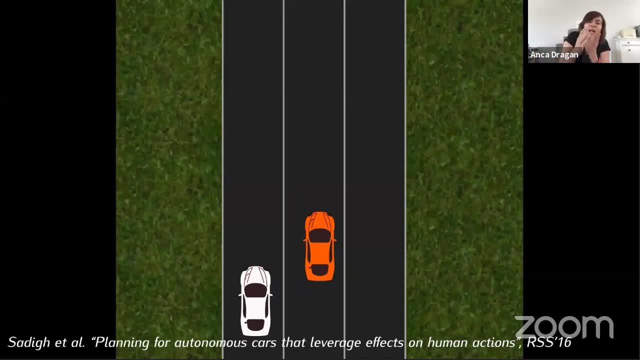 change in its trajectory, like, say, if it were to move slightly towards the left, how that would influence the human's trajectory and how maybe the person would slow down a little bit the more the robot goes to the left. So it has that gradient that enables it to figure stuff out And instead, 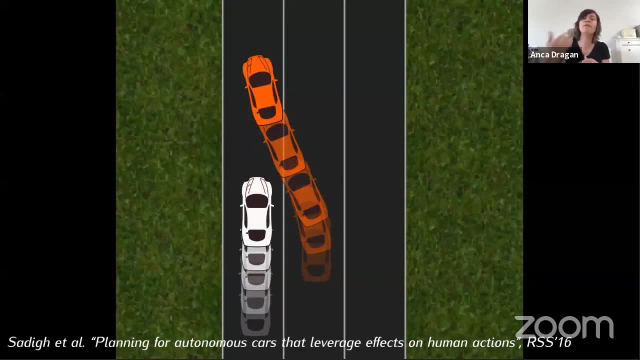 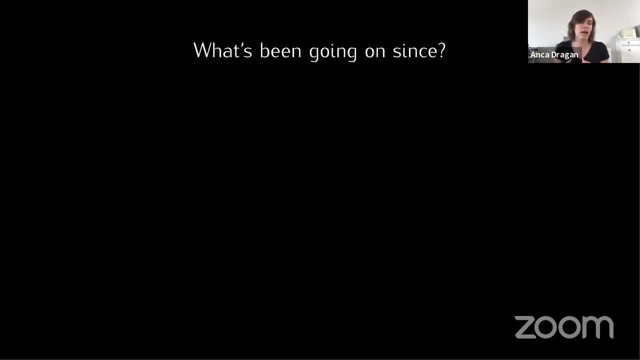 of bailing and merging behind it. you know it'll figure out that it can go in front of the human in some cases and expects that the human would appropriately respond by slowing down in order to maintain a safe distance. So that was back in 2015,, 2016,, right, Since then, I think there's 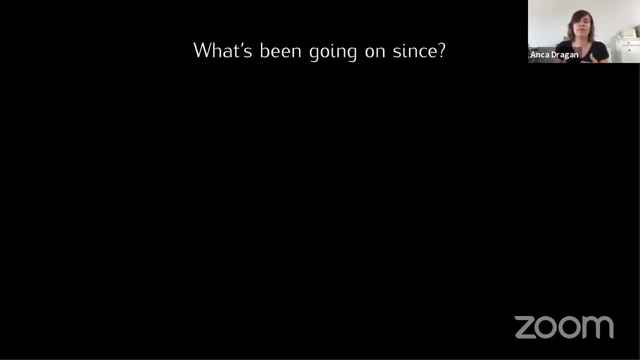 been a lot of work that really embraced this notion that there has to be a coupling between a prediction or forecasting, and planning or in control. And I want to call out: there's been great work from Rowan with Sergey. There's been some great work from Marco Pavona's group with 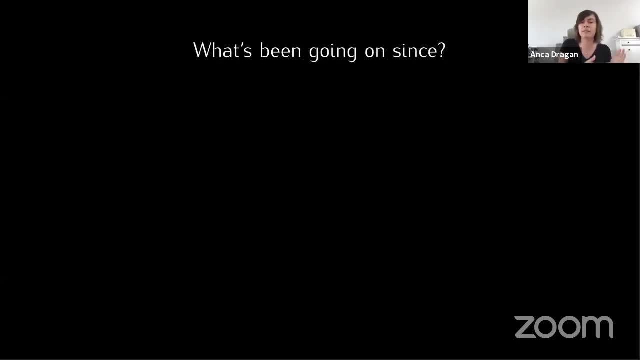 Ed Schmerling, Max Schrager's group and Daniela Russo's group. What I wanted to do today for the rest of our time together, is to share a little bit about how we've been continuing work in this in my lab and sort of give you two examples that I think. 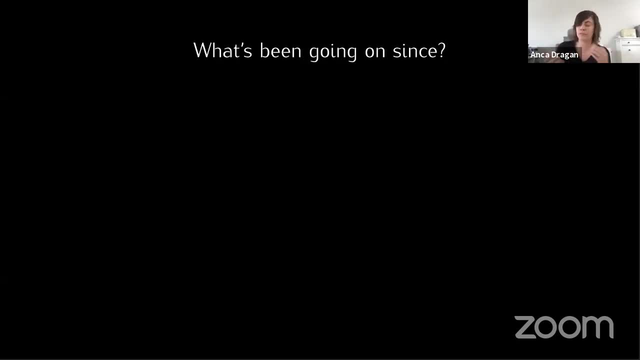 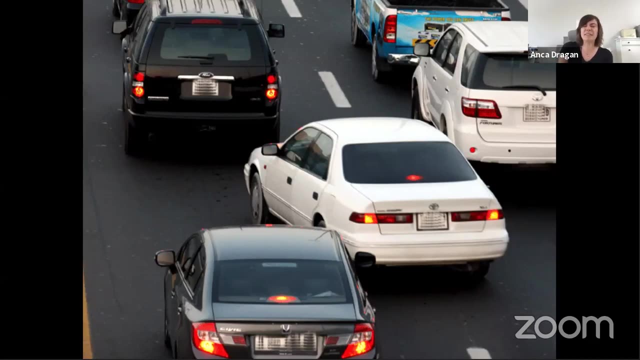 are very nicely complementary that continue this line of thought. So once Dorsa finished her PhD, there was something that really bugged me still, And it goes back to this example right of cutting someone off. So I do this nudging myself in in heavy traffic. I used to do it all the time. I don't do it now. 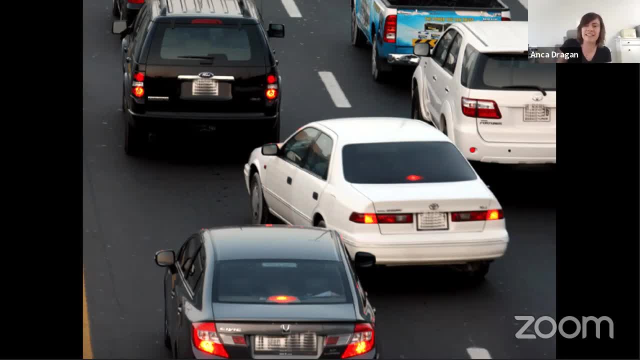 because I'm stuck at home, but I used to do it all the time on the Bay Bridge because traffic is crazy, So that's great. But at the same time, when I'm in the gray car and that car behind, you know, sometimes I slow down, but I don't always slow down, So you know what's going on. 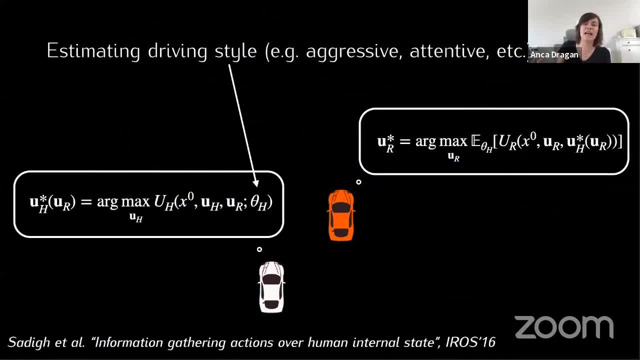 there And yeah, okay, we had captured this type of phenomenon to a certain extent via this notion of driving style that we had. We said different people have different trade-offs, right, that they make between efficiency and safety and such, And the robot we had the robot essentially estimate this driving style parameters. 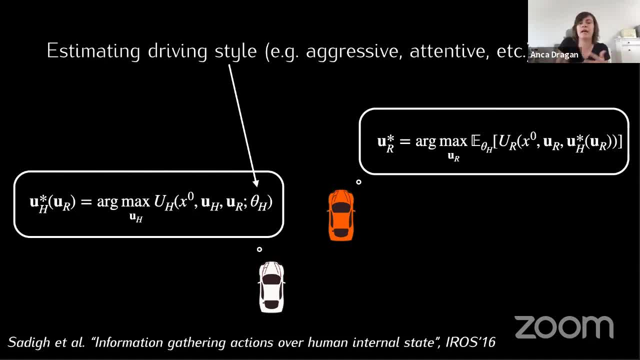 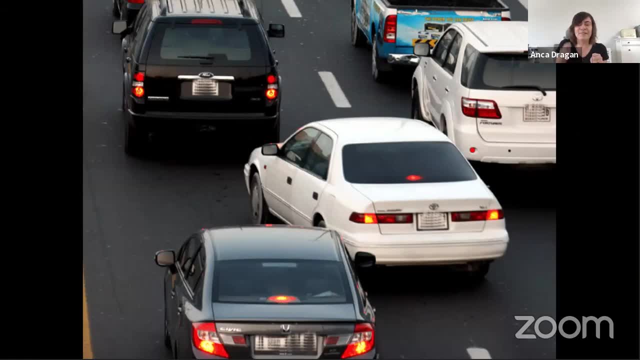 online. So if the person wouldn't slow down, we'd figure this up and figure this out and adapt to that. But here's what bugged me Sometimes when I'm in that gray car, in that situation, not only do I not slow down, but I actually accelerate, Like what's up with that? I accelerate because 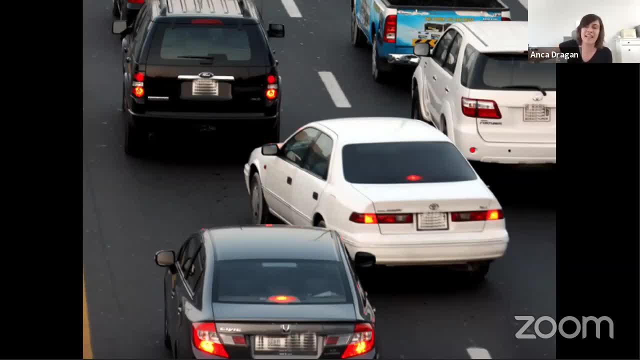 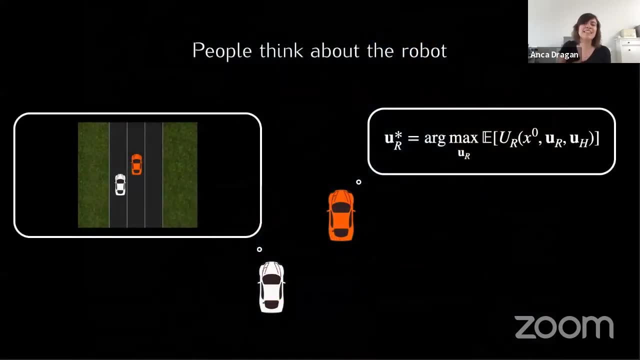 I know that if I accelerate, I can deter the person from getting into my lane and get them back into their lane. So the thing is that, yes, people think about the robot and they react to what the robot does, but they also know that the robot thinks about them and reacts to them, And that 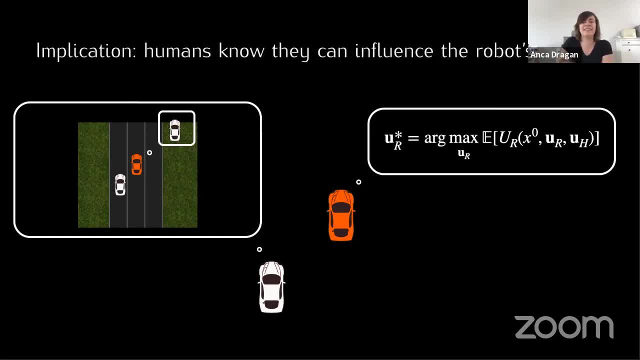 means that they will sometimes try to influence the robot rather than just accept the trajectory that the robot planned and call it a day and react to that. And this is really concerning right, Because now that can lead to a loss of safety if we're unable to anticipate that, if we're 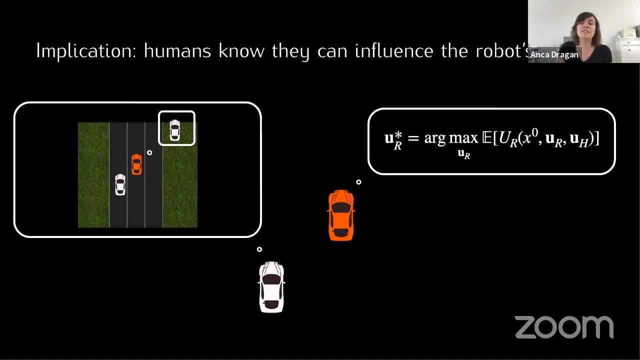 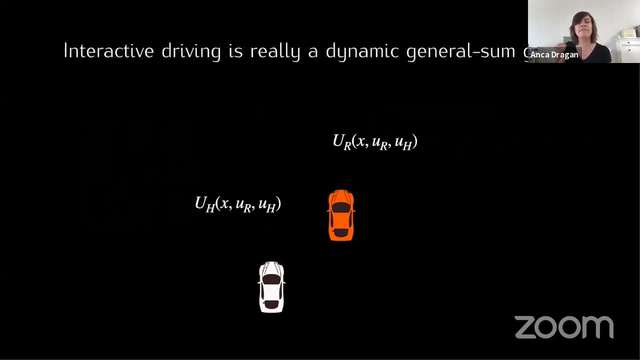 unable to model or capture that. So- and of course I could go on. Now the robot should know that, the person knows that the robot reacts to them, And then the person knows that, the robot knows that the person knows, and it's just turtles all the way. So what's happening here is that whenever you 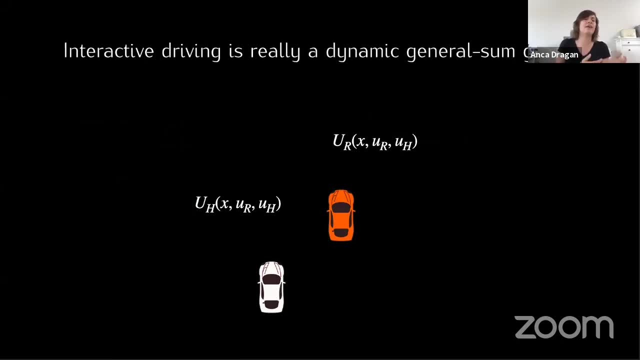 have two agents, both making decisions that are incentivized by some utility or some objective. what you have is a general sum game, And it's a dynamic one, Meaning, if you've mostly heard of games and in the setting of a one-shot game or a repeated game. 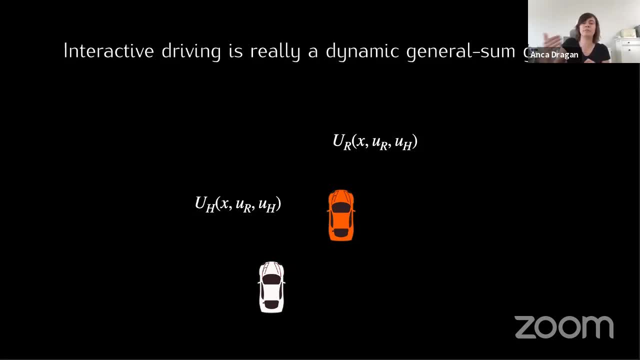 that's not really going to cut it here. This is a dynamic game because the problem is sequential. right, With an action now, I'm influencing what the state looks like later, which influences decisions that will be made later. So this mutual influence between the human and the robot is not 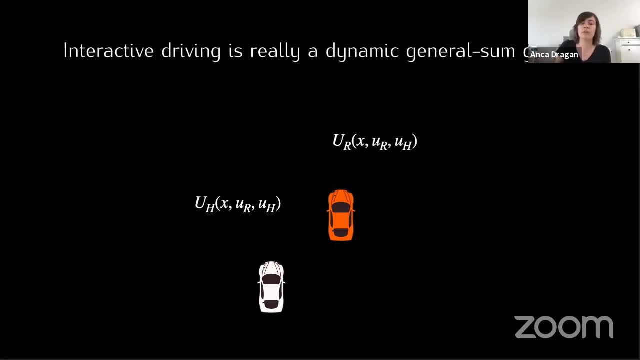 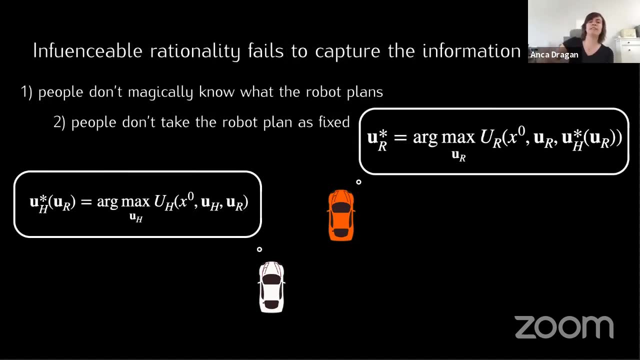 one-shot. it's actually, and it's not even repeated. It's really playing out over time, sequentially, And so when, kind of going back to this notion of influenceable rationale, the person responding to what the robot plans on doing when we model that we were. 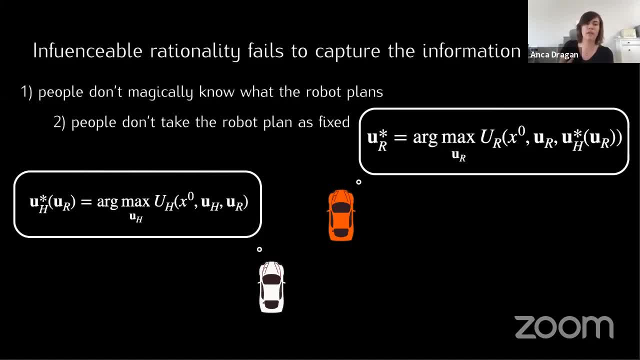 basically, we messed up the information structure in the game in two ways. Number one: people don't magically know what the robot plans on doing. So, even though they will figure out eventually that the lane change is happening, that's when they'll start responding. They won't. 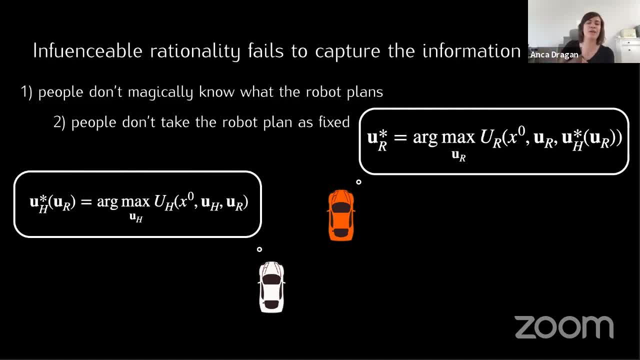 they don't know now that the robot plans on a lane change, so they don't start responding right now. That's one issue. The other issue is that people don't take the robot's plan as fixed. They know that they can actually change and influence the robot. So this other student, Jaime Fisak, 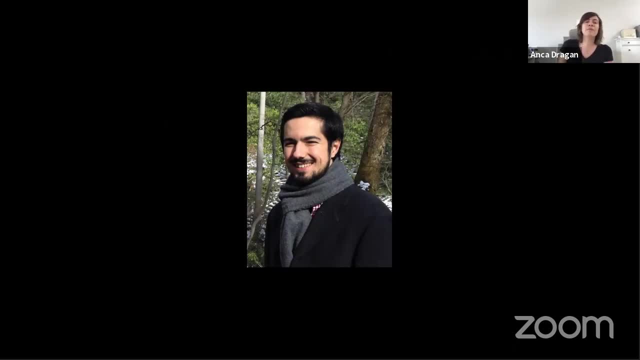 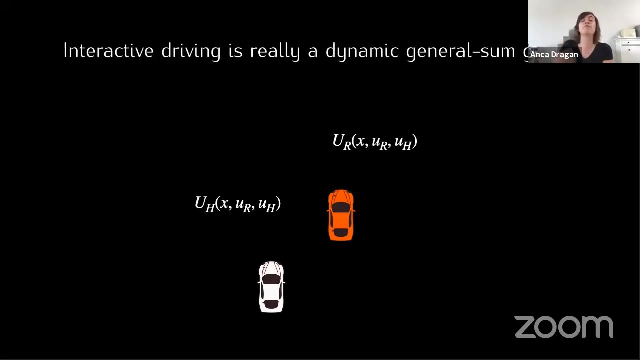 he had a lot of experience in game theoretic control and he took up the challenge of fixing this, of seeing how we could get cars to better approximate the solution to this game in ways that influenceable rationality wasn't really cutting it. And so to understand that, just to 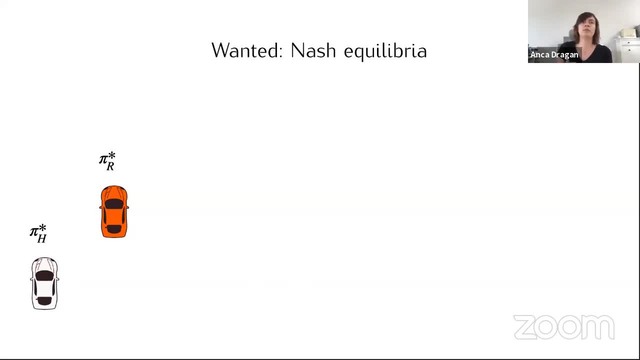 be clear about what that means. what we want is we want to find a policy for the robot and one for the human that form a Nash equilibrium. So it should be the case for the robot that its policy is optimal if you hold the human's policy fixed. So if this is the space of policies for the robot, 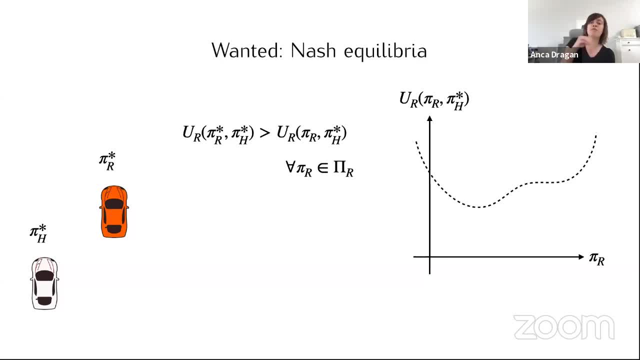 and then on the y-axis, we have the utility to the robot from that policy. when combined with the human's policy, it should be that the robot's policy is the global optimum Right, Meaning that the robot has no incentive to change its policy from that if the human 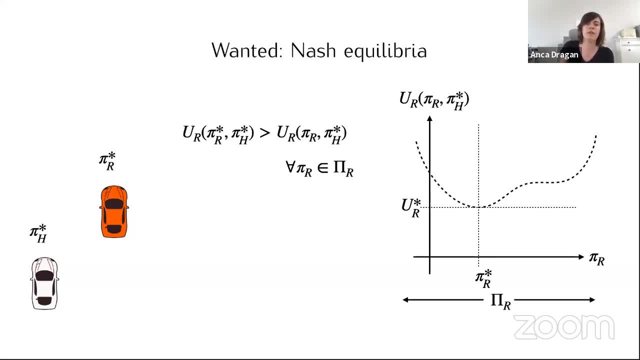 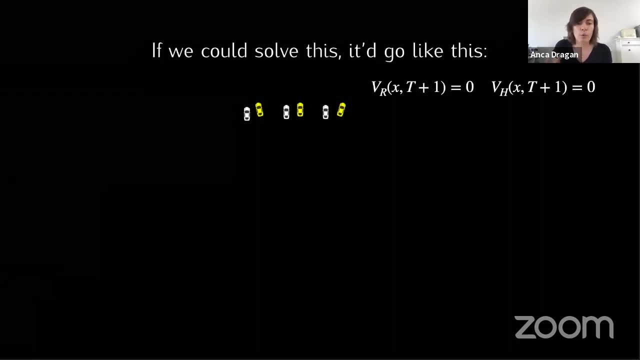 doesn't change their policy, And the same should be true for the person. So that's what we want. We want a Nash. So to solve this we'd have to do something like this: We'd start at the end of the time horizon, We'd initialize the human and robot values to zero, And then we start going back in. 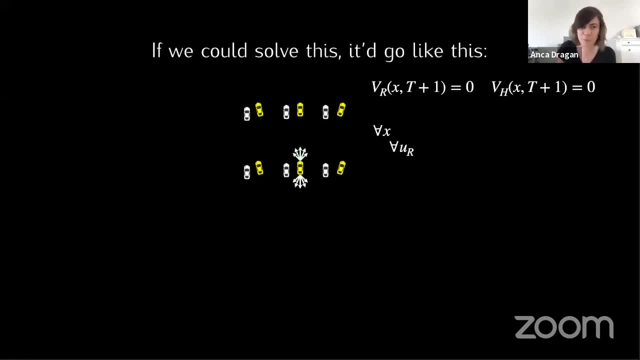 time. So for every possible state, for every possible robot action, for every possible human action, we'd compute a Q value function based on the reward of that one action plus the value at the next time step of the resulting state, And this would give us also a distribution over robot. 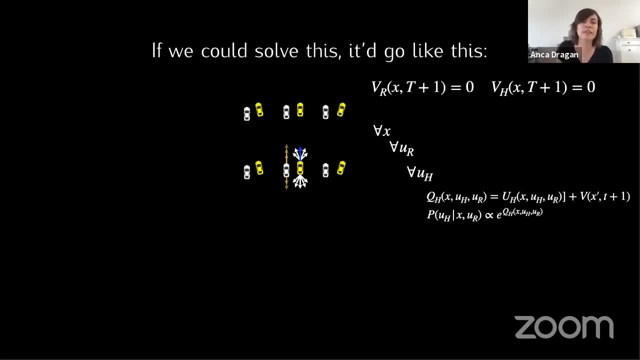 action. So if you wanted to account for something like noisiness in the person, you could say you could use this very standard model that says that people are exponentially more likely to take actions that have higher Q value, And so then you would be able to compute the robot's Q value by. 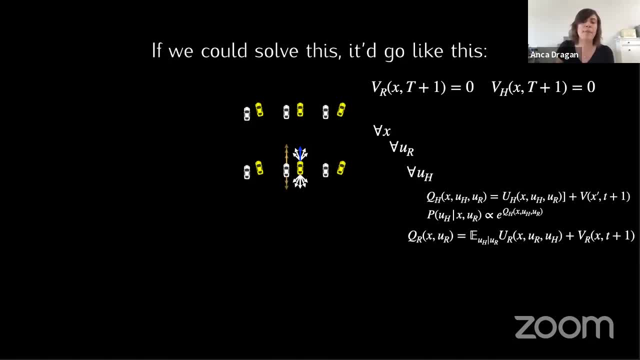 looking in expectation over time, And so that's what we're going to do. And then we're going to convert that distribution and looking at the reward for the robot from that combo of actions for one time step plus the future value, And we'd be able to then compute the optimal robot action and 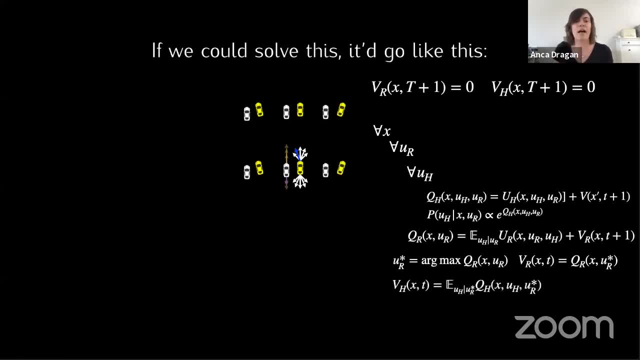 update the time varying robot value And finally update the value to the human. And again, do this for backwards in time every time, for every state, for every action of the robot, for every action of the human. So keep doing this backwards in time until time is zero. 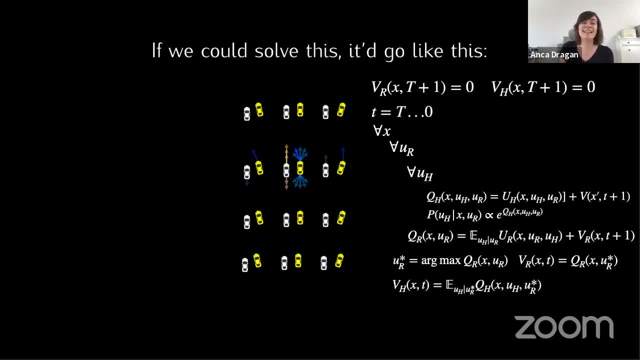 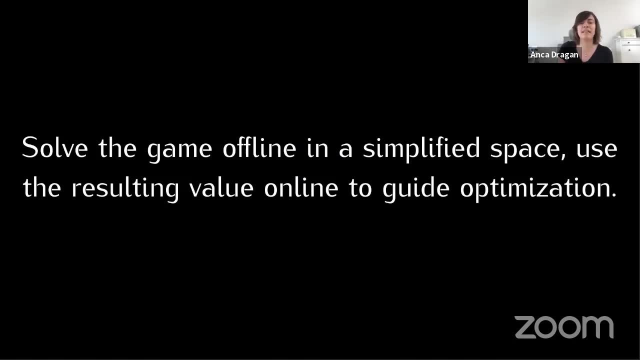 Now, obviously this is not going to work in continuous state in action like we have for cars, And so Jaime had this pretty simple idea: What if we solve the game offline, in a simplified state in action space where we could actually run this dynamic programming, And then online we'd figure? 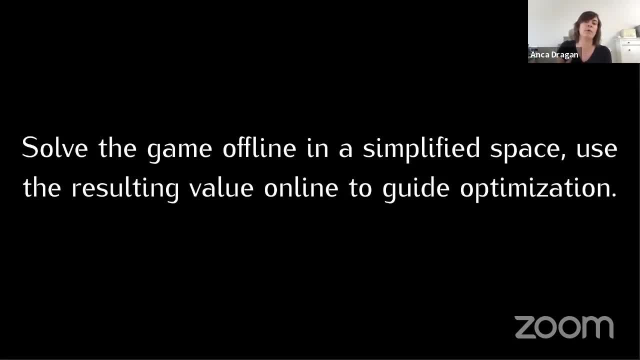 out how to use those resulting value functions to influence or guide the optimizer. So if you're familiar with games in AI, you're going to be able to do this, And then you're going to be able to do this, And then you're going to be able to do this, And then you're going to be able to do this, And 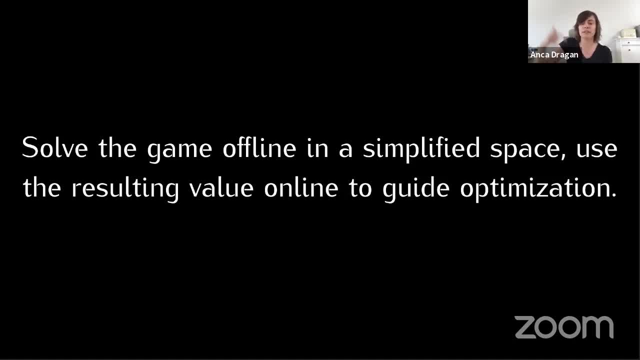 sometimes we refer to this as computing an evaluation function. So it's this thing that you stick at the end of your search tree if you don't want to go in more depth. And, similarly, here we're going to be in continuous land, so 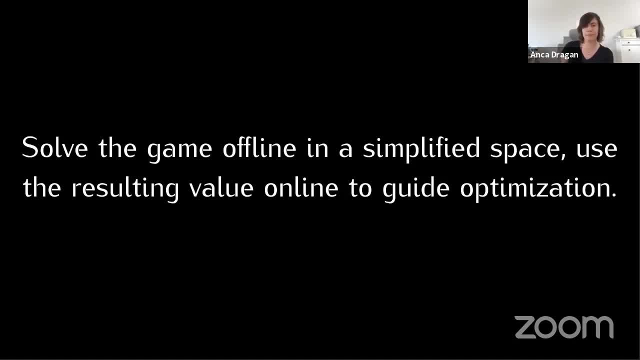 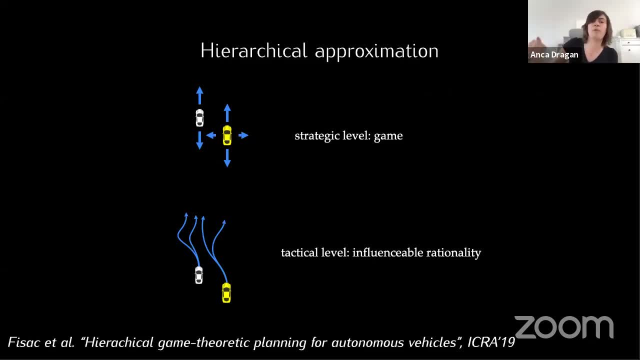 we won't have a search tree, but we'll use this as our cost to go for our optimizer. Okay, so this is our approximation to the game. It consisted of this strategic level, where we would solve the game using dynamic programming in a dumbed down, discretized state in action space, And then we'd have a tactical level that actually 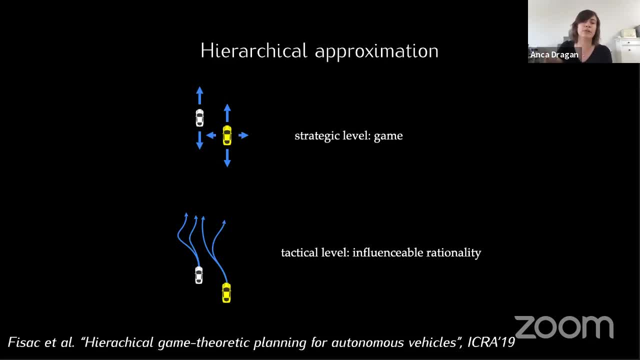 did the work using model predictive control, using optimization and using influenceable rationality or sort of our best kind of guess at capturing this influence. But we would do that for a short time horizon and that would be guided by the strategic level. So the strategic level- here we only cared about the car's position. 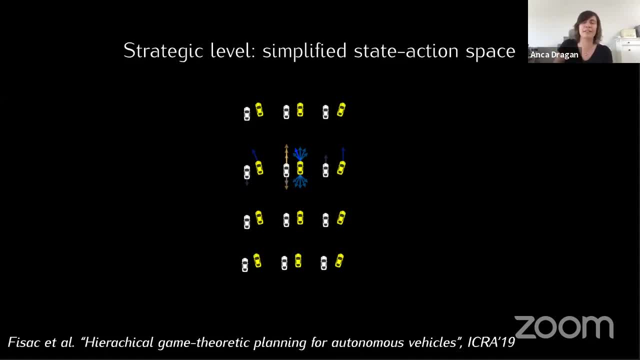 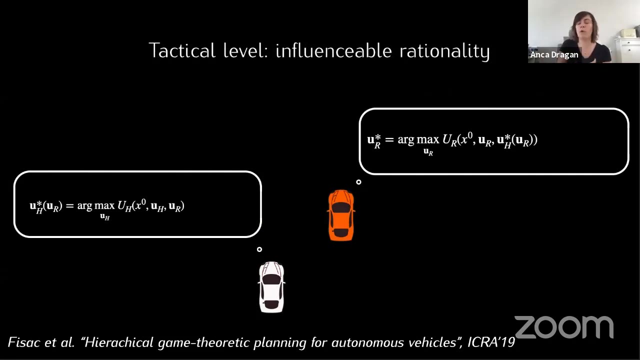 and not orientation, And we assumed that we can directly control velocity. so our dynamics was megalosimplified And of course this is an implementation choice. but you sort of want to do here whatever you can actually be able to run dynamic programming, And then at the tactical level we do the same thing as before. the thing that 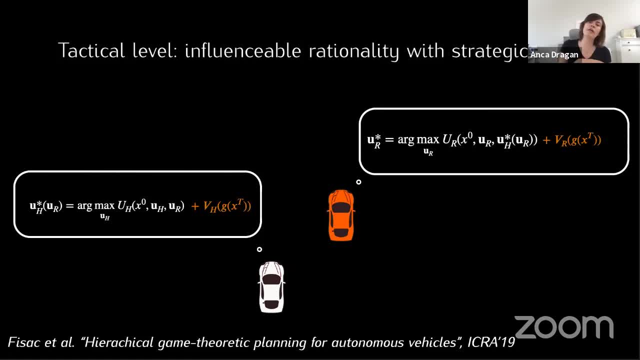 Dorsa did. But now each optimization on the human and on the robot side, we use the computed value from the offline dynamic programming as the cost to go. So we let the value function, kind of guide this optimizer using the higher level strategic information, And I'll share with you that from a practical standpoint this wasn't just cool because it 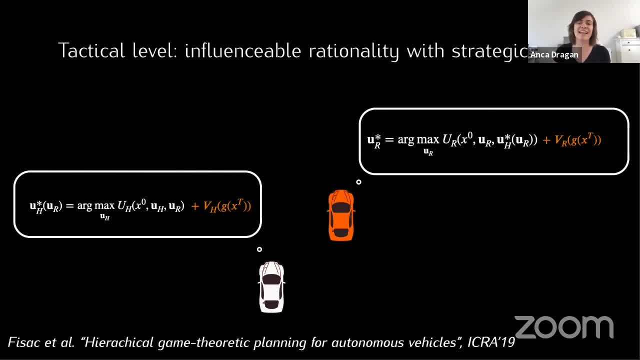 captured the game, But I guess one thing that we noticed was that it it was a great way, as you might expect, to alleviate the optimizers myopia- We can never plan for a long enough time horizon- And and also we were computing, we were using local optimizers, right. 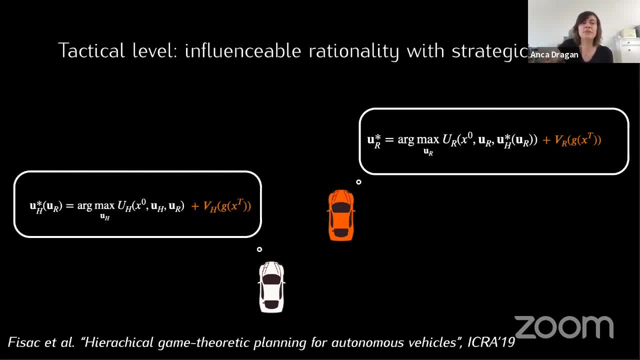 So we computed local optima And these issues, this we were running in, these issues like when the car wouldn't be able to figure out an overtake as the horizon wasn't long enough to figure out that it could actually get back into this lane, And 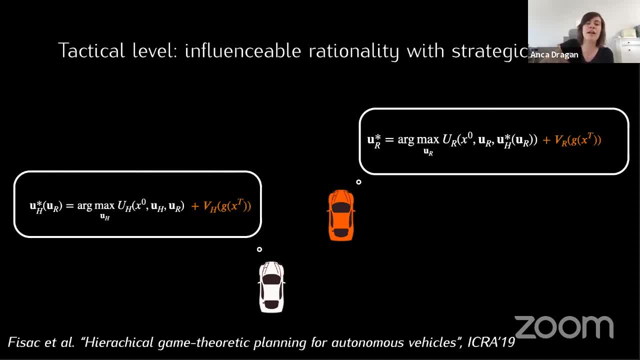 would work out for it, And so we also got a lot of benefits from using this value function, just from alleviating these issues on the optimizer itself, besides the guiding from this strategic interaction level. So I just wanted to make that point, And even if you 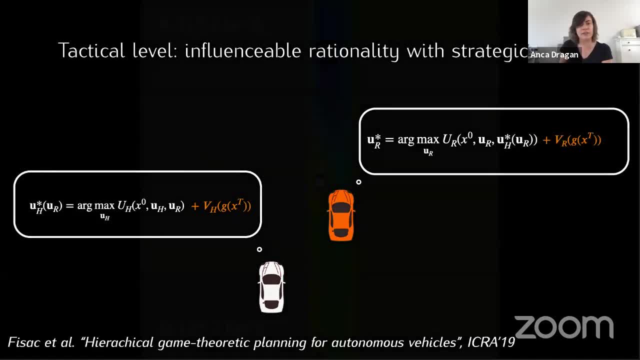 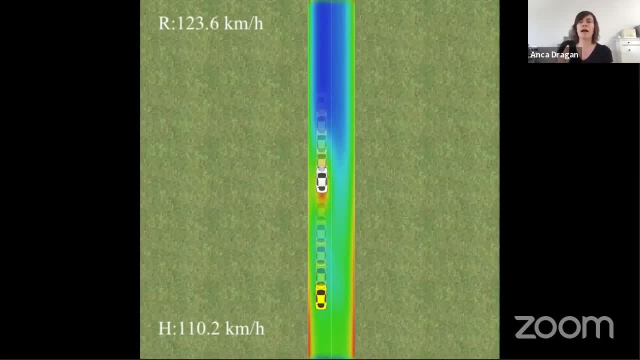 don't want to solve a game, this seems like a useful thing to do. So now some beautiful strategies kind of emerged. So you have the car in the back. So this is a computed solution here. The car figures out that it can go and kind of deter the person to go out of the way. 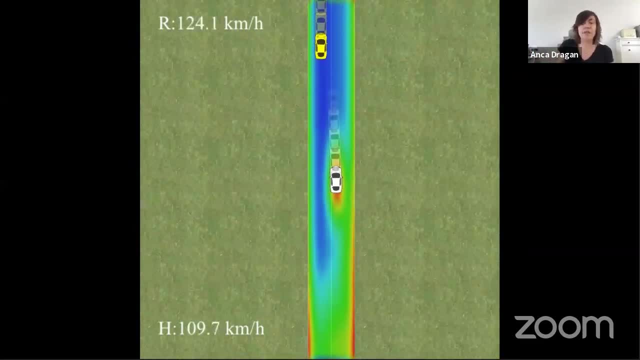 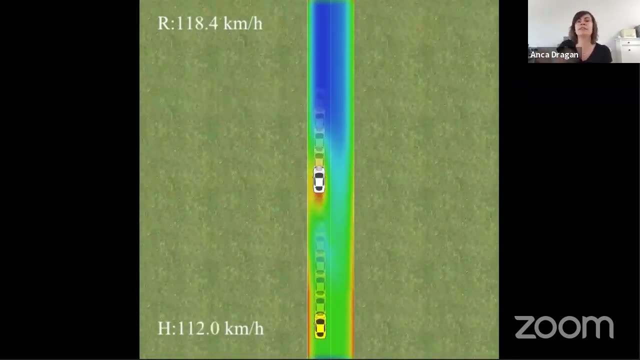 and change lanes to the right so that it can keep going. And if they do that that's great, But if they don't, that's also OK. So what happens is the car kind of attempts this, The person is not reacting, And then the car ends up doing an overtake. 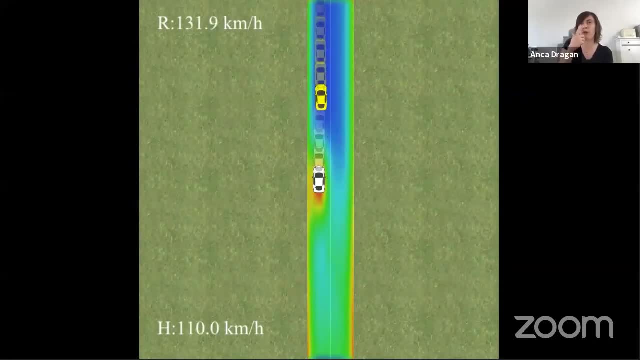 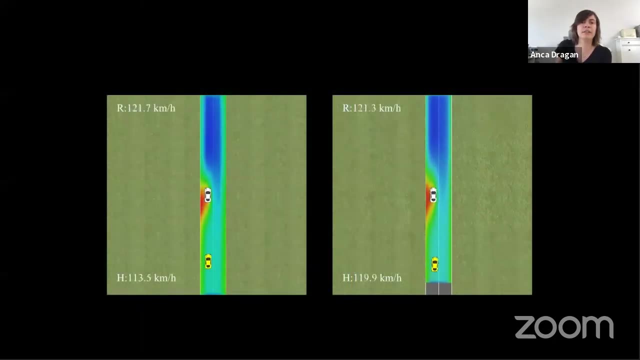 And then the car ends up doing an overtake And the heat map you see here, that's the value function for the robot, And then this is a really- I think, the coolest example. So here let's focus on the left first. So on the left, what happens is the car. 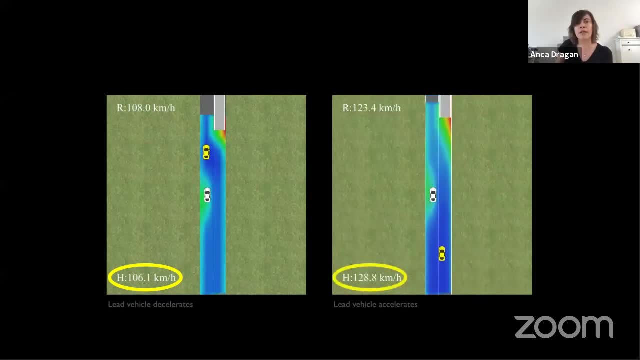 there's these obstacles coming up- And I'll go back and play this again if I can, Maybe not. So the car does this overtake, expecting that the person would slow down, and the person does slow down, And then on the right, it's really interesting. So here on the right, 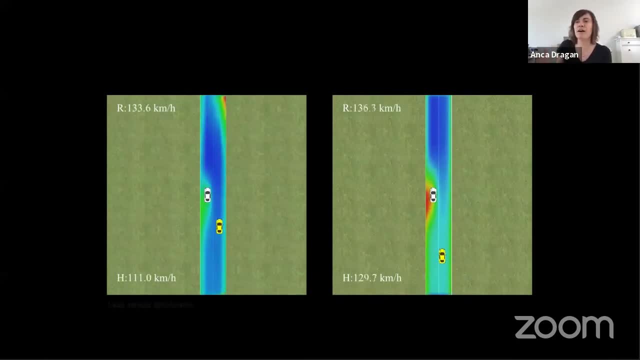 let me do that again. So let's focus on the right hand side now. The car goes, It does this, It tries to do this thing, but the human actually accelerates to deter the car and the car has to slow down and go behind. So I love seeing, like now, this, when we got these sort of results. 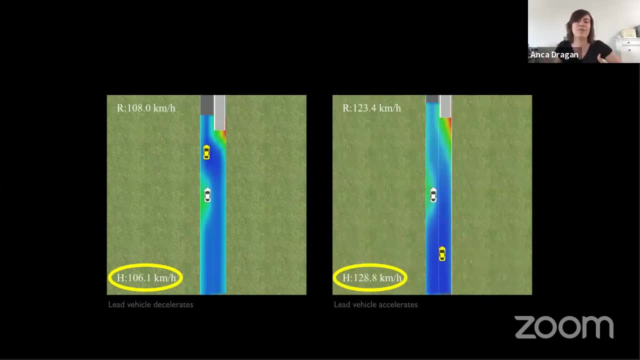 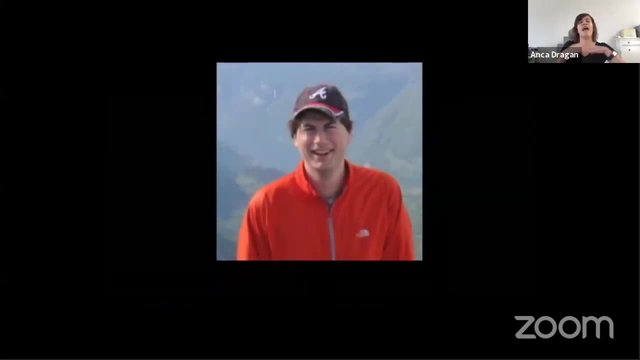 it actually felt to me like coordination and negotiation was happening and these planners are able to do that, So we're going to go back to this, And then the car goes: it does this, It's to handle that, so, um, anyway. so that was Jaime's story and again the idea here was that we could 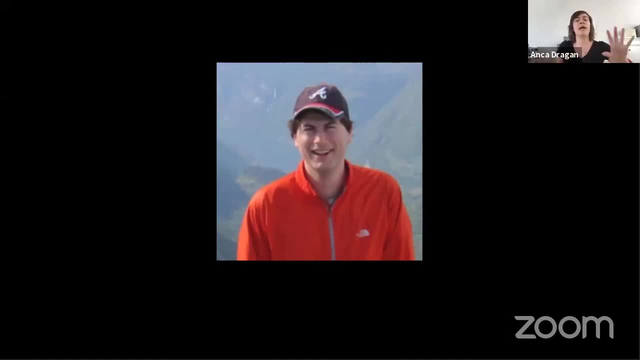 get close to solving the game if we, if we approximated the heck out of it offline and then guided, use that to guide the online solution. and then the last story that, um, I wanted to share with you was David. so David Friedrich College, he's actually a student with Claire Tomlin, but we 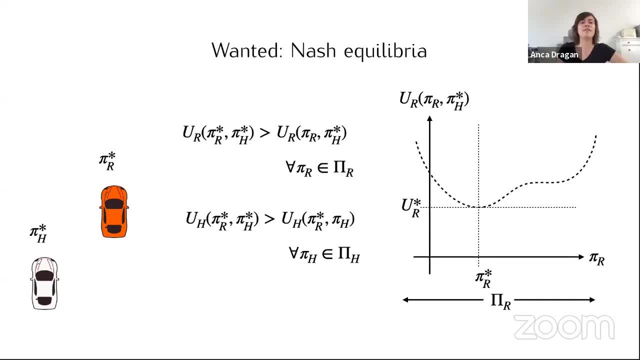 were collaborating on this project together. and um, he took a very different- and I say complementary- approach. so remember that what we wanted to find in these general sum games was a Nash and um. when I say a Nash right, what I define is a global Nash equilibrium, and we're in continuous 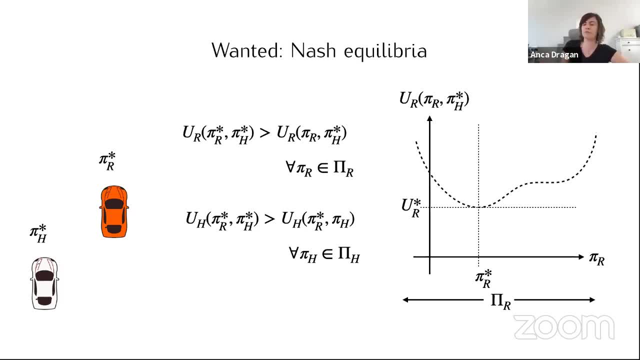 spaces, high dimensional problems. so of course the global Nash is out of reach and the, the hierarchical approximation, was one way to get towards some version of that. but David thought what if we went about it a different way? what if we, from the get-go, stopped asking for a global Nash because 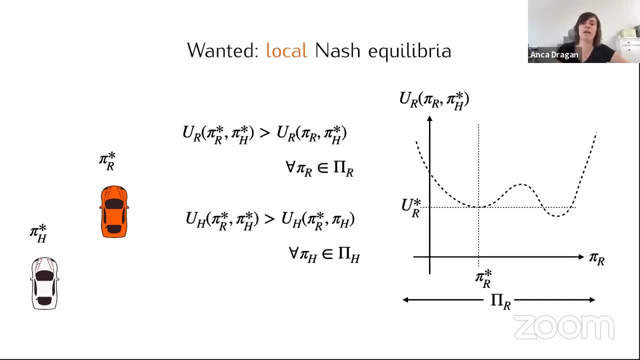 we know we're not going to get that and understood that all we might hope for is a local Nash. so a local Nash works similarly to the global. a local Nash, um, here the policy only needs to be best in a local neighborhood as opposed to global. so, going in with this mindset, David had this: 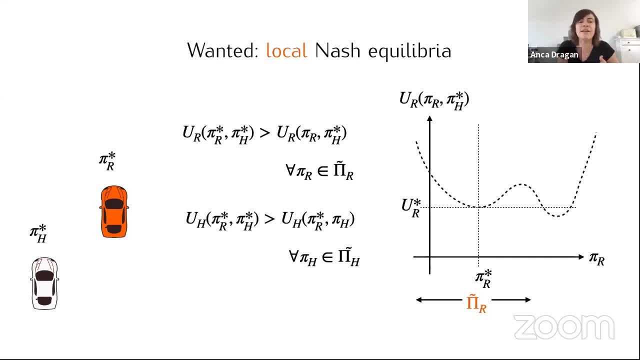 really clever idea, and the idea is honestly so obvious in hindsight that I thought were sure someone had must have thought about this. we didn't find a paper and so we wrote one. but you know, who knows, it might be out there. but here's the idea. um so David's observation starts with: 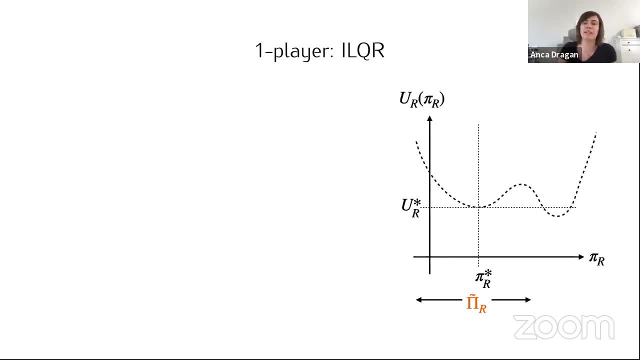 this analogy to single-player problems. so this is your standard optimization here that you want to do: single player, no issues, um and uh. you know, so far we've talked about kind of gradient-based methods. that's what we were using to solve these problems, like, for instance, when we're doing 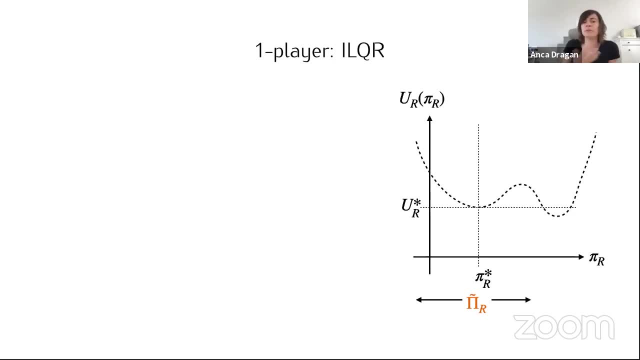 prediction of the human's trajectory for influenceable rationality. we're doing a lot of kind of gradient-based methods. but we're also doing a lot of kind of gradient-based methods. we're using gradient-based methods, quasi-Newton method, So we're using the gradient to approximate adhesion. 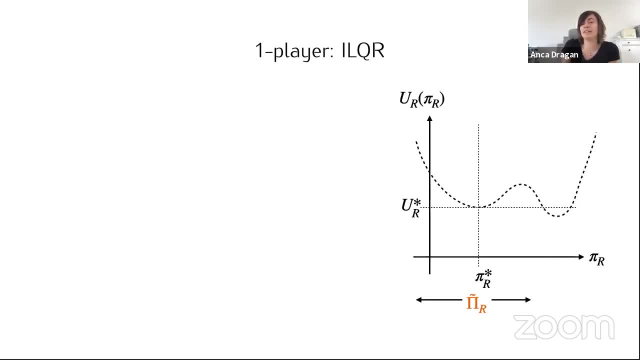 But there's this very widely adopted technique in the driving domain, which is ILQR- iterative linear quadratic regulator. So the way this works, if you don't know about it- and I'm sure most of you do- you end up you start with some initial policy. 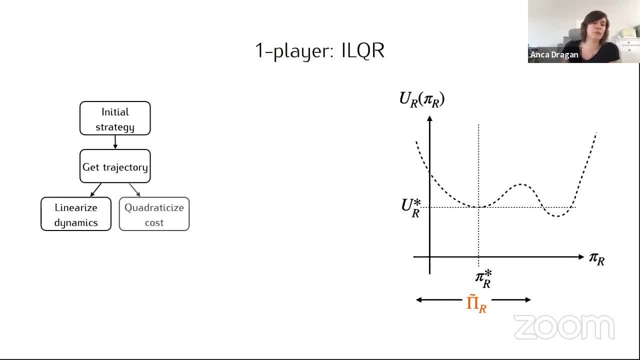 you get a trajectory by rolling that out, you linearize the dynamics, quadraticize the cost, and, lo and behold, now you have a wonderful problem with the quadratic cost and linear dynamics, which we know how to solve very well, And so you'd use that to update your strategy. 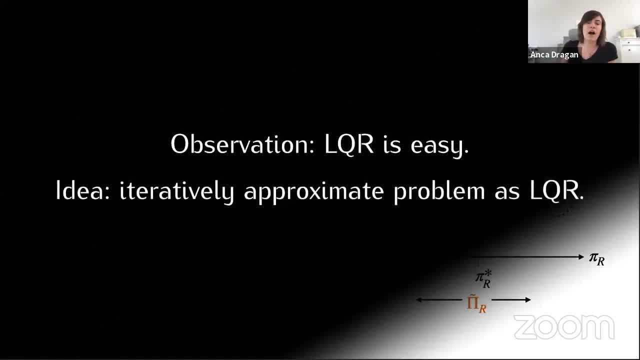 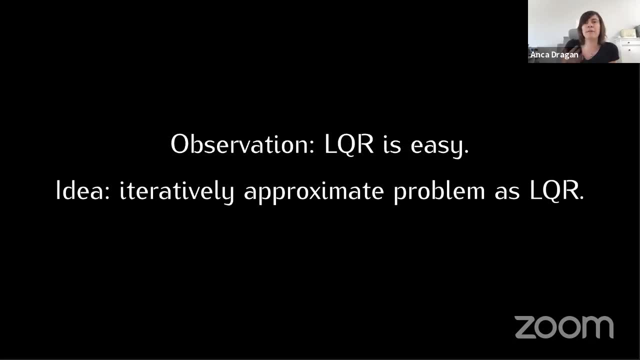 and do that iteratively. So the observation in ILQR is that, well, if I have linear quadratic problems, that's really easy. So let's just use that leverage, that easiness, and iteratively approximate the problem as an ILQR. 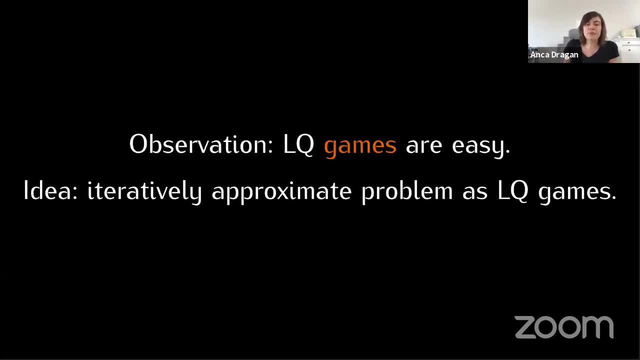 And David noticed: hmm, this is true for linear quadratic games as well. Linear quadratic games are easy. The world is beautiful when you have quadratic cost and linear dynamics. even in games, it turns out, And so the idea was: let's iteratively approximate the problem as an ILQ game. 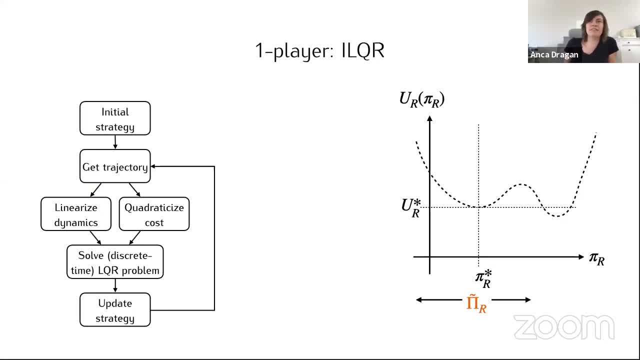 And so we do what we do in ILQR, except that you get to this point where, whoops, my animations are a little messed up, sorry about that. So you still linearize dynamics, but now you quadraticize the costs. because you have multiple, you solve the ILQ game. 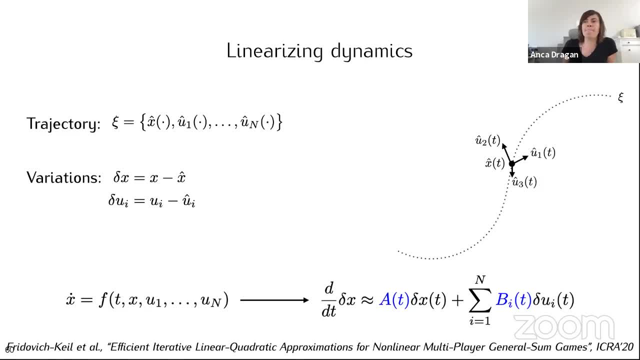 and you update your strategy And so real quick. I don't wanna take up too much more time. So if I have my current trajectory, this generalizes nicely to many different players, not just two. So you have your trajectory, you just linearize your dynamics. 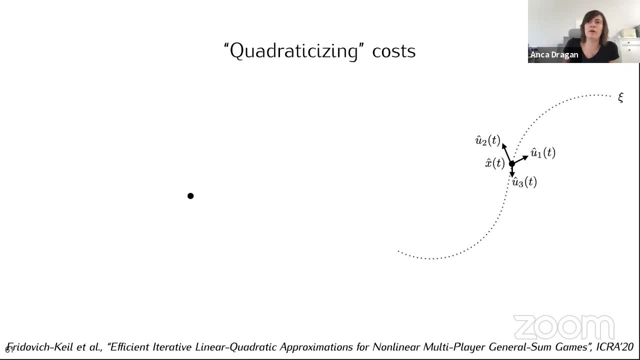 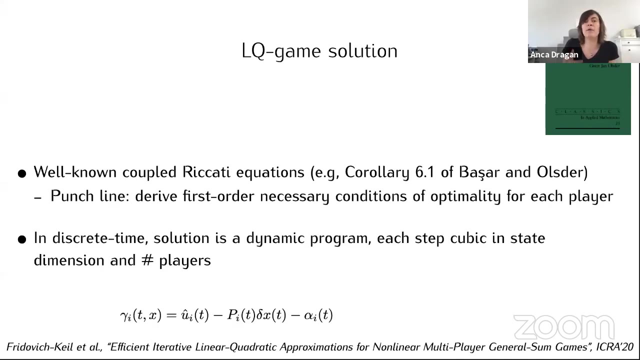 around the current trajectory: You whoops, you quadraticize your cost And then to compute the ILQ game solution, you just have a couple of Riccati equations which you can solve, And the thing that I wanted to point out is: 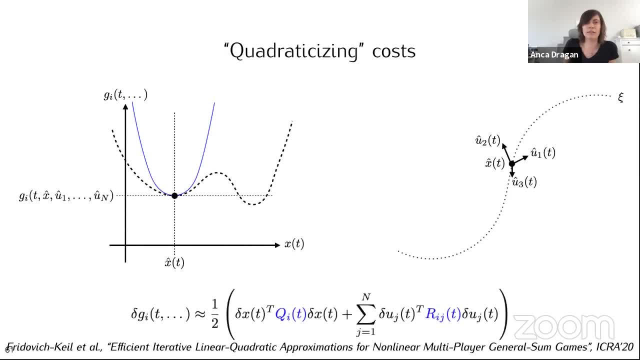 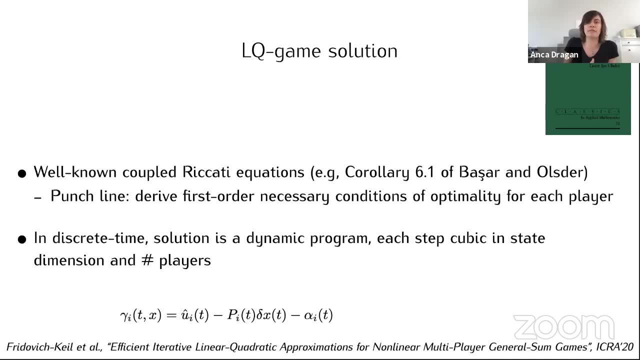 whoops. going back here, The thing that I wanna point out is the runtime, which is really exciting. So, at every step, the runtime is cubic and the dimension, the dimensionality of the state, space and in the number of players, which is, you know. 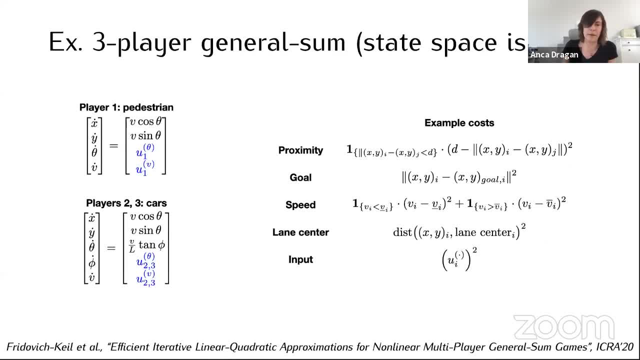 not great, but pretty good, considering that you're solving a game, And so here's an example that we tried out. So this was a three player general sum game where we had a pedestrian and two cars, So the total- the state space- is 14 dimensional here. 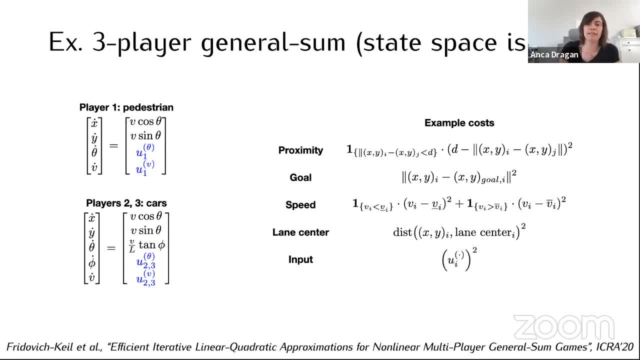 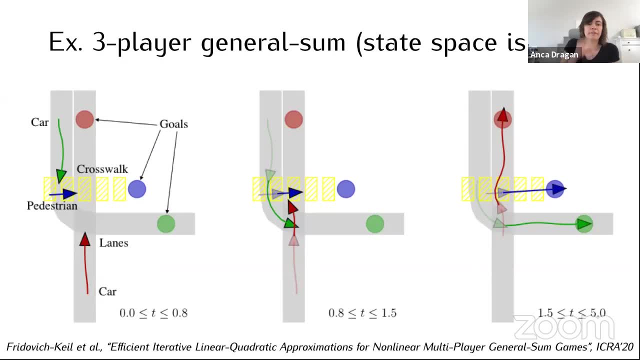 And let's see, there were basically people wanted to avoid collisions and people wanted to stay in their lanes. So here's kind of the solution unfolded, And you'll see some interesting things happen here, Like, if you look on the left, the green car initially slows down and turns slightly. 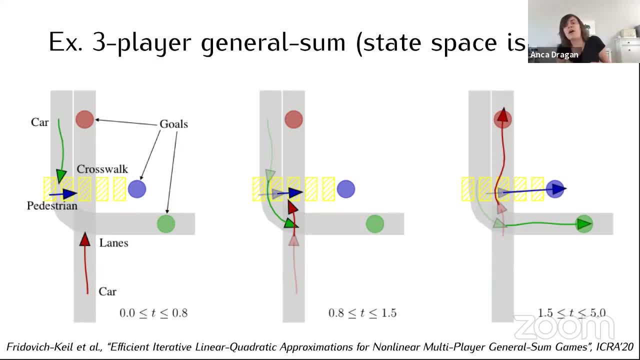 to allow the pedestrian to cross And in the meanwhile the red car sort of quickly accelerates in front of the green car and then it decelerates and kind of turns to give the pedestrian extra clearance And you kind of see this type of interaction unfolding. 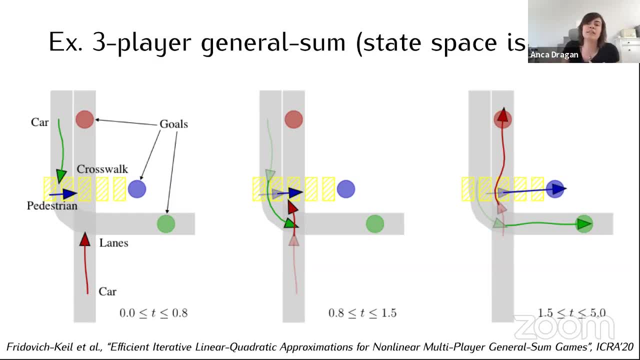 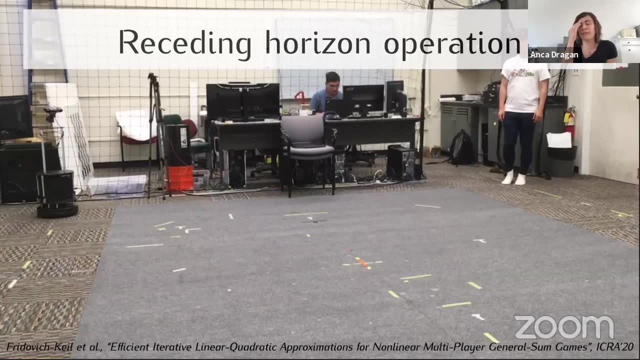 And again, solving this game from scratch would take us under a quarter of a second on a very standard laptop. And then we also tried this with real people, Cause real people are obviously gonna well, I should say, you know, kind of authors. 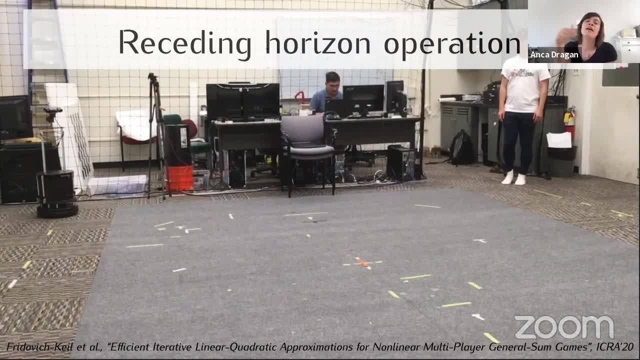 or people very close to authors. They're not quite real people, but the point is that even even people in the know deviate from these strategies computed right. Obviously, the way we move it's not gonna be exactly the solution to this, to the game. 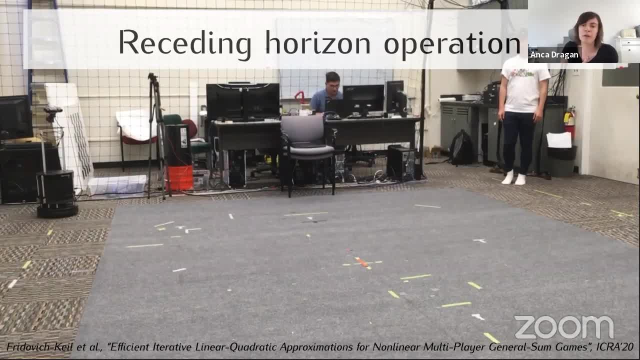 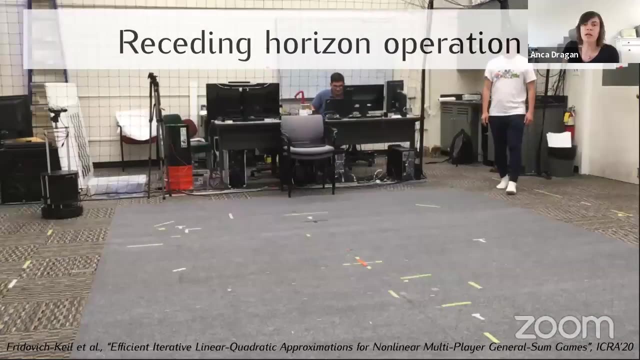 or it's not, definitely not in the way we compute it with our approximation. so the robot? what does that mean? it means that the robot has to recompute a solution at every step. so here we wanted to just demonstrate this as a as a proof of concept of this mode of operation. so you have a robot, we 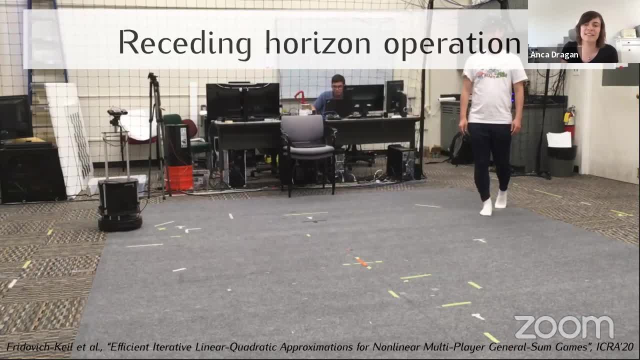 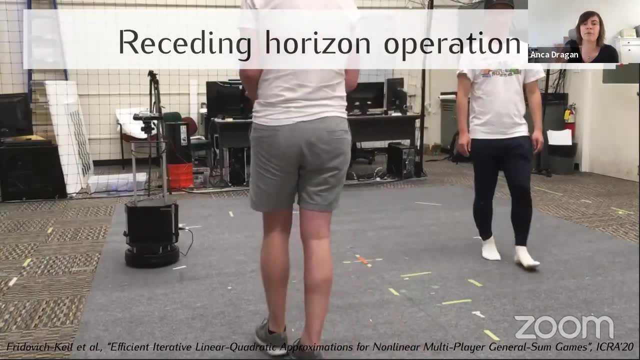 have mocap. everyone's moving slowly. sorry about that. it's not really up to scale, but essentially the the what's happening here is that we're resolving the game every quarter second and each invocation converges under 50 milliseconds, and the idea is that by formulating the problem, 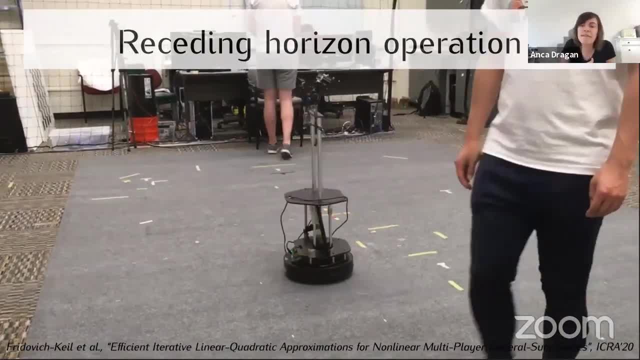 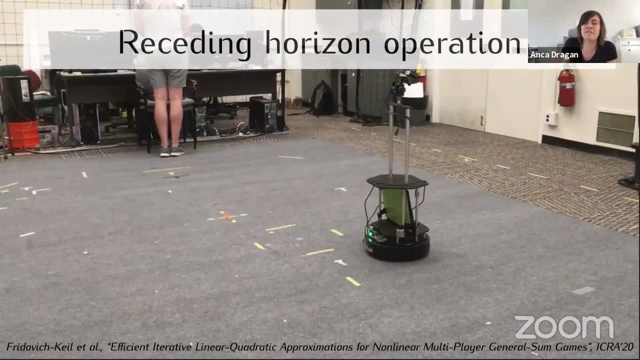 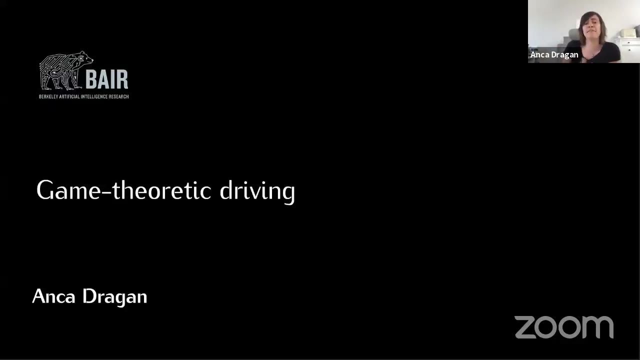 as a game now. the robot will anticipate the human's collision, avoiding behavior, and then, because we're solving this, receiving horizon, horizon invocation, it can handle the human. you know, the humans kind of inevitably deviate from the these perfectly crafted strategies. okay, so that's what i wanted to share in game theoretic driving. this is just a quick update. 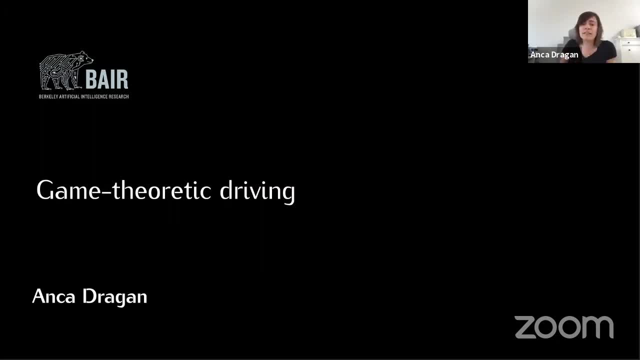 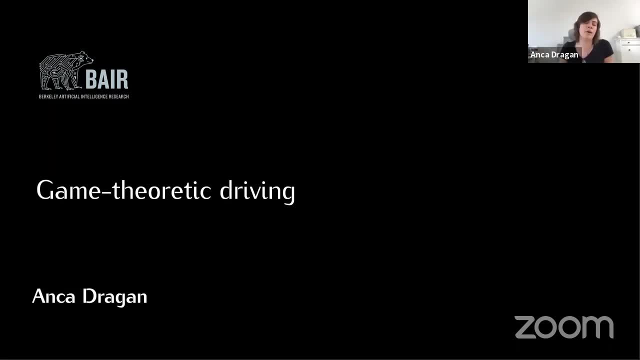 looking forward. of course, there are many things to be sorted out. one thing that i'm particularly curious about is how you can kind of merge these two approaches- the jaime approaches, the david approach- together, to get sort of the best of these, of these two worlds. i think they're very 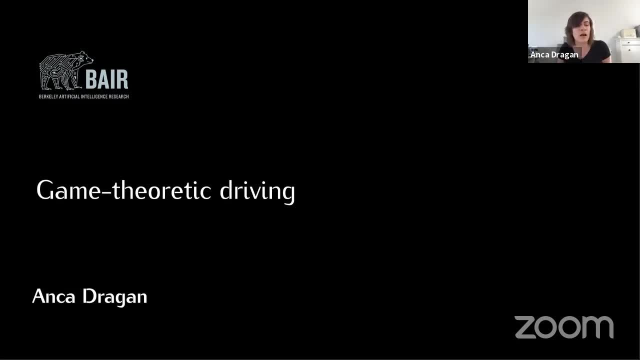 compatible um. so that's one. and then of course, uh, you know also i consider studying science as somebody who's very inspired by science in general. sort of finding ways to really deal with partial information in that is another thing that's very much on my mind, kind of going a little bit beyond what we were able to previously do. 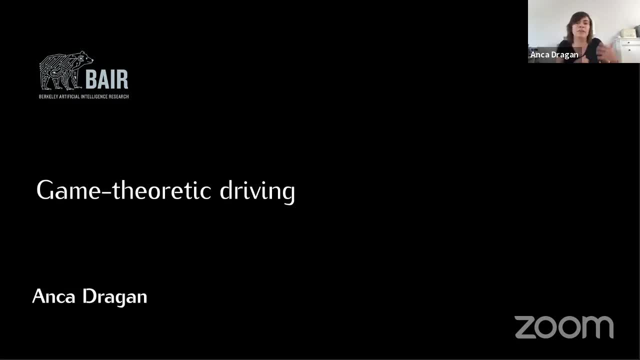 when we were doing some info gathering to figure out, you know, is this person aggressive or defensive, What's their driving style, And then, of course, fixing these models, which I think also talked about in the morning. You know, people aren't really all that rational. 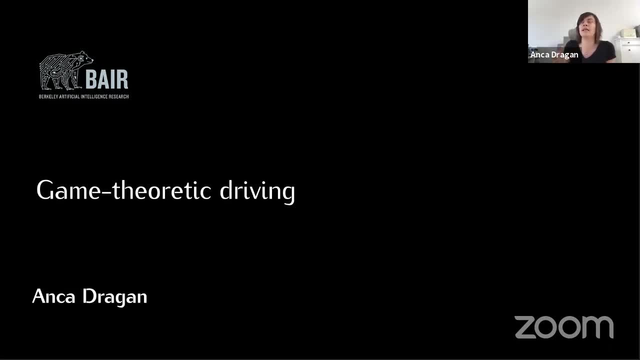 but it turns out they have these systematic biases that we can actually hope to at least devise models that are a little bit more flexible in allowing for that. So with that, I'd like to thank you for listening and I'll stop sharing my screen. 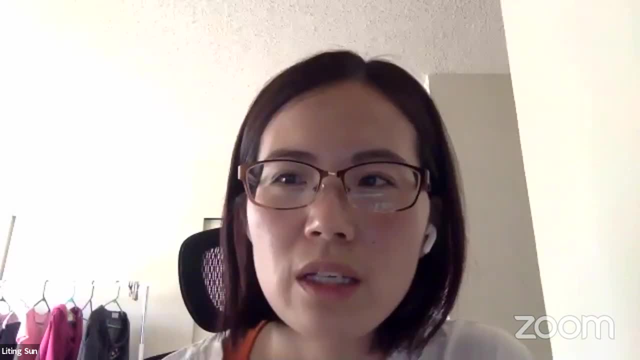 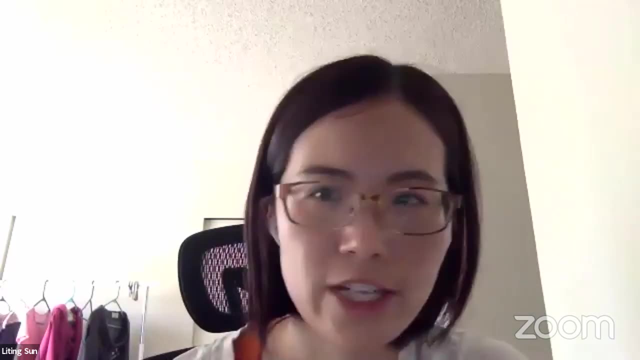 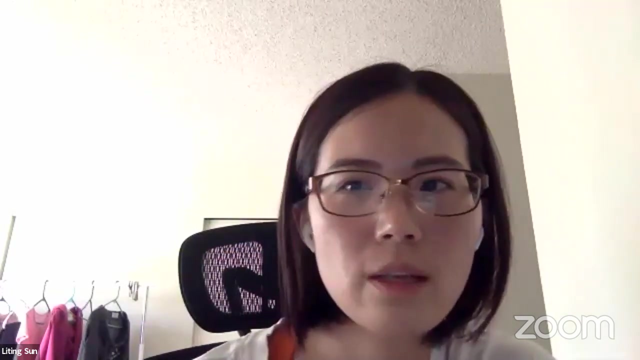 Okay, Thank you very much, Professor Anka-Gagan. So we got some questions Just before I read out the questions. just as a reminder, if you have any questions, please send them over the chat. So the first question for Anka is: how does the runtime scale with number of? 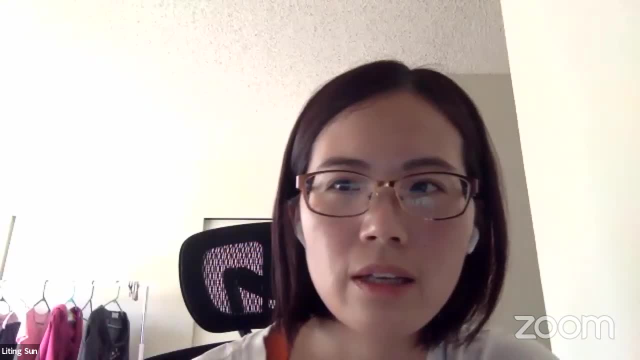 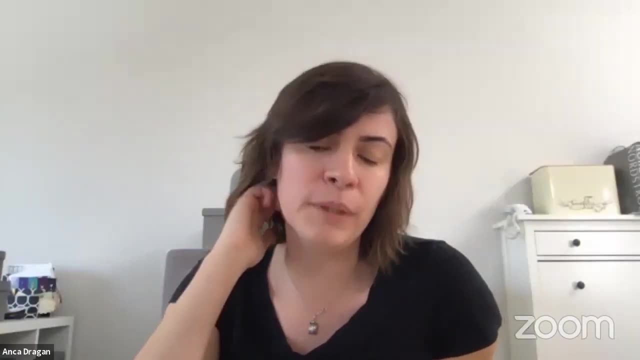 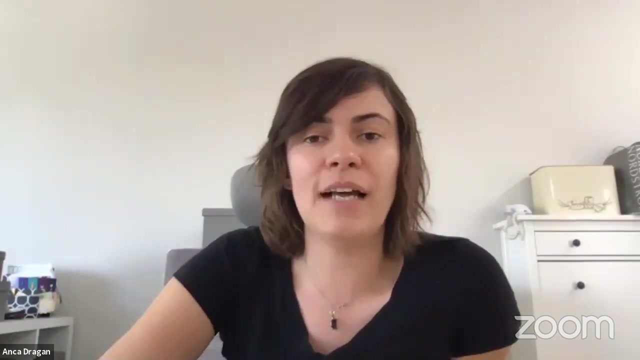 interacting agents And is there any observations? if we wish to scale the situation with many players, Yeah, So with David's approach it's cubic in the number of agents And so I mean that's not amazing but that's pretty great. Back with Dorsa's approach, I think it's pretty great. 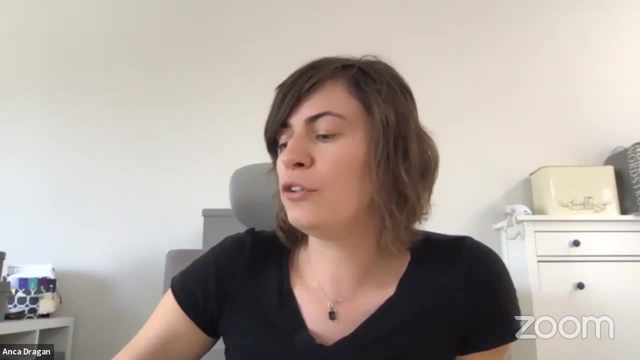 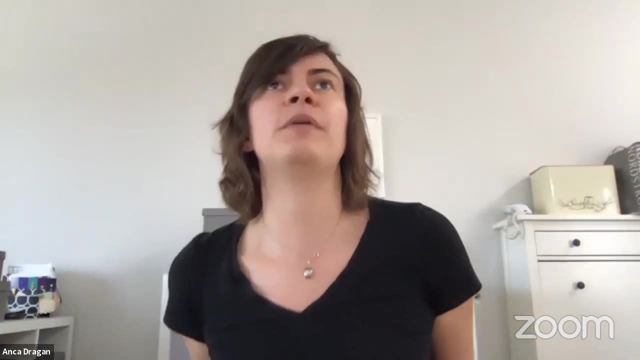 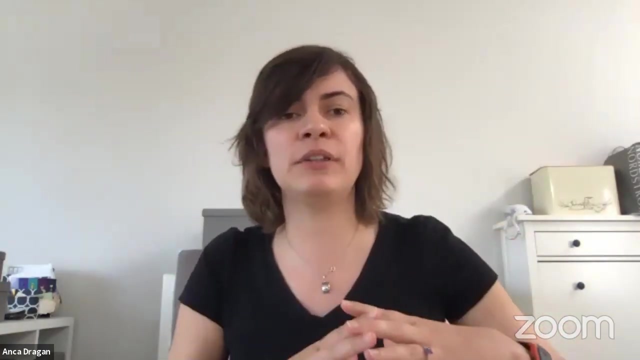 uh, you would. you would sort of do it independently per agent, or i should say, if you want to scale doris's approach to multiple agents, you do this at this um thing where, whatever you're using to deal with with non-influenceable predictions, whether you're doing it per agent, right which 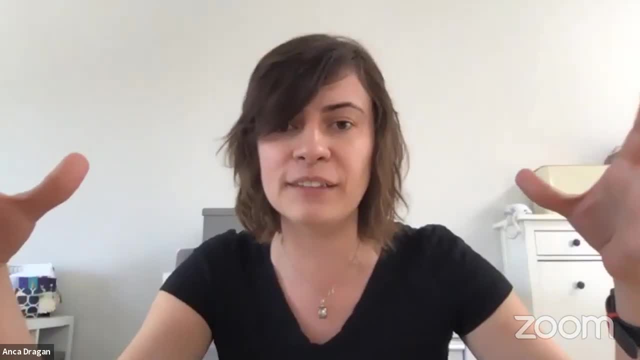 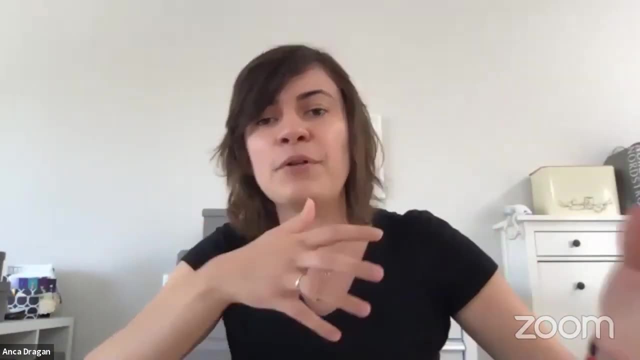 is then linear, or what are you doing? some sort of joint optimization, for instance? that sometimes people do, that they kind of treat all agents as collaborative, collaborating with each other and planning in that space. now you just modify that to depend on the, on the robot's action. so i think 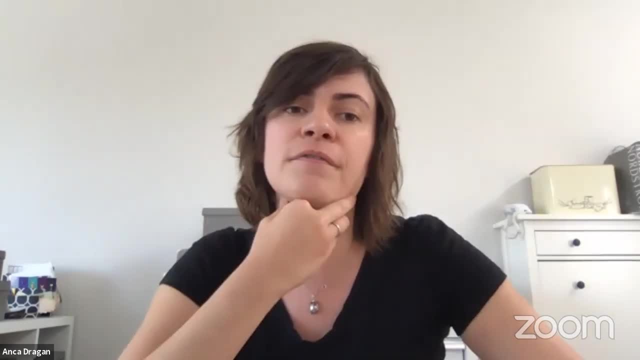 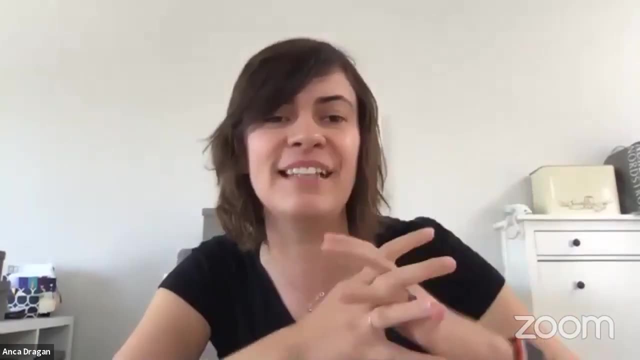 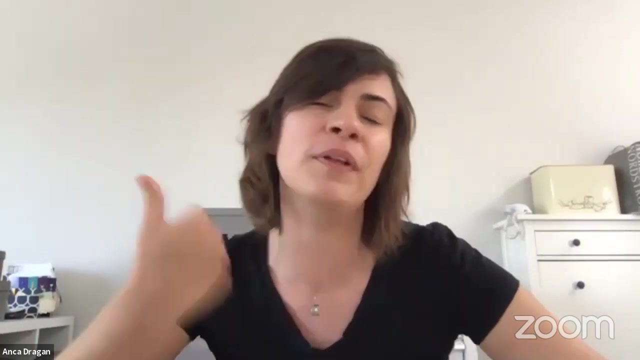 that's. you know, that has the advantage of of it's fairly straightforward to scale, but it it unfortunately has this kind of broken information structure which it got us very far, but it, you know, had some some issues to iron out. so, but with david's approach, it's actually um, that's. 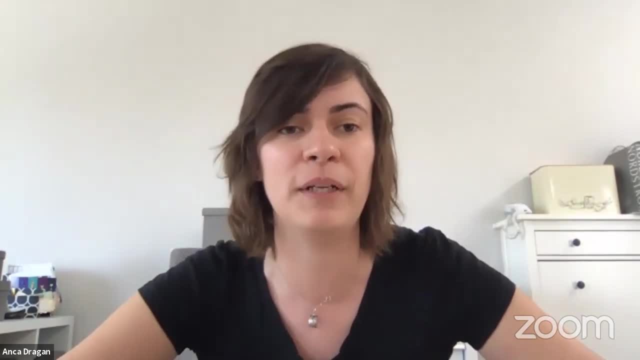 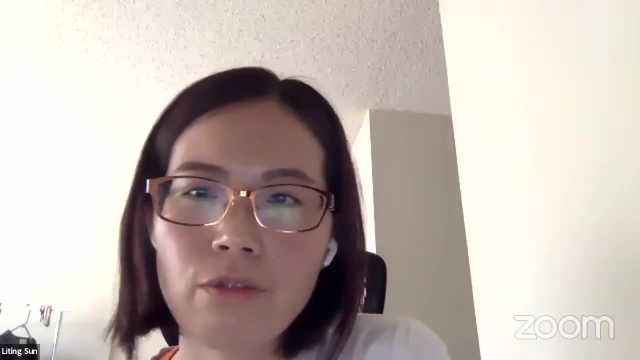 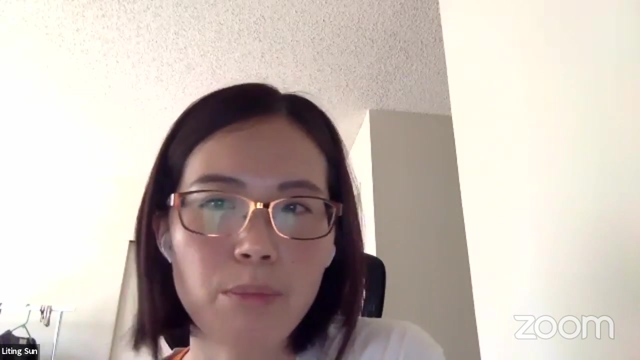 that that is really nicely scalable. l2 games are actually pretty nice to solve, even with multiple players. i see: cool, yeah. and then we got a second question from jack. so, um, how difficult would the reward function used to be learned? and uh, particularly in practice, for example? um, how 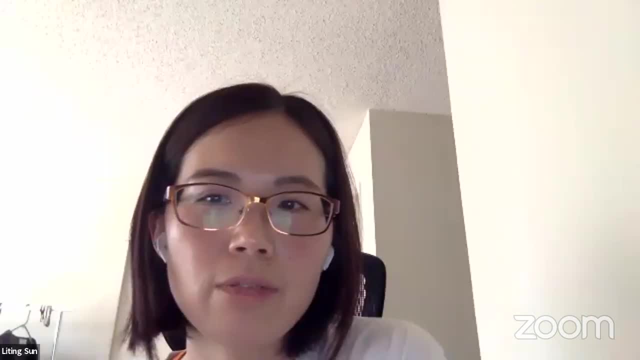 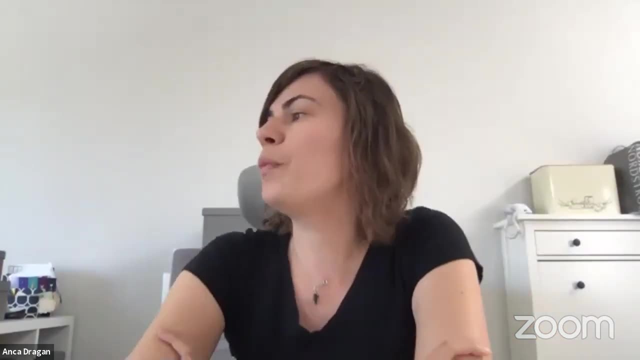 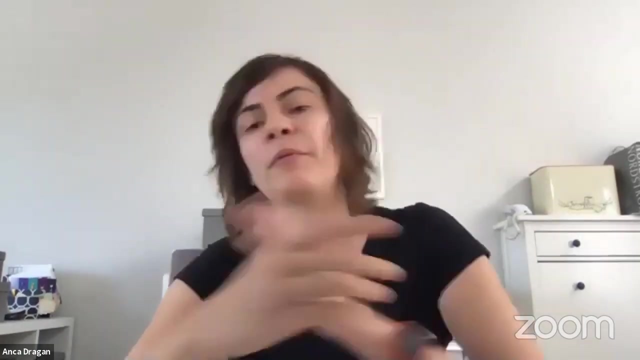 much do the method performance rely on unknown? or why define interacting components to the reward? yeah, no, that's a really good question. so, um, there's, there are approaches that do sort of- instead of inverse reinforcement, learning, or really i'd call that inverse optimal control. instead of that, it's like an inverse game. 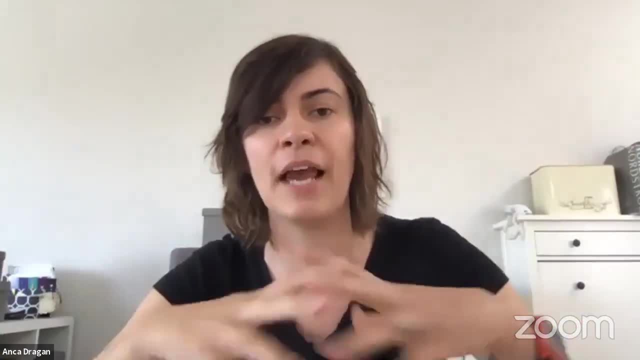 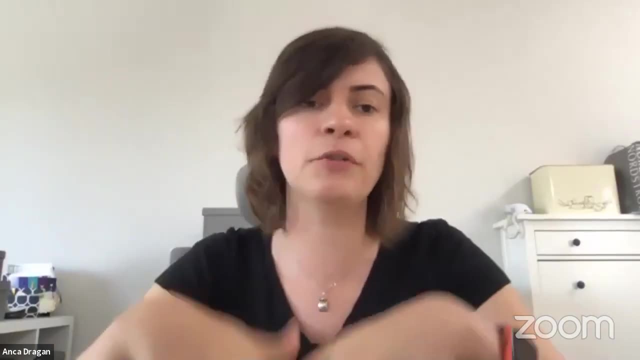 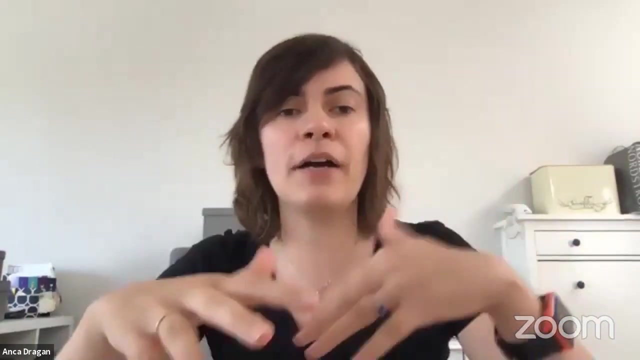 approach. so actually it takes into account the fact that the players are solving a game um the but. but i feel like in general, that's an area that's highly under explored, and so, for instance, with dorsa, um, we kind of cheated and and we would solve the irl. 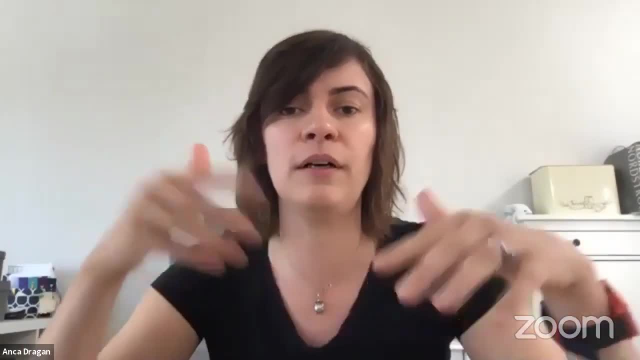 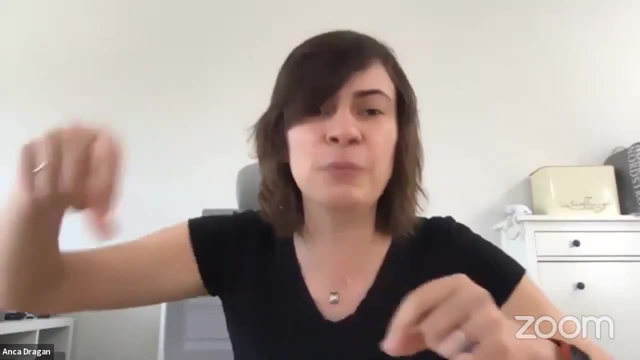 by kind of giving the person access to, to the, the. you know you collect some data and just from that data you don't have a plan right, but you can sort of use what actually ended up happening as the plan and then run the irl based on that. for instance, is one thing you could do. 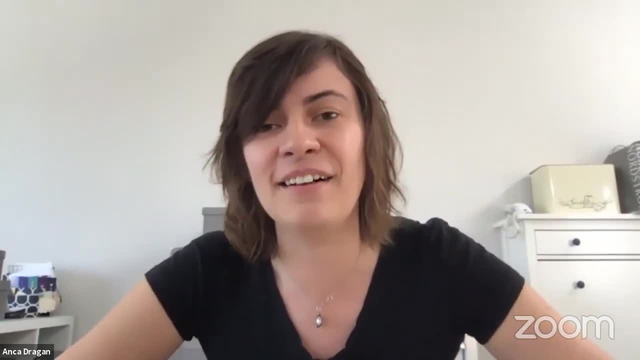 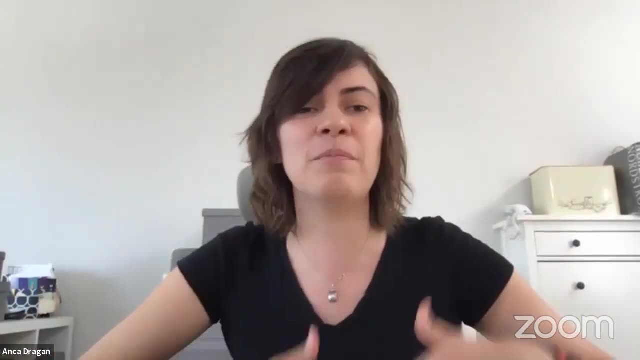 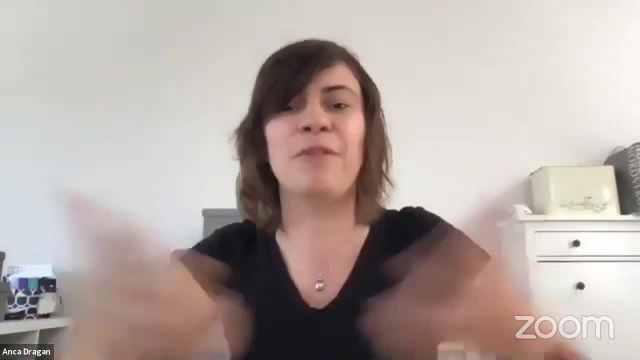 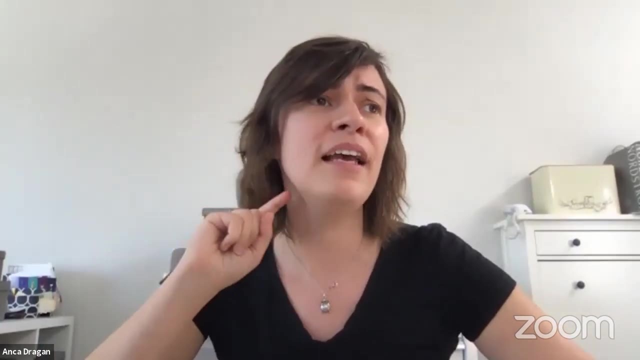 your robot until you don't, and get away with irl methods that don't fully capture that until you don't. the other thing, um, sorry, i want to rant, but something that is very related to this question, that is really hard to do as well, is running irl properly when what you're going to do is model. 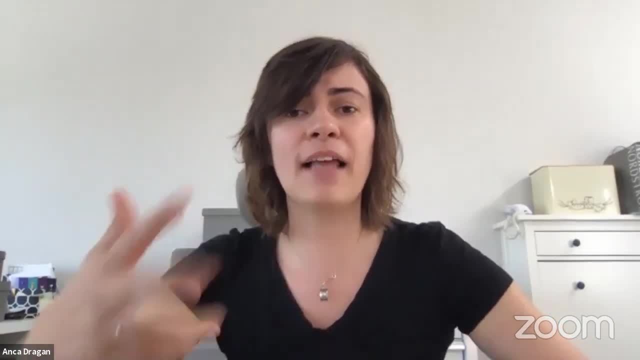 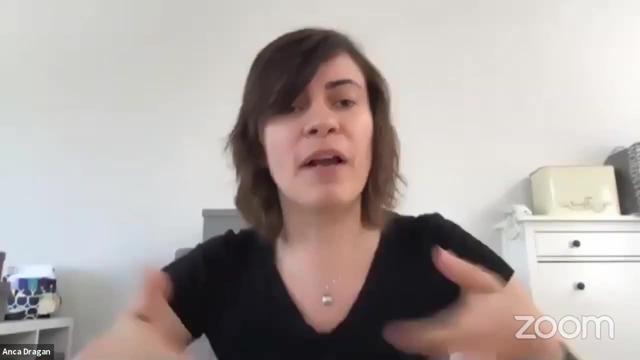 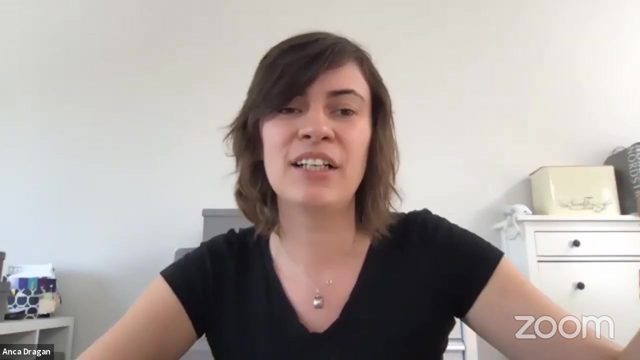 predictive control. so you know the fact that that these things are not plans that you stick with, but you replant at every step, right um you, when we run irl, we always kind of pretend like that's, that's what we're, we're actually going to do, but you don't see the person's plans, you just see. 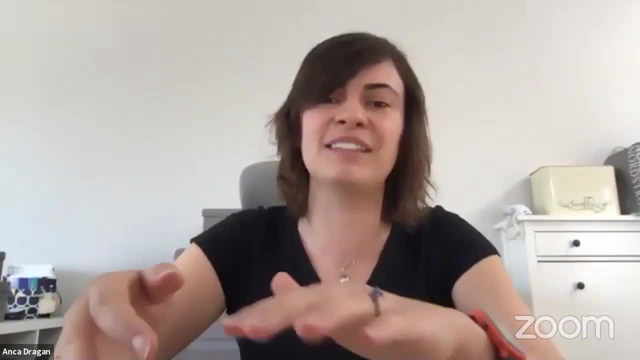 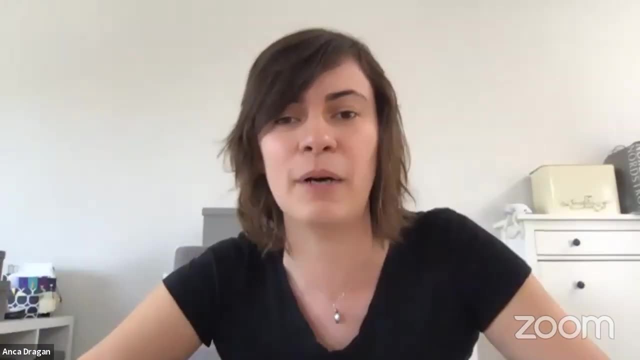 right, the first step of each plan, and we kind of assumed that that was the plan from the get-go, but of course it wasn't, because it gets recomputed at every step. so that's very sorry to hijack the question, but i was very related to that question and i think those two are very important issues. 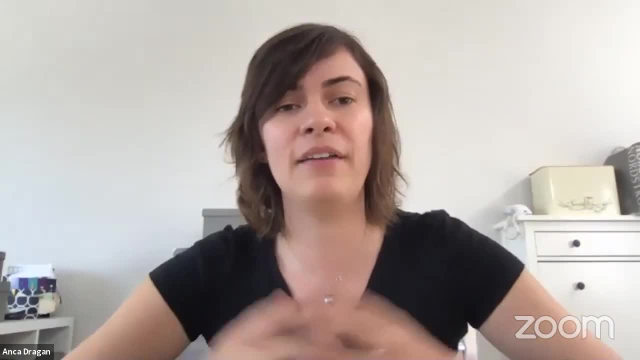 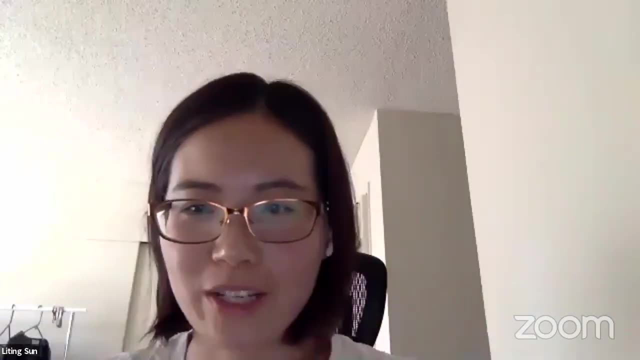 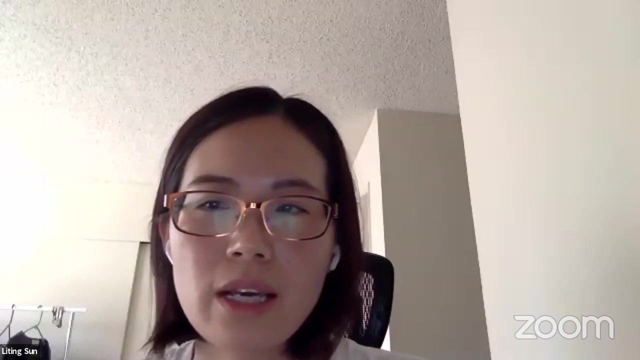 in running inverse reinforcement learning right now. i think people should work on that. i'd love to see work on that. okay, cool and uh. yeah, we have two more questions. so, uh, the third one is from lion paul. so he is asking like in a game theory approach, is there? 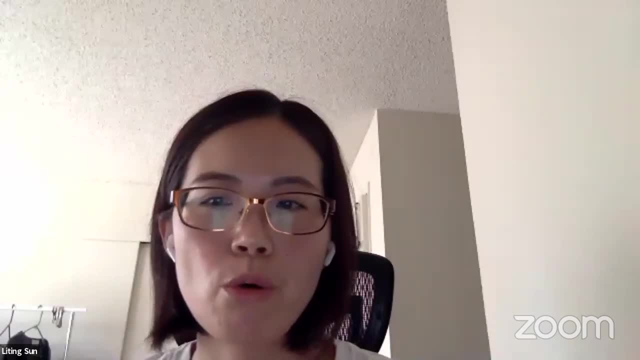 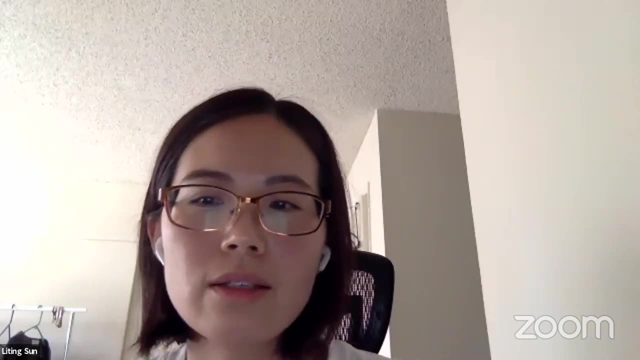 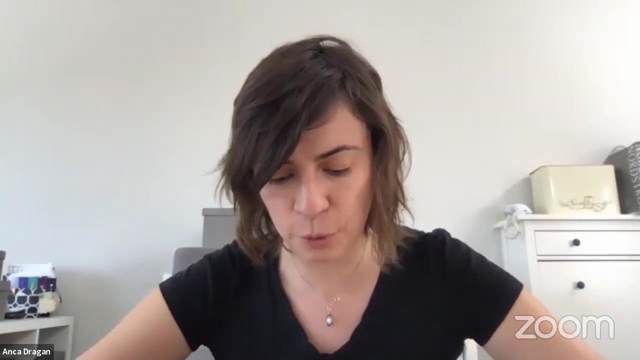 any a way to straightforward, like a three-fold way to add extra constraints, like, for example, the pedestrian had the right of way to cross the crosswalk? are these types of relationships in a in a boat? yeah, so so about that, i mean, my, my method of choice would be to actually add it as 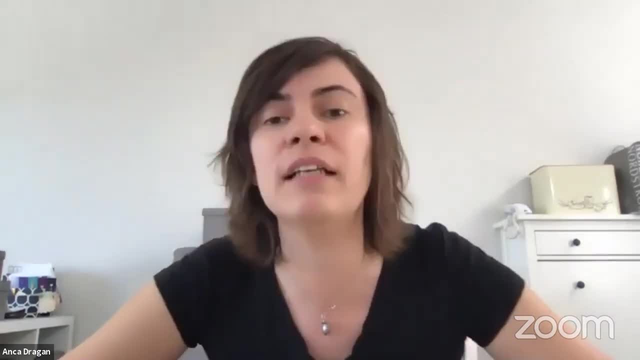 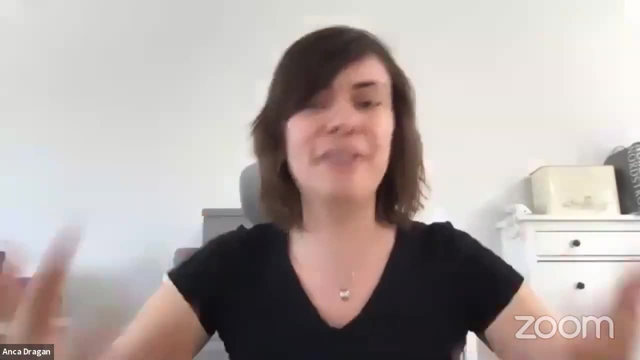 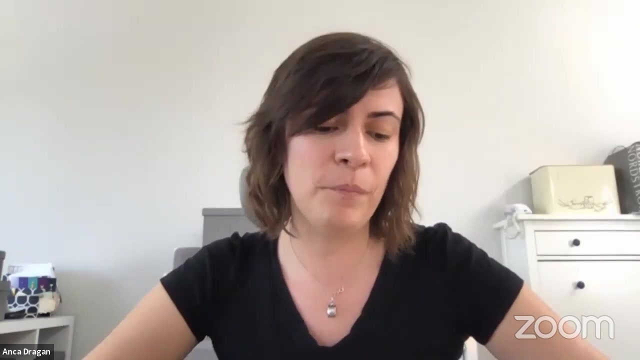 um as a signal in the utility. now the utility um. when you're doing dynamic programming you don't care if the utility is differentiable or not. when you're doing optimization you know you might want to have something differentiable and so hard constraints might be a little more tricky, to tricky to capture um. but certainly 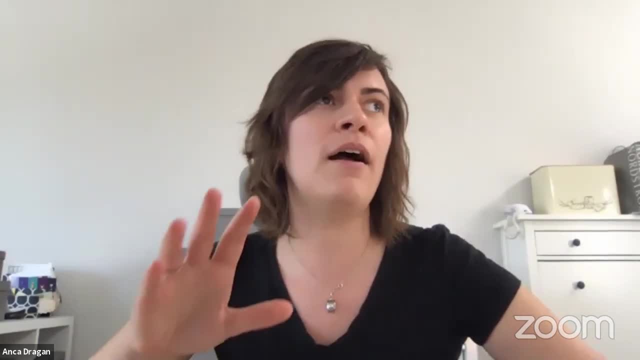 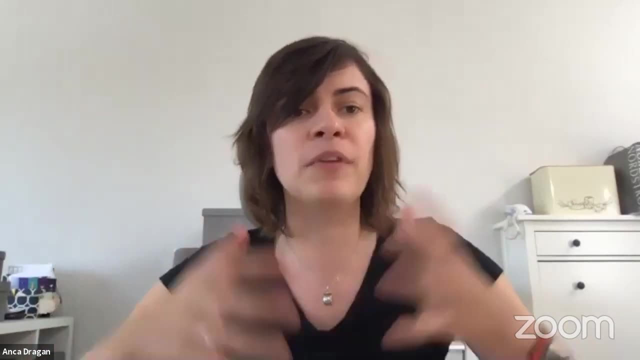 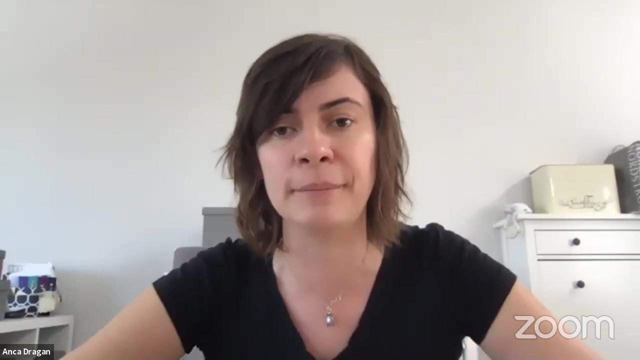 there's work. so there's work in in um, ilqr, with constraints obviously um and and uh, i i don't think it'd be too much of a mathematical endeavor to to try to um scale that work to the ilq game setting um. but i will say that i don't know how you know hard constraints like 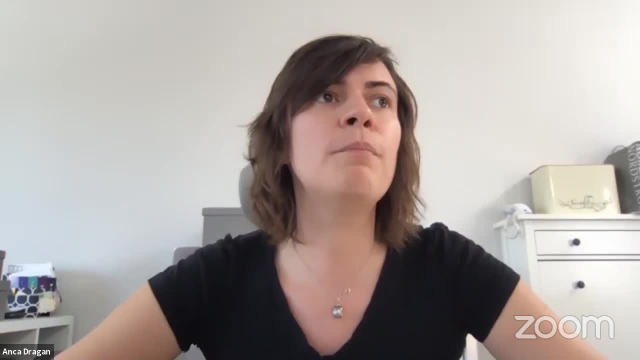 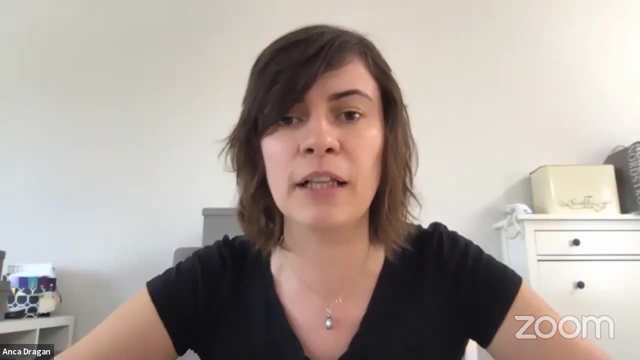 the pedestrian will cross. um, you might not want to do that just because. just because that's the rule doesn't mean that people actually follow it. so that's why i actually prefer the approach that puts it as kind of as part of the utility and not necessarily linear. i'm not trying to okay. 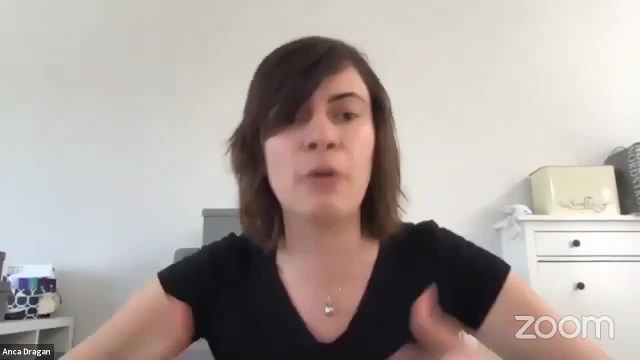 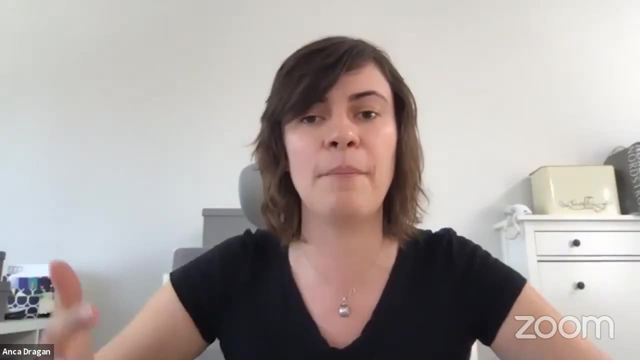 for linear trade-offs because they're total garbage, but but somehow incorporates it, as this is a criterion that influences what's going to happen but doesn't dictate or strictly enforce what's going to happen, because you'll see cars going in front of people and people going when. 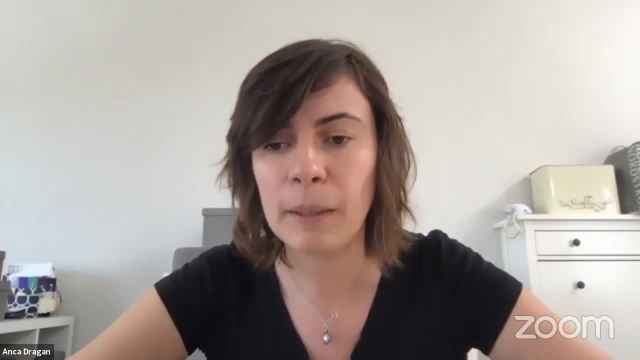 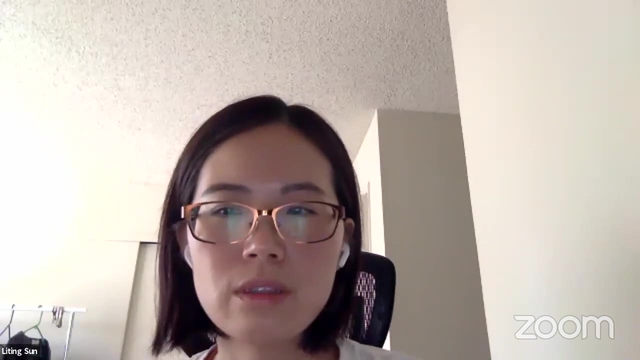 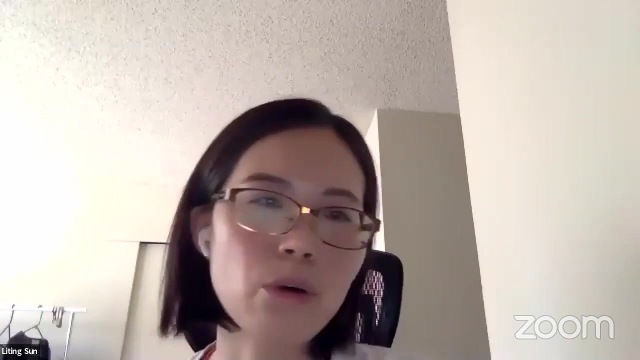 they don't have right away and so on. okay, yeah, um, and then the last question is from rohan. so he's asking: how could the game theory approach to be evaluated and tested in real scenarios, not only in simulation and indoor like a robot environment? yeah, so you have a. 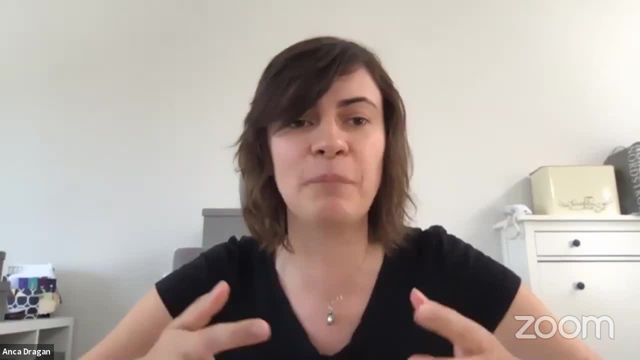 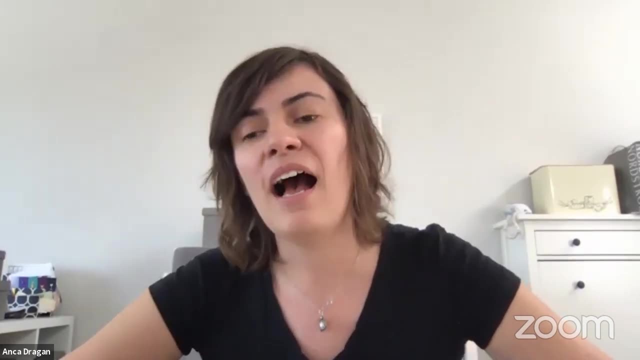 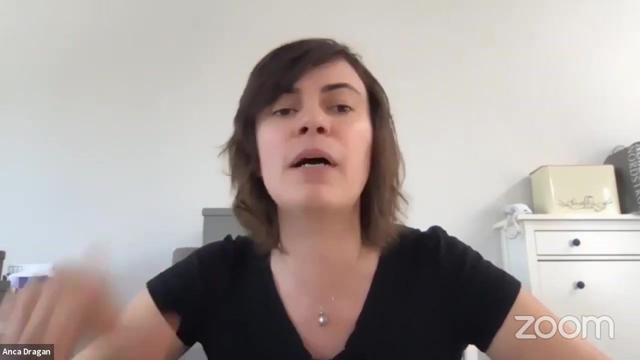 to understand that i run a lab. i don't have a car, so our best proxy for you know real people, real robot, is in, in, in an indoor environment. um, i think that that, uh, the goal of these two approximations that i presented was very much that you can actually run them in the wild. so 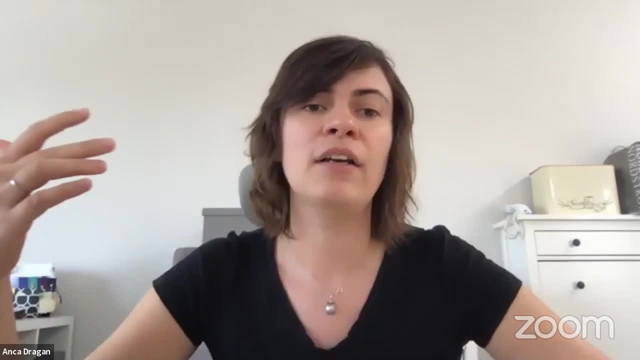 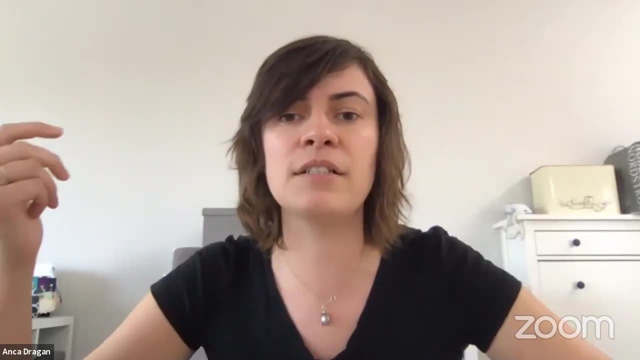 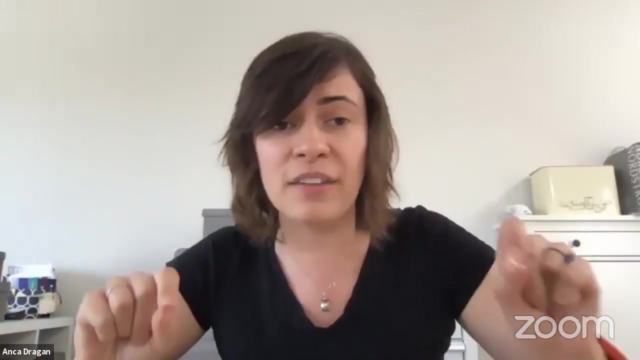 i think that you know, with jaime's approach, remember that you're doing something offline. that then is very cheap. you just have a table that you're indexing in online and, um, that, that drive, and otherwise you're doing a pretty standard optimization. you could do nested, by the way, just a kind of a quick thing there, jaime discovered. 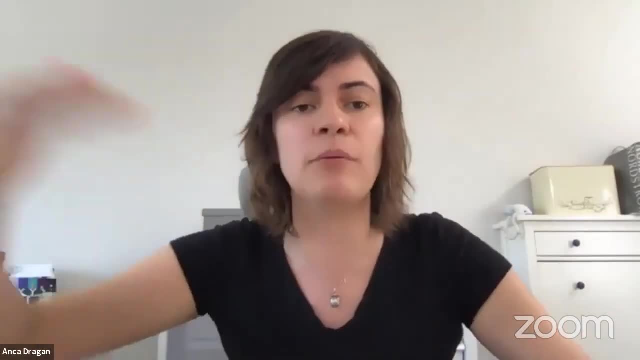 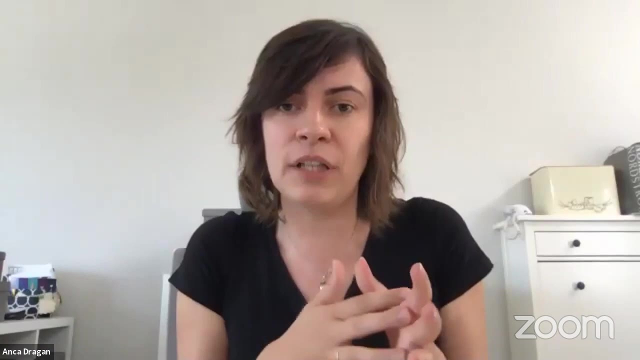 that once you have this value, that's kind of telling you what to do at the strategic level and influencing your optimizer. there's not so much benefit of doing the full nested optimization like endorses meta. at the tactical level, you could get away with coordinate ascent, so that's what 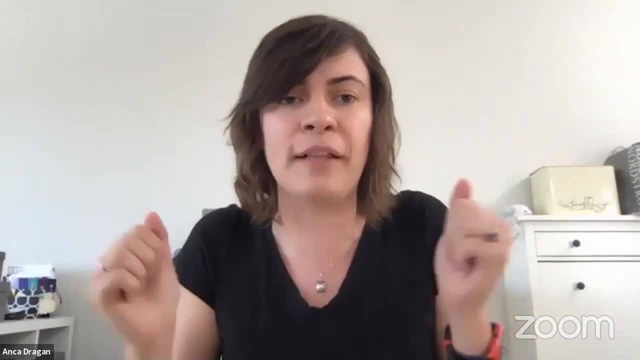 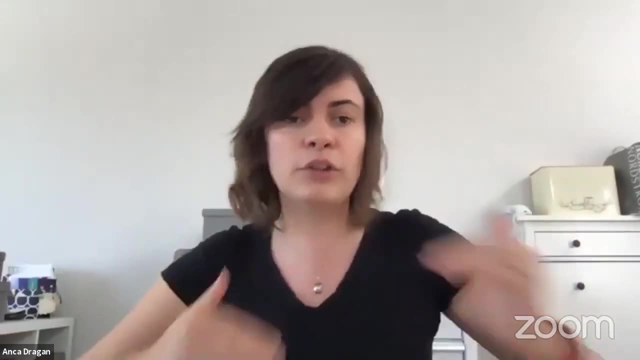 we ended up using in the paper. so coordinate ascent- it's not a great name for this, but it's you. you know you. you take a step on the robot's trajectory, take a step on the human's trajectory, each solving their own optimization problem, sort of in parallel, like that um and. 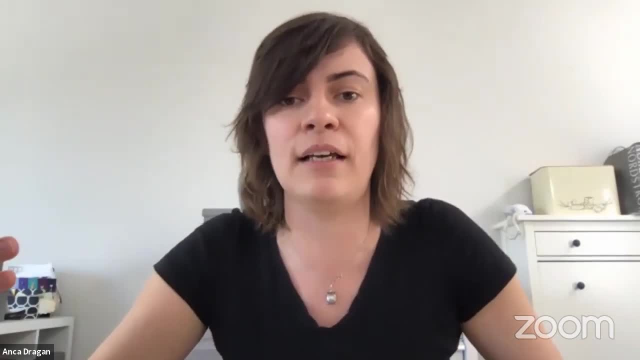 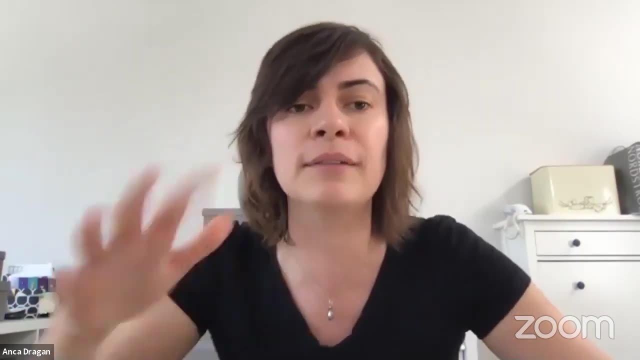 that's really cheap, right, and now you have the value that you're indexing in, and so this is actually very much something that you can do in real time, and similar for david with ilq games. i already talked a little bit. i gave some numbers of what it takes on. you know with what david's 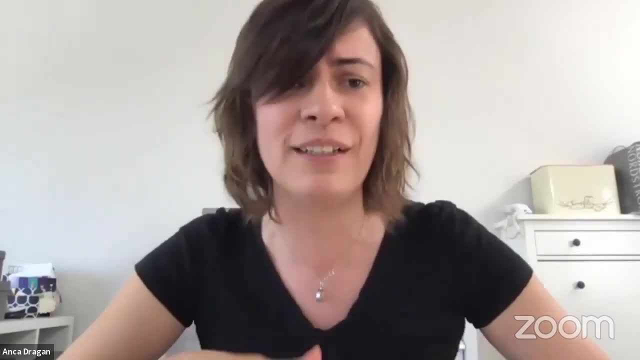 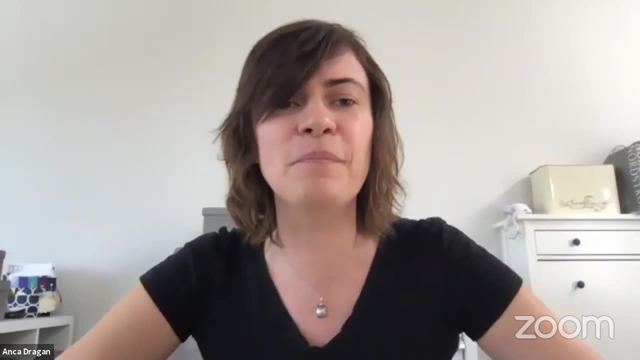 pretty good at c plus plus. actually i wouldn't say this grad student code. he's very, he's legit, um, but he's done much more than i could have ever done, even in grad school, let alone now. but um, but still, you know the the it was. you know, just run it on the standard laptop and you can. 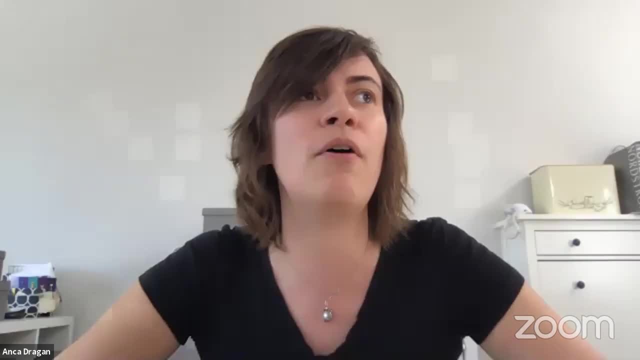 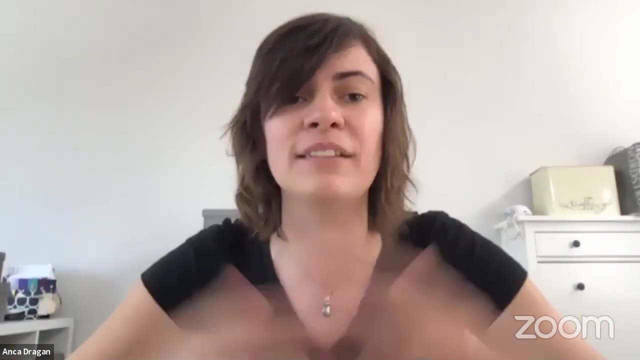 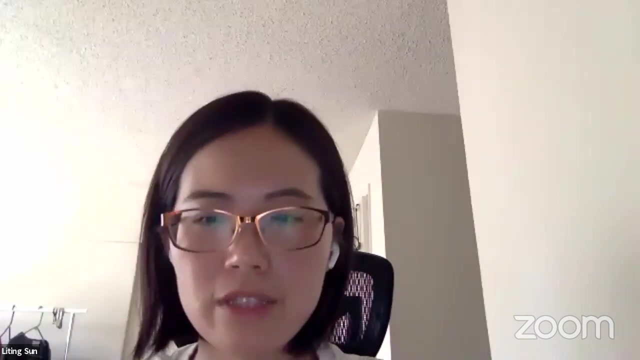 solve this every every with his code. we were solving it in 50 milliseconds. every time we were resolving it like, if that's not real time, i don't know what else to give you. so that that's where that will be very cool. so, uh, i think we're still like five minutes ahead of schedule, so i 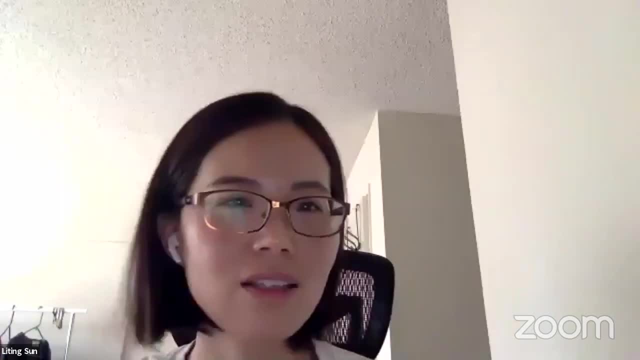 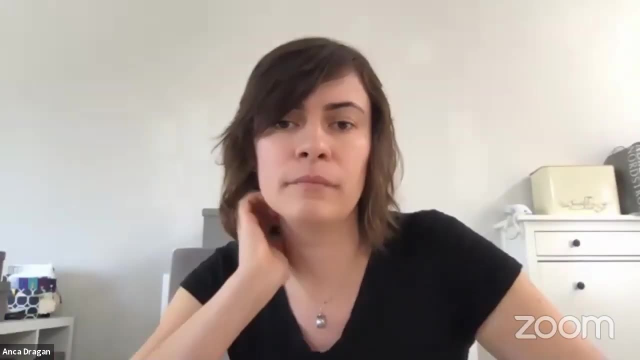 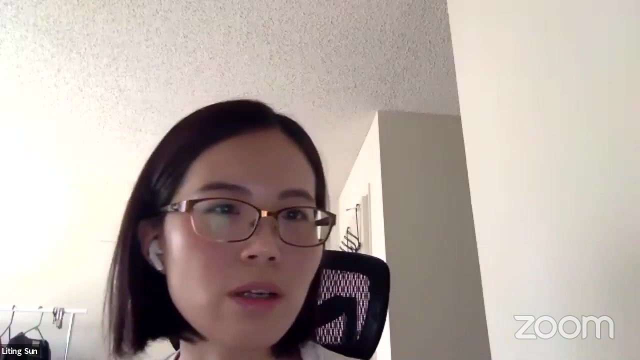 don't know if we have time for any more questions, um, but i think we have time for one more question for you, um. so, yeah, just combining your uh work and uh what thoughts are presented in the morning. so, um, what's your view? like, uh like people right now have uh two kind of two groups. one is using 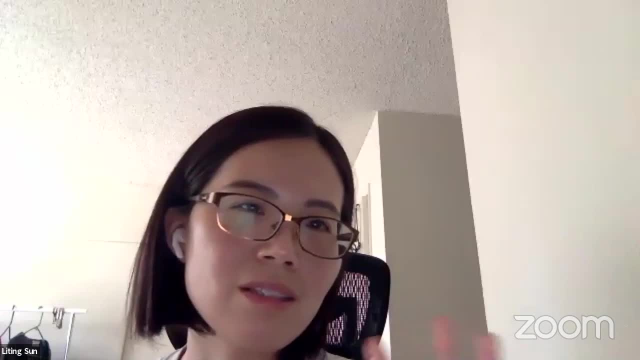 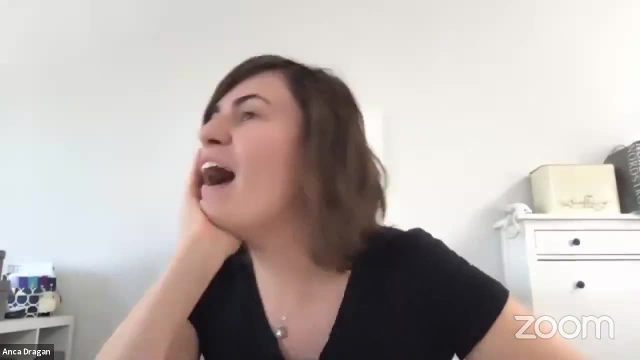 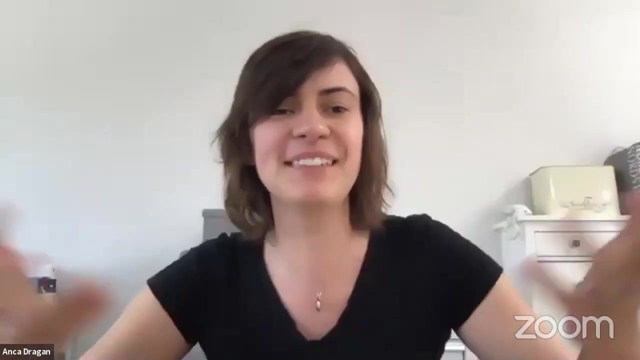 uh, game theory. the other is, um, doing more like end-to-end learning, deep learning methods. so what's your like comments, like in terms of combining both, or like, uh, yeah, which way should we go? yeah, yeah, um, so you know who the heck knows, but let me, i'll, i'll, just i'll muse on the topic, um, so i think. 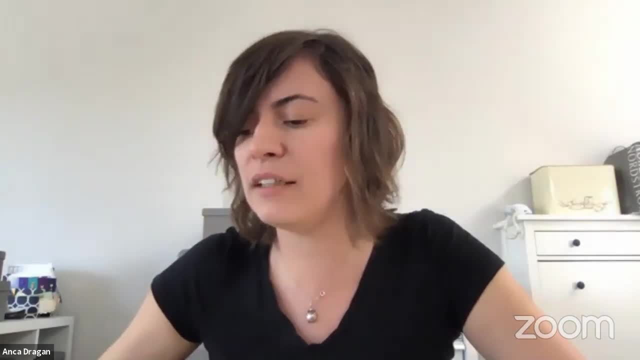 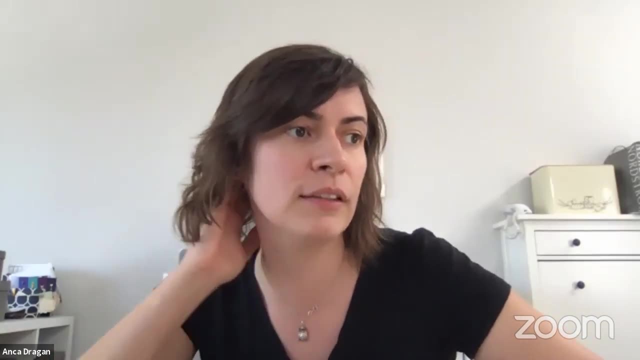 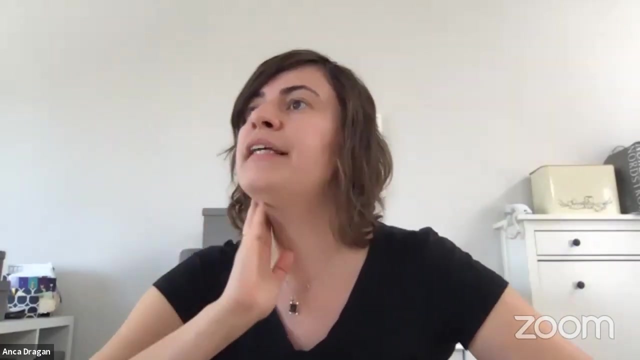 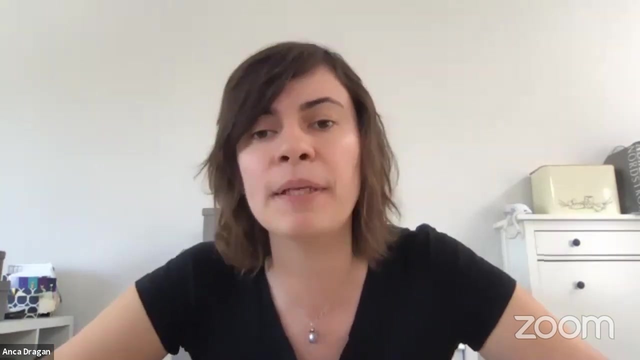 i think that you kind of need both approaches, from just from the perspective that when you do things more- let me call it more imitation, learning, style, policy learning style- you'll end up with these gaps. um, because you're using such a hyper expressive function, class right, you end up inevitably with not being 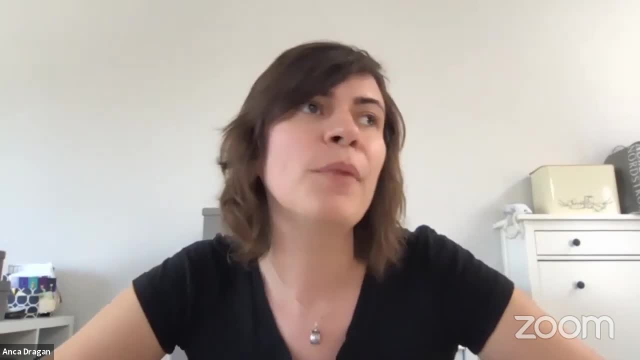 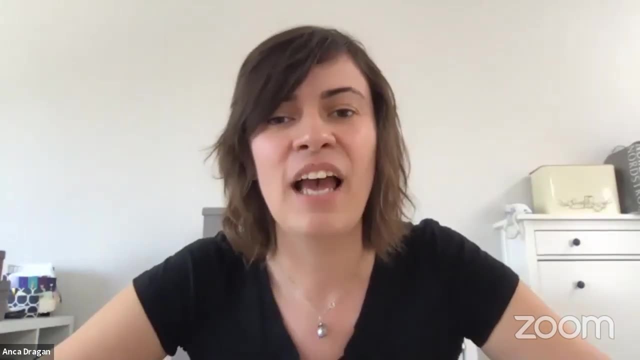 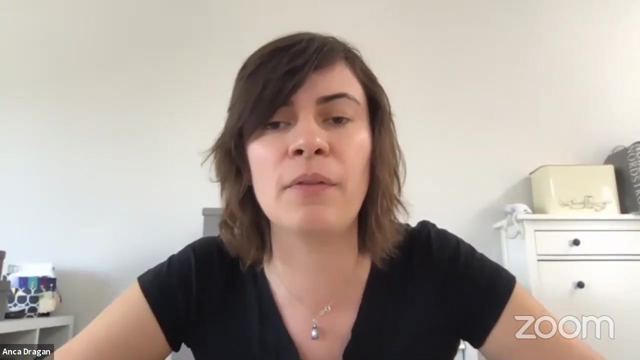 able to really extrapolate past the data you have. so i will, i would default to such a method when it's very close to the data right, and then i would trust something that's based on on more, more the planning approach, for, you know, these situations that are a little bit outside of what we 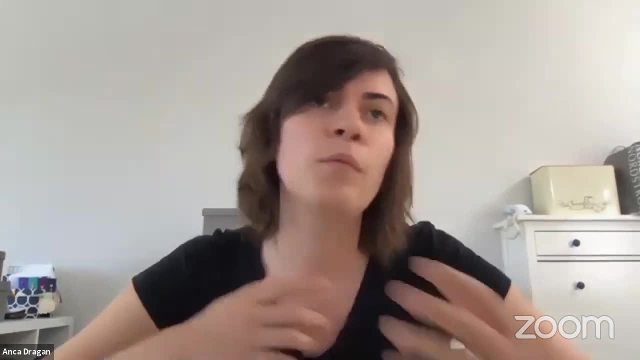 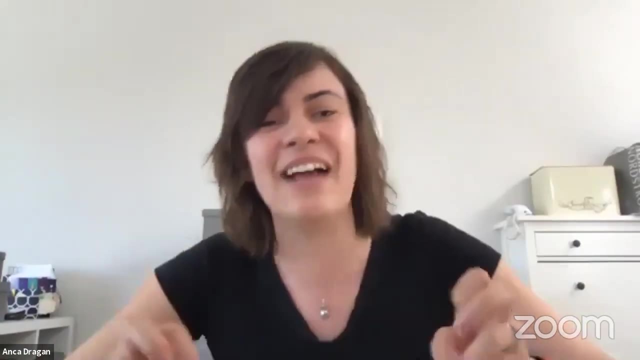 have seen a lot of examples of, and with the right way to get that combo right. what does it mean that you're you're close to the data? right is: what does it mean that you're out of distribution, but does it mean that you're experiencing some form of covariate shift? that's something that 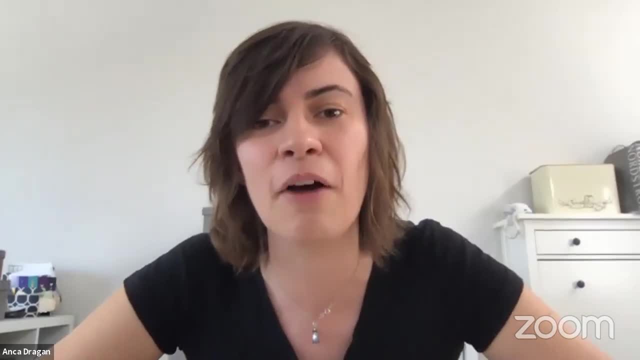 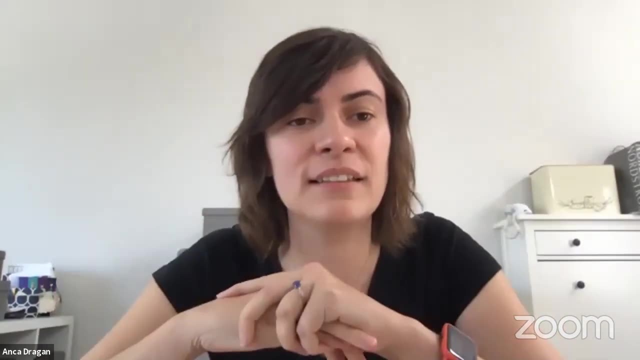 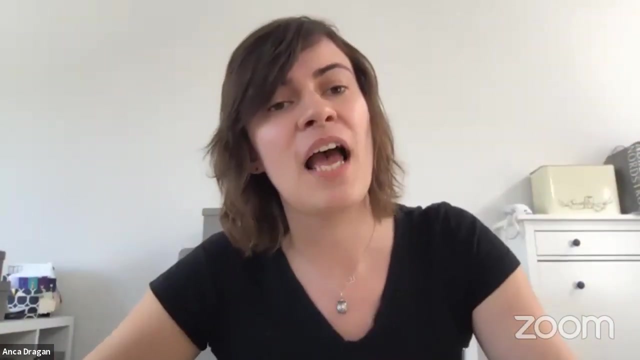 i, you know, i think that's where a lot of research needs need to go into, but just from a very high level, i'd say, policies that are that are very large. deep neural networks are very, very, very expressive, and that's a blessing and a curse because they're just going to be many such. 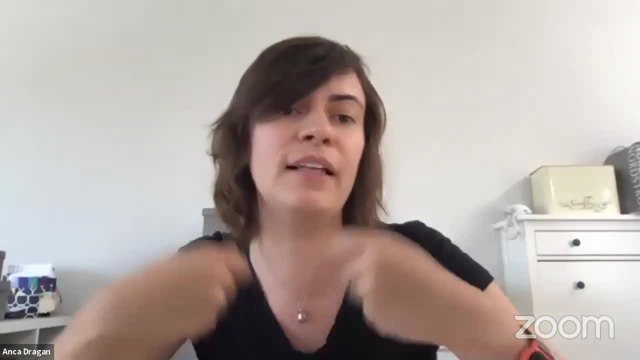 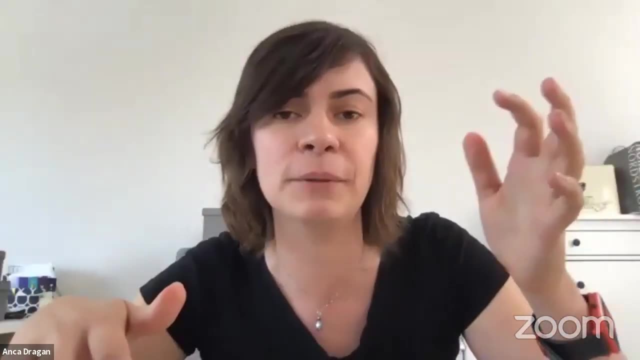 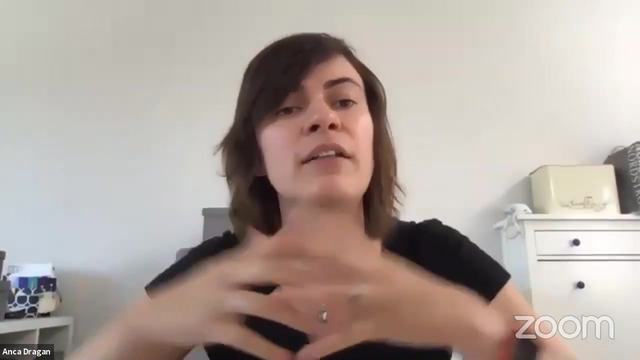 policies that are going to be consistent with the data that you're seeing, and only a few of them are going to do, outside of that data, anything remotely like what a human would do. and so, at the very least, you know, you have to be able to to either figure out that you have uncertainty and are confused in those situations, or, i think, 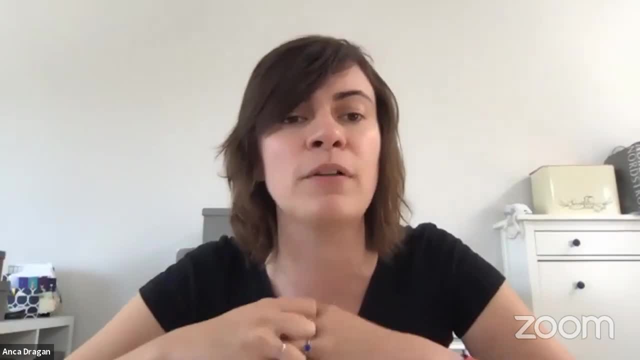 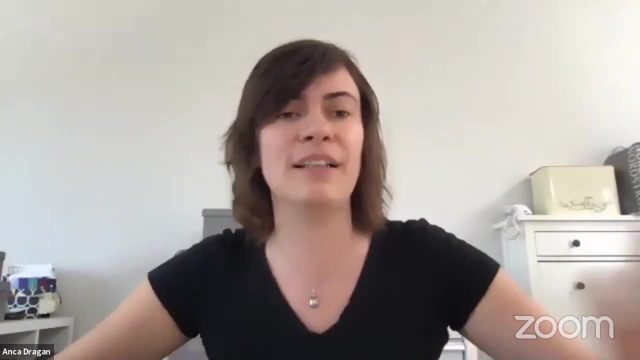 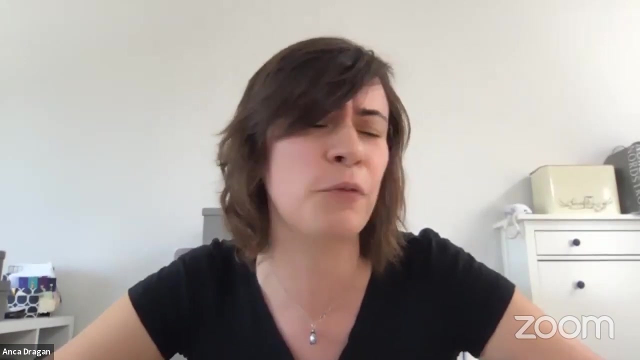 even better. um in, in such a case, sort of default on on something that has that structure, that's not perfect, that underfits for sure, but that you know can, can, can deal with with those types of things. i wrote a, i wrote one paper on this. it's good, it's called uh, it's for hri, it's on the utility of. 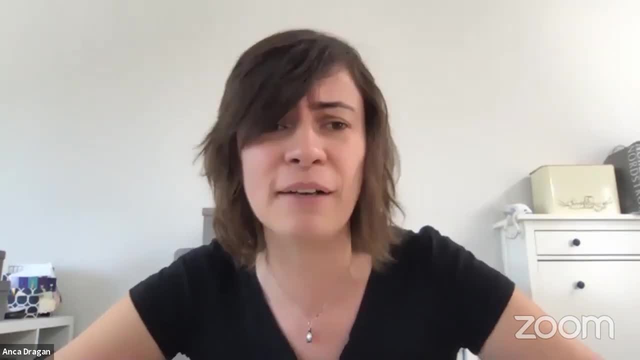 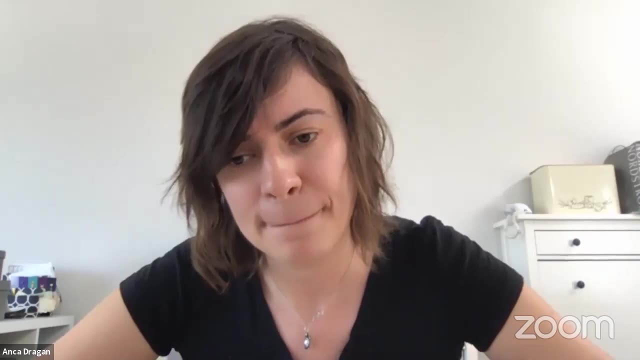 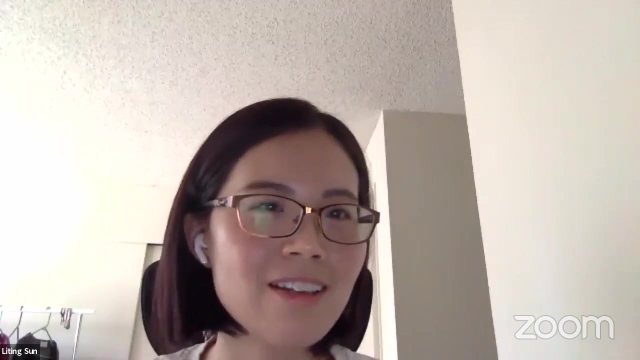 model based modeling humans in hri or something like that. it was a couple years ago where we talked at more length about these issues. okay, cool, um yeah. i think that would be all for um anchor session, so thank you very much for attending and giving the wonderful talk and the discussion. 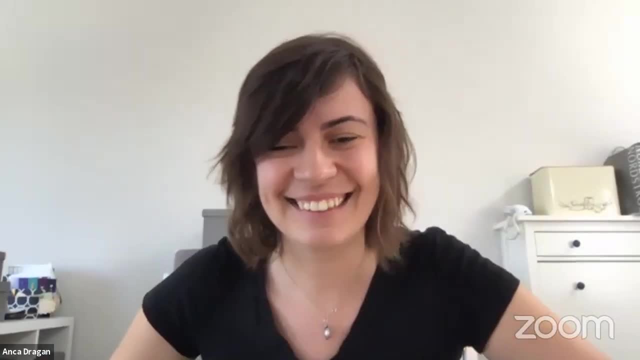 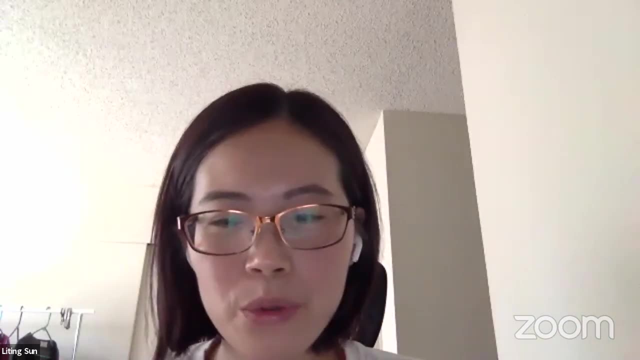 thank you very much for having me and for organizing this. yeah, sure, and if you, uh, do you mind like answer? yeah, you already are sorry, so so, uh, i will go for the next speaker. so our next is Charlie Tang. He's a deep learning researcher. 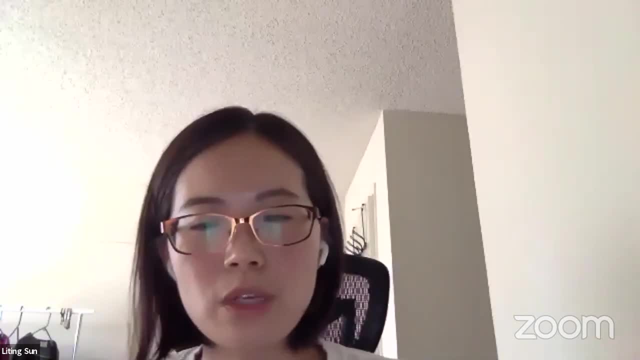 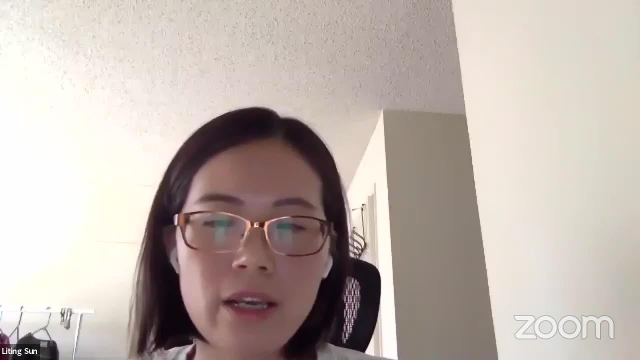 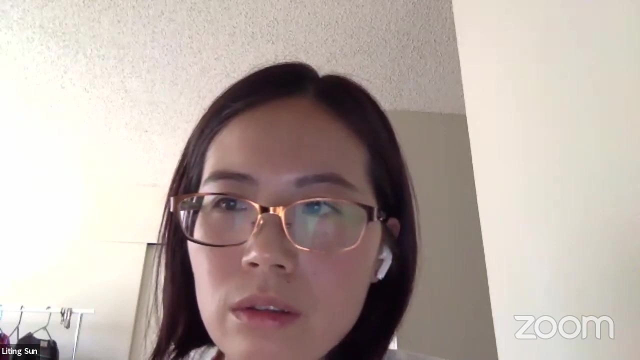 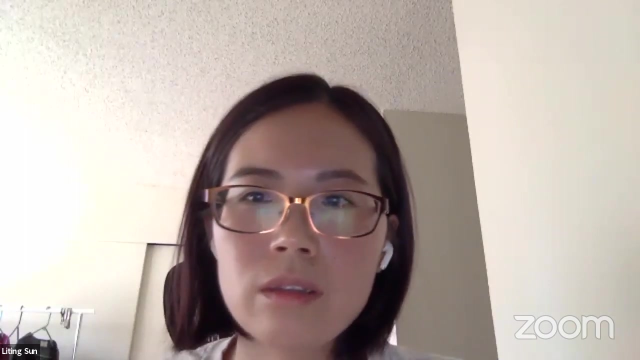 engineer and entrepreneur. He obtained his PhD in 2015 in machine learning from the University of Toronto. His recent work includes many aspects of deep learning in autonomous systems. So, Charlie, I will unmute you. So one second. Can you unmute yourself right now? 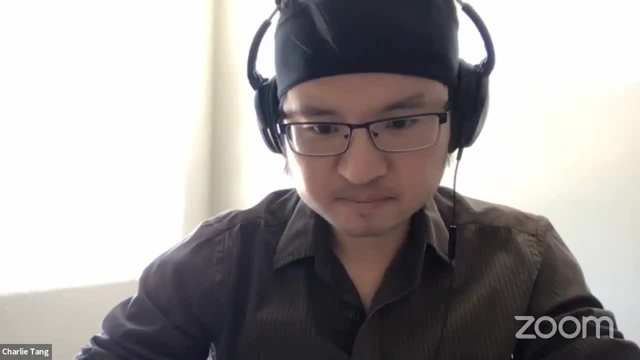 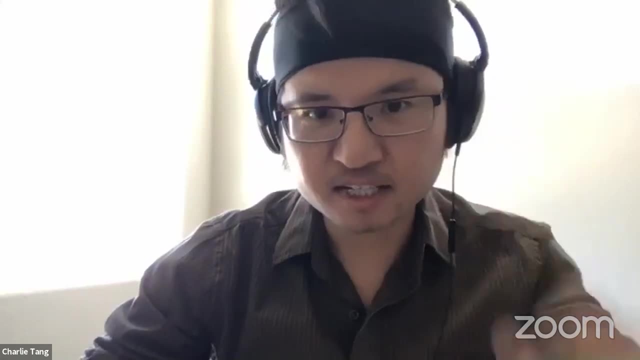 Yes, hi, can everyone hear me? Yeah, it's all yours. Okay, awesome, Yeah, thanks so much, Li-Ting, And I also wanna thank Rowan and Igor for organizing the workshop, And I'm really excited to speak with you guys today. 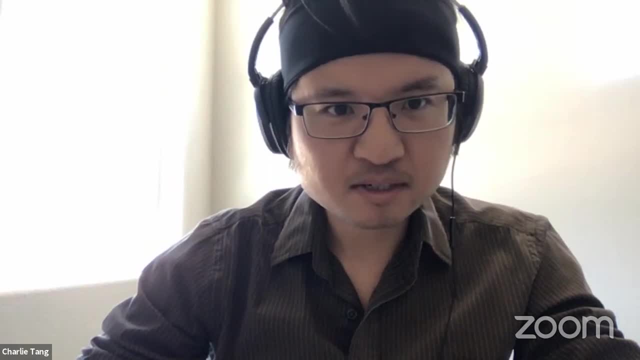 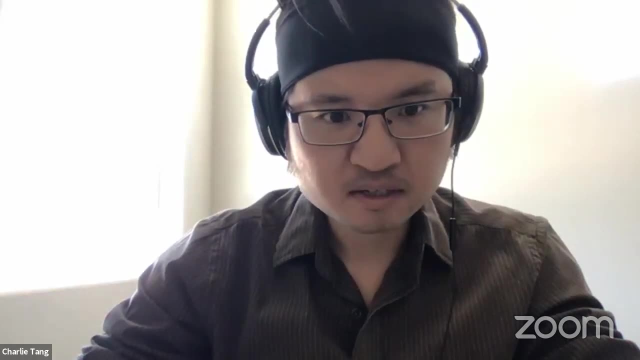 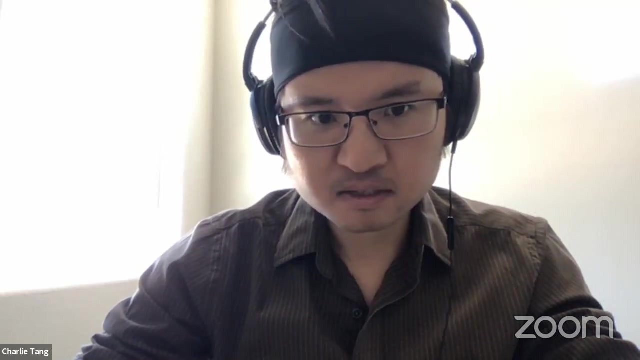 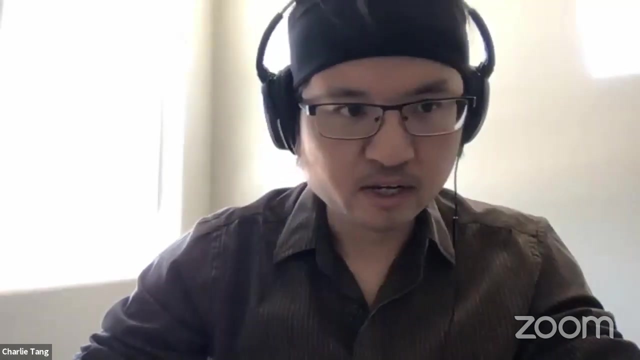 Let me share my screen. Okay, I might have to log back in Apologize real quickly, So give me maybe 10 seconds. Yeah, sure, Yeah, in the meanwhile, like maybe you can if you still have more questions for previous talks. 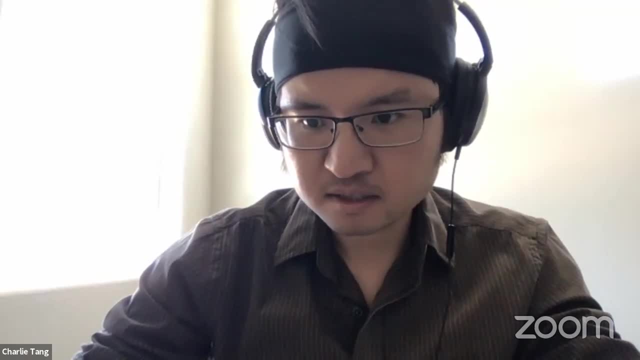 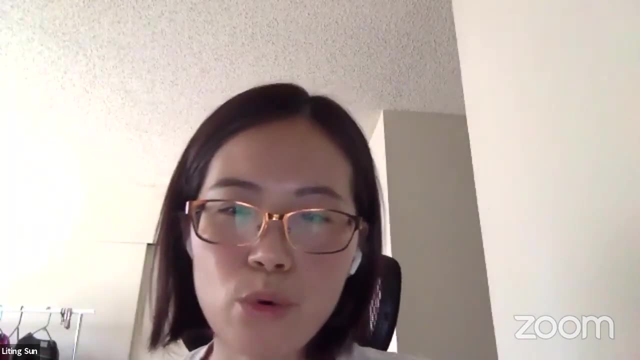 you can still ask them in the Q&A box. So if you have any more questions, please feel free to ask them in the Q&A box And I'll see you in the next session, Thank you. Thank you, We will still post on the chat. 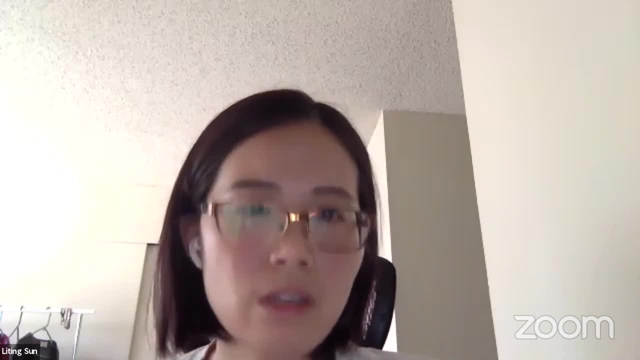 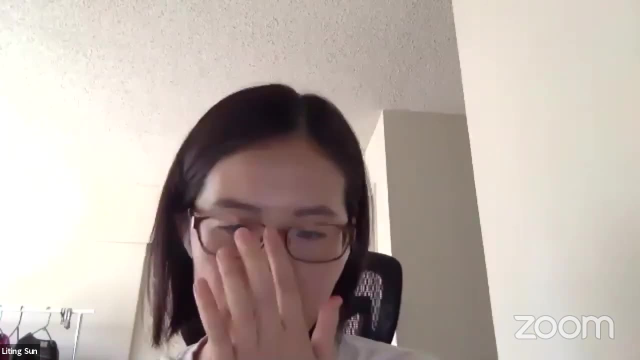 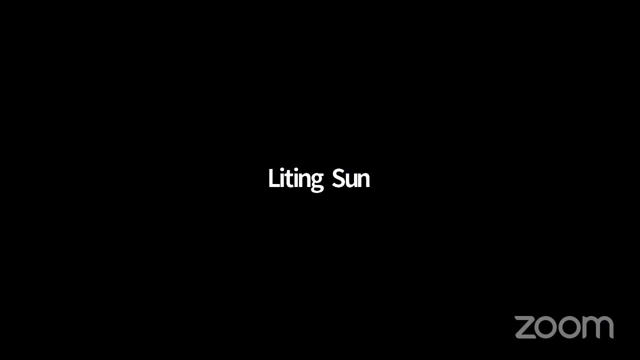 And then we can, because in the afternoon we have a panel session, So we will be able to answer some of the questions. So don't worry about that, And I will see you in the next session. Thank you, Bye-bye. 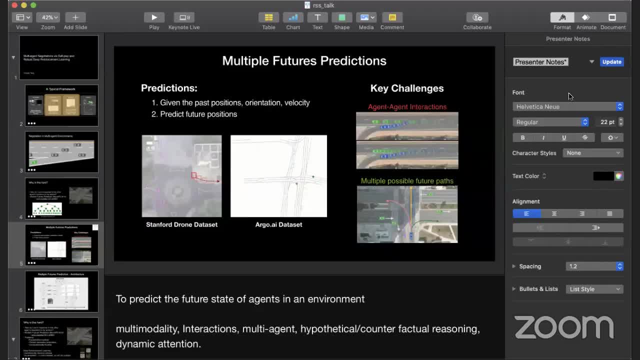 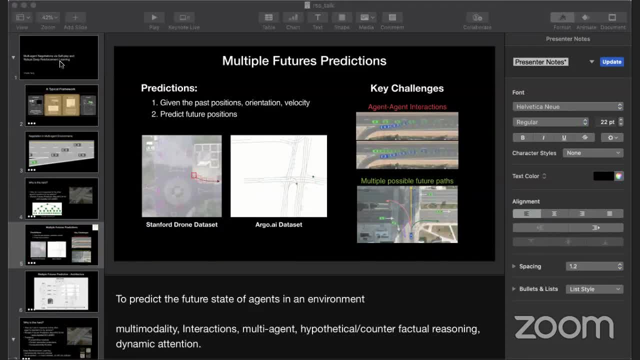 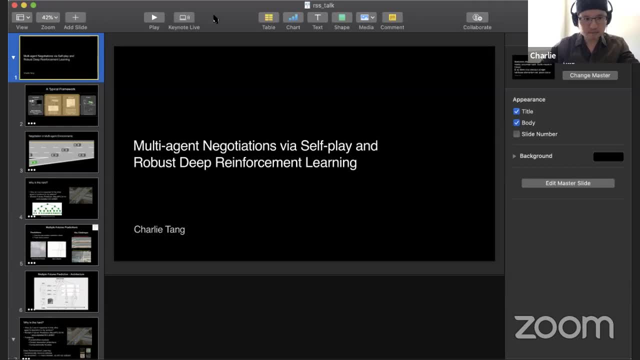 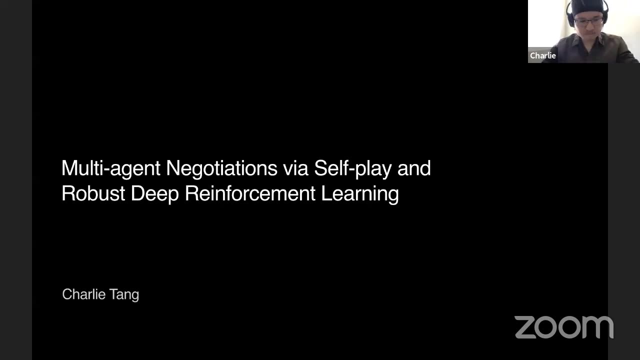 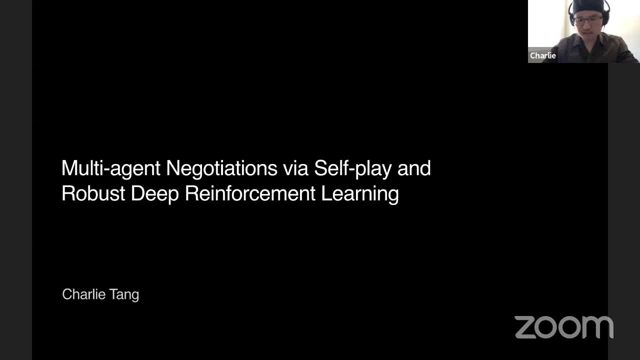 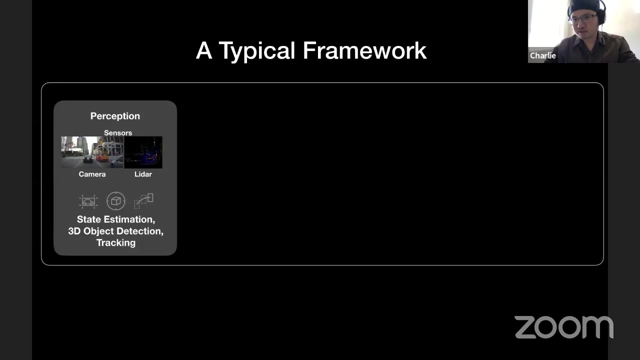 And I want to follow up with continuation on how to do planning with these kind of negotiation And I'll talk a little bit about deep reinforcement learning and how to make it robust. So just an overview on a typical sort of autonomous systems framework. What typically you'll have is you'll have a perception stack. 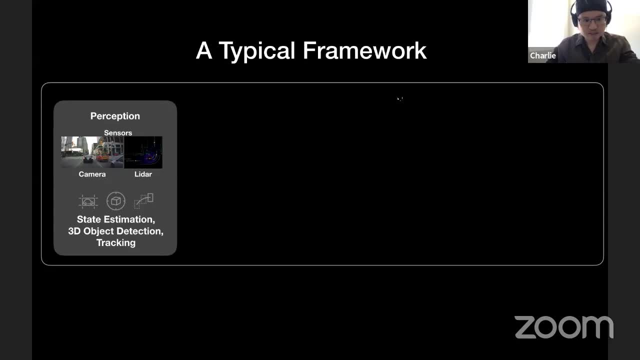 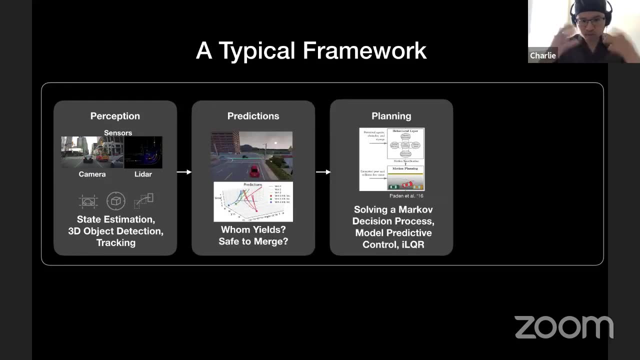 That module that takes cameras or lighters and basically does tracking and detection, And then you'll have the state of the world basically formulated for you and then you'll do predictions and then followed by planning And then in the end you have the controls. 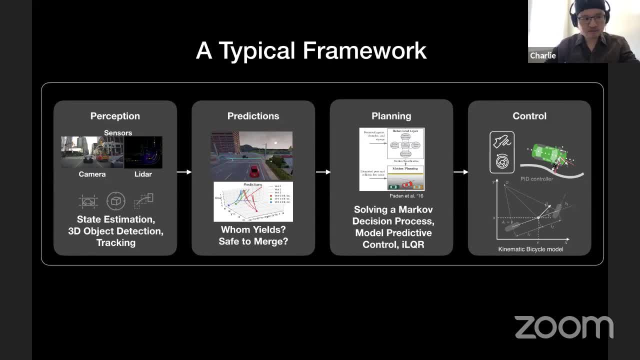 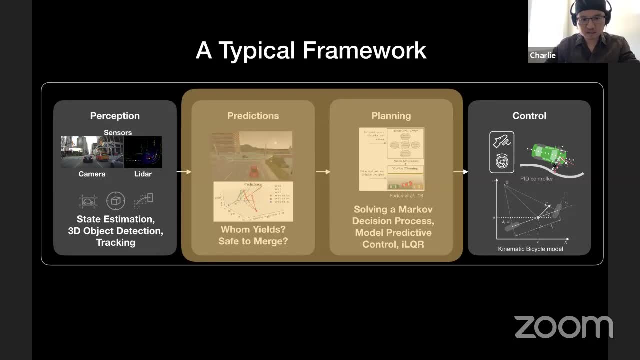 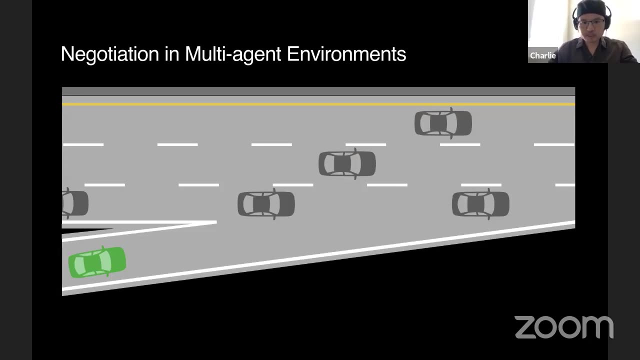 So that's the typical framework And we're going to, for the sake of this talk, we're going to assume that perception is going to be really good, almost perfect. I want to simply focus on predictions and planning part. So the kind of situation we're really interested in is what's known as negotiations. 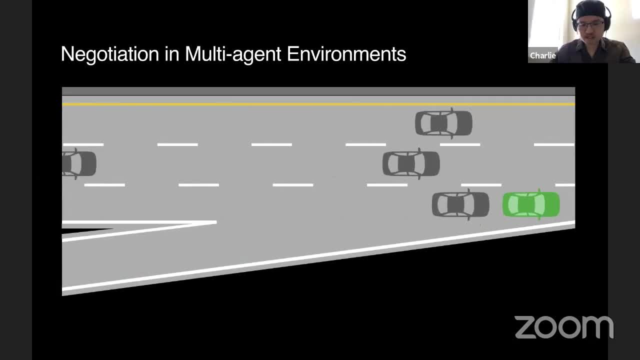 So imagine we're the green vehicle and we're trying to merge onto the highway. So we have to make sure that the gap is open and where we can safely and robustly merge onto the highway. So this is the kind of problem. And so you might ask: well, why is this hard? 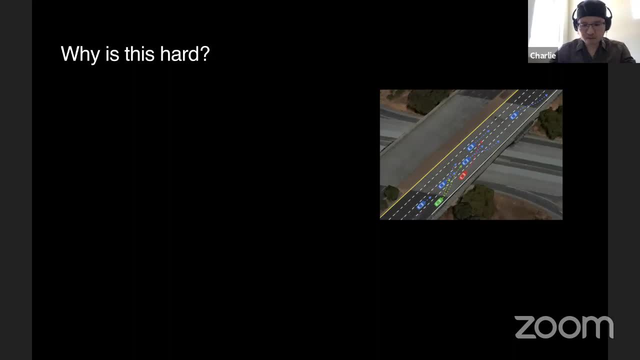 Humans does this every single day. Why is this hard for computer algorithms? And the reason is that we must be able to act in response to how other actions or agents are reacting to our actions, because our actions can influence the behaviors of other agents on the road. 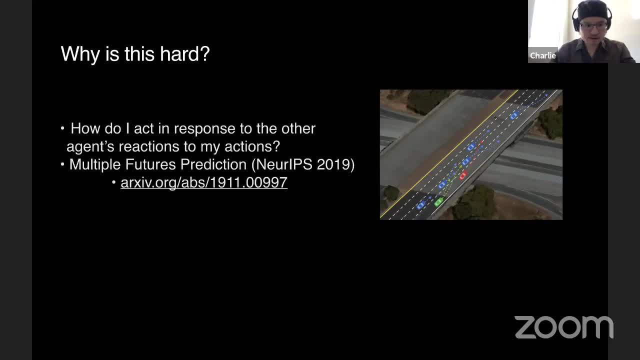 One thing we can do is we can have really good predictions. So we have a paper last year at the NeurIPS on exactly this: How do you do multiple mode, multimodal predictions, And this is a widely studied area. Roman also has worked on this space in the past. 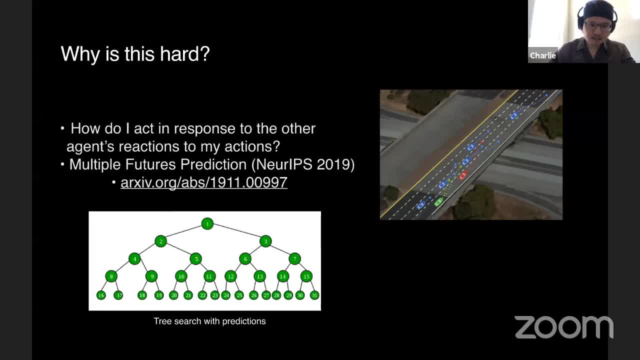 And the idea is that if you have really good predictions, then you can then formulate this entire problem as a search problem. You can use predictions as the edges in this search tree and then find a state that in the future that you think it's going to be good. 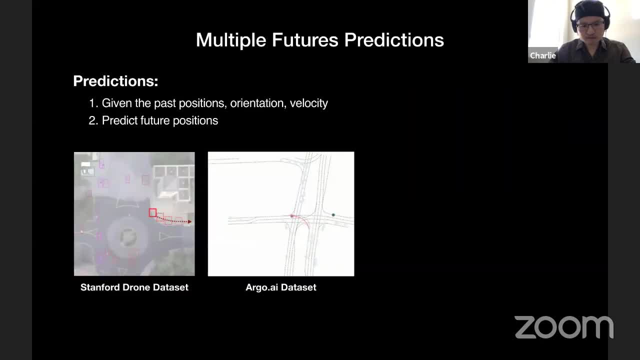 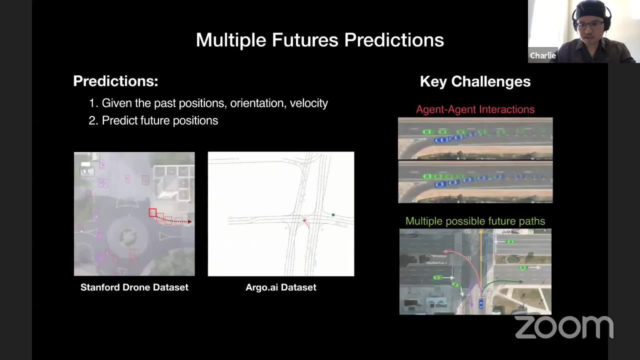 So just a little sort of high level worldview on how do we do multiple mode, multimodal predictions. It's very simple: You're trying to forecast the future trajectories of yourself and as well as other agents on the industry in the environment. But the key here is that you have 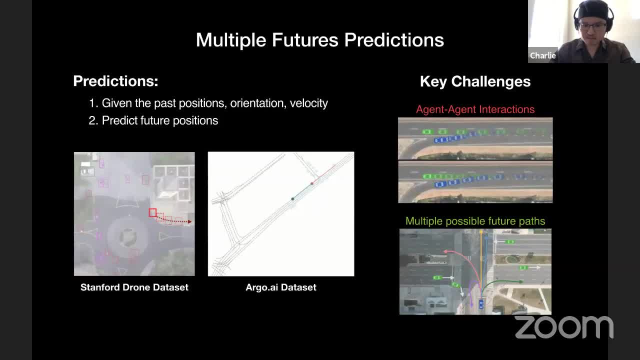 to watch out for multiple possible future paths, So what's called multimodal predictions and also agent-to-agent interactions. So if you look at this example- how the different interactions of who yields to whom really affects the future trajectory that you're able to forecast, 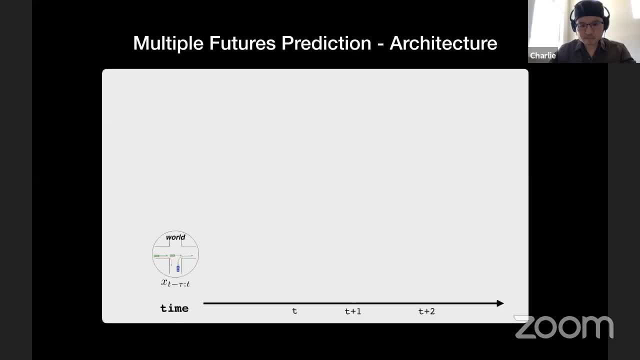 So these are the key problems In this work. we came up with a sort of end-to-end framework that took the state of the world at time t as the input and then really used multiple RNNs to encode the state of each agent independently. 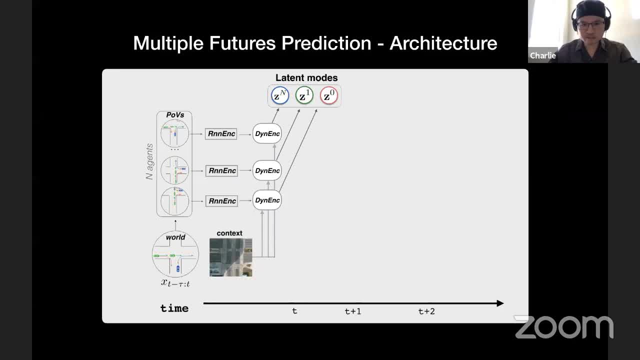 before adding context and also then combining the information and then forecasted the latent variables, discrete latent variables that can represent different modes, such as conservative driving behaviors versus aggressive or left turn going straight. These are sort of these latent discrete modes that we can then estimate the probabilities of before then. 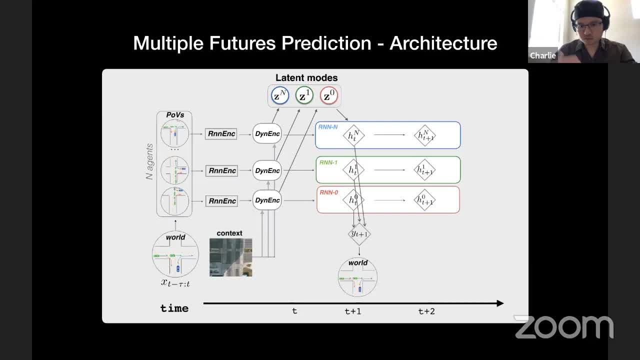 using decoding RNNs to forecast the trajectory of the world, sort of unroll them into the future. So this is the architecture that we used And this is one of many ways that you can learn a data-driven prediction algorithm directly from just simply pure trajectory data. 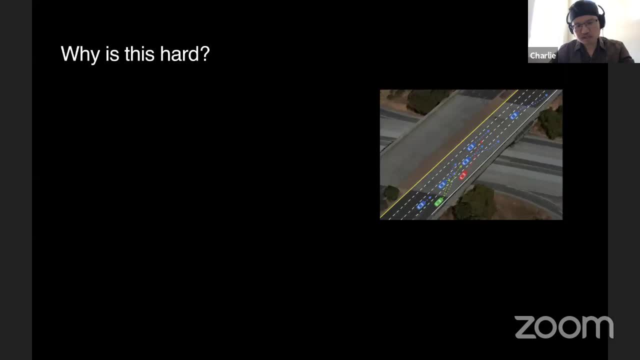 So is that all we need to solve this problem? circling back, And the question is: actually I don't think it's the full solution, And the reason is because the number of possibilities would explode exponentially in terms of the number of agents you have or the interaction you have in the environment. 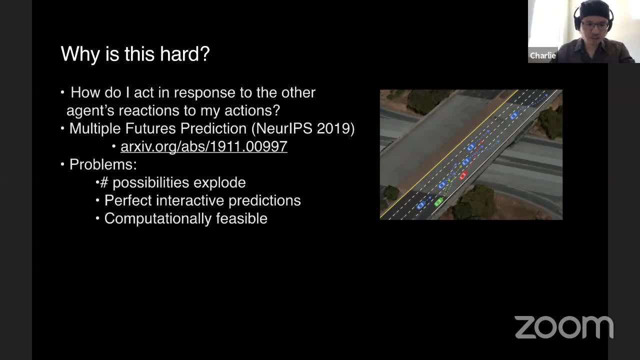 And you really need really good predictions in order to make the system work, And it has to be computationally feasible, So we have to make decisions typically something like every 100 milliseconds real time. So if it takes a minute 20 seconds to compute, a really good solution. 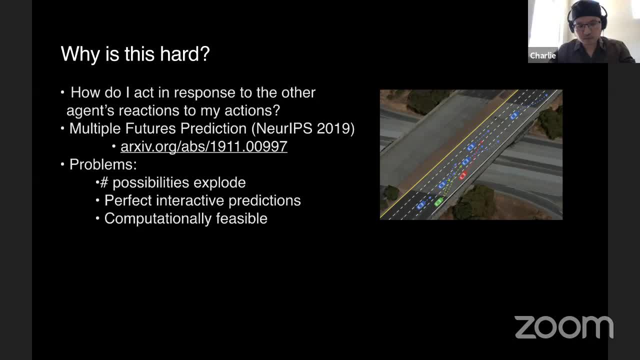 we have a large number of leaf nodes, then that's not going to work. So that's all good If you guys are interested in details. if anyone's interested in details, please check out the archive paper. But for this talk I'm going to focus on something. 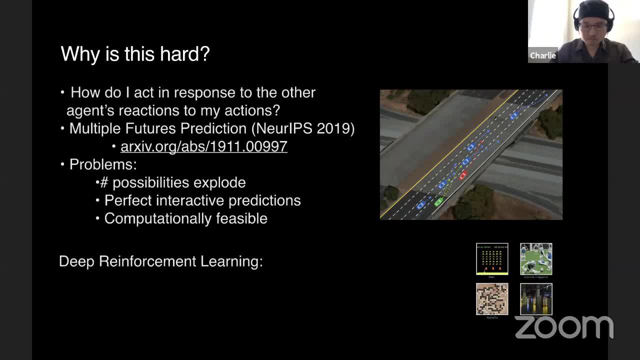 that's more end-to-end. so combining both the prediction and the planning module and leveraging deep RL- deep reinforcement learning- for this At a high level. deep reinforcement learning is able to let us automatically discover policies to do this, Instead of hand coding different policy classes. 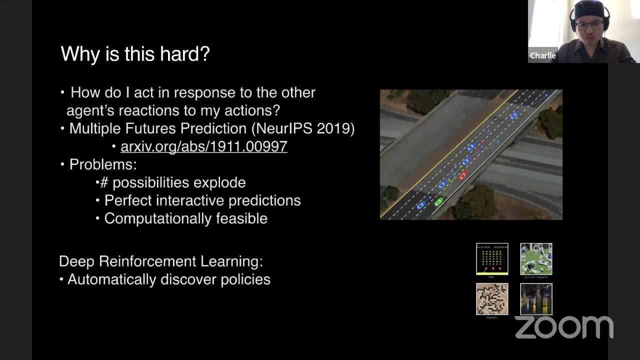 such as a lane change or overtake. we just want to let the deep learning algorithm to find out the optimum policy, And so that's the advantage. But the disadvantage is that it requires simulation, And then, as simulation becomes more and more realistic. 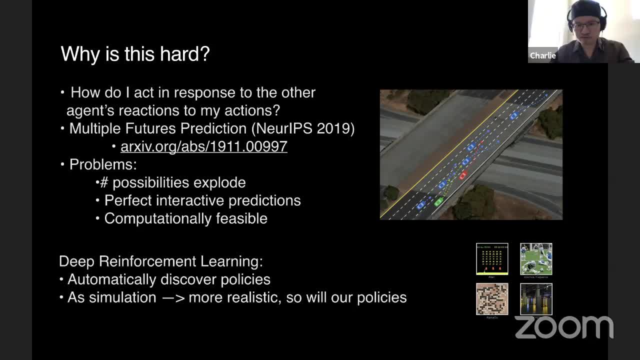 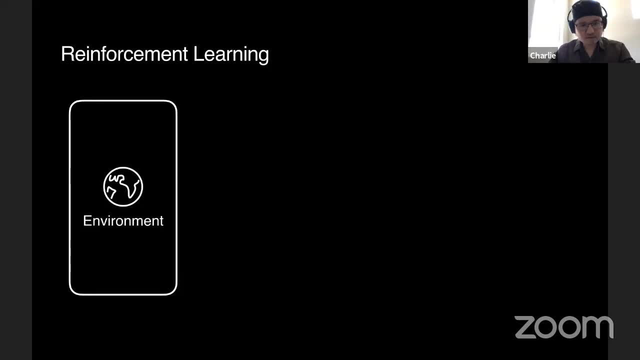 the hope is that our policy would also become realistic and not overfit to the simulation. That's the biggest challenge. it would be overfitting. So for those of you who might not be familiar with RL, I'm going to give just a brief overview. 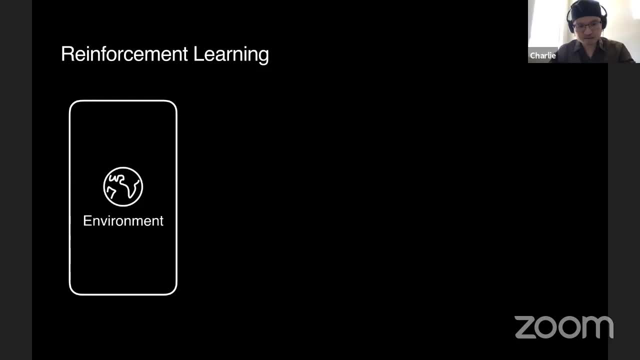 So, with the whole situation, framework of reinforcement, learning, you have an environment. That's the first one, That's the second one, That's the third one, That's the fourth one. This could be your simulation or it could be the real world. 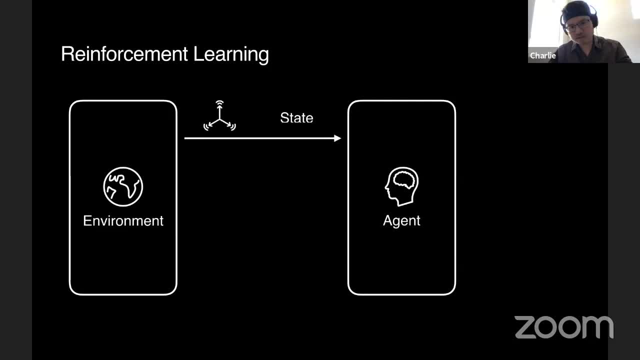 And then you'll have an agent that lives in the environment, that observes certain states And it's able to execute an action within the environment, And then the environment will provide rewards back to the agent. What we care about is the one of the things we care about. 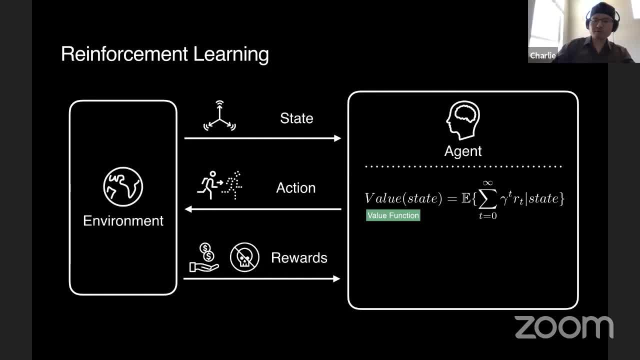 is the value function, which basically specifies how valuable a particular state is, And we also care about learning a policy function that really is that houses what sort of actions to take in any particular state, And then we can use deep neural nets for the policy function. 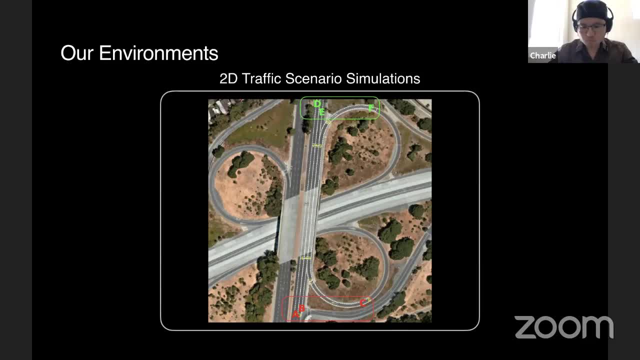 So that's the formulation, And what we've looked at is very simple: 2D traffic simulation, 2D scenario simulation. So here you see that we have a very simple environment overlaid on a satellite image, And the goal here is that you want. 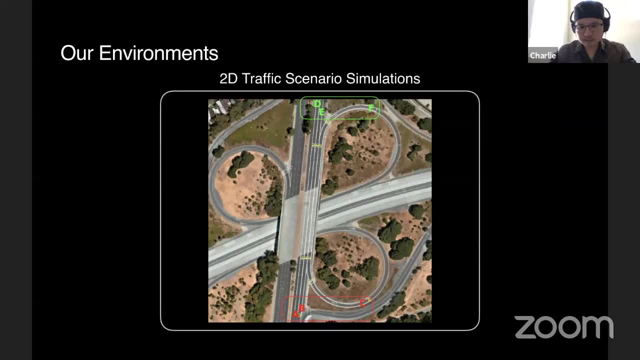 to go randomly from an A, B or C location A lane ID To one of the D, E or F destination lane IDs. This is known as a double lane change or a zipper merge, And it's one of the. it's a challenge. 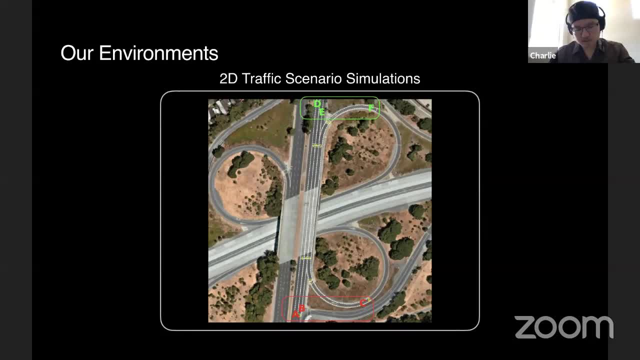 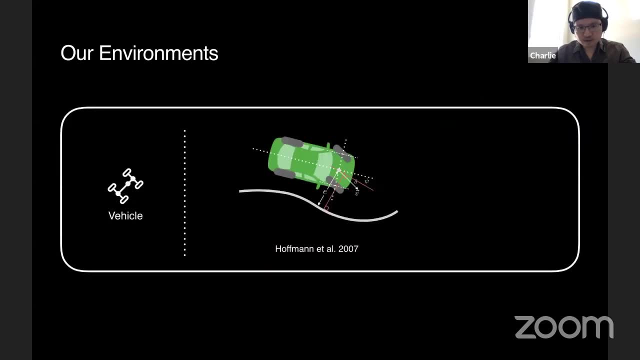 because cars are trying to merge off the highway at the same time when other cars are trying to merge on, So in our case, our agents are obviously a vehicle. We're going to use a standing controller as well as a kinematics bicycle model to simulate a dynamic 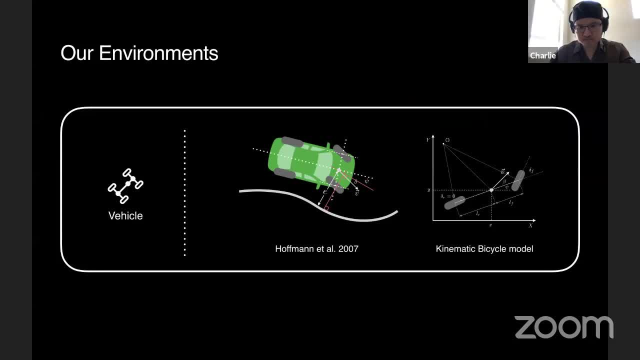 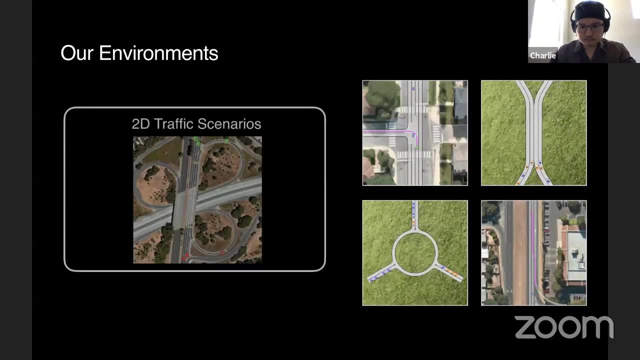 And it gives us a little bit of more realism. The action space consists of both steering, acceleration and turn signals, So here these are some examples of what we can do to simulate different traffic scenarios. You have a roundabout, You have a left turn. 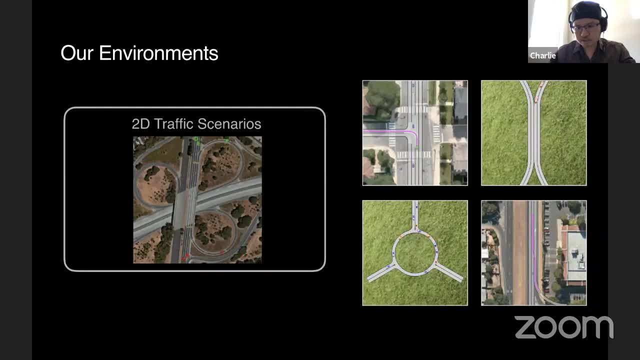 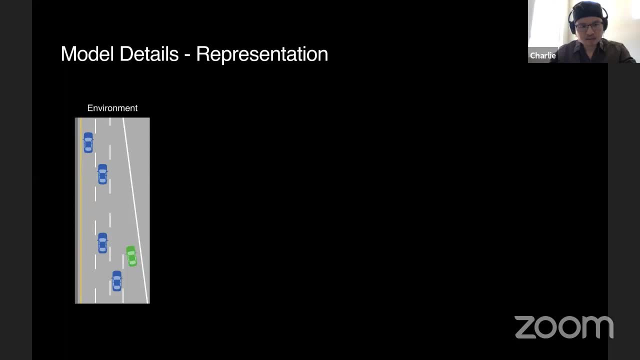 And then you have different merges, So it's fairly flexible in this regard. The way we approach our representation learning is this: So we have an environment that has different agents and different velocities and different states. We need to convert that into a vectorized representation. 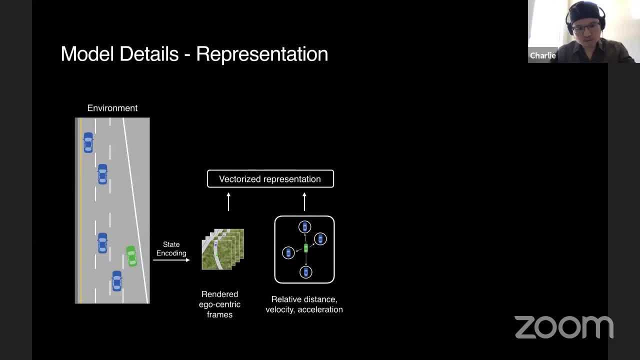 because neural nets like vectorized representation, So this is known as state encoding, And what we do is we take a top-down view and render it into an image, And then we take successive images across times, In this case the past four frames. 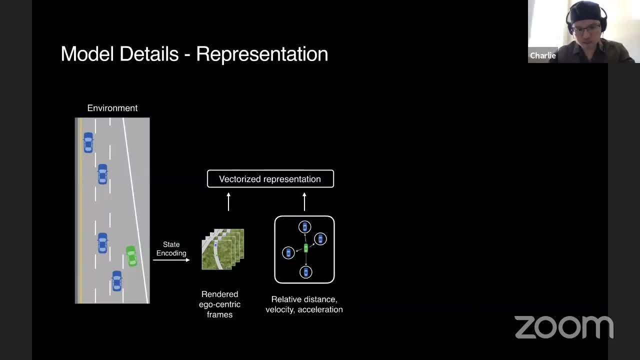 And we treat it as an image. So we perform convolution on this. Then we also have the relative distance of the vehicle ourselves, the software in the car, to the other vehicles in the environment. So these are low-dimensional relative codes And we feed that into a policy function. 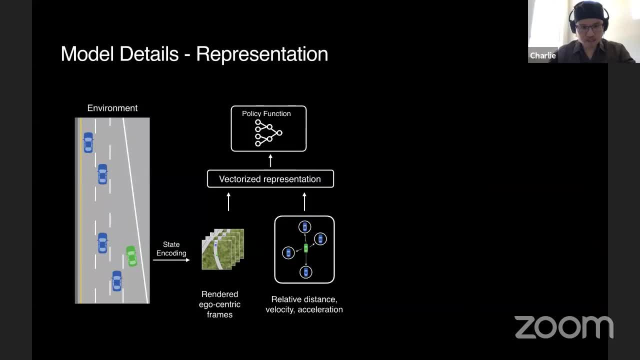 So this is how we encode the environment into something that the neural nets prefer and can understand, And obviously the advantage of training and simulations is that we can parallelize this, So the algorithm we use is a distributed version of PPO And we can create multiple environments simultaneously. 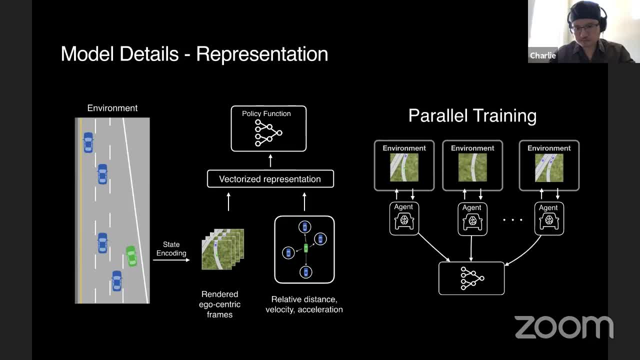 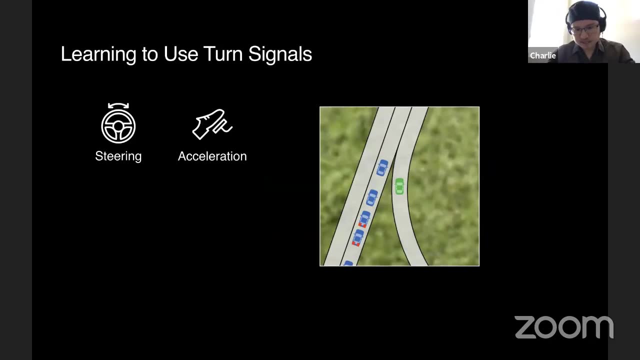 And they'll learn to update the same policy function. And these are examples of doing training. You see that it makes mistakes And it'll restart the environment many, many times. So one of the interesting things we observe after training is that the policies can learn. 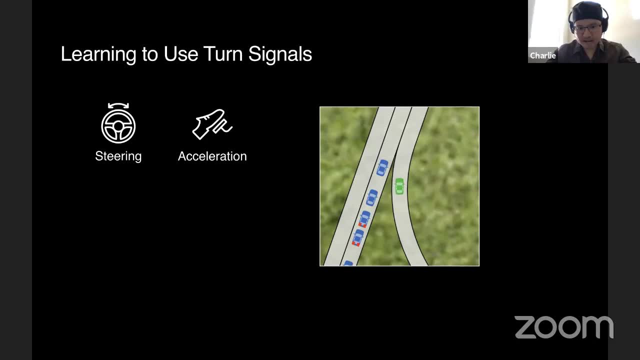 They can learn automatically to use turn signals to induce, open a gap. So in this case, in this merge case, you have lots of basic cars, the blue cars, And there really isn't a gap to safely merge on. But it has learned that if you use turn signal. 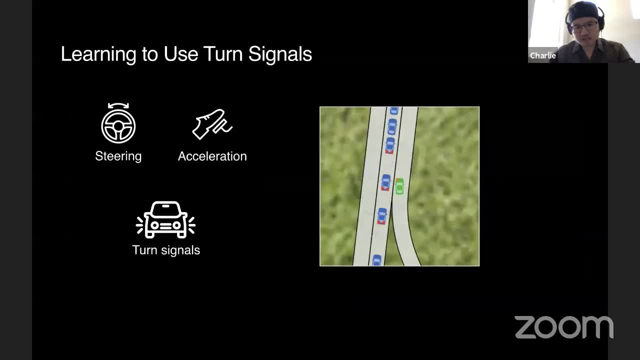 a gap would open up, And it's a good idea to do that. So, again, this is the power of deep RL, meaning that we didn't have to hand code any of these kind of maneuvers or policies, such as turning on turn signal, into the system. 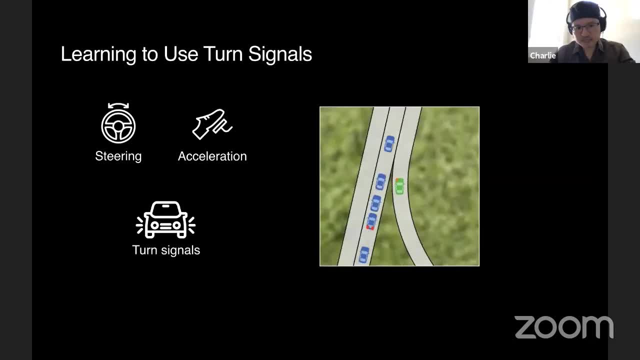 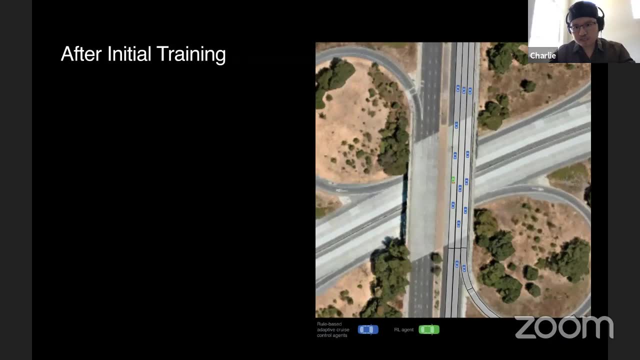 It basically automatically discovered that this is a useful thing to do, And that's the advantage of power of deep RL. So our training setup is this, And what you see here is that the initial policy is trained in the midst of the so-called rule-based adaptive. 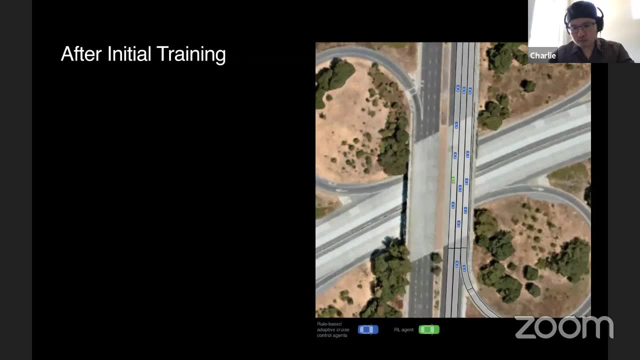 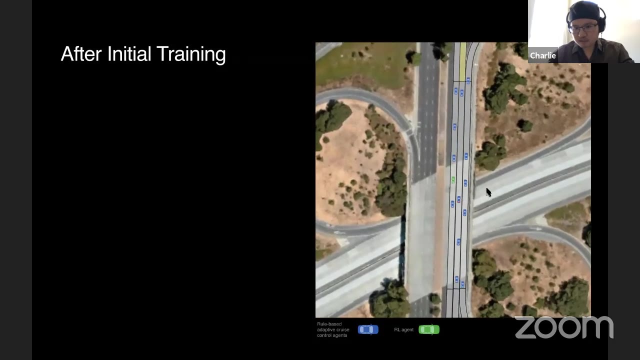 cruise control agents that are in blue, So they're very simple program agents. that basically stays in your lane, does simple lane changes: not to not to collide with the person in front, and so on. So after initial training you'll have 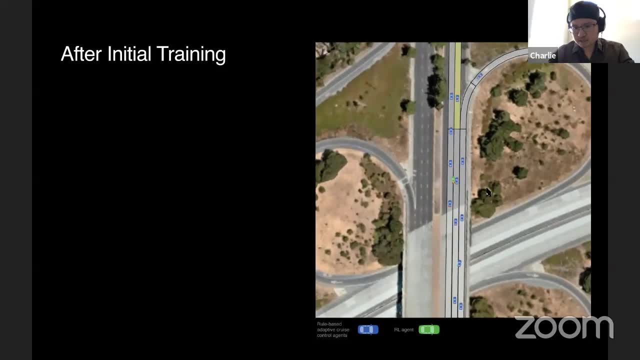 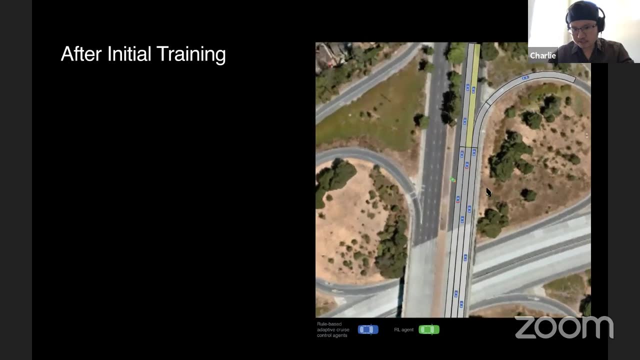 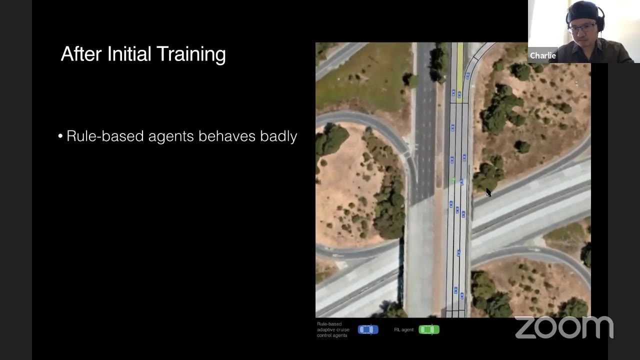 so here's something in edge case that's considered to be failure. What happened was that the blue car sort of tries to merge on the same middle lane And then basically this causes the RL policy to basically go off the side, And this is essentially a problem that simulation would. 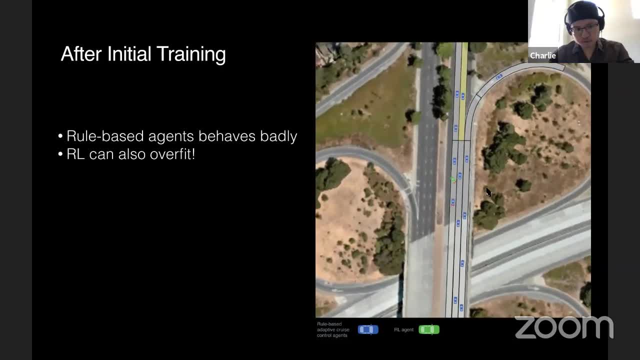 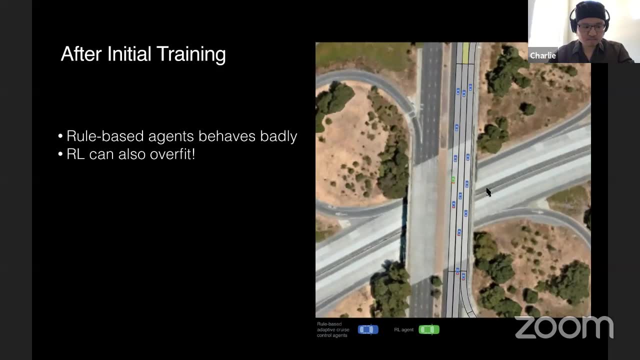 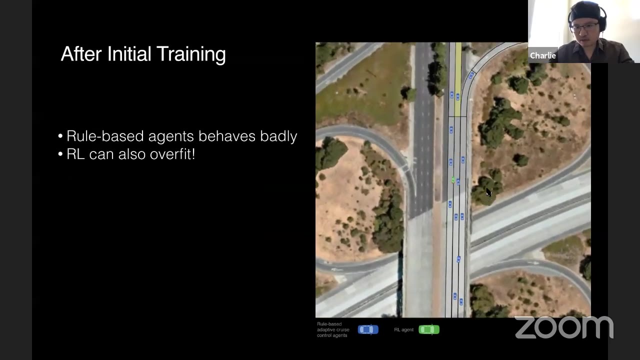 basically a typical problem with simulation, which is the reinforcement learning policy. trained can often more fit And when you have a policy, we have behavior from other agents that they're slightly different or different than the agent that agents that are part of your training environment. 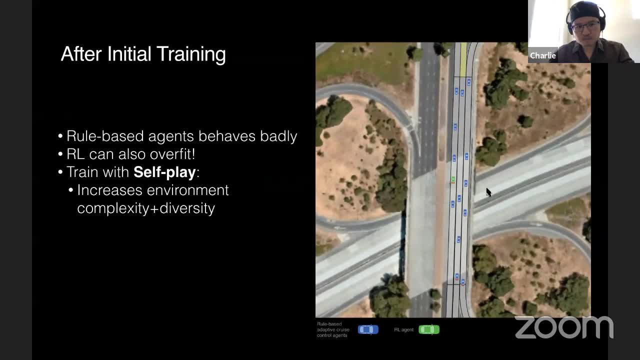 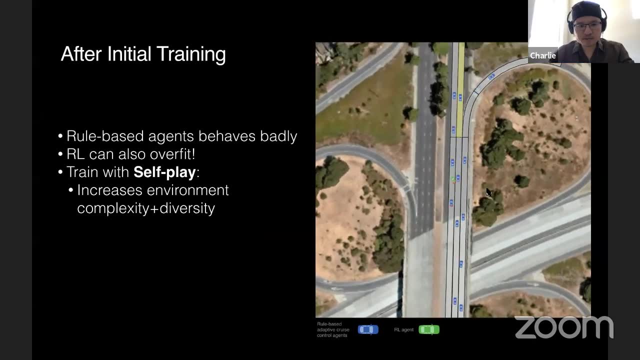 then that's when potential problem can happen. So what we want to do is we want to actually turn to self-play to help with this, to improve our performance, And And the way we do that is with self-play, and I'll talk about this in the next slide. 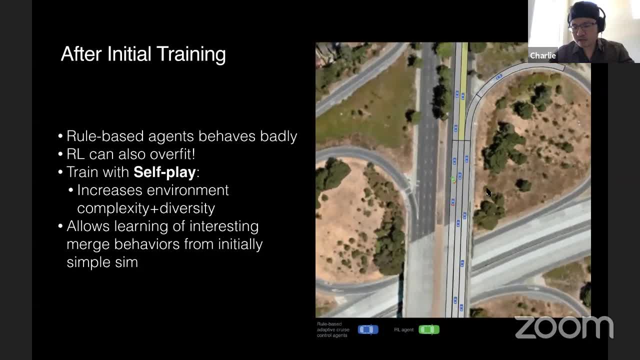 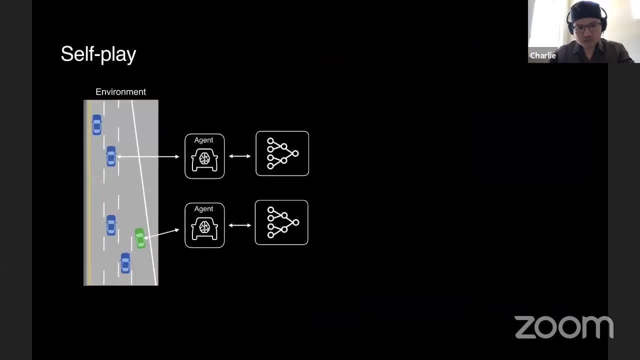 but it really allows us to learn really interesting behaviors from a very, from a relatively simple environment. The environment is simply just essentially a link graph. So how do we do this? Well, so, it's very simple, At the high level, instead of using these programmed AI. 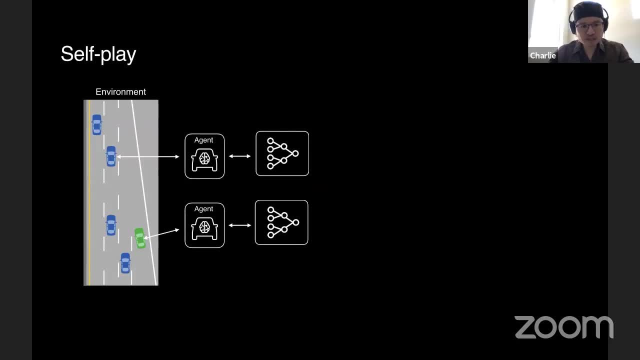 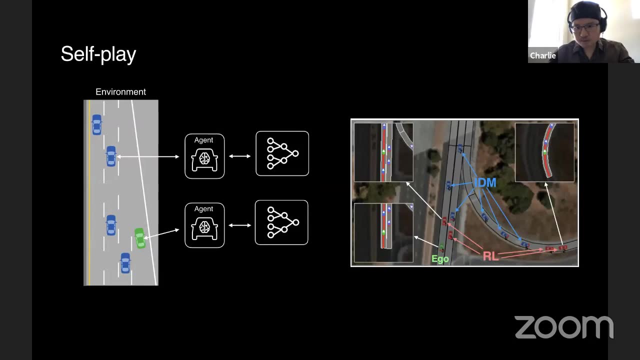 agents or smart agents. we simply replace more agents in the environment with our neural network policies. So, and what you see here is that, doing a typical training run, a typical episode, we'll sample from our existing neural network policy learned and we'll randomly place them as sort of other aspiring partners. 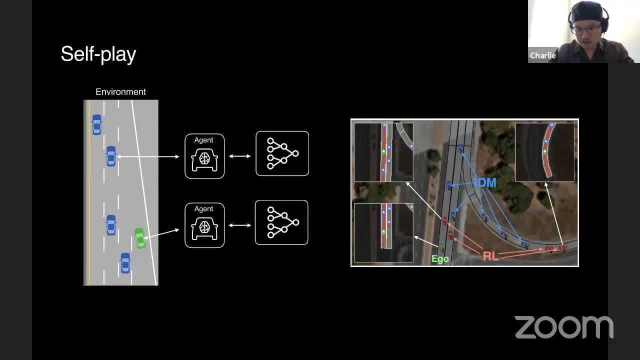 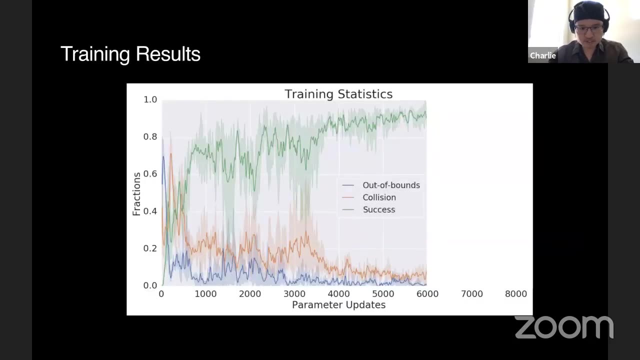 so to speak, within our environment, And these screenshots are exactly the sort of the input rendered representation that these, our neural network really sees. Okay, so if we do this, let's look at how training progresses. So what you see here is the sort of the training curve. 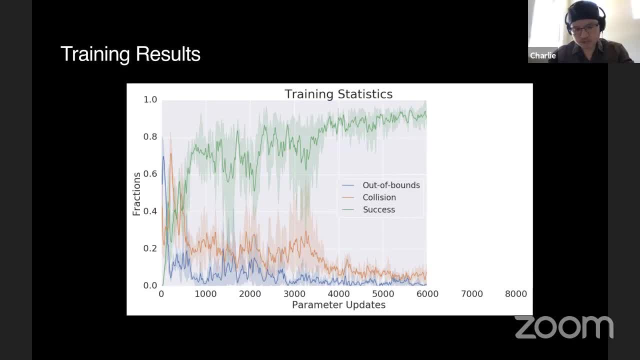 for the first stage, where there's no self-play, The green is the success rate. so how often do you go from A, B or C to D, E or F successfully? And then you have collisions in simulation and you have out of bounds, which means that the car went. 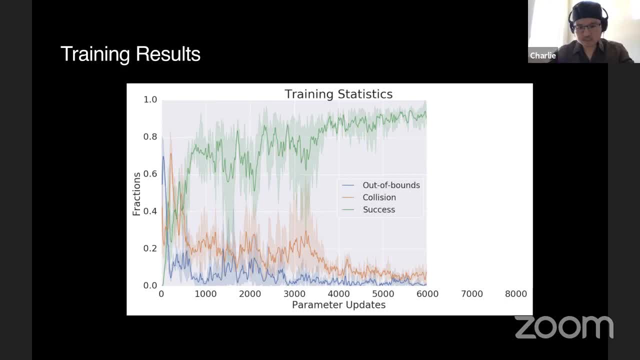 off the road. So the green is the success rate, So this is really good. This is what we expect. As the number of parameters gets updated, we'll have better and better performance. That's stage one. For stage two and three, what happens is that we injected. 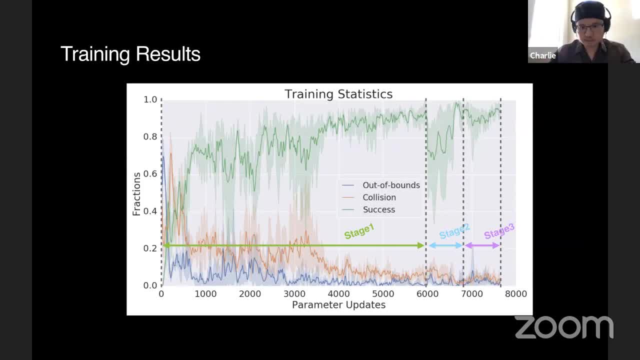 other reinforcement learning agents as part of the environment. So because the distribution of the policy changed, you'll see a huge drop in performance initially, but it quickly. you know, as we train for a thousand iterations it'll go back up And for stage three we'll mix in with different 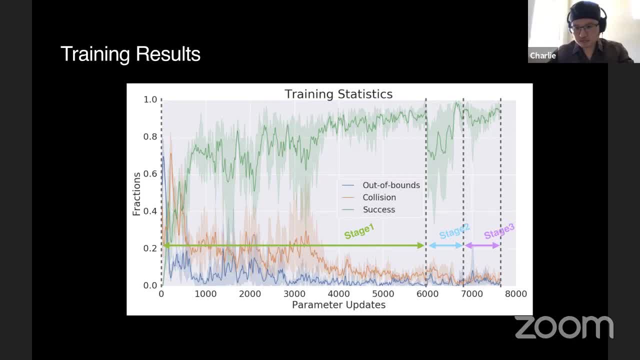 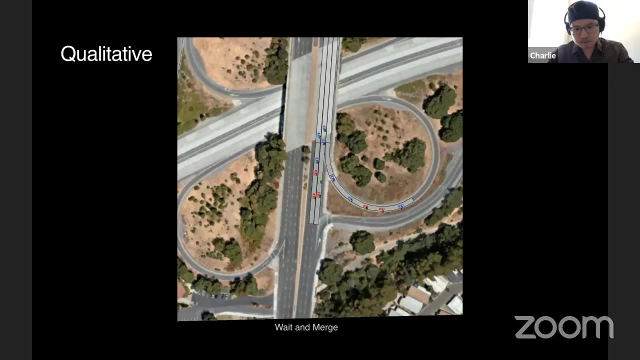 also different set of policy distributions for the other agents in the simulation, the training environment, And same kind of things happen. You'll have different stages in performance with what else to jump, Okay, so that's real quite simple. I mean, this self-play thing is being used in AlphaStar. 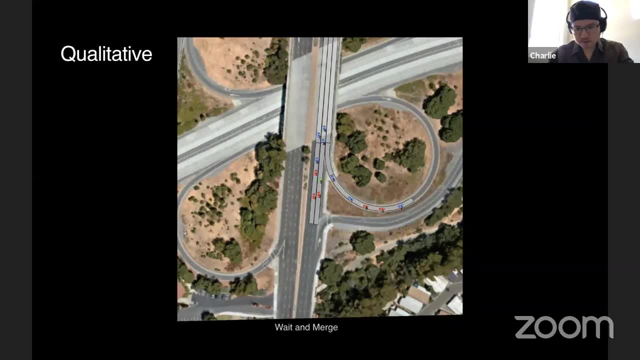 amongst other sort of works from OpenAI, for example, And it's really shown to be a- you know to be- a really good technique for adding diversity right to the environment And when you have more diversity in your training environment. 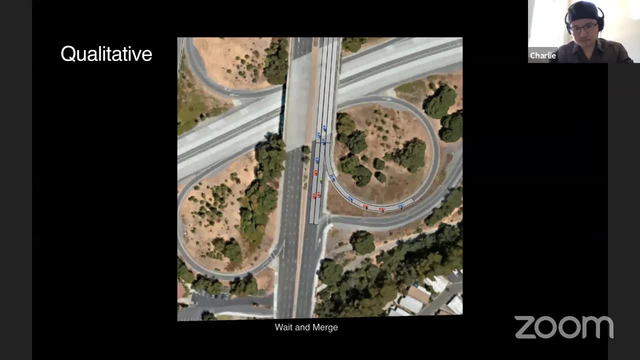 especially for reinforcement learning. you're going to have more robust policy and it will generalize better. So let's look at some qualitative examples of some of the behaviors that are possible, that you know they're being learned. So here you're, looking at the green vehicle. 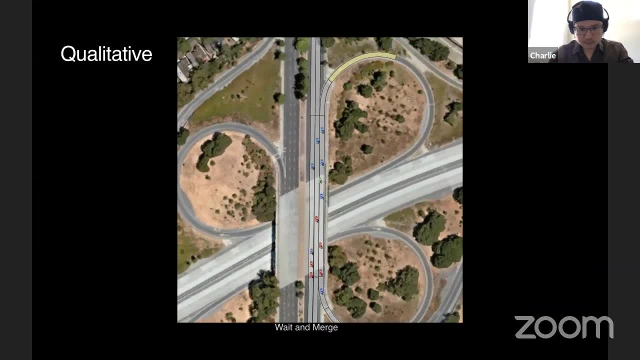 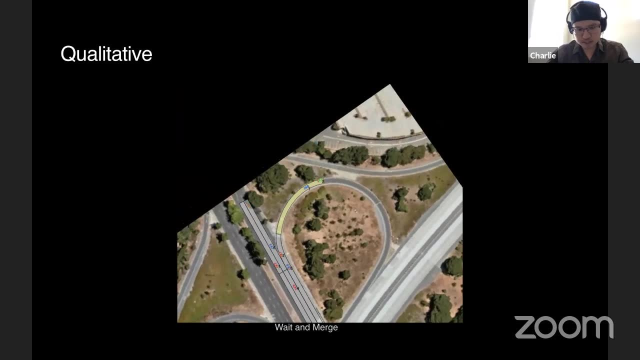 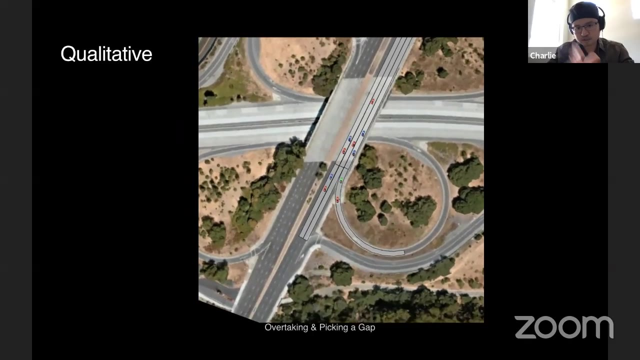 We're trying to do the right lane change And initially it braked Because the car in front of it broke, And then it did a lane change and merged onto yellow. Yellow is the destination lane ID. And here's another example. Now we're trying to merge onto the middle lane. 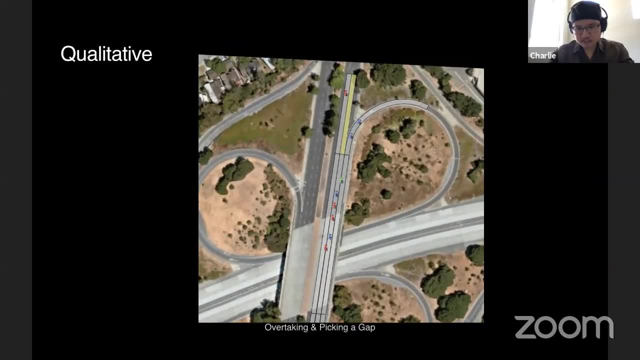 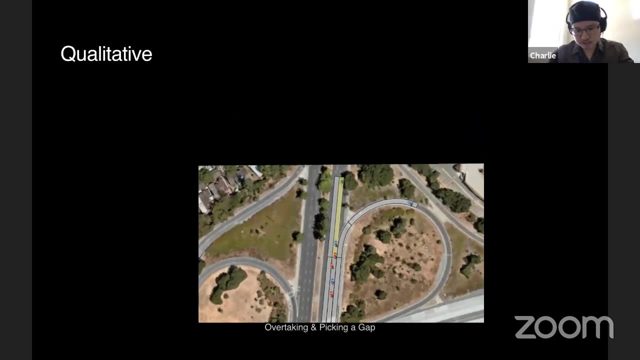 And it waits for a bit and then decides: okay, I'm going to overtake, because these guys are really slow in the middle. The blue cars in this example are the rule-based agents And then the red are other are their reinforcement learning. 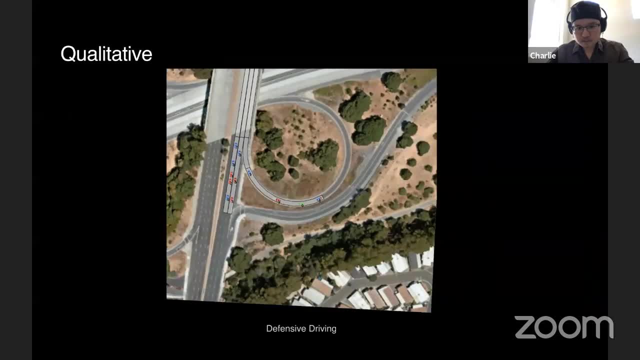 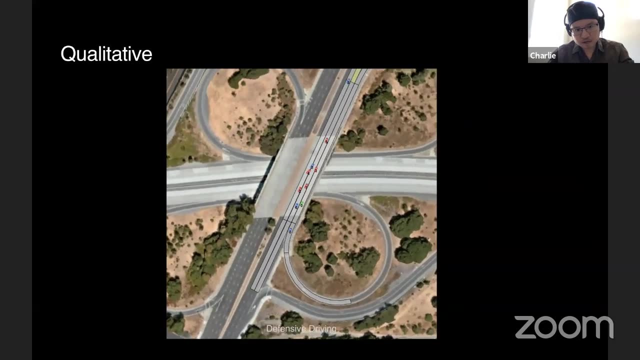 and your network-based policies. Here's another example. This is a similar kind of example, but in this case if you look really closely- I don't know how, maybe you guys can't really see this, but you know- after getting really close to the center lane. 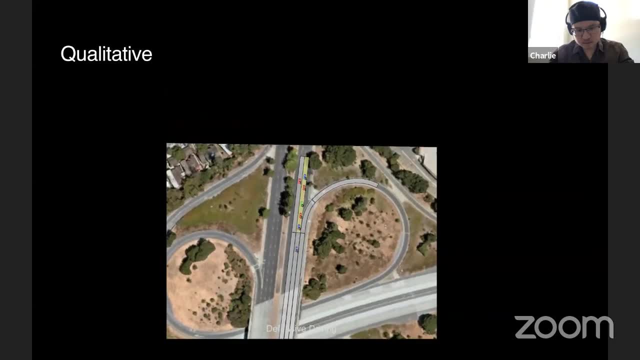 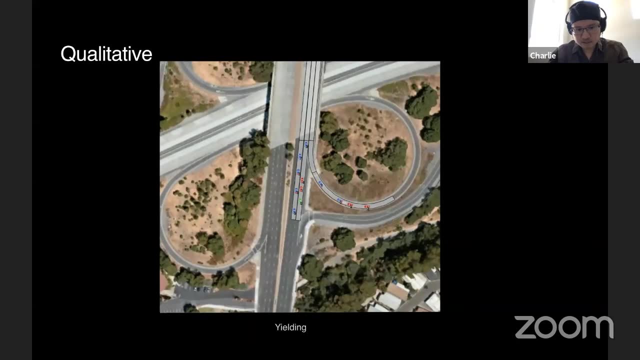 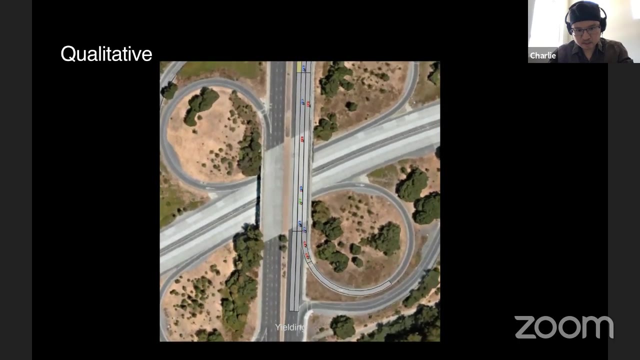 it sort of pivots back to the you know the right lane and to automatically give itself a gap, a margin, And then finally- this is another example- This is a yielding. So this is a- you'll see- an emergency kind of break to yield to the car. 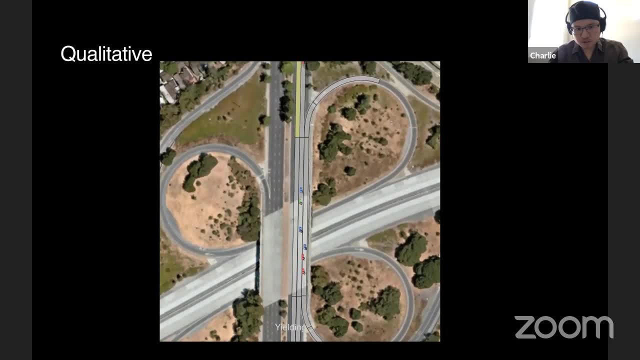 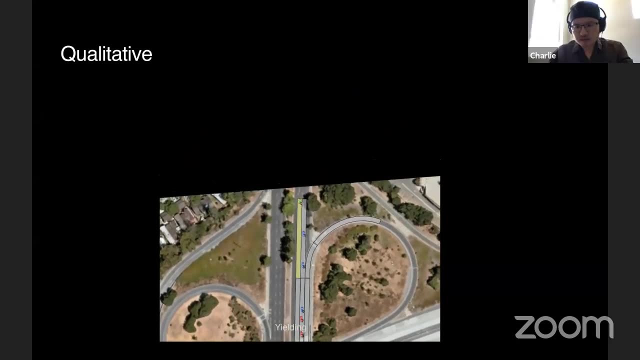 cutting the green car off. So so again, if you look at these kind of behaviors, it's, it's just. it really is hard to hand code many verse like this using traditional logic, because people typically have something like going straight. 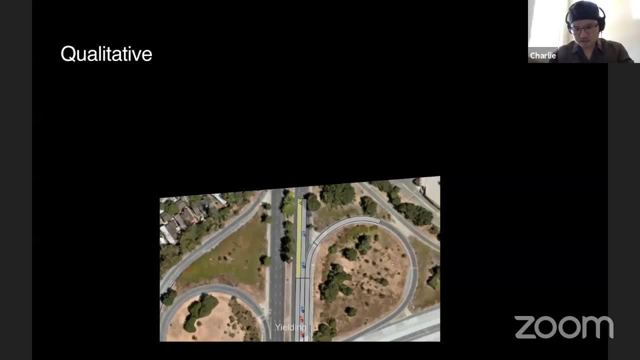 you'll just keep it in the middle of your lane And then, and then it's a finite state machine where now, if you're doing lane change, now you're going to- you'll compute a lane change curve, So the so. 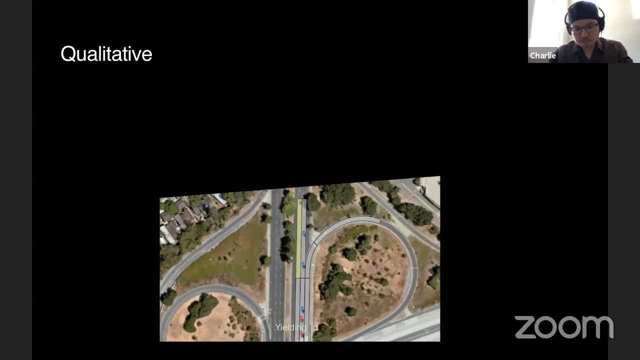 so, compared to those kinds of robotics approaches, the reinforcement learning policies are just more smooth. It's really hard to sort of quantify or qualify what they're actually doing, except that it's trying to maximize, Yeah, The reward that we give it. 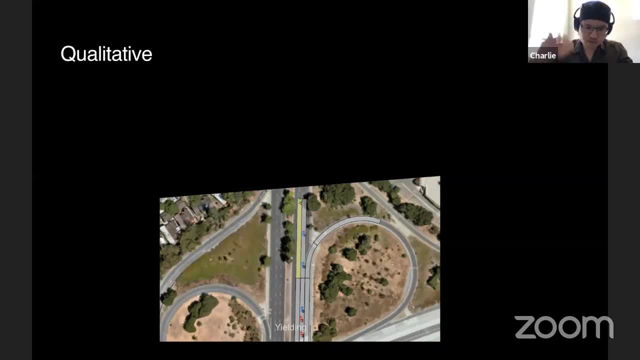 And the reward in this case would be: you get a positive reward for completing the maneuver, going to the correct destination, You get a negative reward for collisions and and also going out of bounds, And then you'll have some velocity sort of rewards for going at a. 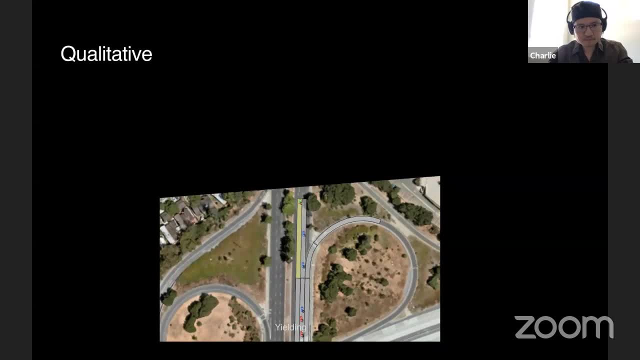 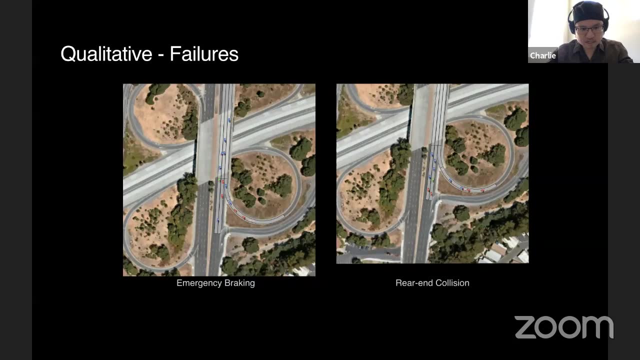 reasonable speed And so on. So is this perfect? Well, it's not perfect. So if you look at the left example, this is the emerging break example. This is kind of interesting. So what happened is that the green vehicle went through this kind of 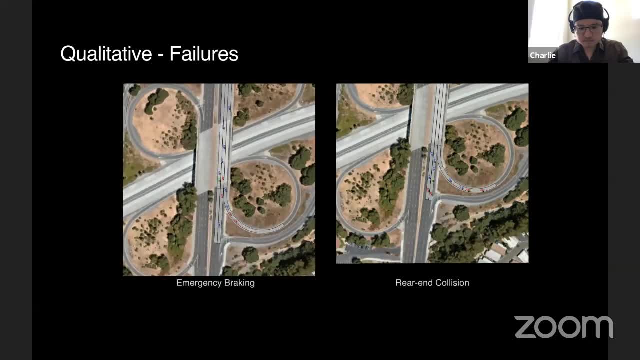 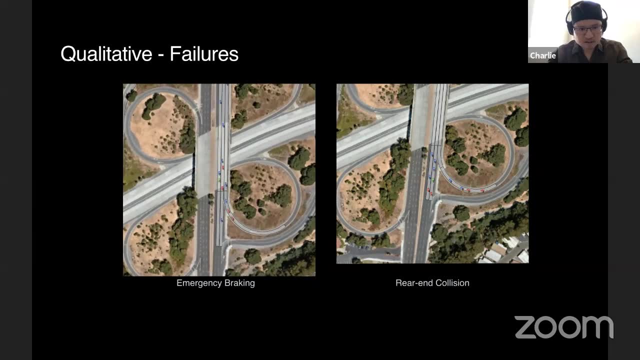 emergency to the desolation, And, And, but it also noticed that it turned its wheel around. So maybe it found that this is a good way to increase the, the braking Distance or or, you know, make it easier to break. 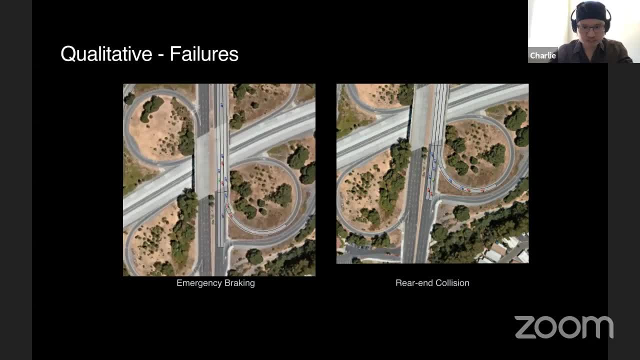 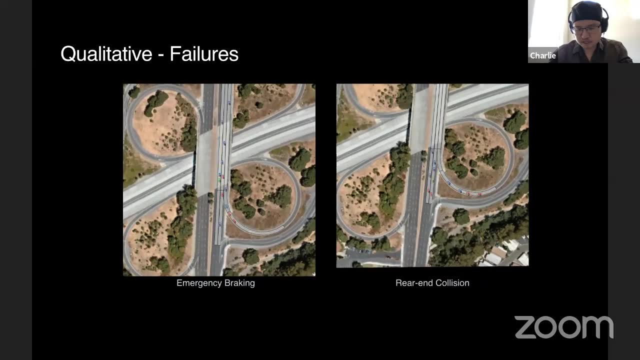 I'm not sure, but this is the interesting kind of thing, that policy that we learned. We also have some rear end collisions. That happens Rarely but it does happen, And so in these cases the car tries to break but it's not. 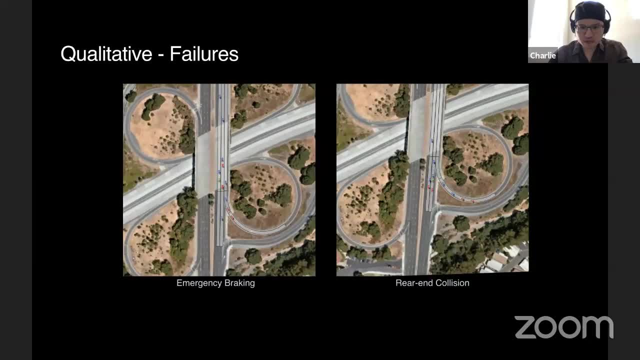 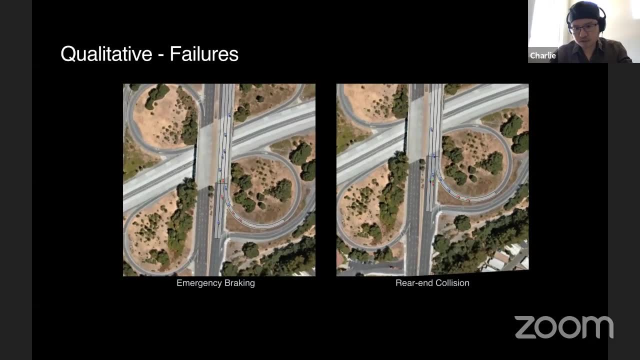 it's not able to break hard enough or avoid a collision. So this is so. I think the these are. the key challenge in the future is: how do you make it more robust? How do you make collisions? Basically, you know How do you make collisions. 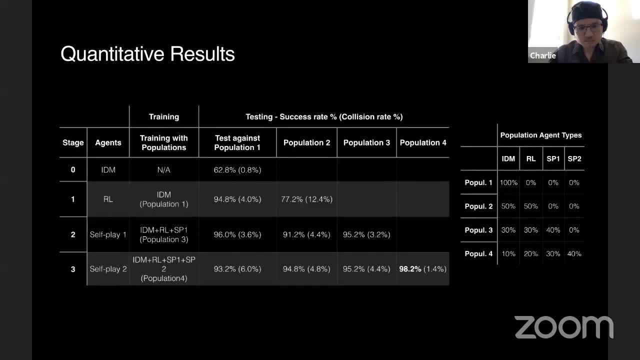 You know How do you make collisions more robust. And how do you make collisions more robust? Basically, eliminate all collisions And And we can look quantitatively. So the result of the simulate, this outplay, is that we are able to. 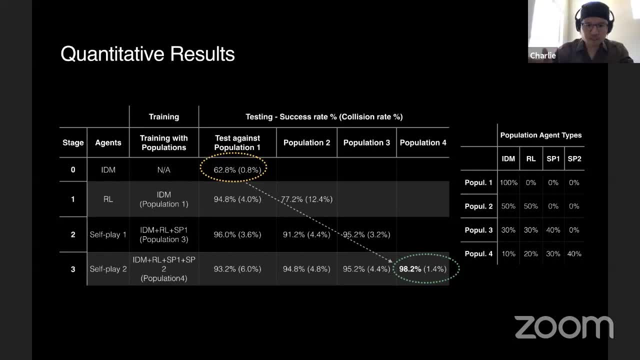 Improve performance from essentially 63% With a simple program policy Out of the up to 98.2%. And then these different populations are Sort of mixture of different, different agent types That we use for different stages: 0,, 1,, 2, 3.. So for stage 2, we're essentially using training with population 3.. And then 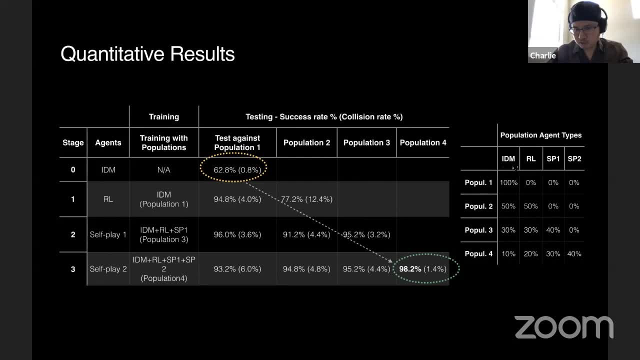 population 3 is a mixture between these programmed IDM agents, intelligent driving model agents, a mixture of RL agents, a mixture of the first stage self-play agents. So there's different ways you can play with the mixture to synthesize the population of training agents that you want. 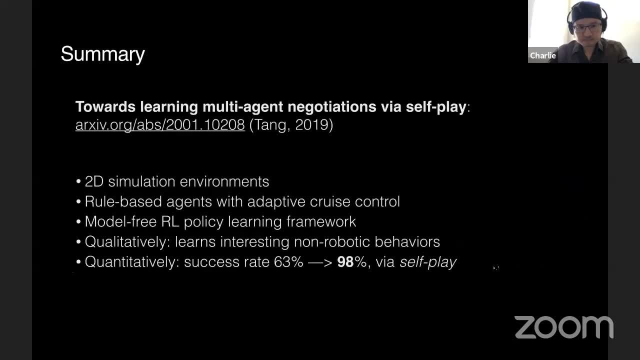 to learn from. OK, so for more details, you guys can feel free to check out the paper archive. But, in summary, we've shown that self-play is really useful, But there are still sort of ways to go in terms of making it more robust and safe. 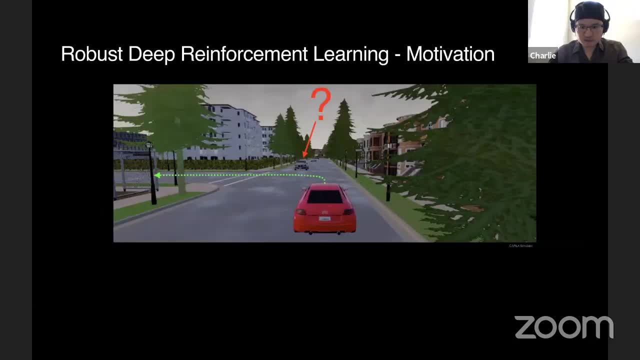 So continue on. I want to talk more about a different sort of different work, but continuation on how to make it robust. This is so in this example. here it's really sort of characterized what we mean by robust, So the fact that we don't really know what the other vehicle in this case 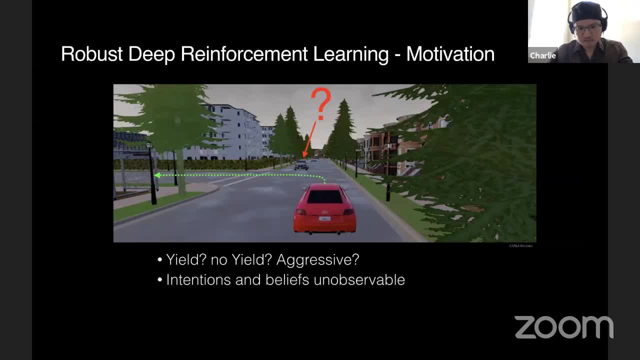 the gray vehicle in front of us is really thinking about is really leads to inherent uncertainty or stochasticity in the future or the future value of the state. So the person in front of us could be: they could be aggressive, they could yield to us or they could not let us. 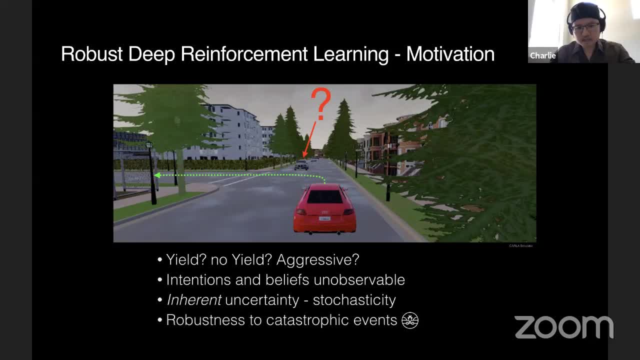 make the turn. So we don't really know. And the question is, in the face of this uncertainty, how are we able to make robust decisions and safe decisions? And so for this we introduce something called what we call worst cases policy gradients. 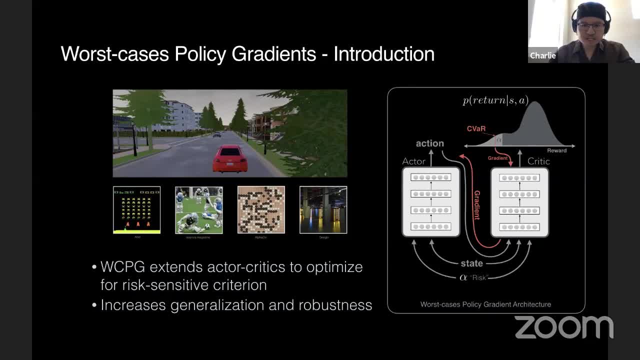 And the idea here is that, because there's inherent uncertainty in the environment, what we want to do is we want to model the entire return, not as a single scalar, but as a distribution. OK, so we're still going to use this. 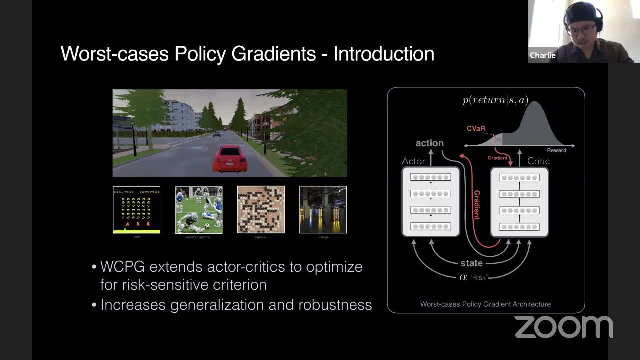 This is something like active critic. This is a standard reinforcement learning technique in the space. But the critic, instead of outputting a single Q value, which is a scalar, is going to learn to model the entire distribution. And then we're going to. 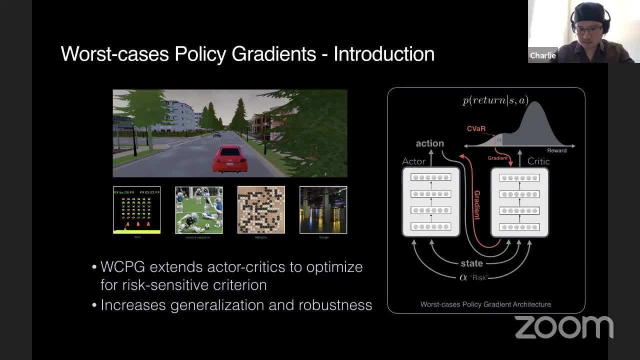 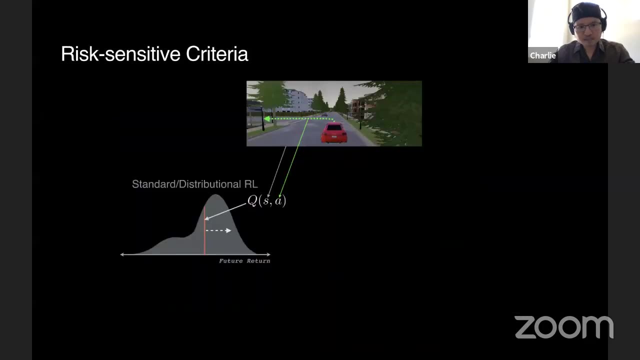 optimize for risk-sensitive criteria. In this case, we'll talk about the criteria in the next slide, But this really is a modification so that we can actually have better generalization, better robustness. How do we actually do this? OK, so in this case, the environment here will be: 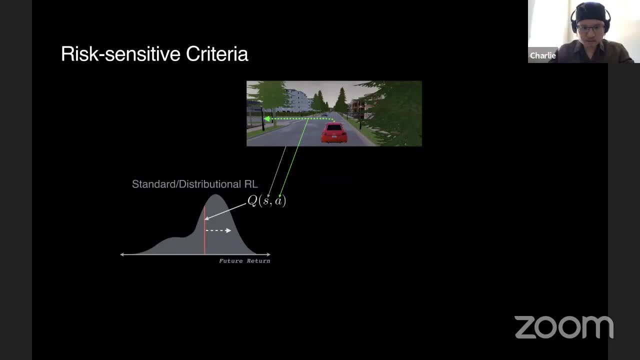 the entire environment of this state. And then our green trajectory could be action. Action could be just simply step on the gas and turn the wheel, or it could be a trajectory. So any of those things could be in action. And now, if you look at what standard RL is doing, or even distribution RL, 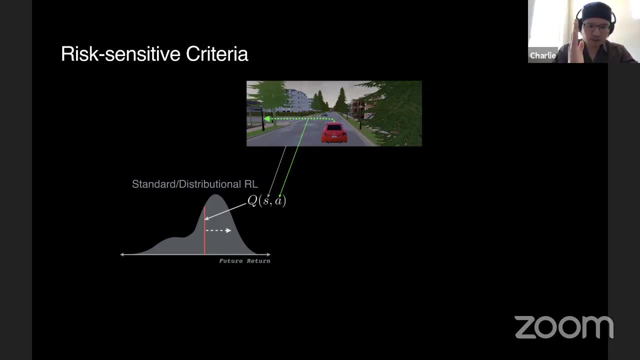 is that it's trying to maximize the red bars. The red bar indicates the Q function. the Q function It's trying to reduce the expected future return. So it's trying to adjust the policy so that we can push the red bar to the right Now, in contrast with worst-case policy gradient. 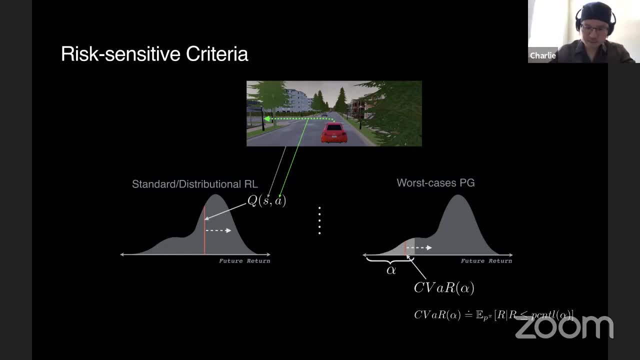 what we're proposing is that we're proposing to optimize not for the entire expectation of the entire distribution, but rather the expectation only up to the alpha percentile of the distribution. So what we're saying is that we don't care about the average return. We care about what the best return would be under the worst possible scenarios. 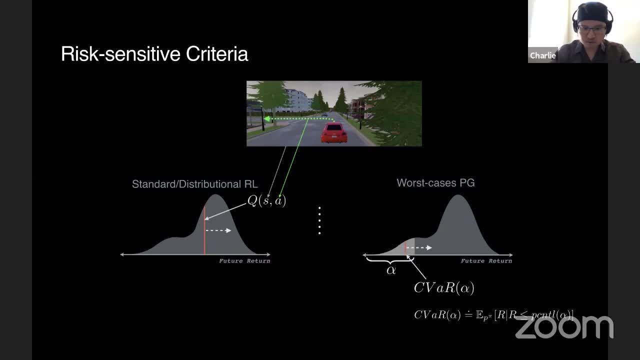 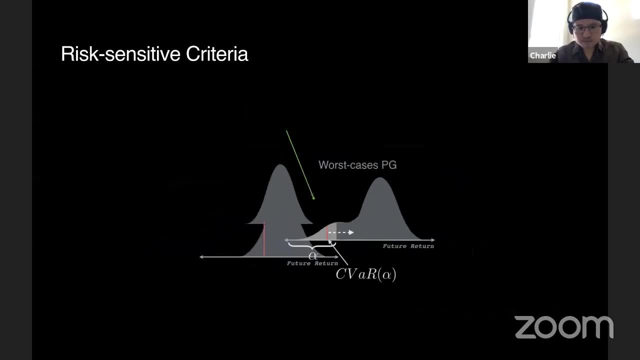 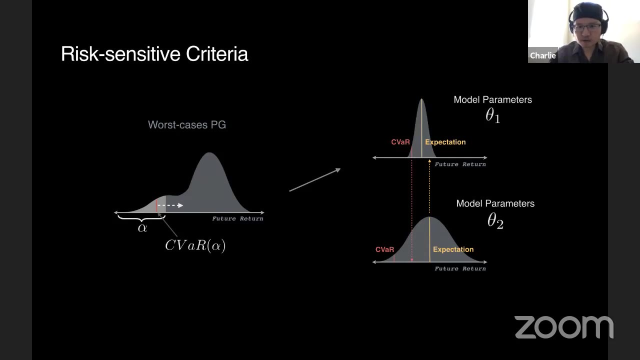 So future returns is scalar value. The worst-case scenario is where the future returns is negative, in this case, a collision or near miss. So that's essentially the main difference. Now, if we do that, what that really means is that we would prefer the policy. 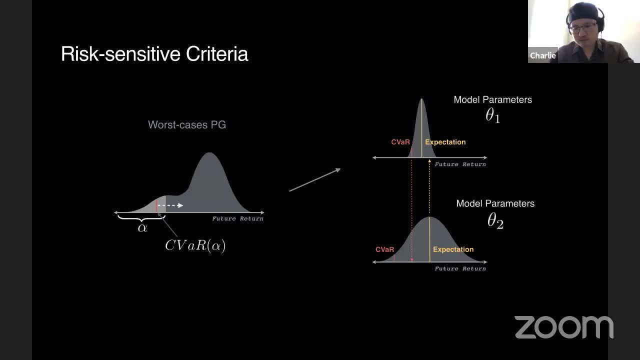 theta 1 over policy theta 2.. Even though if theta 1 has a lower expectation, that's the yellow, And the reason is because it has a lower variance, So it has a higher conditional value at risk. That's what CVAR means. 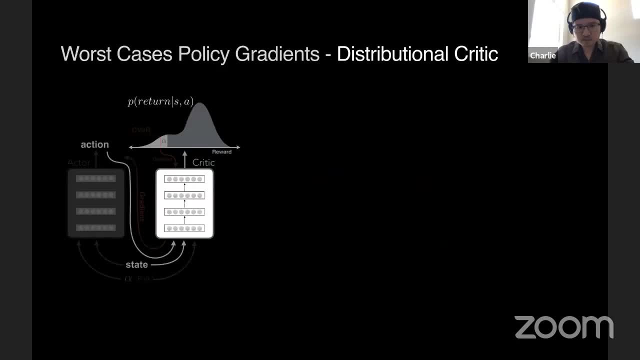 So that's what we're essentially optimizing for Now. how do we actually do this? So, again, the first thing is that the return is not a scalar anymore. The return is actually distribution, So it's a random variable that's called z, And what we're going to do is we're going to make our 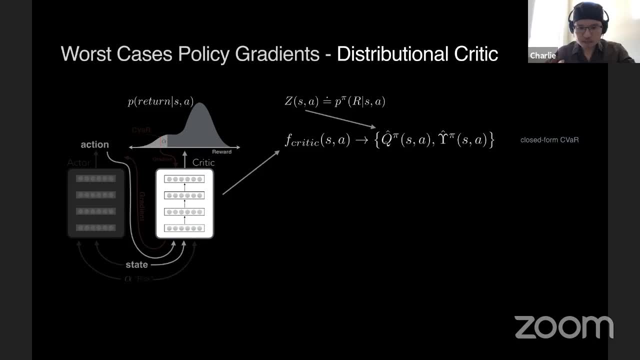 critic to model both the mean and the variance over the z. So we're assuming this is a Gaussian distribution And the reason is that this will lead to a really nice closed-form computation for the CVAR. And because we have a distribution, then we have an equivalent. 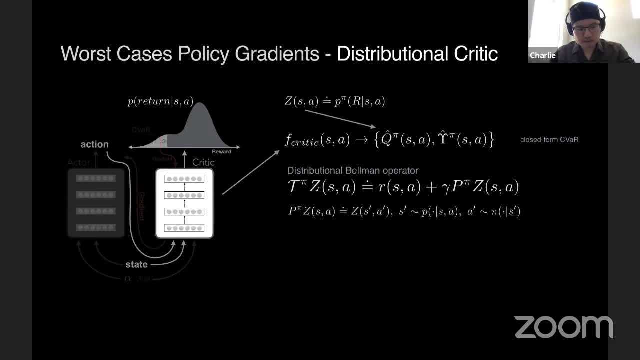 distributional Bellman operator. So instead of the normal Bellman operator, the Bellman equation will have a distributional version of it, And I won't go into too much details of the math. But the update is basically. there's two parts to it. The first part is the standard. 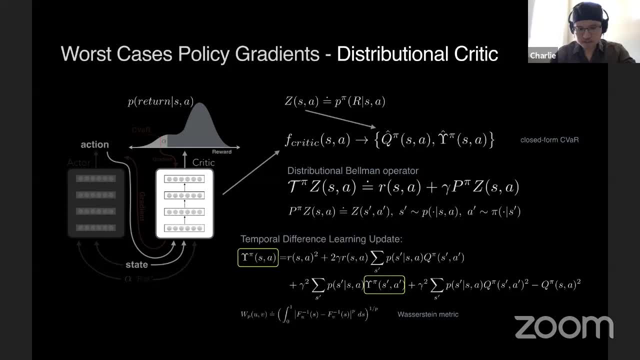 update with the q, the Bellman update that you use for q-learning. The second part is this epsilon, which represents our variance of the z of the future return, And the derivation basically shows that we can also relate the variance from state s prime and a prime which is the future. 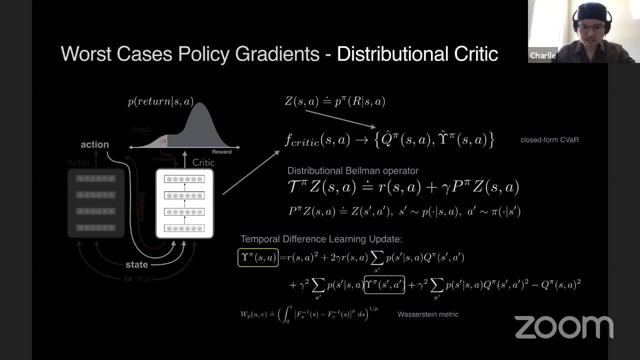 state to our current state as an a. So this is sort of the equivalent backup for the variance, in sort of this way, The td learning sense. And then, once we have that, we're going to update the. So this will be the target epsilon, target distribution of the future. We're going to optimize the. 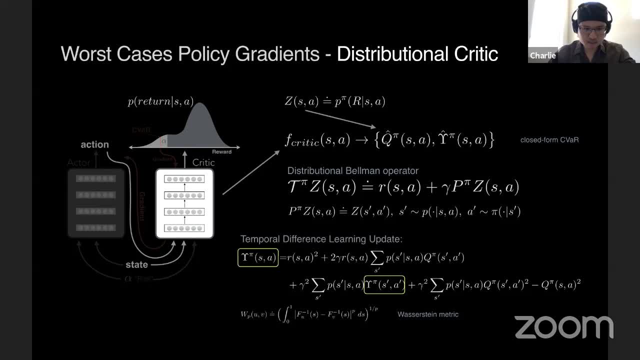 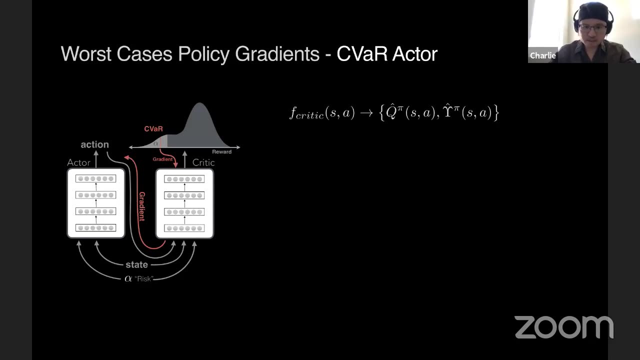 Wasserstein metric from our predicted distribution with the target distribution. So this is just So. now we have a way to update our critic. So with that, how do we update our actor? So what we do is we take our critic and we And given our estimate of the distribution over z the future return. 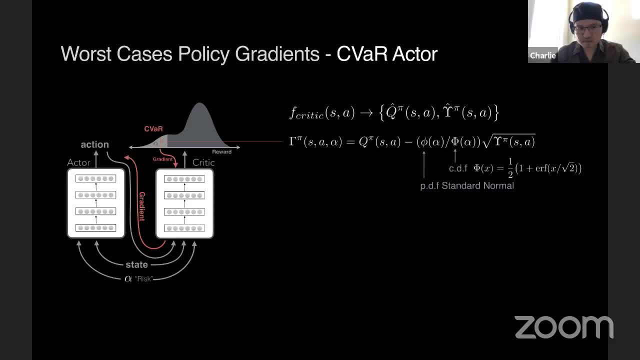 we can compute this gamma pi value And this is the conditional value of risk, And we can compute it in closed form because this relates to the CDF and PDF, the standard normal distribution. So it's really quick to compute And this is highlighted in red. And so what we're going to do is we're going to take the 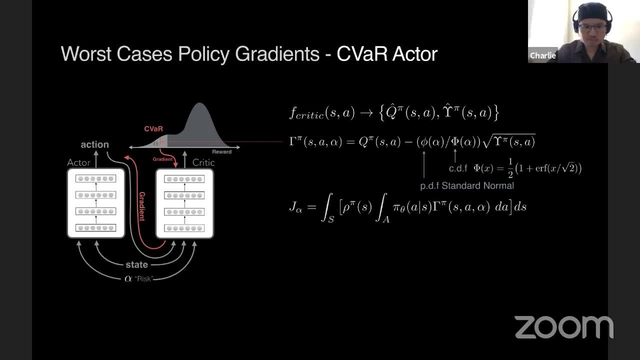 conditional value of risk up to gamma pi, and we're going to back propagate it through the, Through our critic, and then also through the Through our actor. Our overall objective- this is the standard policy gradient objective- is denoted as integral over the states and then integral over the different actions weighted by this. 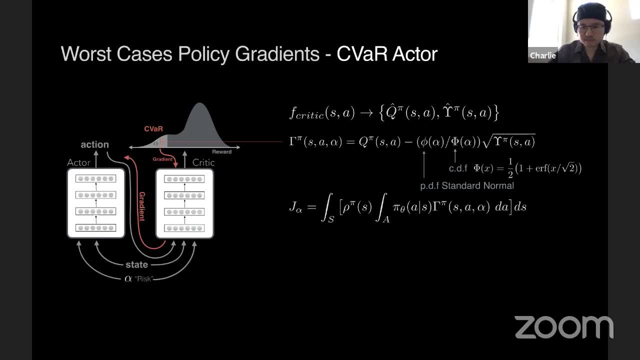 CVAR, conditional value risk, epsilon pi term that substitutes essentially our Q function And we have a theorem in the paper that shows that, using sort of the similar approaches to policy gradient theorem, we can turn this into a, The gradient to a gradient expectation. 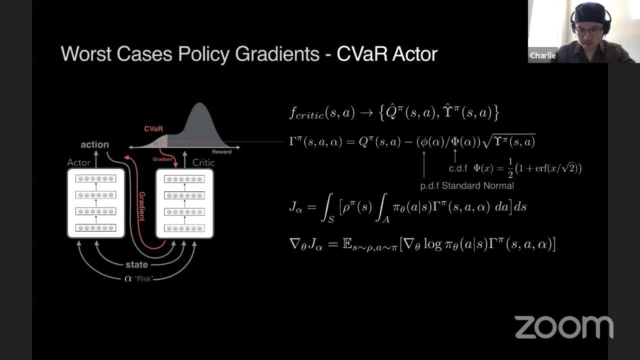 and the gradient of the log of the policy, again weighted by this gamma value. So the one interesting thing here that we have that falls essentially out of the fact that our gamma pi is conditioned by the alpha, is we have this alpha knob right, So you can think of this. 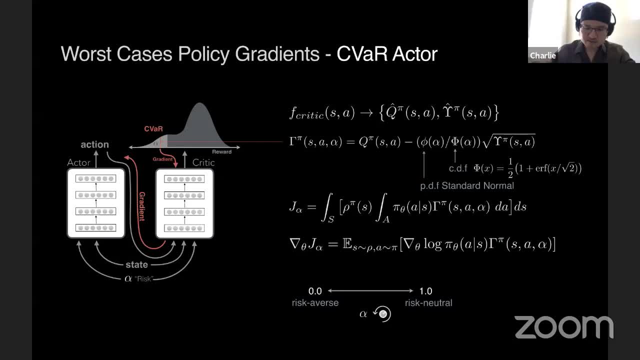 as a scalar that goes from zero to one, And if it's pro to zero, the policy itself will become very risk-averse. if alpha goes to one, this becomes risk neutral And essentially would basically fall into a standard sort of active critic DDPG kind of style. 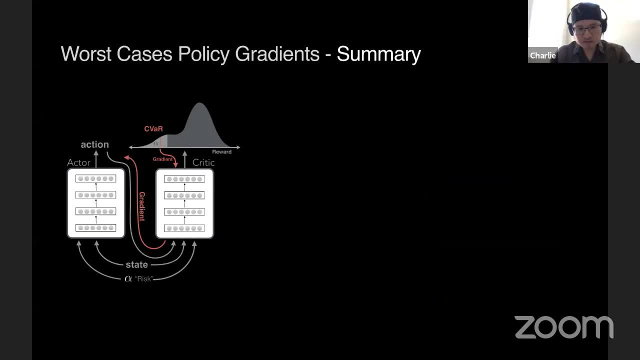 And this really gives us a sort of a family of policies that will be risk-aware, And so that's kind of interesting. So in the end, In In summary, worst case policy gradient we're proposing is the combination of distribution of RL conditional value at risk. 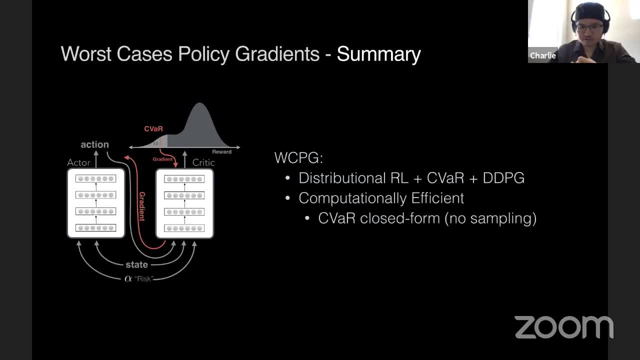 and then the standard deep deterministic policy gradients. It's computationally efficient because we don't have to unlike others or papers. there's a few other papers related to optimizing for CVAR. A lot of some of them require sampling. In this case we don't. we have a closed form computation. 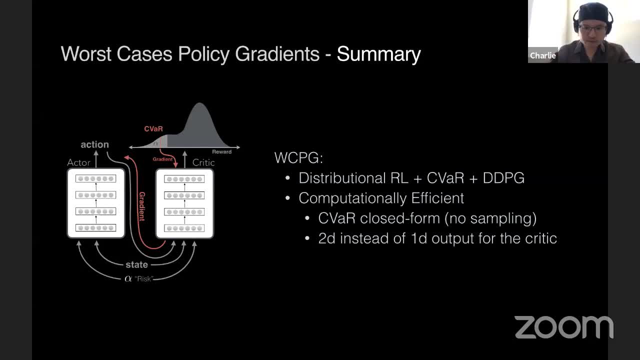 And at a very high level, since instead of having a 1D output for a critic, we have a two-dimensional output. And then there's tensions where you can have a mixture of Gaussians or a mixture of other kind of distributions as well. 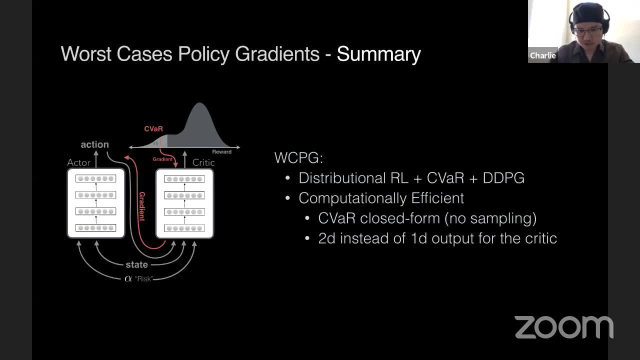 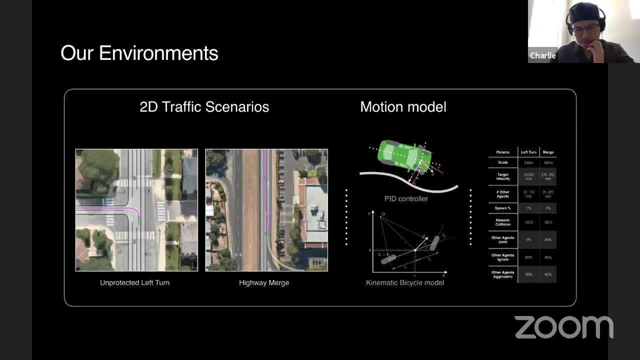 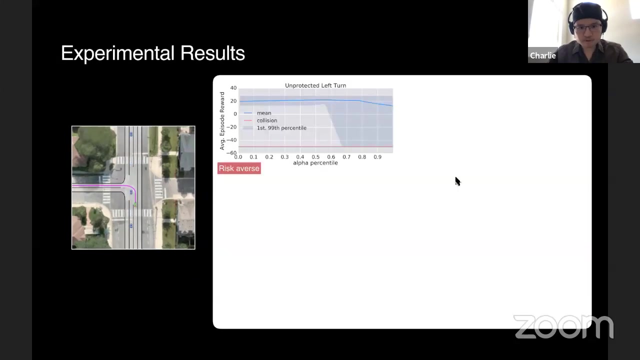 But right now, with the simplest case, essentially just one more dimension for your critic, And again this leads to a family of risks into the policies. Okay, so what happens here is a similar environment. we put experiments on that showed earlier, And I want to show you some experimental results. 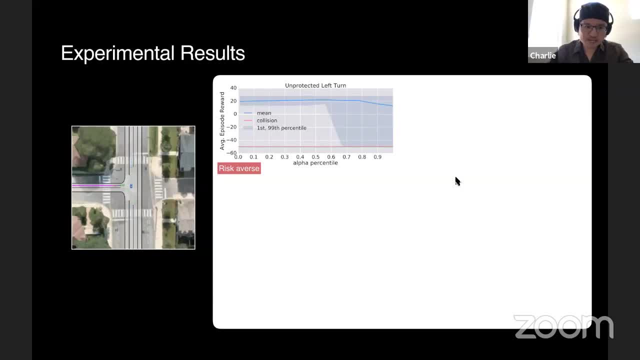 So when you're looking at this plot, it's basically a plot of the average episodic test reward as a function of the alpha that I showed earlier right. So as we turn alpha this way, it becomes slower, lower. the variance decreases, as expected. 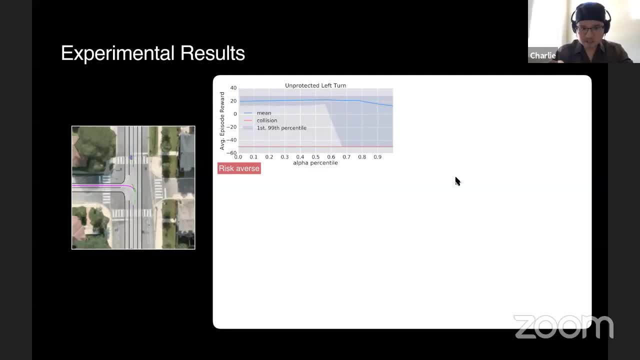 and we don't have any collision, So collision would in this case, give a negative 50 reward. As you see, it's basically limited collisions, which makes sense. What also that leads to is that the average time it takes to finish this episode. 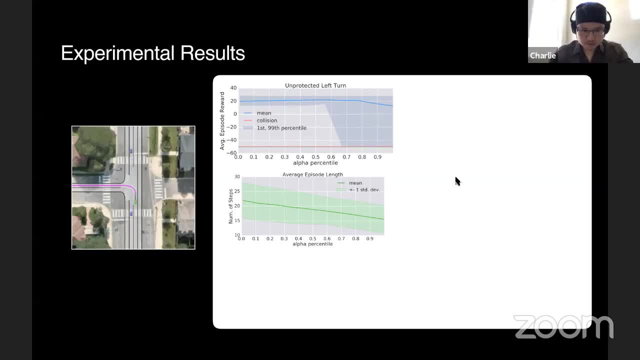 of making an unplugged left turn would be increased, because qualitatively, it just wastes longer wastes for a bigger gap before it makes the maneuver, which makes sense as well. And then, lastly, the estimate uncertainty also decreases as a smaller alpha. 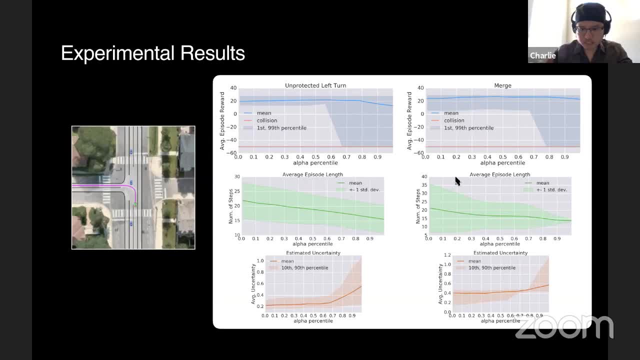 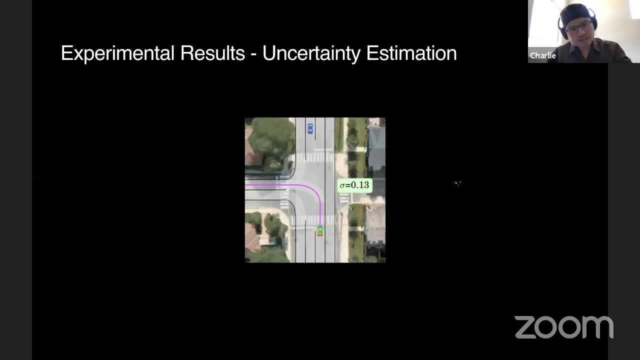 So that's how expected For the merge scenario. it's similar kind of trends, which makes all sense as well. Okay, so one of the interesting things that, because our critic can now estimate uncertainty over the future discounted returns we can actually look at in real life. 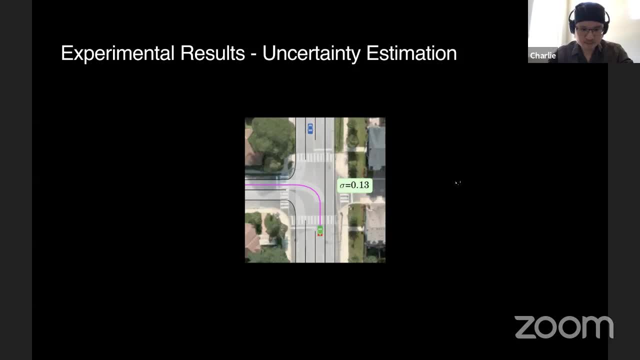 how real time? what does the estimate say, right? So in this example, as we approach, as the green car approaches the intersection, you see that the sigma, which is the estimated uncertainty, rises and it reaches a peak when we're crossing. 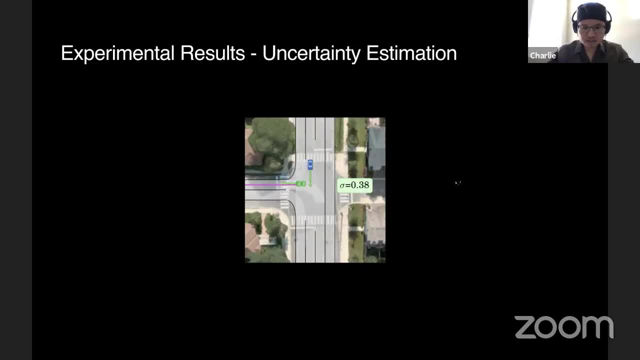 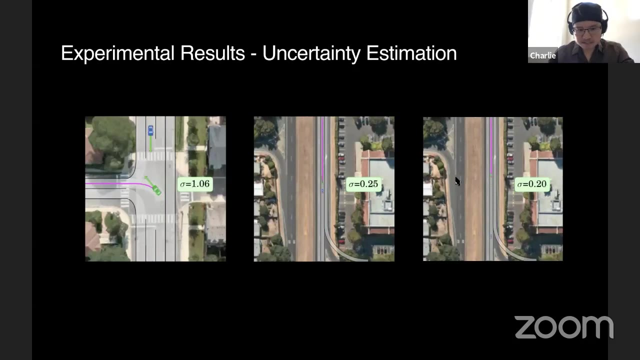 onto your uncommon vehicle And it quickly it'll decrease as we sort of approaches, approaches, the finishes, the maneuver, which also makes sense. Here are more examples of, under other situations, how this does. So again, this all makes sense. 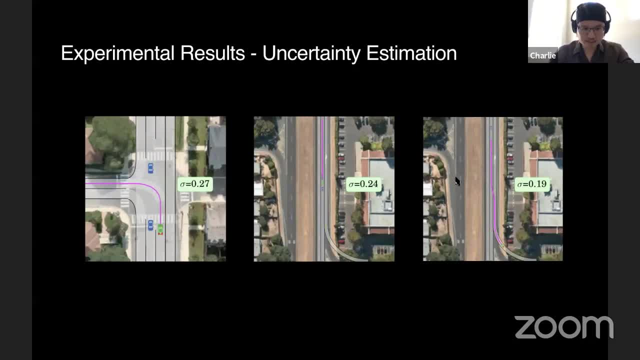 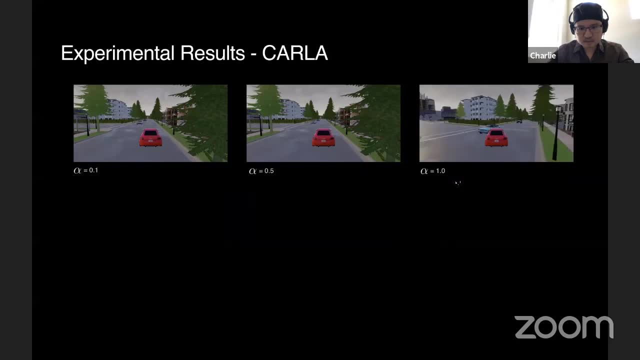 This is exactly what we intended- the framework to learn- And you know that's that. We also have tried similar experiments in CARLA, similar kinds of left turn scenario and a merge scenario. And you know we've tried similar experiments in CARLA, similar kinds of left turn scenario and a merge scenario. And you know that's that. 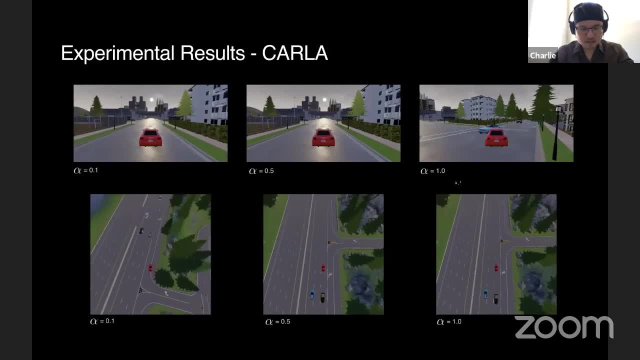 In all these cases, you notice that when alpha is smaller, it takes longer to finish and deliver. It's more cautious, more conservative. In fact, in this case there's actually a collision simulation that actually happened with alpha. It's got to be one. 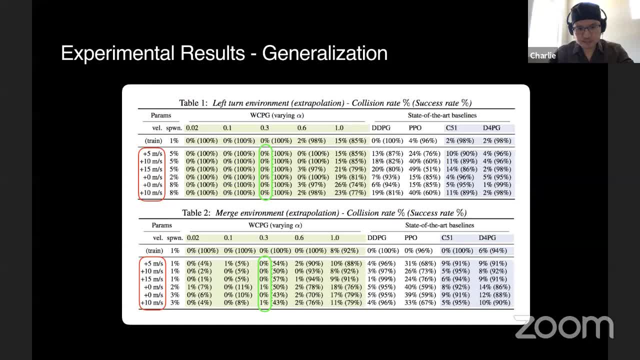 Quantitatively. what you're looking at here is generalization performance. okay, So we're taking at: the top table is the merge, sorry, the left turn- And then the bottom one is the merge, And what we're doing here is we're. 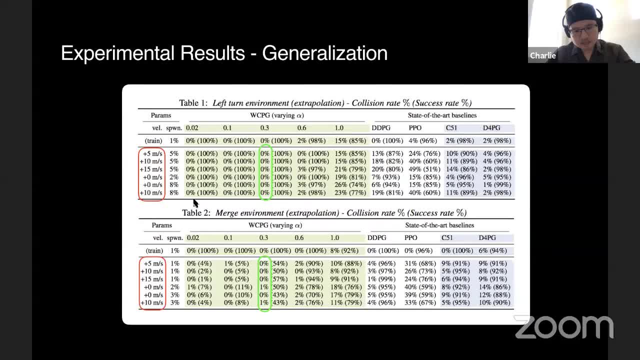 for the testing environments. we're going to actually add more velocity to these different the speed of the other agents. We're going to spawn them more. That creates more vehicles and roads. So basically, test out generalization, So these high parameters of the environments. 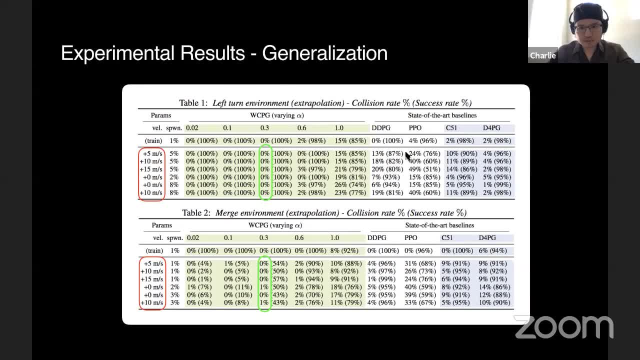 have not been used in training And what we see is that, with standard approaches like DDPG and proximal policy, gradients, optimization and even the distribution of RL1, like C51 and D4PG, it's just, it's really, really hard. 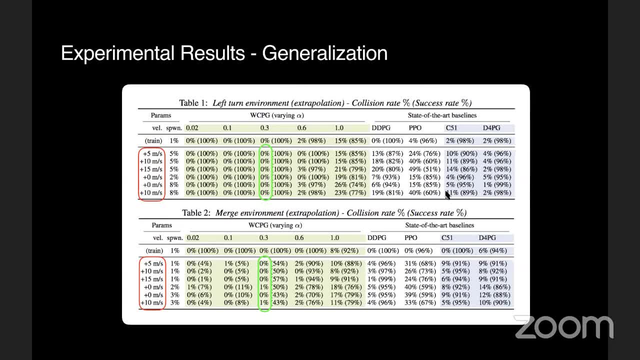 to get the collision rates to zero. It's just because they're not. they're not optimized for risk aware, risk sensitive criterion. But with worst case policy gradients we are able to push it close to zero even though there's still some collisions. 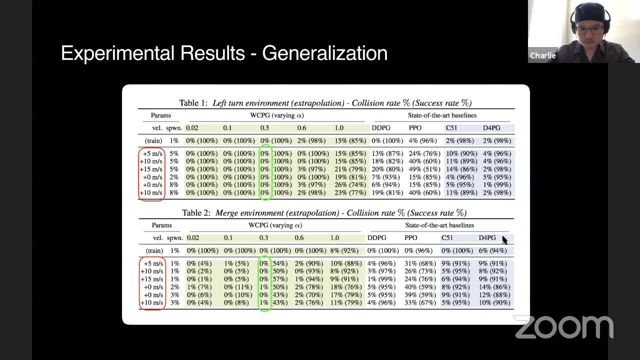 when we set alpha to be small. So this is, this is and this is really where, in order for this to be on the road, for this to go on in real life, we really need to make sure that the collision is definitely zero. 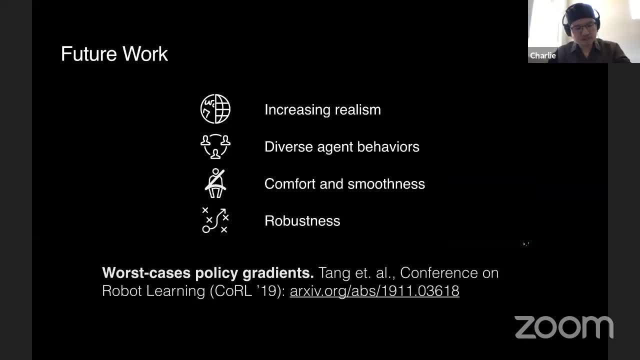 So again, this is in summary. this is: I think this is interesting work, but it's far from finished. We really need to ensure robustness, not just only in simulation, but in all sorts of different environments and potentially one day, to real world. 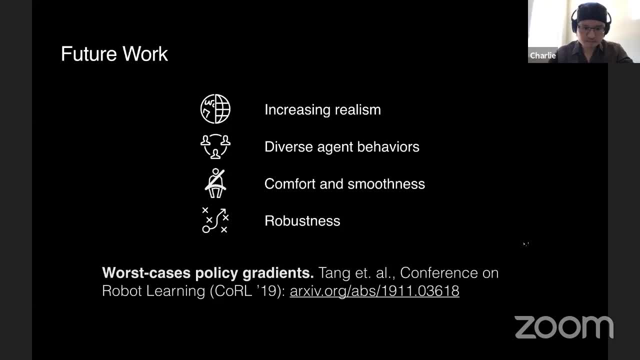 We need to increase the realism. We need to increase the realism of the simulation, And then we need to make also make sure that the policy is comfortable and also the trajectory is smooth. So for new mission, this paper is also on archive. 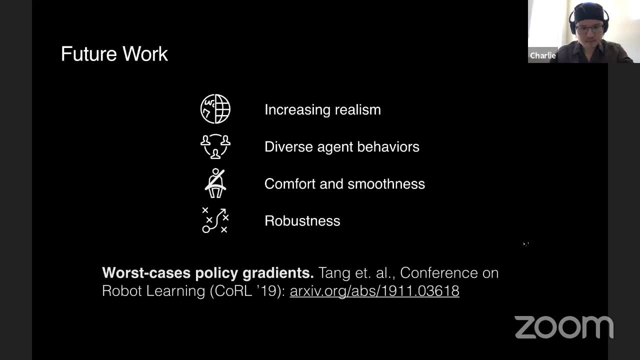 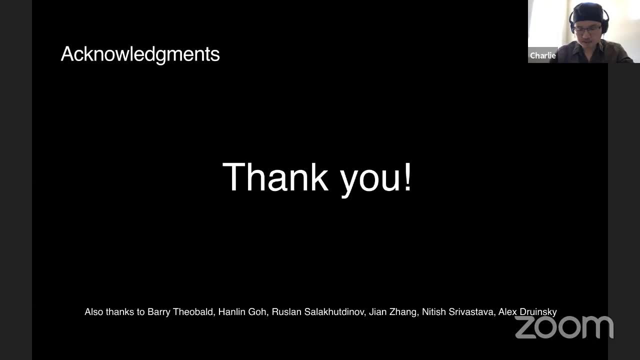 it's published in Coral last year. So with that, thank you very much. You know, I think people are converging on these kind of very interesting tech techniques with the RL, So yeah, So thank you And thanks to my collaborators. 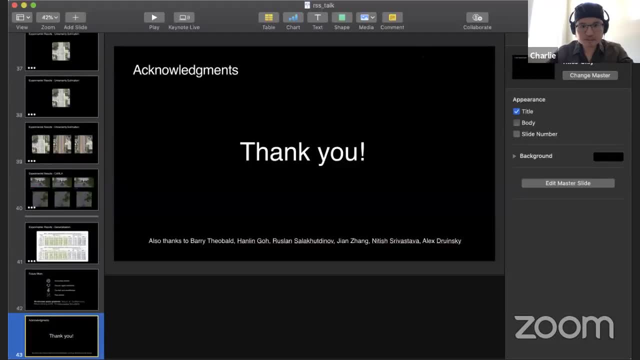 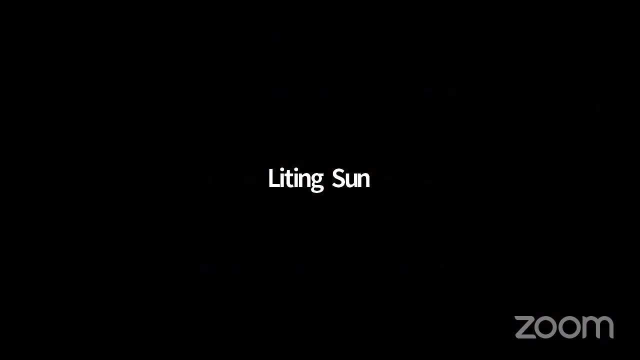 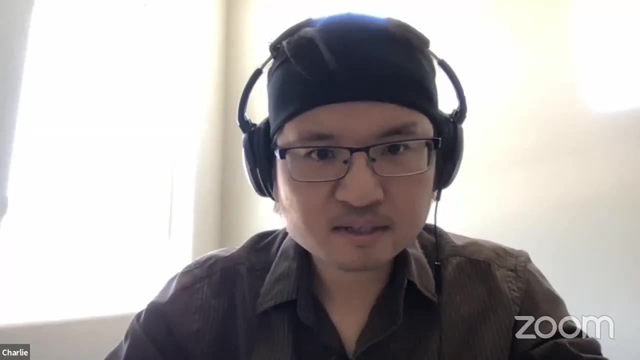 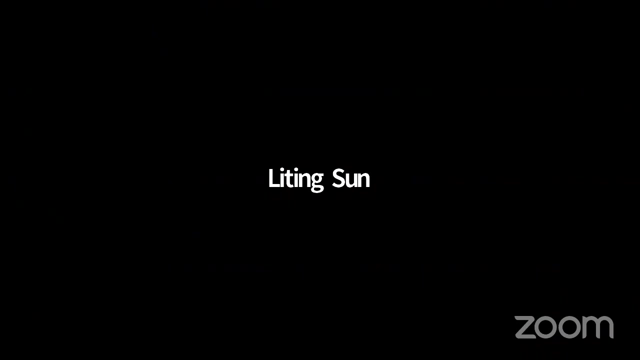 And I'm happy to take some questions. Okay, great, I think we got several questions. Okay, So one is. so the first question is: are there any traffic? Are there any other traffic-participated program to make room when there is a right turning signal? 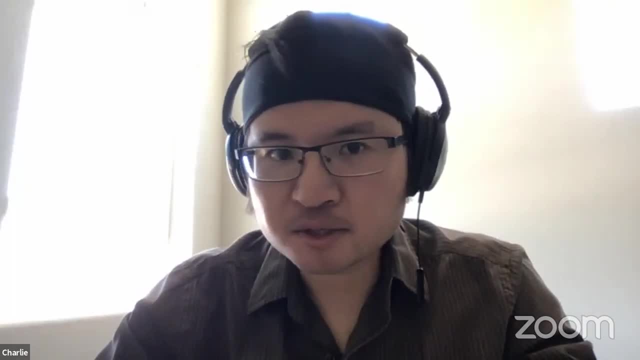 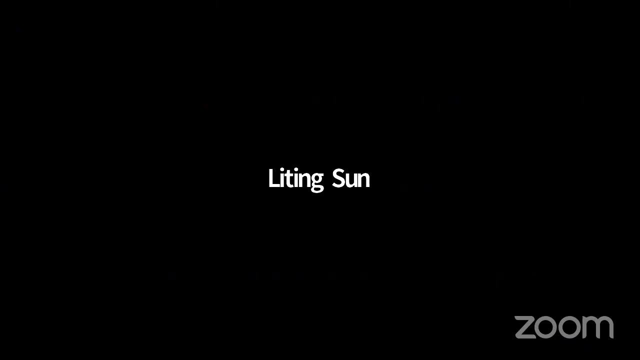 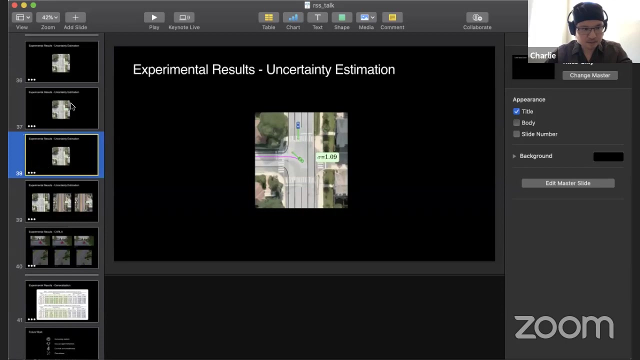 That's a really good question, Zao-Tang. So see here, let me share my screen again. So, in order to have stochasticity, this is a really good question. in the environment, in this case, what happens is that oncoming vehicle. 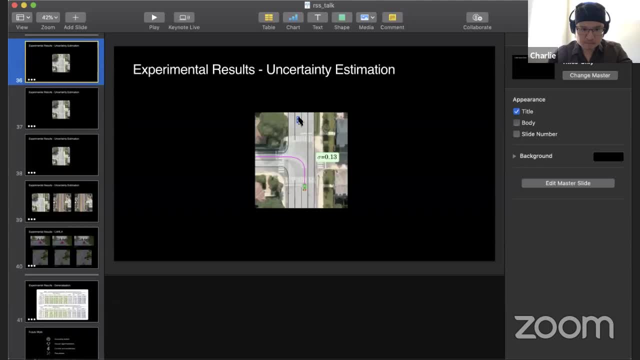 would have a randomly samples from one of three types of modes. So one is, you know, be aggressive and don't yield. The second mode is actually yielding, So we'll break if it sees the green vehicle is trying to make a left turn. 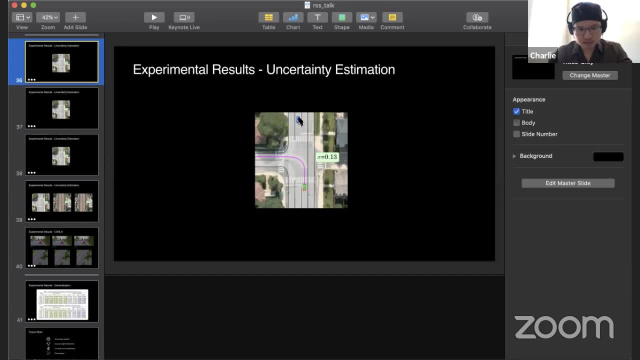 And the third mode is simply ignore it, ignore the vehicle. So, and because of these three modes, that it samples randomly, this really leads to more. in my opinion, a more realistic simulation of what the actual environment like in the real world happens are like: 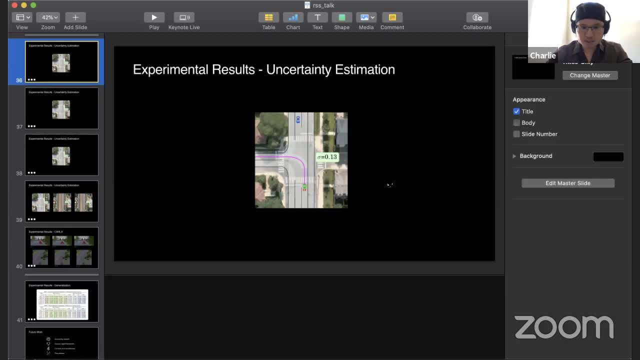 And so, and that leads to uncertainty. So, to answer your question, it's randomly, stochastically, picking one of these three modes. Okay, So the second question is that, during the self-play, is it possible for successive generations to keep switching between passive and aggressive behaviors? 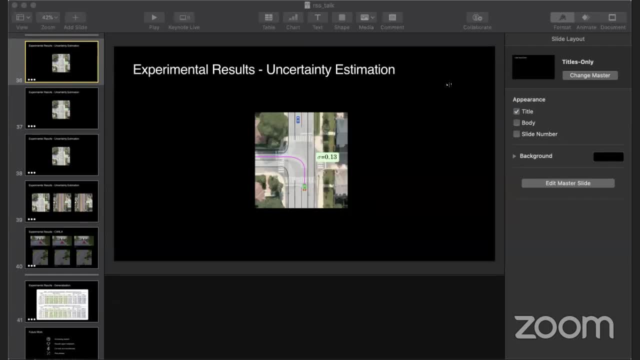 As they realize, they think: oh, oh, oh, oh, oh, And that they can either take advantage of or take refute from previous generations. Okay so, yes, So so what happens is that, in self-play, there's many ways to do this. 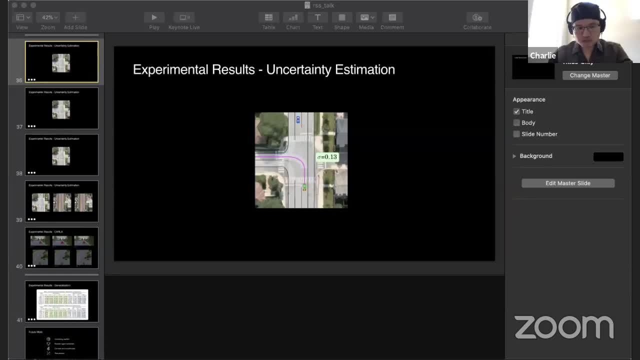 And typically you would keep a population of different agents. So- and by population I mean the checkpoint, the weights, RO weights. So what we can do is so I don't actually do this now, but it's not a problem. 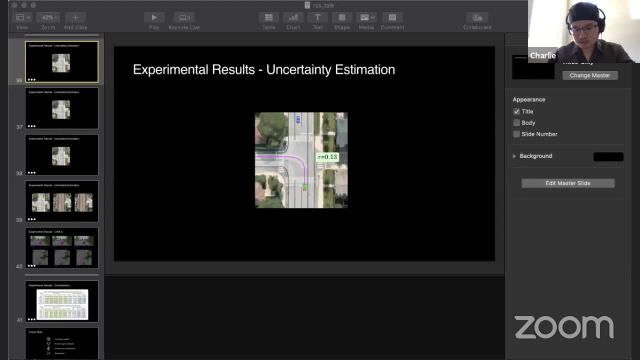 as an extension. what you can do is you can actually cluster these policies according to the kind of behaviors And then you can make sure that you try to get as diverse sort of set of agent policies as possible during training. So in this case it doesn't, you know, in this case, 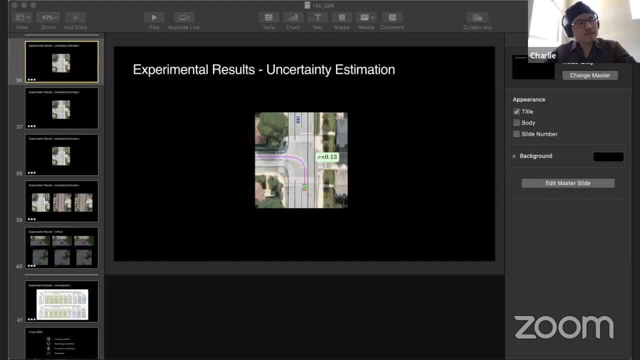 this is it doesn't it, doesn't it sort of converge? And so I don't have a definitive sort of thought on how does it they're converged or does the policy keep, sort of? I guess this is the question you're asking, right? 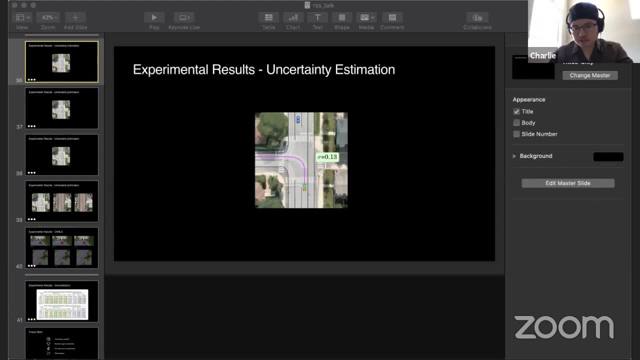 Because it goes from oscillate, does not converge. So I think that's really good future work to examine what happened as it converged to Nash, for example. but this is a general sum game, So I think it's, I think we can take inspiration also. 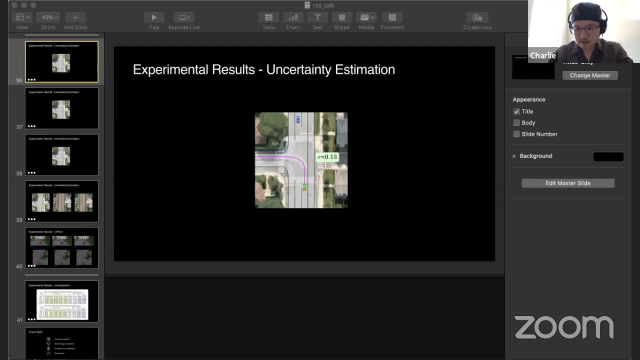 from alpha star kind of work, where it's just you just have a set of diverse policies that are there And then so they don't necessarily converge because these different policies are trained with different training distribution. Okay, and then we got a third question. 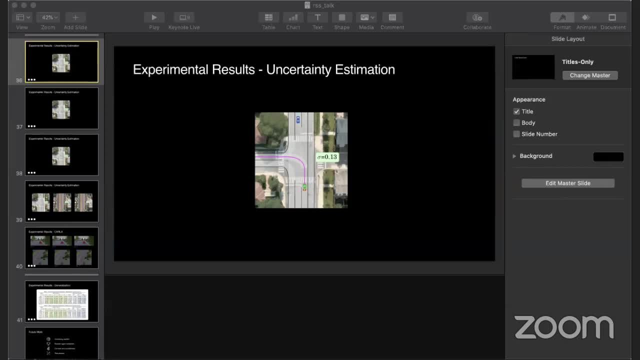 is that. does the policy from Southplay provide any information into which aspect of the presentation prediction are important? Yeah, that's a good question. So it's, I think it's just it's you might be able to just deconstruct. 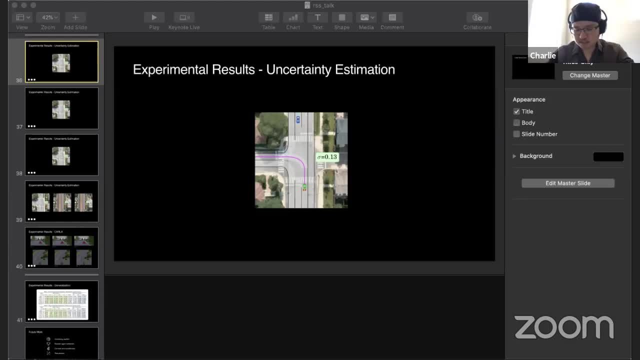 or introspect as to which aspect of predictions is important, but it's really hard to do, And so, and the reason is because the policy that's being learned is simply gives action next time step action, and it's training the model-free kind of sense. 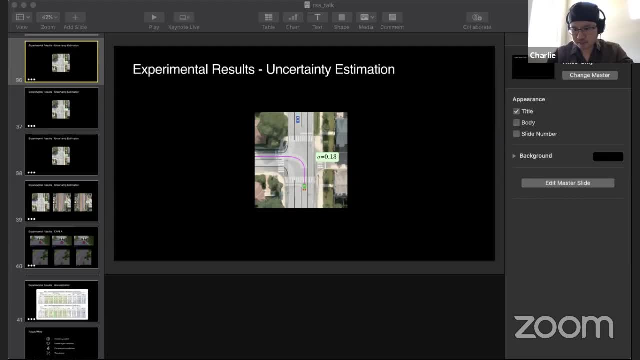 So- and I think there's another question here- I see in the chat model-based RL. So that's actually also a good question. So if you do model-based RL kind of simulation, then potentially the longer horizon plan that you come up with might have better correlation. 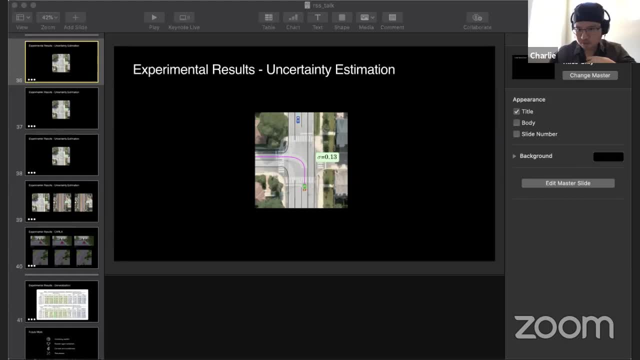 or maybe tell you which aspect of prediction is important, But right now it's. it's hard to really see which aspect of prediction, just because they operate very differently With predictions. again, it has to be interactive predictions, right, It has to. you have to predict. 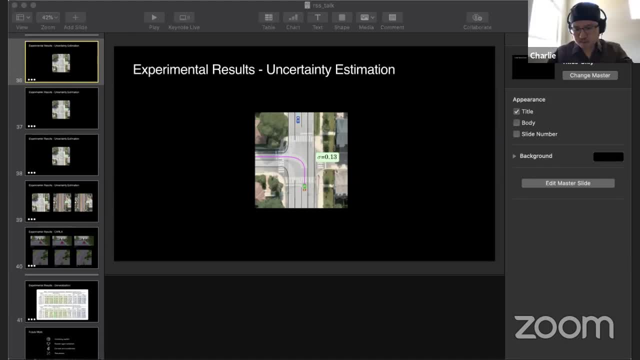 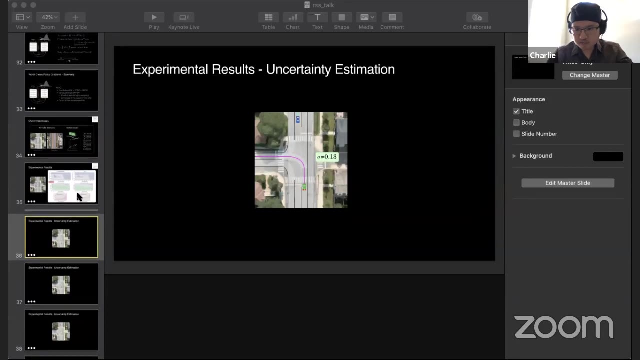 how others will react to your actions. So so I think it's interesting, but it's not. it's not really apparent to me what aspect of predictions is important. Now, we do have you know in, we do have attention-based encodings. 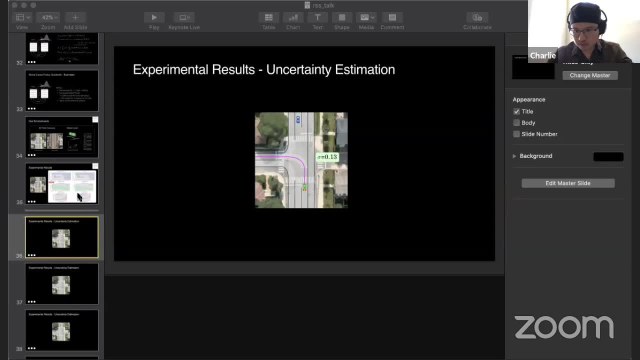 and what that does is that tells you which agents are relevant, because if you use attention, you can actually tell that as part of the encoding process, which other agents or cars on the road is not really relevant for for my predictions or my actions. 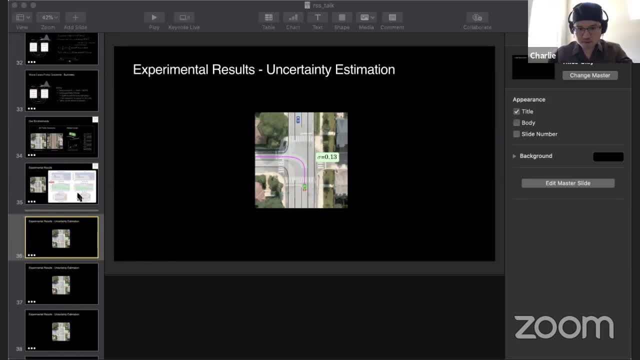 So, and that's what you expect in terms of the distance to the ego or self-driving car really is inversely proportional to how important they are. Okay, I think, following that question also, there's one more, like one more question. 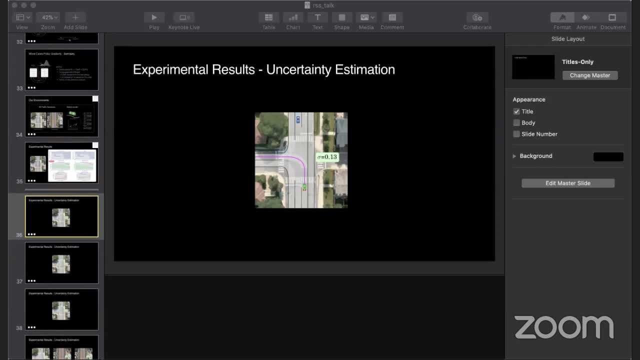 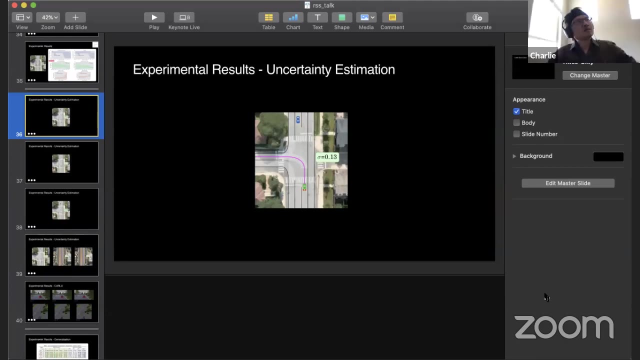 Do you have any insights into how the learned agents are predicting the world, or are they purely reactive? So yes, So right now, with the self-play, it's it's purely reactive And so. but the thing is, I'm always surprised by how interesting behaviors 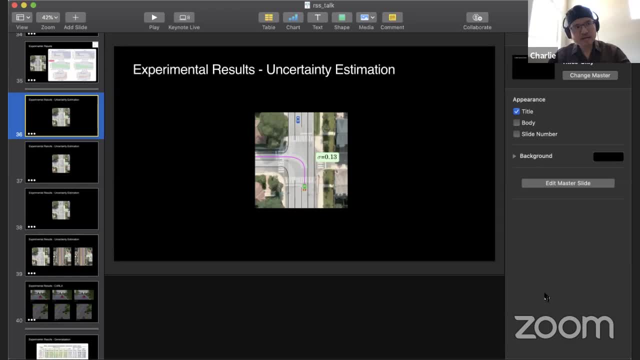 can learn just from a reactive policy And it has to really has to do with distillation of the you know examples into a reactive policy. So I think I think will forward, I think maybe one of the few examples that you see, 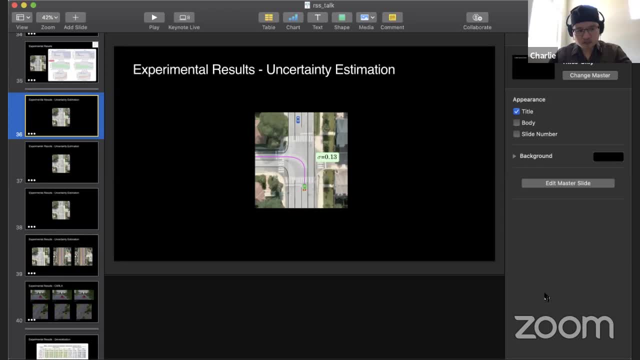 from the collisions could be helped by using a model based sort of policy. So, with a model based policy, if you think about it, it's basically saying that, if my assumption is right, right, if I'm assuming that the vehicle in front of me- 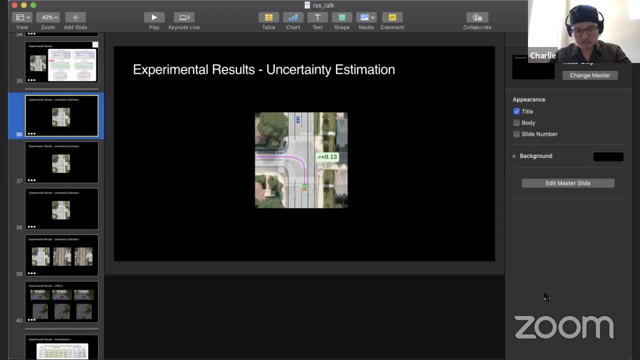 will have constant deceleration or constant velocity, both model-based like MPC or ILQR. you're guaranteed to not to collide right If it's within the reason of my deceleration of my car. So that's what you get. 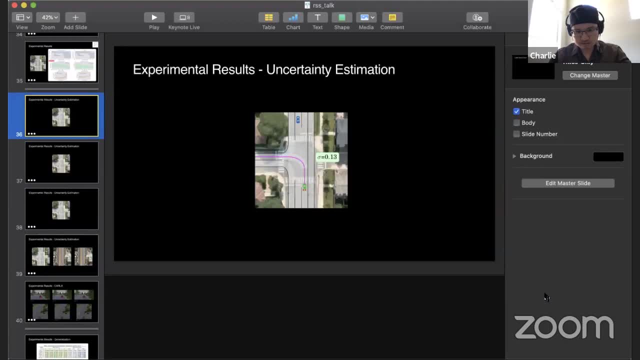 So that's the advantage of guaranteeing non-collision in these kinds of scenarios. The disadvantage is that if you're in a dense merge scenario, right If you wanna squeeze into a closed gap, right If you wanna induce open a gap. 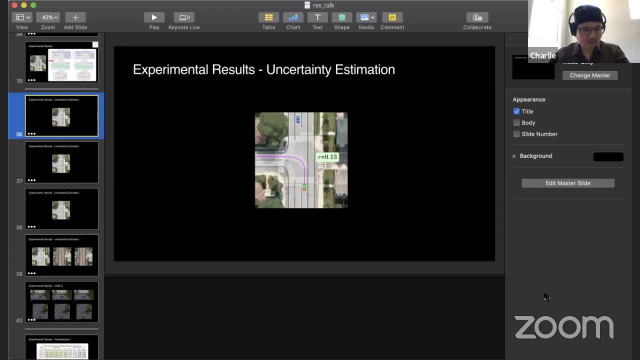 then model-based is not gonna help you that much, because you have to be able to, because your assumption of constant velocity, constant acceleration, constant steering just goes out the window, And I think that's where model-free comes in. So I think, as a human driver, 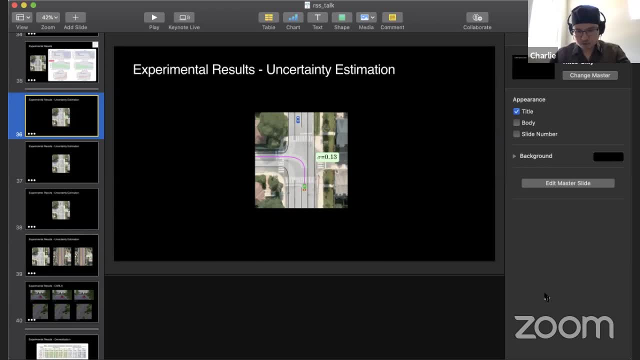 I suspect we have a mix of both things. If we're just cruising on a highway or a freeway, we're probably in the model-free kind of mode. But now, if we're trying to make a sharp turn onto a busy major road- and at least for me, I see myself. 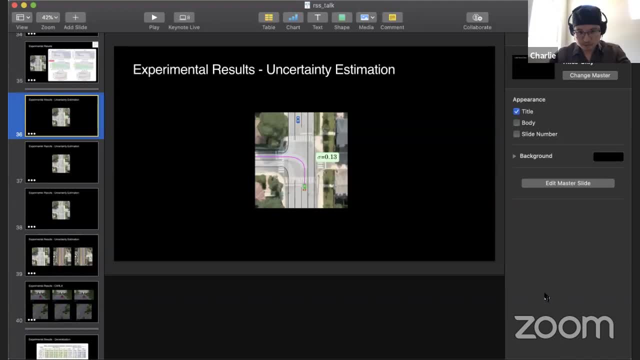 trying to intend to do that. I can anticipate or visualize how in the future, and that will be considered to be model-based planning. So I think the question is: how do you combine the two to achieve more robustness? I think that's a. to me, that's a good future direction. 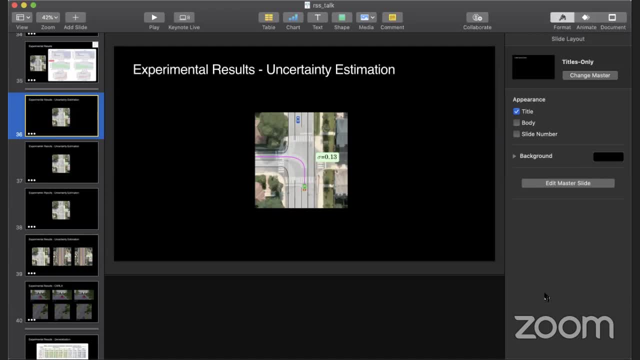 Great, thank you, Charlie. So I think, due to the time limit, we have to go. Do you mind like replying in the chat? Sure, absolutely, absolutely, Thank you. thank you guys again. Thanks so much, And then you can unstop share your screen. 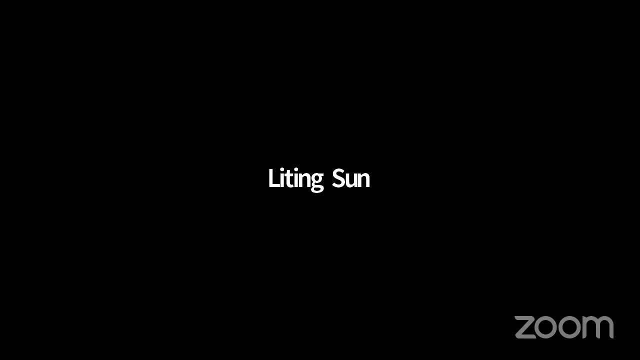 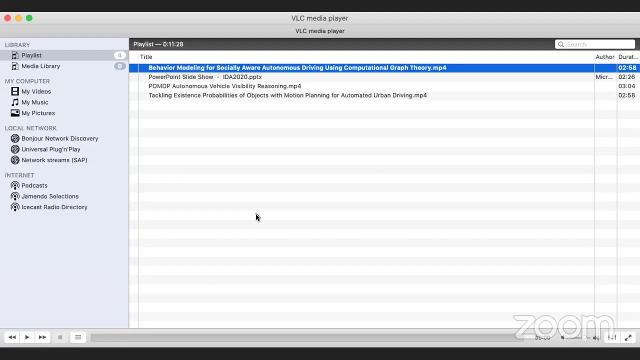 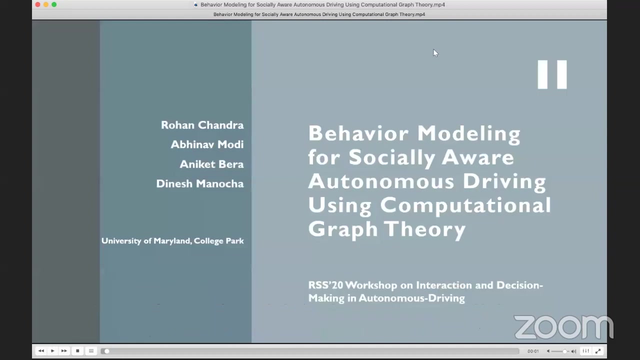 So next. so next we will go to the contribute talks. I will share my screen and then play the prerecorded videos, So it's going to be a little bit difficult. I think we're looking at the questions. I think they're coming in. 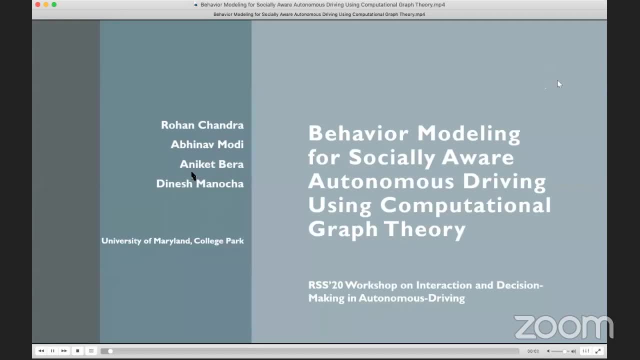 I'm just going to go through them one by one And then I'll let you talk about them. I'm Rohan Chandra and I'll be talking. Yeah, the first one is from Rohan. His topic is behavior modeling for social aware, at times driving. using computational graphs and algorithms, And I think it's really interesting. Yeah, And I think he's reading the question And I think it's really interesting And I think he's reading the question And I think he's reading the question. 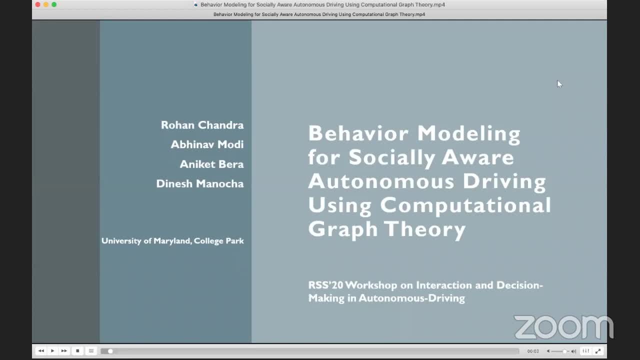 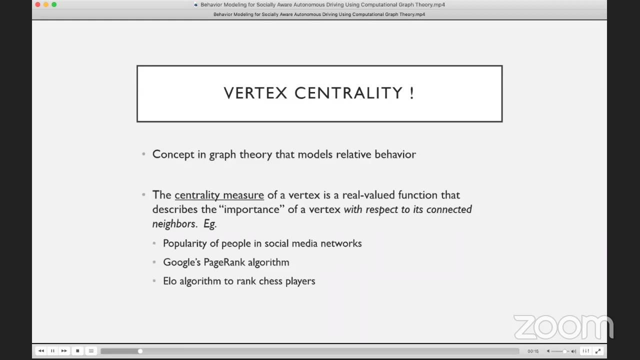 And I think he's reading the question: graph theory Talking about behavior modeling for socially aware autonomous driving using computational graph theory. The key idea is to use the concept of vertex centrality, which is fundamental in graph theory that models relative behavior between vertices. 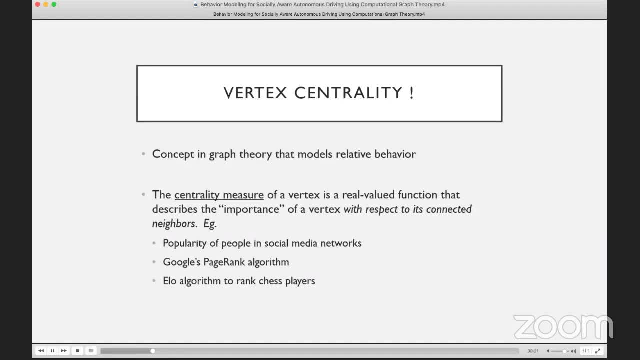 The vertex. centrality is a real-life function that describes the importance of a vertex with respect to its connected neighbors. It has been used previously in several important algorithms, such as Google's PageRank algorithm, as well as the Edo algorithm, to rank just dates. In our application, we model traffic. 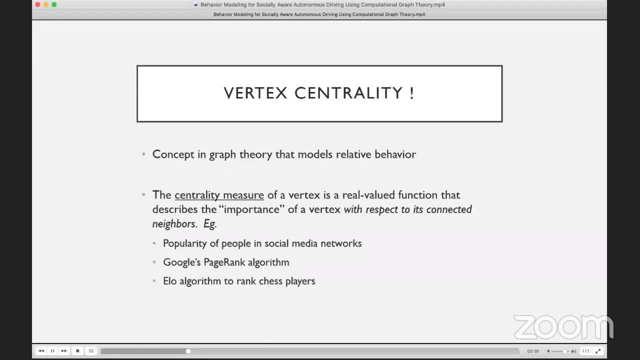 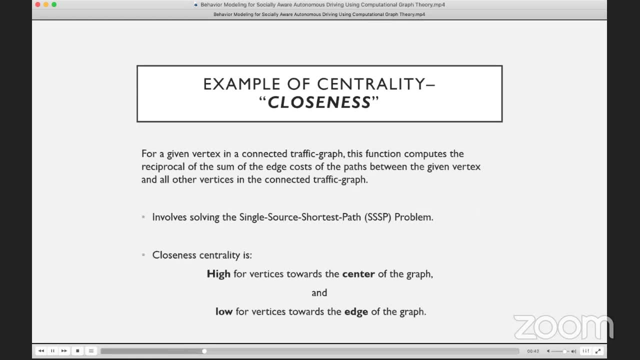 through a graph and apply vertex centrality to measure the behaviors of the vehicles which represent the vertices of the graph. An example of the centrality is the closure centrality, which effectively measures how central a vertex is placed within a graph. In our application, we use this closed centrality to model certain behaviors like 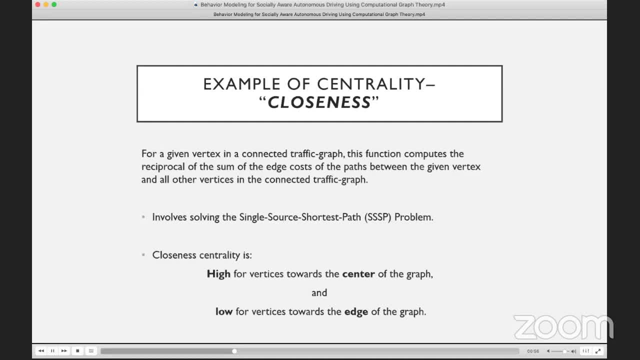 overtaking lane changing and zigzagging through traffic by noting the closest centrality of these vehicles, which would be high towards the center of the graph and low towards the edge of the graph. The main advantages of using centrality is that it is invariant to sense and noise. it is deterministic. 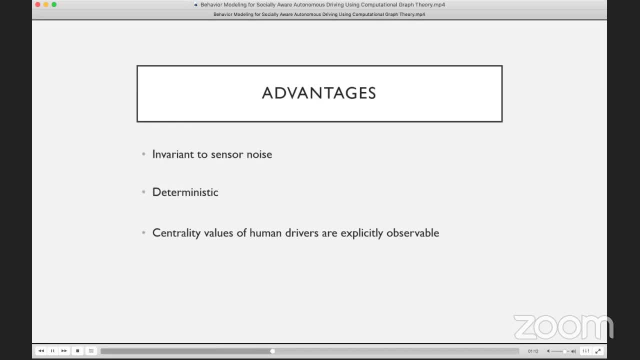 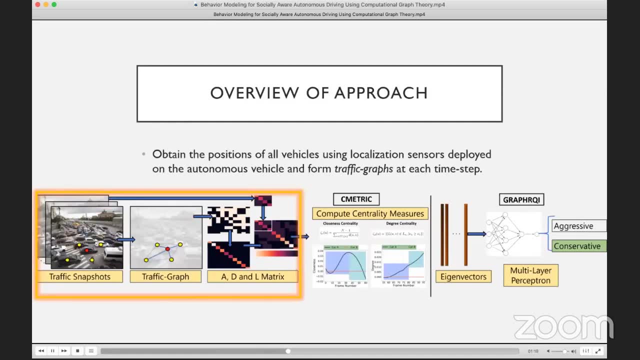 and that the centrality values of human drivers are explicitly observable. We begin by obtaining the positions of all the vehicles using sensors and form traffic graphs at every time step. We can then measure the closest degree as well as the eigenmeter centralities for every vehicle. We perform polynomial regression to generate. 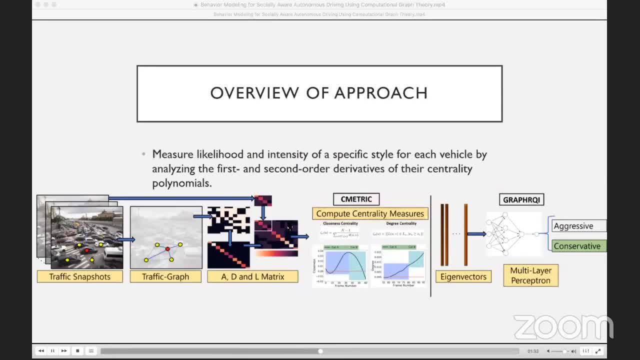 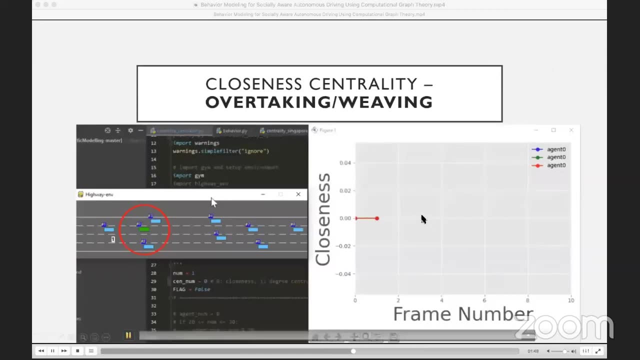 univariate polynomials of the centrality as functions of time. We can then measure the likelihood and intensity of several driving styles by analyzing the first and second order derivatives of the centrality polynomials. We now present some results. In the first video we model overtaking and weaving of the 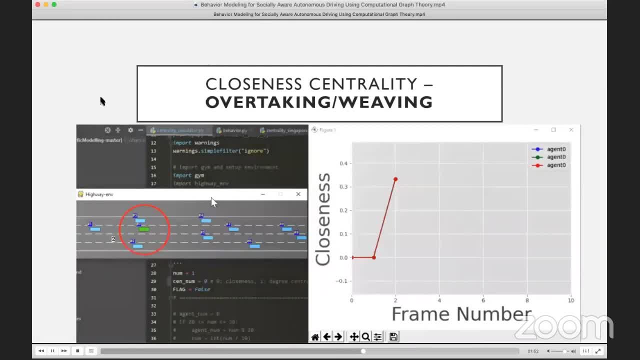 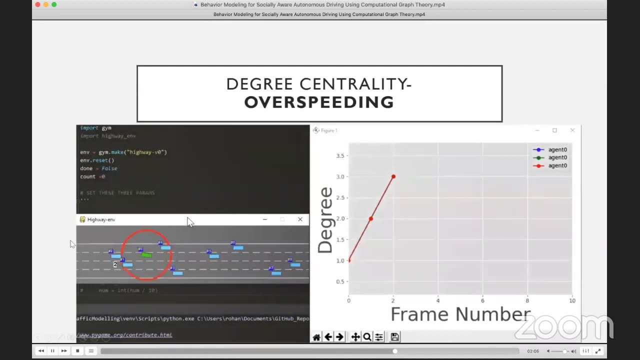 green vehicle by noting that the closed centrality is high when it is in the center of the road, but as it moves towards the side of the road, the closed centrality will reduce. We additionally model the overspeeding nature of this green vehicle. As it overspeeds through traffic, we note that the degree centrality 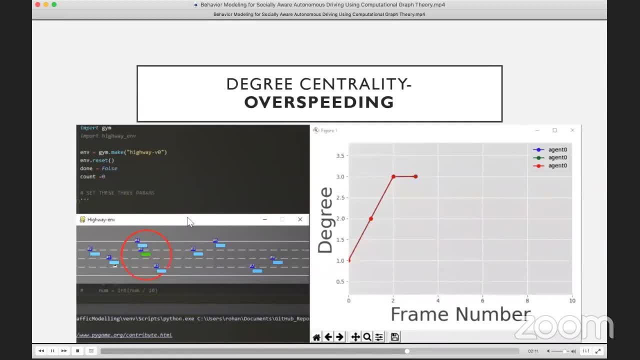 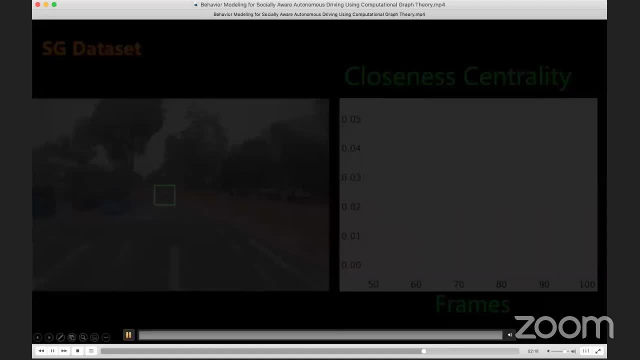 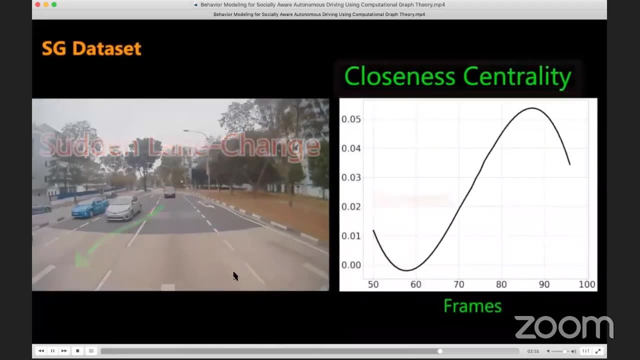 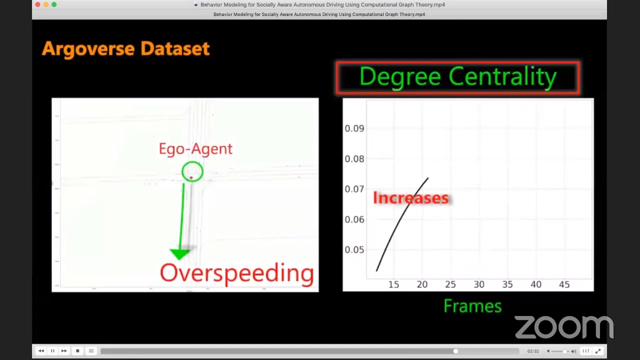 more dramatically increases. Finally, we show several real-world results on real-world traffic data sets. This is a list of the data that we have collected that we have used to test the driver's ability to run the scolding of the cars. The vehicle is awesome and how the car is set up is very interesting. 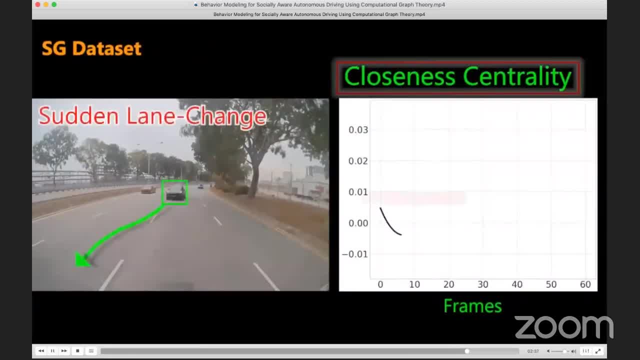 For example, we can measure the speed and speed of the driver's car, the speed of the car, the speed of the car, the speed of the car and the speed of the car in which the driver is driving. This is a list of the data we collected from the test. 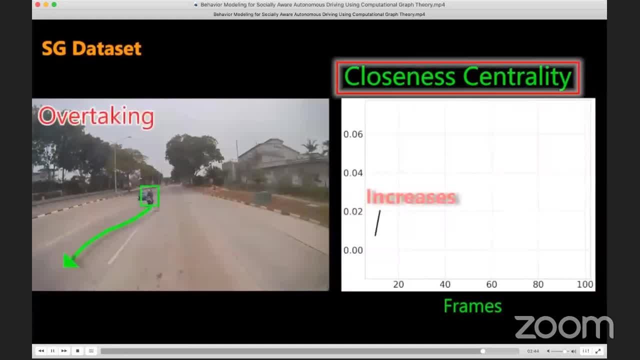 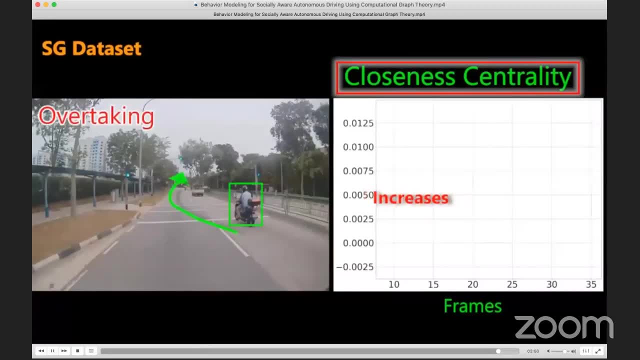 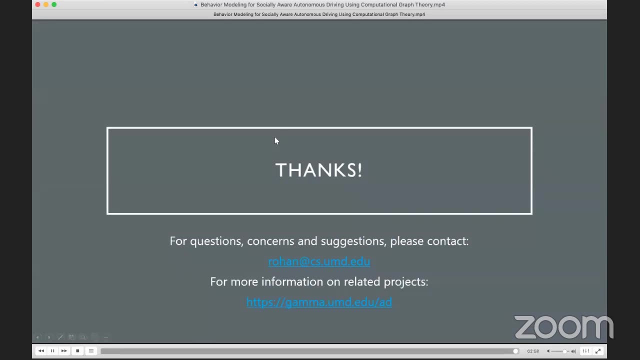 The score is on the bottom line for the target vehicle On the right front page. we can see some of the results of the test on the front page and the result from the test results on the side of the. please visit the following website: I'm Eric and I'm going to discuss. 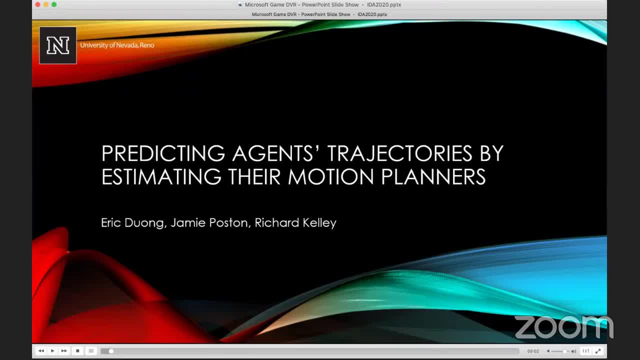 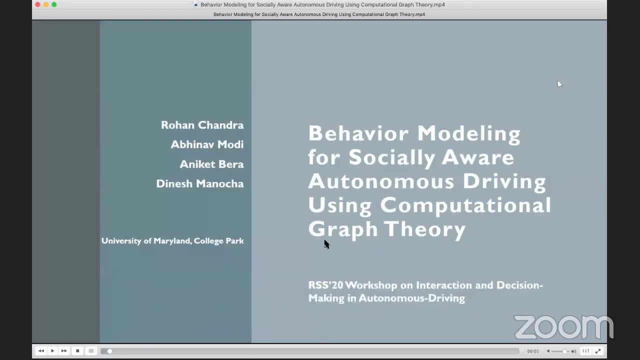 Okay, do you have questions for Rohan? I actually got one question, So I'm sorry I have to unmute. Hello, Rohan, are you here? Yeah, I'm here. Yeah, actually I have one question. 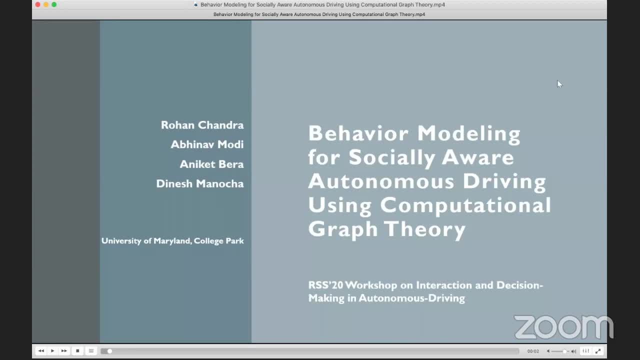 So when you are formulating the graph, so which agent are you considering, Like? for example, in this scenario, we have 10 agents. Are you considering all of them or you pick several of them? Do you consider? Yes, I consider all the agents. 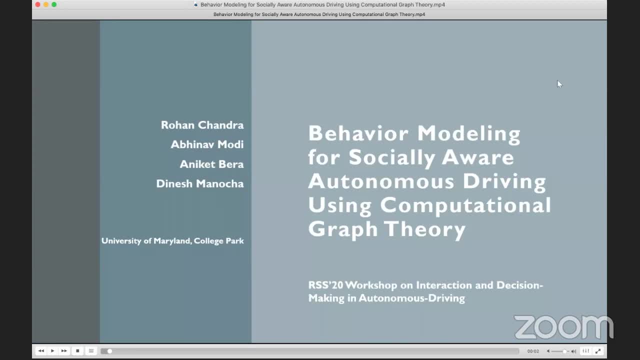 and form the traffic graph with all the agents And then, depending on which centrality you use, you can either choose to process all of those agents or you could choose a neighborhood and restrict the agents to that neighborhood. So, for example, for the closeness, centrality. 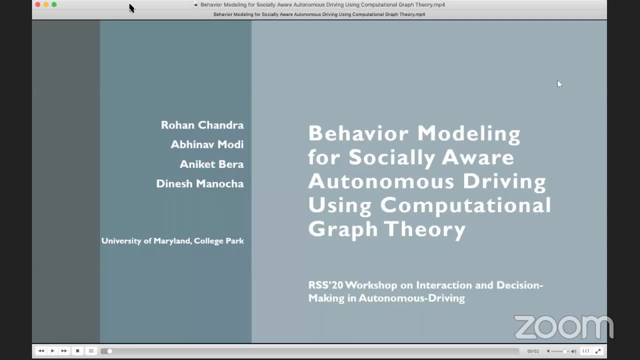 you need to consider all the agents in that particular traffic graph And if you're doing the degree, then you consider neighborhood. Okay, Cool, And we got one question from the audience. So Yeah, I see the question. So how is centrality? 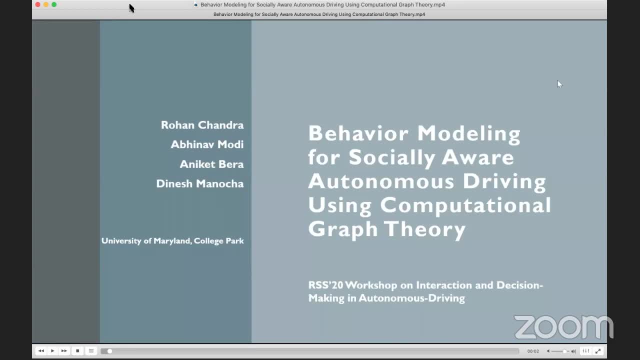 within a larger system, right? Yes, That is a good question, And that is the second half of the problem. The first problem is how you model and define driving behavior, because you know driving behavior is very There's no formal definition to behavior, you know. 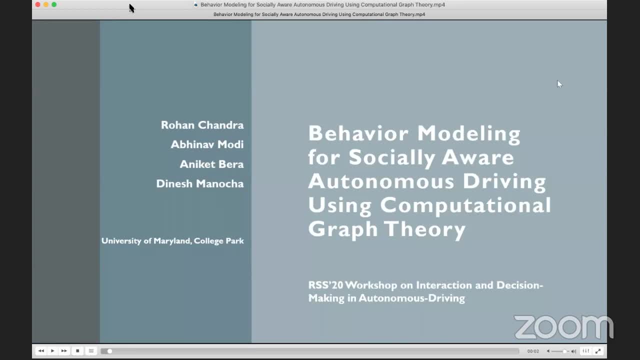 So the first part of our work is to actually model the behaviors. And now the second part of the problem which I'm working on is once you have predicted, once you have modeled or recognized or interpreted a behavior which could be a driving style such as over-speeding. 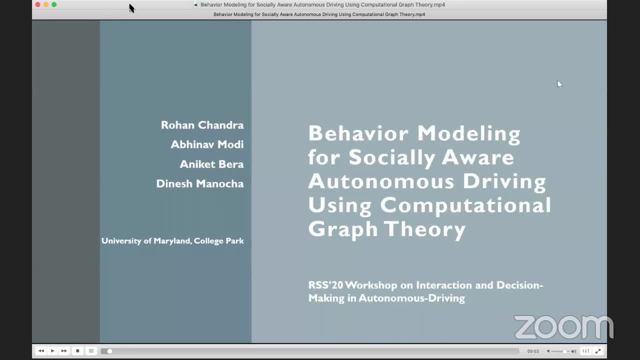 overtaking, zigzagging through traffic and so on. how do you use those definitions and interpretations to do planning and prediction? So yeah, that is the next work and I'm currently working on that And I'm So how I'm approaching that problem is. 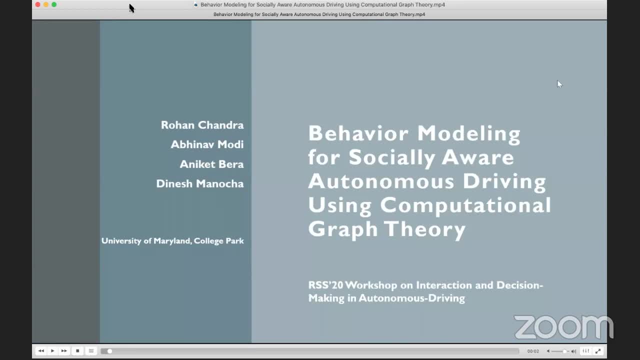 I'm essentially extending the mathematical part of the thing. So I'm essentially trying to reduce the decision-making part to solving the system of polynomial equations, And that's still a work in progress So I can't really expand on much over here. 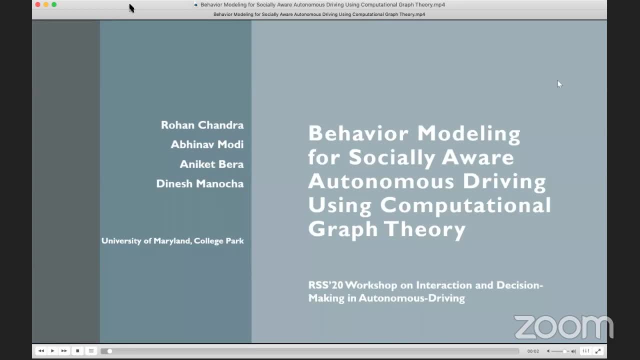 because I still haven't figured the complete things out, But I'm planning to to work on this more and I'll keep everything I want updated as things move on later on. Okay, cool, Thank you very much. So we will move to the next country of talks. 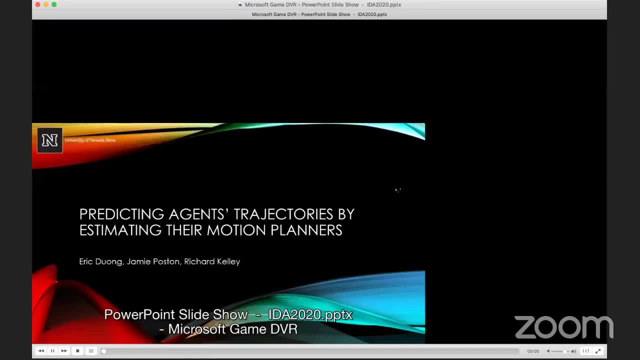 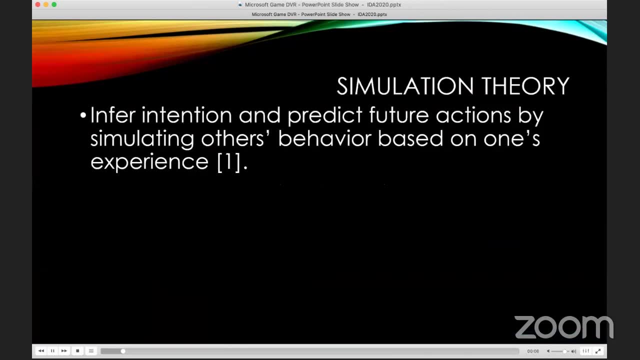 So that's from Eric Dong. Hi everyone, I'm Eric. I'm going to discuss about predicting agent trajectories and estimating their motion patterns. Our paper is inspired by the simulation theory, which specifies that a person infers intention and predicts future action of other people. 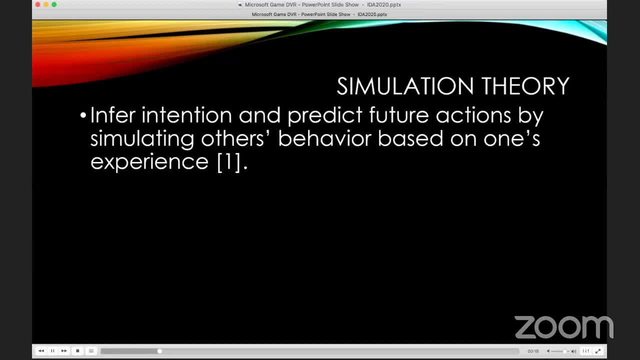 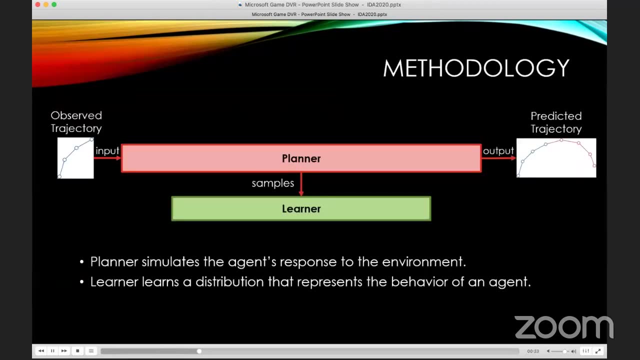 by simulating their behavior based on his or her own experience. Based on this idea, our method predicts an agent's trajectory by training a motion planner to simulate the behavior and response of an agent to the environment. We have a planner that takes an observed trajectory as input. 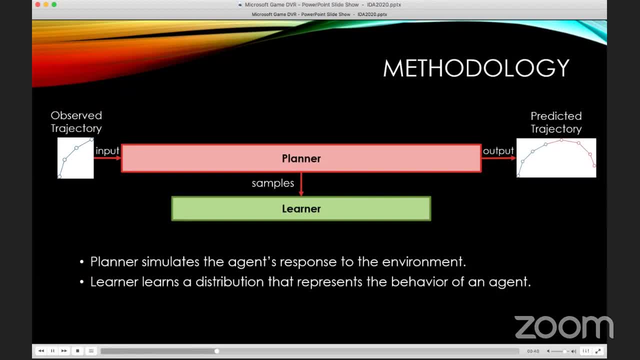 and predicts a future trajectory. as output, This planner simulates the agent's response to the environment by sampling from a learner that models the agent's behavior. The planner can be any motion-planning algorithm and the learner can be any model that represents the behavior of the agent. 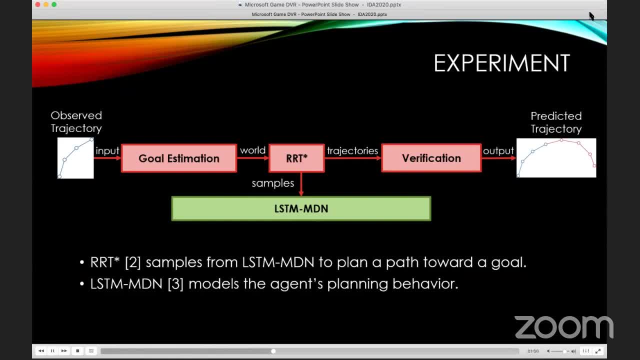 To test our method, we used a rapidly-exploring ManumTreeStar algorithm to simulate the agent's planning behavior. We have RT-star samples of the OSM-MDN model, which is short- or long-short-term memory mixture density network that represent the agent's planning behavior. 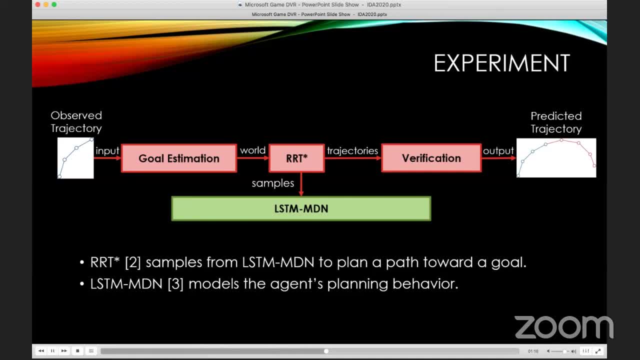 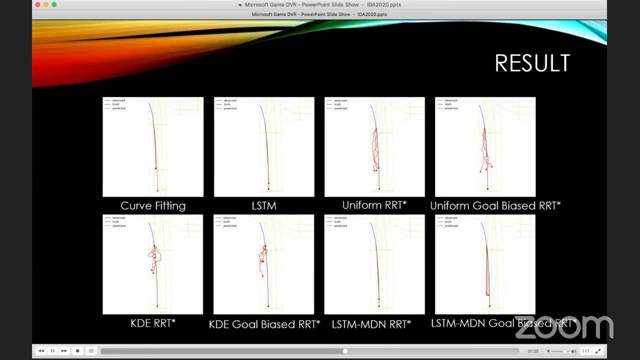 The trajectory planned by RT-star becomes a predictive trajectory of the agent. We test our model with other baseline methods. We can see that traditional methods such as curve fitting and even long-short-term memory occasionally can fail to model an agent's response to the environment. 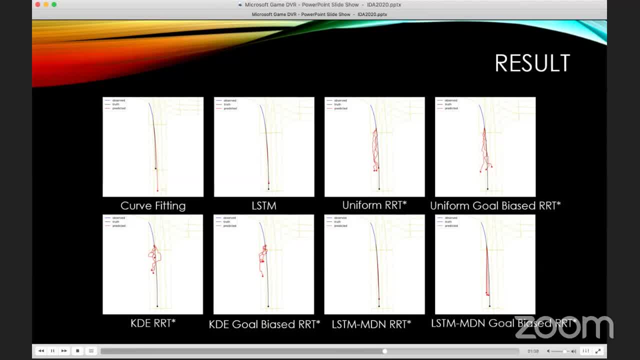 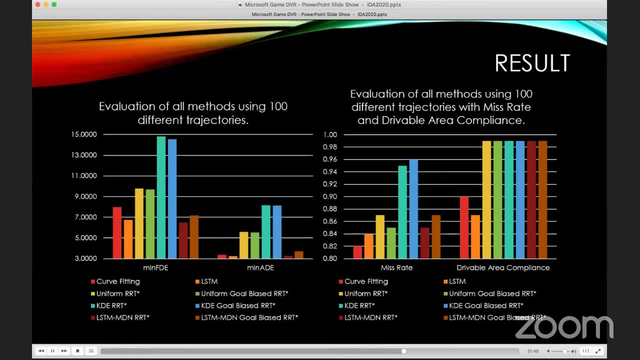 Our model, the OSM-MDN RT-star on the bottom right accurately models the agent's behavior in the environment. We test all methods using 100 different trajectories. The results of the traditional methods are presented on the left of each metric and the results of our method are presented on the right. 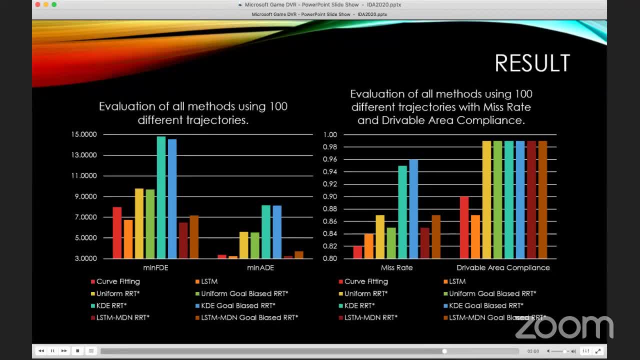 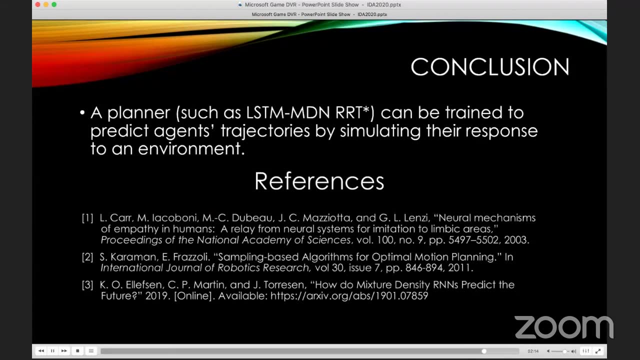 You can see that our method performs similarly to the traditional methods. However, with RT-star as our planner, we ensure that all trajectories stay within the drivable area. From our results, we conclude that a planner such as OSM-MDN RT-star 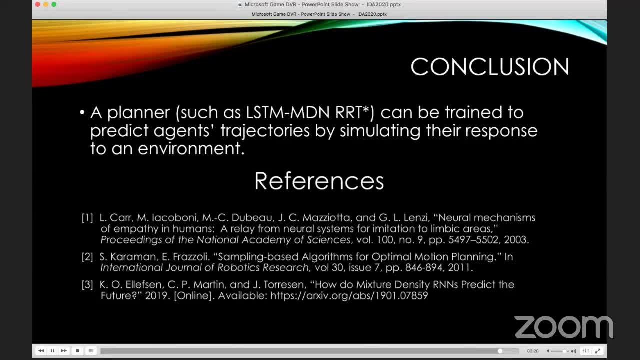 can be trained to predict agents' future trajectories by simulating their response to the environment. Thank you for listening. Okay, Eric, you can unmute yourself. Okay, great, Yeah, actually, I also got a question, So can you comment a little bit more? 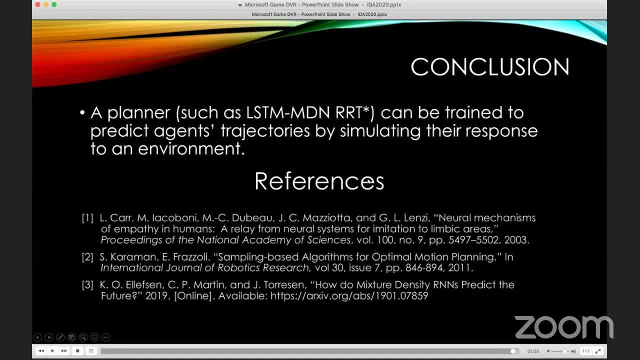 on the generalization ability of this approach, Like I see in the example you use, like a merging or highway, Is it okay to generalize to like, for example, intersections or other scenarios like that? Yeah, so I hope you can hear me. 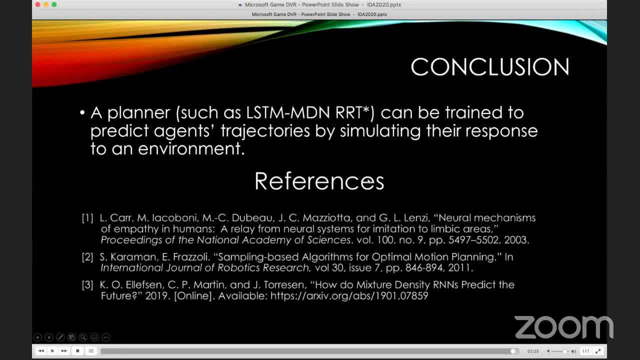 I think this approach can be generalized to like a lot of situations because effectively our experiment is just showing one, like just a small group of algorithms, But effectively you can model the agent's behavior based on different, like environmental factors. 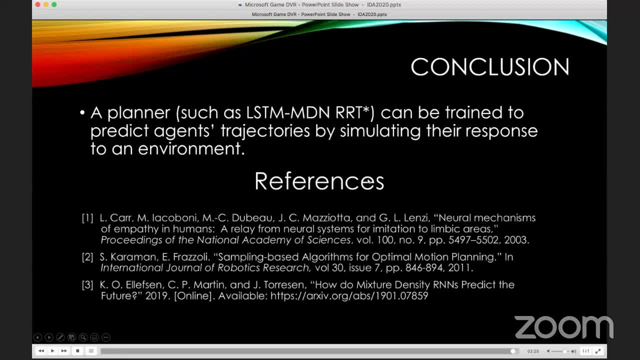 So if you provide a lot of information, say if you add an intersection and then you train how the agent may plan on intersections, then you can also model their behavior that way, using a path-learning behavior. On a larger context, it doesn't necessarily apply to autonomous vehicle. 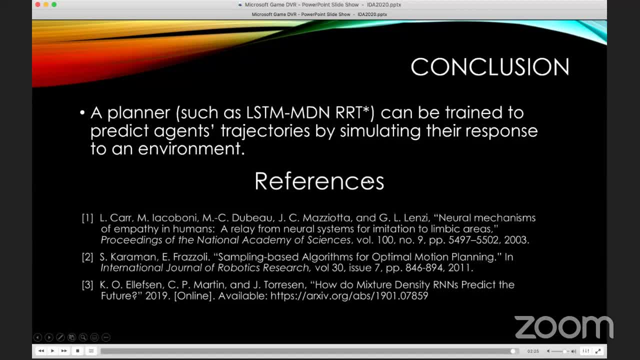 You can also use it for robots in, like you know, indoor or in a room location as well, as long as you have the training data, or if you have a way to train a path-learning algorithm and also provide some environmental context to help the algorithm predict the trajectory of the agent more accurately. 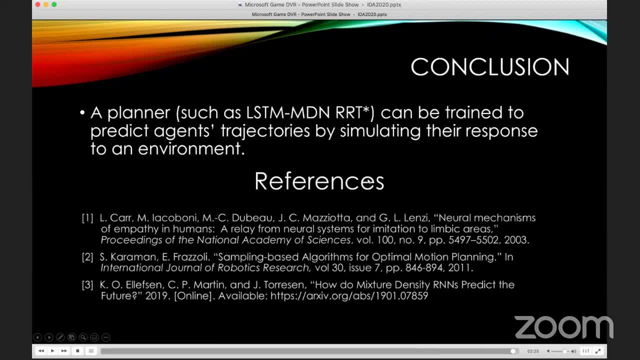 So I hope that answers your question. Yeah, great. Yeah, hopefully in the future we can see more like scenarios using this kind of approach. Thank you very much. Okay, then next one. we'll go for the third talk. 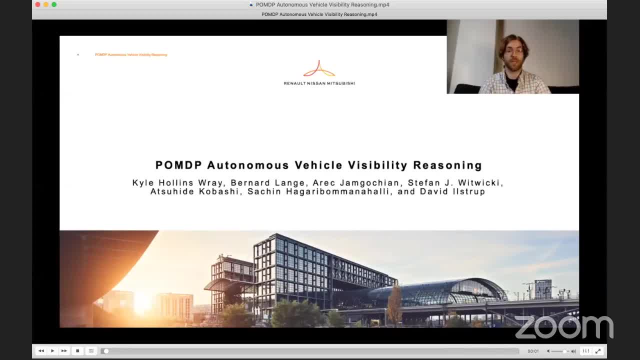 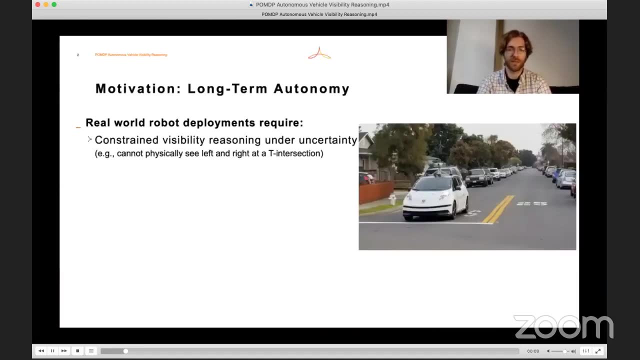 Hello everyone. The third talk is from Kyla. His topic is PalmDP Autonomous Vehicle Visibility Reasoning. My name is Kyle Ray. Today I'm going to talk about PalmDP Autonomous Vehicle Visibility Reasoning. Consider this autonomous vehicle at a T-intersection. 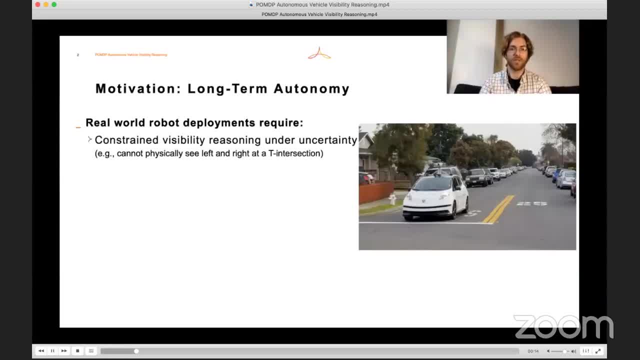 It can't necessarily see to the left and right due to a physical object being in the way, like a fence. Now we have multiple distinct problems here, some involving multiple vehicles, multiple pedestrians. However, these can happen at the same time. 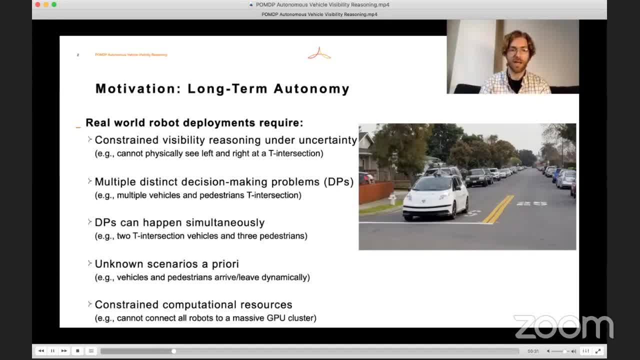 We don't know what we're going to encounter before we drive, and any solution we create has to be done with constrained computational resources. Our solution is to decompose what would otherwise be a rather large problem into small, tractable ones and fuse their solutions online to reduce long-term autonomy. 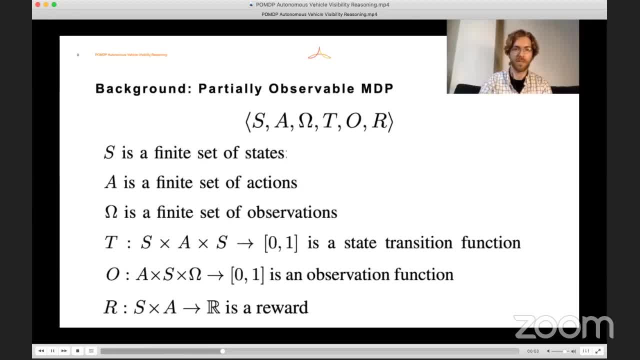 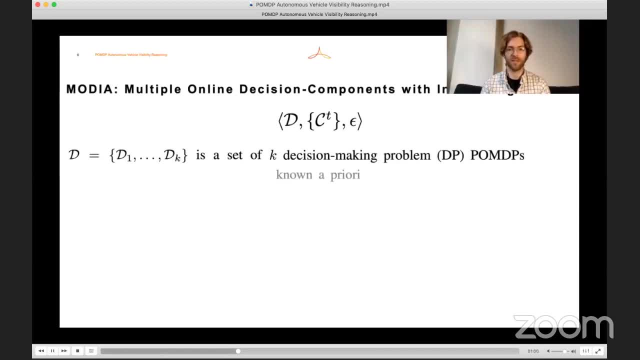 We use PalmDPs as our primary decision-making model and, in what we call MoDIA, Multiple Online Decision Components with Interacting Actions. we have a set of these DPs. Each DP describes a very particular solution, such as dealing with one vehicle on the left. 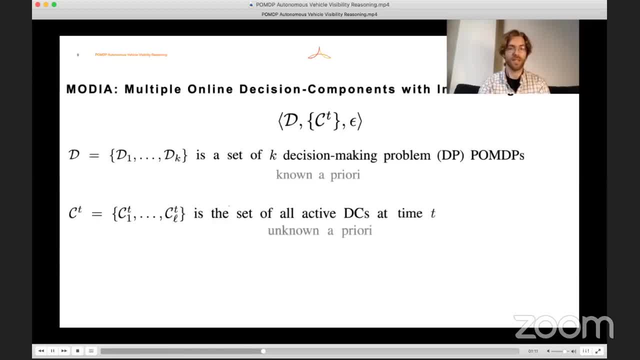 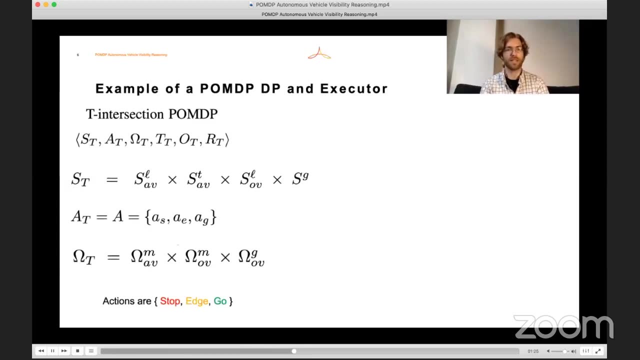 at a T-intersection Online. when we detect them, we instantiate them as decision components. Each decision component then recommends an action and any conflicts among these recommendations are resolved by an executor. Looking back at the T-intersection, its PalmDP has the state of the autonomous vehicle's location. 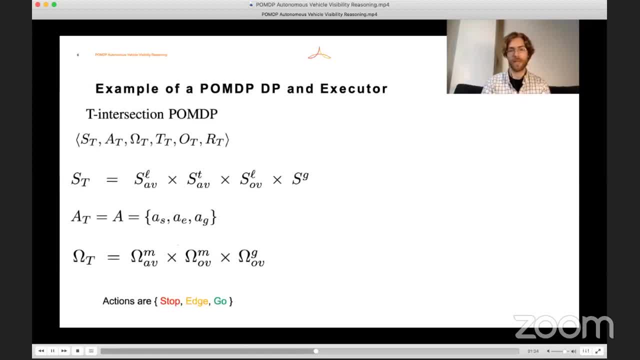 the time, the other vehicle's location and a notion of gap. Our actions are to stop, edge slowly forward or to go. Each of these DCs then recommends actions at particular points along the route. These are called arbitration points, And if there are any conflicts among these recommendations, 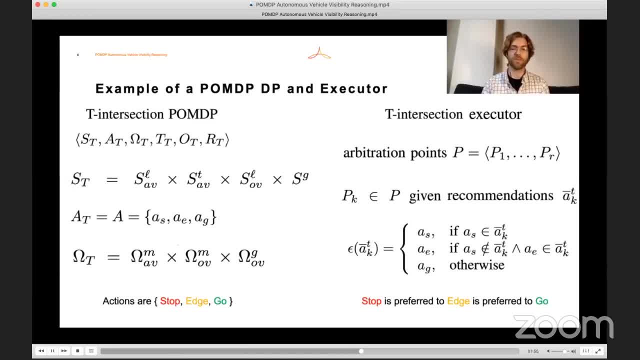 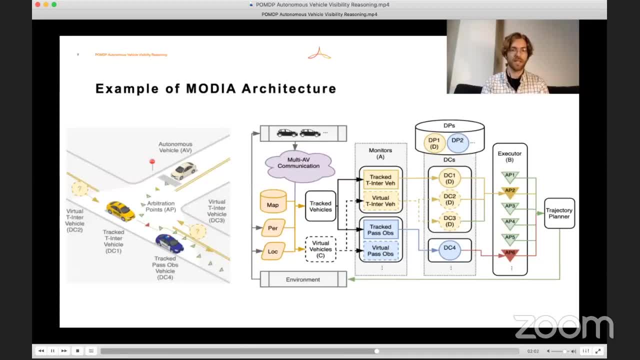 the executor resolves them, such as: stop is preferred to edge is preferred to go. Visually, it looks like this: We have our arbitration points and, importantly, we instantiate virtual vehicles just out of view, and these virtual vehicles are treated as DCs in their own right. 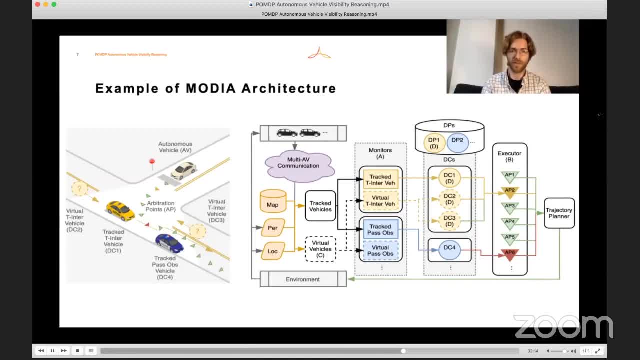 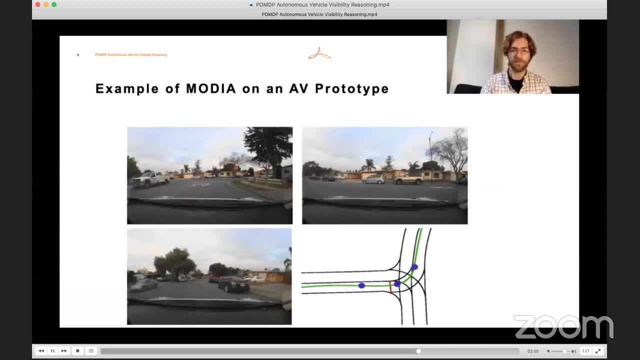 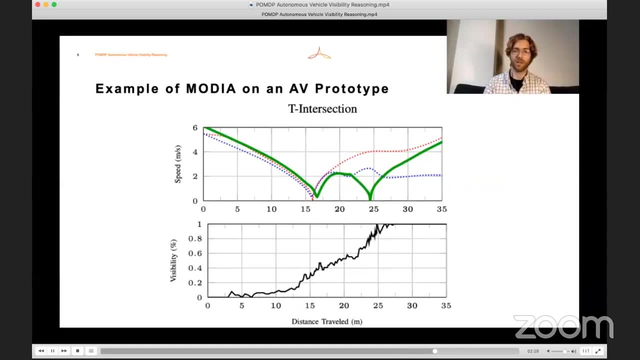 All the DCs then recommend their actions at particular arbitration points and the executor applies its function. Here's MoDIA running on an actual AV prototype. You can analyze its behavior by comparing it with two baselines: The red stops at the stop line and then goes. 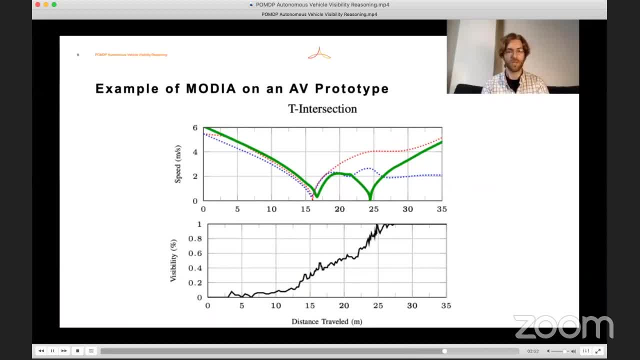 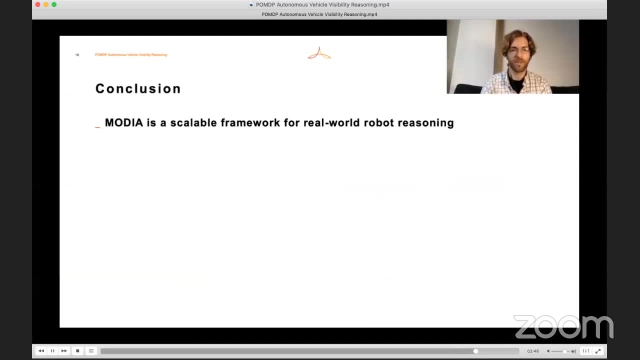 the blue stops at the stop line and then edges, and green is MoDIA. When we see MoDIA stops at the stop line, it edges slowly forward for visibility and as it increases its confidence that there are no other vehicles, it can confidently go forward. 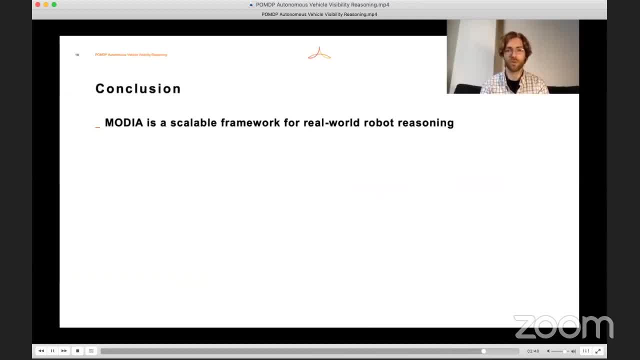 So, in conclusion, MoDIA is a scalable framework for real-world robotics. It has these three components- DPs, DCs and an executor- and we have successfully deployed it on a fully operational AV prototype bringing PUMDPs into the real world. 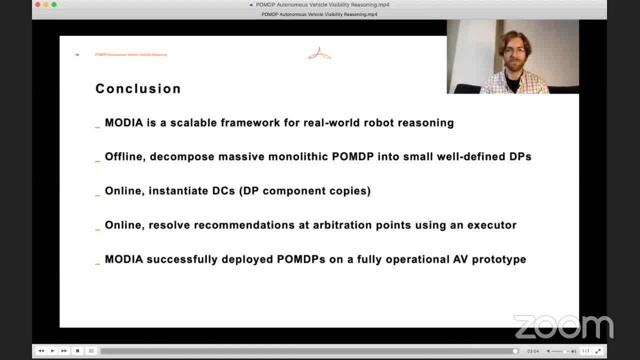 Thank you for your time. Thank you very much, Kyla, can you? yeah, okay, sure, great, I saw you unmute yourself. Yeah, I found this is a very interesting idea, So, but can you comment a little more on the optimality of the solution? 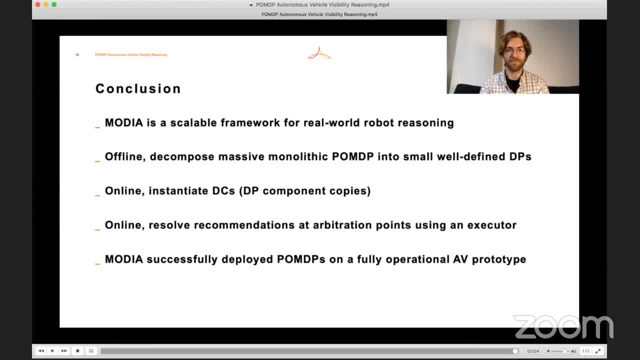 which is obtained by the recommendation, from the recommendations? Yeah, for sure. So, because we're decomposing it in the sense of each individual PUMDP, you can take suboptimal actions And actually we can evaluate what that would be by looking at. 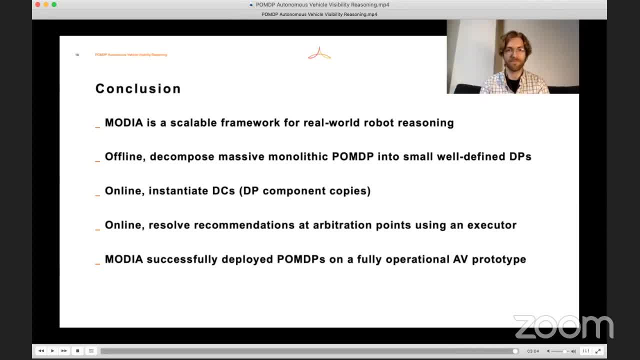 you know, just running the math for changing your actions. say, if you always took the edge action. So there's a relationship between MoDIA and what happens with a constrained PUMDP, in that you're essentially subject to constraints from multiple different objectives. 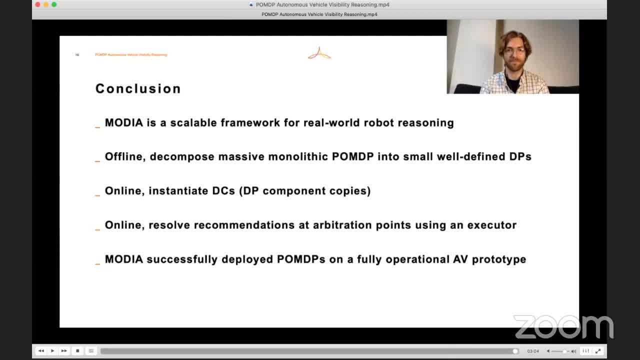 and your policy changes accordingly. Okay, and so is there a way to like somehow, like constrain or quantify this kind of suboptimal optimality? Yeah, so in a previous paper we looked at minimizing a notion of regret. 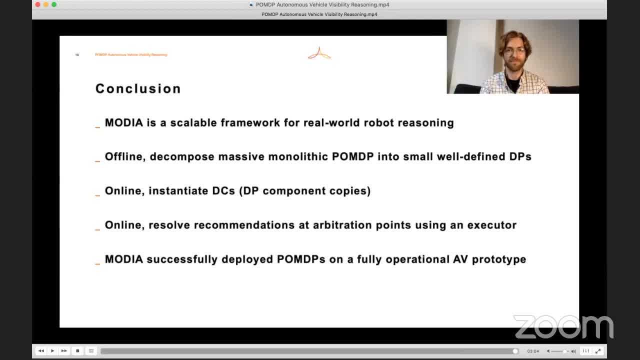 But, because this is the core assumption- is that you don't know what you're going to encounter a priori, because you're actually driving the actual robot around. So because of that you can't, like a priori, determine what the regret would be. 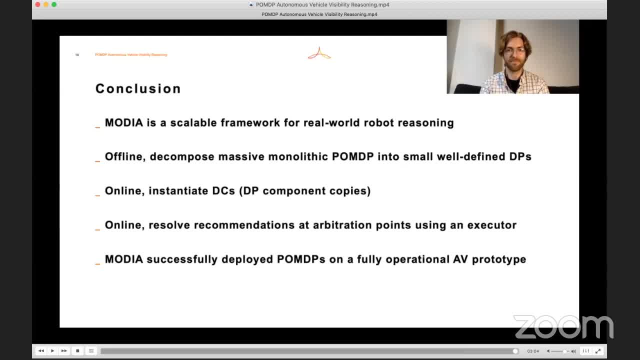 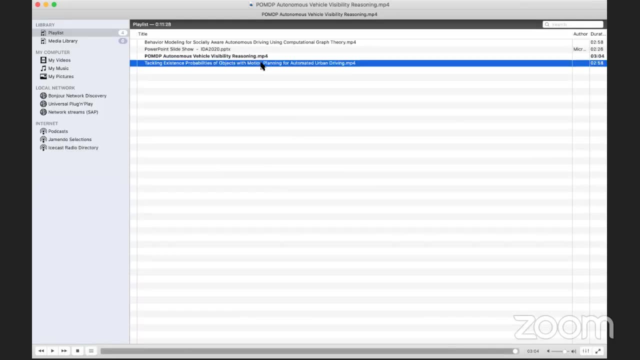 but you can prove that at any given time, you minimize one-step regret among the models, And so that's what we did. Okay, great, Thank you, very much. Cool, Thank you, Yeah. Okay, let's go for the last Contribute Talks. 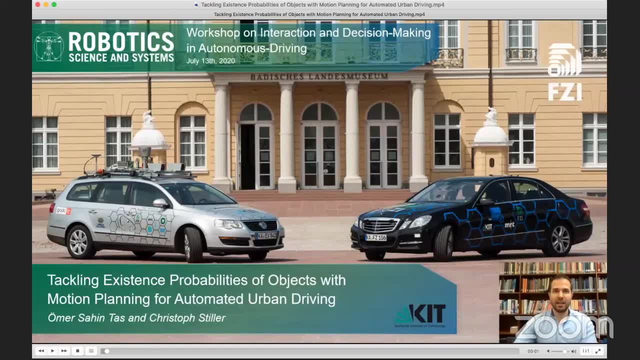 Hi, this is John. This is from Omar Sahin. His topic is about tackling existing probabilities of objects with motion planning of of how how many automated urban driving? Hello, I'm a PhD student working on motion planning for automated vehicles in Karlsruhe, Germany. 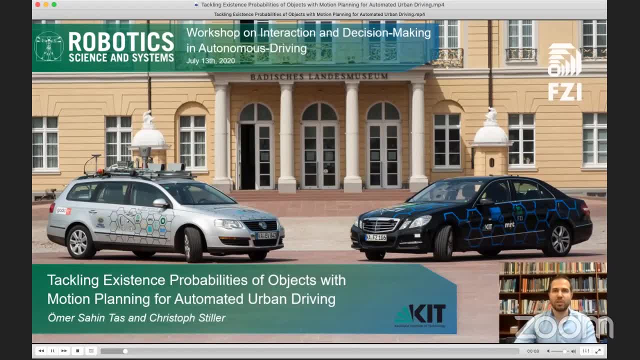 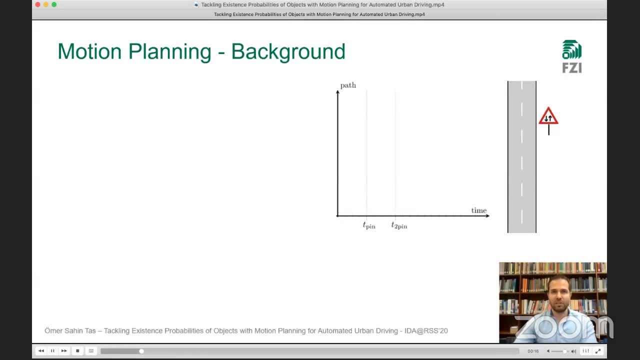 Today I will present to you my paper on tackling existence probabilities of objects with motion planning for automated urban driving. To ease understanding, I will start with the basics. On this slide, on the right side you see a street. On its left, the part-time diagram is plotted. 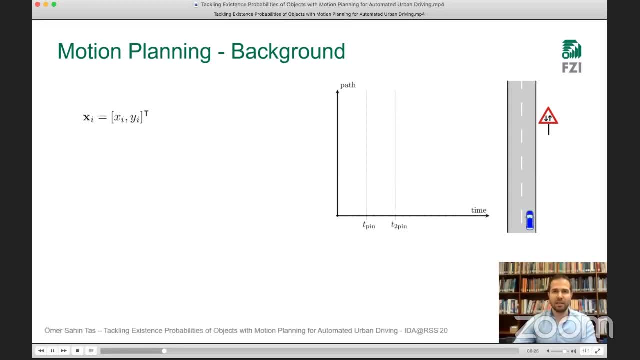 Cartesian coordinates are mapped to the part-time diagram. The depicted blue vehicle is the IGO vehicle. The selection of the blue vehicle can be obtained by solving an optimization problem over the planning horizon. The first part of the motion until taping is taken from the previous solution. 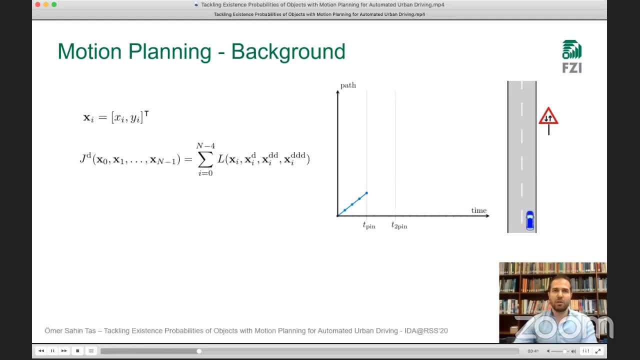 This resembles some time periods slightly longer than the computation time. The motion until here is fixed for a temporal consistency. Now that there is a vehicle in the front to highlight the main contribution of this work, we will predict its motion deterministically. here, Given some cost, function and constraints, we can solve the optimization problem to obtain a motion. 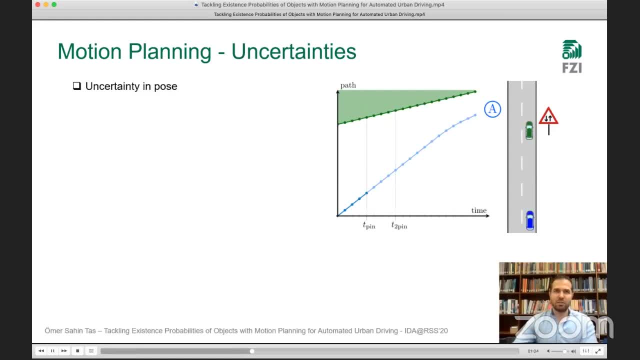 State-of-the-art motion planners consider uncertainty in cost and uncertainty in prediction, which includes uncertainties in route whenever intention and motion profile. However, there is a further type of uncertainty, which is uncertainty in resistance. There are some works which cover uncertainties after the field of view, but there is no work that tackles quantum detections. 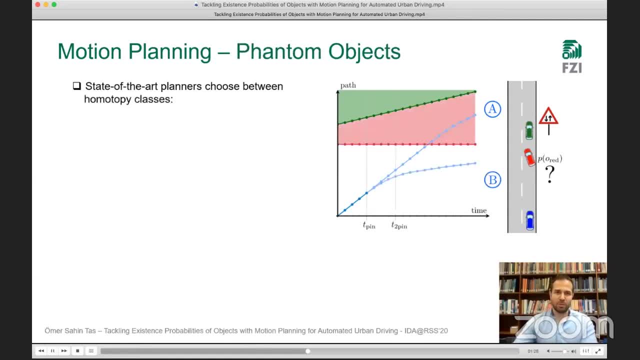 State-of-the-art planners choose between homotropic classes. They decide to pass, ignoring the potential existence of the phantom object, or they act conservatively and yield to it. Our motion planner considers the urgency to react to a potential phantom by executing an undecided motion. 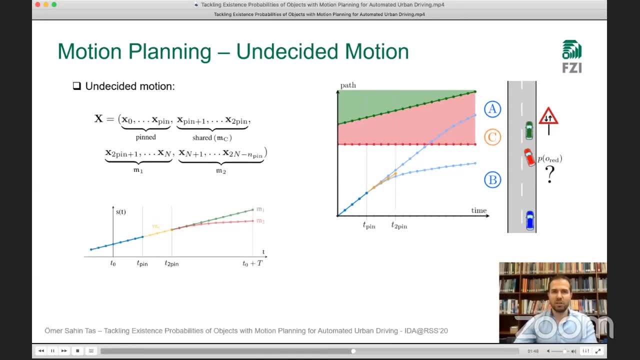 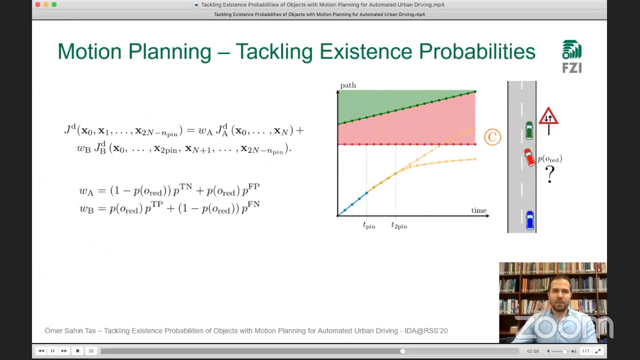 The key point in planning an undecided motion is to modify the optimization parameter vector so that it accounts for the both maneuver options. Here you see the pinned part, the shared part until the next planning time step, and the distinct maneuver options. The distinct ones will be replanned in the next time step. 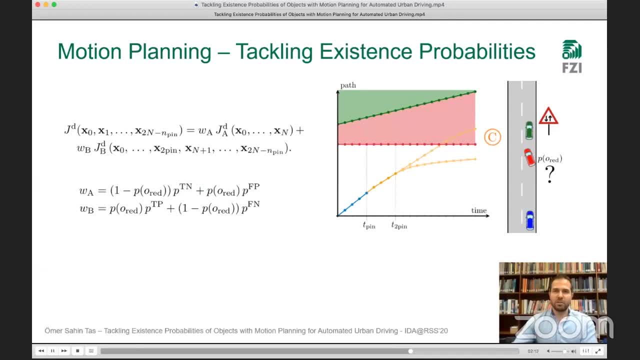 To handle existence probabilities, we weight the cost terms of individual maneuvers. We calculate the weights by considering the existence probability of the object and the detection probabilities of the detector. In some cases, even though the existence probability is high, the distance probability is low. 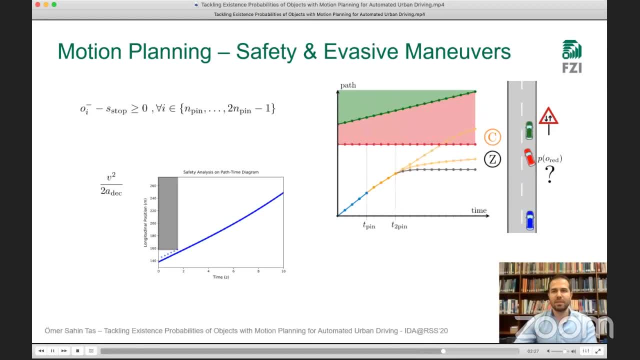 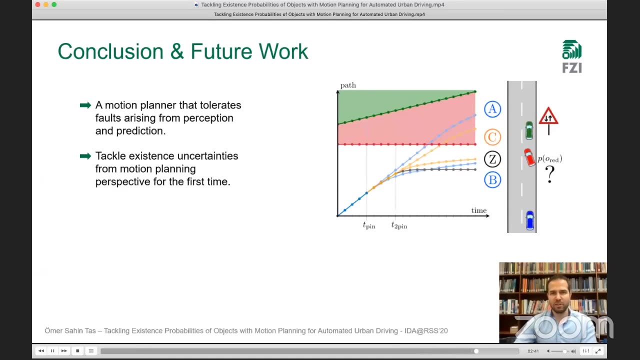 The existence might set in shape over time. To guarantee safety, we apply a constraint that ensures the vehicle to come to a safe stop after executing the neutral motion. To sum up, we present a method that allows the planner to tolerate faults arising from perception and prediction. 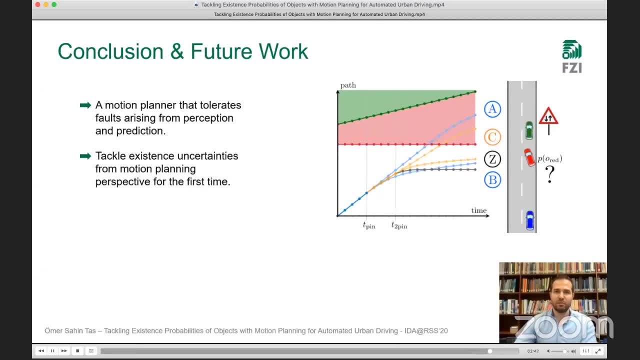 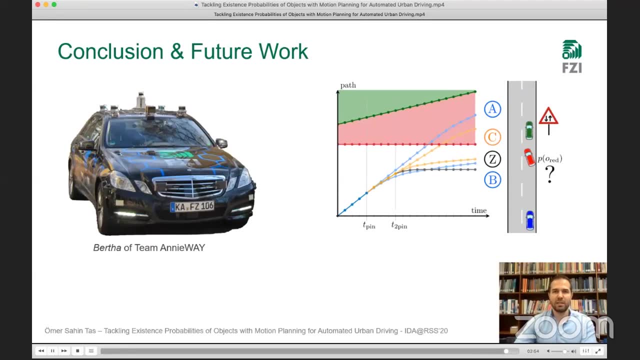 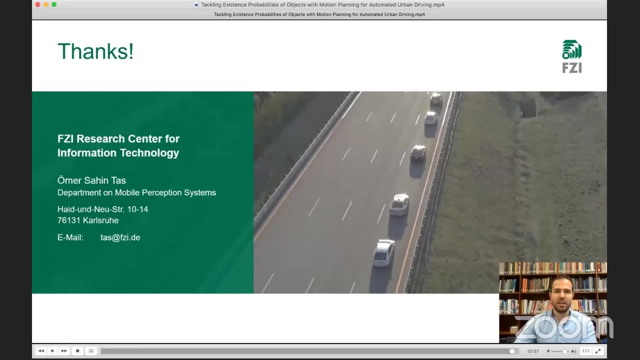 We tackle the existence uncertainties from the motion-planning perspective for the first time. Our future work focuses on increasing scalability and robustness of the approach. After that, we will integrate the planner in our automated model. Okay, okay, great. Sorry, you have unmuted yourself. 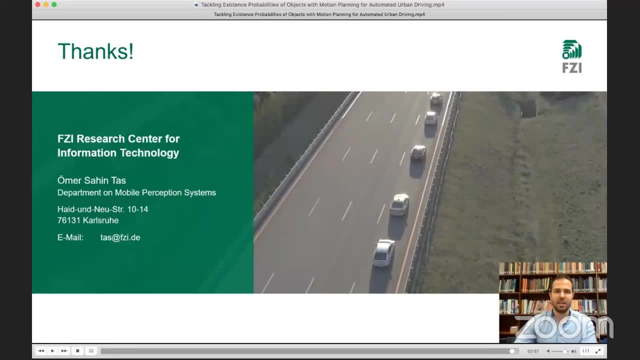 Yeah, Okay, Yeah, very nice work to dealing with the uncertainties. I have a little bit more questions regarding the safety constraints. So you separate the planning horizon into, like a determined one and a filter one, And filter one is considered uncertainties. So how about the safety constraints? 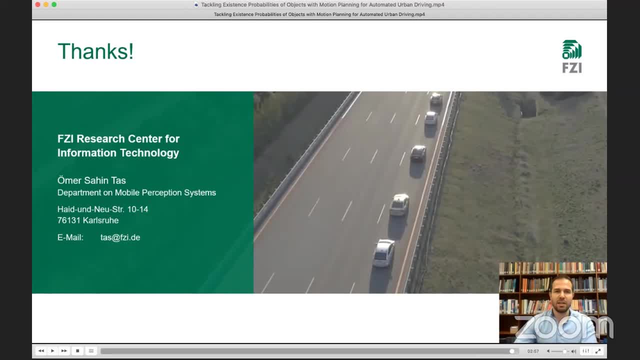 Do you need to consider all the safety constraints under different homopathies? Yeah, In that you see in fact all the safety constraints. I didn't present that in the paper in the presentation, but you can find them in the paper as well. 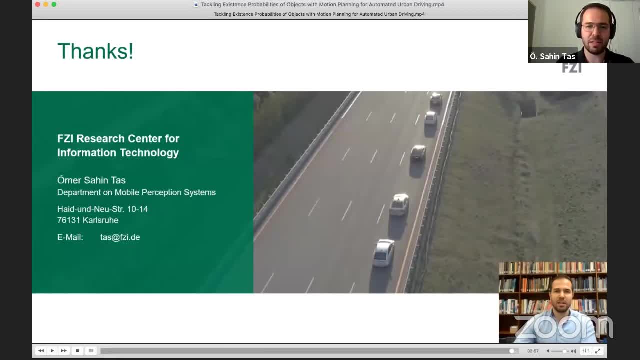 But the crucial one is the replanning. So we plan, we make a receding horizon planning And in that we. The key difference is in which time steps we constrain the safety constraints. The rest is, as we presented in our IV 2018 paper, handled with soft constraints. 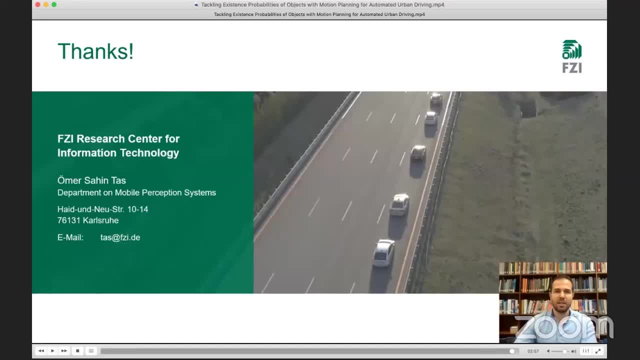 Okay, great. So you are like treating the constraints as soft constraints, not hard constraints? No, not exactly. So you are making a replanning, So what you have to do is you have to ensure that your motion, which will be fixed in the next planning time step, 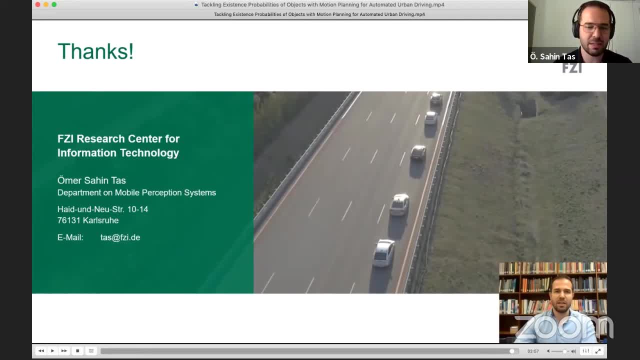 satisfies all the constraints. Even the scene in the current situation evolves so that it's- how can I say, the worst case for the automated vehicle. If you can guarantee the safety for the next, so to say, replanning time, the rest will be discarded. 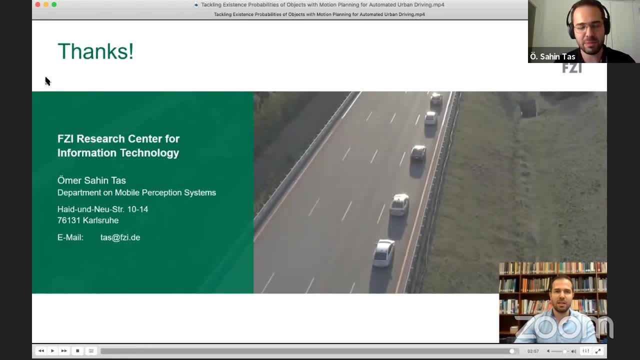 It will be replanned during the next replanning time step, So you can treat them with a soft constraint. Okay, great, That answers my question perfectly. Yeah, I think that will be. Thank you very much, Sahid, for participating in the workshop. 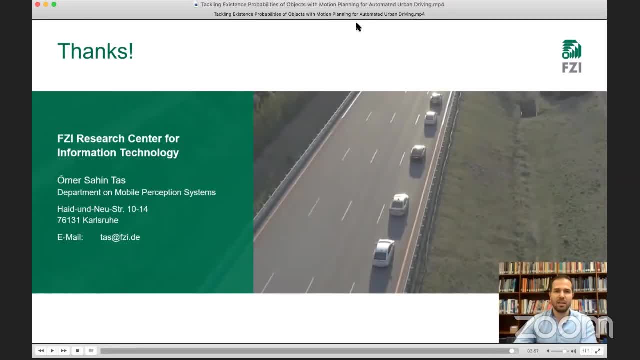 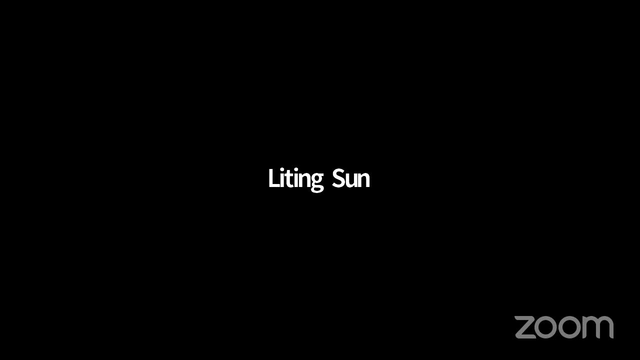 Yeah, Thank you. Okay, I think that will be all for this morning session. Again, I think we are a little bit several minutes ahead of schedule, So I think right now we are going to enter the break session. the break. 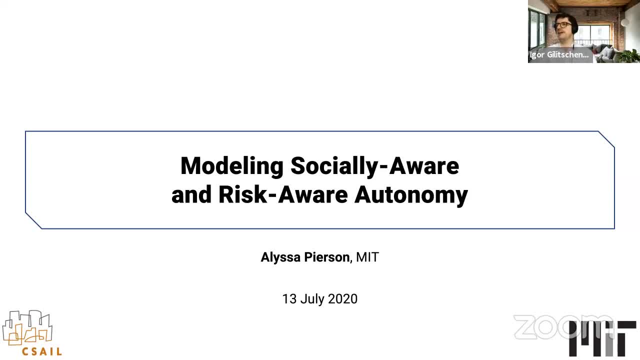 back to our afternoon session. so it's does sharing work for you? Yeah, perfect. So I will briefly introduce you and then we can get started. So welcome back to our afternoon session. It's my great pleasure to introduce Alyssa Pearson. Alyssa Pearson is usually my office mate, but in this special circumstances we mostly see each. 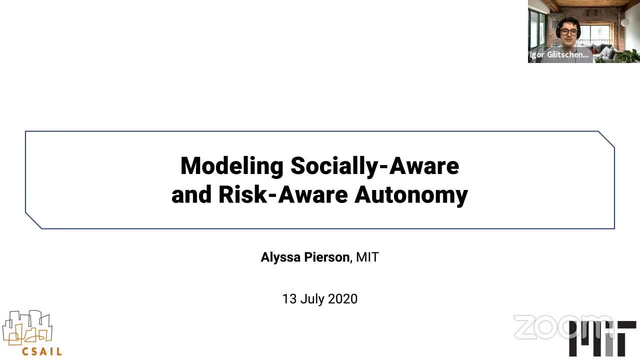 other via Zoom, And Alyssa is a research scientist at CSAIL And before joining us she was working on her PhD at BU and Stanford, And now she is working on actually exactly what the title of the talk is- Modeling Social Aware and Risk-Aware Autonomy- And it's really a super cool work. So I 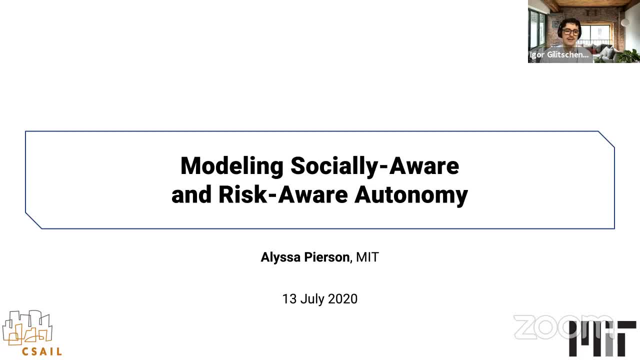 look very much forward to your talk And I can also announce people who are interested in her work. You can check her out at MIT and soon you can check her work out at BU. Alyssa will be joining the Department of Mechanical Engineering at BU. 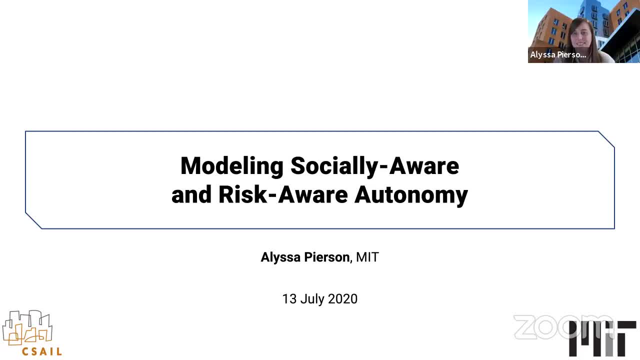 In January. January is correct. right, That's correct. Yeah, in January. So yeah, we look forward to your talk. Thanks for joining us today. Thanks, Igor, And thanks everyone for tuning in. It's been a great day so far in the workshop. 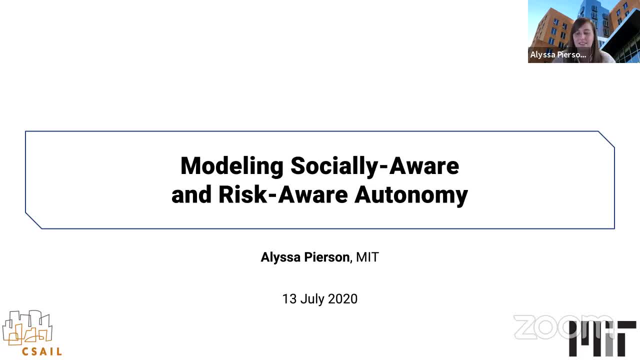 listening to a lot of interesting and fascinating talks, And so I hope you find my work interesting as well. So for my talk today, I thought I'd talk a little bit about some of the different types of problems that we're using to model both socially aware and risk-aware autonomy within our lab. So, as 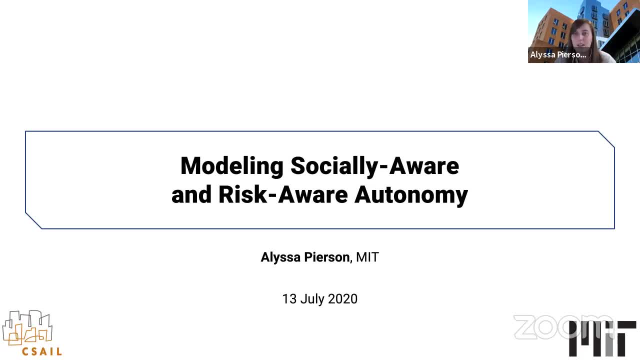 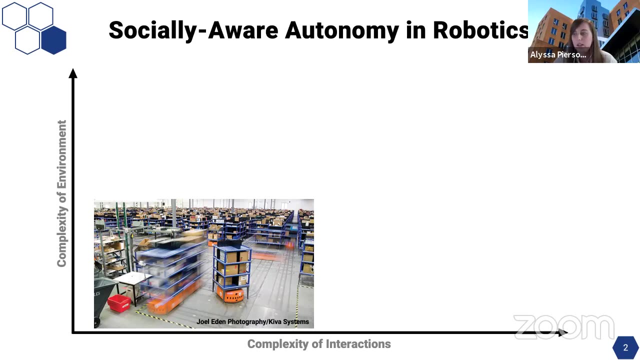 Igor mentioned, my name is Alyssa Pearson, I'm a research scientist at MIT, CSAIL, And specifically I'm working in the distributed robotics lab, And so when we think about socially aware autonomy and robotics, there's a lot of different domains that we can think about, And I tend to think about these. 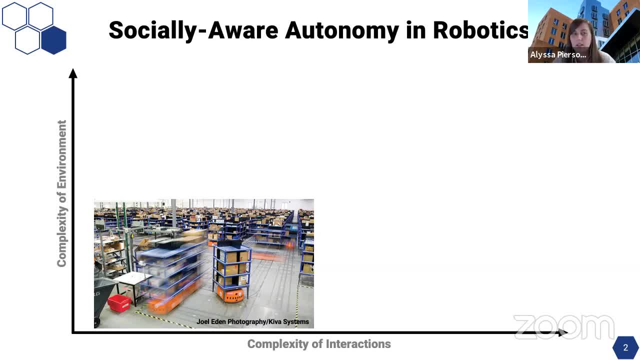 different problems, as both scaling in the complexity of interactions and the complexity of the environment, And so we can think about the autonomous robots that work in a warehouse without human supervision or in close proximity, but not directly around other humans. We can increase that complexity to think about the robots that work in agricultural monitoring. 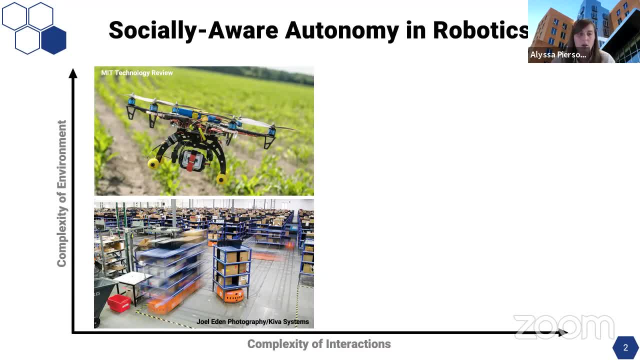 different types of drones for crop monitoring, or maybe thinking about the types of robotics used for herding animals, where we're starting to think about the types of robots that work in large, large plants to deal with much more complex interactions. But really what we're all. 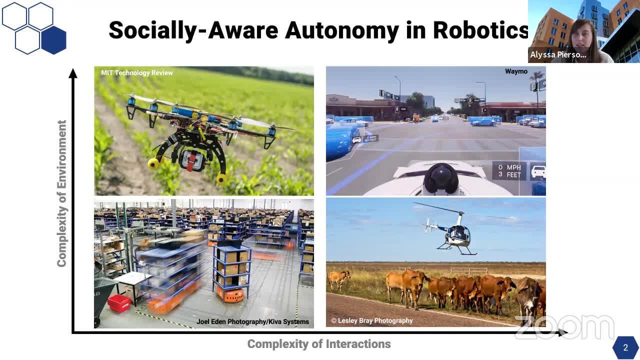 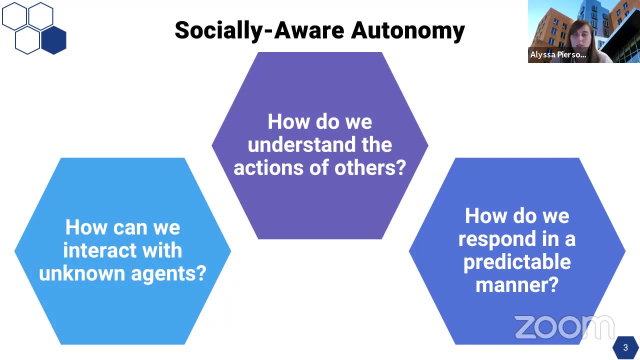 interested in here today is the most complex environment and type of interaction, and that is autonomous driving with humans. And so when we think about trying to design this socially aware autonomy, I like to think about it as breaking down into three big questions. First, how do we 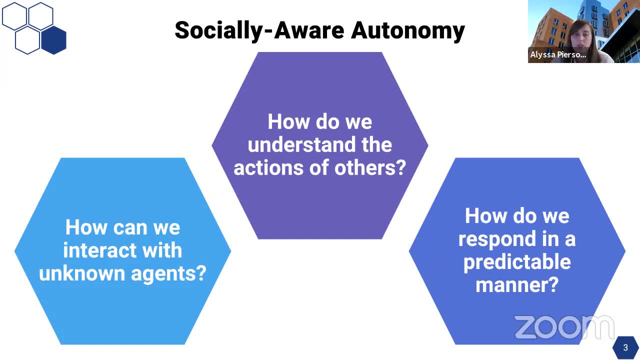 understand the actions of others And how can we respond in a predictable manner? And finally, how do we interact with those unknown agents? And that third question, that unknown agent interaction, I'll be talking about as I also transition into the risk-aware autonomy in the 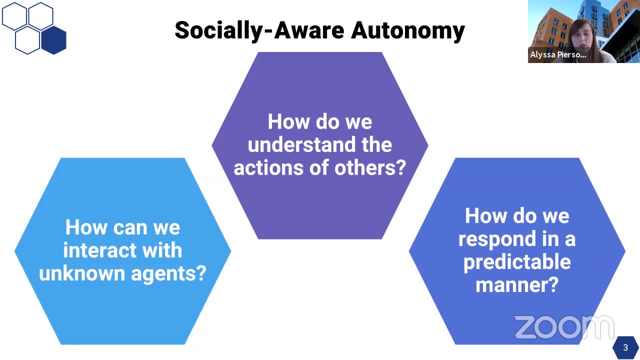 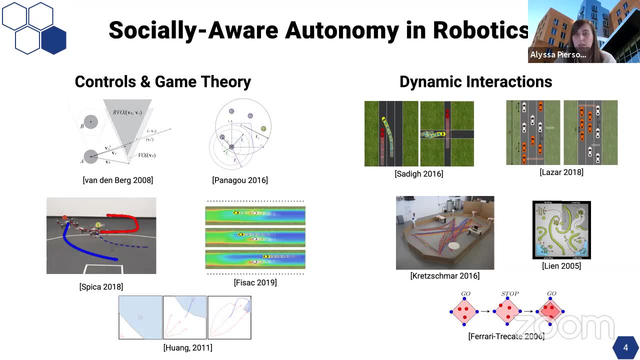 later part of my talk, But to begin with, with socially aware autonomy, our work looks at a lot of this modeling in both the controls and game theoretic space, as well as how we can model these dynamic interactions, And you have heard a lot about other approaches, especially in the keynote. 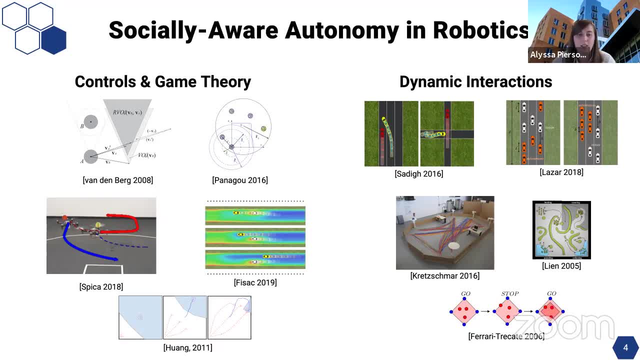 today, as well as the fascinating spotlight talks, And, in particular, what we're going to be looking at is how we can use tools from game theory and tools from Lyapunov-like control theory to guarantee performance of these different systems under varying social models that we can. 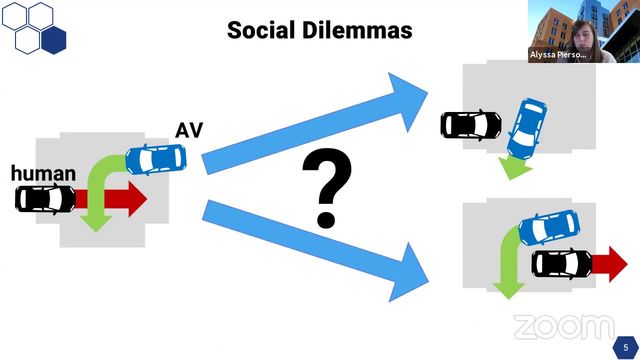 prescribe to them. And so, starting off, one big question we've looked at is looking at these social dilemmas in driving. And what do I mean by a social dilemma? Well, social dilemmas are when the collective interests within a group are at odds with the individual interests of any given agent in the system. 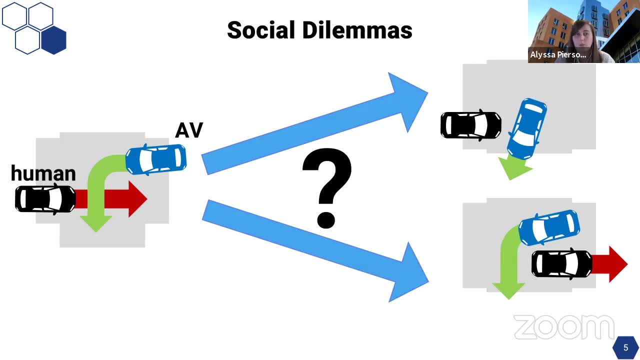 So let's take this example. You've got an autonomous vehicle in blue that needs to make an unprotected left turn and there's a human driver in the oncoming lane of traffic. How does the autonomous vehicle know what the human will do? Will the humans slow down and yield, allowing that? 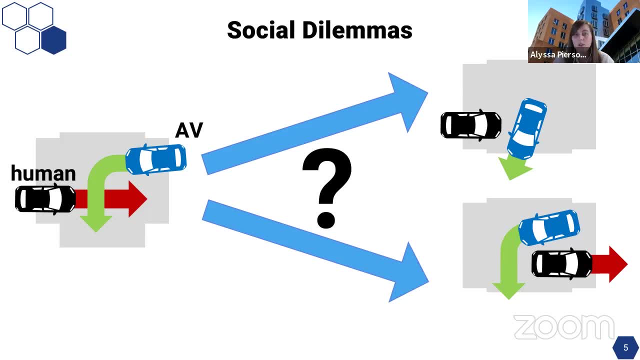 autonomous vehicle to make the left turn. And what do I mean by a social dilemma? Well, social dilemmas are when the collective interests within the same system are at odds with each other and there's a human driver in the oncoming lane of traffic. How does the autonomous vehicle know what the human will do? Will? 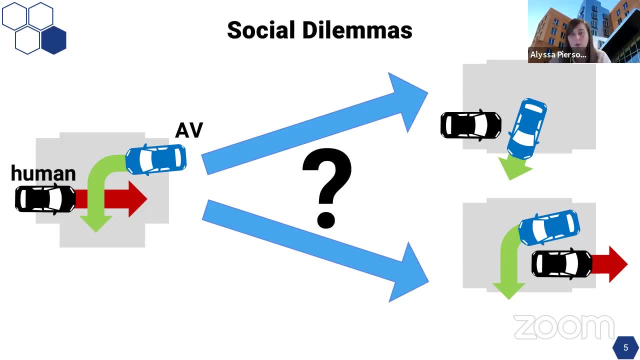 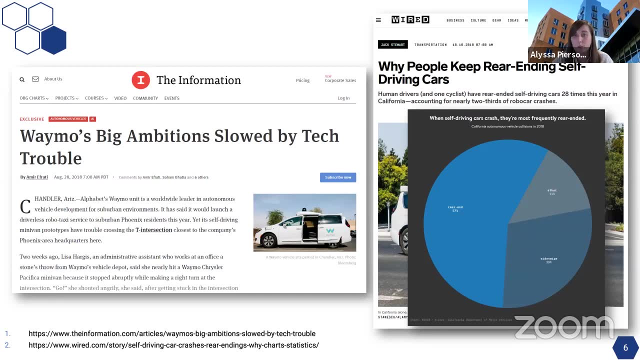 the human will do? Will the human driver make a left turn first, Or should the autonomous vehicle wait for the human driver to pass before attempting this merge? And this is fundamentally important to safety and scalability in these systems- We see already that in some of these deployments of 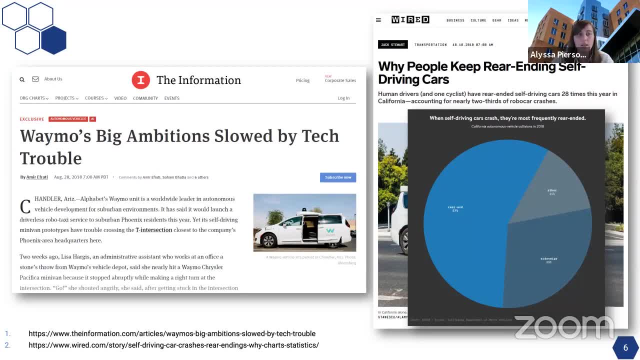 autonomous driving. right now, these autonomous cars aren't necessarily acting in an understandable way and a predictable way for these human drivers And, as a result, are These autonomous cars aren't necessarily acting in an understandable way and a predictable way for these human drivers and, as a result, are are essentially diversified due to the change in situation in the system and how they're. 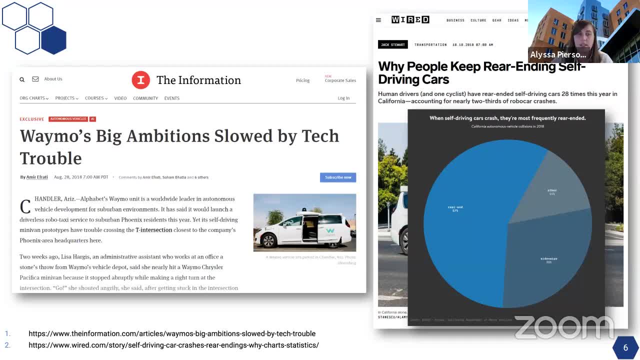 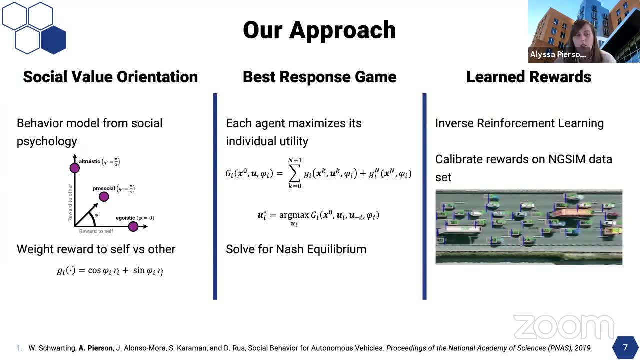 getting into accidents that we don't typically see in sort of the human-to-human driving space, And so our approach to look at this was to look at tools from behavioral and social psychology. So, specifically, we're going to use something known as the social value orientation. 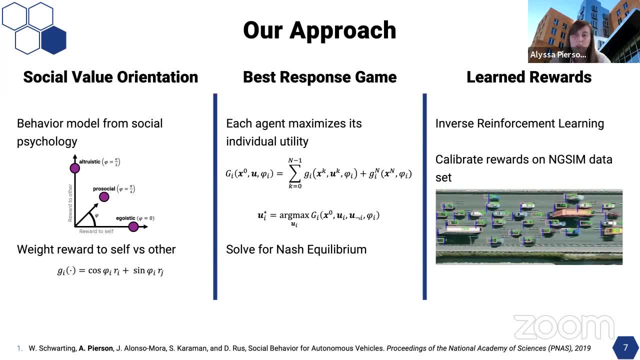 which is a metric that weights the kind of social preferences of an individual agent against another agent. We're going to integrate that into a best response game, which hopefully by now you're very familiar with after the wonderful talks by Dorsa and Anka earlier today. And then, finally, we're going to learn the rewards of the system calibrated. 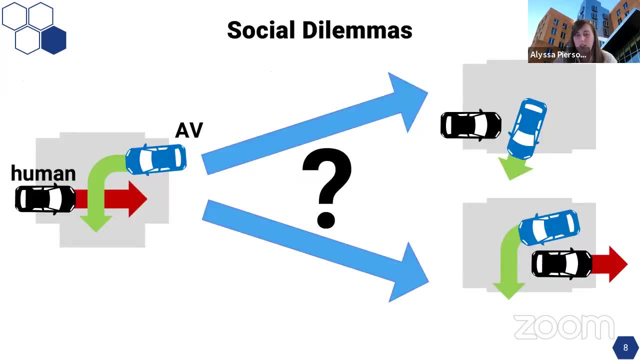 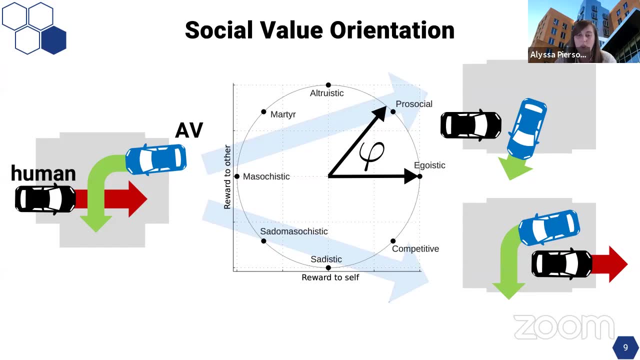 specifically on the NGSIM data set. And so, when we go back to the social dilemma, we propose that it's the social value orientation that can help us resolve this conflict And if we can understand the SVO, or if we can predict the SVO of these other vehicles. 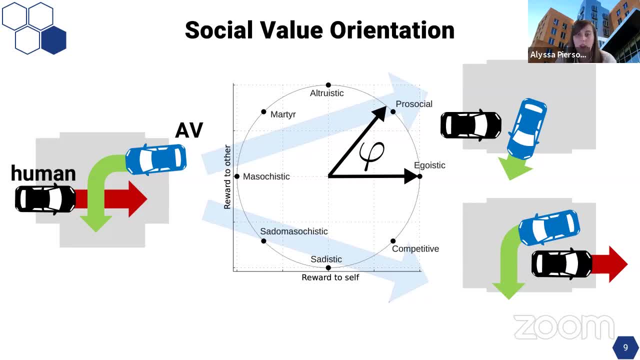 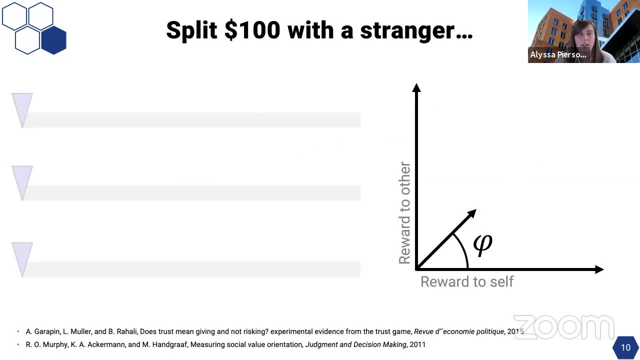 then we can better predict which outcome the system will have. So what is SVO? Well, the classic experiment in social psychology is to say: split $100 with a stranger. Now you may decide that you don't need the money and you're going to give the stranger the full $100. 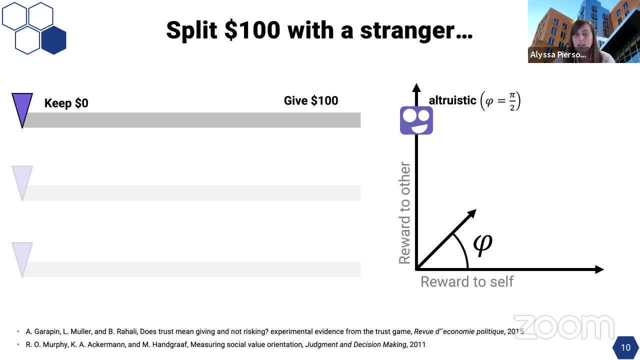 and you keep none of it. In this case, the reward to the other person is the full reward and the reward to self is the full reward And the reward to self is zero to you. And that would be an altruistic decision. And we're going to represent that reward to self versus the reward to other as this angular 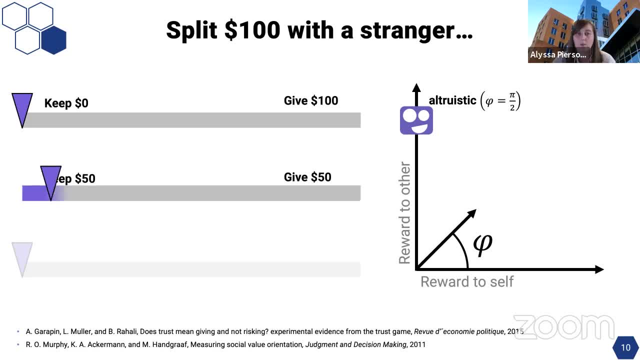 notation fee, You might say: well, I'm going to keep $50 and give $50 away, And in that case that's a pro-social decision. That angular pile over four represents the equal reward to self and the reward to others. And finally, you might say: I don't know them, They're a stranger. 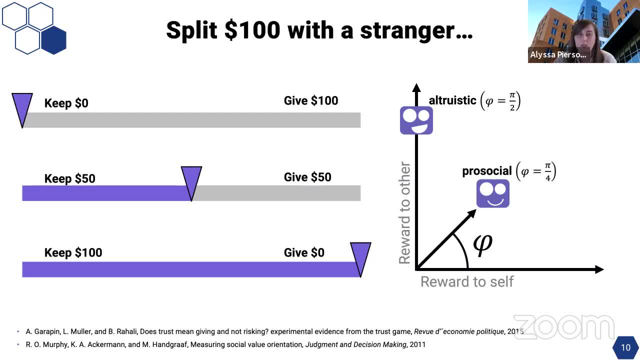 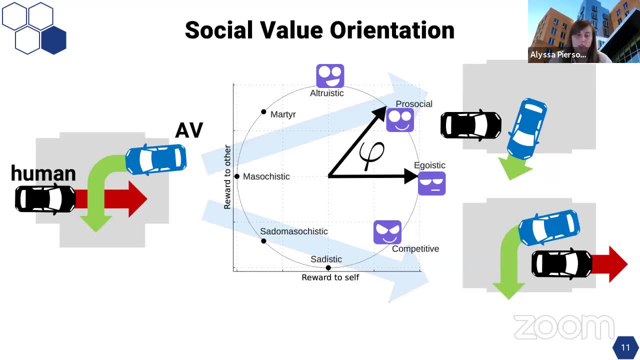 I'm going to keep the full $100 and give none to the stranger, And that would be an egoistic decision Now. we can then take this in our work and we're looking at how we can take this social value orientation, all of these social preferences, and map it down into the autonomous driving space. 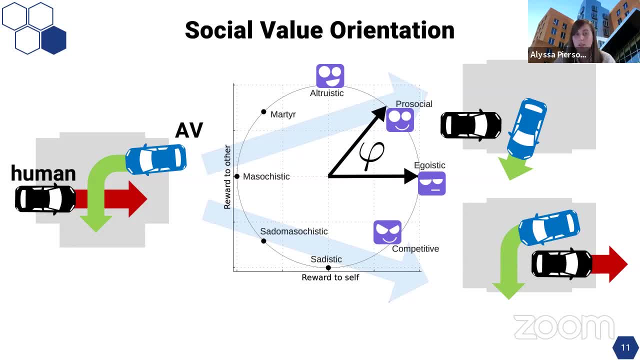 And so now we're going to look at what defines an altruistic driving decision and what defines an egoistic driving decision, And in fact we're even going to see a little bit later that there's a notion of competitive decisions. Now, a competitive decision in the previous analogy of 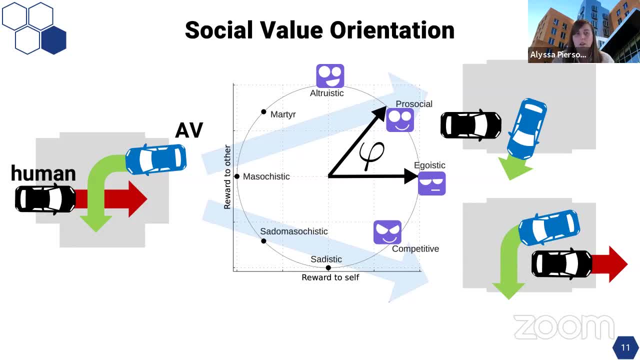 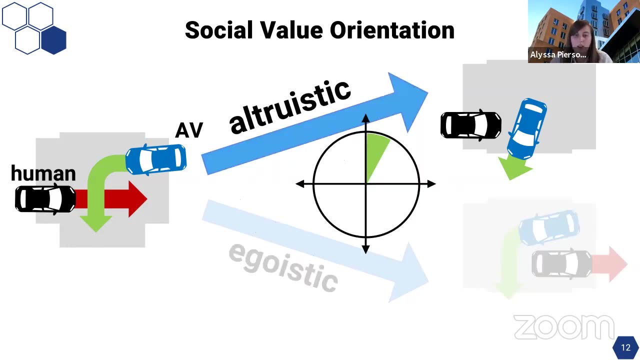 sharing $100 is where you take a full reward to yourself as well as look for a slightly decreasing reward to another person. So in that example, it would be as if you kept the $100 and then also managed to steal $5 from the stranger, And so what we propose is that an altruistic decision. 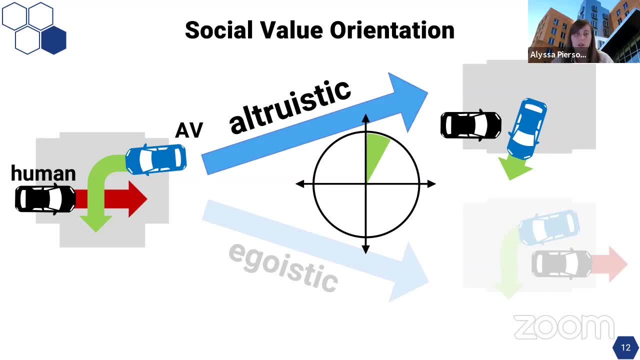 on the human. if the human has an altruistic driving decision- it's going to be an egoistic social preference- Then that's going to be the indication that the human will yield for the autonomous vehicle to make the turn. And conversely, if the human has an egoistic social 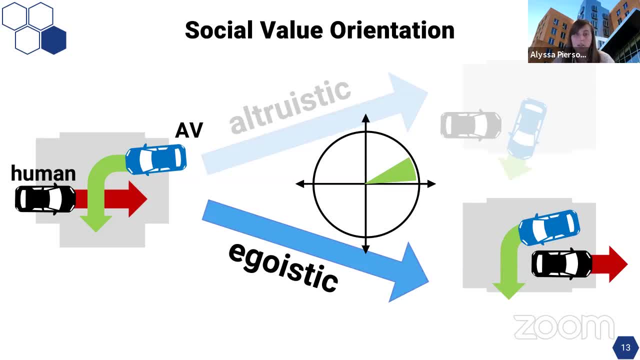 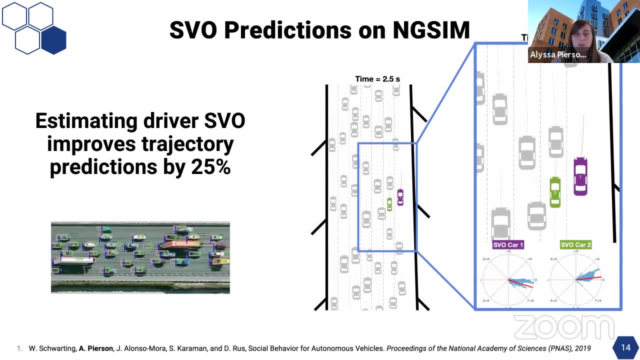 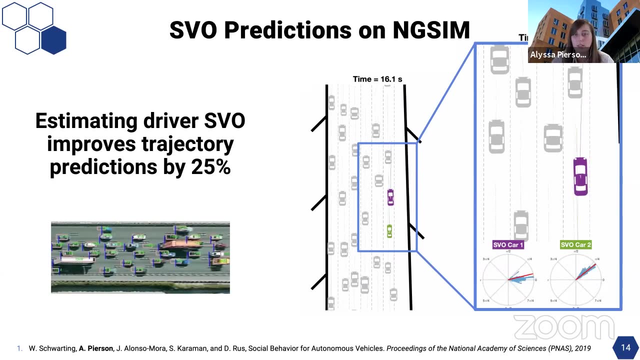 preference, then the autonomous vehicle should wait, because the human driver will not yield for that autonomous vehicle, And so within our work we've actually looked at how we can validate this within human driving data. So we've looked specifically at the NGSIM data set. 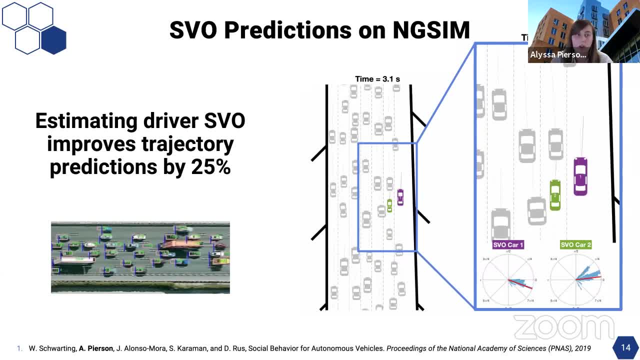 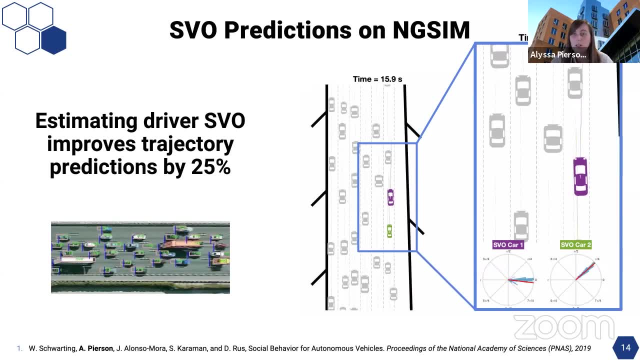 where we have different cars merging on the highway driving, So this is purely human drivers. right now. We're not looking at autonomous vehicles just yet And we're looking at how these SVO preferences evolve over the course of interactions, And what we've found is that by 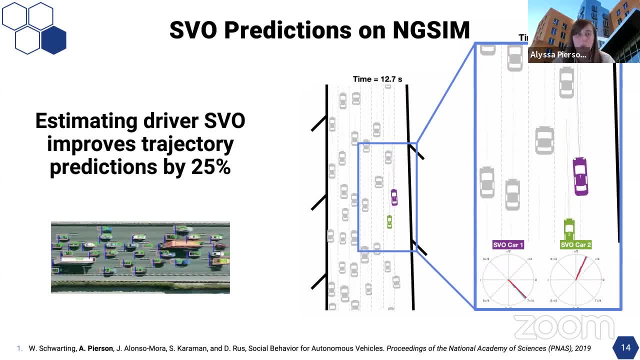 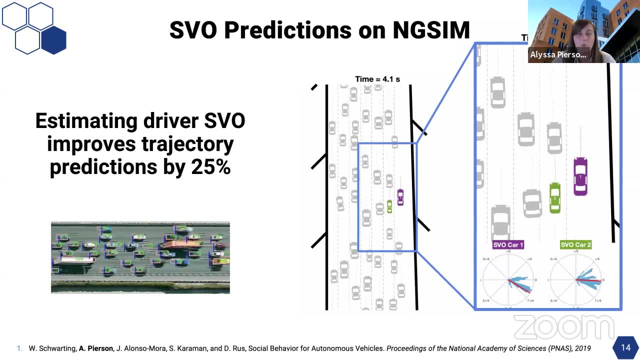 integrating SVO into our prediction model of how the humans behave, we can improve our trajectory predictions by 25%. And in this video on the right, what we're seeing here is we're seeing these SVO predictions and we're seeing these SVO predictions and we're seeing these SVO predictions. 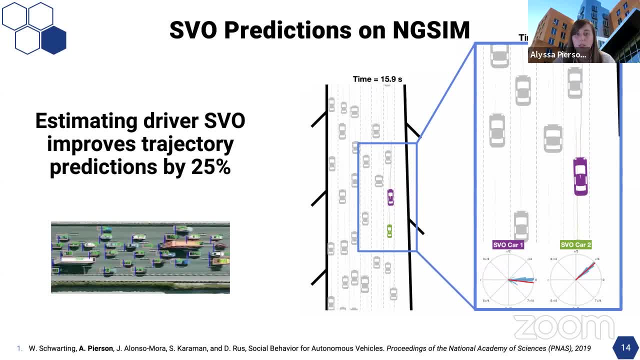 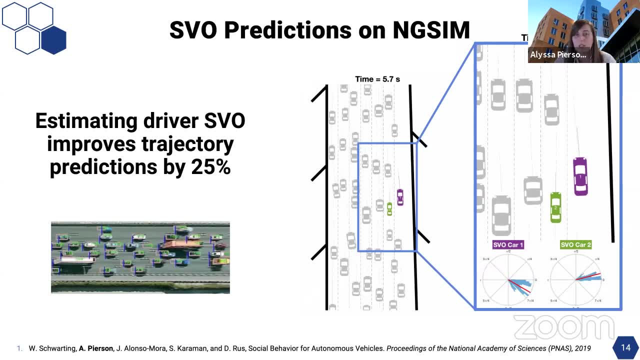 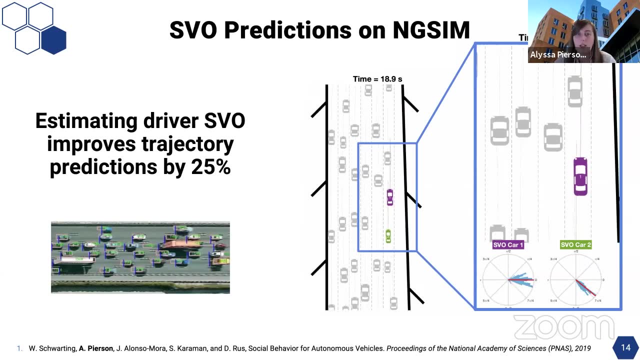 occur during a merge onto the highway. So we've got the purple car merging onto the highway with the green car And what we can see is that during the merge the purple car actually becomes a little bit more competitive to nudge in and to get into that lane And that the green car 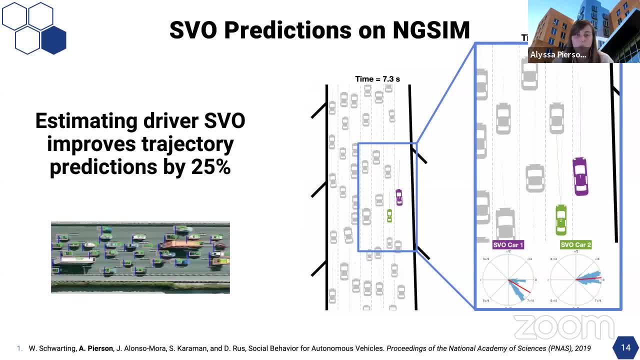 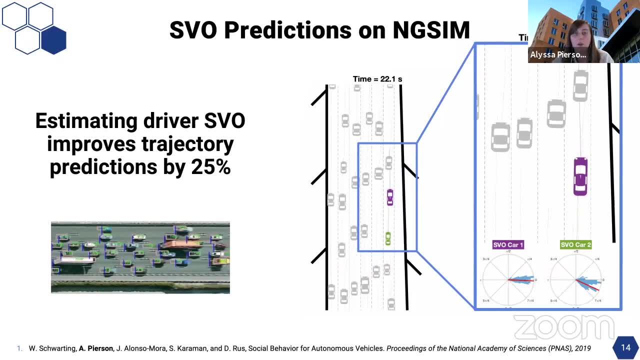 actually to allow room for that merge to happen, becomes a little bit more prosocial, allows the purple car to slide in, before then becoming more egoistic in preference and closing that gap for any other cars. And overall, as we look at trends in the data set, 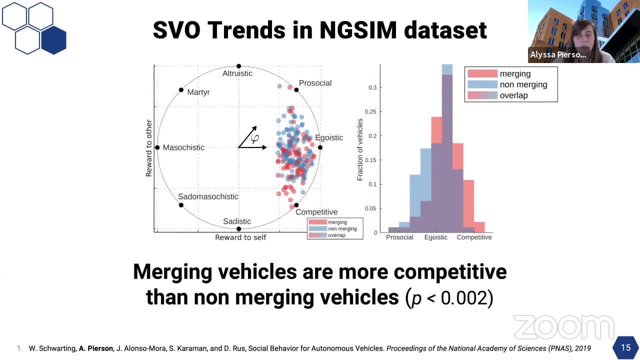 we found that merging vehicles are more competitive than non-merging vehicles, which is a nice result, because this is an intuitive explanation- and sort of what we as human drivers would expect- that to make a merge in dense traffic, you need to be a little bit. 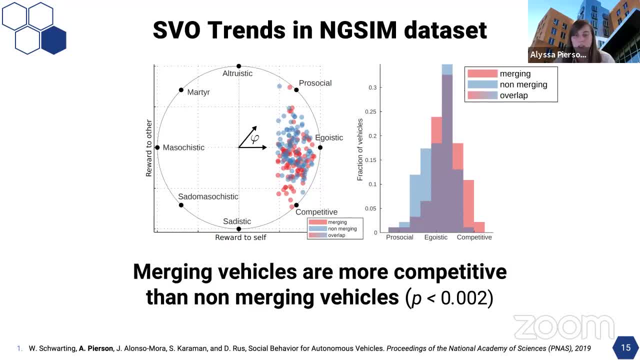 competitive to actually nudge in and change lanes. And so now I'm going to talk a little bit more about the underlying model and how we can then take this behavioral model and apply it to autonomous driving. So what we're going to do is define the 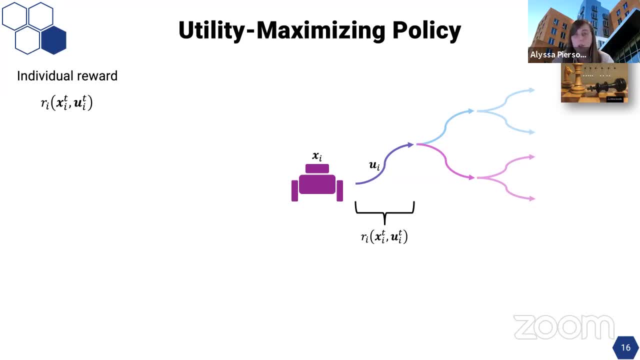 system and define all the agents of the system as having utility maximizing policies. So, going back to dynamic programming and optimal control, what a utility maximizing policy says that every agent in the system has some individual reward it can get for any action that it can take, And over time. 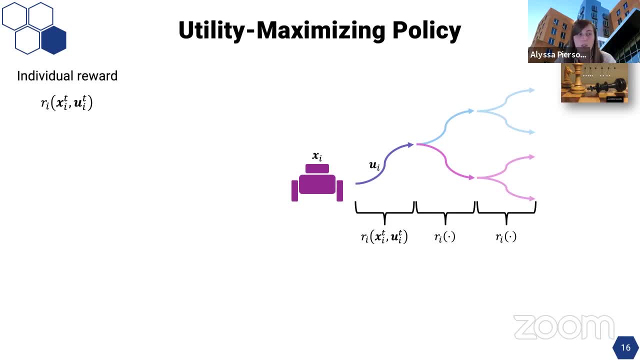 it's going to make a series of actions and collect a series of rewards, And so that utility is going to be that summation of all those rewards over some time horizon, that it's making decisions And we can look forward in time and we can find the control policy that 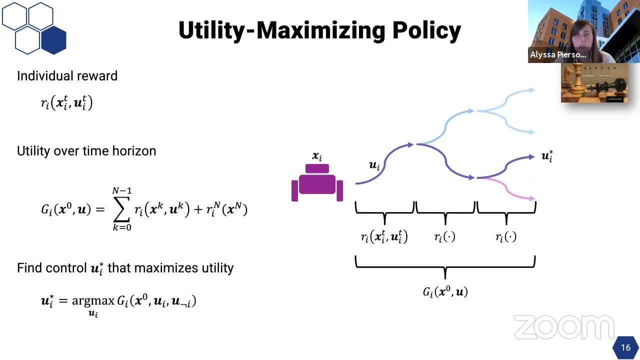 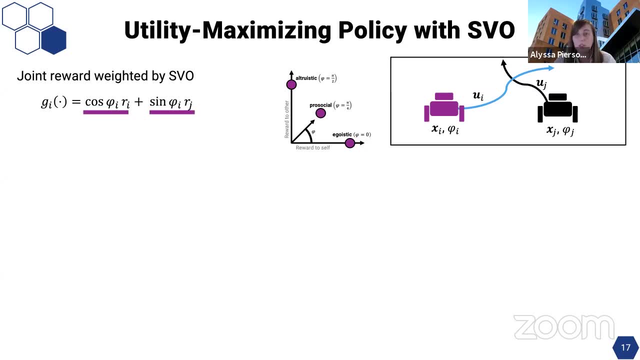 maximizes those rewards over that time horizon. Now, how do we integrate SVO into this? Well, instead of looking at individual rewards, we're going to look at a joint reward policy weighted by SVO. So instead of using just the single reward in the policy, we're going to assume that it's. 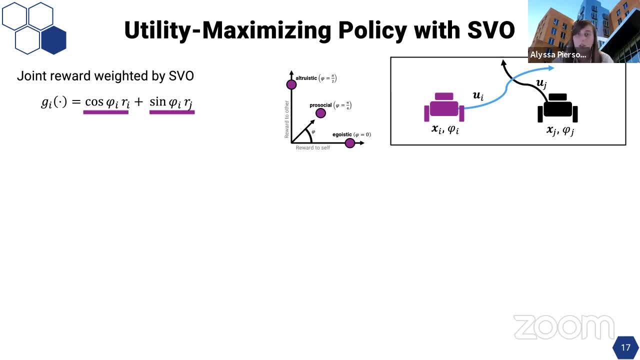 going to the single reward in the policy and the cones over the Caucasusâm, that the agents also have some awareness of how the other agents might act or be rewarded in the system, And we can still look at that utility over the time horizon And so sum up all those rewards again. 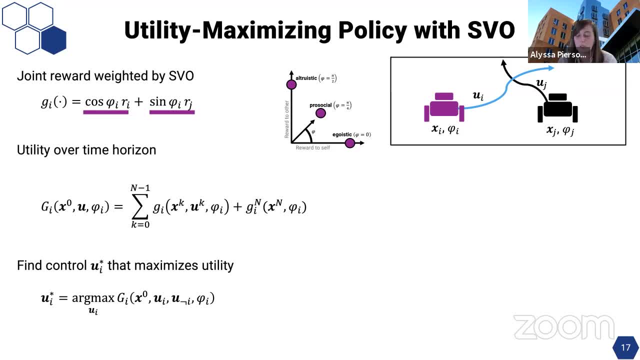 But here that individual maximization policy, individually maximizing policy- is going to be dependent upon an individual's SVO preference and how much they care about the reward that other agents are getting relative to the royalties they deserve, reward that they're getting. And so an egoistic agent which would have that SVO preference of 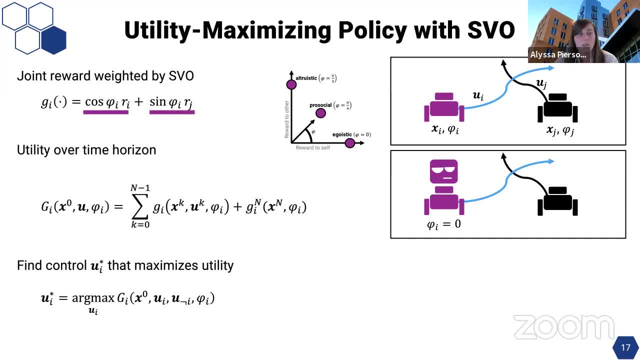 zero angle is effectively going to be the same as an individualistic agent. It's not going to account for the other agent's reward at all in its decision making, And so its optimal control path might not change when other agents are in the system. So if there's a point of potential, 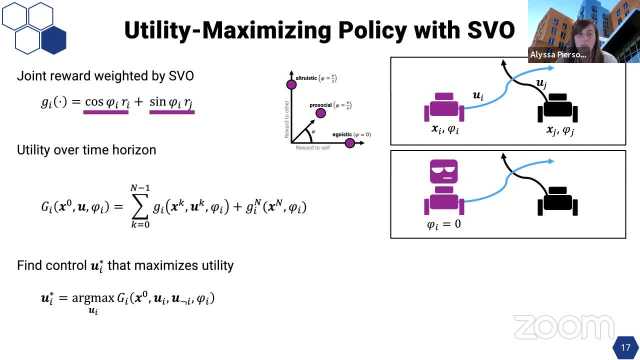 conflict down the road it may choose to not yield because it doesn't want to slow down or take any decrease of reward for this other agent. But that altruistic agent is, on the other hand, going to account only for the reward of the other agent. So in this little cartoon, 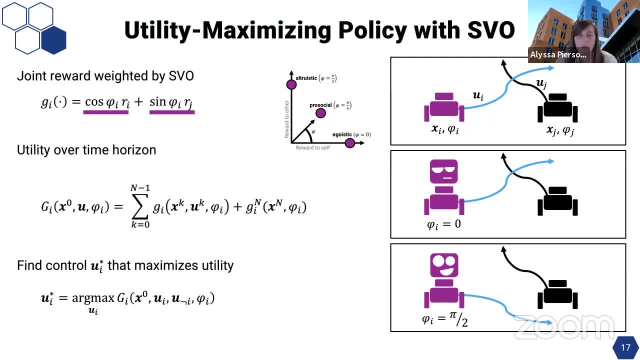 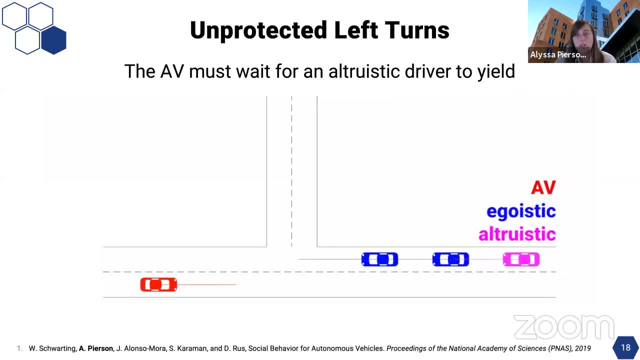 once it predicts that another agent might want to go the same way it wants to go, it may completely change its path, And so we can apply this policy to the other agent, And so we can apply this policy to the other agent For an autonomous vehicle making a left turn here in some simulations, And what we see is that 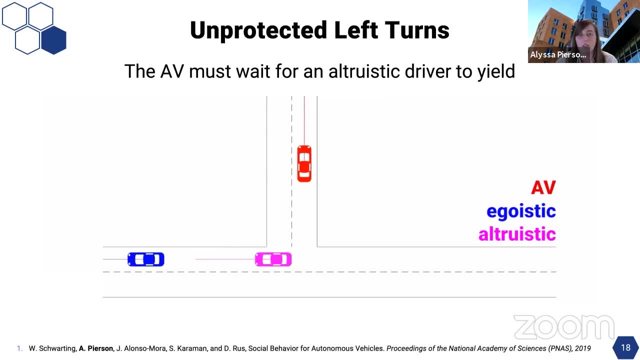 this vehicle is predicting the SVOs of the other cars oncoming- And we've got two egoistic cars in blue followed by an altruistic car in pink- And by predicting the SVO of those egoistic cars, it's predicting that those cars are not going to slow down and take any decrease of reward. 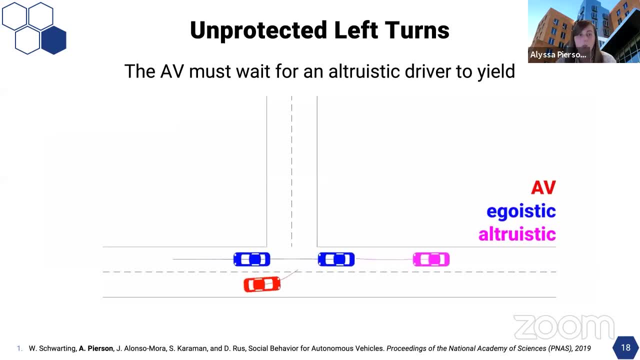 for it to make that turn, whereas that altruistic car is going to make that turn. And why we think this is really exciting is that now we see that the altruistic car is slowing down just enough to make a wide enough gap for that car. So that altruistic car knows that the AV 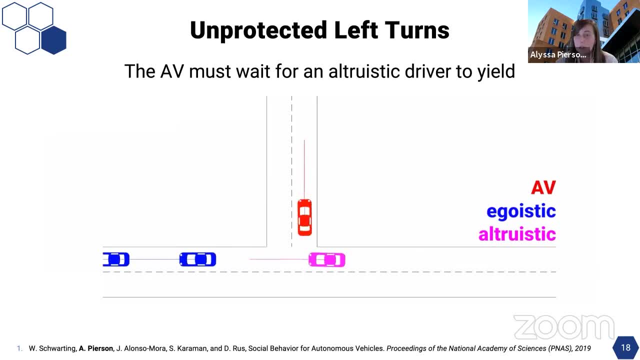 autonomous vehicle wants to make the left turn And it doesn't completely stop, It doesn't freeze, but it slows down just enough to make a gap. And the autonomous vehicle, by using this SVO model, is equipped with just enough decision-making to recognize that the SVO is going to slow down. 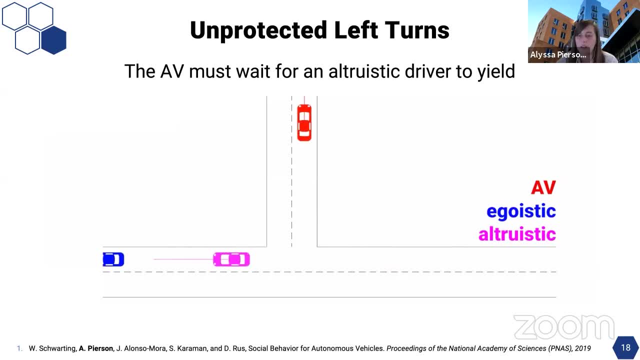 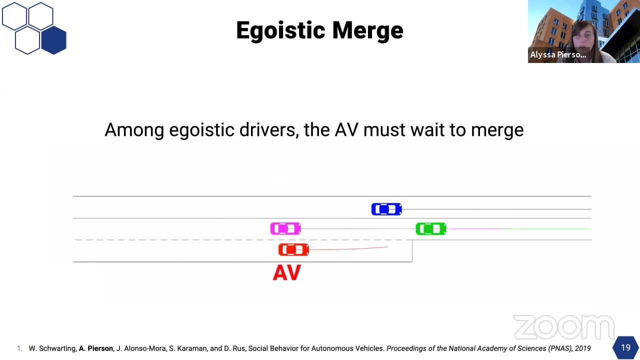 and recognize that small social cue and make that turn. Similarly, we can look at this in merging scenarios, where if the autonomous vehicle is trying to merge- and it's all egoistic drivers- it will need to wait until the other cars pass to merge into a lane. 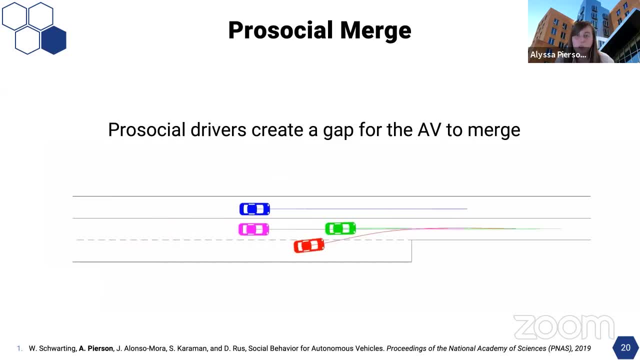 When we have pro-social cars. these pro-social cars will first create a gap for the autonomous vehicle And the autonomous vehicle, by predicting that these cars are pro-social, will recognize that cue and make that turn. And if the autonomous vehicle is trying to merge, 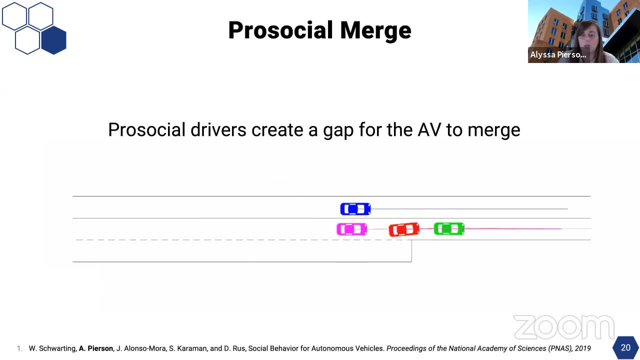 it will need to wait until the other cars pass through the lane, And if the autonomous vehicle is trying to merge, it will need to wait until the other cars pass through the lane, And so these are some of the ways in which we're thinking about how to apply social value orientation. 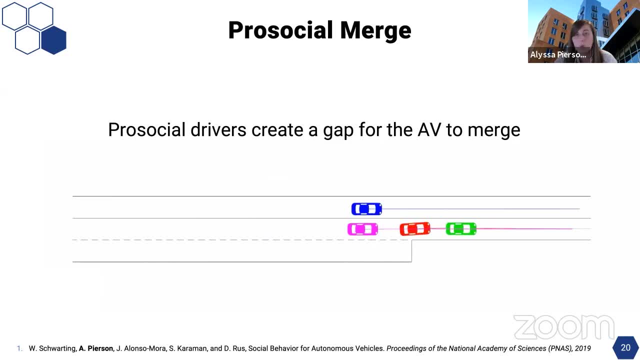 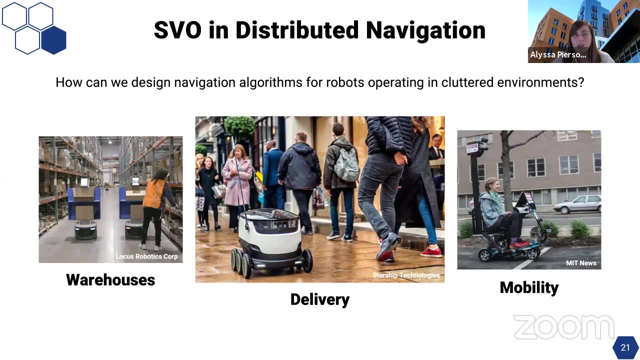 to autonomous driving. But there's a lot more to autonomous navigation than just these merges and turns. And another area we're looking at is how do we look at SVO more generally in distributed and cluttered navigation. So now we're looking a little bit more broadly at applications like 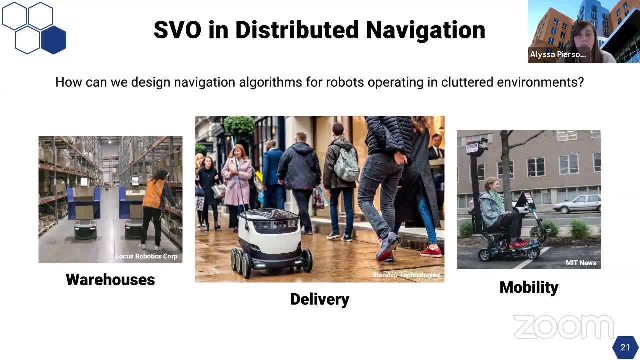 delivery drones, warehouse robotics and personal mobility robots, where you're going to be operating in more cluttered environments, less structure and having far more interactions with a group. Is there a way that we can still take some of these tools from social psychology and 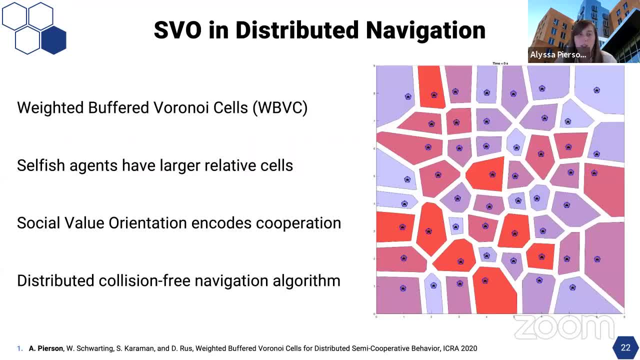 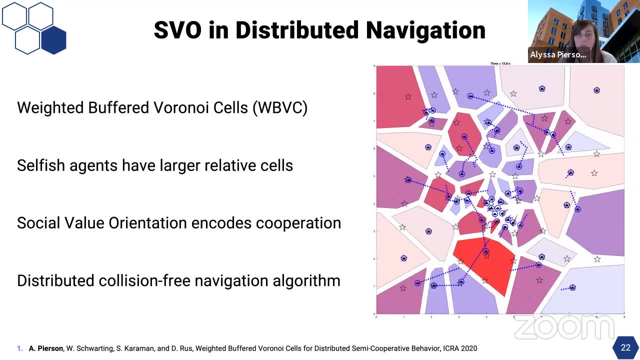 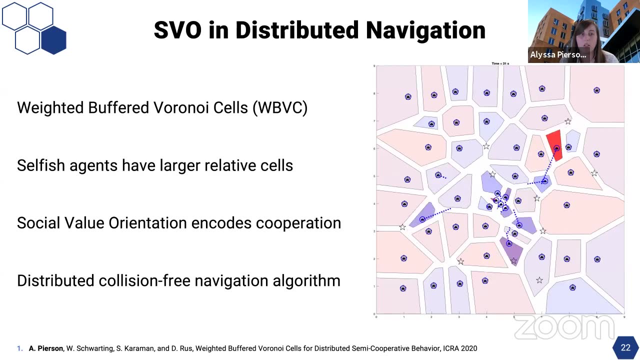 apply them into this navigation, And so what we propose is that we can fundamentally encode some of these cooperation practices, And so we're looking at how do we look at SVO more generally in the context of this navigation. So I'm going to take each of these two references into a geometric encoding by creating 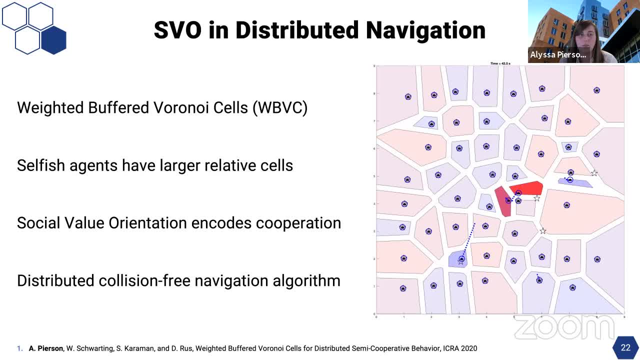 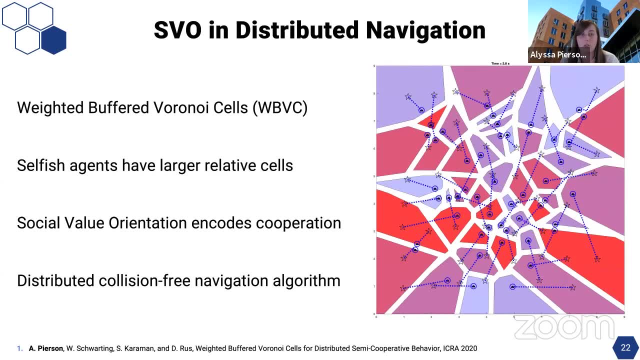 this weighted, buffered Voronoi cell And with this geometric encoding we define that selfish agents will have larger relative cells and, conversely, the more altruistic agents will have lower relative cells. And so when agents are moving throughout a space and trying to predict what 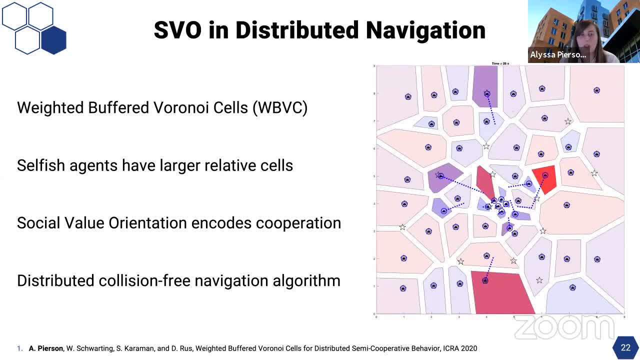 is a safe region to maneuver to. these slight social preferences will be enough to diversify that into more orderly relationships. So if I look at a person's name and they have a certain type of yield- the semi-cooperative, selfish versus non-selfish behavior- And so now I'll talk a. 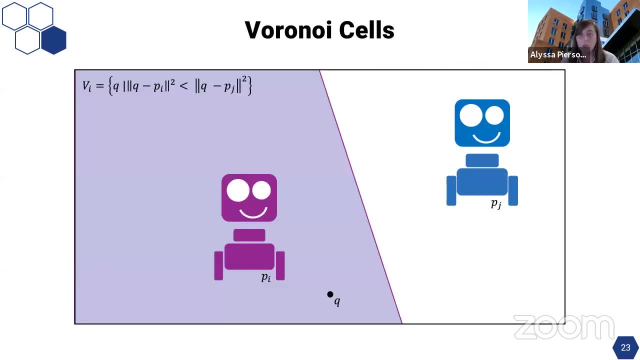 little bit more about what that means. So for a brief introduction, for those that don't know, a Voronoi cell is defined at all points Q within a cell that are closer to a robot PI in purple than a robot PJ. So here I've shaded the Voronoi cell of the purple agent and you can see that. 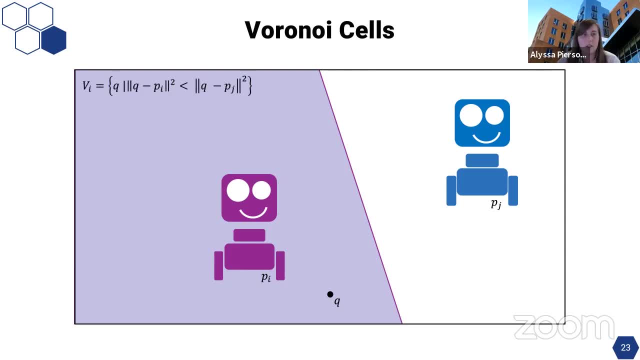 there's this nice geometric decomposition of space. And then, a few years back actually, some of my former colleagues out of Max Schwager's lab started looking at this idea of a buffered Voronoi cell. And we can think of buffered Voronoi cells as social distancing for robots And so what. 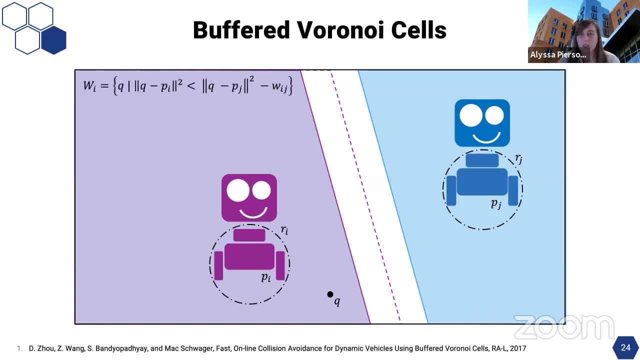 buffered Voronoi cells do is they add a weighting factor into the definition of the Voronoi cell. So now the cell is defined, It is all points in the cell closer to a robot accounting for this weighting factor. that creates a gap between the different cells And this creates a safety radius So that weighting is. 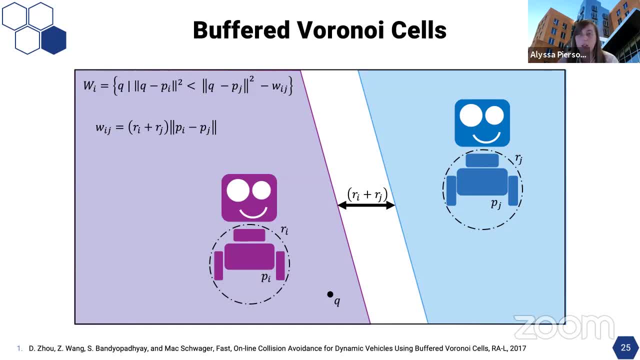 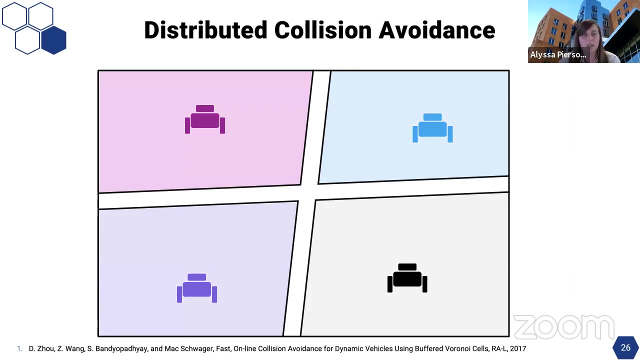 defined by the radius of the robots, to guarantee that wherever those robots are within their cell, they're not going to collide with any other robots in the space. And this is common in distributed collision avoidance, where we can look at robots and say, okay. 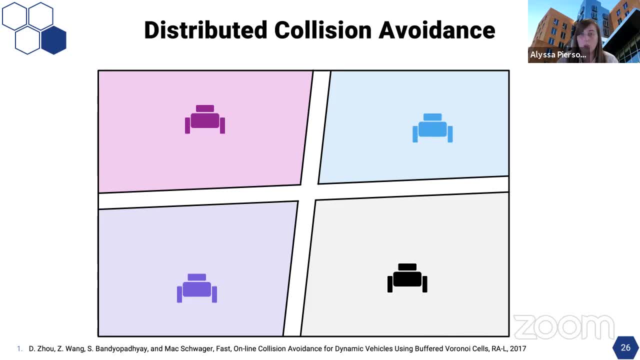 go out of the area of the environment and start planning paths within your cell. And if you always plan actions within your cell and everyone else plans to also stay within their Voronoi cell, you get these nice collision avoidance guarantees as the agents move throughout the space while 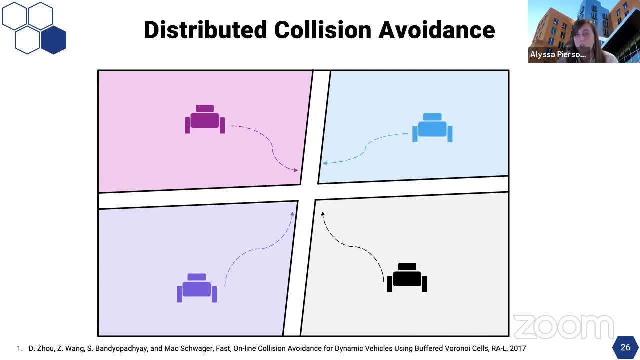 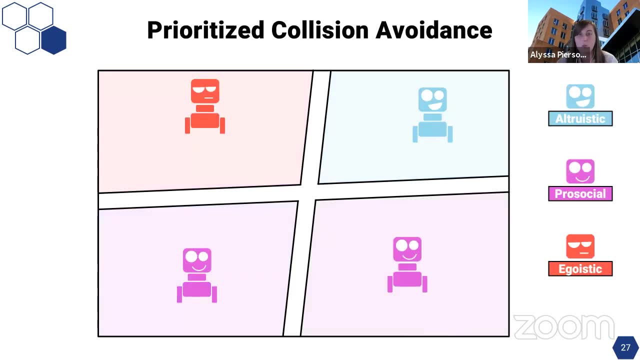 still maintaining distributed behavior, because agents are only using local information to make these decisions. And so when we looked at this, we'd like to say, okay, well, is there a way to have prioritized collision avoidance? And we can look at this, and we can look at this, and we can. 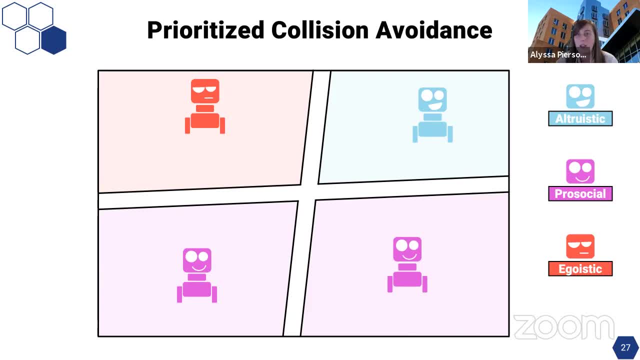 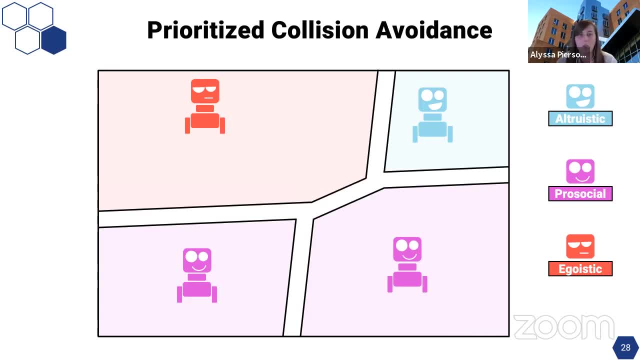 How can we modify these boundaries to account for an egoistic agent wanting a larger portion of the environment? And here that larger portion of the environment means it has a priority to navigate to points in that environment. And so what we're going to do is we're going to look at the 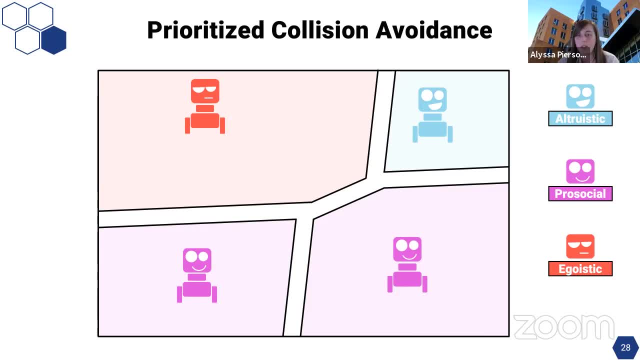 same notion of SVO to create these asymmetric cell weights that give these larger relative cells to the selfish agents while still maintaining the same sorts of collision avoidance guarantees generated from the original buffered Voronoi cell work. And so when we say that there's relative 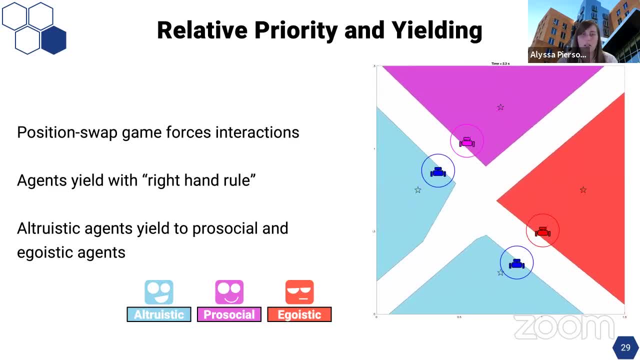 priority in yielding. what we're looking at underlying here is we're going to start looking at a positional order, And so what we're going to do is we're going to start looking at a positional order. And so what we're going to do is we're going to start looking at a positional order And we look at a position swap game. And we look at a position swap game where agents pick another agent in the environment and they have to swap initial and final positions, And we do this because it forces a lot of interactions, So the agents are going to need to move in close proximity to other agents as they navigate around. And, underlying this, each agent is going to try to drive as close to its goal as it can, while staying within its cell. And when it gets to the edge of its cell and can't go any further, it's going to expect that the agent is going to be able to move in close proximity to other agents as they navigate around. And, underlying this, each agent is going to try to drive as close to its goal as it can, while staying within its cell, And when it gets to the edge of its cell and can't go any further, it's going to expect that the agent is going to be able to move in close proximity to other. 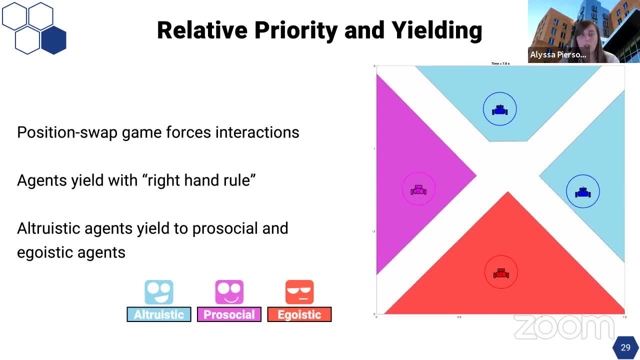 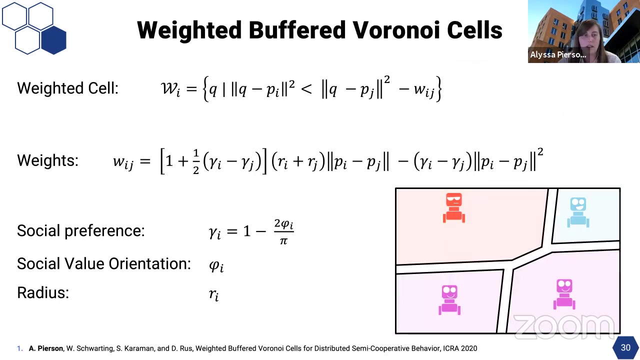 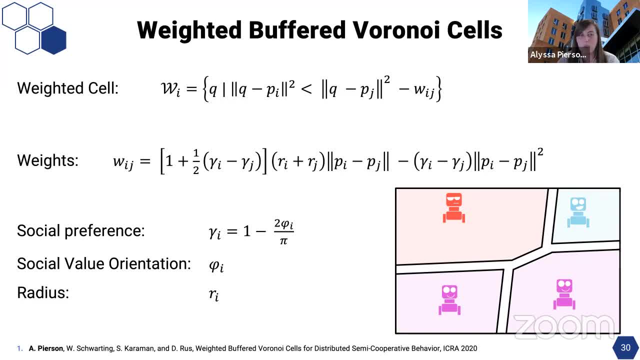 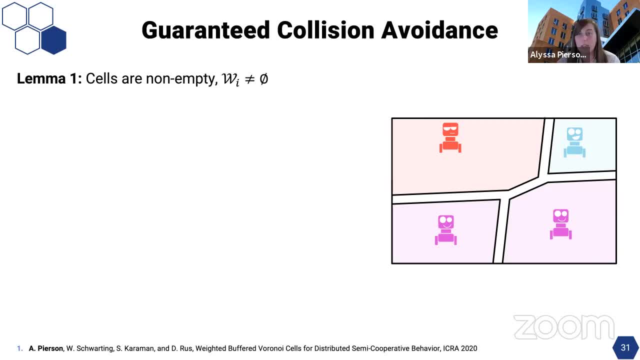 So one property of these cells is that they're non-empty. So the agent will always have at least its own position within the cell. The minimum distance between any two points in any two cells is greater than the radius of each of those robots, And the cells are not overlapping. So if a point belongs in one agent's voronoi cell, it's not going to be in any other agent's cell. 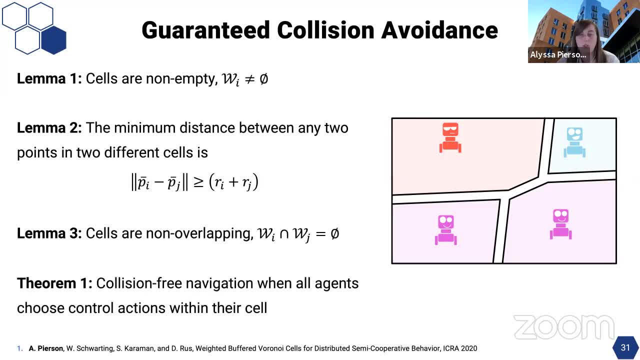 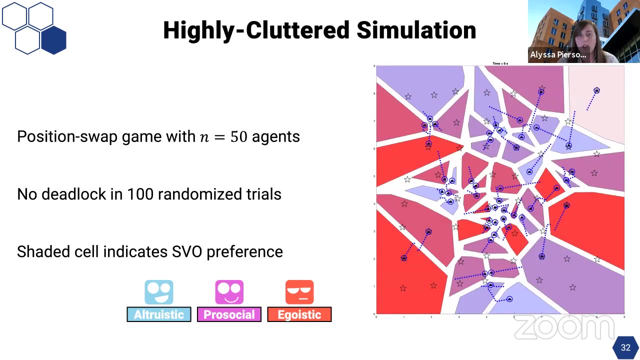 And so if agents choose to navigate two points within their cell, then that's how we can guarantee this collision-free navigation overall in a nice, clean way, where we're only looking at collision avoidance through geometric methods for defining the region. And what's nice about using these local geometric decisions is that it scales quickly to many agents. 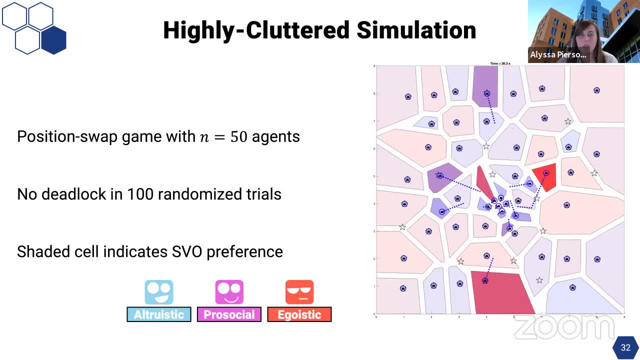 And we can have, And we can have highly cluttered environments where you're not worried about. you know each agent only needs local information to make its decisions And so you're not worried about kind of slowing down by trying to optimize for all these agents. 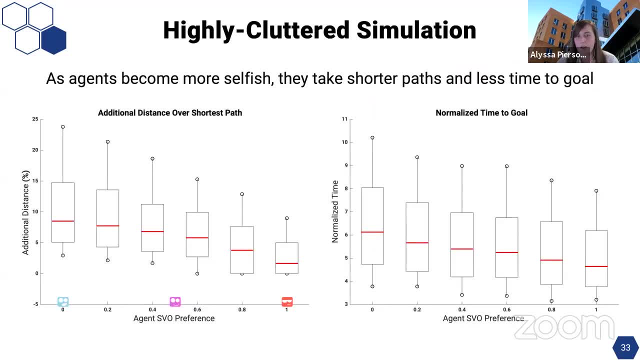 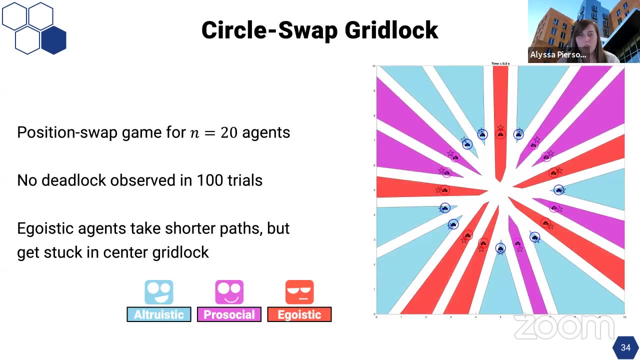 And I'll just quickly say that our results showed that indeed we wanted the selfish agents to take shorter paths and shorter times, And indeed that's what we saw, is that as agents become more selfish, they do take shorter paths. But what was sort of interesting is we also looked at a very particular case of the position swap game, which is called the circle swap. 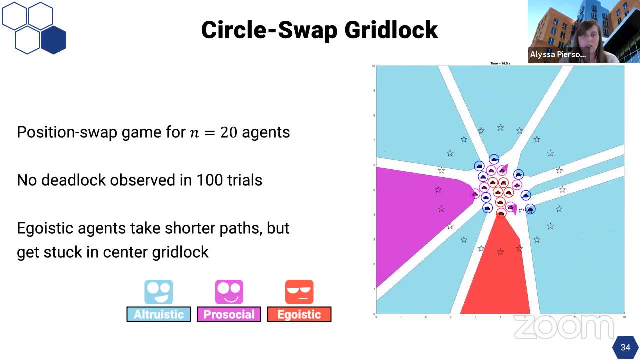 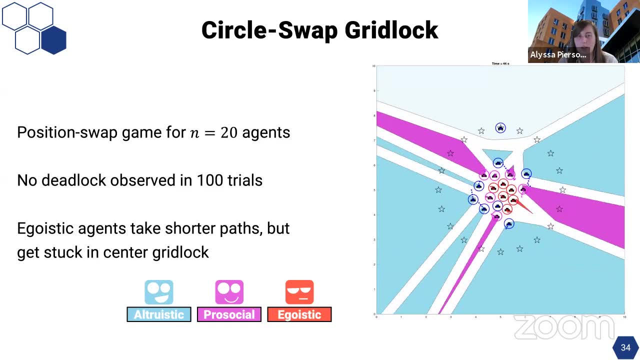 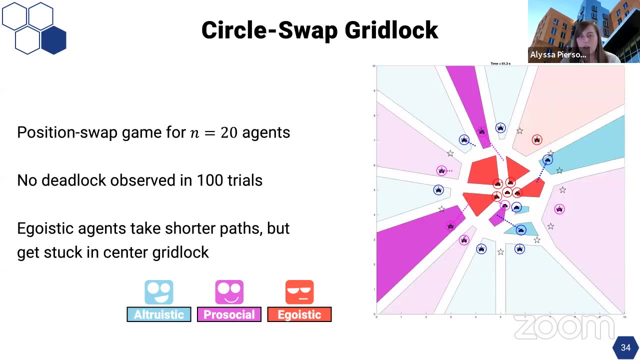 And it's thought of as in the multi-robot literature. it's the one where you have the most interactions, because agents are pretty much all needing to cross at the center of the circle to get around, And here what we found sort of interesting is that the egoistic agents still take shorter paths. 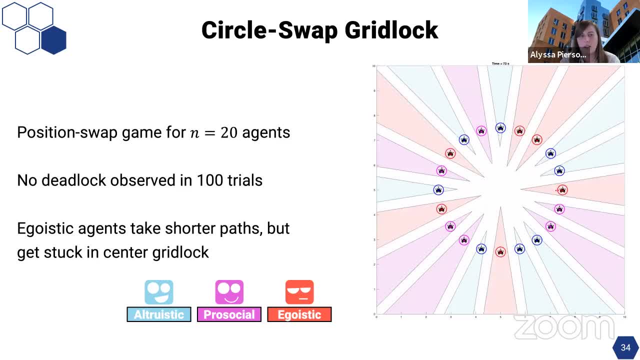 But they don't get to their goals first, And it's because that kind of rush to go forward and rush to go quicker through the environment actually ends up getting them stuck in gridlock and getting them kind of frozen in the center until the more altruistic and pro-social agents can move around. 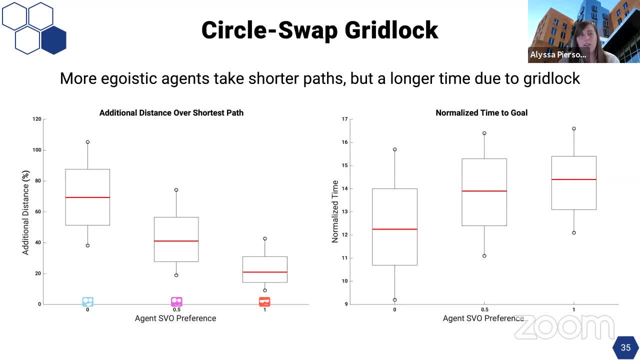 And so, unlike the last example, even though they're still taking shorter paths, they're actually spending more time getting to the goal because they're stuck in gridlock. And so those are a few ways we're thinking about how we can integrate social value orientation into this socially aware planning. 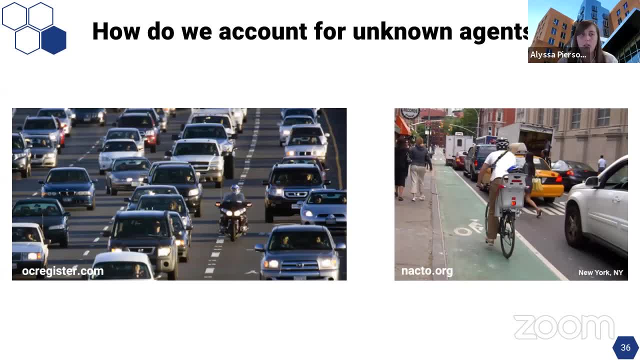 And for the last few minutes, I'd like to also talk about the other side of it, the risk aware planning. So a big question is: well, how do we account for these unknown agents And really, how do we build safety nets when we're talking about operating in highly cluttered, highly dynamic environments? 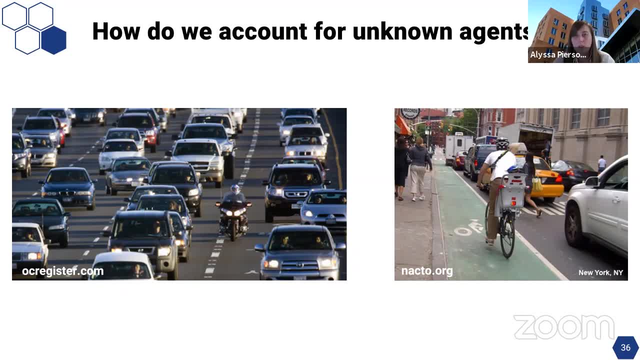 So how do we account for density, That's, freeway traffic as well- as how do we seamlessly go into urban environments where you have people jaywalking, cars parked illegally in lanes, bicycles, pedestrians and all these dynamic, rich things going on? 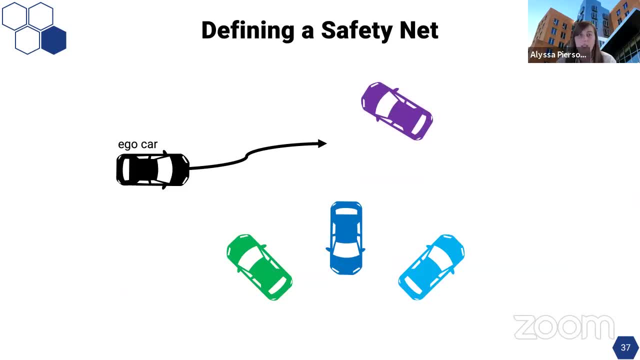 And, ultimately, we'd like to think about how we can define a safety net for these cars, And one way we might think about defining a safety net is: you might say, OK, well, I've got the car and I've got all these other agents throughout. 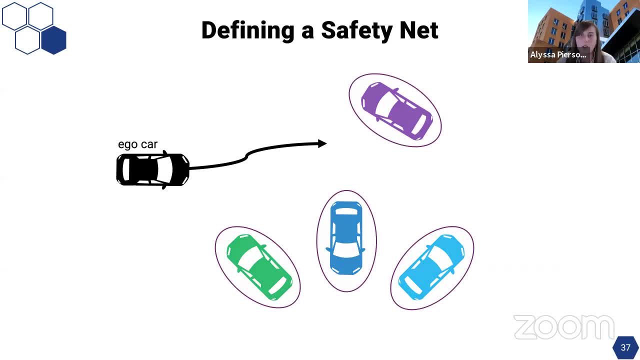 I've got the environment and maybe I'll just kind of create a padding. I'll create an unknown that represents some uncertainty I have, And the more uncertain you are and the more agents suddenly you start to over, constrain your environment and you can end up where the ego vehicle now no longer can find a path through those cluttered environments. 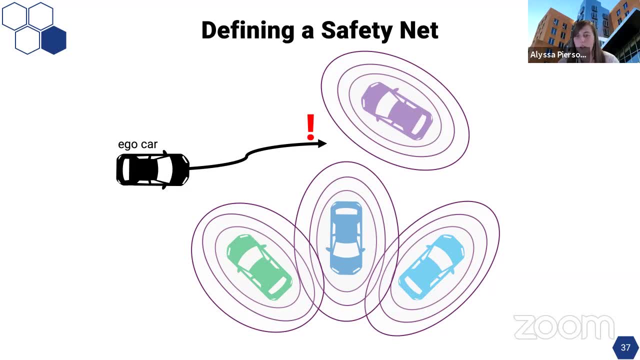 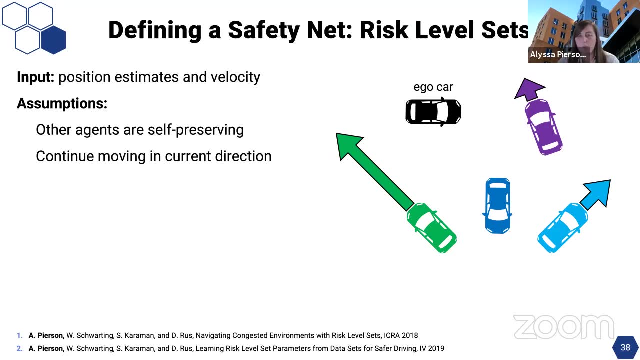 And so instead we'd like to think of a safety net in a slightly different way, And we think of it as now. let's say, We know just there, We know both their positions, but we also know something about their current velocity and we assume that they're kind of going to continue in that direction. you know for the next, you know immediate kind of time step or action. 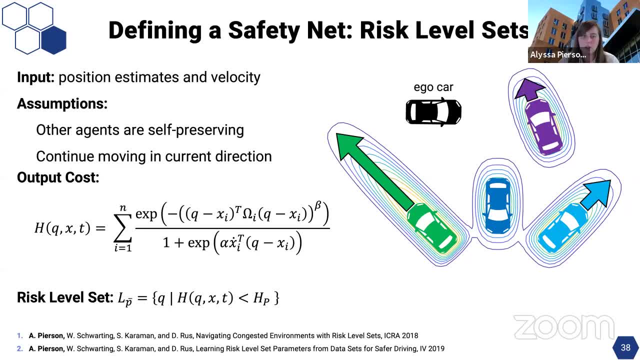 Well then, we can create this kind of congestion cost function that takes those position estimates and skews them by the direction of their velocity, And so, instead of having these kind of radially symmetrically converging, Constrained safety nets, We now have these skewed safety nets that we're going to call. 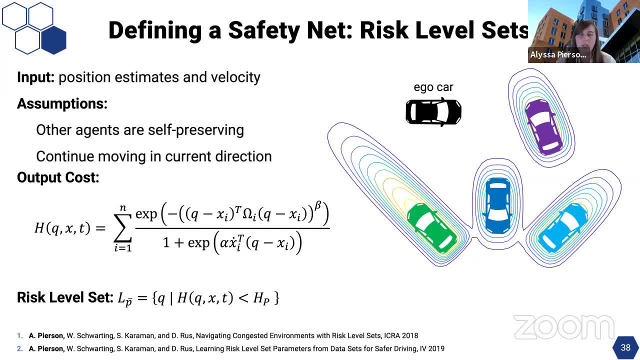 You know these, these different, different level sets, and depending on how conservative or aggressive you may want to be, We can choose a level set of of that cost function and we call it a risk level set, as that's a value of our threshold of the cost function. 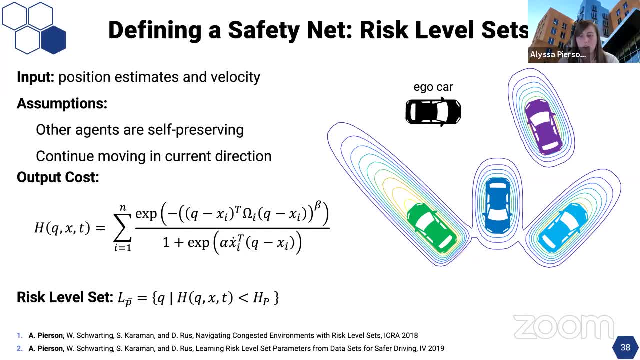 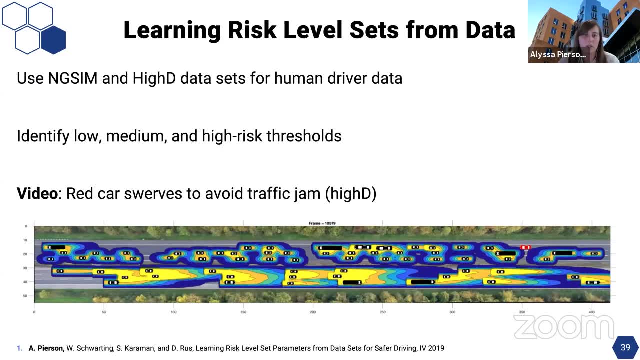 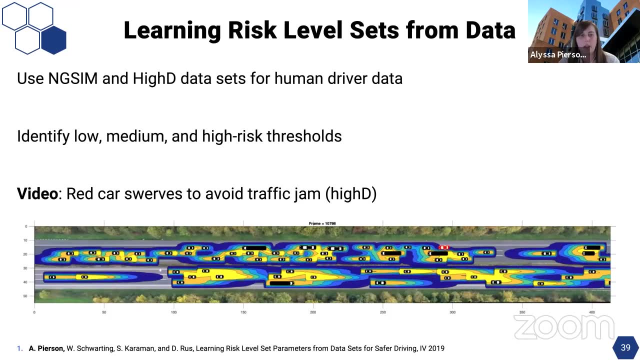 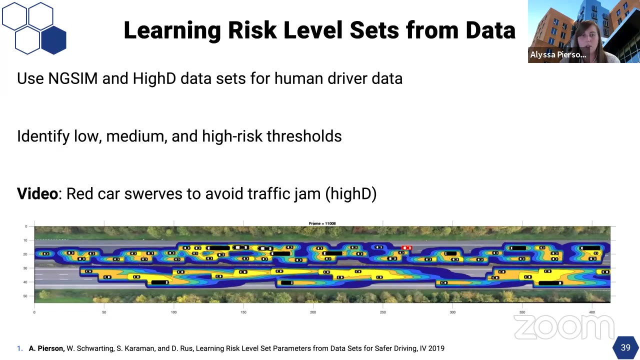 To kind of define your conservativeness or aggressiveness, And how we've looked at these Is We. we think they're extremely useful in a couple ways, And one is that we can use them to observe Human driver data and by quickly calculating these risk level sets we can start to understand some of the underlying distributions, or what are some of these risk tolerances. 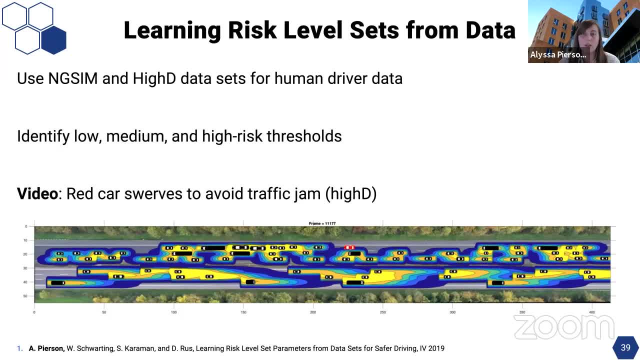 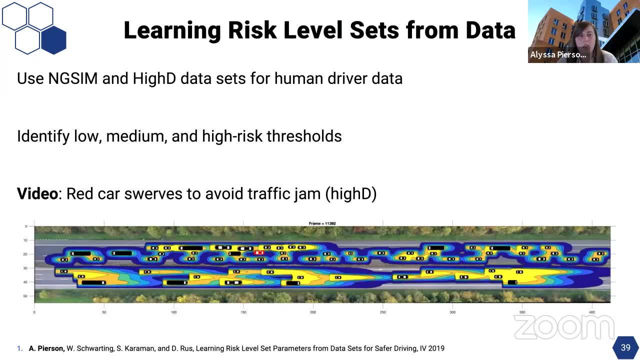 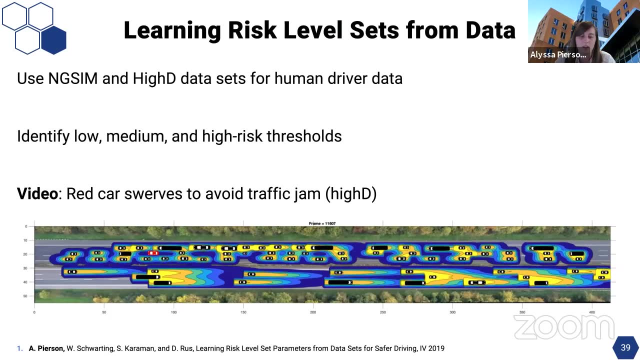 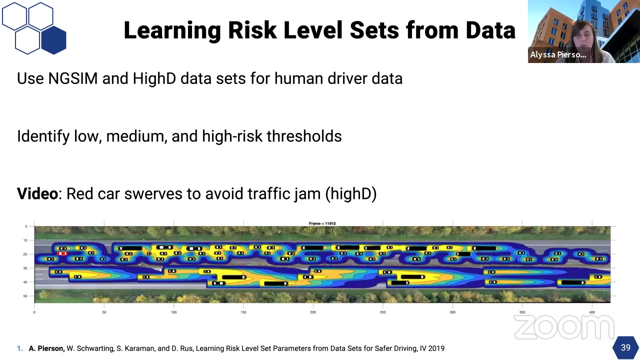 That human drivers have and, furthermore, if we can identify what it means to be low, medium or high risk, We can then also quickly parse These data sets and find examples of cars doing evasive maneuvers, doing these sort of, You know, edge case behaviors that would be hard to necessarily just pick out of a data set if you didn't have some way to quickly, quickly understand it. 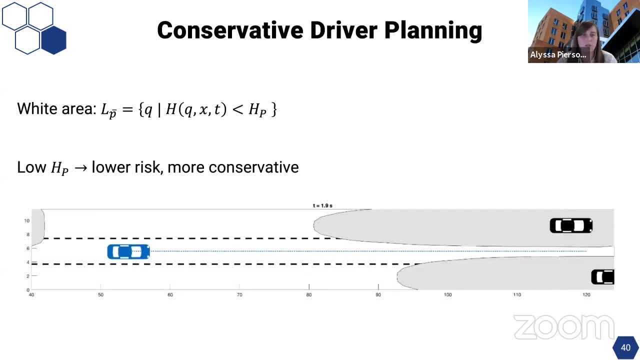 And then we can also take these level sets and we can start to apply them to autonomous vehicle planning, And so we can look at what maybe a low risk car looks like Where it takes it only plans actions within this low risk threshold that it's calculating around these other vehicles. 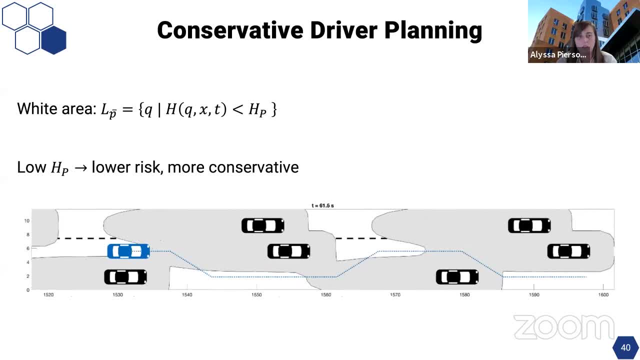 And what we see is, if you have a lower risk, then you're going to be a lot more conservative. So here the gray regions indicate all the areas seen as too risky for the car to navigate, And so it keeps its distance from the other cars. It maybe makes a lane change, but doesn't really do a lot of other types of actions. 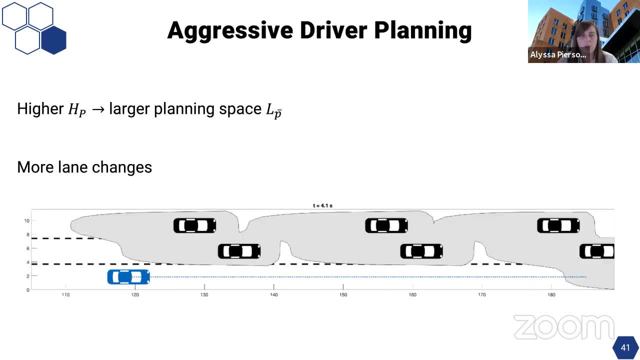 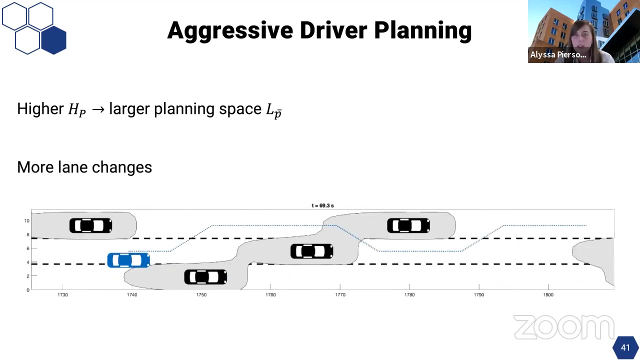 Whereas if we start to increase that risk Threshold- now those gray regions, that kind of restricted planning space gets a lot smaller and we see a lot more aggressive behavior emerge. We see more lane changes and we see more, More of the car moving up against other cars, And so we think this is a useful tool in creating sort of a safety net for both modeling and predicting what other cars might do. It's not a complete solution. 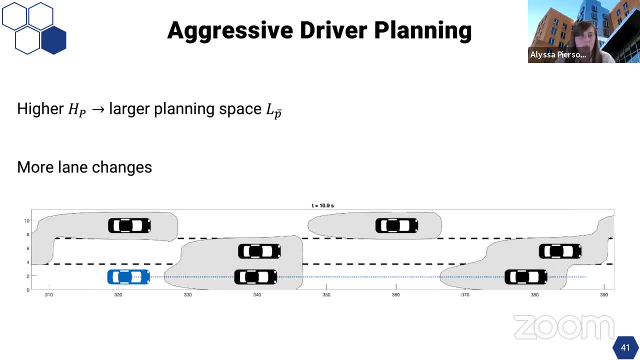 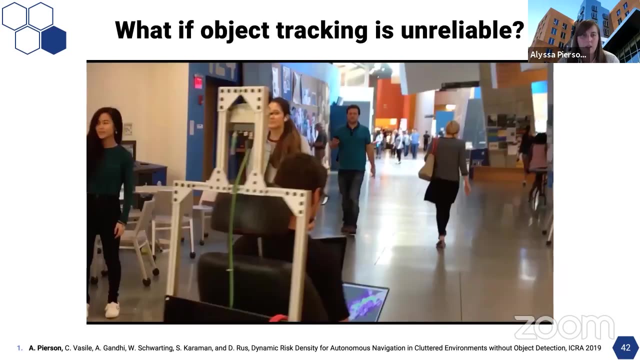 The behavioral model, but really, as I said, it's kind of one one piece in how we might account for the behavior of other agents. and When we thought about this we thought: well, knowing positions of velocities is a pretty small requirement, but let's make it harder for ourselves. What if we don't even have reliable object tracking? So what happens if we don't have reliable position tracking and velocity estimates? 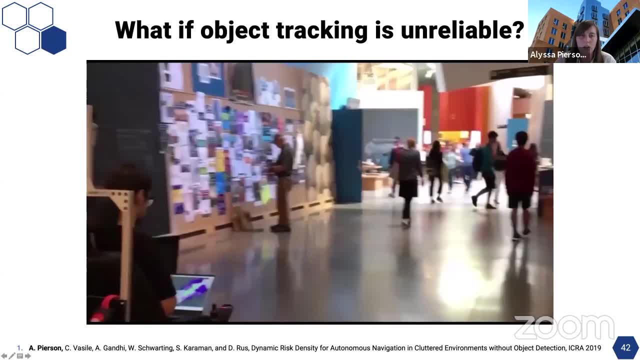 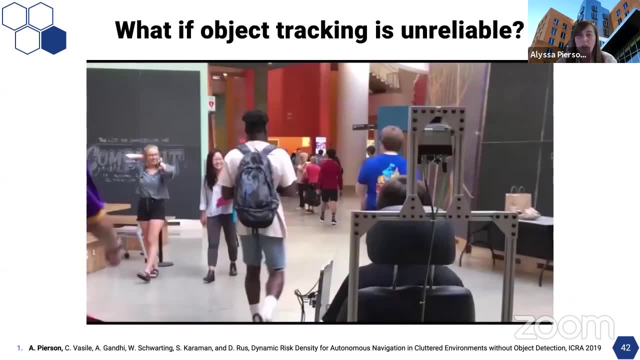 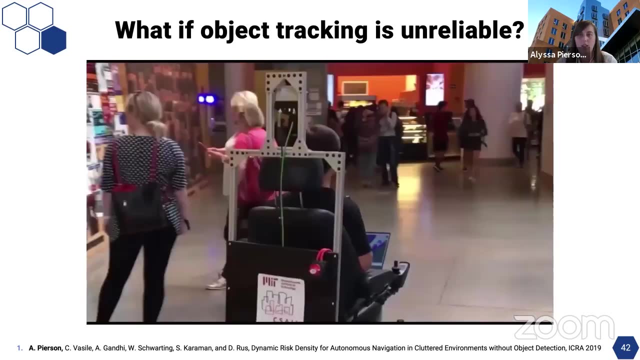 And so What we looked at here is: we looked specifically at our autonomous wheelchair platform as a proxy for a vehicle interacting with pedestrians in an environment, and What we're looking at is: can we have this robot navigate in cluttered environments and can it operate around unknown humans and static and dynamic objects? 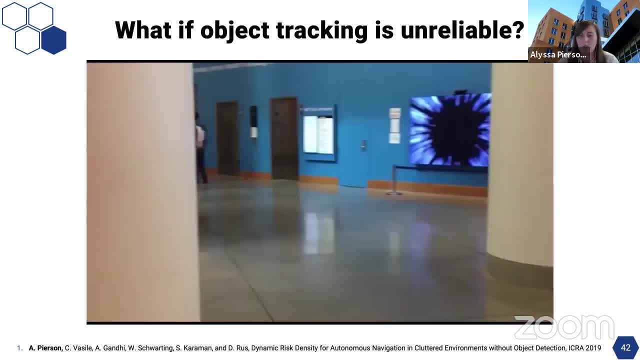 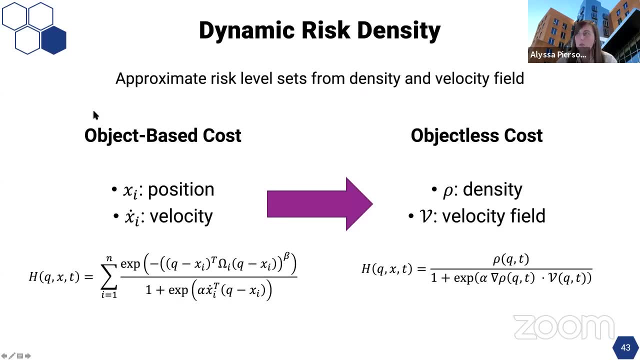 While still maintaining safe navigation and keeping the passenger safe. And so, to do this, we looked at our similar cost formulation, but instead transformed it into what we call this object list cost variation, and what we propose is the dynamic risk density. So here, instead of having object based position and velocity, So instead of having tracked objects throughout the environment, 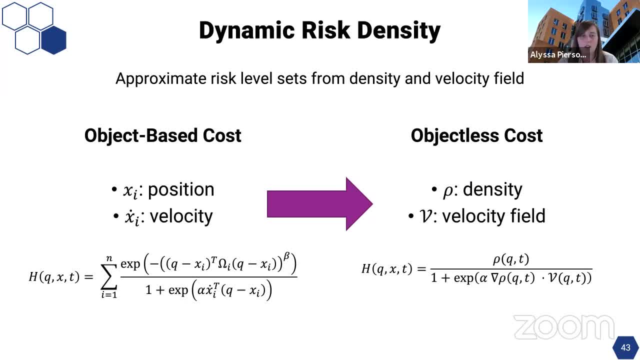 Instead, you have a density which you can get from your Lidar As well as an estimate of the velocity Field which is looking at that, how that density field evolves over time, And we can get sort of this density flow throughout the environment to estimate the risk of different actions. 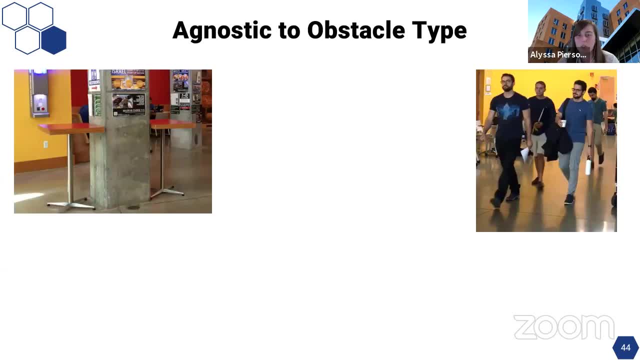 And why we're excited about this is because it the safety net becomes agnostic to the type of obstacle. It will keep the passenger safe around both these static obstacles like columns and dynamic obstacles like crowds, as well as all the random things that might fool. 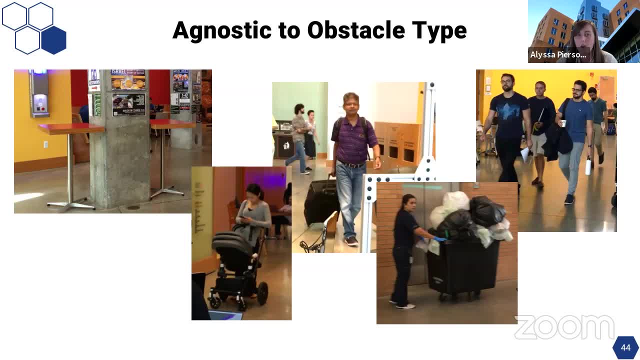 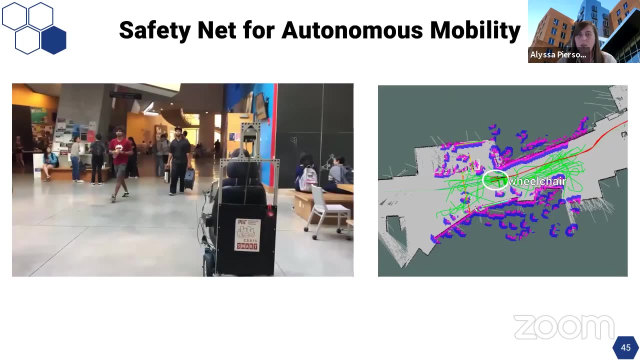 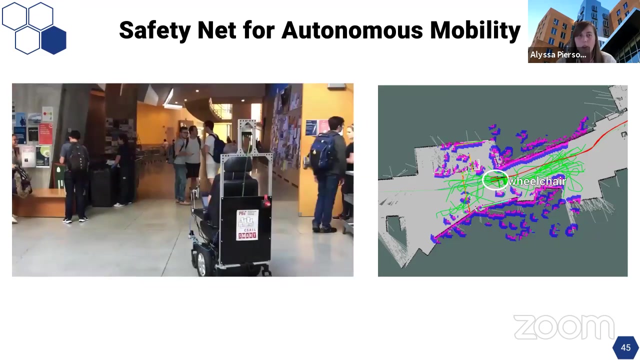 A prediction pipeline, So we don't have to worry about wondering if the person with the suitcase, because they're holding a suitcase, will no longer be detected or or missed by by our- our pipeline. And so in this way, we can think of this as a a new cost map that the robot can use and it becomes this safety net for autonomous mobility, So it's something that we can. 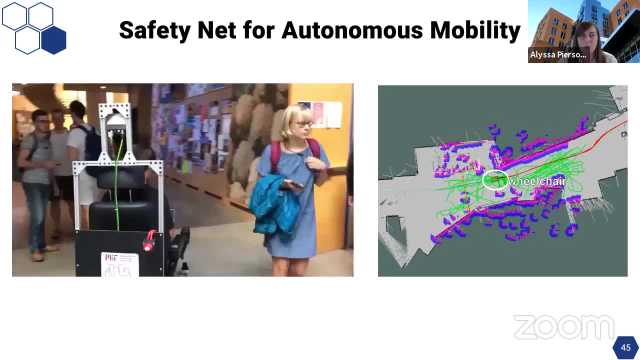 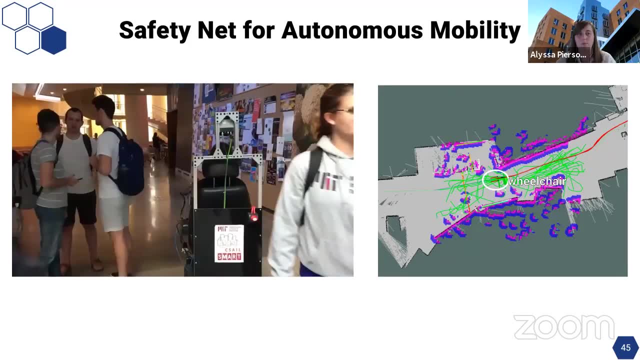 By biasing it with this velocity information, we can make it a little bit more agile. So it's something that we can. by biasing it with this velocity information, we can make it a little bit more agile. So it's something that we can. by biasing it with this velocity information, we can make it a little bit more agile around all of these unknown elements and certainly build upon with other, more complicated tool sets. 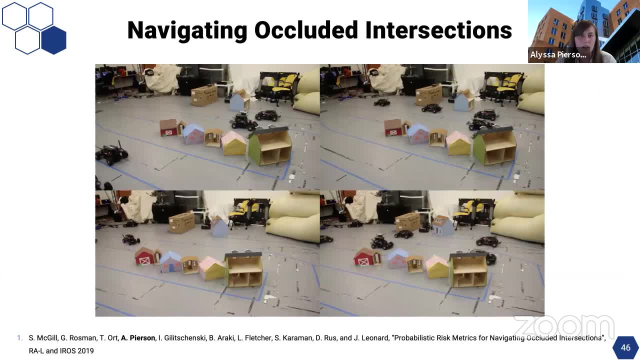 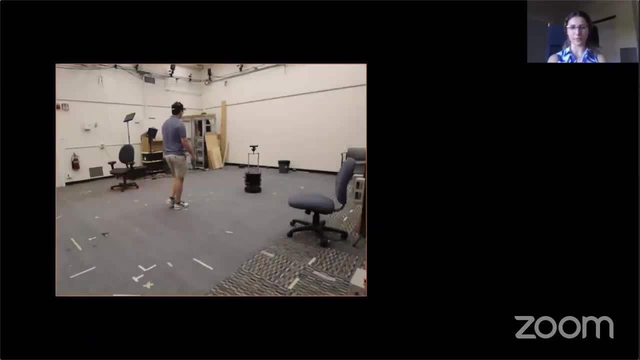 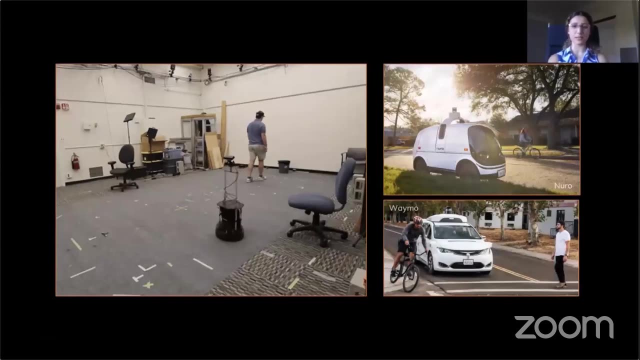 Robots are increasingly operating in close physical proximity to people. Here's an example of a pedestrian operating around a ground vehicle in my lab, but we're also seeing these robots in the wild. In scenarios like these, it's critical that autonomous vehicles are able to predict where people will move, to plan safe and efficient trajectories. 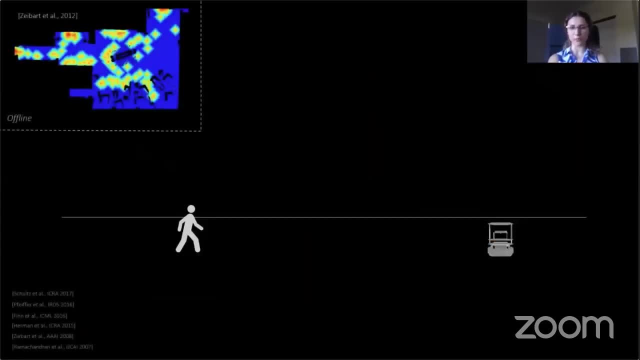 To build such predictive models of people, we can look to the increasing quantity of human data and learn models of human behavior. offline, For instance, we can use data to learn what different goals in a room a person might have, as well as how they tend to act given the intent to reach one of these goals. 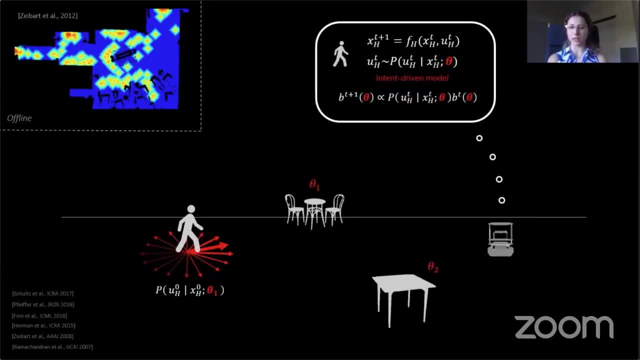 For instance, we can use data to learn what different goals in a room a person might have, as well as how they tend to act given the intent to reach one of these goals. Then the robot can use data online to infer the human's intent via Bayesian inference. 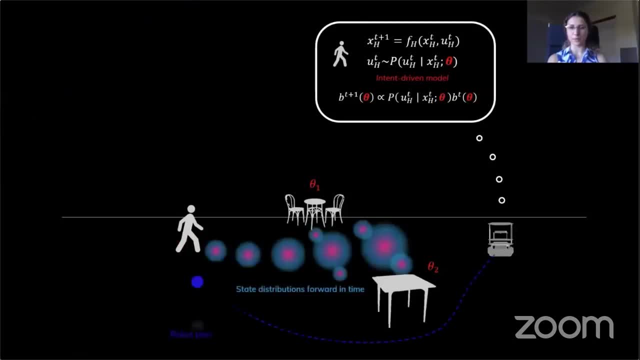 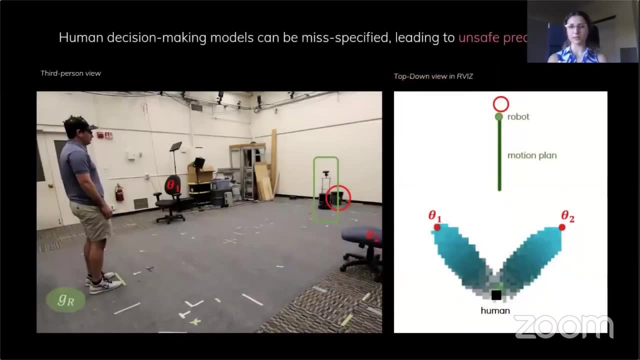 When the learned decision-making model is combined with the dynamics model, we can generate state predictions forward in time which the robot collision checks against when motion planning. Unfortunately, these learned models are not always correct. For example, here the human is walking towards a third unmodeled goal that the robot does not know about. 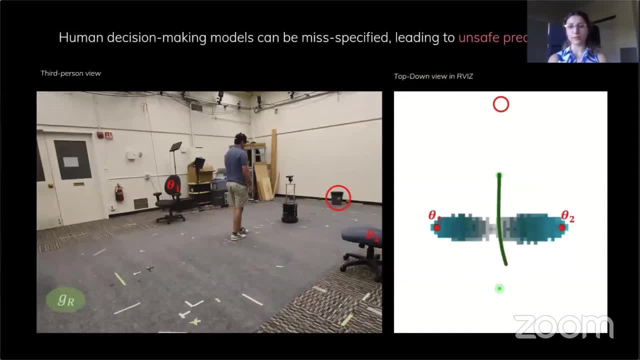 When the robot relies on this incorrect model for prediction, it cognitively plans an unsafe motion which results in a collision. When the robot relies on this incorrect model for prediction, it cognitively plans an unsafe motion which results in a collision. 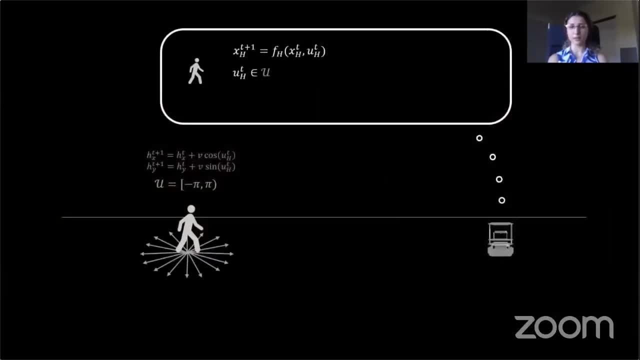 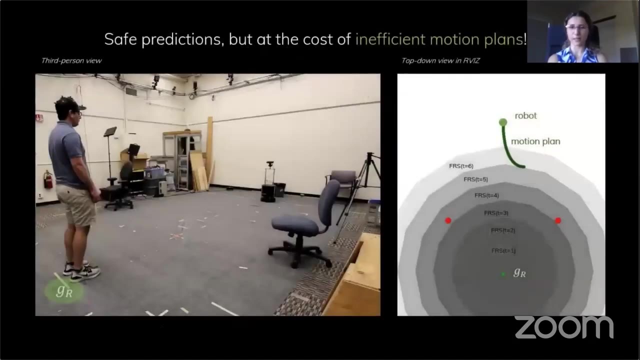 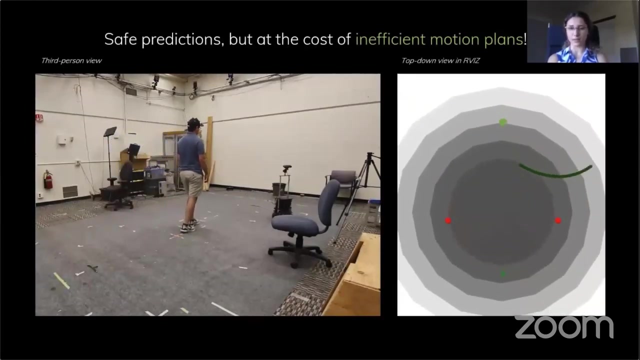 To eliminate such safety violations. conservative motion predictors from robust control theory remove the learned decision-making model entirely. Using a conservative set of human actions, these predictors safeguard against all possible human trajectories, which is formally called a forward-reachable set. While surely safe, these predictors often come at the cost of efficiency. In fact, to avoid the human here, the robot has to leave the testbed entirely. 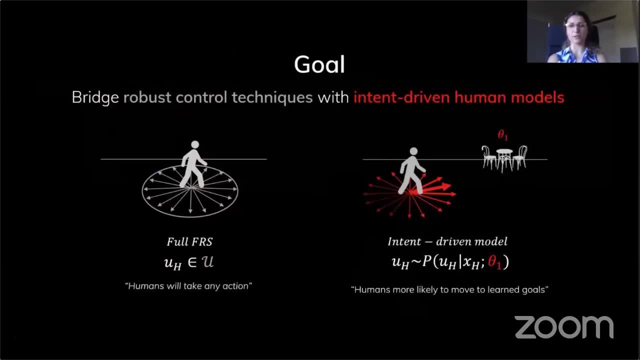 In this work we seek an approach which bridges the two. We seek an approach which bridges robust control techniques with intent-driven models to get a predictor which is more robust to misspecified human models but can still leverage the learned intent to safely reduce conservatism whenever possible. 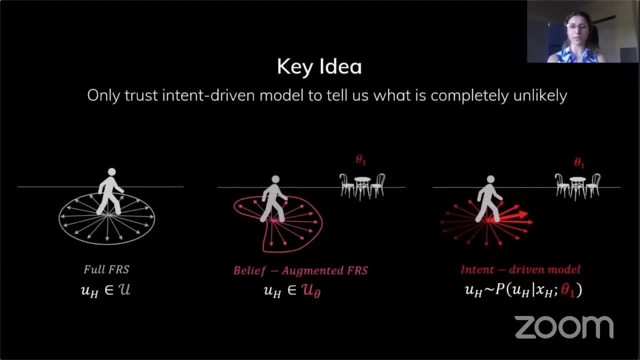 Our key idea is to trust the intent-driven model to tell us only what is completely unlikely. After using the intent-driven model to prune away sufficiently unlikely actions, our robust predictor will safeguard against all sufficiently likely actions, equally much like in the full, forward-reachable set. 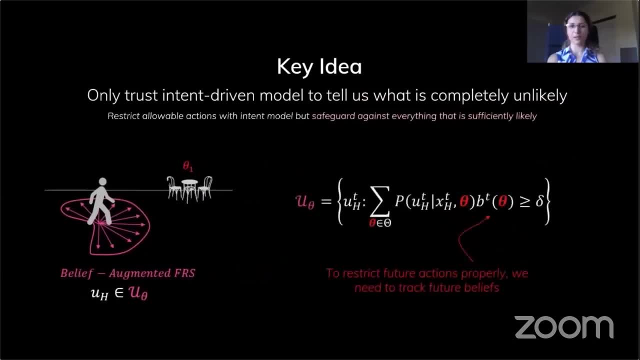 Our robust predictor will safeguard against all sufficiently likely actions, equally much like in the full forward-reachable set. To properly restrict the set of feasible human actions over the prediction horizon. we need to take into account how the likelihood of any future human actions depends on the history. 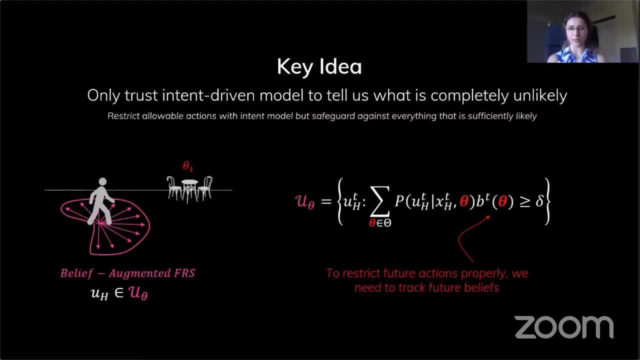 of actions. The belief precisely encodes this through the Bayesian update. Thus, our predictor explicitly tracks the updated belief as it makes predictions and safeguards against future human actions based on future beliefs In our running example, since our framework relies only on this set of likely and unlikely. 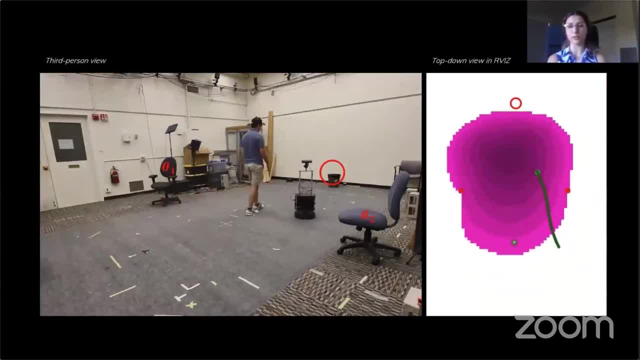 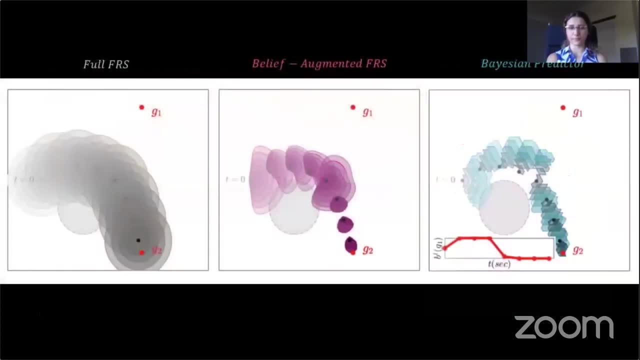 actions for predictions. it classifies the human moving straight as a sufficiently probable trajectory, enabling the robot to remain collision-free while reaching its goal. Our predictor also helps in a variety of misspecified human model scenarios, For example, when there is an unmodeled obstacle. our predictor, once again remains cautiously. 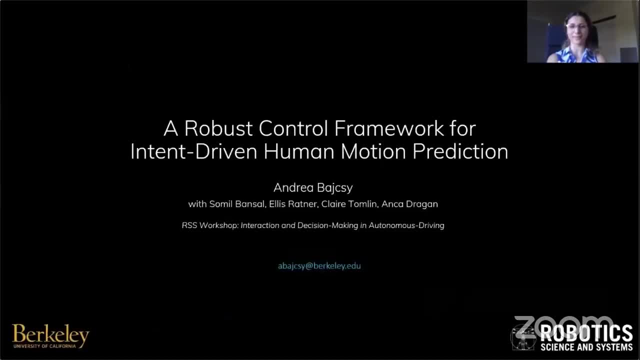 conservative, but not overly conservative, Thanks, Okay, Thank you, Andrea, for your talk. Can you hear me? Yes, I can. Okay, Perfect, So I have also a first question and again I want to invite everyone to simply ask questions. 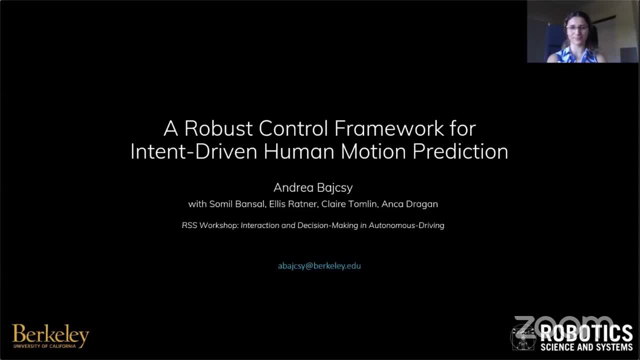 in the Zoom group chat. My question is: what assumptions do you make about the environment and how can these assumptions be enriched? So how can you make more complex assumptions, like typical trajectories or in certain areas agents might be slower than in other areas? 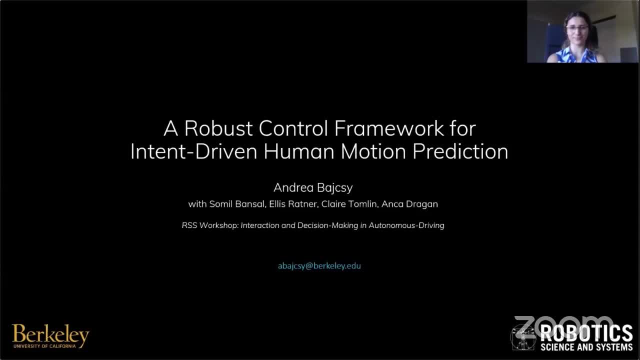 Yeah, Great question. So in the examples that I showed here, as you could tell, there weren't any salient obstacles that people had to avoid, Although I didn't demonstrate these in these examples. actually adding in obstacles is quite straightforward in these robust control methods that we were using here. 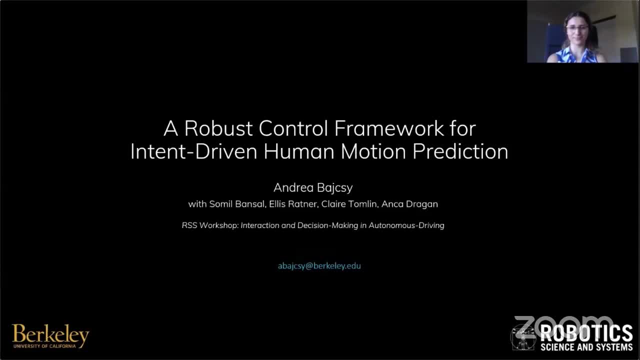 It's sort of a matter of adding in a different constraint set that you're optimizing against when you're safeguarding against certain trajectories. So adding in, for example, you know, lane boundaries or obstacles that the agent might be avoiding is relatively straightforward. 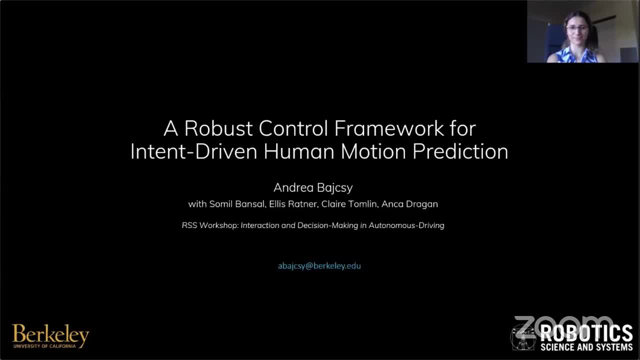 Now these other kind of components of how an agent might be optimizing their intent and their motion, like slowing down in certain parts of the environment. that's a little bit harder And I would classify that as more part of the intent. So, for example, that theta component that was, you know, highlighted in red, can also 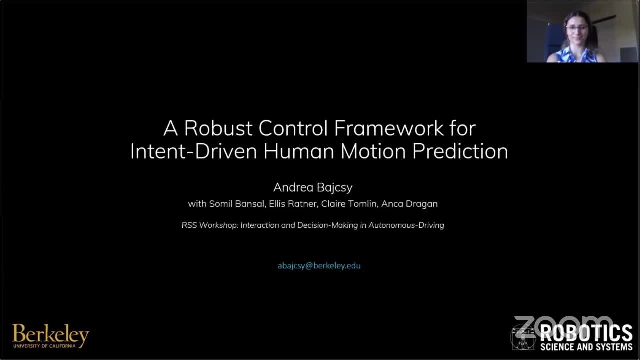 be, in addition to things like salient goal locations where the person's moving in general, can encode things like how a person trades Okay, How a person can take off Their preference for moving closer or slower around other people, or how you know much. 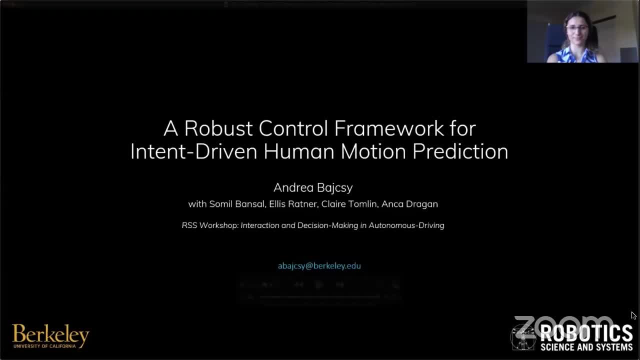 they want to like be aggressive or passive when they're a driver. So, in general, this notion of intent can capture these things which you can learn from that data offline. However, I actually haven't run specifically examples where that data is encoding more. 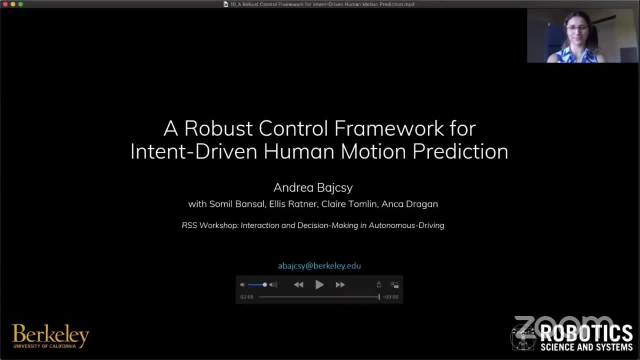 rich notions of intent beyond goals in the examples that I've shown so far, but we're really excited to see how this framework can extend to more robust content. Okay, Thanks so much. There is a question by Ed. Ed is asking: how should a system designer pick a time horizon to balance conservatism? 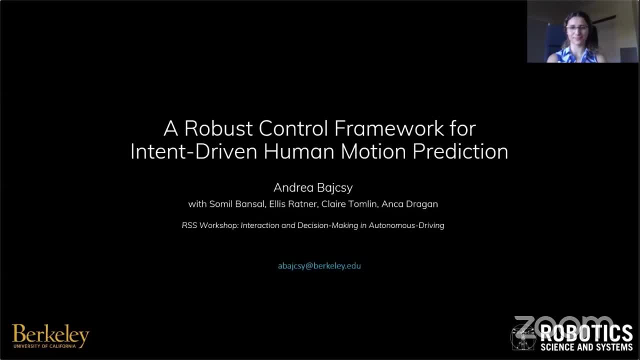 while maintaining safety in FRS computation. That's a great question, So we actually had some discussions around how to choose a time horizon. Now, one thing that I'm currently investigating- and it's not directly part of this work, but it's ongoing work I'm doing- is you can also use reachability as a concept to help you. 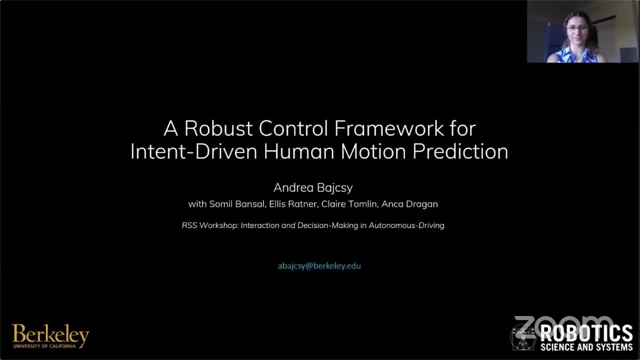 guide a worst case time horizon. you might need to be able to accurately estimate a person's intent and therefore you need to be conservative, for you know, in the worst case, this length of time. So using reachability tools or using these robust control ideas can help us actually. 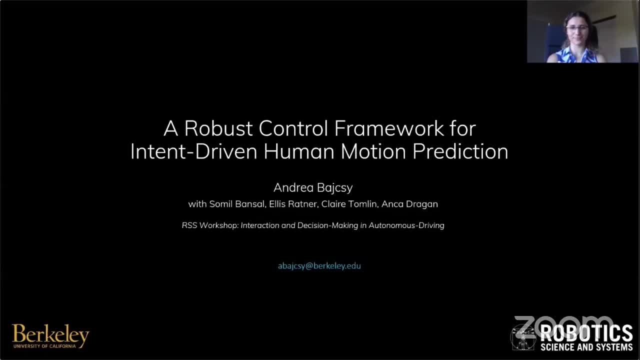 find, In a somewhat principled way, these these worst case time horizons for which we need to be conservative in our motion predictors. but that's actually still very much ongoing work And, Ed, I would love to chat more about this with you if you have that time. 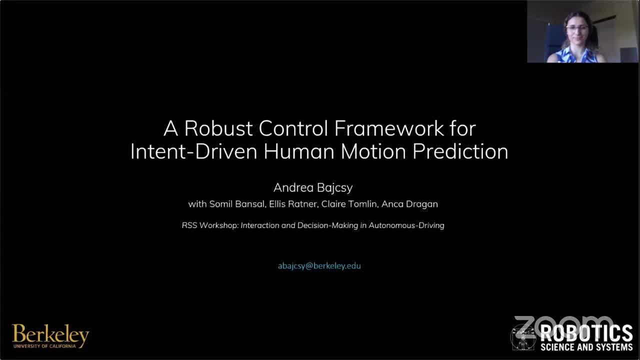 Okay, Thanks so much. Yeah, I would say we are moving on to the next talk. The next talk is called A2GNN: Interaction-Aware Trajectory Prediction via GDL Graph Double Ascension Network. Thank you, Good afternoon everyone. 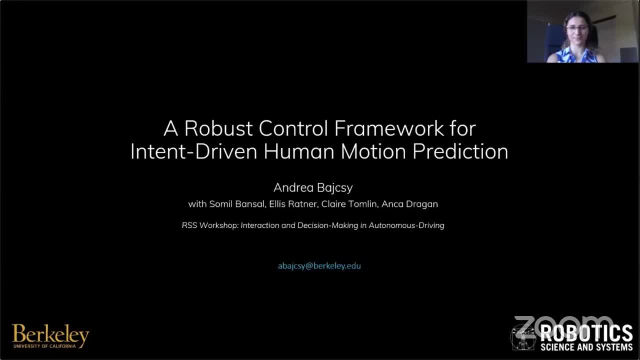 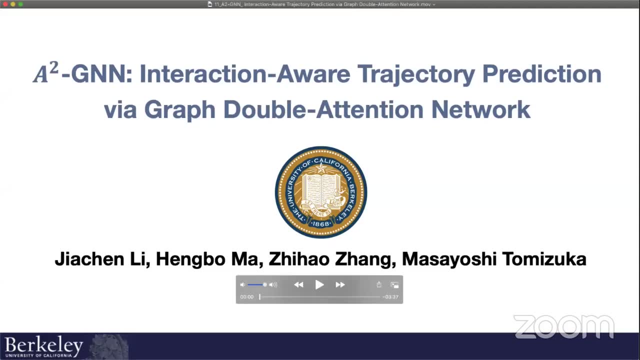 We are here to talk about GDL or GDL-enabled Tribe. It's an interactive channel. We have a large group of people on GDL-enabled Tribe who work with graph double ascension network, And if you are interested in learning more about GDL, we are happy to be with you. 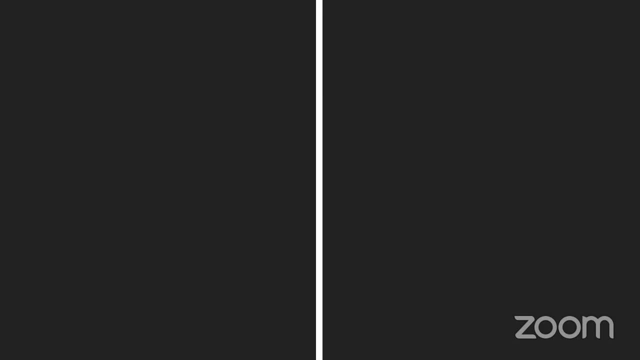 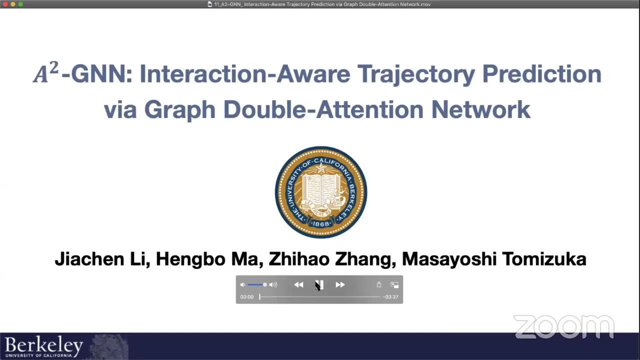 And if you want to keep up with our professional work, we are happy to have you on our team, And we also want to thank you all for your participation and for participating in this talk. Thank you, You're welcome. Thank you very much. 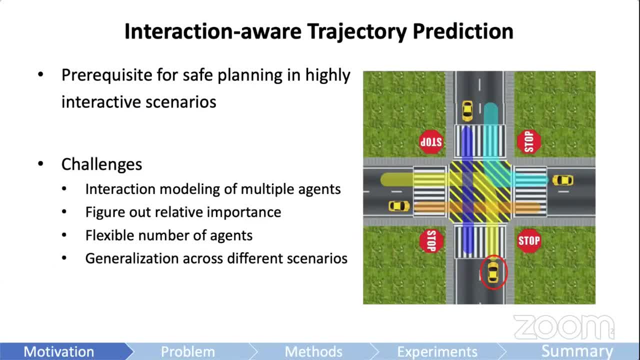 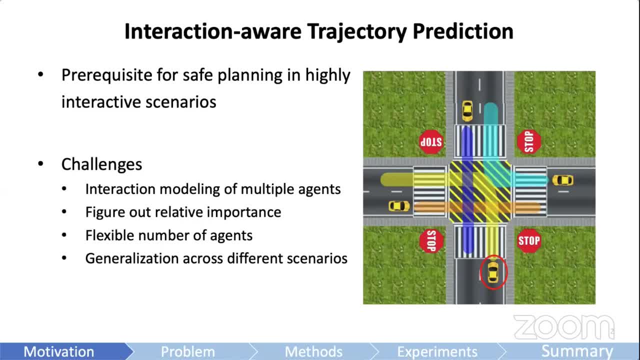 biggest challenges in the multi-vehicle prediction task, since human behaviors are hard to model and there's no ground truth for the behavior model. Also, we need to deal with flexible number of agents and different scenarios. Our goal is to take a step forward to handle these challenges and provide a generic 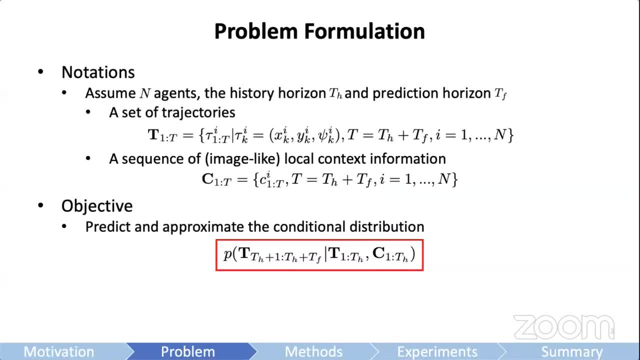 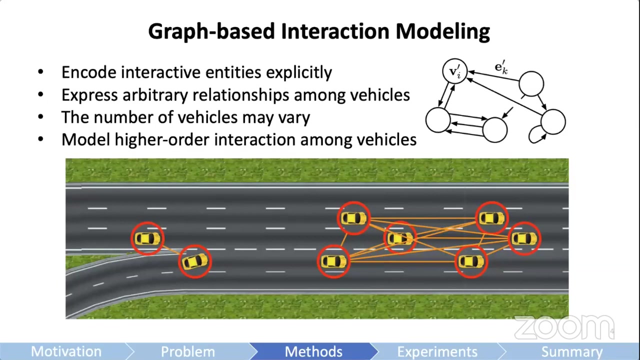 prediction framework. Here is our problem formulation. The objective is to predict the conditional distribution of the future trajectories of each agent, given their history trajectories and the environmental context information. Thank you For interaction modeling. it is intuitive to describe the traffic situation with a graph representation. 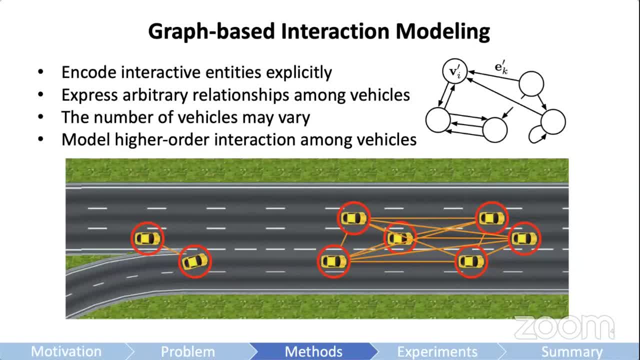 We treat each vehicle as a node and their relation or interactions as edges. This graph representation has several good properties. It can encode arbitrary relation among vehicles and the number of vehicles can be different. Moreover, it can model hair-order interaction among vehicles through multiple loops of message passing. 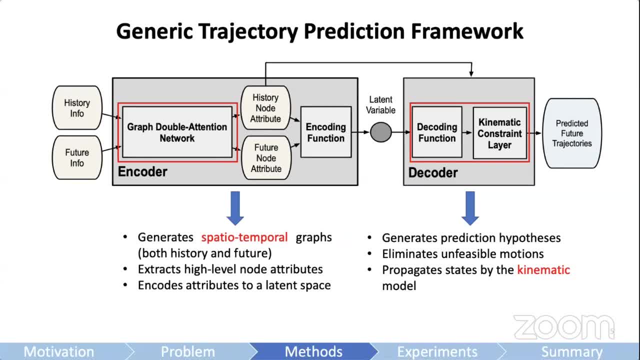 We employ a standard encoder-decoder architecture. The inputs of the encoder are history and future embeddings, which are extracted by a deep feature extractor. Then spatial temporal graphs are generated. The graph double attention network is applied to figure out relative importance of each agent at each time step and extract high-level node attributes. 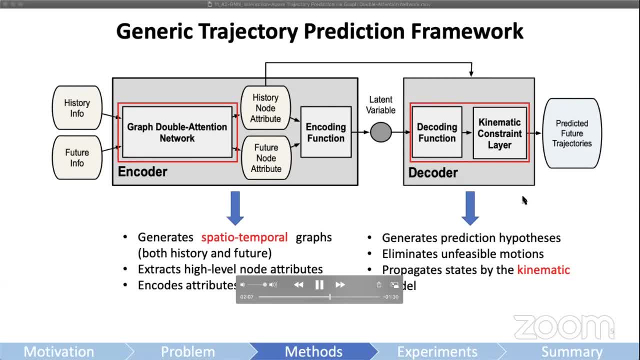 These attributes are encoded to a latent space by the encoding function. The decoder takes in a latent variable and history node attributes to generate action hypotheses. The vehicle states are propagated by the bicycle model. to guarantee kinematic feasibility, We use the same method for the vehicle. 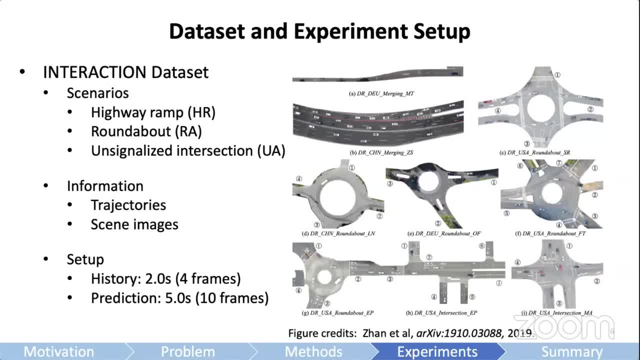 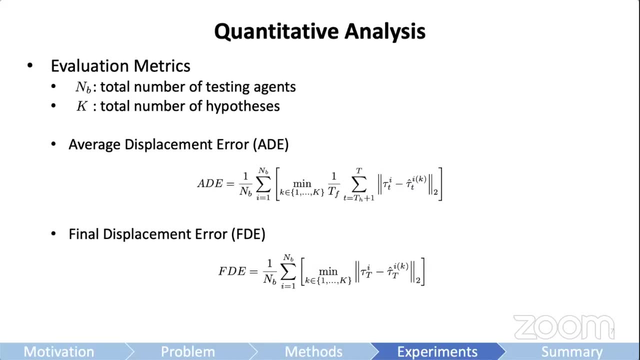 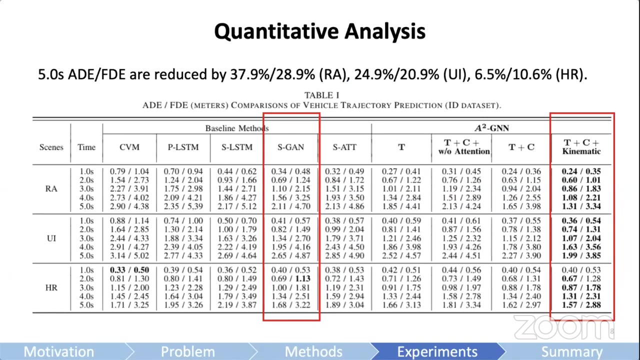 We use the interaction dataset, which includes three highly interactive scenarios. The history and prediction horizons are 2 seconds and 5 seconds. We adopted widely used evaluation metrics: average displacement error and final displacement error. It shows that our method can further reduce the prediction error by a large margin compared with the best baseline method. 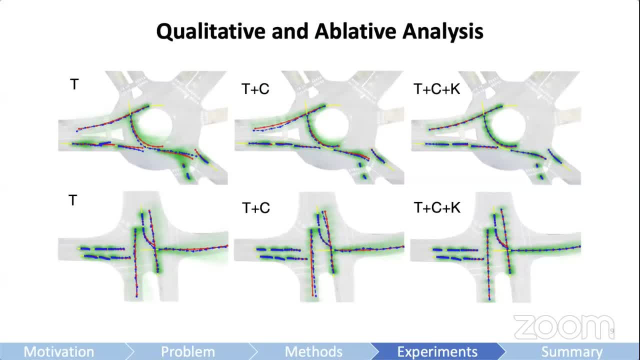 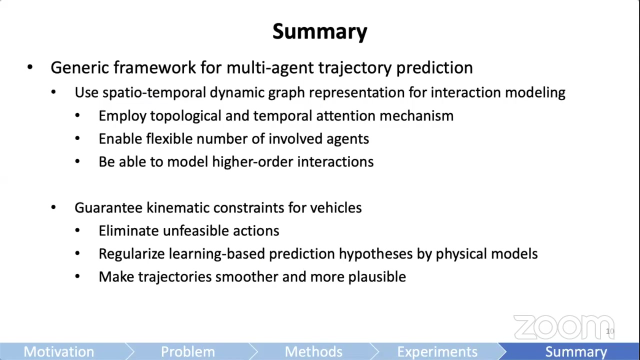 Here are some visualizations of prediction results. Using context information makes the prediction more compliant to road geometries, and enforcing kinematic constraints makes prediction smoother and more plausible. Please refer to the paper for more details. In a word, we propose a generic framework for multi-agent trajectory prediction using spatial temporal dynamic graph representation. 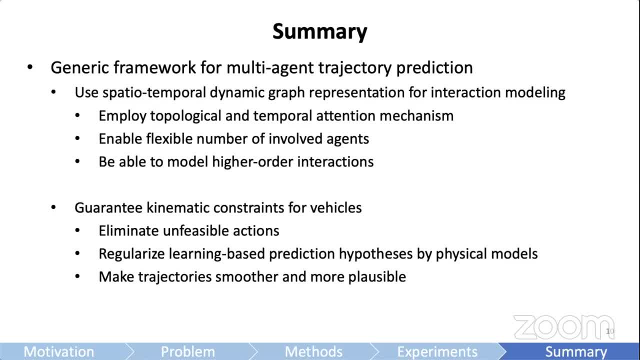 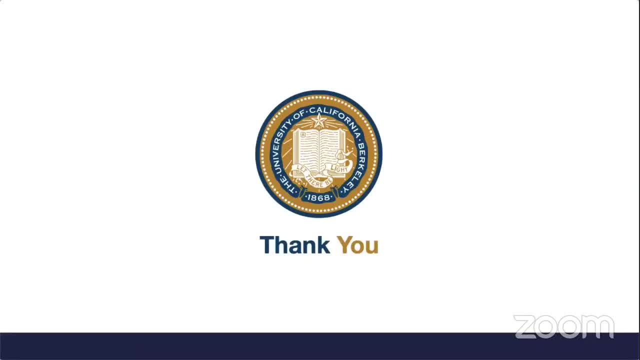 for interaction modeling. Feasibility constraints are also enforced by incorporating a kinematic model of vehicles. Thank you, Yasheng. thanks so much for this very interesting talk And again I want to open this up for questions. Let me start. 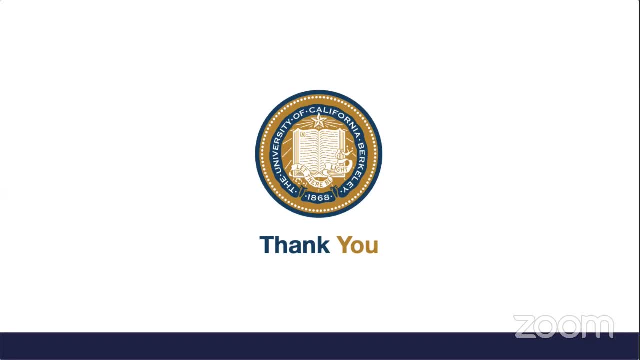 I noticed something when looking at your results. We had the videos in advance. It was otherwise too fast probably to read them, But the numbers were very interesting. So for the very short-term prediction, the adding context has helped a lot and the kinematic constraint has helped only a little. 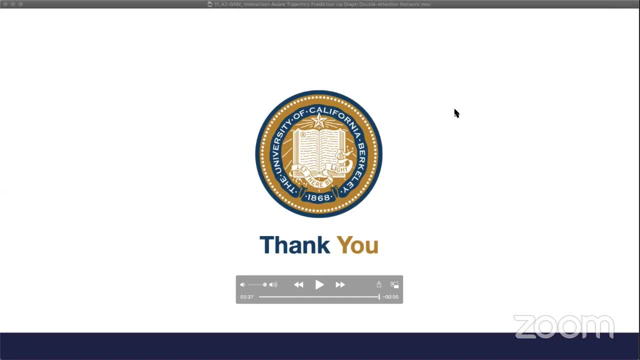 But as you went further to the long-term, the role of the kinematic constraint increased. Can you comment a little bit on this? Do you have an intuition of which of the additional things that you added- For example, context versus kinematic constraints- are important? in which mode of operation? 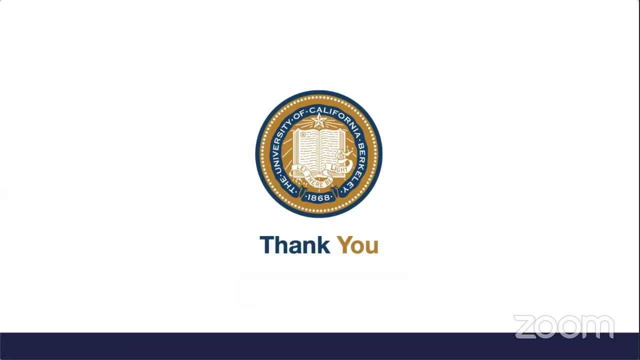 Okay, Thank you for your question. So can you hear me? Yes, Okay, Okay, So for the kinematic constraints. so I think the intuition here is that if our scenarios include some curvature curved rows, then sometimes we need more. 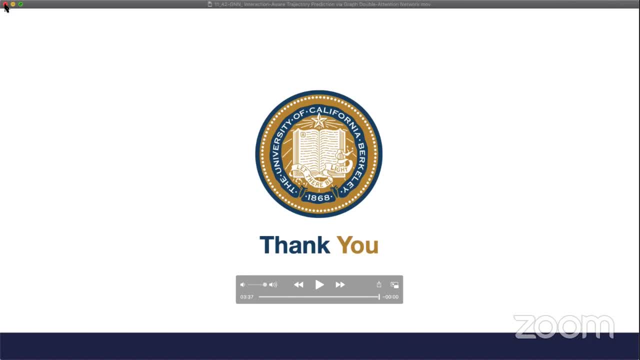 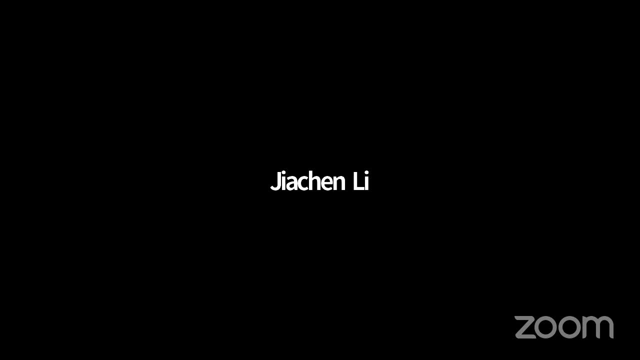 We need a more smoother prediction of the trajectories, And if we incorporate some kinematic constraints for the vehicles, then the variance of the prediction hypothesis will be smaller than not incorporating any constraints. So as long as the time goes by, the long-term prediction can. 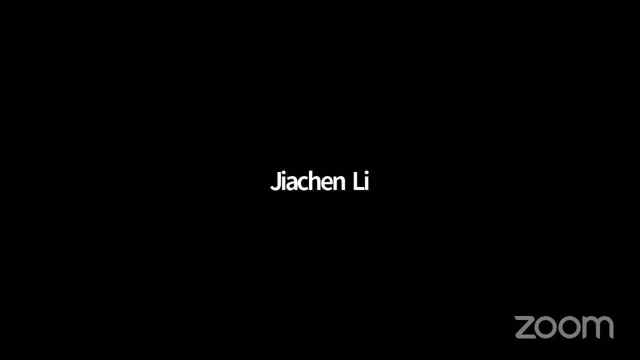 can be benefited from these kinds of constraints And also if we incorporate some context information, then the model can know that what the scenario will be in the near future. So for the long-term prediction, the kinematic constraints and the context information will be more important. 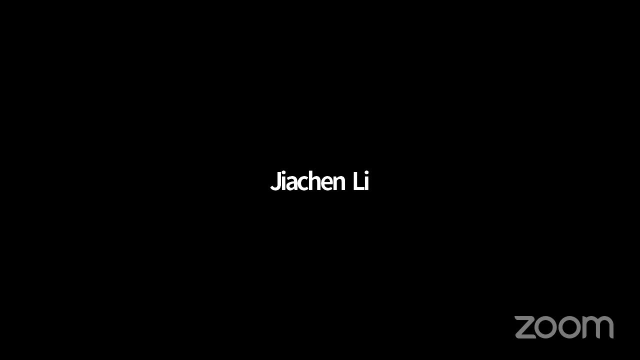 But for the short-term prediction it is just like maybe constant velocity, something like those kinds of patterns. So did I answer your question? Yes, Thanks, so much, Okay, Thank you. I actually have many more questions Very, very interesting. 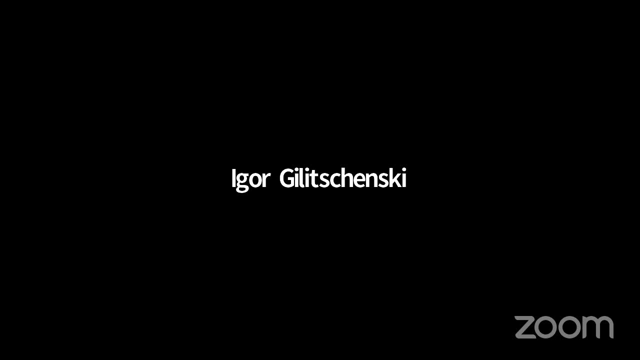 But in the interest of time I would move on to the next talk. Again, everyone is very welcome to ask questions in the chat. I assume. I assume all the authors will be around for the conference, at least for the workshop. So the next talk that we're having is: 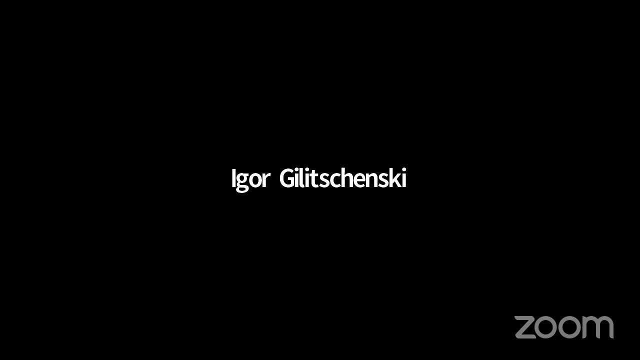 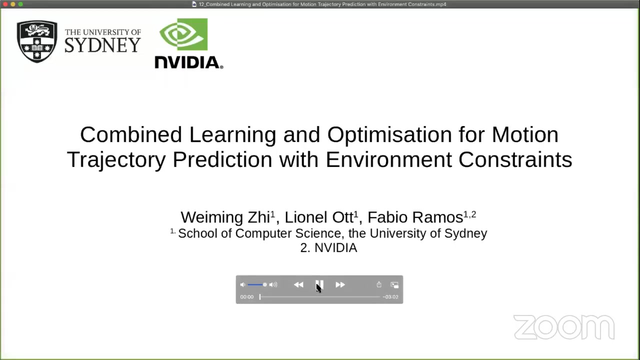 Combined Learning and Optimization for Motion Trajectory Prediction with Environment Constraints by Wei-Ming Chi Hi. My name is Wei-Ming Chi and I'm from the University of Sydney, and I'll be talking about my work on combined learning and optimization for motion trajectory prediction. 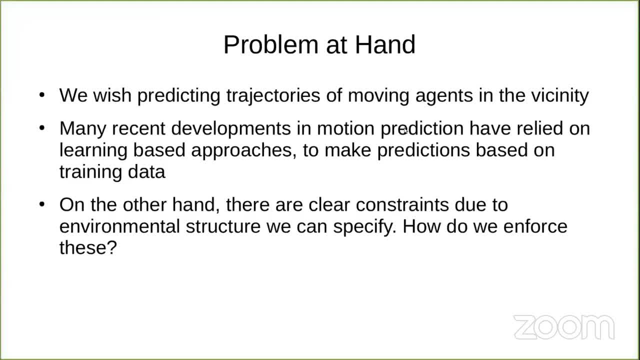 So the problem that we have is we wish to predict trajectories of moving agents in the vicinity, And many recent developments on this problem take a learning-based approach to make predictions based on training data. So, on the other hand, there are also clear constraints due to environmental structure. 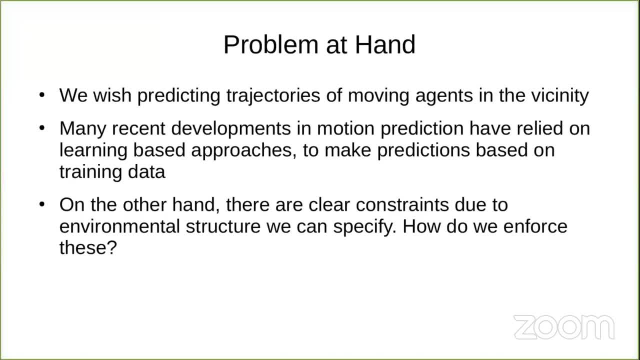 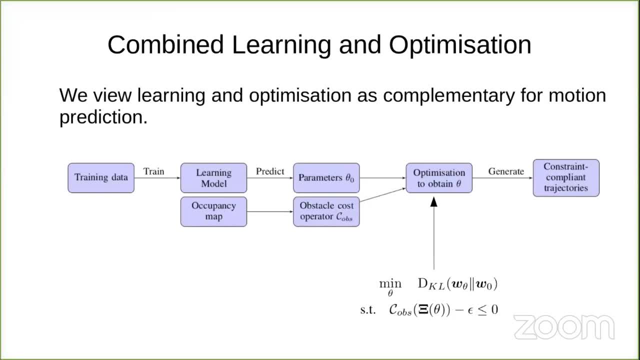 that we can specify. So how do we enforce these constraints? So we propose a combined learning and optimization approach and we view learning and optimization as complementary for motion prediction. So we have a learning component which allows our trajectories to imitate our training data. 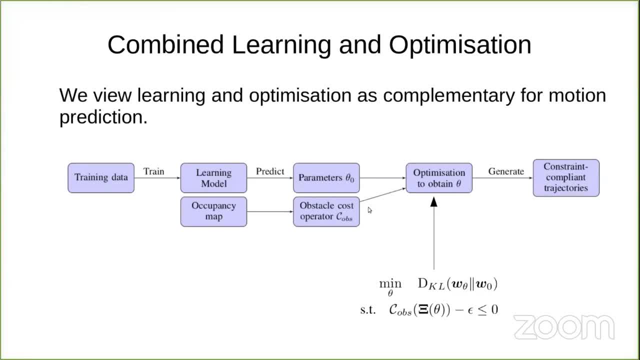 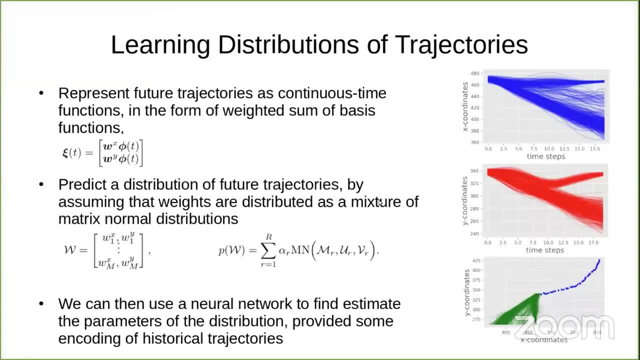 On the other hand, we also have an optimization component to allow us to specify constraints. So, on the learning component, we represent future trajectories as continuous time functions in the form of weighted sums of basis functions, And we predict distributions of future trajectories by assuming that these weights are distributed. 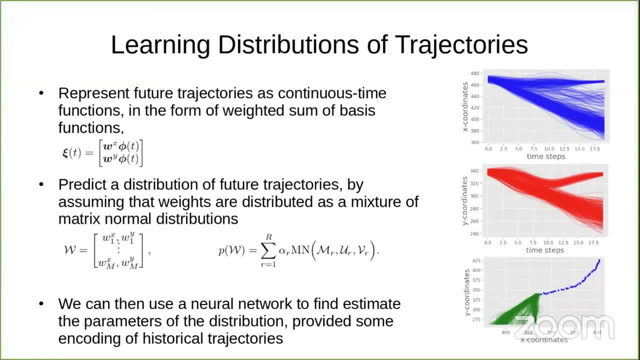 as a mixture of matrix, normal distributions, And then we can use a neural network to estimate the parameters of this distribution. And on the right here you can see distributions of trajectories. You can see that this is also multimodal. So next we want to optimize these distributions of trajectories. 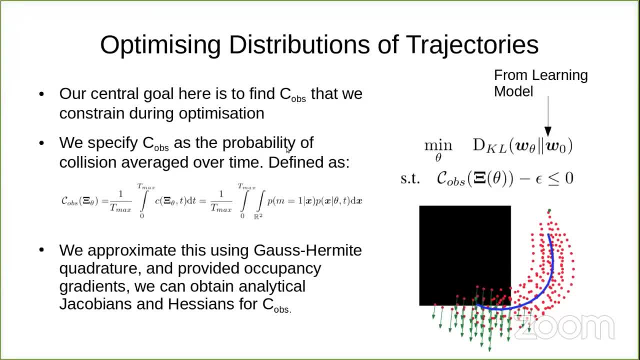 and our goal here is to find this obstacle cost, which we define as the probability of collision over an entire distribution of trajectories defined as this integral here, And we can approximate this using quadrature methods and, provided occupancy gradients, we can obtain analytical Jacobians and Hessians. 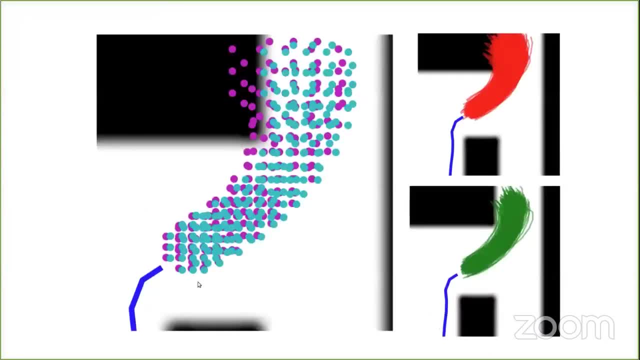 making the optimization easier, And here is a case study. So this magenta distribution of trajectories is solely from learning And we can see that it collides with occupied space or occupied regions, while the cyan trajectory is from learning and optimization And we can see that it complies with environmental constraints. 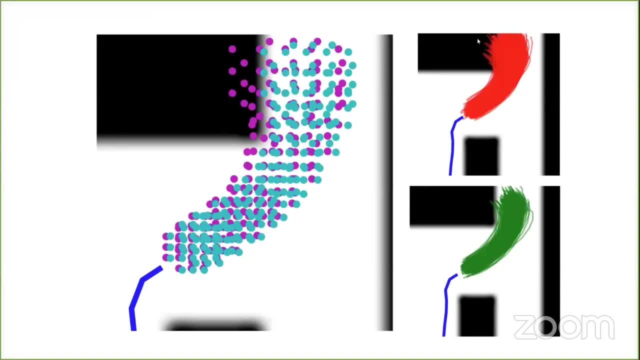 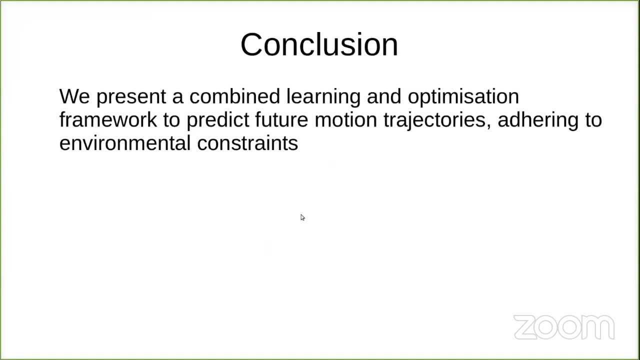 And on the right. here you can see: these red trajectories are generated from the non-compliant distribution of trajectories, while the green are generated from the compliant And, in summary, we present a combined learning and optimization framework to predict future motion trajectories And our future motion trajectories adhere. 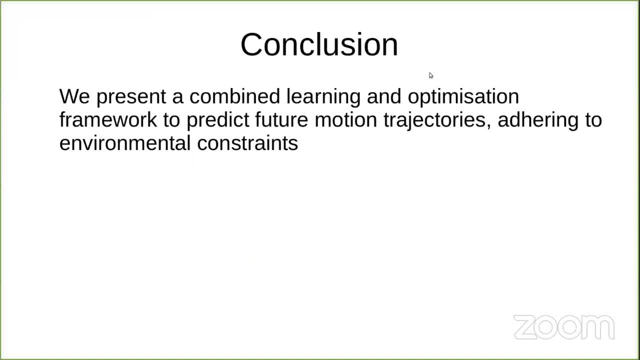 to environmental constraints. Armin, can you hear me? Yep, yep, I can hear you. Awesome. Thanks so much for the talk. Again, as the reminder, simply write questions in the Zoom group chat. I start with the first question. 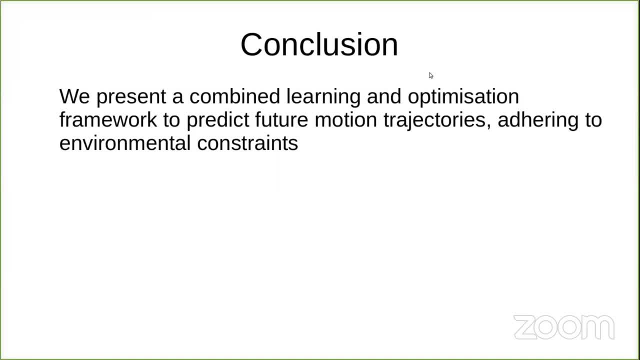 So I really like the approach. I was wondering how easy is it to integrate in this type of approach more complex constraints. On the one hand- I was thinking of more complex social modeling- And on the other hand, something like dynamic obstacles or like some sort of dynamics. 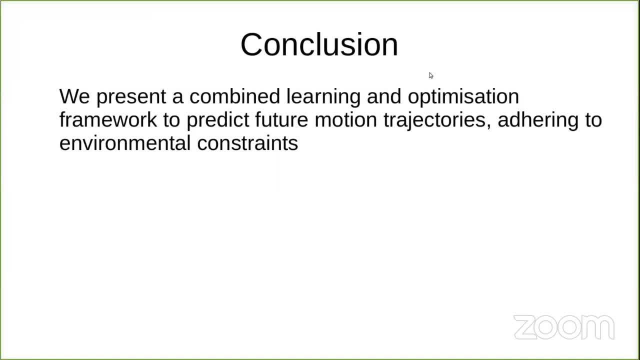 of the vehicles that are involved. It should be fairly OK, as long as you can write it as a cost. I've tried other constraints, like velocity constraints, So if you know beforehand that these moving things that you're trying to predict are below some velocity, 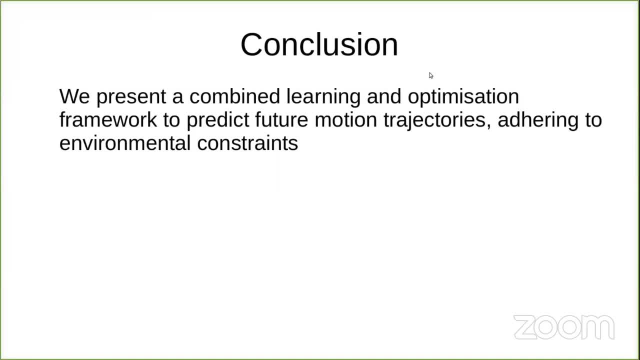 you can have constraints on that. So specifying the constraints as long as you can write it down and as some sort of constraint that you put into an optimization problem, And normally the optimization actually works quite well, because if you use the prediction as a kind of warm start for the optimization, 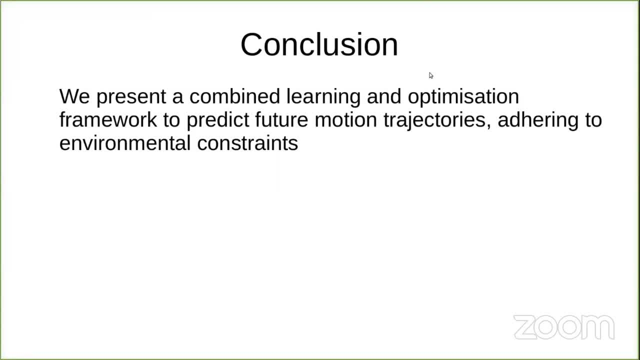 it's, the prediction is actually already quite close to an optima. So, yeah, So, as long as you can write it down as a constraint, hopefully you'd be able to use this. Thanks, Alright, Thank you, Bye, Bye. 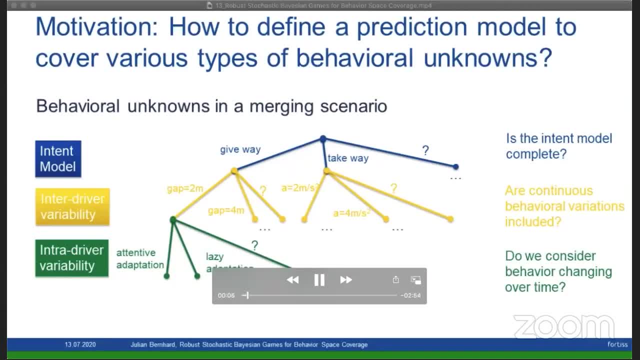 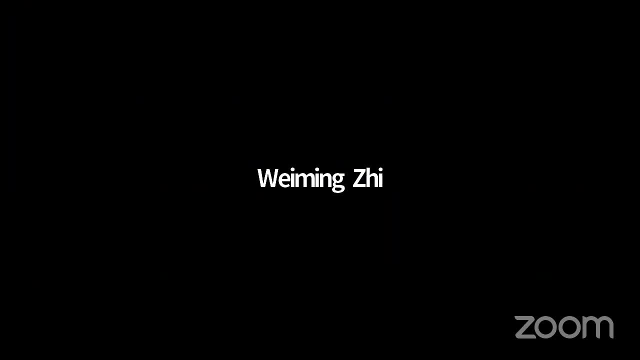 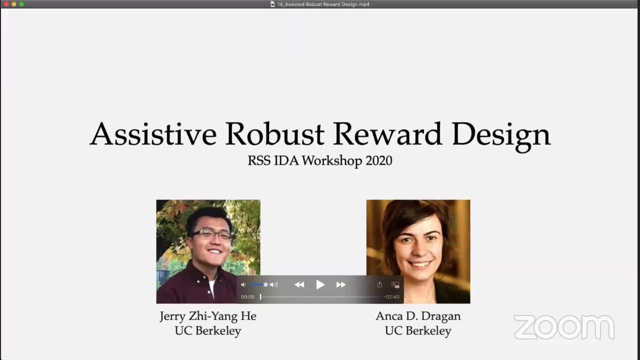 Thank you. You are quickly resolving the sound issue One second. You are quickly resolving the sound issue One second. While we resolve the sound issue, I will first. we will first start with the last video and then get back to the second to last video. So the talk that we will be hearing now first is Assistive. 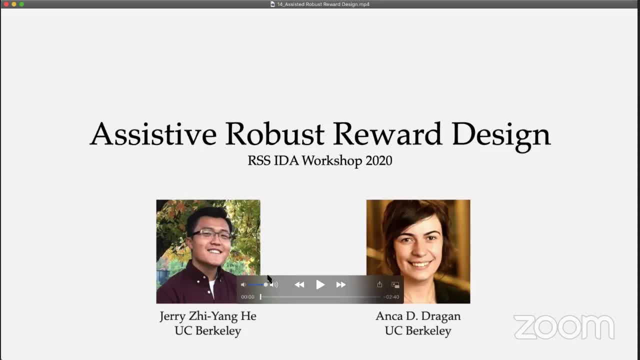 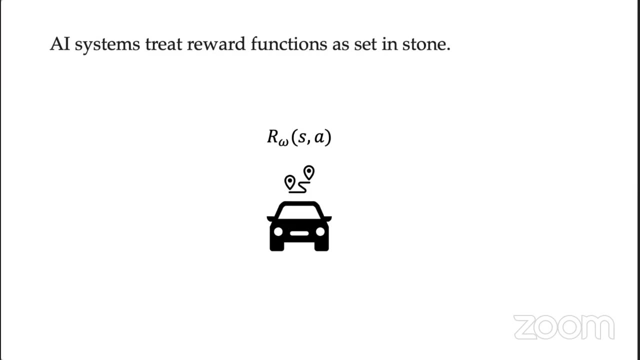 Robust Reward Design by Jerry Chi-Yang He. We present Assistive Robust Reward Design. Real-world AI systems rely heavily on their reward functions in order to operate correctly. For instance, an autonomous vehicle is guided by a reward function that prescribes good driving behaviors. 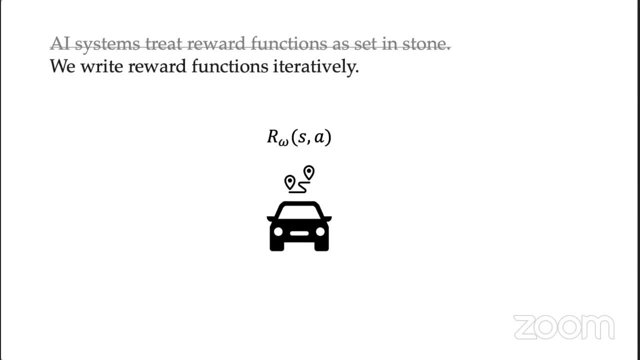 While the system treats this reward function as set in stone, we seldom ride this reward function once and for all. In fact, we frequently update this reward function to account for different factors, such as safety and efficiency, As we develop and test our systems in more. 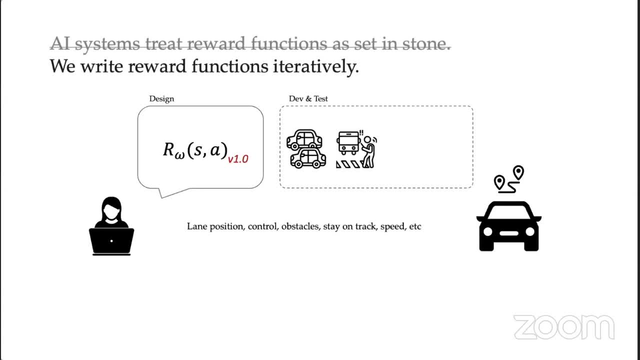 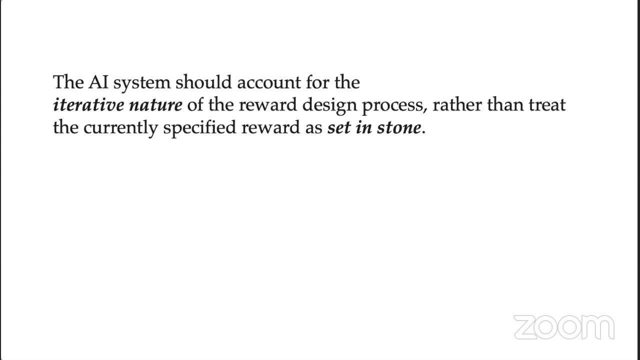 real-world environments. we go back and forth to revise this reward function. Even after the system is deployed, we may still encounter failure cases. that needs to be addressed by the change of reward design. This motivates us to rethink the current AI systems for self-driving and other applications. 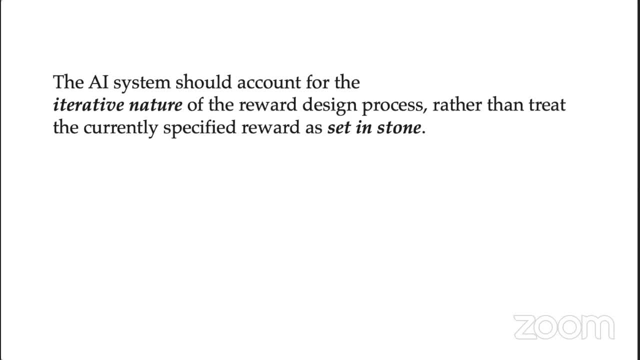 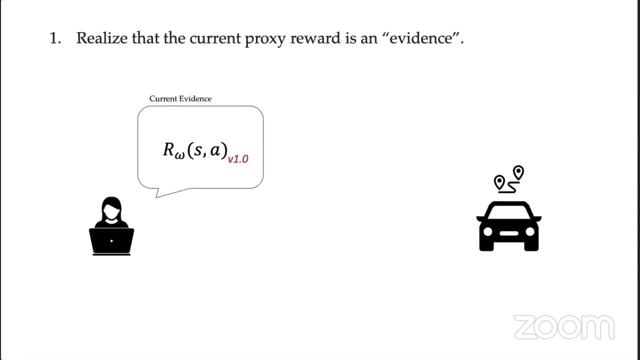 We argue that the AI system should account for the iterative nature of the reward design process, rather than treat the currently specified reward as set in stone. Let's break down what this means. First of all, the AI system should realize that the proxy designs from the designers are not golden standards, but only evidences of the true. reward function. The AI can then use this reward function to determine the reward function. The AI can then use this reward function to determine the reward function. The AI can then use this reward function to determine the reward function. The AI can then use this: 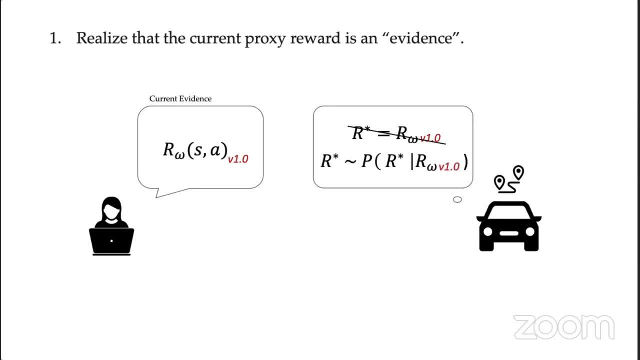 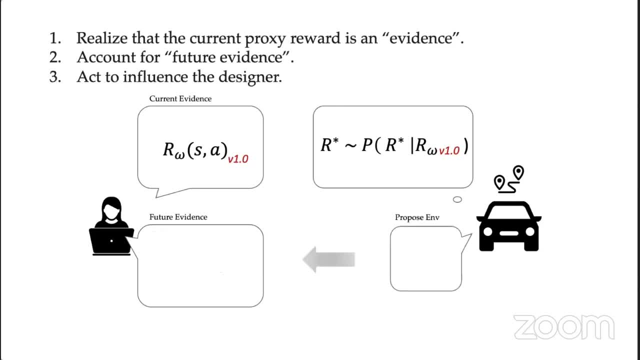 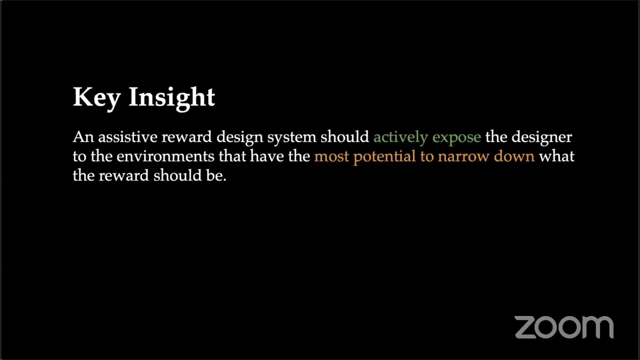 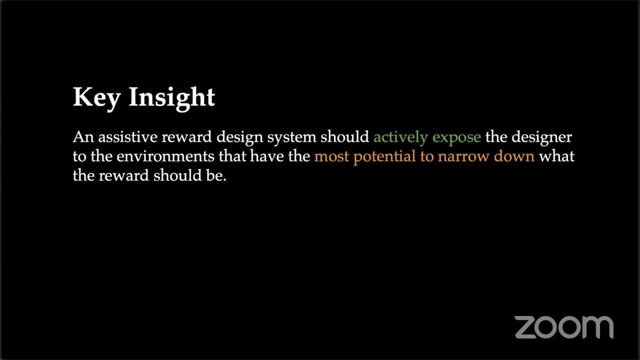 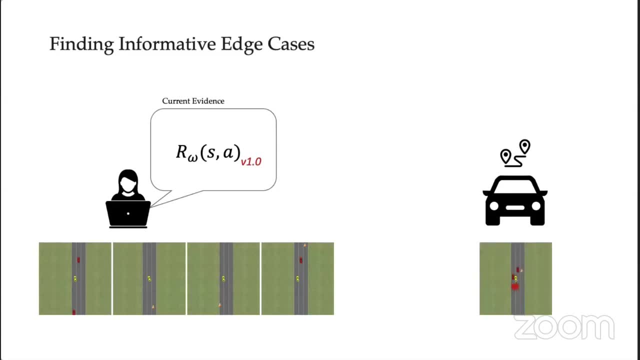 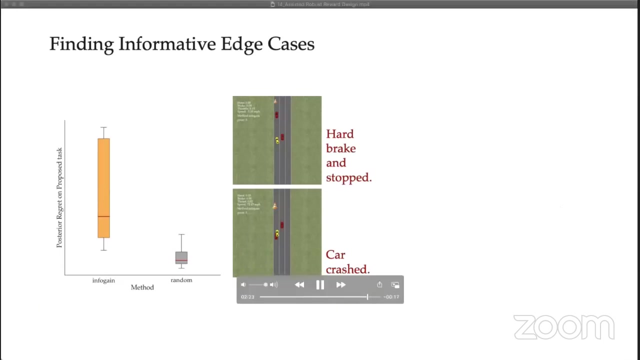 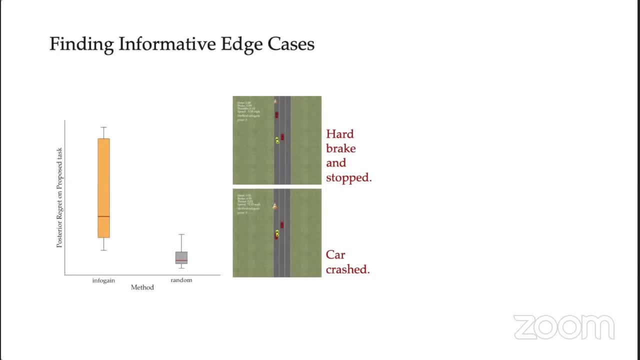 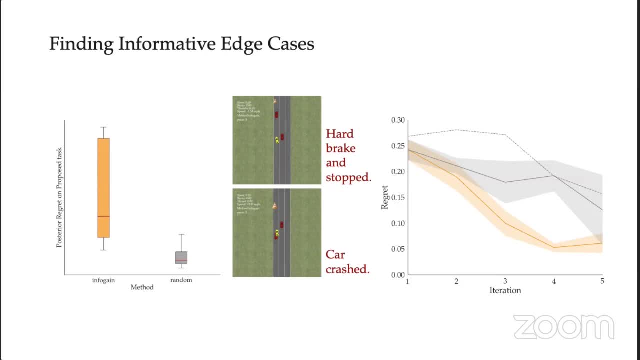 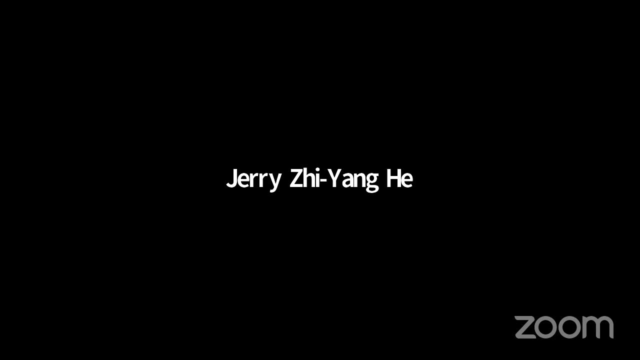 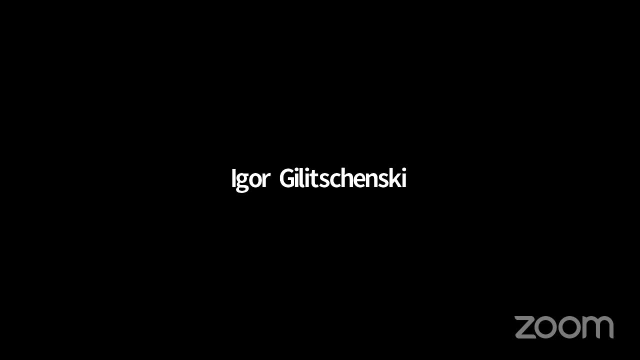 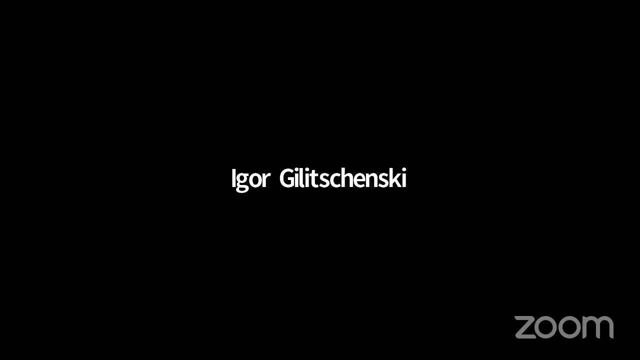 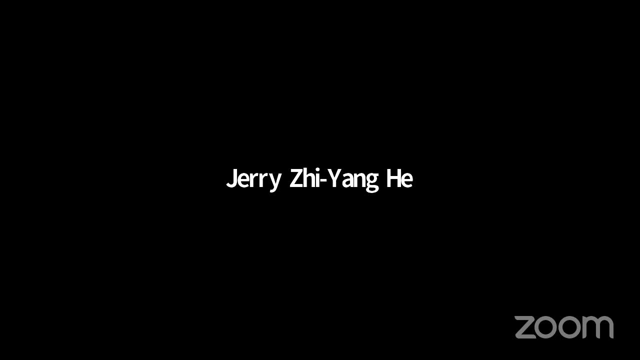 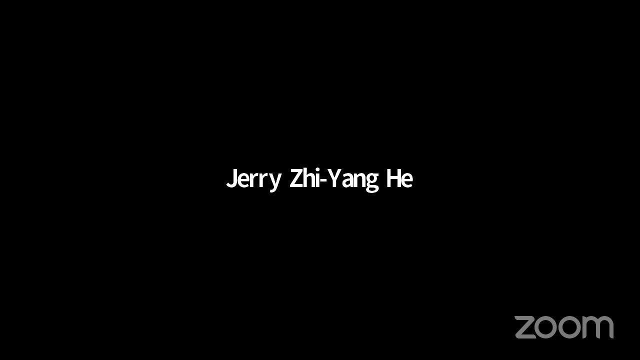 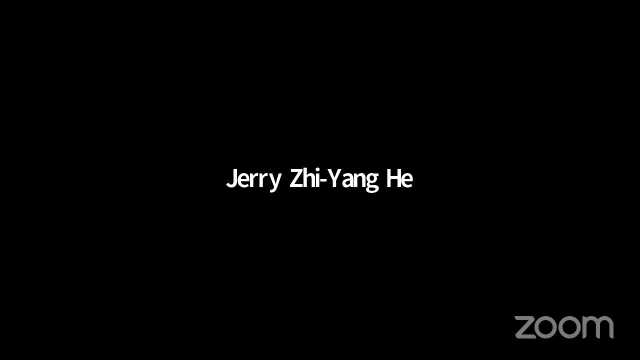 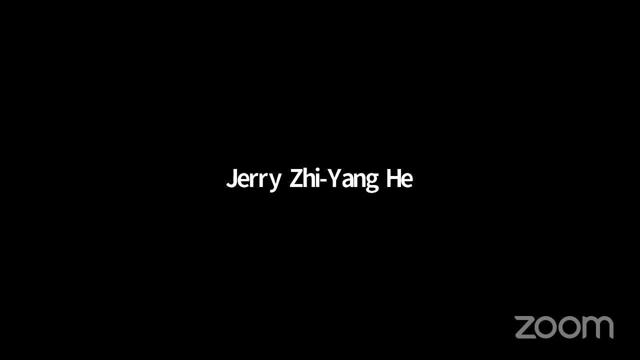 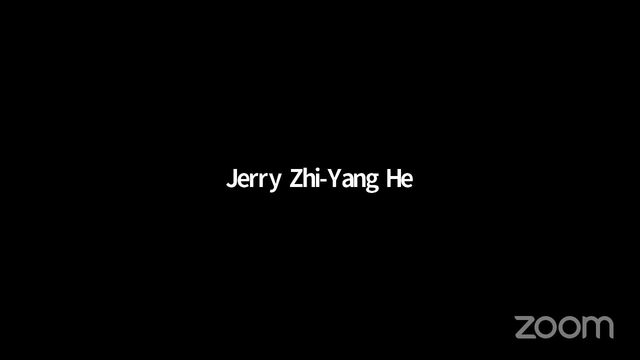 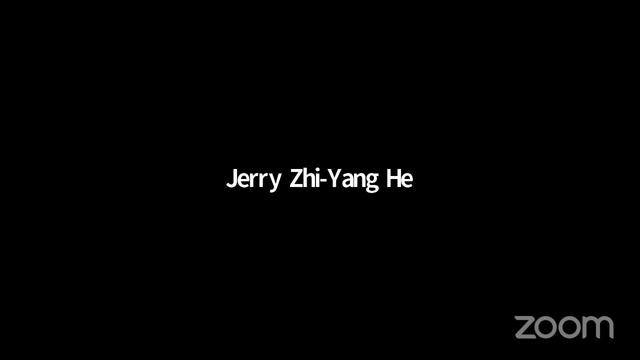 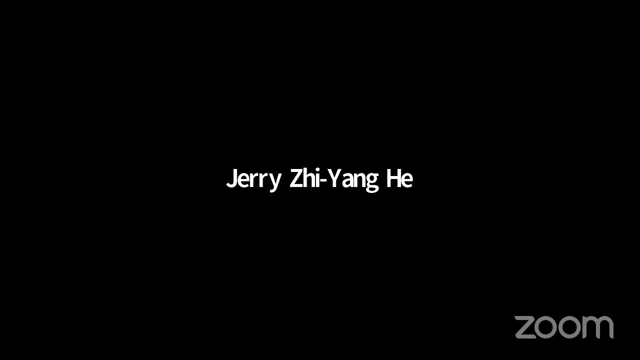 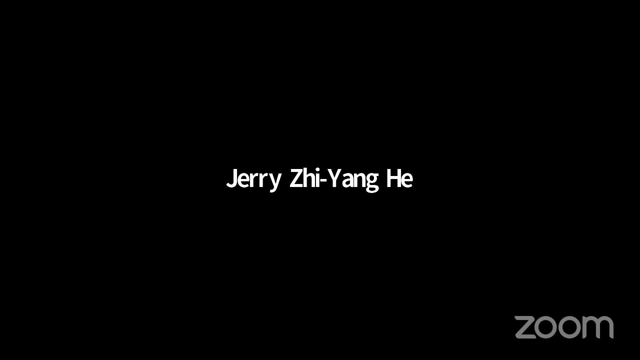 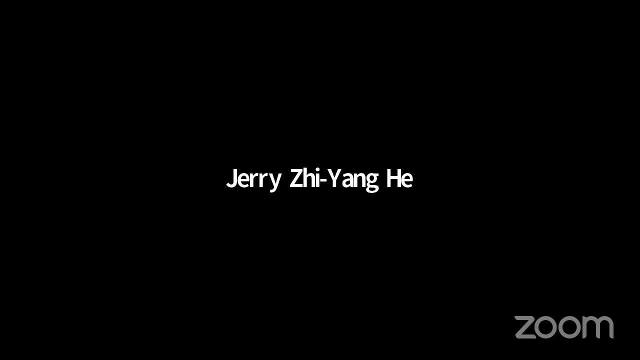 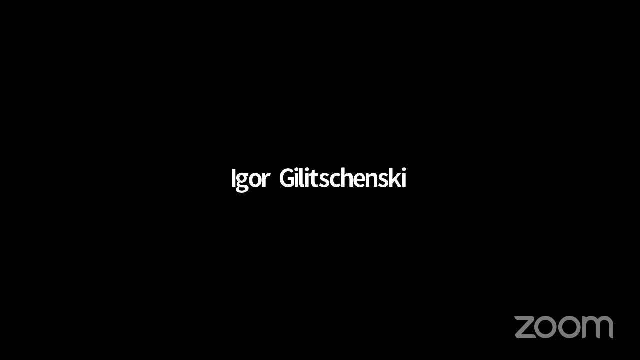 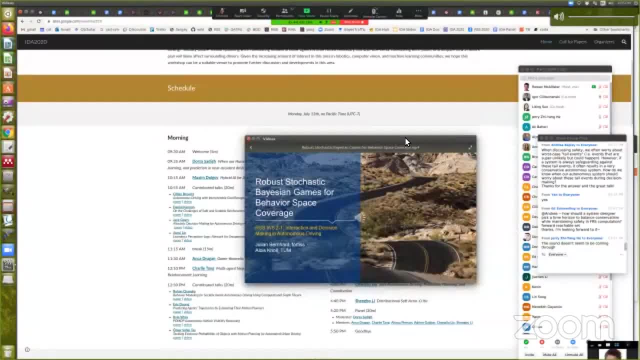 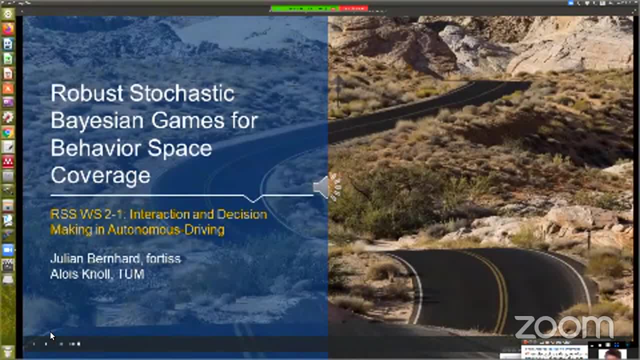 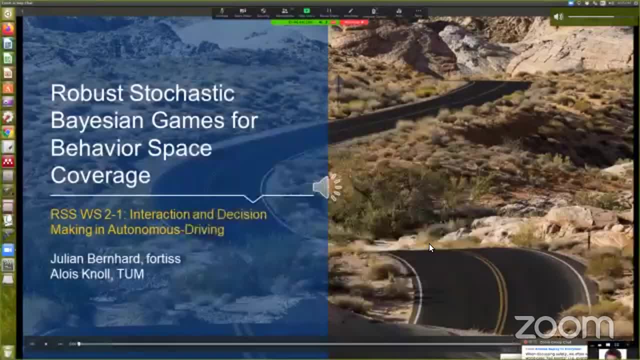 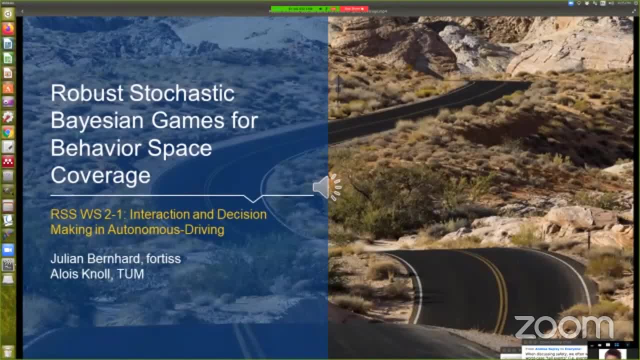 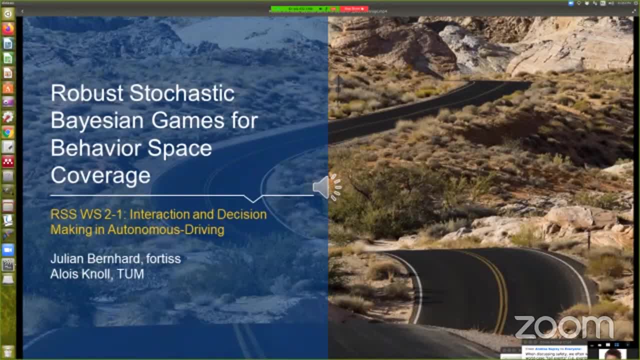 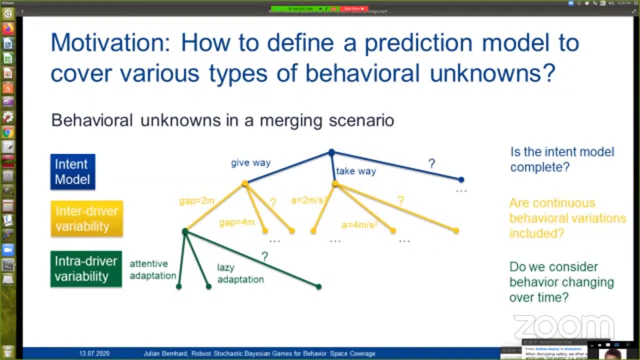 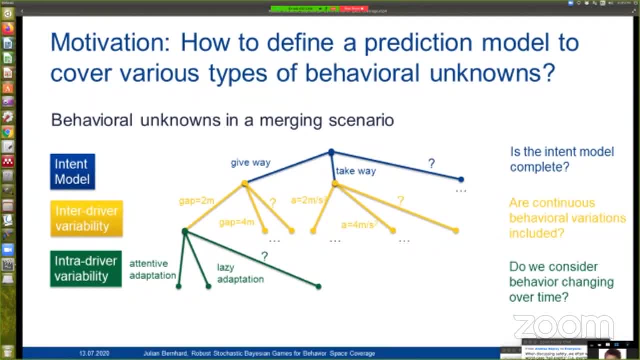 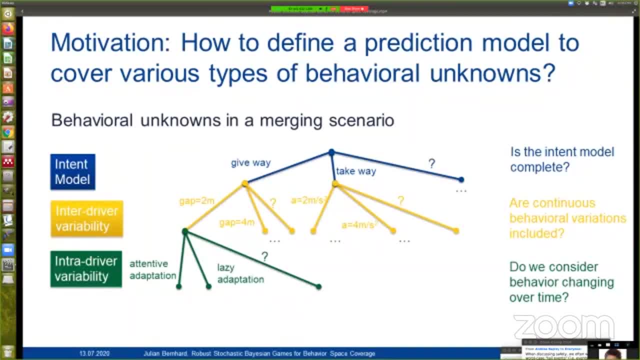 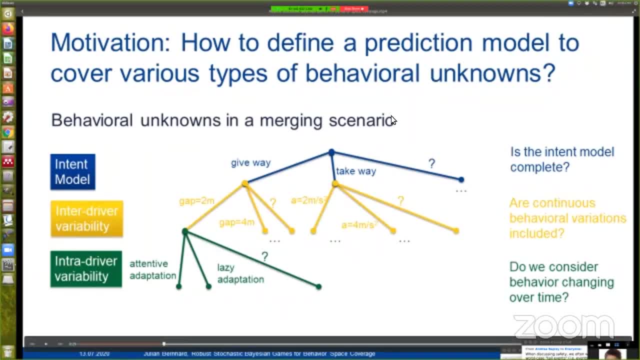 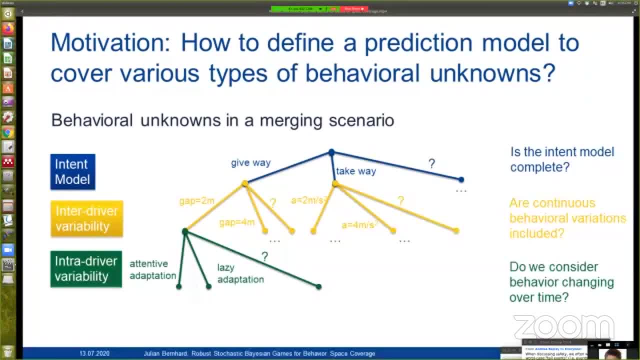 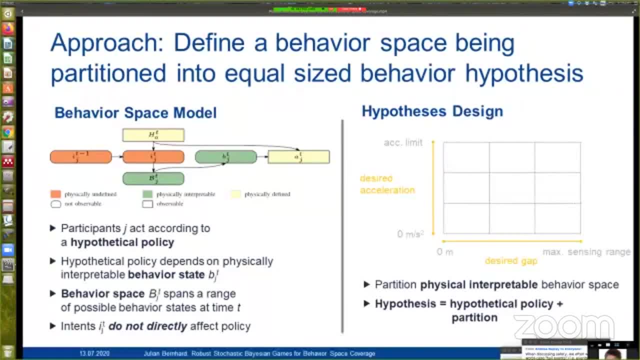 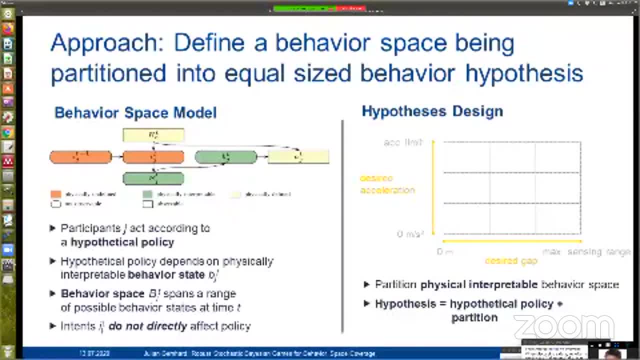 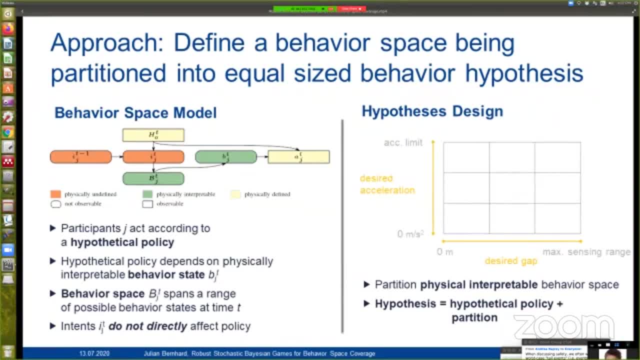 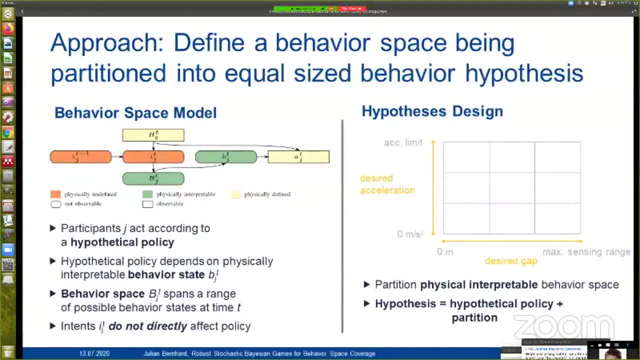 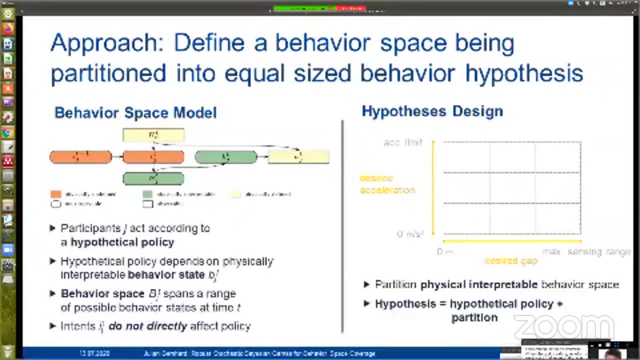 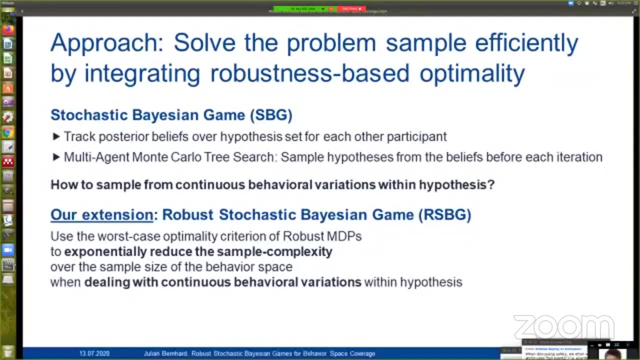 maximum sensor range. The desired acceleration of another vehicle must be between 0 mps squared and the physical acceleration limit. We then partition the behavior space to define the hypothesis set. We solve the problem sample efficiently by integrating robustness-based optimality To solve the standard stochastic. by using game one can track posterior beliefs over. 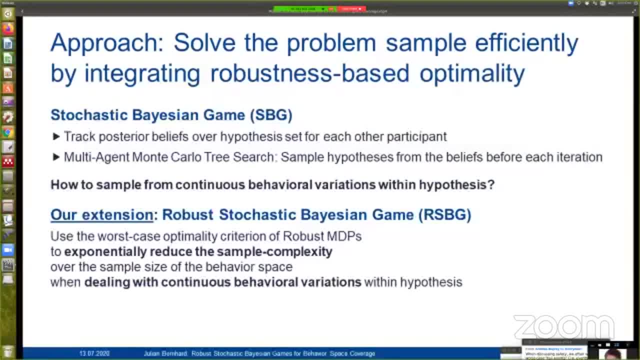 the hypothesis for each other participant and then use a multi-agent Monte Carlo tree search algorithm and sample different hypotheses from the beliefs before each iteration. We integrate the worst-case optimality criterion of robust Markov decision processes into the stochastic by using game. In our paper we prove that our extension, the robust stochastic by using game. 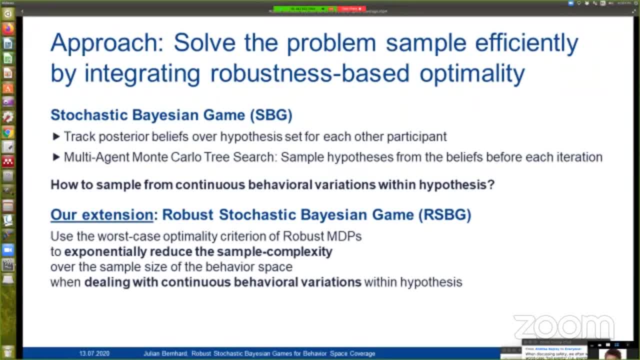 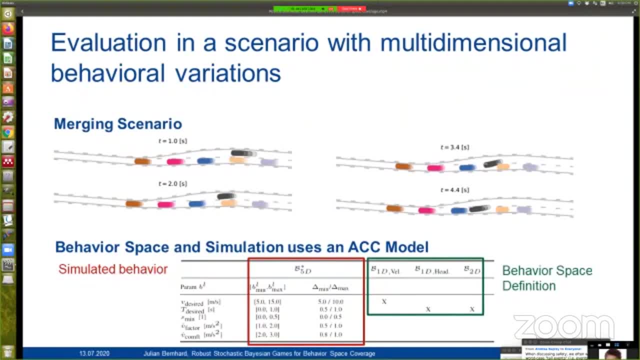 reduces the sample complexity exponentially. when dealing with continuous behavioral variations within hypothesis, We analyze our approach in a merging scenario where we simulate that the unknown behavior of other participants covers a five-dimensional behavior space based on an adaptive cruise control model. We sample unknown boundaries of behavioral variations for the 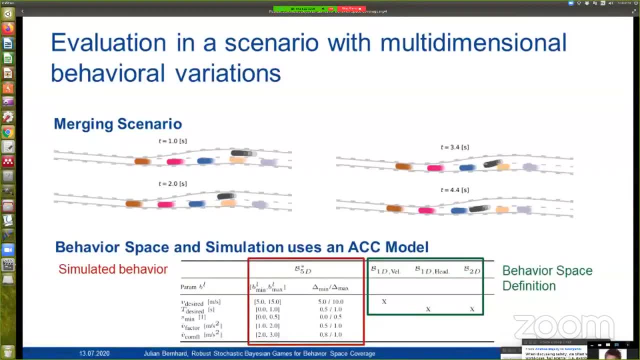 parameters of the aircraft. We then use the stochastic bias in game to simulate the stochastic for each participant in trial. We use lower dimensional behavior spaces for building the hypothesis set, defined over the desired velocity, desired time, headway or both parameters. We calculate percentages of collisions in successful merging and the average scenario time. 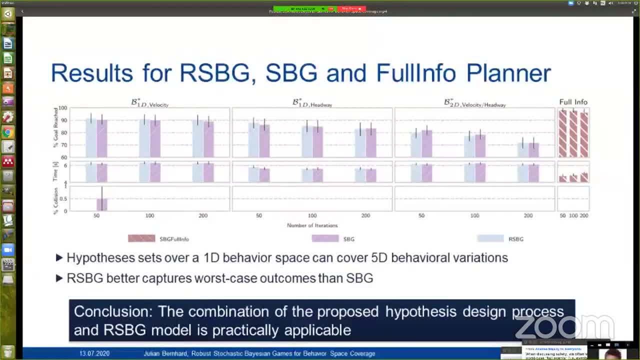 and show the results for different numbers of iterations. for 200 trials, The SPG and RSPG planners achieve near the same performance as a full info planner having access to the true behavior of other participants. The SPG shows some collisions for 50 iterations. 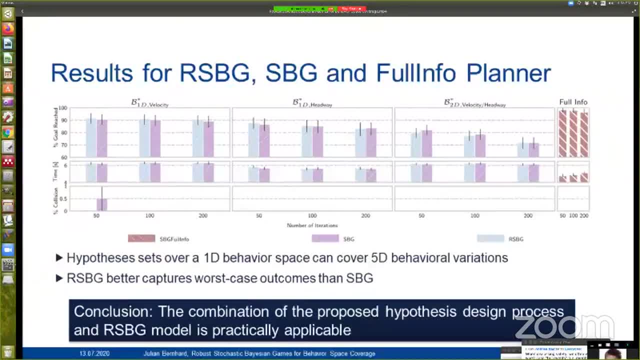 This indicates that hypothesis sets over a 1D behavior space can be used to cover 5D behaviorable variations. Also, the RSPG model better captures worst-case outcomes than SPG. We conclude that the combination of the proposed hypothesis design process and RSPG model is practically applicable. 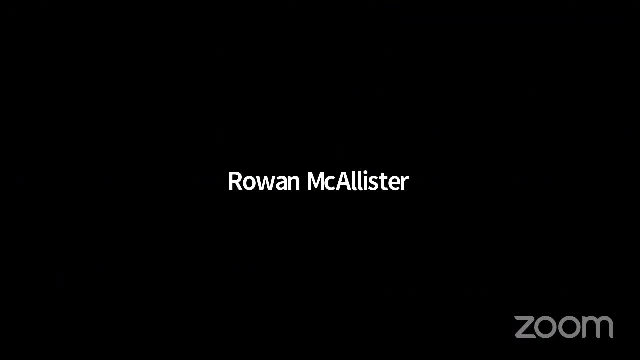 Thank you for your attention. I'm not sure if No, I don't think Julian is here. I think we've caught him at a difficult time for Europe, But if you have any questions, we've linked to Julian's web page in the schedule. 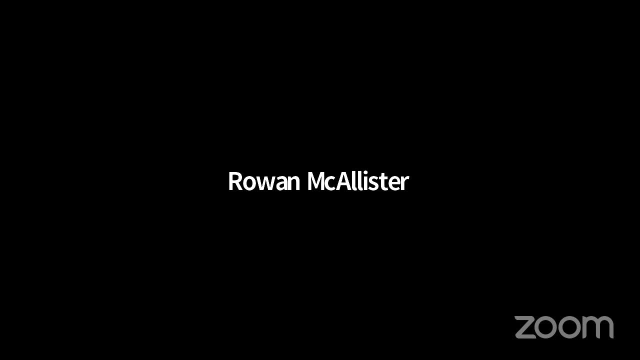 His name is a hyperlink, So feel free to ask him any questions. And I think with that, and especially since Julian is not around and we're running a little bit late, we'll move straight on to our next speaker, who is Professor Chengliu Liu. 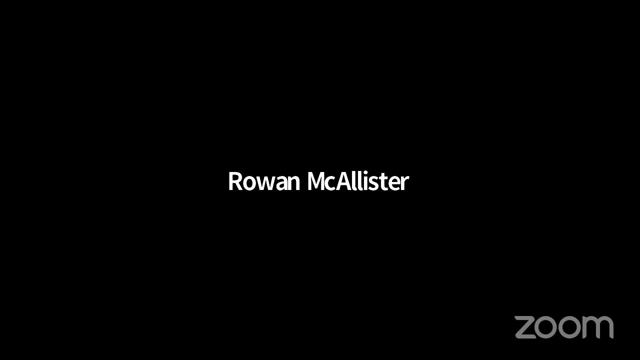 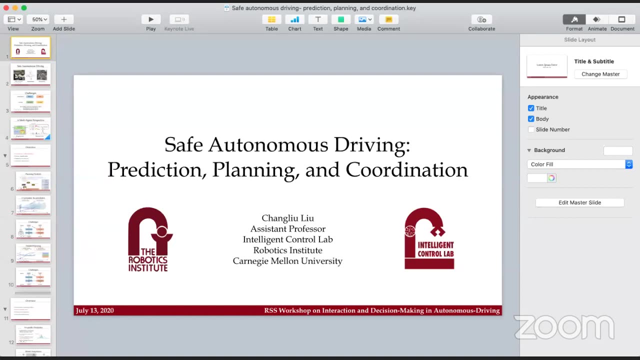 who is an assistant professor at the Robotics Institute at Carnegie Mellon University. Her research interests lie in the design and verification of intelligent systems with applications to transportation and manufacturing. She published the book Designing Robot Behavior in Human-Robot Interactions, which is great for this workshop. 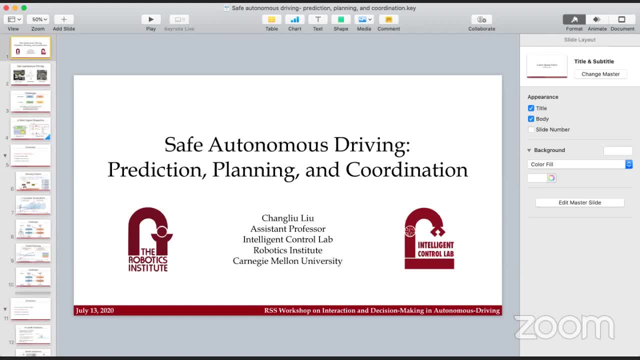 with CRC Press in 2019.. She's the recipient of the 2019 Amazon Research Award, And her talk today is titled Safe, Autonomous Driving: Prediction, Planning and Coordination. So thanks so much for joining us today, And we look forward to your talk. 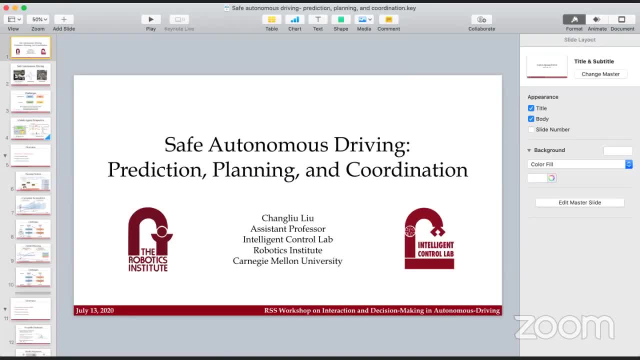 Whenever you're ready to start. Thank you, I'll give everyone a minute. Oh cool, Thanks for unmute me And thanks for the introduction. Okay, Hello everyone, I'm Chang Liu. Today I'm going to talk about safe autonomous driving, So let me go to the full screen. 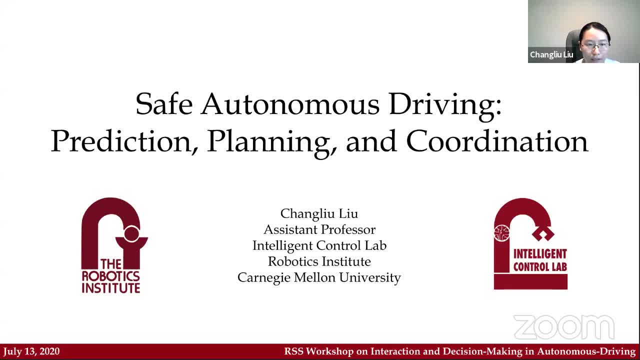 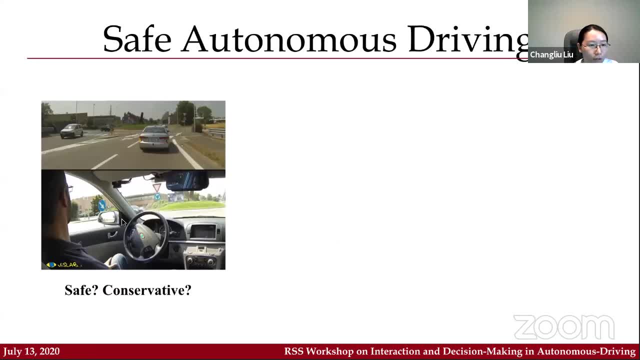 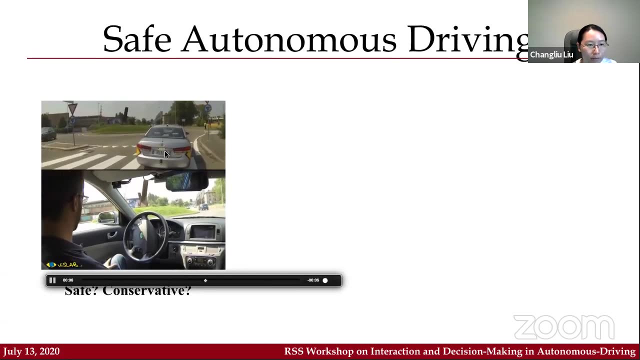 Okay, Can you see my slide? I suppose yes, Okay, So when we talk about safe autonomous driving, what are we looking for? So, for example, if the autonomous vehicle bumping into another vehicle in the roundabout, the vehicle should yell, So that's a safe behavior. 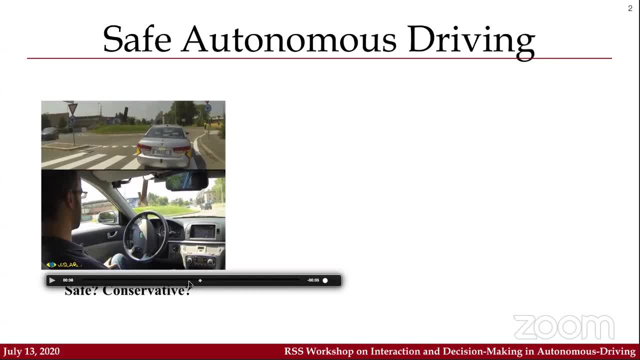 But the second case when another autonomous vehicle goes in, the vehicle yells that's safe, But actually there's no clear. There's a conflict between the other vehicle and the ego vehicle. So from an efficiency perspective this behavior is actually not desired. It's too conservative. 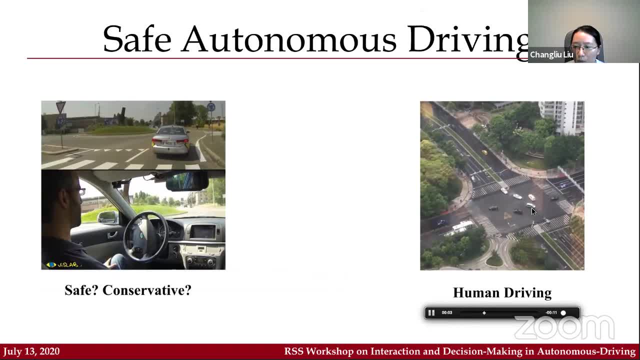 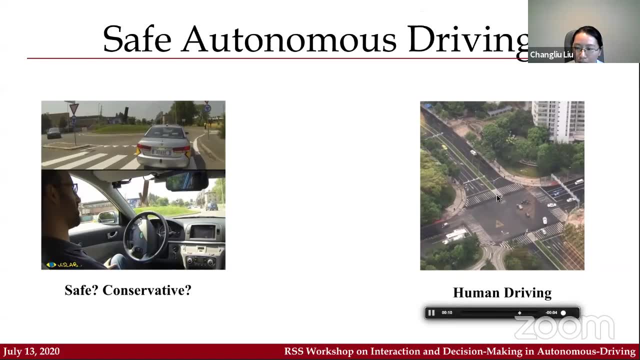 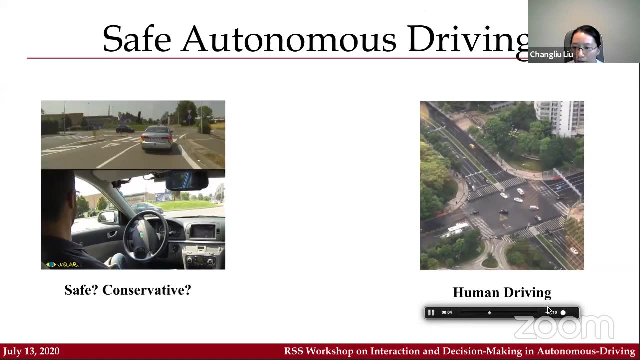 And let's look at how human drivers will do So. this is a video I took at a middle-sized intersection in Shanghai. There's left-turn vehicles and straight vehicles. There's no left-turn light to regulate the behavior of the left-turn vehicles, but the human drivers managed to cross each other. 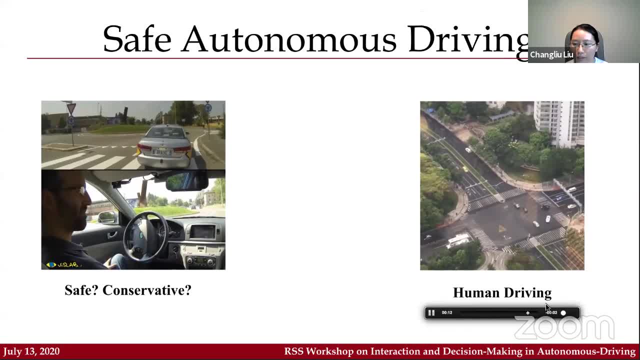 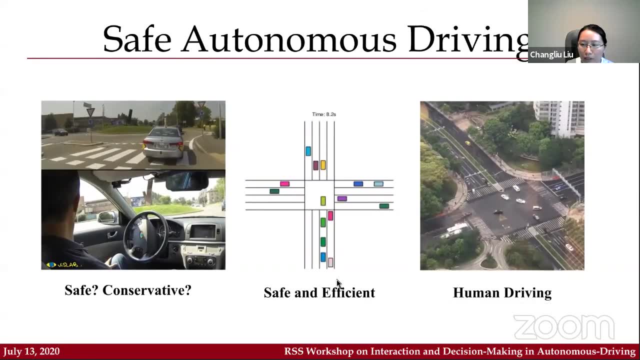 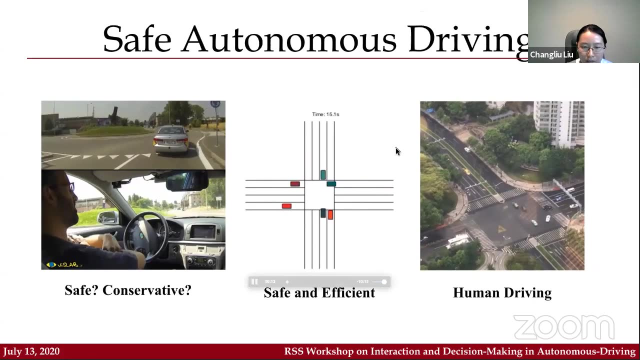 Okay, Good point. Now let me screen the recording. So of course, this is the third legal problem with autonomous driving. There's two grooming characteristics. One: we have our own expectations, which is on public traffic. There's all of us. 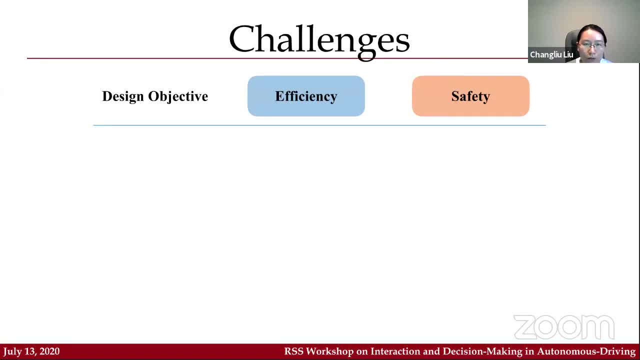 On line. That's good. Am I seeing the jump Yeah About zero as a result of that Gotcha? Okay, So let's go ahead. This one isiblest make their behavior safe and the other is within the safety bound. we want to make their behavior. 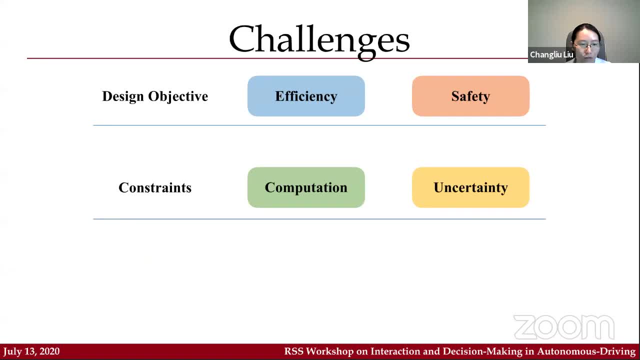 as efficient as possible and doing the design. what are the constraints we have? so the first constraint we have is the computation constraint. usually those autonomous vehicles will not have super power, super computation power to reason about all the possible features, features, um. so then there is a computation limit to um ask. we need to make sure that the autonomous vehicle 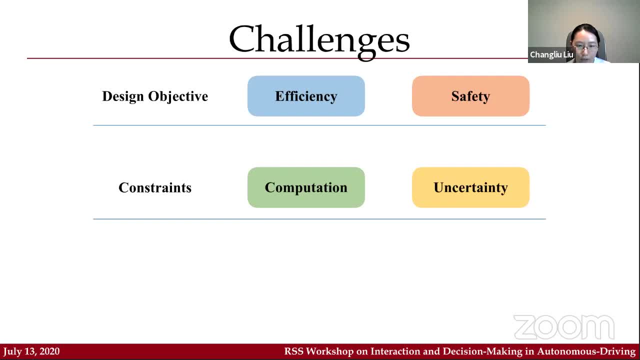 can compute a desired result as soon as possible and generate response in real time under the limited computation power. and then the second constraint is about the uncertainties. there are a lot of uncertainties when the autonomous vehicle drive on public road. it needs to interact with other road participants, including human driver, human driven vehicles. 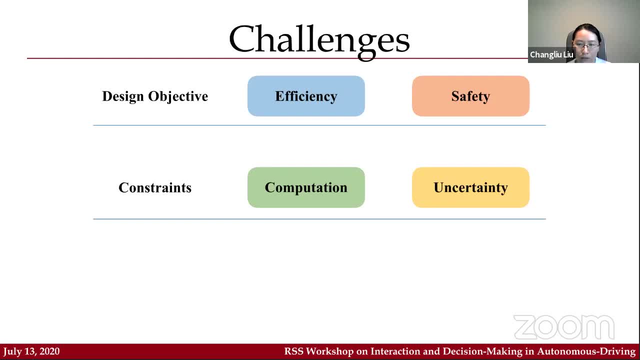 as well as pedestrians, and those uncertainties will complicate the interaction um in the autonomous driving, as well as making it hard to achieve safety and efficiency. so the overall research problem that we are addressing is how can we design the behavior of autonomous vehicles in those dynamic and certain environments under 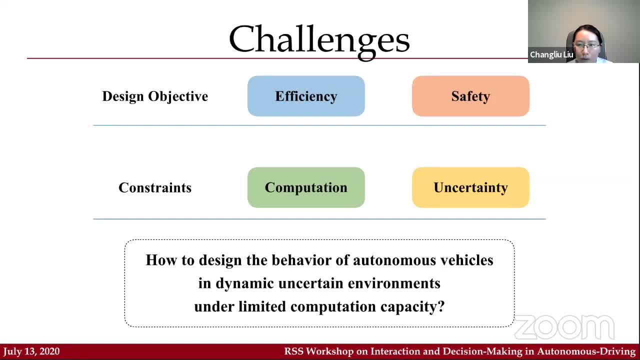 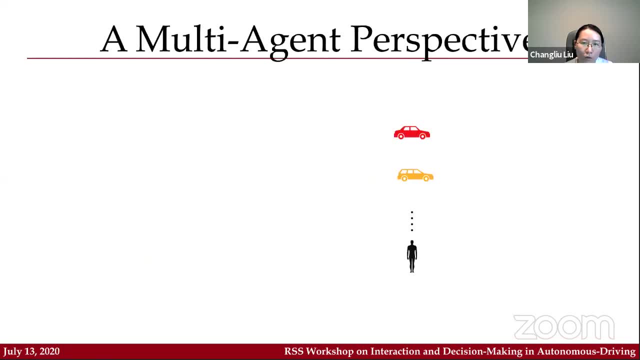 those limited computation capacity in order to maintain safety while maximizing efficiency. and before we look at several ways for us to um do the design, let's first try to understand um the system or the environment the autonomous vehicles are driving in from a multi-agent perspective. oops, i don't have my cursor. okay, so suppose, um our system, um the autonomous vehicle, that 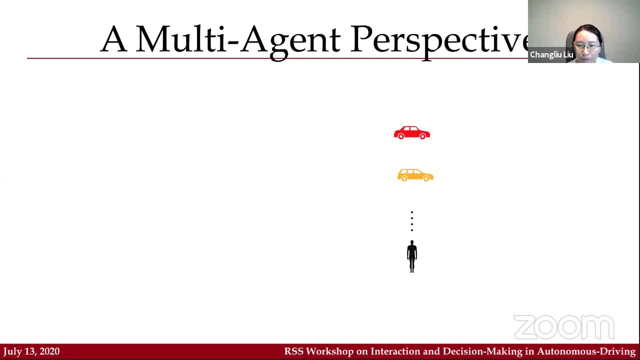 we design for is this red vehicle, and it is surrounded by many other vehicles, including the yellow one, and some pedestrians. and, uh, all the vehicles and the pedestrians can be viewed as agents and they have their own dynamics. the red vehicle has its sensors to sense the states of the others and then 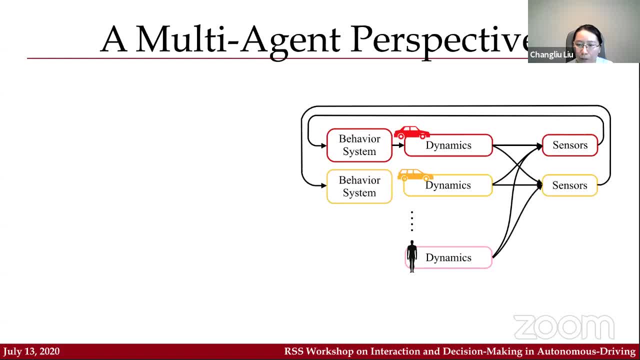 make decisions based on the sensory information. meanwhile, all the other human driven vehicles- autonomous vehicles or pedestrians- have their own sensors to sense each other and then make corresponding driving decisions or movement decisions. So the design objective for us is to specify the behavior system for the ego vehicle that 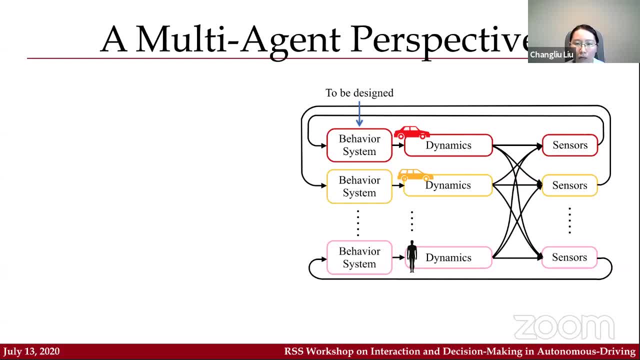 we care about, that is the red one, And when we talk about a behavior system, what we are mentioning is that mapping from the data received from the sensors to the action that will be applied to the physical hardware, that is, the vehicle in this case. 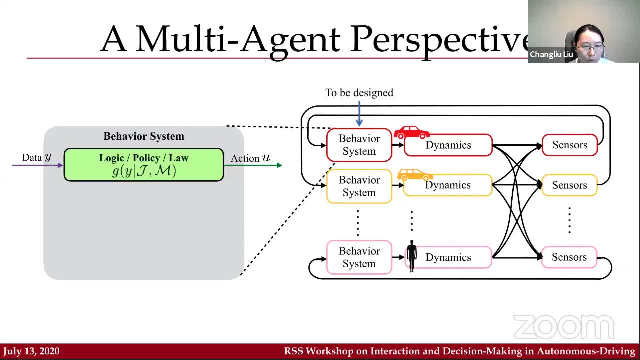 And usually for this behavior system, we will first have a logic or policy or control law that maps the received data to the action which minimize a cost function given a model, And we call the cost and the model as the knowledge. So minimizing a cost is actually equivalent to maximizing the reward. 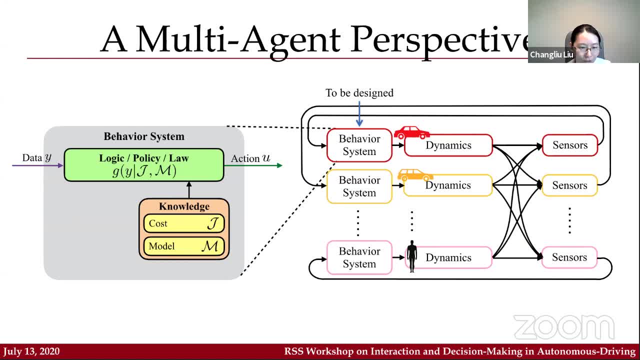 These are just different fields use different names: Control people tend to use cost and the AI people tend to use reward. But those knowledges- it's difficult to fully specify the knowledges offline and then apply them to the online driving, because there can be unexpected scenarios. 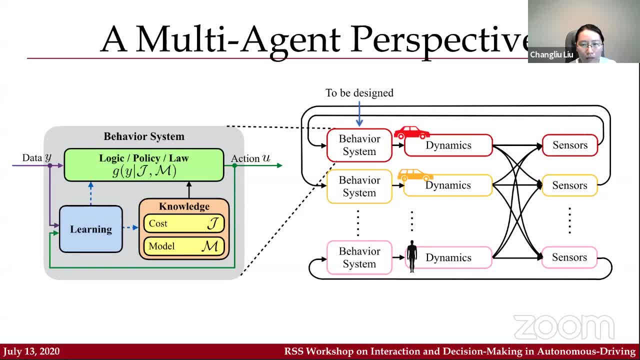 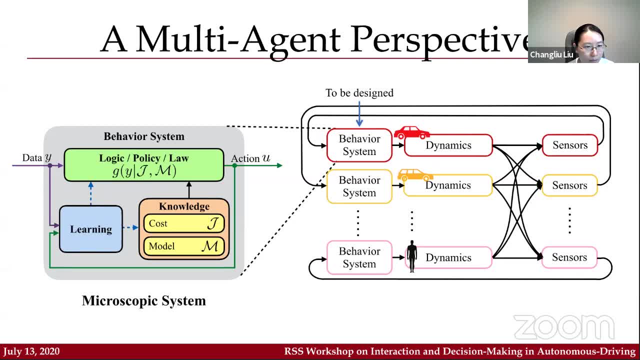 And I think it's really important to characterize the systems that the autonomous vehicles lie in. We always call the behavior system, that is, the kind of the controller or decision-making center for the – for a single vehicle, as the microscopic system, While we call the multi-vehicle system or the transportation system as the microscopic. 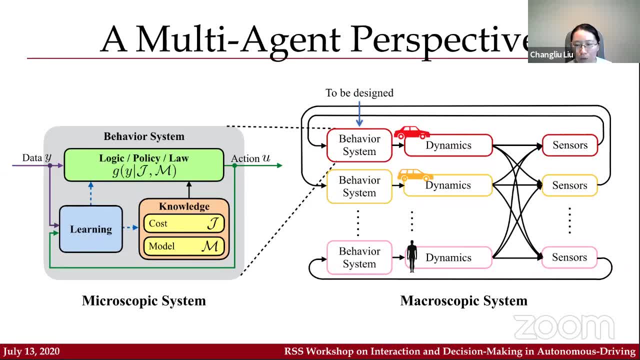 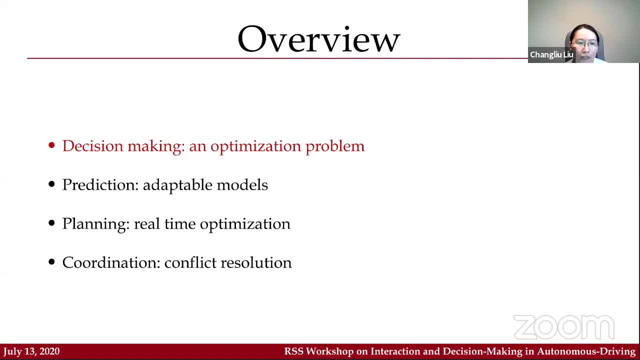 system which involves a lot of dynamic – physical dynamic systems, as well as their associated behavior systems. So in today's talk we are going to first post the decision-making problem as an optimization and then talk about how we can ensure the, how we can design the behavior of the autonomous. 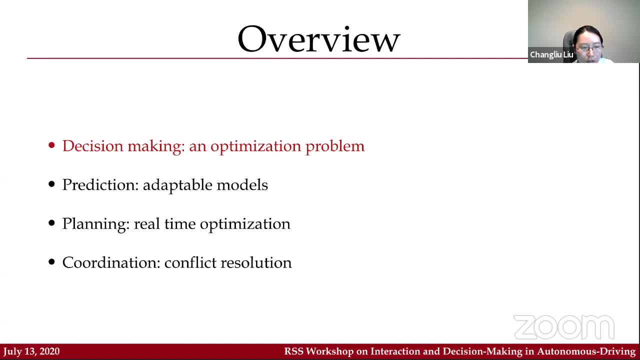 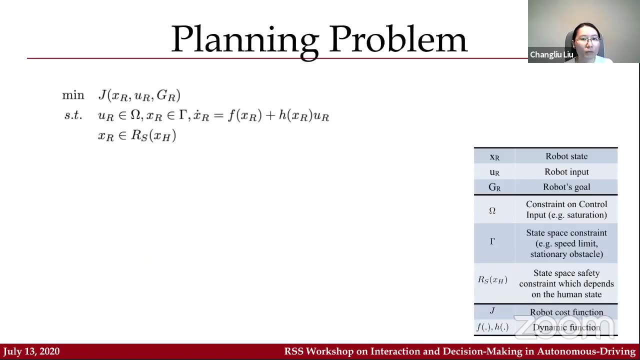 vehicle through prediction, planning and coordination in order to maximize the efficiency while guarantee safety under the uncertainty of the interaction as well as the computational limits. So we formed a planning problem as the following: optimization where let's see where we minimize a cost, function for task performance and motion efficiency. 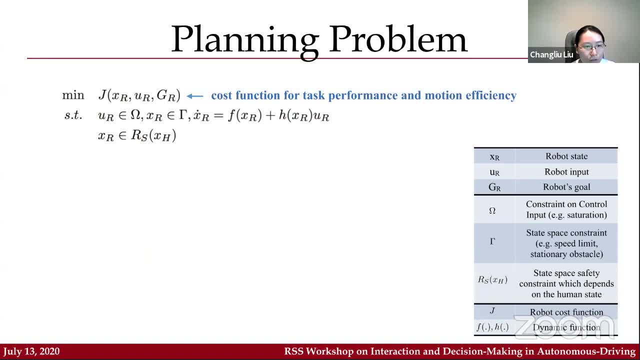 So in this slide are: the subscript R refers to the ECO vehicle and the subscript H refers to the surrounding road participants. So for the planning problem, planning problem for the ego vehicle, we have a bunch of constraints. the first line of constraints correspond to the dynamic and feasibility constraints which we have. constraint on the 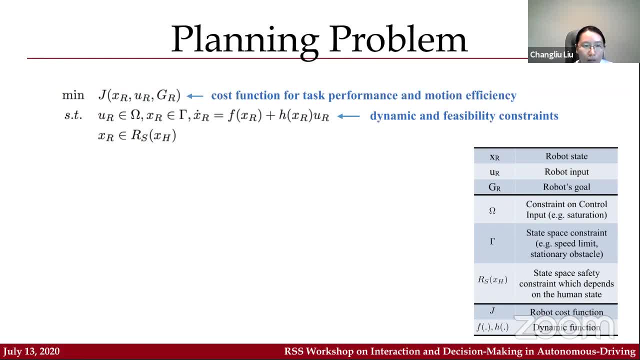 control constraint on the state, as well as the dynamics, as an ode here. then the last constraint is interesting. we want, while the autonomous vehicle is driving on public roads, we want it to interact safely with others. so then, the last one is the safety constraint during this interaction. 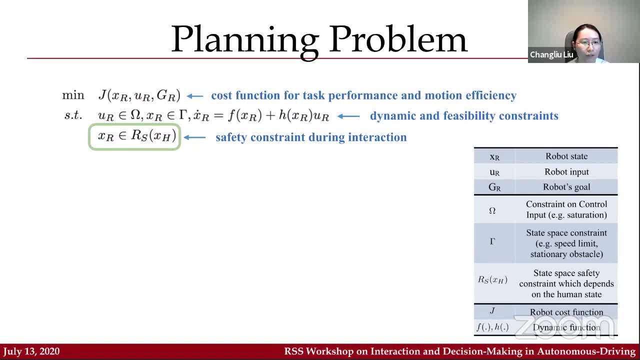 xh is the state of all the other road participants. we want the ego robot's state to be within a safe set with respect to the state of others. so if we look at the following situation: if the gray part gray vehicle is the ego vehicle, the yellow vehicle is and the surrounding vehicle we want 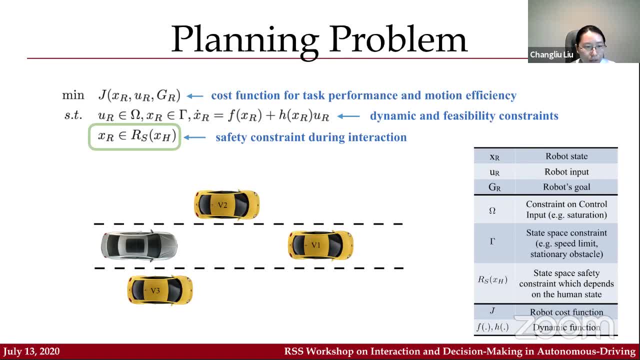 to make sure the gray vehicle will never collide with the others. so this can. safety constraint is the state of all the other road participants. we want the ego robot's state to be within a safe. it's actually very difficult to deal with because we have model uncertainties and also sensor noises. 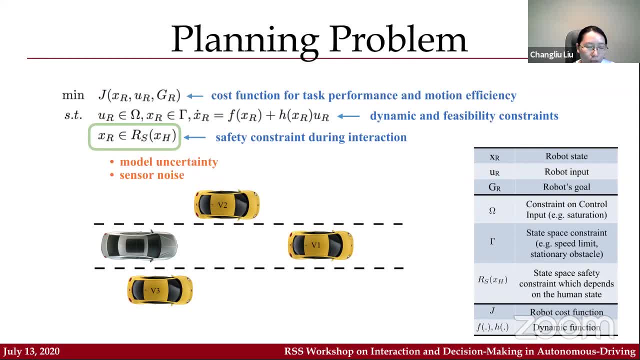 that means we cannot fully correctly predict the future behaviors of others, and if we want to solve this problem in a long time horizon, the accumulation of the uncertainty will make the behavior of the ego vehicle very conservative, and let's look at one example why this happens. so in this example, we want the robot. 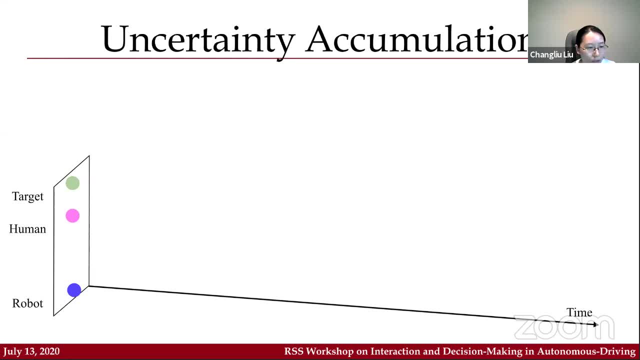 to go to its target while avoiding this human in this confined space. so what the robot will do is first predict the human trajectory, together with some uncertainty, and then plant's own trajectory as this yellow curve here, then execute this trajectory while observing the human trajectory as showing the black curve here. then, in the next step, the robot repeats the whole process. 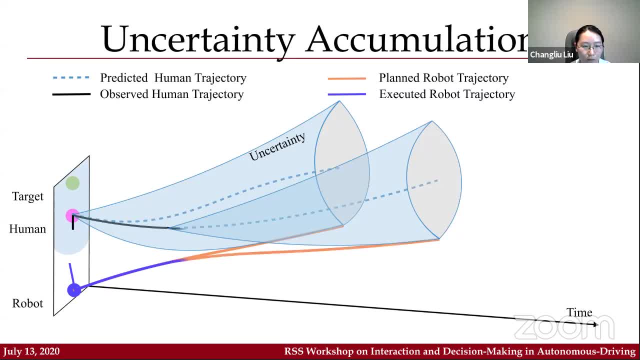 predict the human trajectory with some uncertainty, and then plant's own trajectory, and then execute it, so the robot can repeat this process again and again. but this actually does not help the robot get any closer to the target, as it is almost terrified by the uncertainty in the prediction. 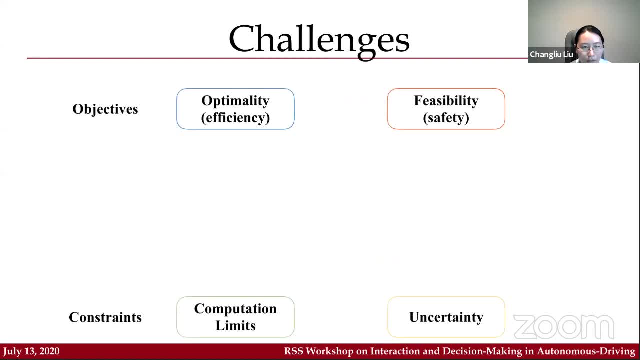 of human behavior and what is going wrong here. let's go back to our previous design objectives and constraints. so we have first objective to that is to be optimal and also efficient. if we want to be optimal, then we need- actually need to do long-term, long-term horizon planning, because otherwise it is very easy for the robot to be trapped into local 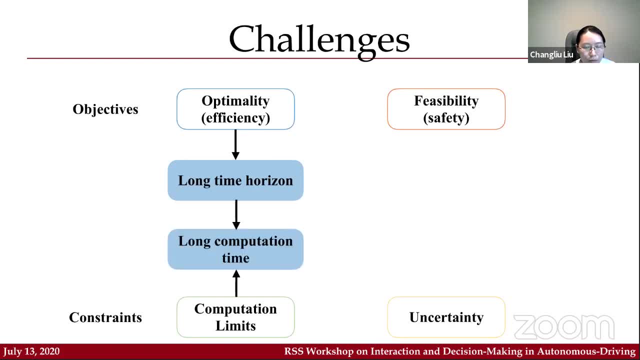 optima, but then under computation constraints. if we do long-term horizon planning, that means we need long computation time and since there are uncertainties, long computation time means there will be larger uncertainty accumulation. and since we want to also maintain feasibility, that is, the safety of the system, then larger 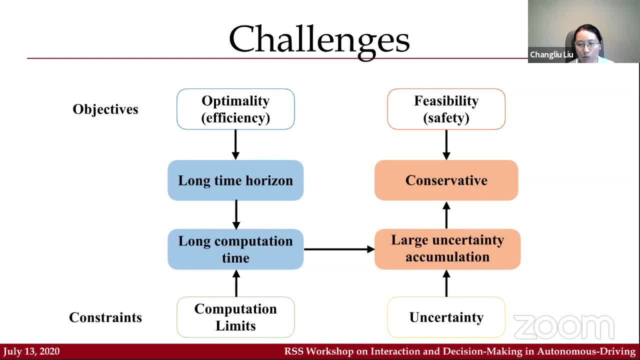 uncertainty accumulation requires us to be conservative in our motion planning, and then this directly contradicts with our optimality pole. okay, but how can we solve this paradox? there are a bunch of ways to solve it. for example, we can release some of the constraints, increase the computation- uh, improve the computation power so that we can compute faster. 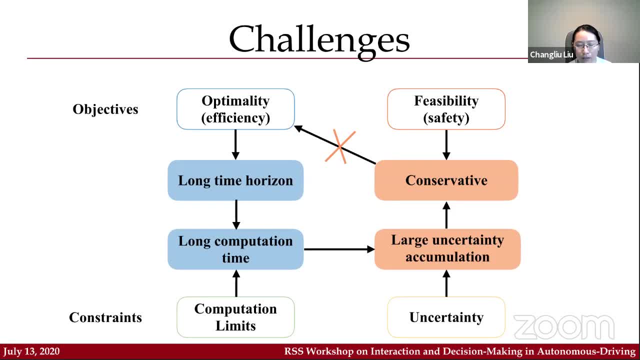 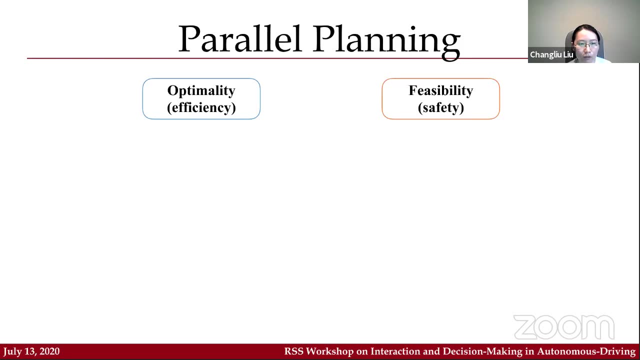 or improve our prediction so that we can have less uncertainties. so the first approach we'll talk about here is to, instead of addressing this planning problem in a single scheme, we can address the problem in a parallel scheme. that is, we have planners to address different objectives, so in this case we can have a efficiency controller to address the 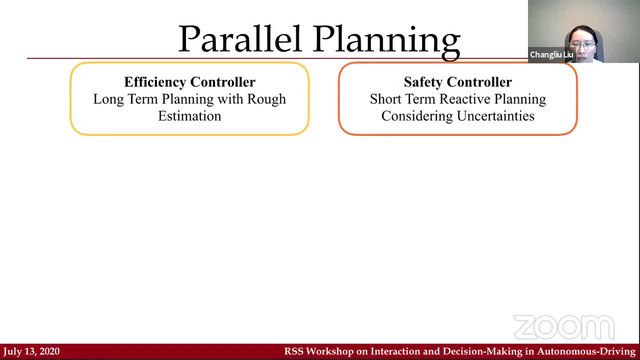 optimality goal and then a safety controller to address the feasibility goal. how does it work? the efficiency controller now only considers the rough estimation of the human without uncertainty, while the safety controller will consider all the uncertainties in the short term and do reactive replanning. so, using the previous example, the human will still generate, the robot will still generate. 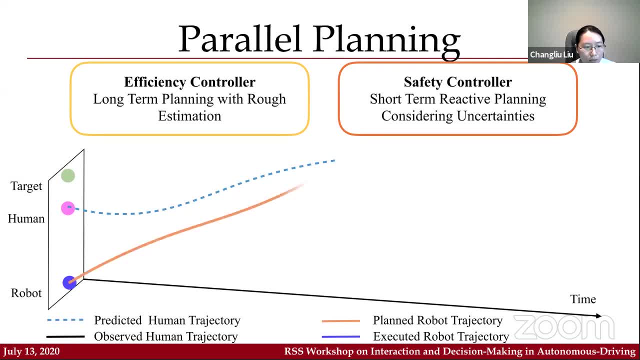 a prediction for the human in the efficiency controller, but this time the robot will plan a trajectory without worrying about the like accumulation of uncertainty in the long term. then this long-term trajectory will be sent to the safety controller for monitoring. in the first time step, in the safety controller, the uncertainty of the human behavior will be predicted, and then 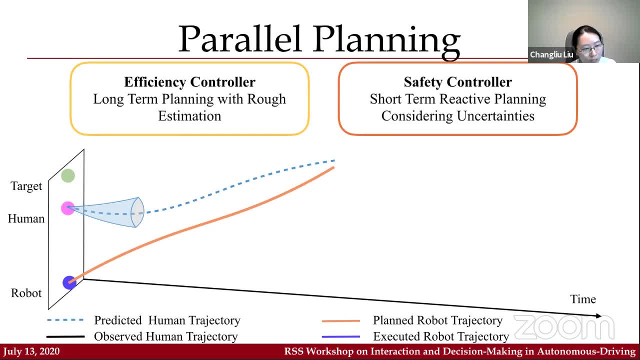 the short-term safety controller will check whether the long-term plan is safe to be executed or not with respect to the human uncertainty. in this case it is safe, so then the long-term plan is executed. in the next time step the long-term plan actually intersects with the uncertainty coin, so it's not safe anymore to execute. then the safety controller generally 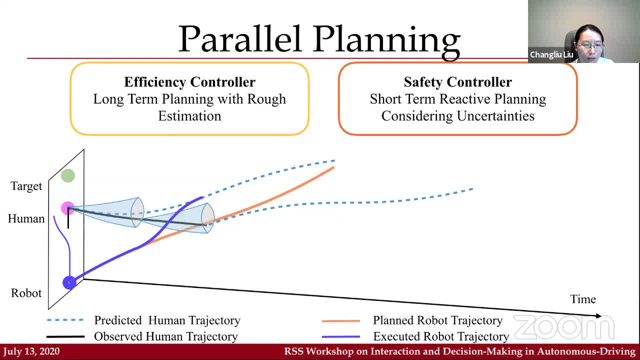 a detour. Meanwhile, the efficiency controller will generate a new prediction of the human and then a new plan for the long term and overrides the old long-term plan. Then the safety controller will monitor the new long-term plan and it will safely guide the robot towards. 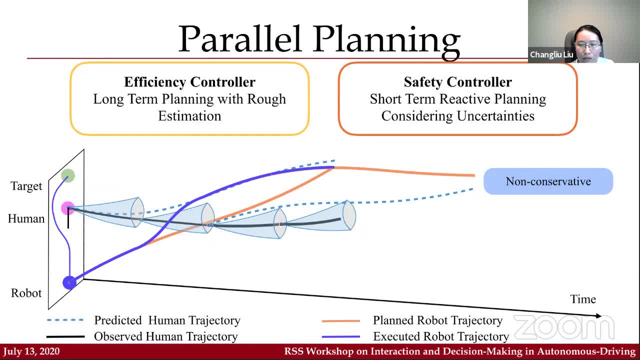 the target. So this approach is non-conservative as compared to the previous one. It also avoids the local optimal problem that a lot of this reactive or short-term planner may have, since we still have a long-term guidance and, in this case, since we have the safety controller, the 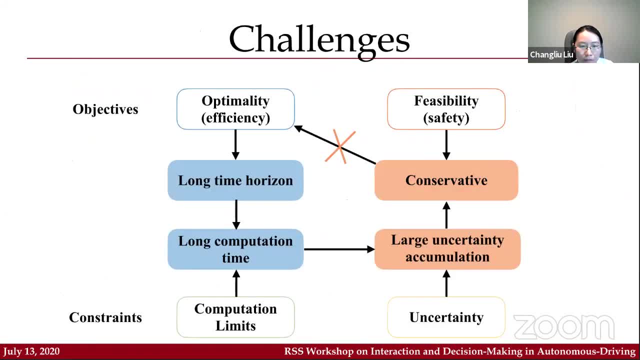 uncertainty is still addressed, but in the short term. Okay, so that's one way to address this paradox, and later we are going to talk about the other two ways. First is to improve our prediction to reduce uncertainty, and the second is to design better algorithms so that we can solve. 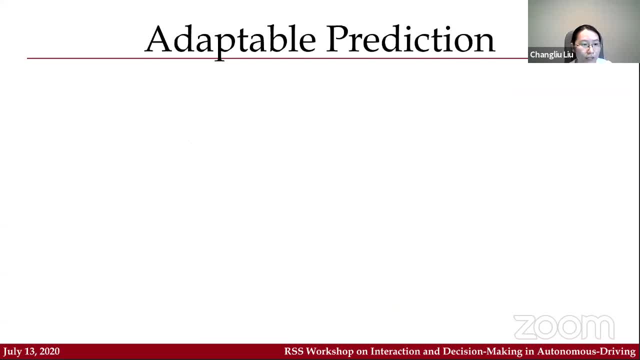 the optimization faster. Okay, so for prediction, there are a lot of methods to predict surrounding vehicles, as also we've seen a lot of methods in the previous sessions, and that a good prediction can help us improve the safety level of the autonomous vehicles and we can learn those. 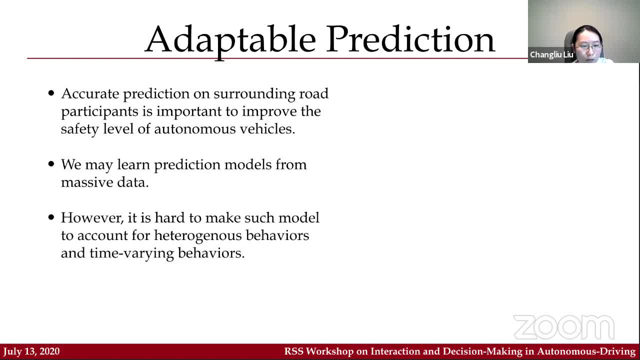 prediction models from massive amount of data, but the problem is that it's very hard to make such model account for. And we can learn those prediction models from massive amount of data, but the problem is that it's very hard to make such model account for. 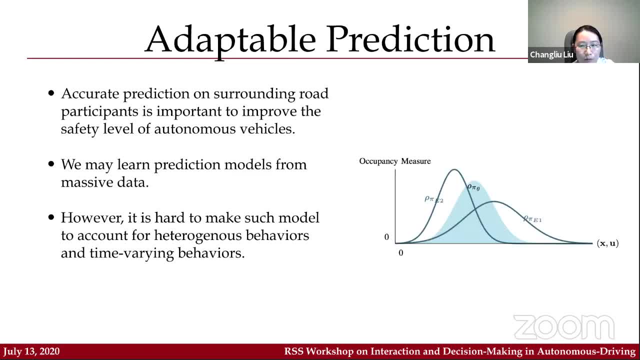 for heterogeneous behaviors or time-varying behaviors. So in a lot of cases we might have different distributions in the occupancy measure, but in the end, while we are doing this massive amount of training, we actually average out those distributions And by doing that we are actually reducing. 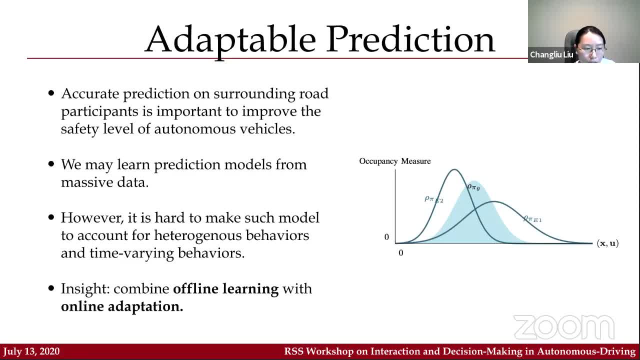 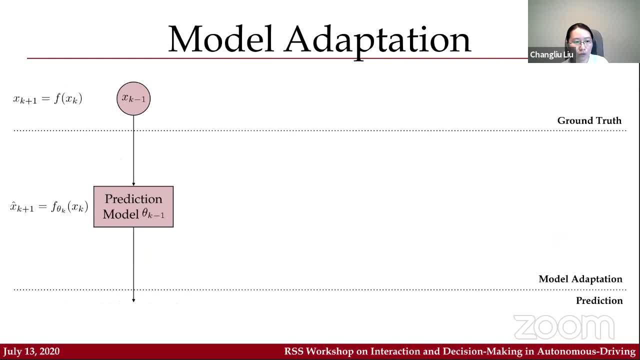 the accuracy of our prediction. So how can we mitigate that? The insight we have is to combine offline learning with online adaptation. And how does it work? So suppose we want to predict a system that has the dynamics xk plus one equal to fxk. 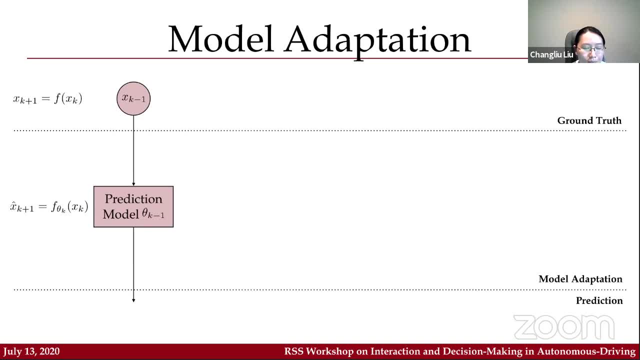 Then we build up prediction model f, theta, k, with parameter theta And as the ground truth evolves, we cannot observe the true function, but we can observe the state, And every time when we make a prediction we'll compare it in the next time step. 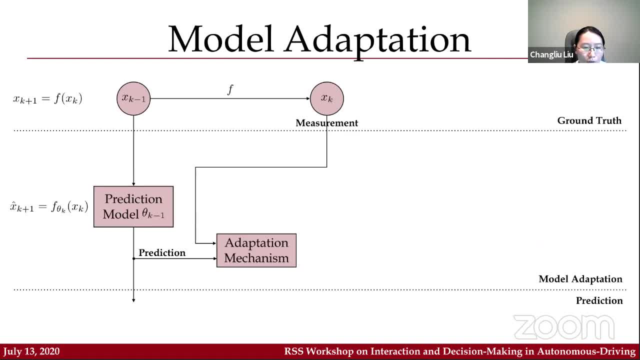 with the true measurement and see how big is the error, And then use an adaptation algorithm to modify the model parameter in the next time step And then use the new modified model parameter for the new prediction and keep this process again and again. In this way we can make sure that our prediction model 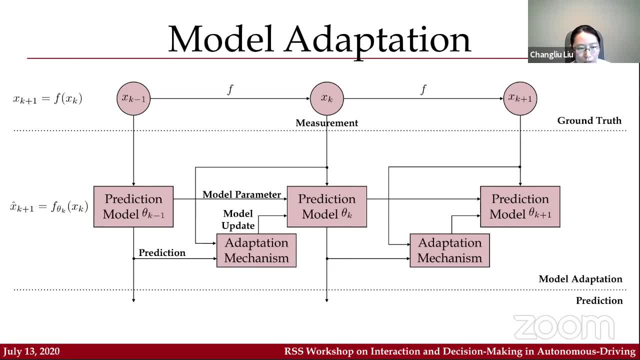 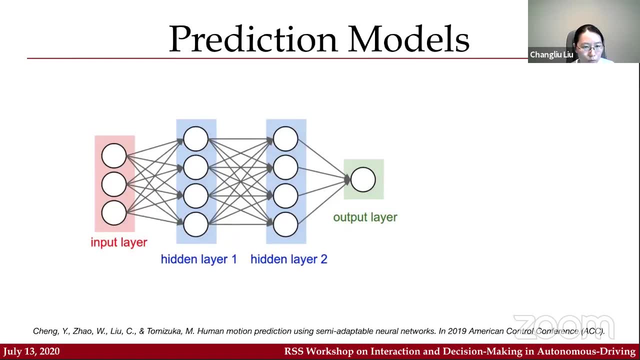 is locally overfit to the data, so that we can reduce the prediction error. And in terms of the prediction model, which is a function that we use for the prediction, we can use different kinds of prediction models. We can use different kinds of functions. 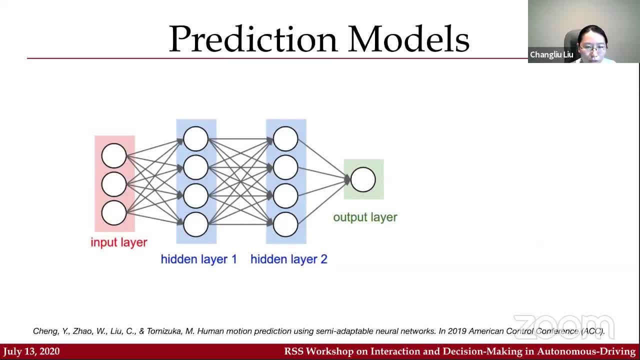 For example, here we use a neural network, but neural network has a bunch of a lot of parameters. It is unnecessary to adapt all of them online, So usually what we do is to regard the first few layers of the network as feature extractors. 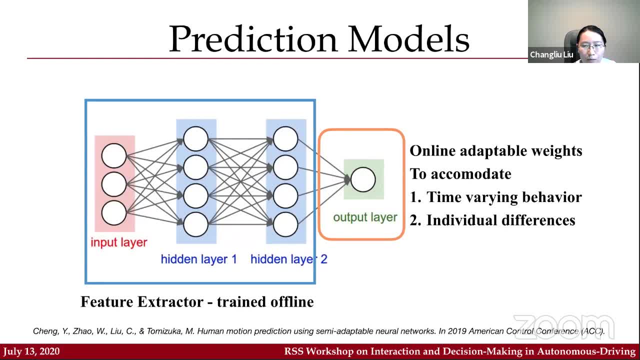 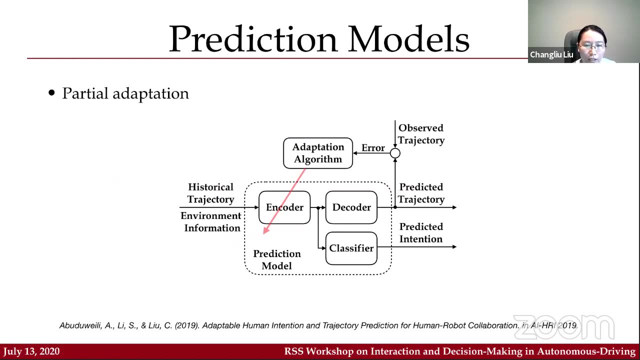 and then only regard the last few layers as online adaptable parameters which can help us adapt the high level features to better fit time, varying behaviors and individual differences, And even if we don't have real time labeled data, for example, if we want to predict intention. 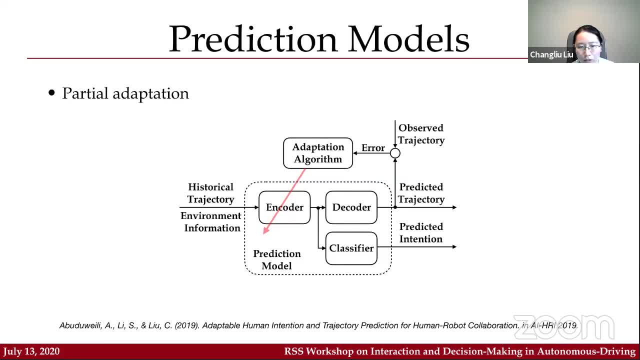 then it's very hard to have labeled intention in real time for us to adapt the prediction model. Then we can develop multitask model and use the available data, for example trajectories, to adapt common parts in this model so that we can generate real time adaptation. 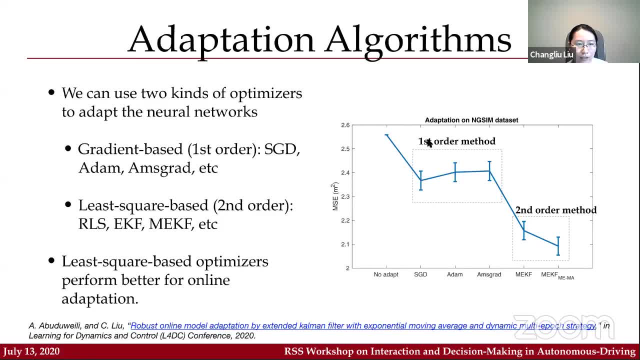 for those unlabeled data In real time And also for the adaptation algorithms. there are a bunch of ways to do the real adaptation. Actually, the adaptation is similar to the offline training, So definitely we can use gradient based method, which is also called first-order method, for the adaptation. 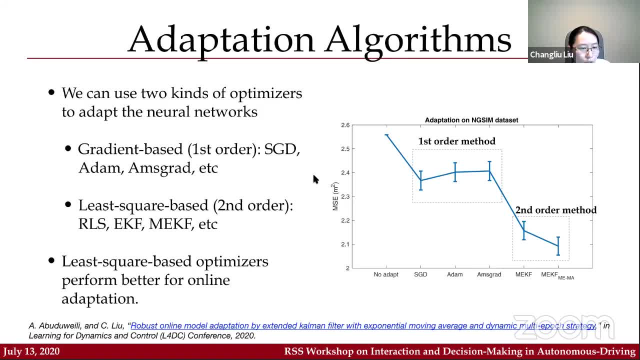 as well as second-order method, that is, least square based method for adaptation. So although first-order method has demonstrate great success in the offline training, actually for online adaptation, we see that least square or second-order methods perform much better than the first-order method. 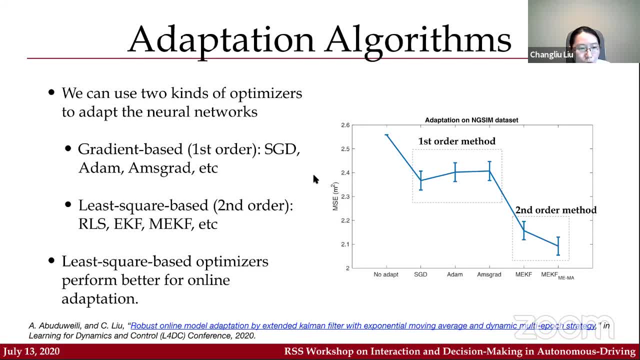 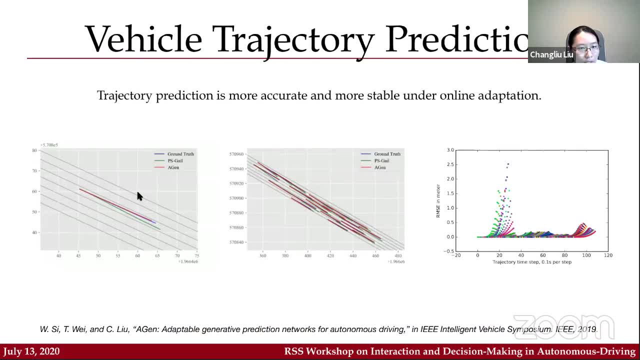 One reason is that for online adaptation, we want to explore local overfitting, So then the second-order method will be more efficient here. And here is some data we generate. result we generated for the adaptable prediction for NGC, which is the NGC data set. 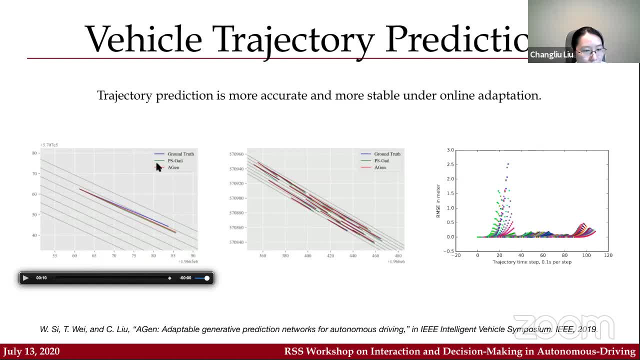 In this case, the blue one is the ground truth And the green one is the offline learning algorithm- PS scale- that we used to generate the prediction model, And then the red one is PS scale plus our adaptation algorithm. As we can see, this adaptable prediction is more accurate. 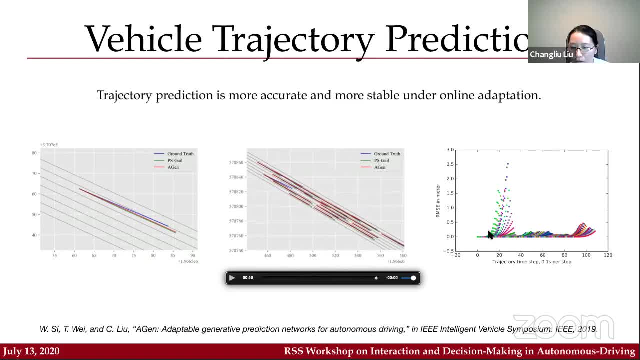 and stable than without this adaptation. And for the errors at different time step, we can see: for the initial predictions, we can see that the initial prediction is more accurate than the result. And for the errors at different time step, we can see: for the initial predictions. 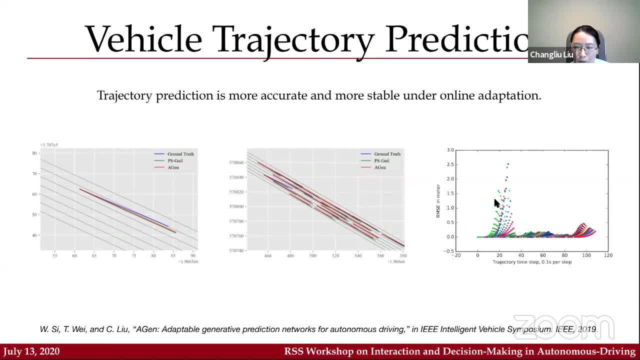 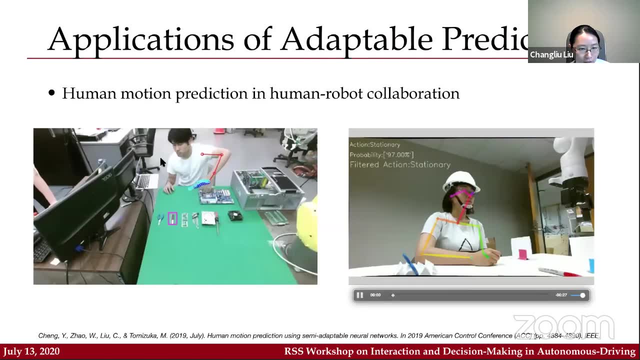 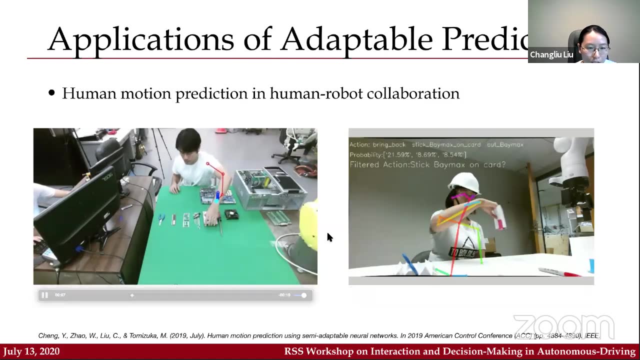 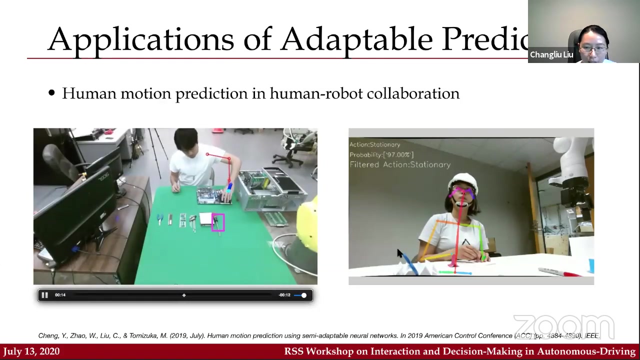 we will have big errors, But after this adaptation, those errors will be minimized as the time moves. Okay, and here are also two other applications of this kind of adaptable prediction in human motion prediction, where similar methods are used as the previous case. 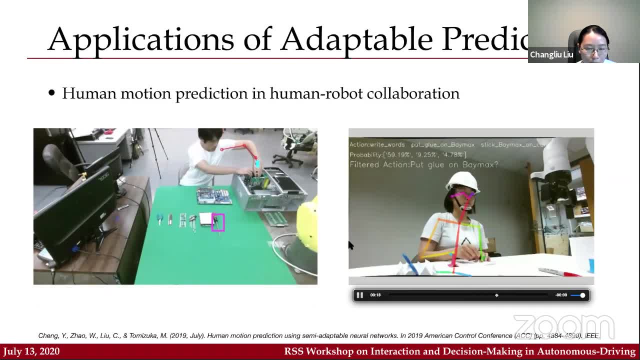 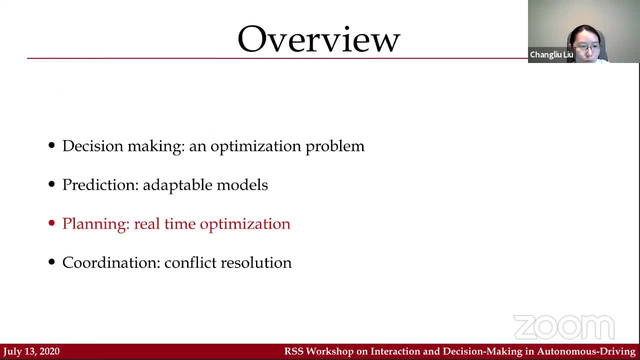 and we can efficiently adapt the human upper limb to the human upper limb, And we can easily understand how to do this with different parameters of objective as well as human intentions. Okay, so that's the prediction side, And then for the planning side, 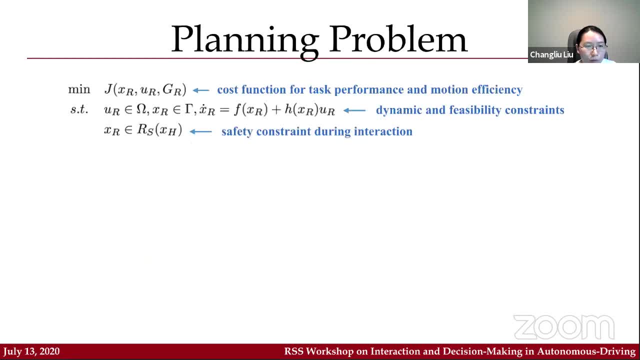 in order to overcome the computation limits, we need to develop efficient optimization algorithms. So this is the optimization we introduced earlier. In order to take advantage of off the shelf optimization solvers, we can discretize the problem into a general nonconvex optimization. 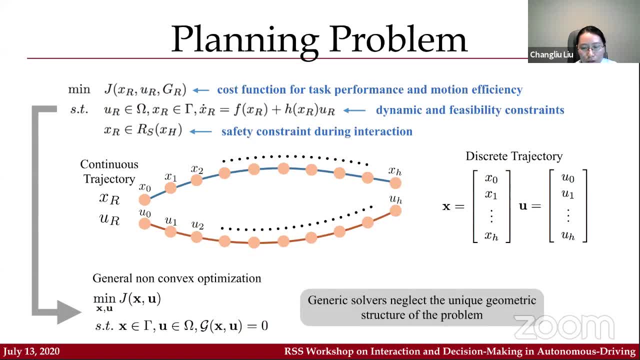 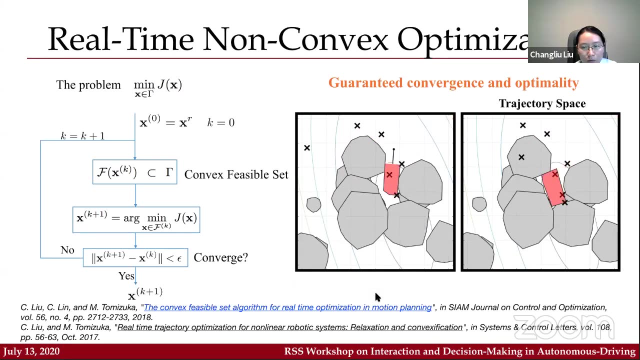 The problem of using off-the-shelf generic solvers is that they usually neglect the unique geometric structures of the problem, so that it will require a lot of time to solve this non-convex optimization. The insight we have is that there are unique structures in the planning problem for autonomous vehicles and we can directly leverage these features in designing optimization algorithms. 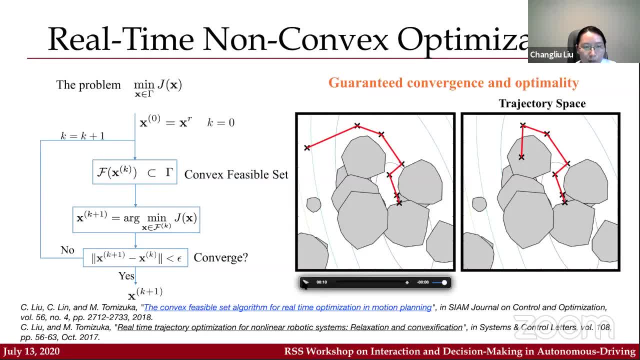 For example, in a lot of cases the non-convex actually only comes from the constraints. So in this way we can locally convexify the problem and then only solve the problem in a convex feasible set and then use iterations to minimize the approximation error during the convexification step. 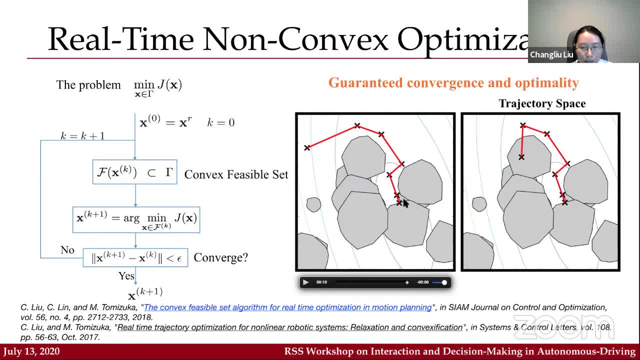 And by doing that we can safely find the optimal, at least a local optimal, and this method has guaranteed convergence. But this animation here is just illustrating, like a simplified 2D space, What is going on in the trajectory space is like that: 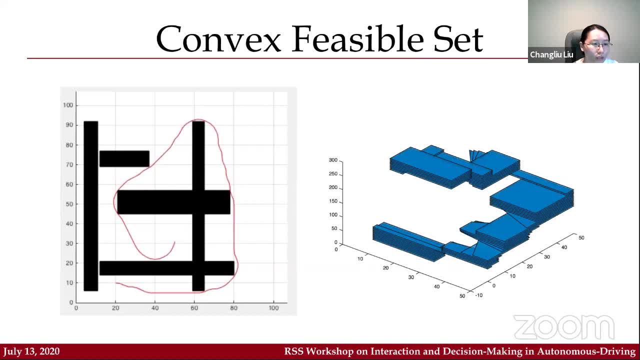 Suppose we want to navigate through this maze following a reference trajectory, but we want to enlarge the safe margin of this reference trajectory, Then we first need to convexify the whole problem by generating a convex tube around the reference trajectory And finally the computed convex tube. 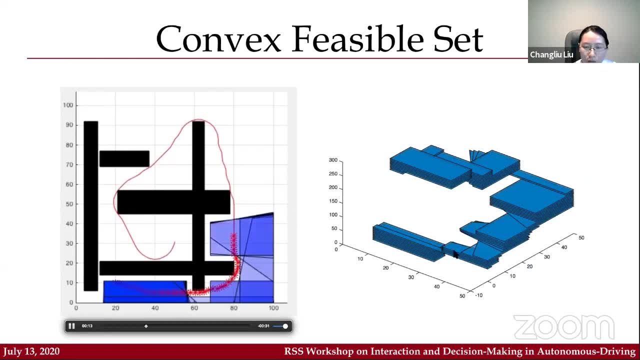 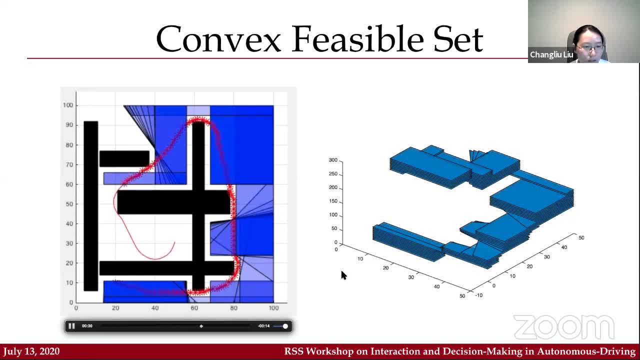 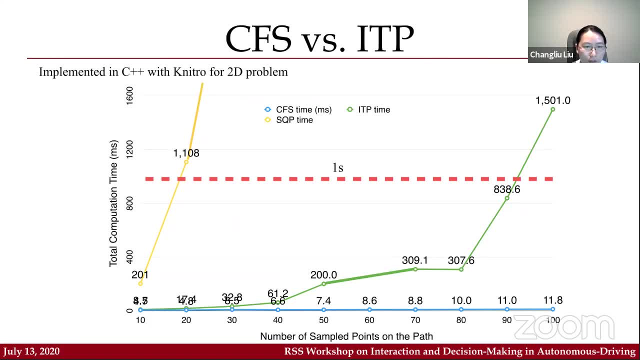 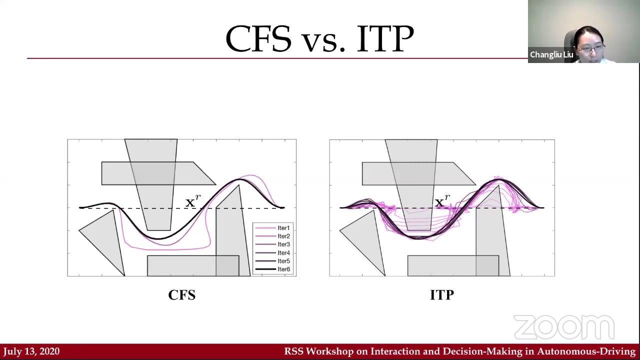 And after that it's computationally efficient for us to get a solution And we have compared this convex feasible set method with other off-the-shelf methods And it has demonstrated great efficiency compared with others And for the trajectories generated by CFS. for every iteration it is actually smooth. 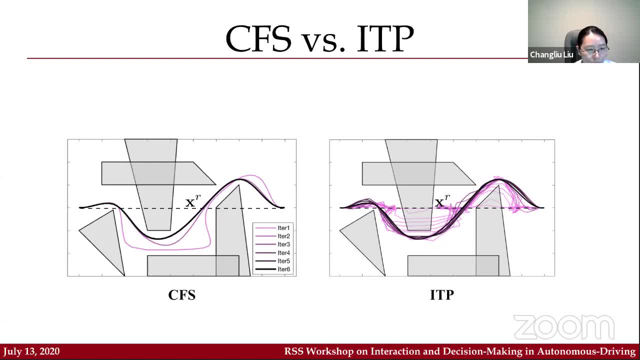 and it only takes one iteration to make our reference trajectory. in this case, it's the dashed line, which is infeasible to make an infeasible reference to be feasible, which is this light pink curve. which is this light pink curve? 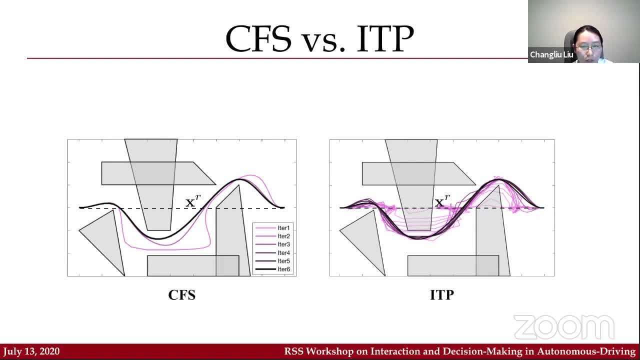 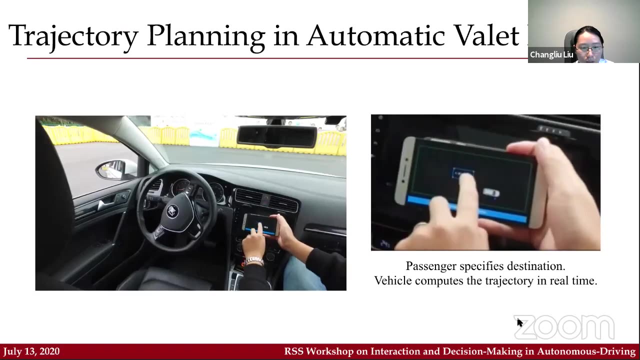 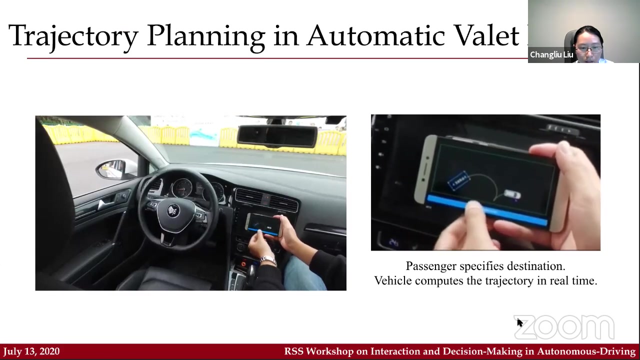 And then five iterations to converge to the optimal trajectory, while the off-the-shelf interior point method takes a bunch of iterations to make the trajectory feasible and even more iterations to converge to the optimal trajectory. Yeah, we have applied this method to a passenger-vehicle interaction case where we allow our passenger to specify a target location And then just by one click we can generate a trajectory in real time to drive the vehicle towards the target. 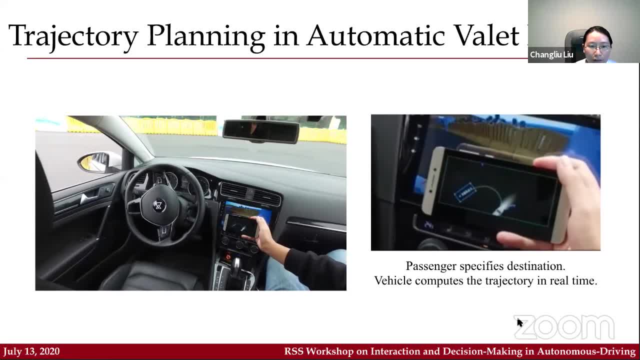 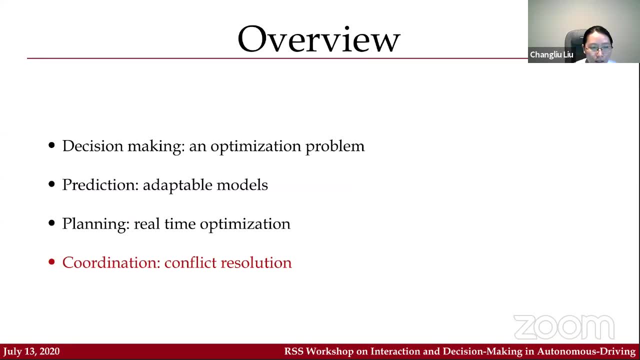 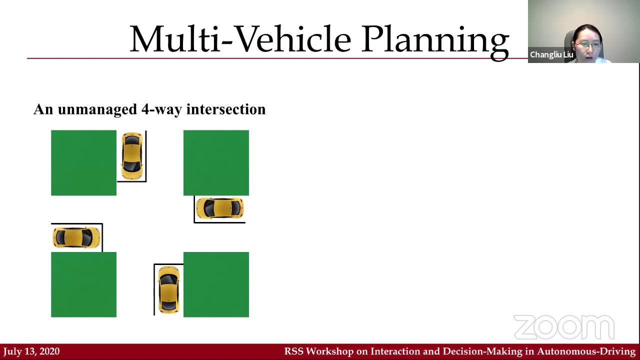 And this can be applied to automatic valet parking. Okay, so the last thing is about coordination. So if we designate a vehicle for a target location, we can generate a trajectory in real time, But if we design the behavior of a single vehicle, this actually also can not solve all the problems. 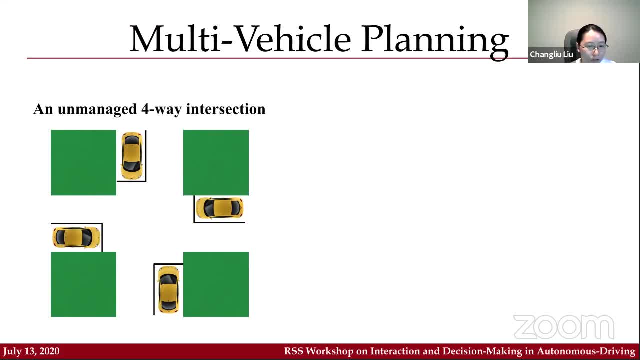 For example, if the four vehicles here are all autonomous vehicles and they arrive at the uncontrolled intersection at the same time, so there's no priority among those vehicles. If the behavior of those vehicles are designed samely, they will inch forward to test the response of others, and if others yell, they will stop, If others don't, they will just go. 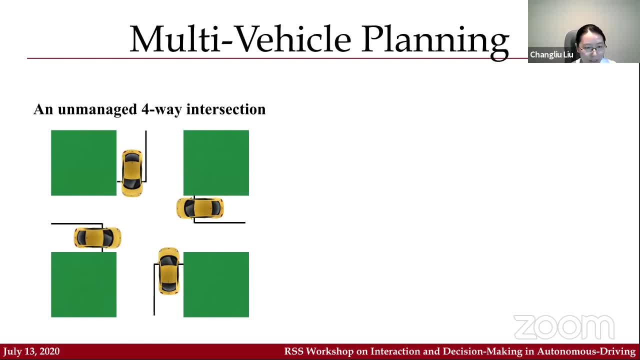 If all the four vehicles do the same thing, then the whole system may be trapped into this yell stop and then yell stop loop. And in order to solve this problem, we actually need to introduce communication and coordination of those vehicles to allow them to figure out the passing order before they actually get into the intersection, as shown here. 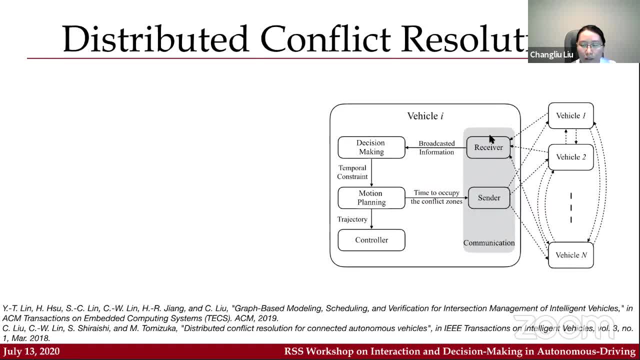 And technically how it works. This is by building a communication module for all the vehicles which it can send information to And then, when the vehicle is passing, it can send information to the other vehicle and the receive information. But we are not requiring other vehicle. 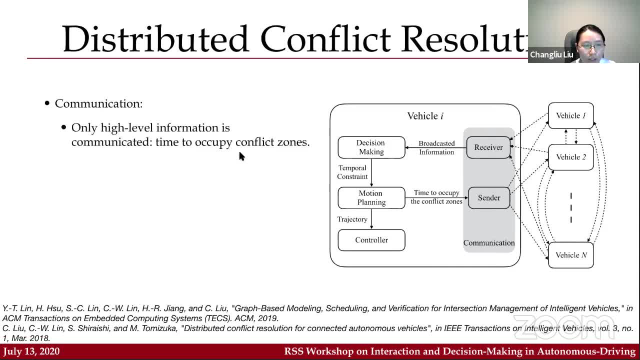 to communicate very detailed information. Only high-level information is communicated, For example the time to occupy the conflict zone or the intersection, And the dis-communicated information can substitute the prediction module in the individual vehicles And we can directly use the communicated information. 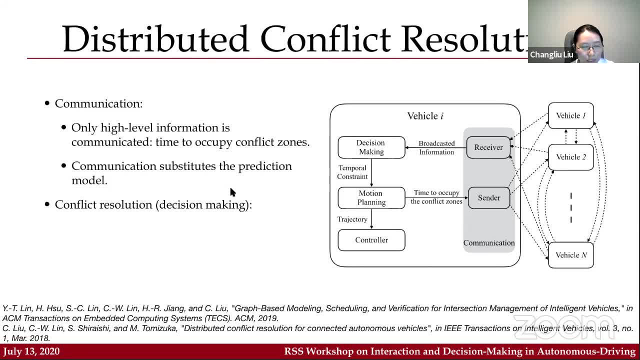 as the constraints in our motion planning problem, And after we receive this communication information, then the next step is to do conflict resolution in the decision-making module. It correspond to solve a conflict graph based on all the information received from others And if all the agents are using. 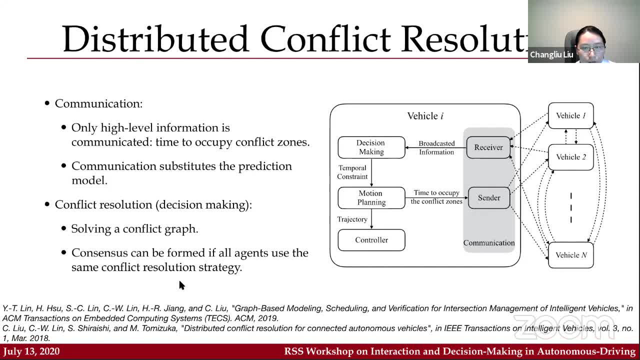 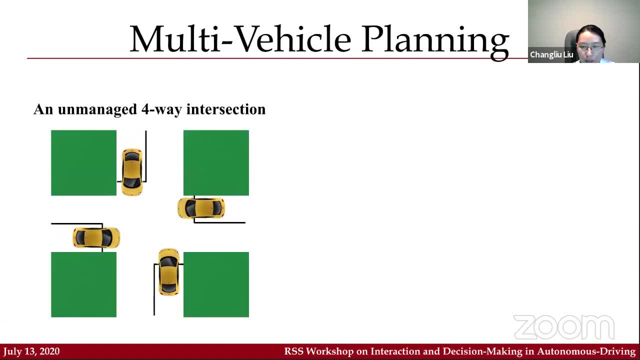 the same conflict resolution strategy we can form a consensus among all the agents And then the animated situation in the last slide has shown here. So we see that in the last slide is theGH-N of the conditions that the vehicles find the conflict and then the other areas that are facing any conflict. 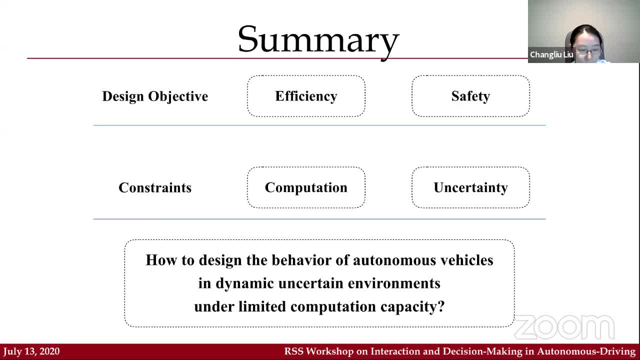 And then there is an indicator, is the opportunity to actually funny which the vehicles can figure out the order to cross the intersection without even stop. Okay, So in a summary, this is the slide we see earlier, other possible futures and also we have a lot of uncertainties during the interaction. 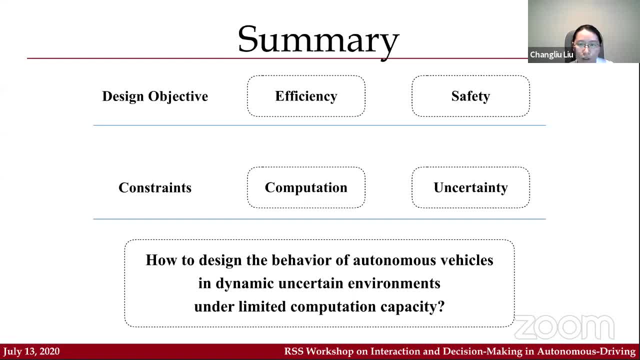 so we discussed different approaches to address these problems. the first approach we discussed is the parallel planning approach, that is, to decouple the planning problem into two planning problems with different sampling frequency. so then we can have the plan: a planner that has low sampling frequency to address the efficiency, and then a planner with high sampling frequency. 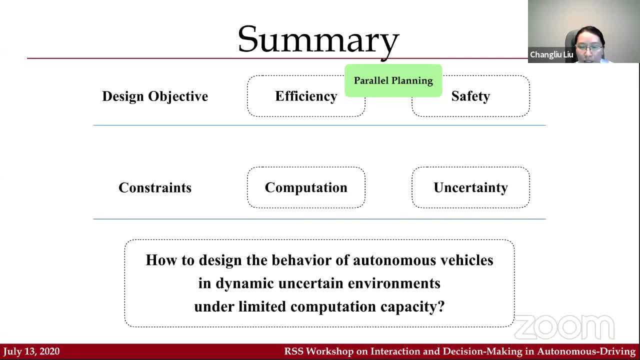 to address the safety with uncertainty. and then we discussed about the prediction method, especially the adaptable prediction models to reduce the uncertainty in the prediction. and then we discussed about the real-time optimization method to make the planning more efficient. that also can help reduce the replanning frequency. 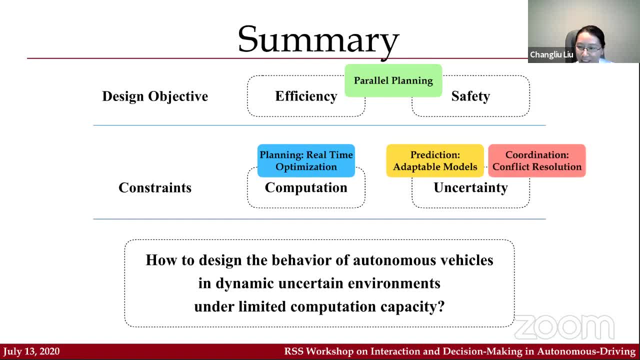 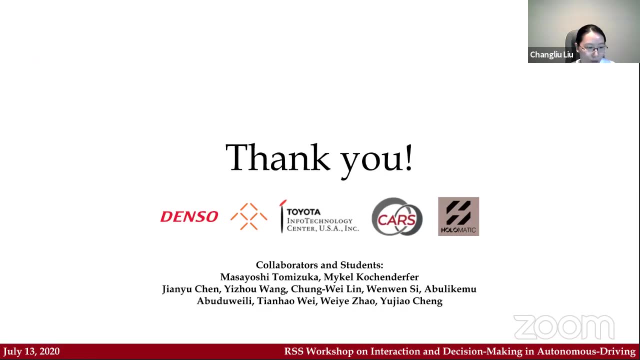 here, increase the replanning frequency. and lastly, we talked about coordination stuff or conflict resolution mechanism. that is also a way to help reduce the uncertainty through communication. okay, so I would like to thank all the sponsors for the work that presented here, and also all the collaborators and the students who contribute to the work. and that's for my presentation. I'm 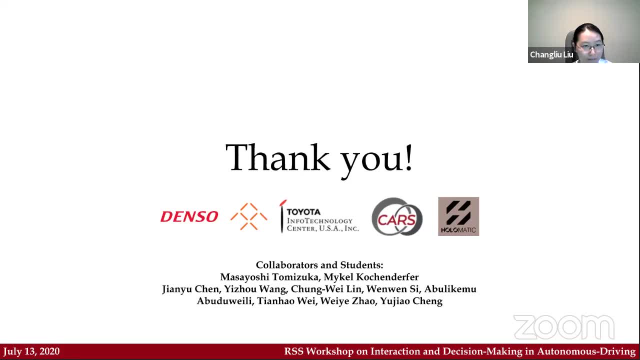 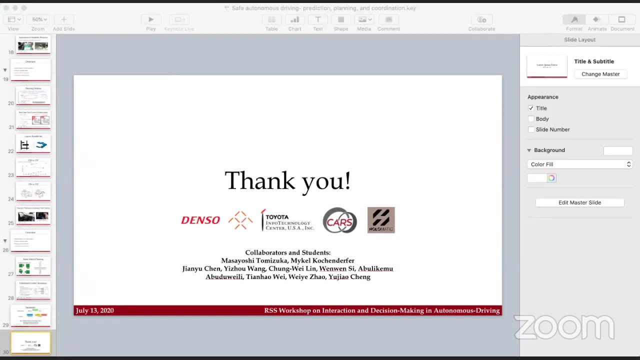 happy to take questions from here. great well, yeah, thank you so much. so if anyone has any questions, and especially for those that have just joined, we're communicating via the zoom chat. so if you, if you have any questions, feel free to just add them. add them into the chat and we'll start reading them off from there. 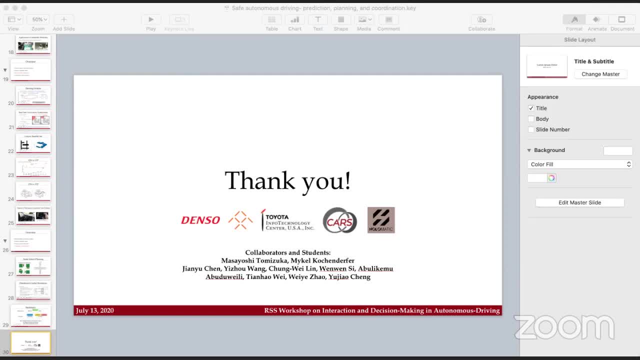 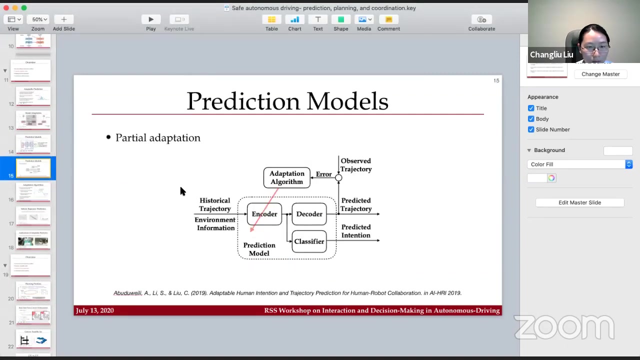 okay. so we have one question here: the, the local online adaptation is interesting. which layers of the network are you adapting? are they also working on multimodal prediction models? yeah, so for here we are adapt. so in this case, for example, we have both prediction for the trajectory and 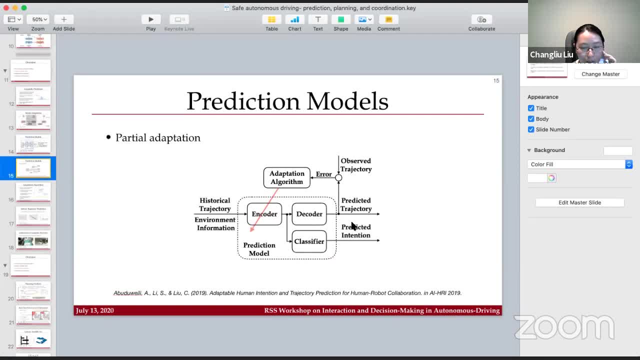 prediction mode, intention. and since we don't have ground choose for intention, we only use the ground choose for trajectory to adapt the common encoder and though we are only adapting the last layer of the encoder, but this means we need to pass the gradients through the decoder and all the way get to the last layer of encoder. 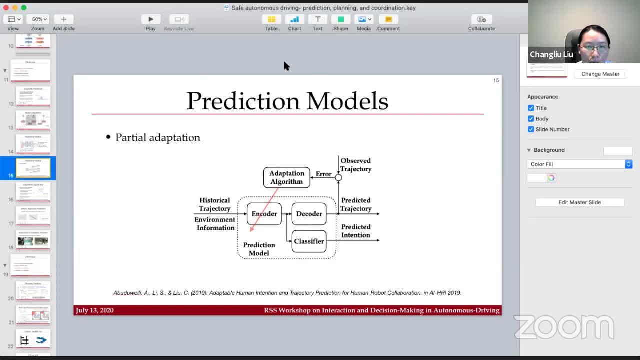 um, for the multi-model predictions, I I don't think, uh, we have any problem applying the adaptation algorithm there, because adaptation algorithm is a kind of an optimizer, as long as your multi-model per multi-model prediction model can be learned offline using, like, say, stochastic gradient descent. 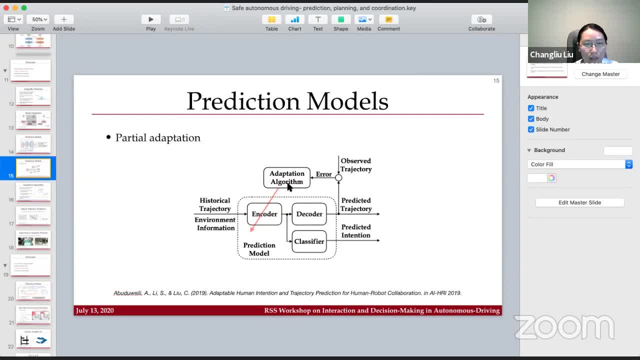 we can then also use stochastic gradient descent for online adaptation. okay, great, uh, and we have uh. so we have a second question here from um ego. so the four-way intersection uh example was cool. uh, what are other scenarios in which you envision uh communication to be required? yeah, I would say in a lot of um conflict. 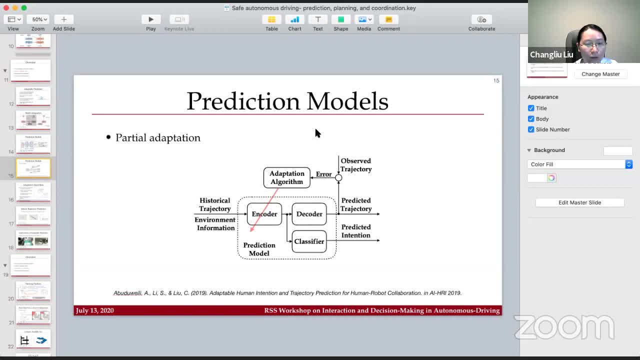 conflicting scenarios, communication would be very helpful, for example, in the merging case. if two vehicles have the same velocity and expect to arrive at the merging point at the same time and there's no explicit priority between the two, then definitely, if we can form a communication mechanism to let them negotiate before they arrive there, it will be very helpful and the 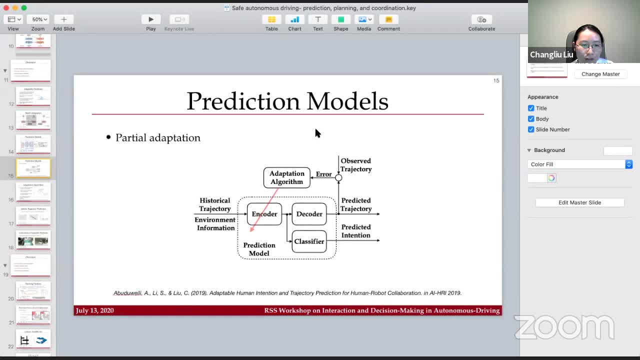 negotiation is actually um kind of a way to move the conflict resolution problem earlier than it occurs in the real physical world. okay, great, um, uh. and then we've got a third question from looking: um, so is adapting the last layer always sufficient to capture the local behavior information? 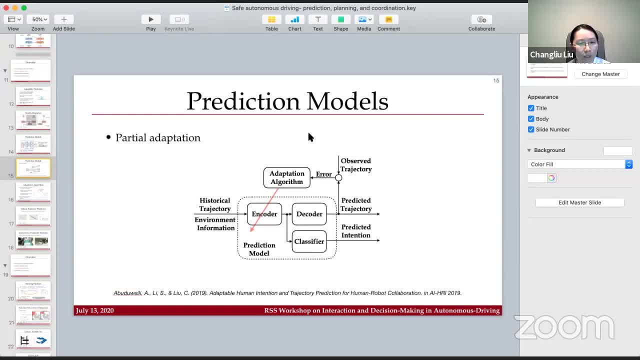 um, in our experiment it is um, but I think that depends on your model. so for our model the input is the trajectory and the output is kind of high level features, um, so that we can use decoders to generate um predicted trajectory and the classifier to classify the intention and in this way um, uh, lower levels of the first few layers of the network is. 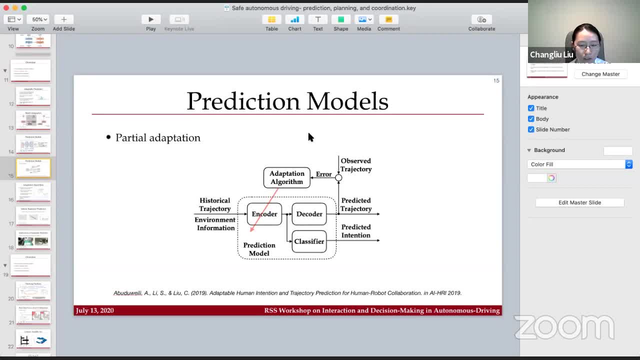 actually getting low level features and the higher level is getting high level features. and um, for a lot of cases and also for human behaviors, their low level features tend to be similar. the differences, and the major differences is always in the high level. so in this way, adapting. 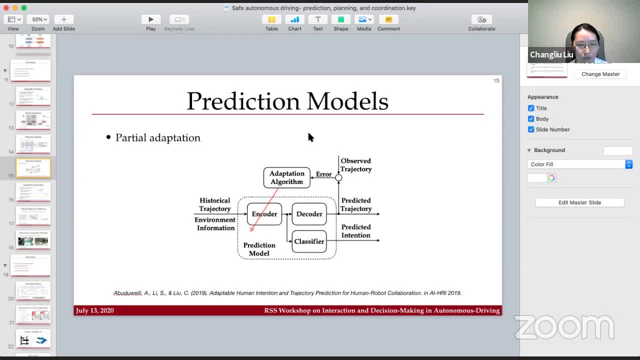 the last layer, or maybe last few layers, is sufficient in our experiment, but there can maybe other cases, maybe not in the human motion prediction domain, that the differences across data is not in a high level feature of a low level feature, and then in this case you need to adapt. 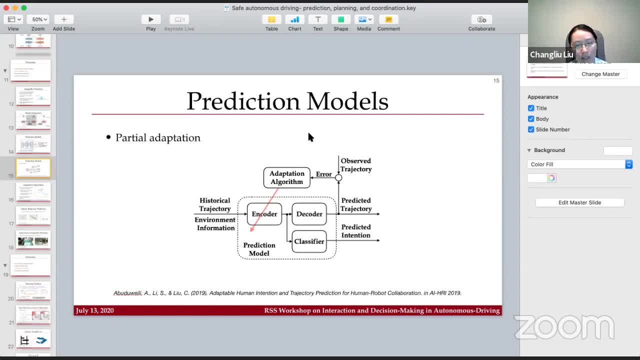 the low level, adapt the first few layers of the networking instead of the last few layers of the network. okay, great, and um I? I also had a question um with uh. with uh one of the the final parts of your talk. you're talking about um coordination between vehicles, uh, through a communication of. 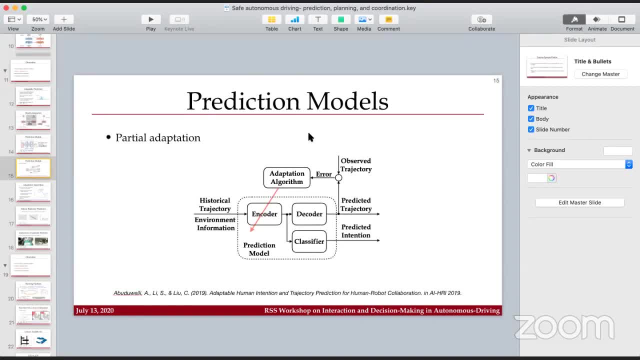 high level intent as a way to reduce uncertainty? um, do you think there's any interesting extensions where, even though the point is to reduce uncertainty, um, we could still model some uncertainty about? you know, I want to turn at this point in time, but I'm not exactly sure. 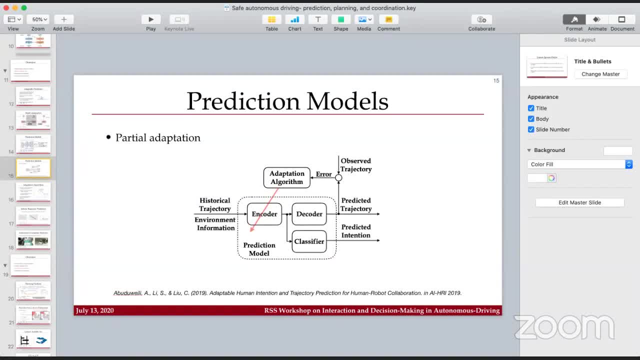 when I'm going to get there, and and, and, and, basically communicating their own uncertainty to other vehicles. um, rather than a single single intention. um, yeah, same, thank you for unmute me. could you please repeat your question? there's a train. uh, I didn't hear your question clearly, sorry about that. oh yeah, no, no problem. um, so the question was: uh, in. 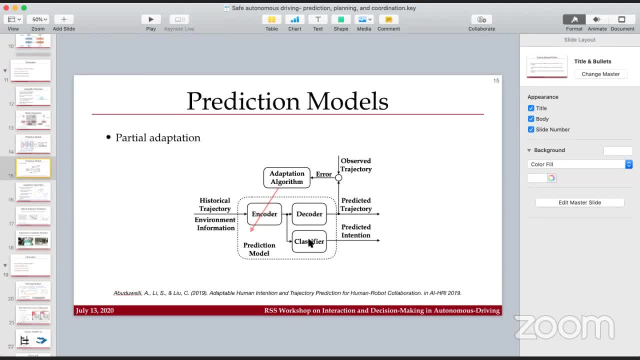 the latter part of your talk you were talking about, um, we can use information and communication between vehicles about their high level intent as a way to reduce uncertainty about what might happen in an intersection. um, do you think there's any uh interesting extensions where maybe the vehicles could communicate not only their intent, uh, but. 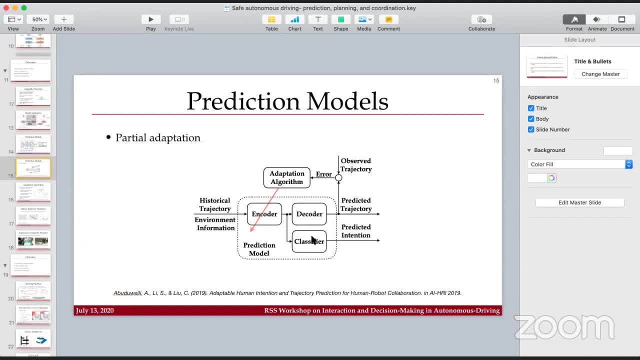 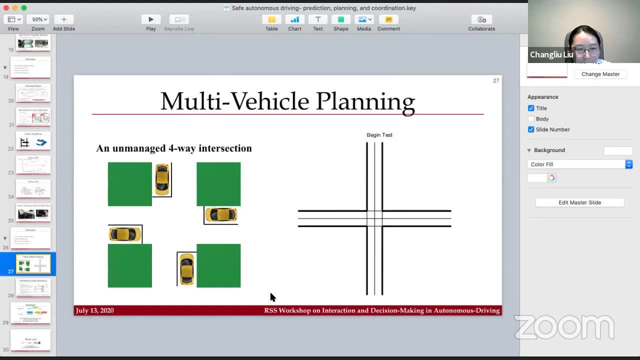 maybe uncertainties about when they may get to the intersection, in case there's, say, a human. there's it's a mixed autonomy scenario and there's human drivers where we can't fully predict what they may do. yeah, that's, that's a very good question and that is also one thing. 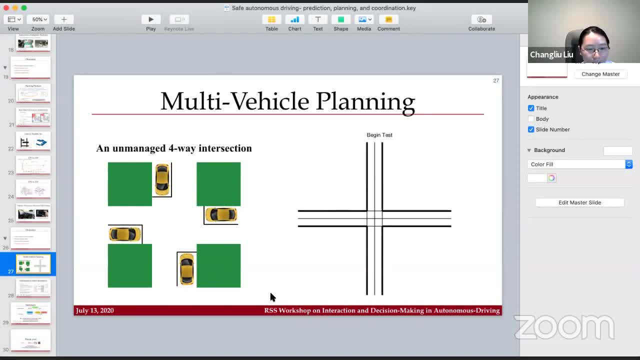 we're currently working on, because there are a lot of limitations of the work I introduced here, and it can only work if all the vehicles follow the same rule and all the vehicles are connected to each other and if there's one human driven vehicle who does not follow the same rule. 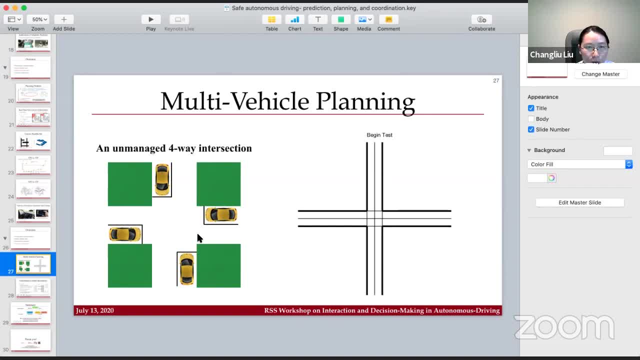 the whole scene will break. yeah, but that's true. if we can allow the vehicles to the connected vehicles to communicate more information, we can also tolerate like kind of non-cooperative vehicles in the environment, for example, human-driven vehicles. the point is, we then need to divide the intersection or the local transportation system into two groups: the 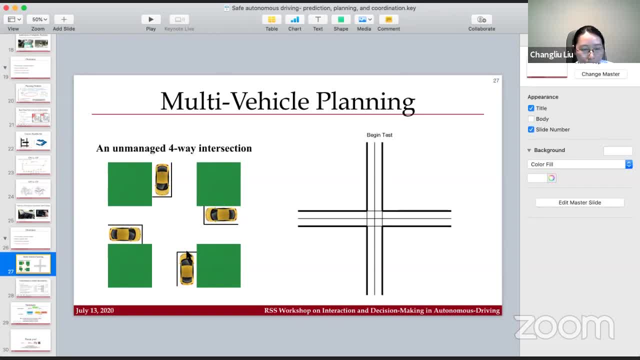 first group is all the vehicles that can communicate with each other, and then the second group is the vehicles that do not communicate, and it will be very helpful for the autonomous vehicles to share the uncertainty or prediction of others and jointly form a more accurate understanding of others behavior and so that they within the first group they can figure. 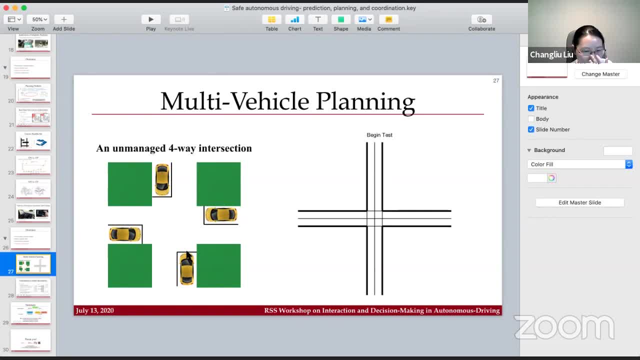 out a more efficient plan and in this way it's actually solving the autonomous driving problem in a higher level. where we have, we combine all the connected vehicles into a large autonomous car. basically it's not autonomous car, but in the planning problem it can be made as a joint decision. 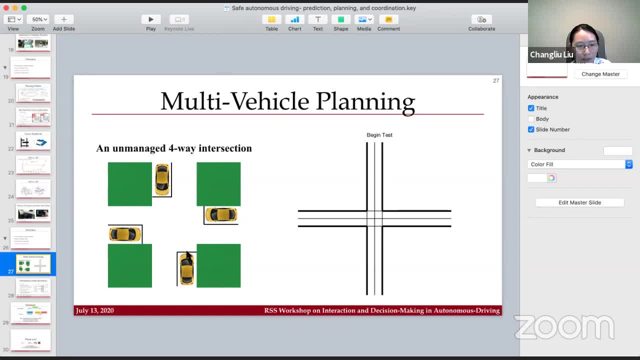 problem, and then all the others, is the surrounding environments, surrounding, uh, like participants, road participants that we need to predict. for does this answer your question? yes, yes, that's uh, that's great. um, yes, that's um, that's uh, yeah, that uh, and that is, that's all out, that's all our. 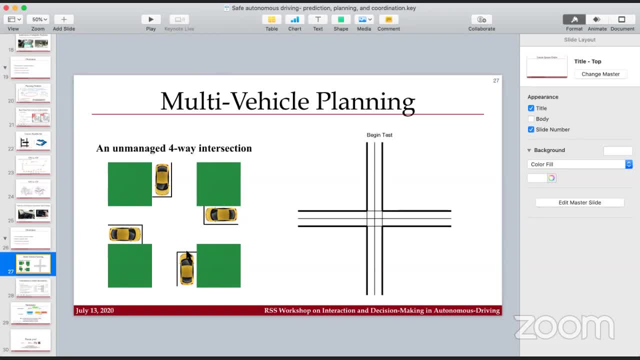 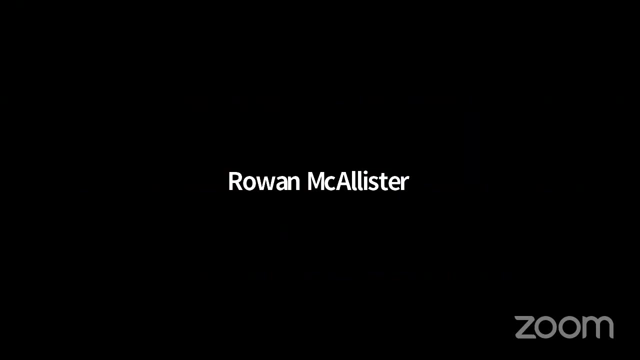 questions. um, so, yeah, thank you. thank you very much, uh, for that talk and um, we look forward to seeing you at the um, at the panel, after our next speaker. well, thank you. thank you, okay. um, so our final speaker is Professor shingbo lee. um, if you are there, Professor, 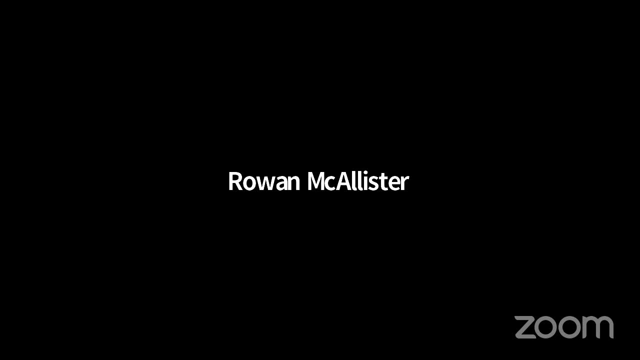 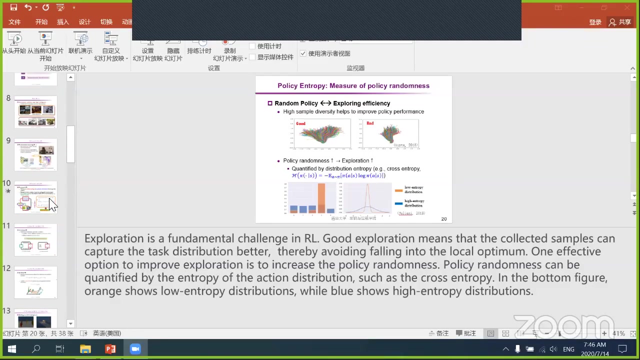 um. you can now start sharing sharing your screen um so so. Professor shingbo lee is an associate professor at Tushingwa University, leading the intelligent driving lab. his active interests- research interests- include intelligent vehicles and driver assistance, reinforcement learning and optimal control and distributed control. for estimation, he's the author of over 100 peer-reviewed journal. 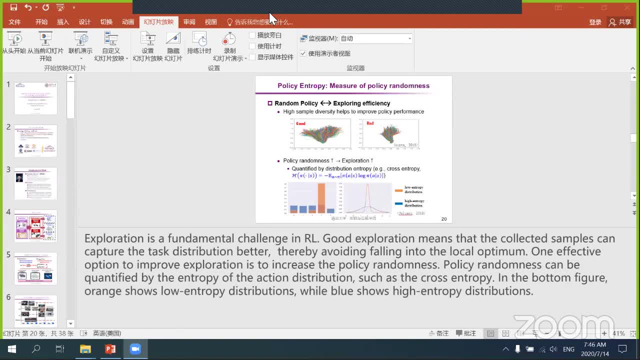 and conference papers and is the co-inventor of over 30 patterns um. I believe he was the recipient of the best paper award in the 2014 IEEE ITS uh, the best paper award in the 14th Asian ITS, and also serves as the board of directors for the IEEE ITS society. 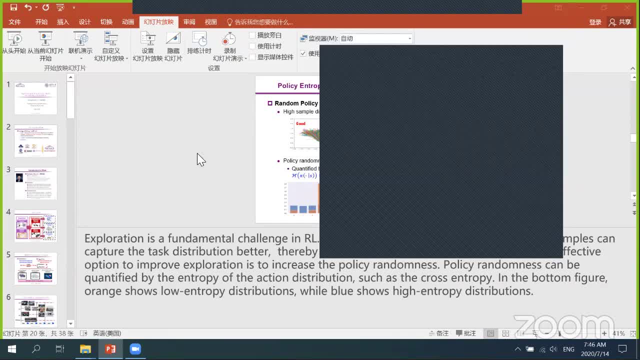 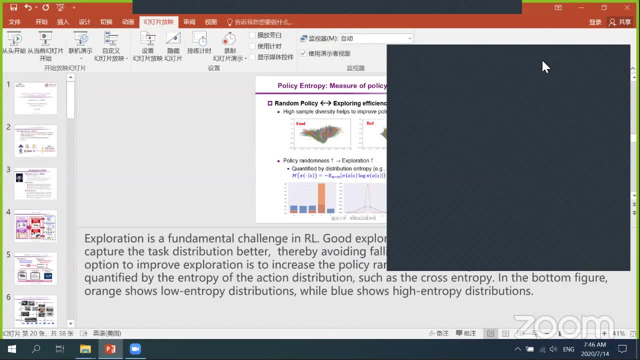 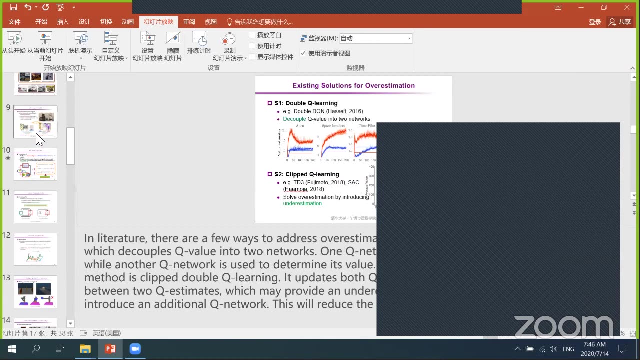 uh, so his talk today is titled distributional soft active critic, um. so thank you so much for joining us and, um, we look forward to your talk whenever you're ready. hi everyone, can you, can you hear me? yes, I can hear you just fine, can see and we can see your slides, okay, thank you. thank you very much for your introduction. 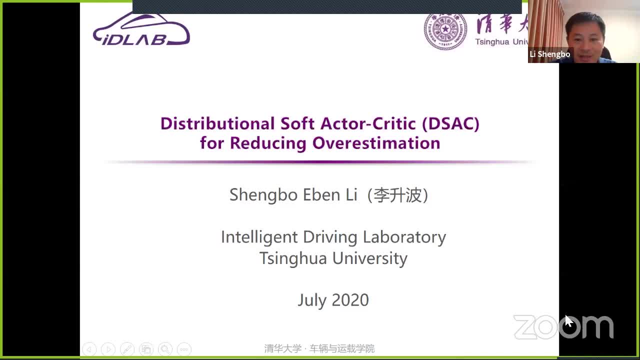 and uh, and also, and can you, can you see my screen? share screen? yes, we can see your screen. yep, okay, so i'll start. so thank you very much for inviting me to join this workshop, and it's my great honor to be here. so my name is shenbo and today i want to give you a talk. the name is: 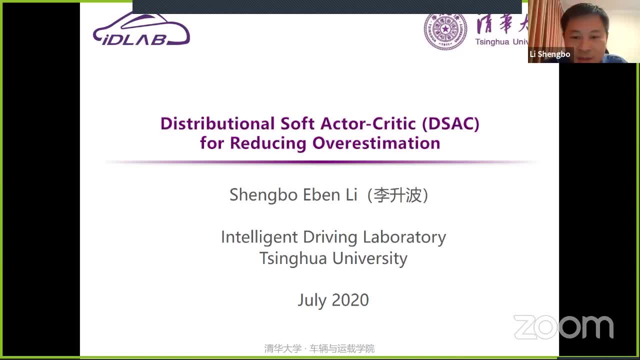 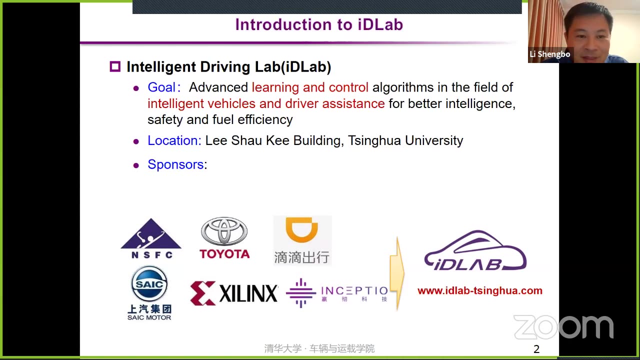 distributional soft actor critic for reducing over automation. basically, it's a theory about reinforcement learning technology. uh, before my talk i i'd like to introduce my lab at chinhua university first. so currently i'm leading a lab the name is intelligent driving lab, show as id lab. so we focus on advanced learning and control algorithms in the field of intelligent 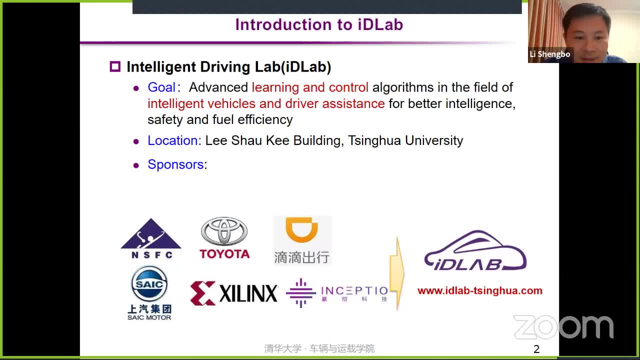 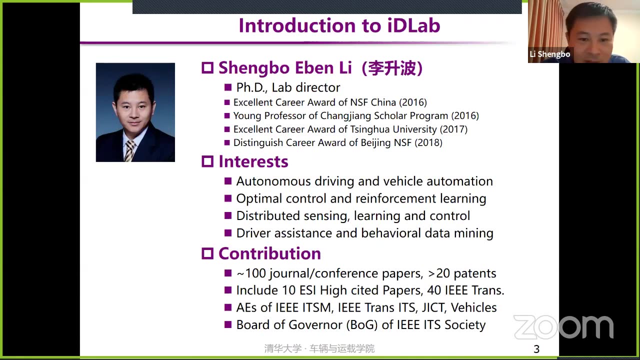 vehicles and also the driver assistance system design. so in order to get better intelligence, safety and fuel efficiency. so they are my current sponsors. thank them very much. and this is about me, and my research interests include autonomous driving and vehicle automation, optimal control, reinforcement, learning and also distributed sensing, linear control. so so i also served as the 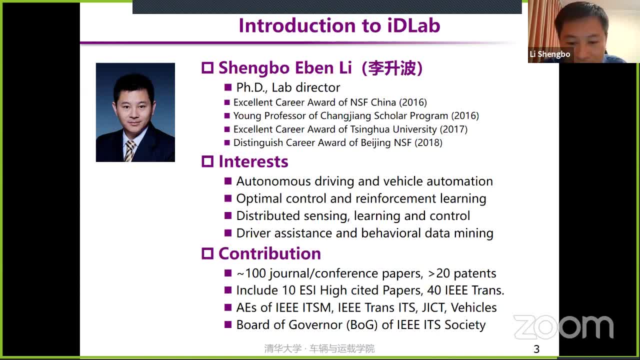 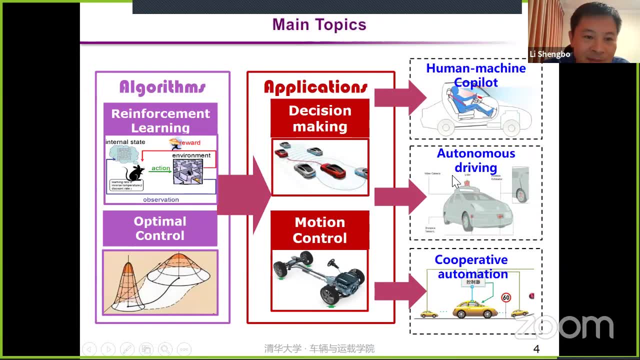 associate editor of ieee journals and and also the beauty of ieee ics society. so basically, my lab is working on the interdisciplinary research of reinforcement learning and optimal control. so we apply the developed algorithm in decision making and also motion control of such autonomous systems like human machine, co-pilot, autonomous driving. 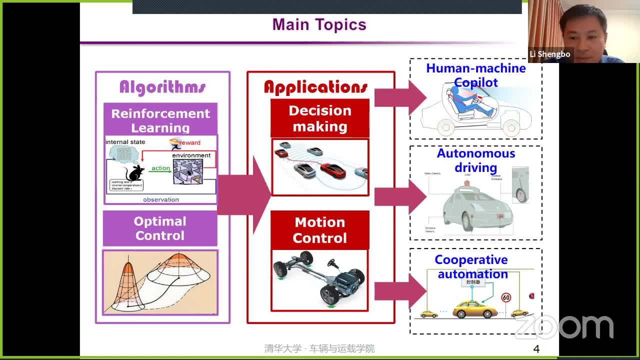 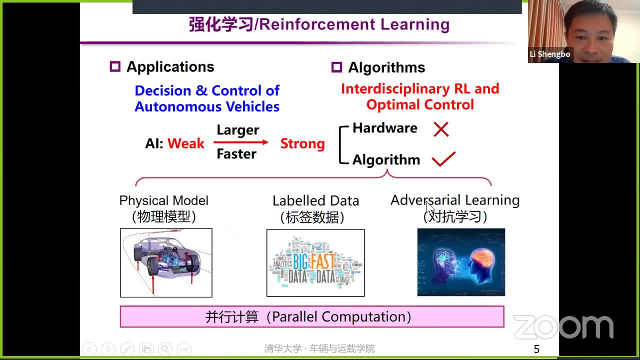 systems and also cooperate automation by the vehicle to vehicle communication and for the reinforcement learning. this is the major topic today. so we want to say we focus on the algorithm design part, especially how to combine the model and label data together, and also include a touch topics like adversary learning into reinforcement learning and how to apply. 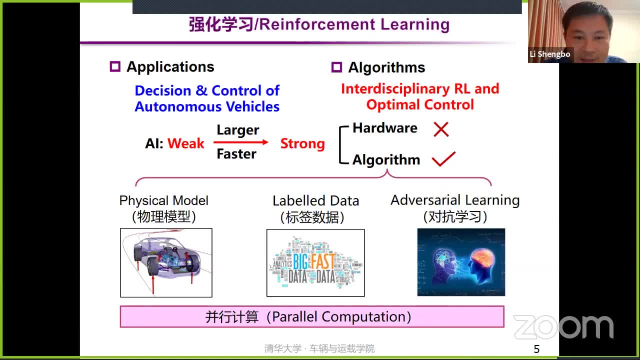 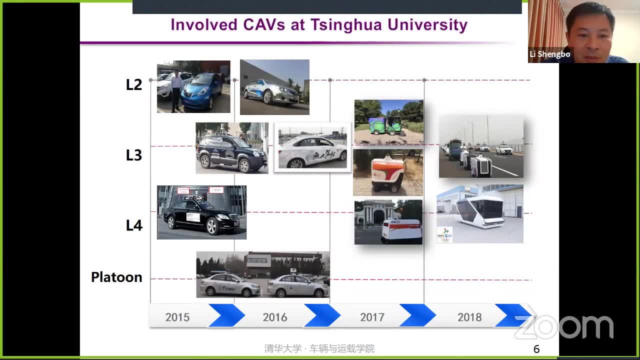 the parallel computation, so in vehicle size. this is the major topic we are working on. so in the past few years we have involved a few autonomous vehicle prototyping, car design, and these are the other photos of them. so very short introduction about my lab and now our talk. 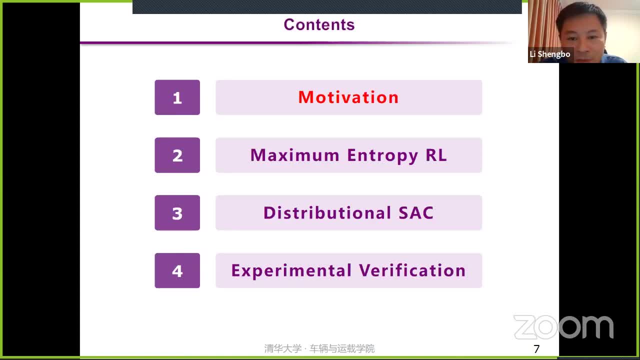 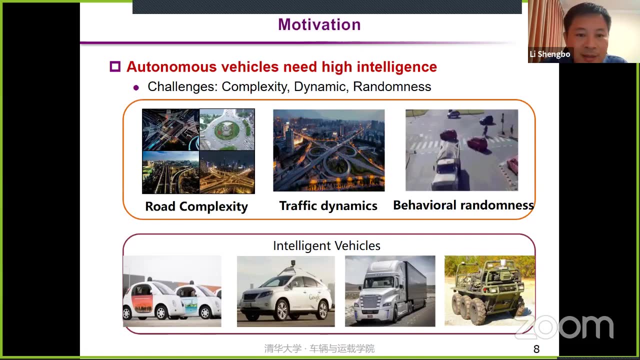 about. you know today's topic, so distributional, soft, active critical algorithm. so i'll start from the motivation. so we all know that autonomous vehicle need very high intelligence, especially in the decision making part. so this is because we have very strong road complexity, traffic dynamics and also the road users have random behavior. yes, so we want to know: developed uh intelligence which? 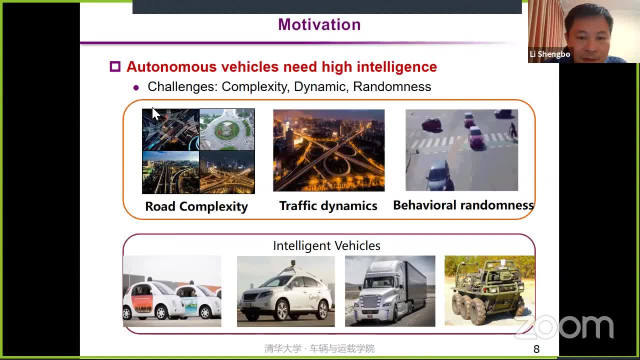 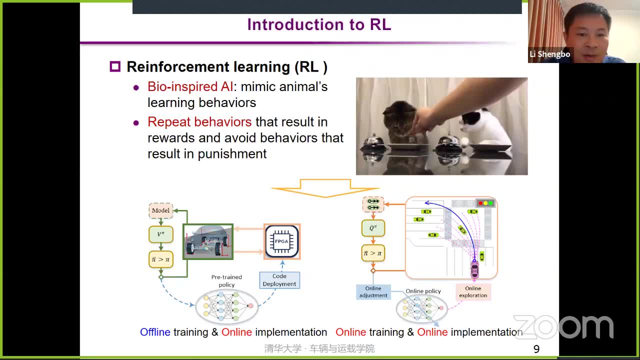 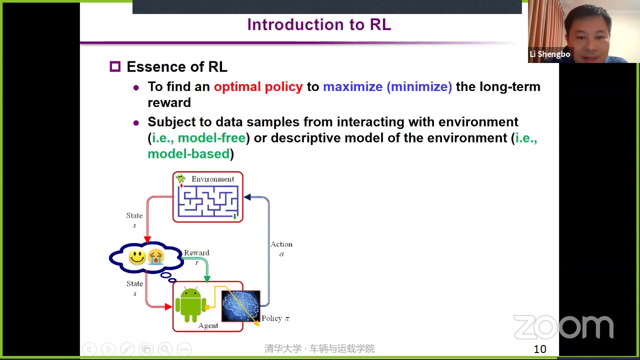 can conquer those, these wolves. so to manifest so a broad range of in two ways. So one is offline training a policy and then online implement this policy. The second is we do both online training and online implementation. So we will mainly talk about the second part, which is a model-free method. So if we look at the details or mathematics of 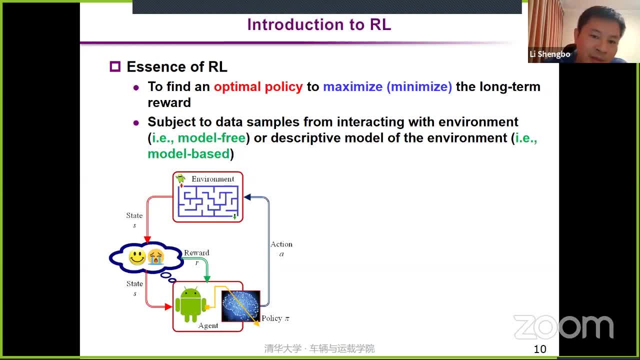 reinforcement learning. it has close relationship with optimal control. So basically, it aims to find an optimal policy that maximizes or minimizes a long-term reward while subjecting the samples from interacting from the environment. So basically, this is the model-free IELTS And also it's subject to the descriptive models of the environment. So basically, it's a. 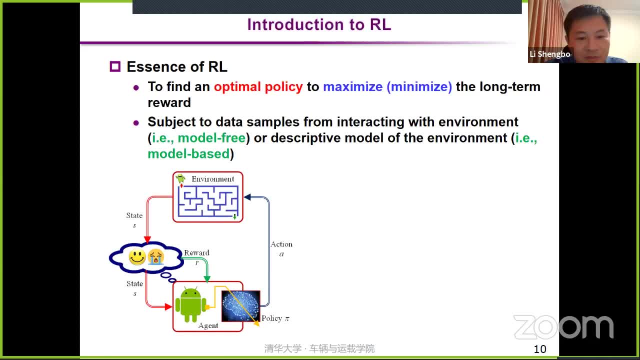 model-based IELTS. Model-based IELTS is very like optimal control theory, So in mathematics we can unify the model-free and model-based IELTS into one unified framework. So this is to minimize this cost while subjecting a few constraints in order to get the optimal policy. 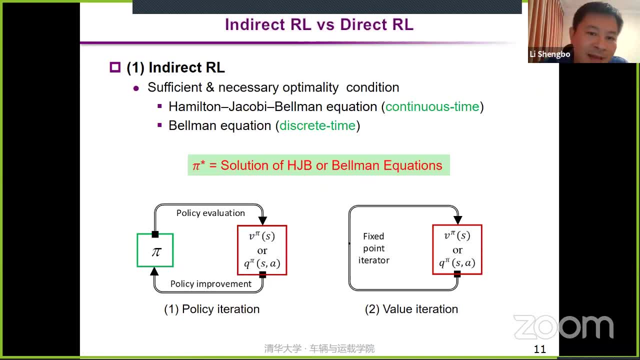 Today there are two ways to solve reinforcement learning, So we call it indirect method and direct method. So indirect method: basically it relies on sufficient unnecessary optimality condition. So in continued times this condition is described as the Hermitian-Jacobi-Behrman equation, or 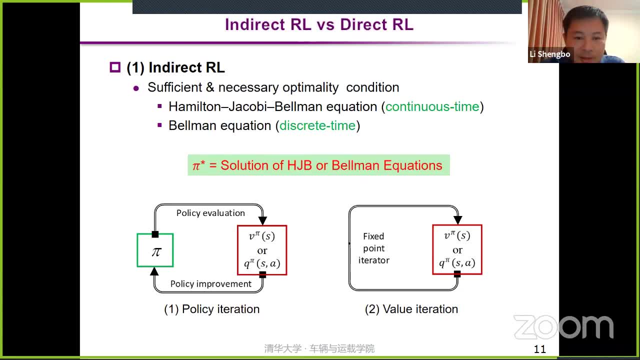 just the Behrman equation in discrete time domain. So the optimal policy is actually the solution of the optimal policy. So the optimal policy is actually the solution of this AGP or Behrman equations. So we all know that we have two ways to solve these equations. 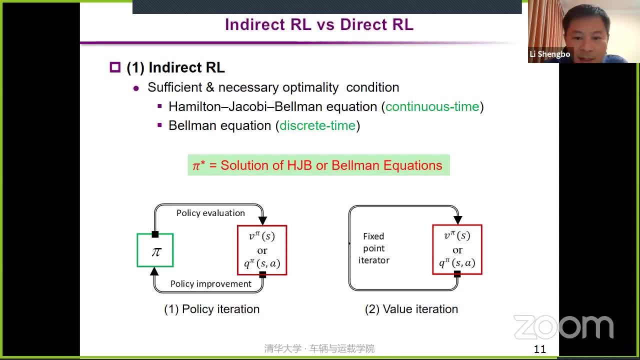 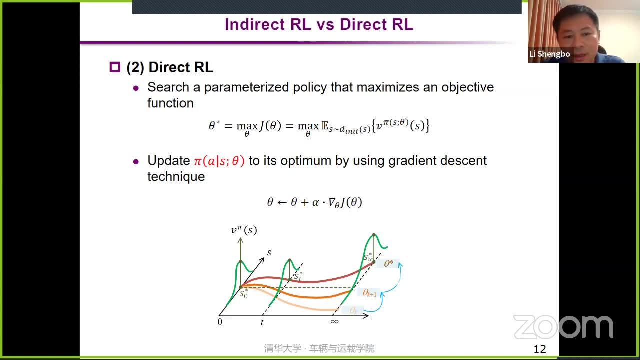 either policy iteration or value iteration. The other method we call it direct solutions. Basically it's a search permit, a parameterized policy that can maximize or minimize an objective function. So the common method is called gradient descent technology. So the common method is called gradient descent technology. So this one is called 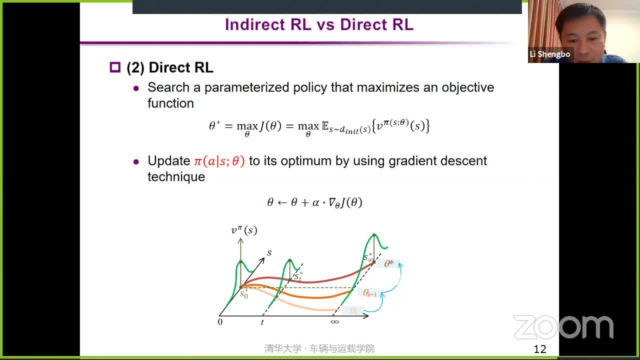 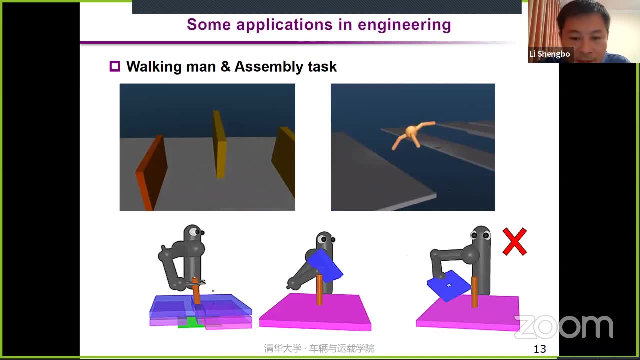 So we can repeat this process until we find the optimal. So these are the two ways we saw the reinforcement lining, And this technology has achieved a few success, in engineers, For example. here I leave some of them. So working man: assembly tasks. 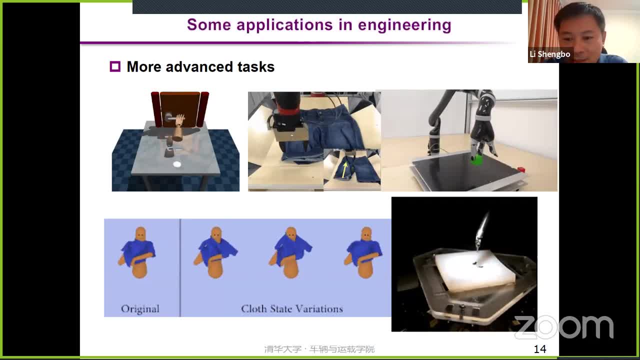 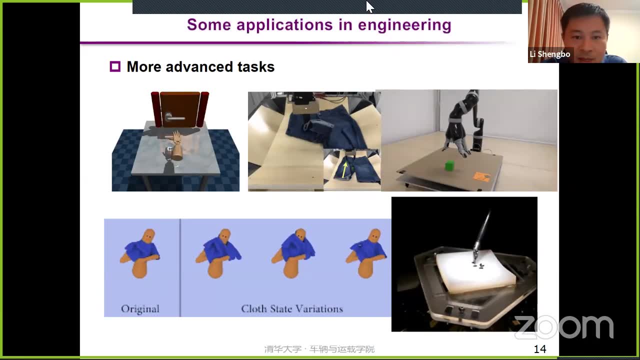 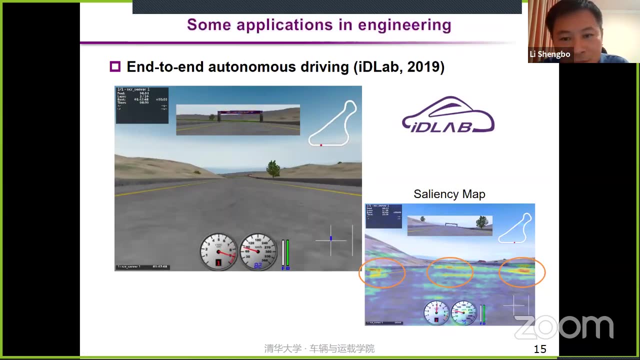 and more advanced work. like you know, wear clothing and pick up a box, pick up some parts in a dynamic platform, And also we can apply it into the field of end-to-end autonomous driving. So this is the video we have recorded in my lab. 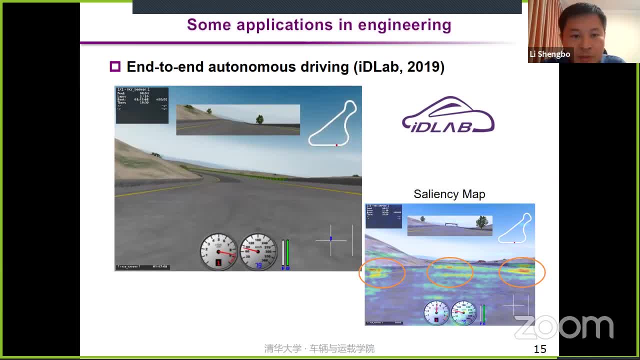 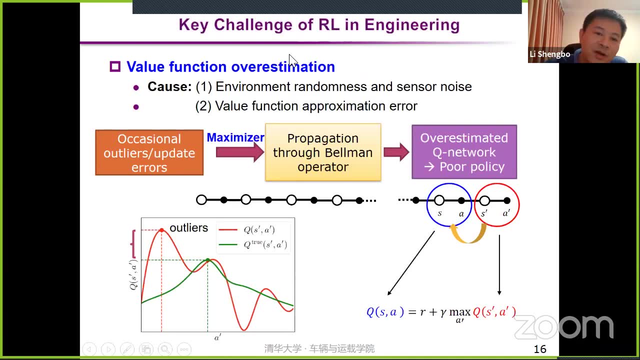 to use reinforcement lining technology to do that autonomous driving task. Basically it works, But we also found a few challenges for this technology in engineers. One major challenge is the very function over estimation. So this is caused by two issues. So, for example, the ____ randomness. 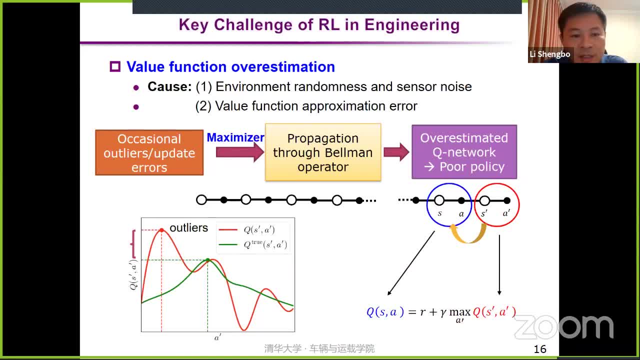 or the ____ noise or the where function approximation errors. That clearly happened outliers and all ____ errors can cause the error be prohibited through the, which will cause the over-admitted Q value network. So finally, we make a very bad policy. So this is the reason. 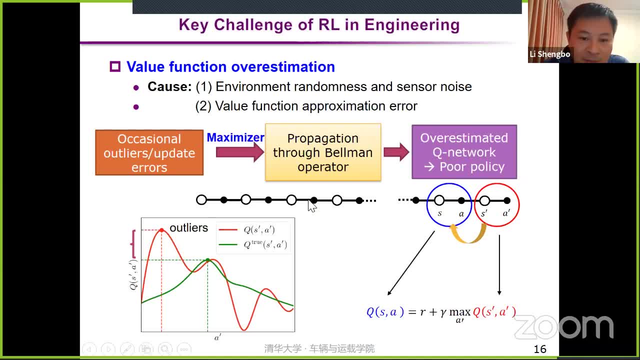 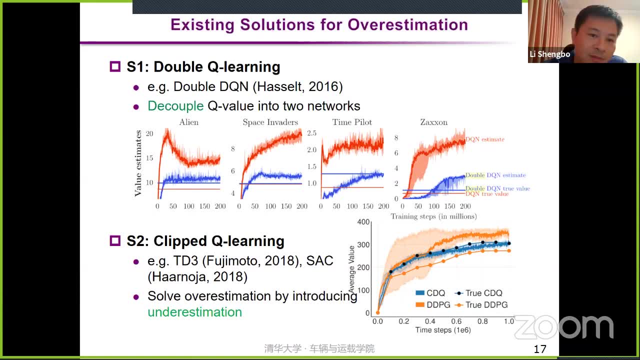 And how to conquer this reason has been eradicated by many researchers in the past few years. So two famous solution is the double Q-Line and the clipped Q-Line. So the double Q-Line decouples the Q value into two network, So use one network as the target. 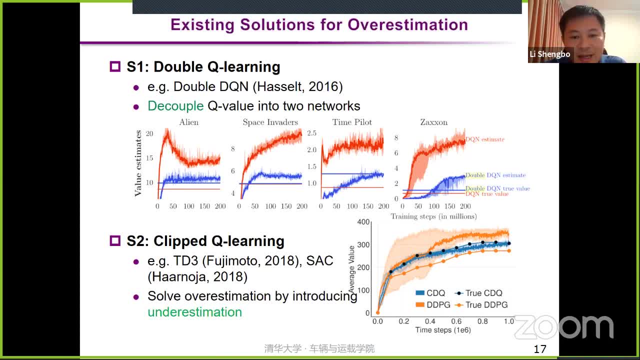 the other one as the trend value which can reduce this issue to some extent, And the other method actually solves the over-admission by introducing under-admission. So both of them may suffer from still suffer from the over-admission issue. And also we want to see 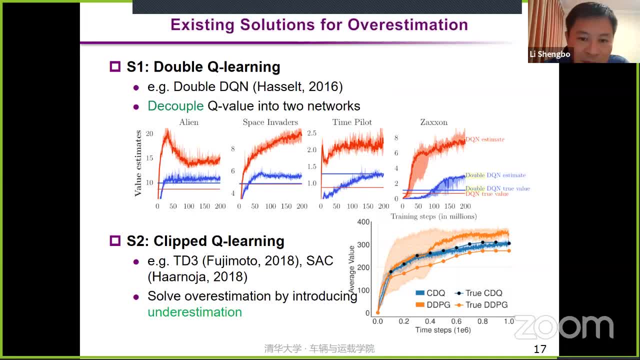 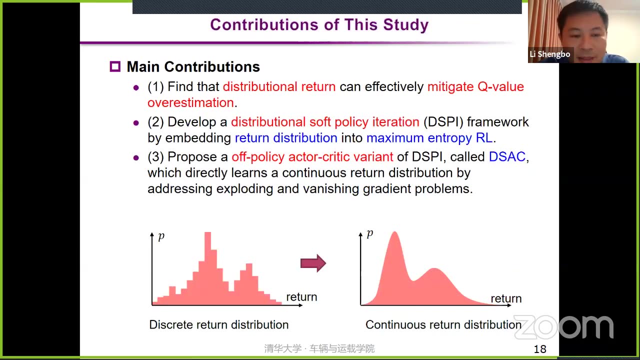 So the two methods actually introduce an additional neural network into the learning process which may add a few computing burden issue to the system. But in our study my team has proposed a new method called distributional self-active creativity. Basically we combine the distributional idea. 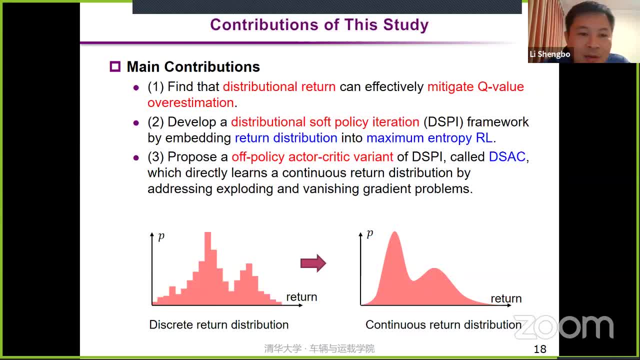 with the self-active idea together. So in our study we have find: first, the distributional return can effectively mitigate the Q value over-admission. This is the first finding And based on this finding we developed a distributional self-policy iteration framework. 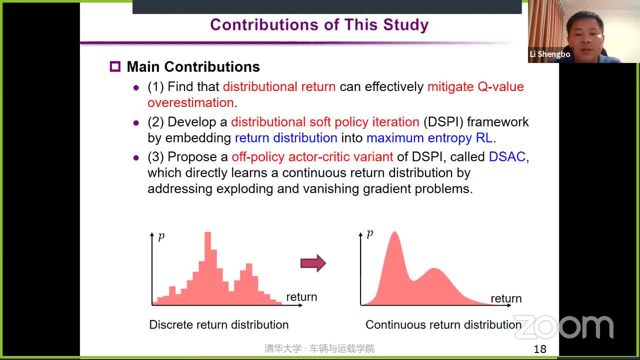 which embeds the return distribution into the maximum entropy, And this is the result of the reinforcement learning. So, finally, we propose an off-policy active critic algorithm, so-called DSEC, and which can directly learn a continuous return distribution by addressing the exploding or vanishing gradient problem. 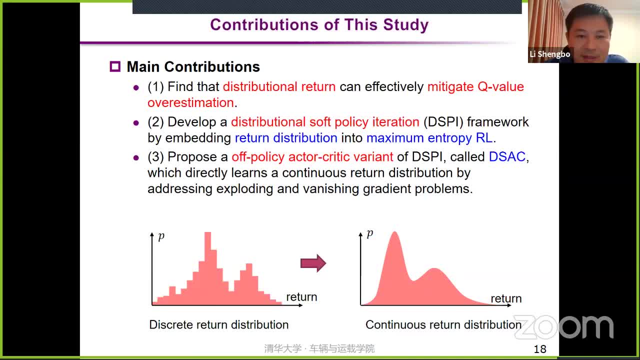 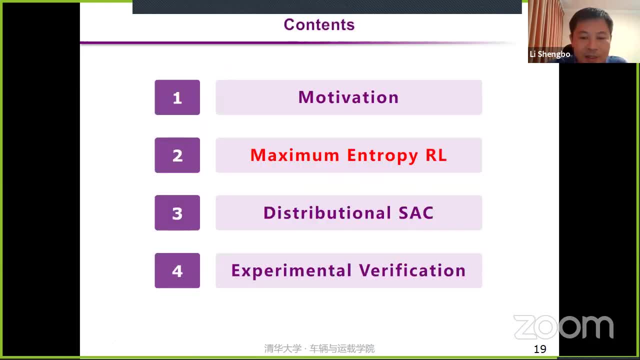 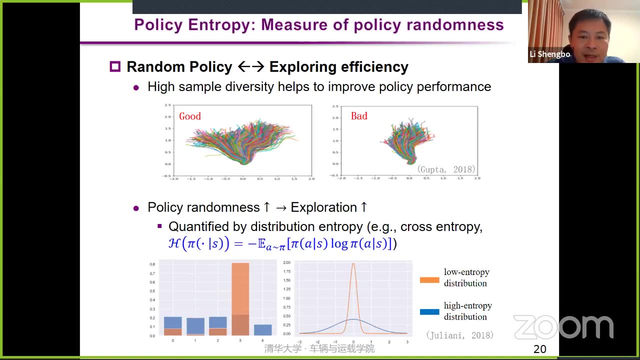 So this is the main contribution of this study. So I will explain the details in the following slides. So first, the basis of this method: maximum entropy, reinforcement learning. So we all know that the exploration efficiency is very important for the model-based reinforcement learning. 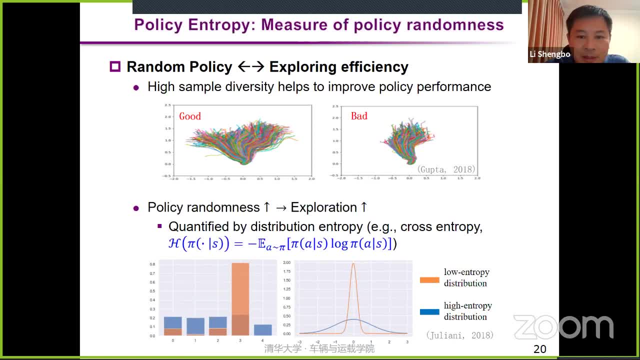 And so one way to increase the exploring efficiency is to use that random policy, And the high simple diversity can help improve the policy performance. So find out about here. we have two figures, So the first one has good exploration, The second figure has bad. 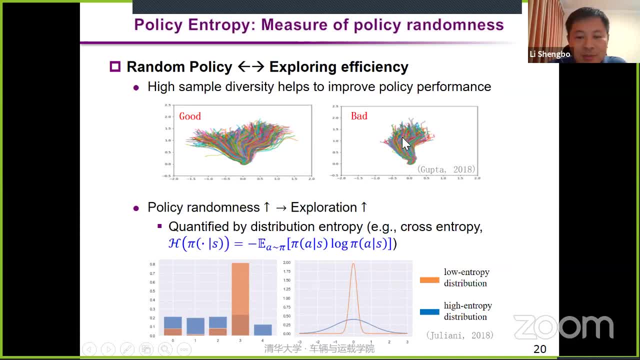 or has worse exploration efficiency, But there's always a balance between better exploration and also the policy randomness. How to measure the policy randomness is one technology we need to use in IELTS, So the policy entropy is a good measure of the policy randomness. 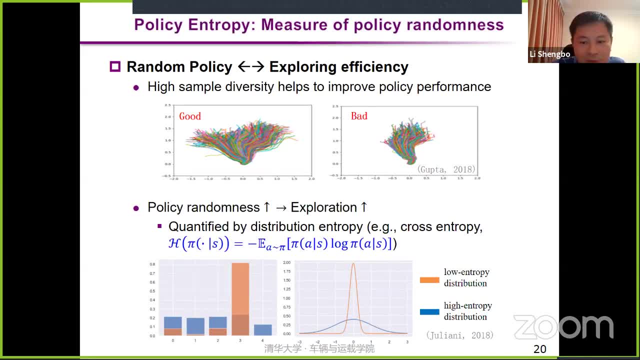 And we can use this entropy to describe how large the policy is random and combine it into the object function to reduce or increase the entropy in order to balance the randomness of policy with the exploring efficiency. So this is a basic idea. And the second one, 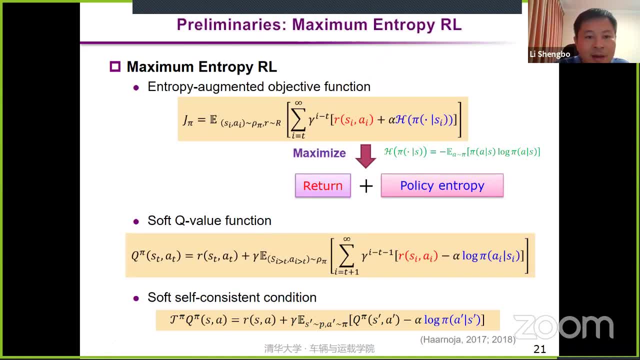 and this method is called maximum entropy IELTS Basically. so we add a policy entrant term into the objective function or directly into the reward function, And so this reward includes the traditional return function and also a new policy entropy term. So, using this way, 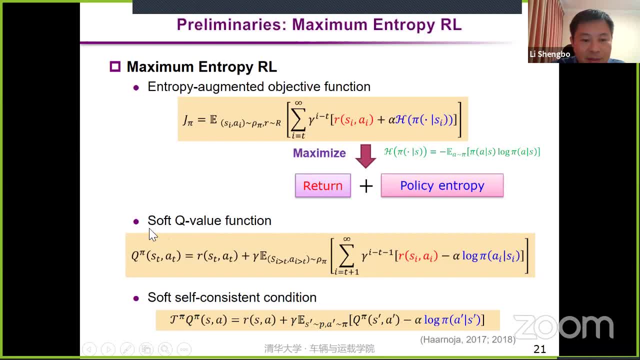 we can convert the traditional Q value function into a, a soft version. We call it a soft Q value function And also we also have the soft self consistent condition and also soft Berman operator. So this is the basic idea of the maximum entropy. IELTS. 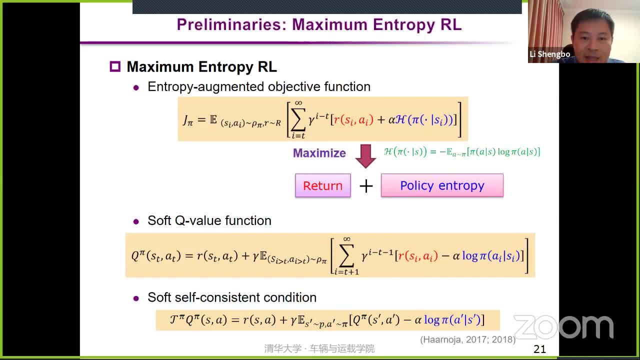 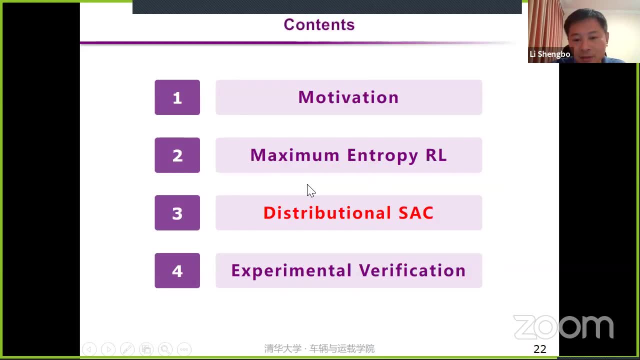 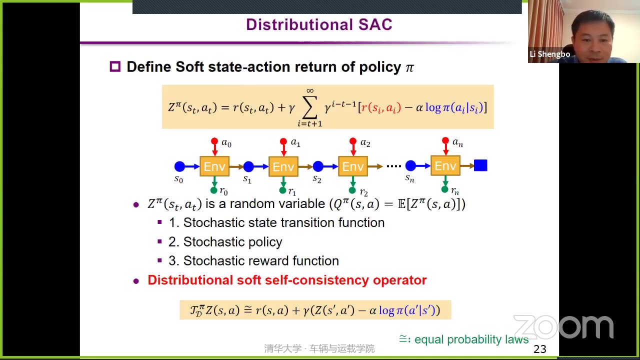 And then my GSEC algorithm actually based on this maximum entropy IELTS. So now let's talk about the GSEC. So the GSEC need to combine the distributional function into the maximum entropy IELTS. So first we need to define a distributional function. 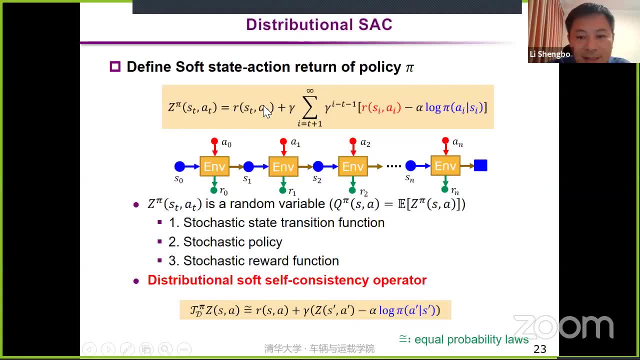 So what is the distributional function? So here is the definition for the distributional function. So basically we change a fixed value of the return into a distributional function. So it's kind of a new random variable And the expectation of this variable. 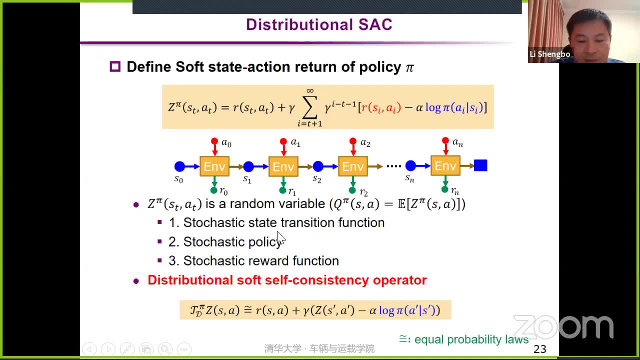 will become the traditional Q value. So this randomness change is reasonable because of several reasons. First, the environment might be stochastic, right, And also the policy is stochastic, So in many engineering. so we select stochastic policy And also sometimes we may have stochastic reward function. 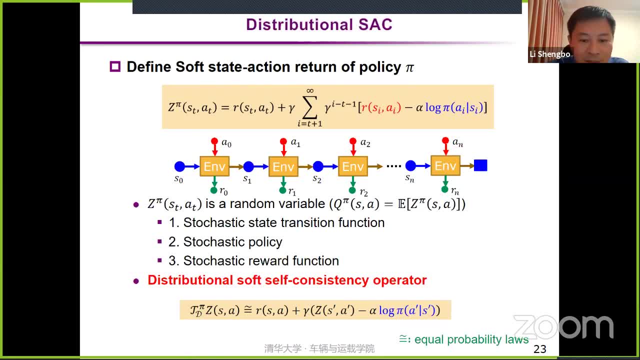 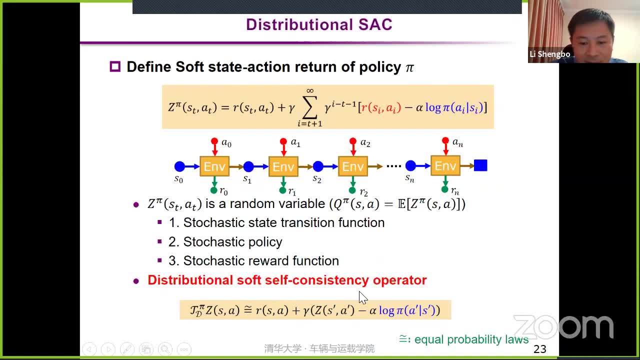 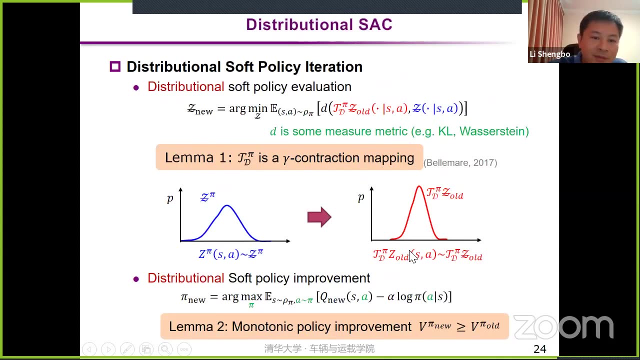 And we can have a distributional version of the self-consistent operator or the bare-mind operator. So here we should the self-consistent operator in a distributional return format, Since we have the distributional Q value. so now we can easily design. 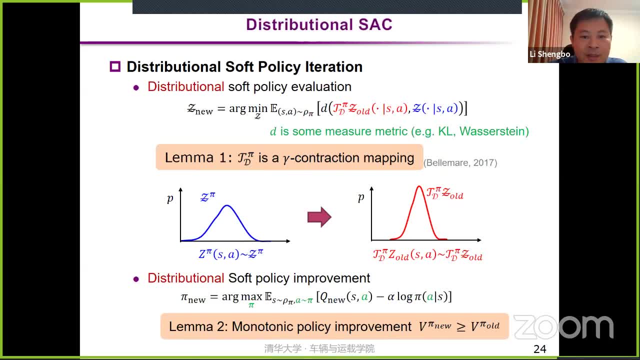 the reinforcement learning technology by using the policy gradient method. Policy gradient gradient iteration actually have two steps. One is the policy variation, the second is policy improvement. So we can reformulate the two steps by the distributional function and also the soft idea introduced in the maximum entropy IL. So we can also prove that even 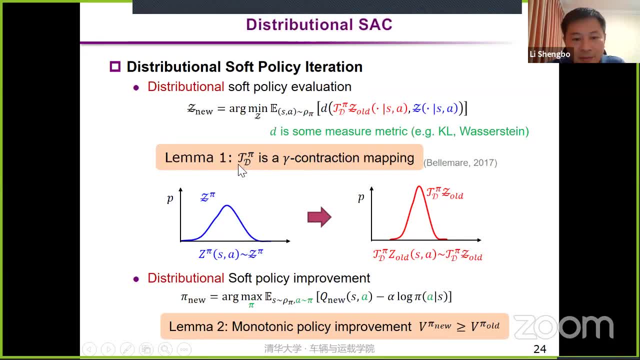 though combined with the distributional function, the self-consistent operator is still a GAM contraction mapping, which means it can converge, And we can also prove that the new policy improvement step still holds the monotonic increasing behavior, which means the overall algorithm can converge. 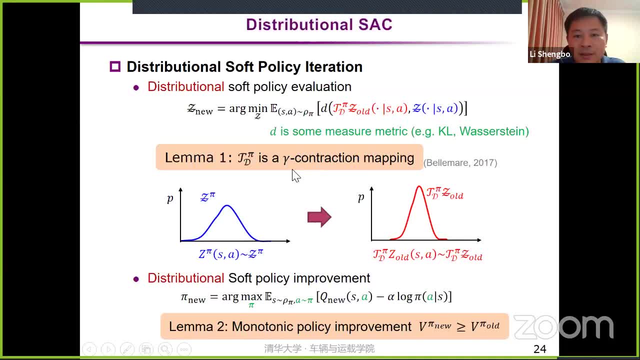 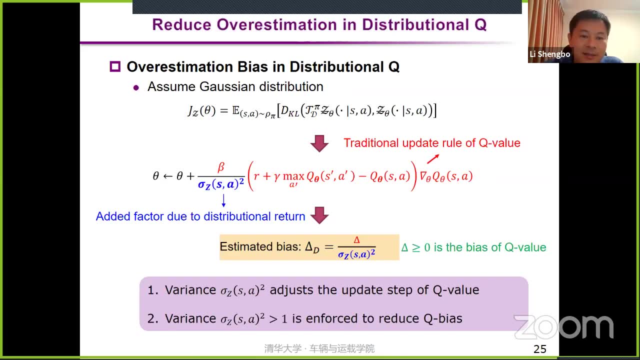 Okay, So this is the basic idea behind the distributional SAC. So now we want to improve why this method can reduce the over-attimation. So let's give a short introduction So we can roughly derive the over-attimation bias in this method, if we can assume that policy randomness also 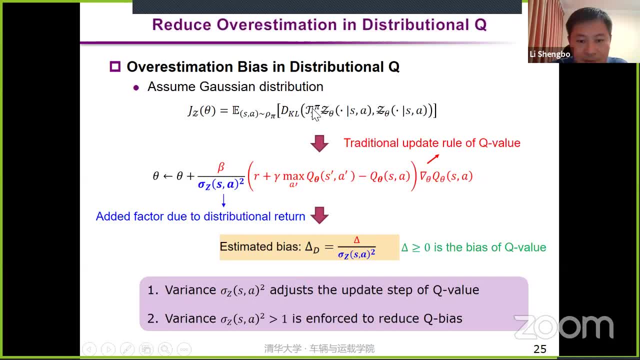 and other randomness are Gaussian distribution. Okay, So the final result is very interesting. So let's look at this equation Here. the delta D is the admitted bias of the new method. The red delta is the bias of traditional Q value method And we can see that two methods actually has a factor: delta Z and delta Z. So delta Z is the value of the new method and delta Z is the value of the new method, and the delta Z is the value of the new method And the delta Z is the value of the new method. So it's a very interesting situation. 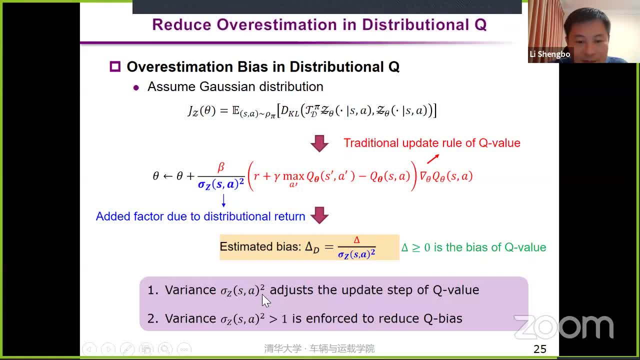 So this is the sigma of the sorry is sigma Z squared. It's the variance of the Q value function. It's kind of has the ability to adapt in the update step of Q value And also if we can select base coefficient always bigger than zero, so we can reduce the Q bias. 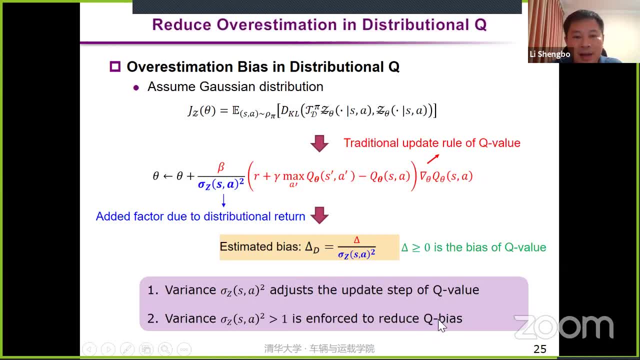 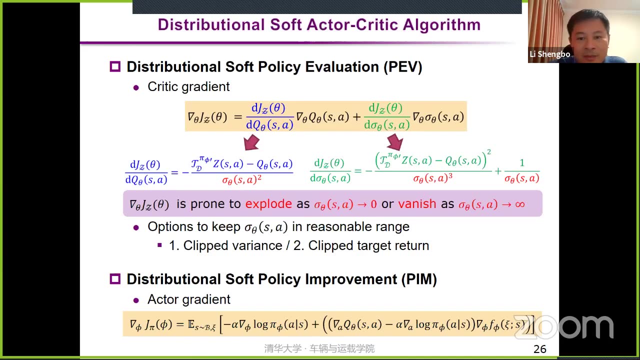 So that's the question. Okay, So this is the idea behind why this new method can reduce the over-intimidation bias, And now let's look at how to design a method which can combine with the deep neural network. So we can design DSAC in the way of active critique, and the critique gradient is to: 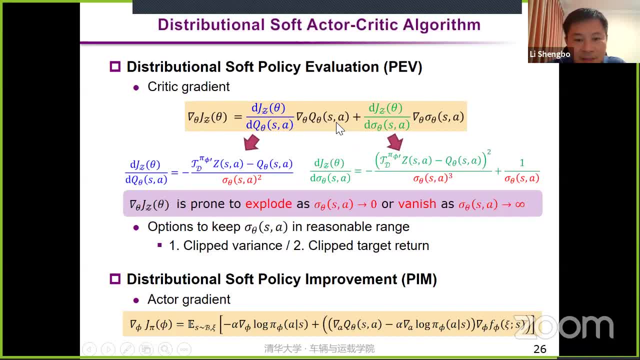 minimize objective function which can measure the distance between the new key value and also the target key value. So the gradient actually has two terms If you look at the details. so we find in this new method so both the two terms have the denominator of sigma, theta term. 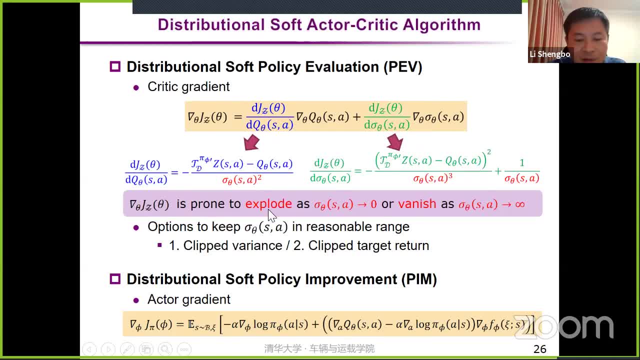 So if the algorithm is not well selected or the parameter is not well selected, we may have the explode or vanishing gradient issue. So because sigma theta may go to zero Or goes to infinite. So this is one challenge And in the algorithmic design we need to keep this value into a reasonable range. 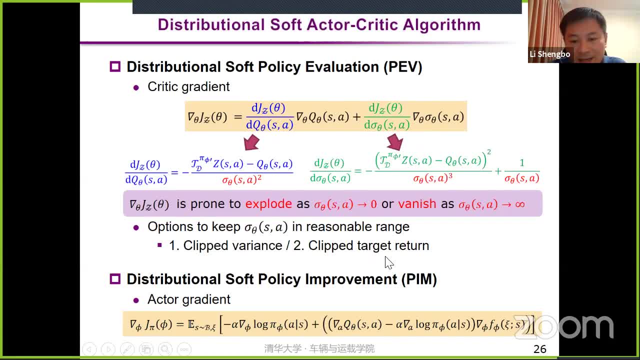 For example, to clip the covariance or clip the target return. Using this way, we can avoid this issue And also we can easily derive the active gradient. so choosing this equation. So basically, so we can convert the DSAC into the traditional active gradient. 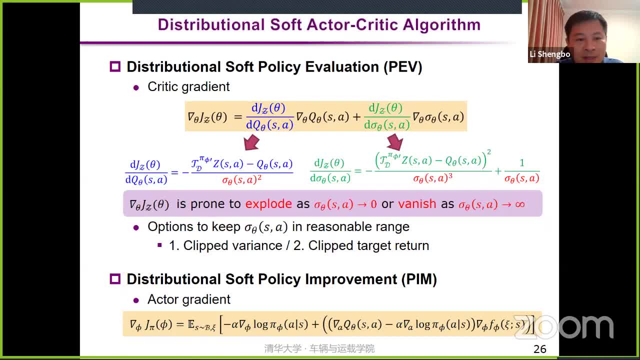 So, basically, so we can convert the DSAC into the traditional active gradient And since you have to have a similar approach, you can also try this. But what we can actually do is we can also try to combine this algorithm with the neural. 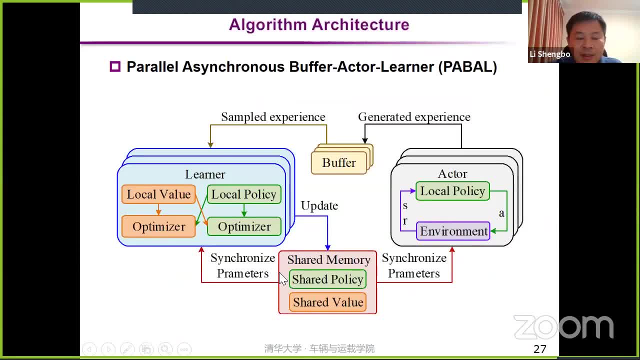 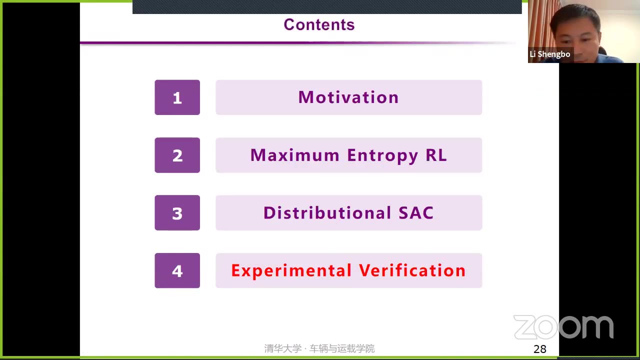 network And also we can combine the parallel updating framework, which can accelerate the training speed of this algorithm. So now let's talk about the experiment verification to see the performance of this new algorithm. So if you look at this value, you can see that the current data in the upper left-hand 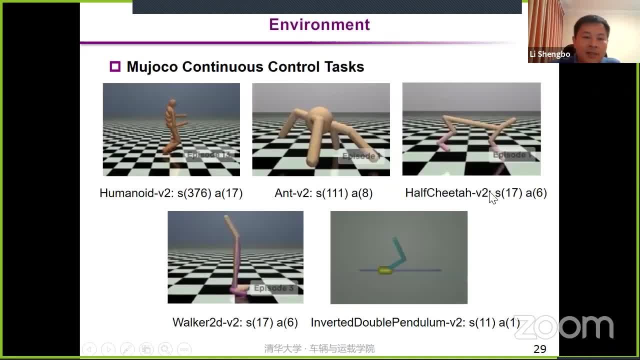 field is greater than the current data in the upper right-hand field. So then in the outside area you can see more or less of the linear data which was created algorithm, And here we select five continuous control tasks from Mujuka. So, for example, 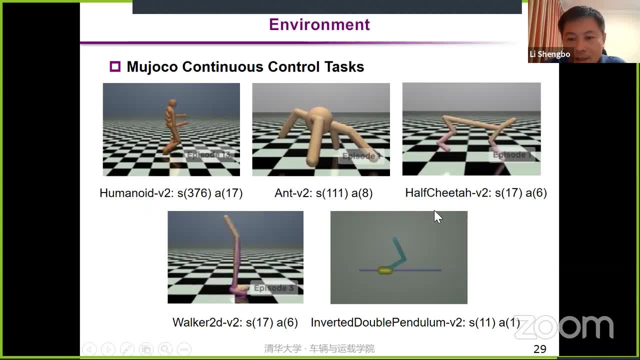 the humanoid ant and half-chatter and walker and also inverted double pendular. So here the s is the state, the number is the dimension of the state. So we can see, the first task has a very high state dimension and also a relatively high action dimension. So we 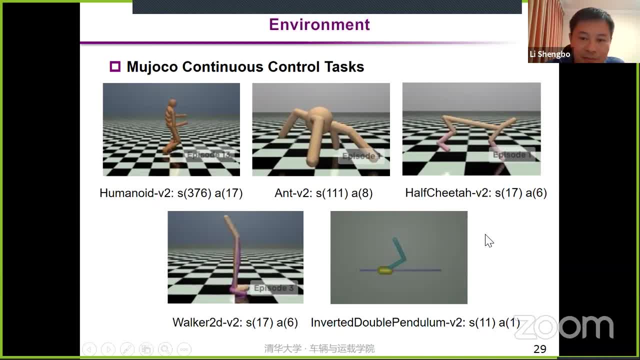 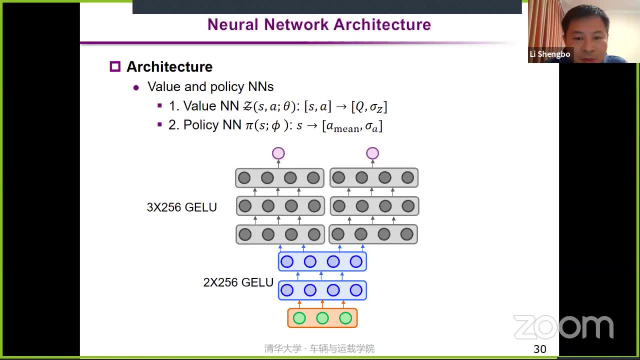 can see these five tasks has a good representation And the selection of the neural network architecture. So we select a relatively similar neural network for the value approximation and also the policy approximation. So basically it's a five-layer system. So we can see that it's a fully connected neural network, including the input layer. 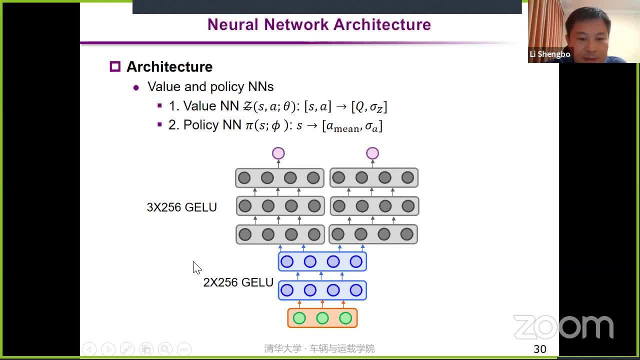 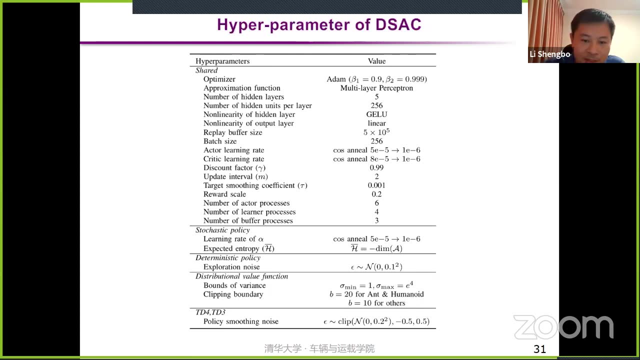 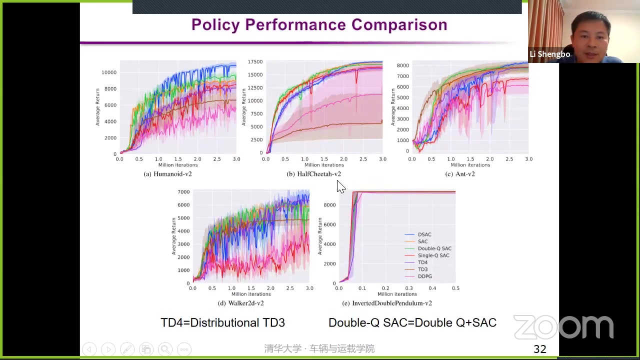 and the output layer. So there are three hidden layers And also it's a fully connected neural network. So here are the hyper-parameters of the DSEC and we can select those parameters, very like the traditional DSEC algorithm. So now let's look at the policy parameters. 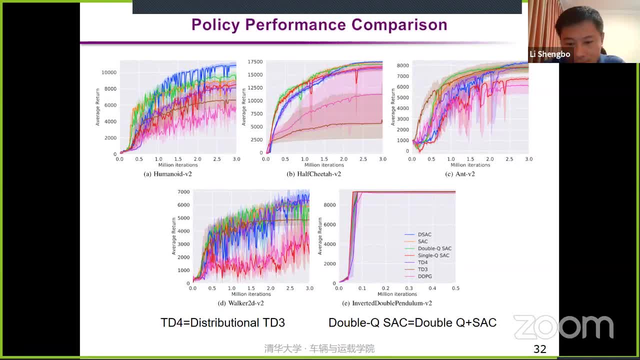 and the performance comparison of the DSEC and also other baseline methods. So here we selected six baseline methods, including the base version of SSEC double-q, SSEC single-q, SSEC TG4,, TG3, and also DDPG as the baseline And the blue line is the performance comparison. 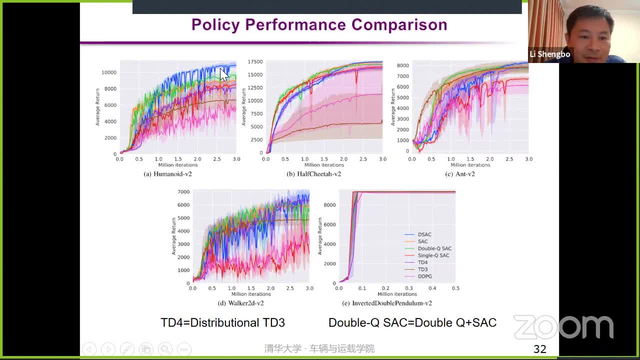 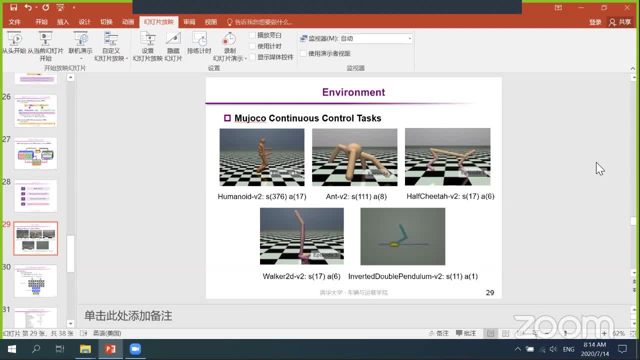 performance among all the methods in compressing And we can see basically the DSEC has the best. So the first question is from Igor And the question is: where do you see the application of deep reinforcement learning within the driving stacks of autonomous vehicles? 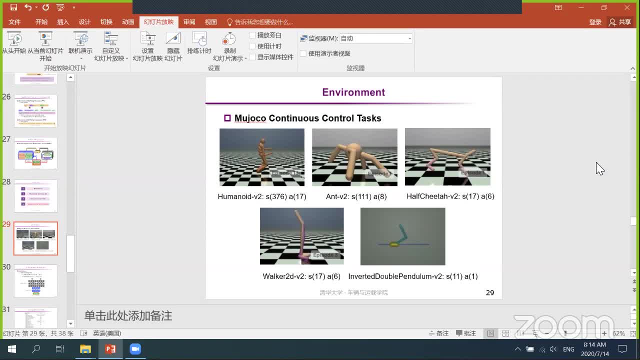 Oh, I see. Okay, I should say, to apply reinforcement learning technology in autonomous vehicles is a really challenging problem And there are several reasons. First, boot IO technology is model-free based and we need the sampling data to train the policy. 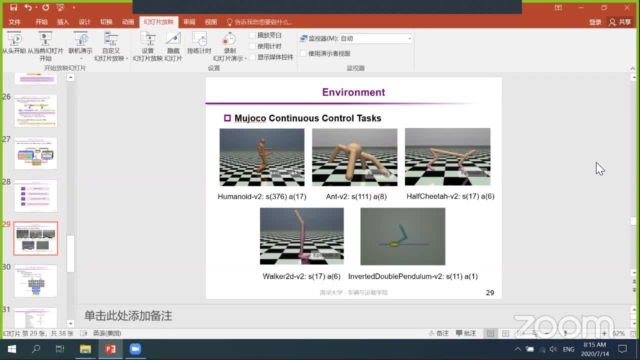 So how to get the sampling data? So we need to interact with the environment. So the interaction with the environment is a major challenge for real autonomous car And this is one reason. And also we see that reinforcement learning, if it goes deeper, we need to combine it with neural network. 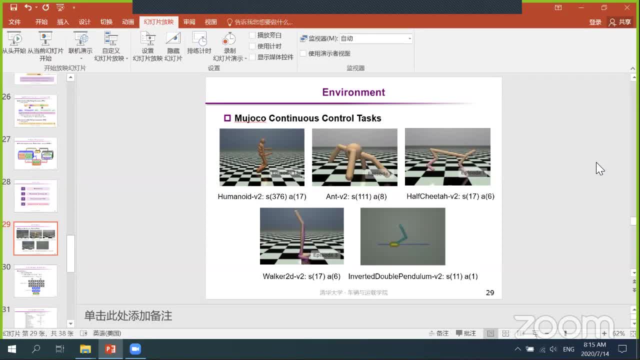 And it has very high computing efficiency requirement on the onboard controller, which may be a bigger challenge than interaction with the environment, And I have seen a few universities and also research studios working on this topic. Most of them still work with virtual environment, like the CarSim or the Moduco simulator or other simulators like the Pris game. 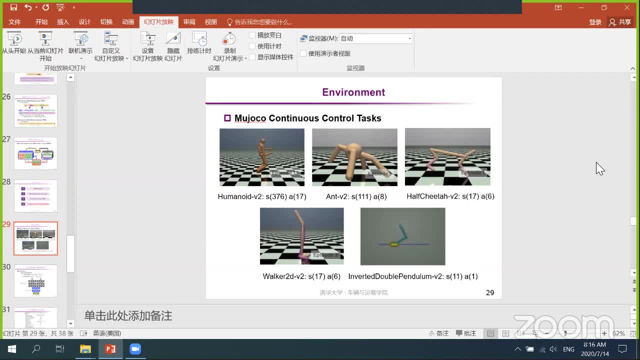 So there's one company in the UK So they are working on reinforcement learning application with real cars, But the safety is a major challenge for this method, So I would like to see So. reinforcement learning is a good technology. It may succeed in the future for autonomous vehicle, but there's a lot of work to do. 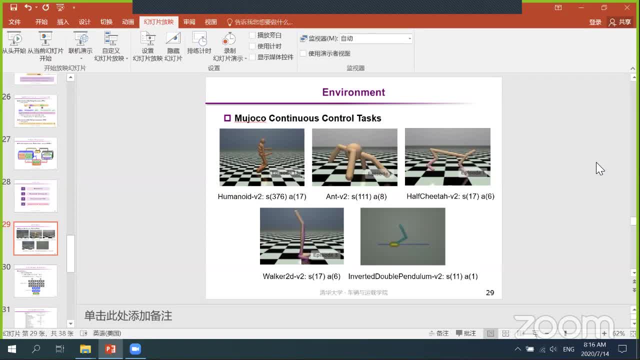 Yep, Well, actually a question that I have is: so: I come from, I guess, a reinforcement learning background as well, And I find it quite interesting, like the combination of reinforcement learning with autonomous vehicles. But what one of the- I guess one of the clashes I've always found is, you know, because it's such a safety critical system. 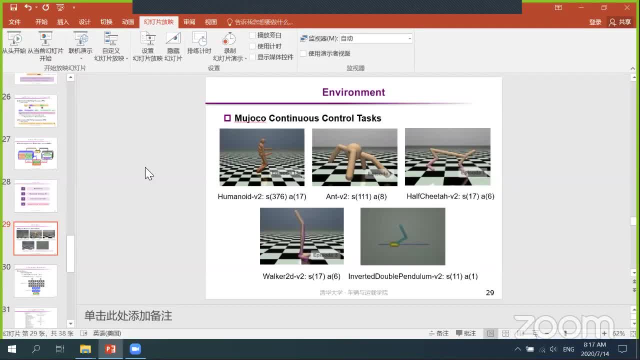 You know, what can we say with respect to applying reinforcement learning to autonomous vehicles? And is there, is it, is it, is it possible to come up with guarantees? And and sometimes, sometimes I think this is this is hard- But with, say, distributional software to credit, do you think there's, there's, a chance we could, we could give maybe more probabilistic guarantees or or confidences about the performance, like the performance, say, with reduced biases or or or things like that, to 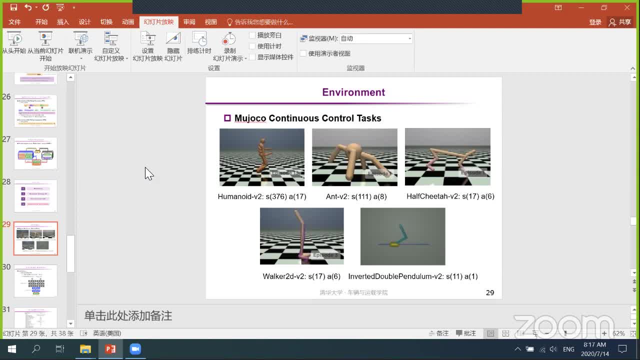 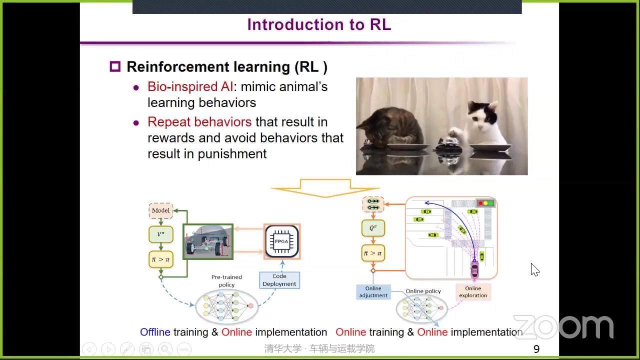 To, to, to kind of make Some some safety statements in the application of autonomous vehicles, But very good comments. Can I give more information about these comments? So I like to repeat this figure again. And in my idea I think, reinforcement learning- we have two kinds of new applications. 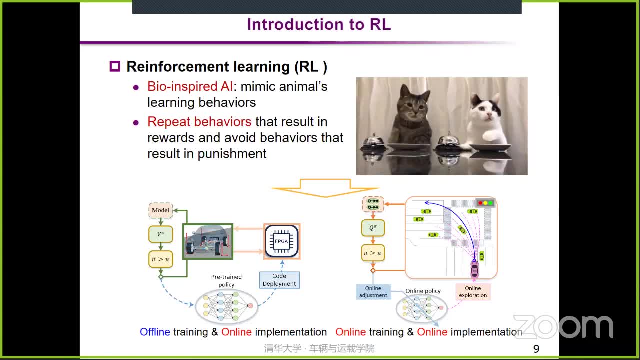 So I think reinforcement learning, we have two kinds of new applications. So I like to repeat this figure again And in my idea, I think reinforcement learning, we have two kinds of new applications. I think reinforcement learning, we have two kinds of new applications. 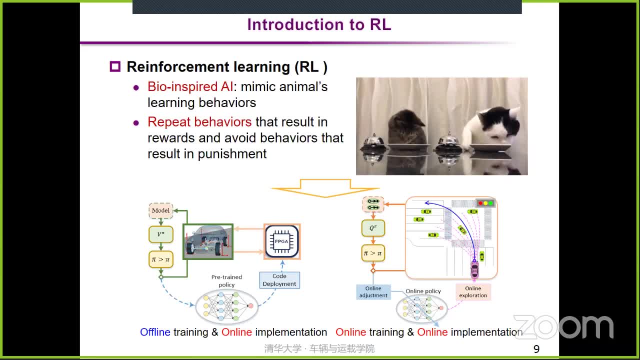 So I think, reinforcement learning, we have two kinds of new applications. You can modify the Vietnamese education ability. You can also call it using the buyer experience learning, more awareness. I mean, I just want to point that now, From the validation of the original forearm treatment, 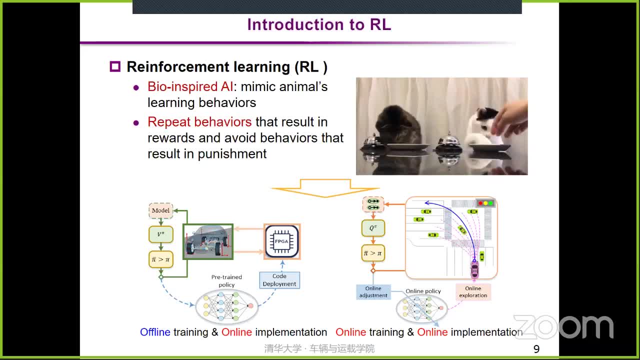 Effect why you are relationships More rigid, worried. Yes, Okay, go to next slide. Thank you of the optimal control problem Because, for example, MPC is very popular in many control field, And if we can put the solution of MPC into a neural network. 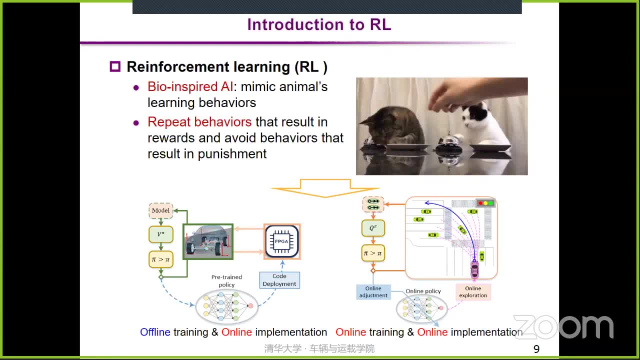 and then deploy the neural network in that MCU or FPG so we can kind of reduce the competing body. So the other way to use reinforcement learning is to use its ability to do the exploration or the self-learning ability. So basically this we need to combine. 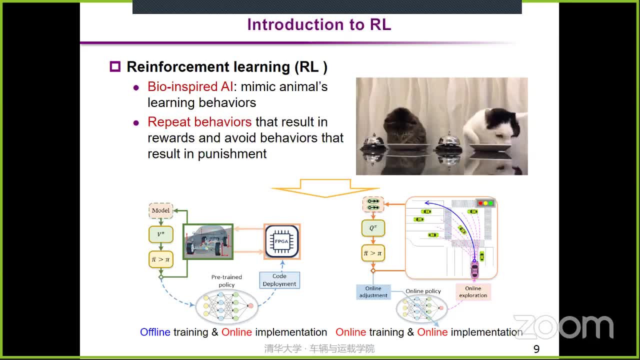 with the model free version of IO So we can let the vehicle to do several different behaviors and to randomly explore the environment and then get a better policy. So either of them need to consider the safety issue And so far we don't want to know that the car in the traffic. 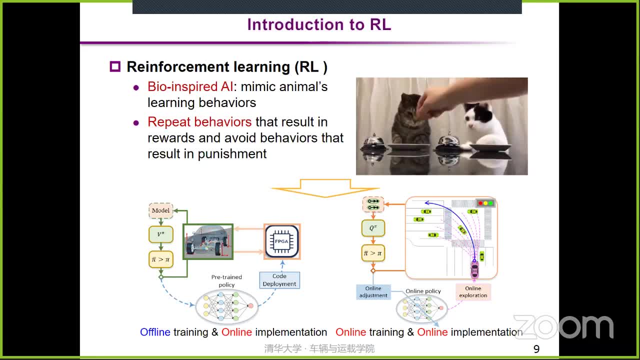 can have collision with other cars or some static object. So the safety issue is a very challenging issue. So there are several methods now in consulting the safety issue. So the first one is to consider the safety issue And the second one is to consider the safety issue. 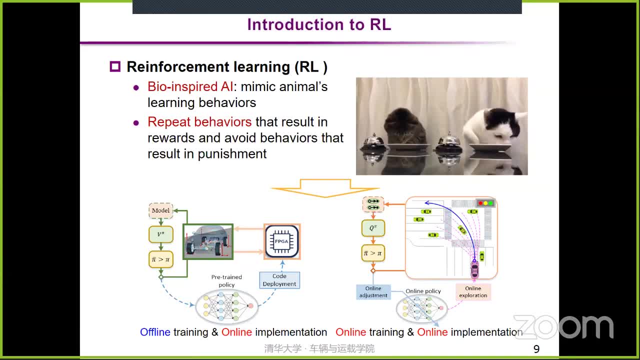 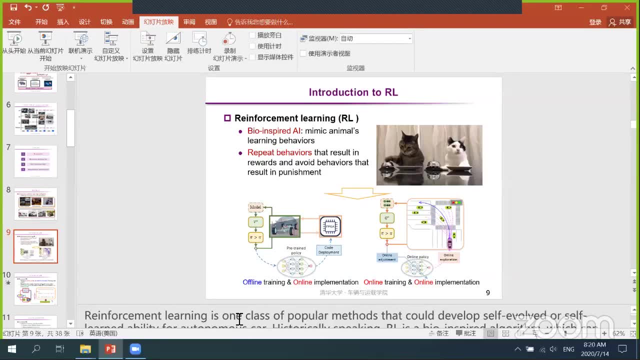 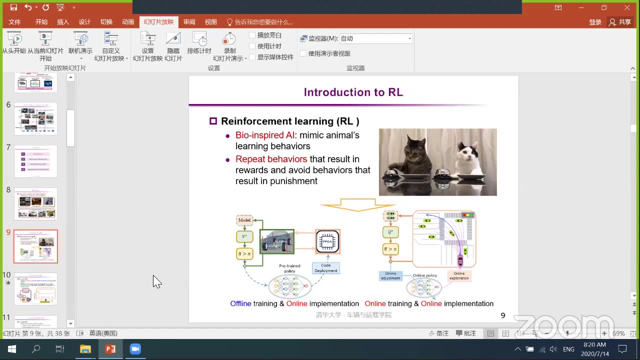 The safety issue is a problem, but there we have a long way to go. Okay, great, Yeah, thank you. Thank you very much, Professor Lee. So what I'll ask for you to do now is if you could stop sharing your screen. 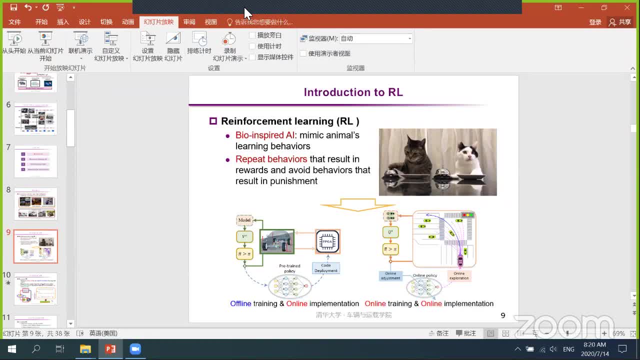 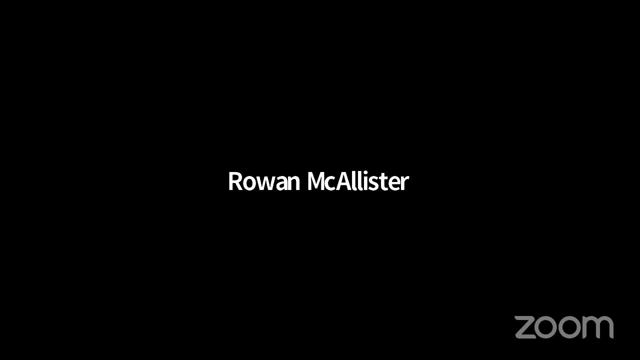 but stay on the Zoom call and we'll transition to our final event for the day, which is a panel. So the panel today is going to be moderated by Dorsa, And the way it's going to work is we have some offline questions that were precompiled. 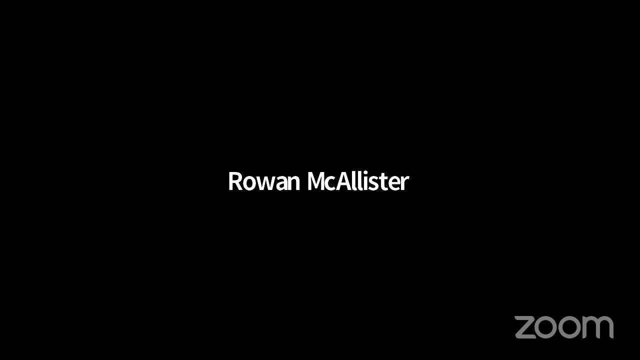 but we're really interested in audience questions as well, And so, again, anyone that's signing in to this call at the moment, if you have any questions for the panel, please enter them into the Zoom chat And we'll get to those. 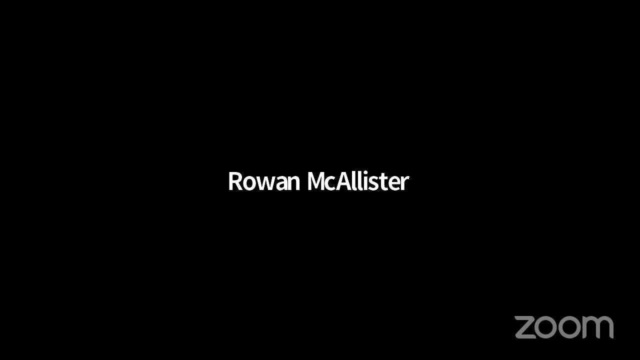 And then we will be looking at those as the panel progresses with its discussion. So very happy to have Dorsa to moderate the panel. For those that have arrived midway through, Dorsa is an assistant professor in the Computer Science Department and Electrical Engineering Department. 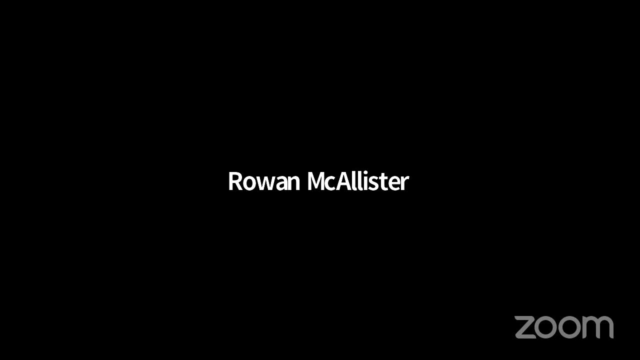 at Stanford University. Her research focuses on the role of digital technologies, such interests like the intersection of robotics and machine learning, and control theory, And her group works on efficient algorithms for safe, reliable and adaptive human-robot and generally multi-agent interactions. 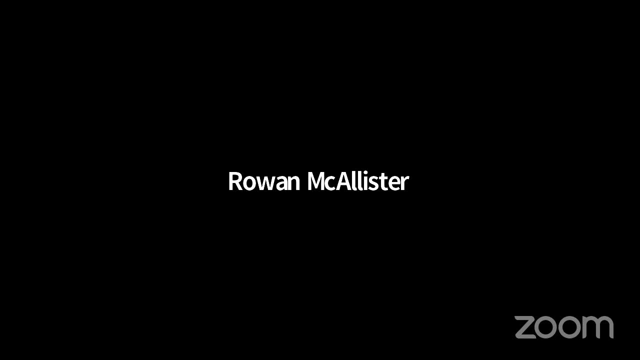 And I think most of our speakers will be at the panel, And so, Dorsa, whenever you're ready, feel free to go ahead, And if you have any questions, feel free to take over. We'll make sure that all the participants are unmuted. 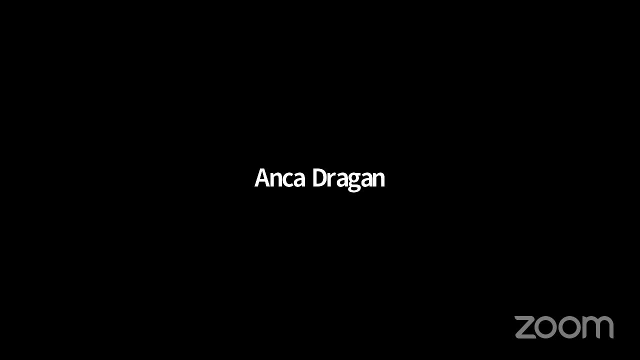 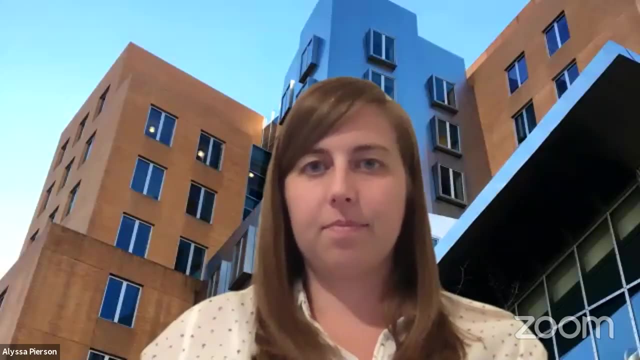 Hey everyone, Hello, Hello, Hello. Dorsa is still muted, Dorsa, can you not Dorsa? sorry, Hold on, Sorry, Dorsa. Yes, yes, yes, There you go, Okay. 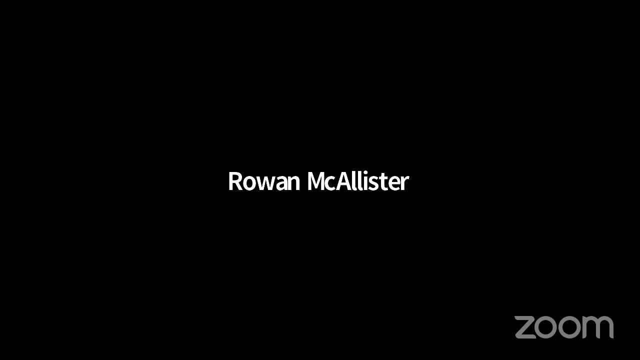 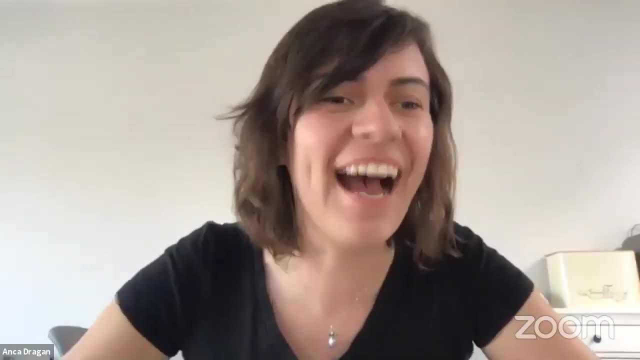 I was like: I can't unmute myself. Okay, Okay, So, Dorsa, can you unmute yourself? Okay, Okay, So, Dorsa, can you unmute yourself? Okay, Okay, Okay, So, Dorsa, can you unmute yourself? 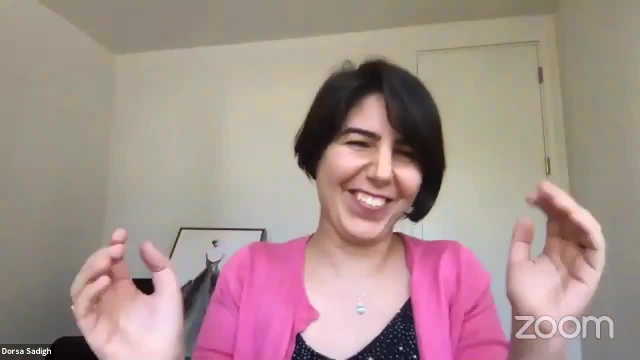 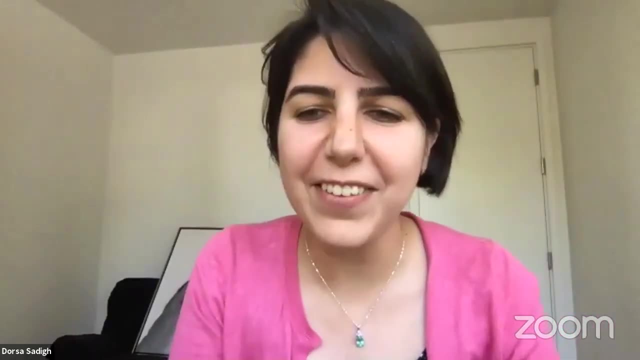 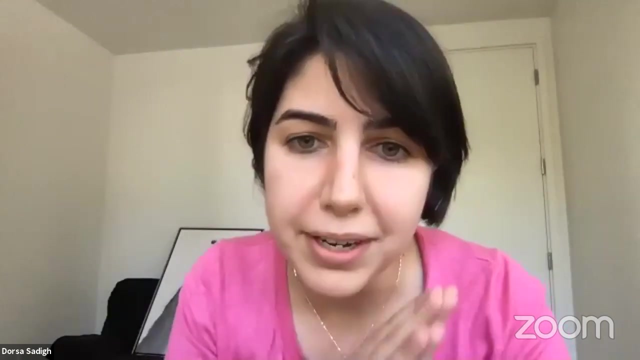 Okay, Okay, Okay, Okay, Okay, Okay. All right, Now this is going to be fun. All right, Hello everyone. Okay, So we have, we have, I think, most of the speakers here. So I think today in our panel we have Anca, Dragan, Charlie, Tang, Elisa, Pierson, Adrienne. 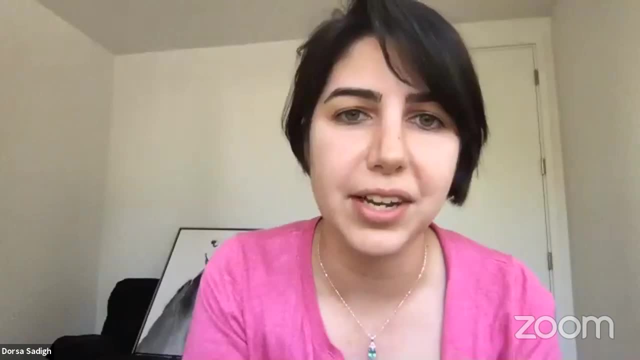 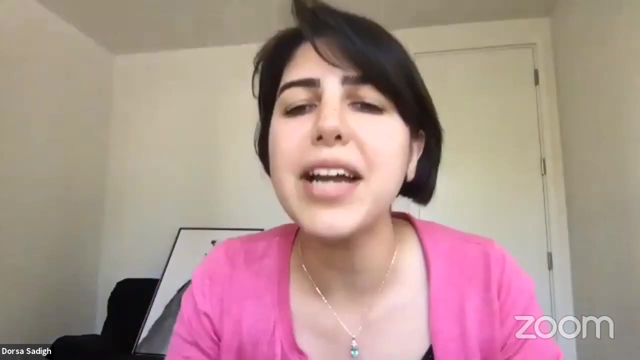 Gaden, Chang-Vu Lu and Chengbo Wu, who we just heard from. Is everyone here? Can you guys hear me? all well, Perfect, All right. So I think we have about half an hour, but we can go a little bit over if we need to. 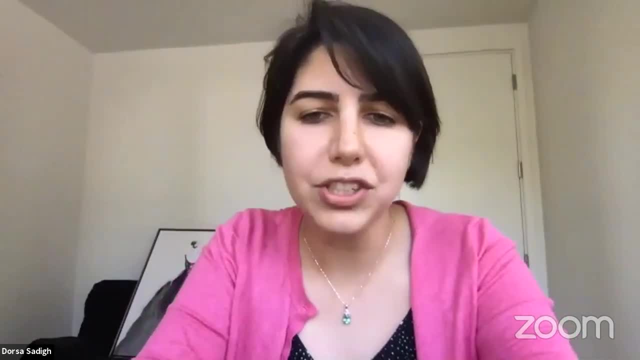 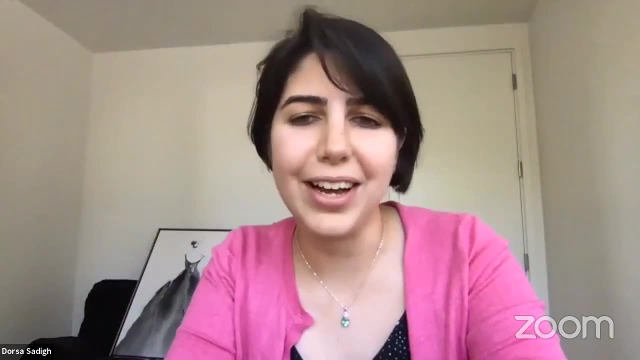 And I was wondering if we could start off- Okay, the panel with a few questions, and then we'll open it to the audience and hear from the audience and I. we were thinking the opening question could be something along the lines of why don't we have 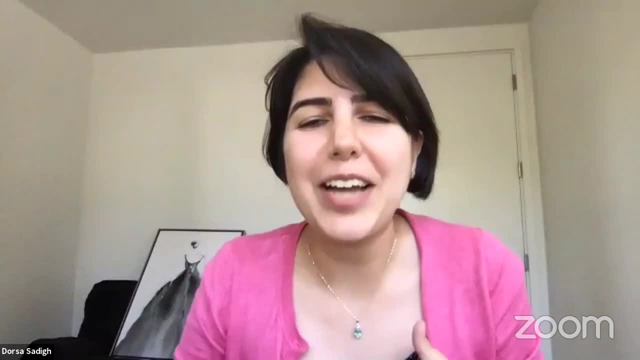 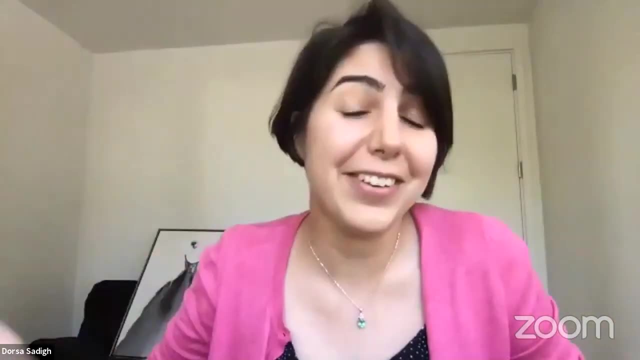 autonomous driving yet and and um, I know you might be tired of this question. I remember like when I started working on this, like we were thinking you'll have autonomous cars by 2020 and and we don't really have that yet. but if you were to pick like one major roadblock for not having autonomous 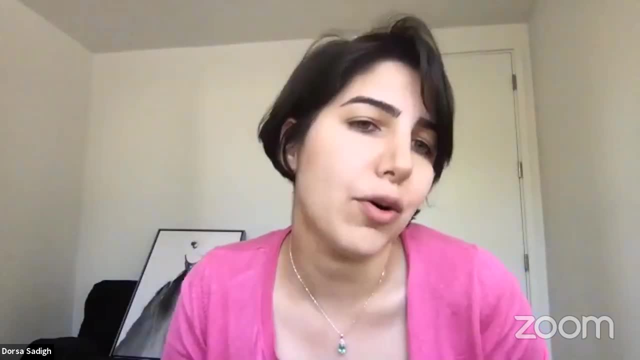 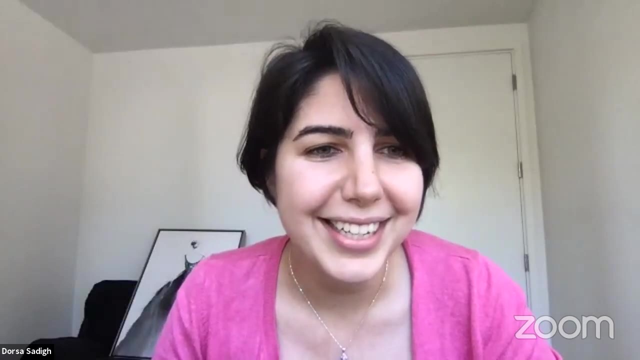 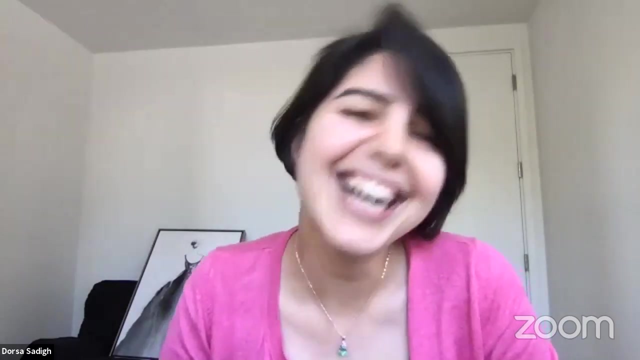 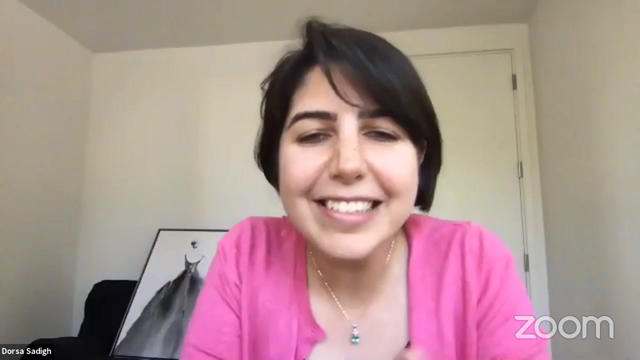 cars today. yet what would that be and how would you go about it? and I'll just open this up to to any of you guys. okay, did I pick on people? do you want to design someone first? maybe because that way it's easier versus waiting politely? yeah, so so I had this order on my list. how about we go in generally with this order? Anka Charlie. 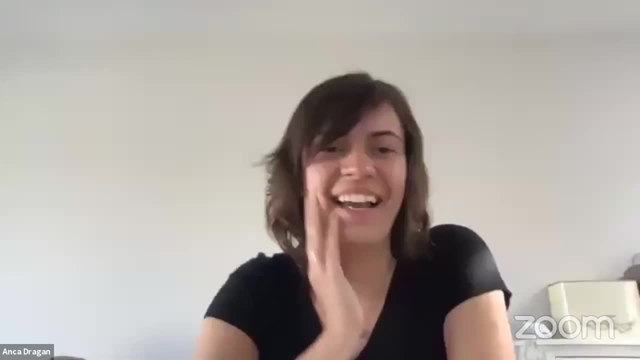 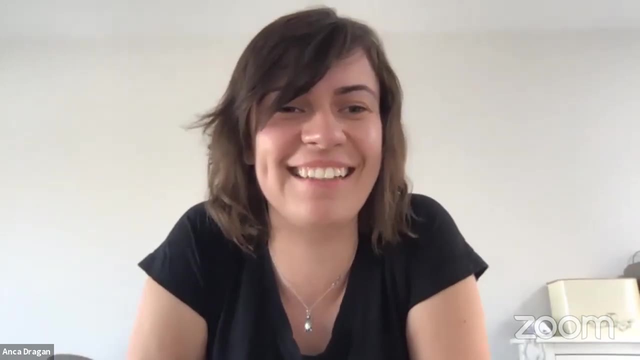 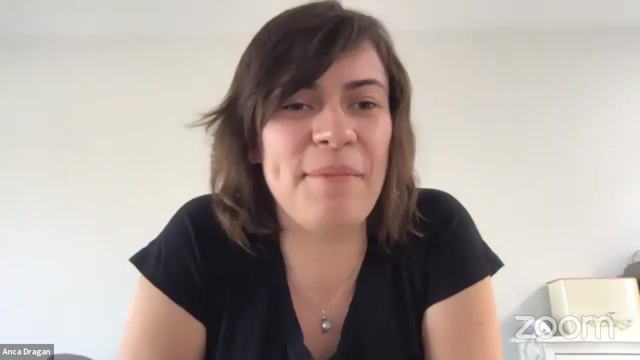 Elisa Adrian, Okay, but I don't always want to go first, but I'll go first now I'll give the cop-out answer, which is which is people, people are hard, like uh, uh. I would say that, if you know, take, uh, take a really hard driving environment like, say, San Francisco, because that's where I live and that's. 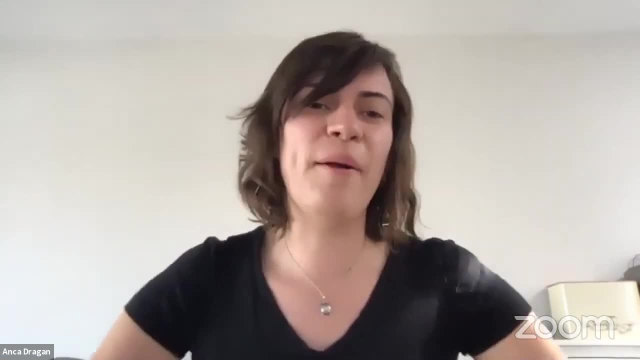 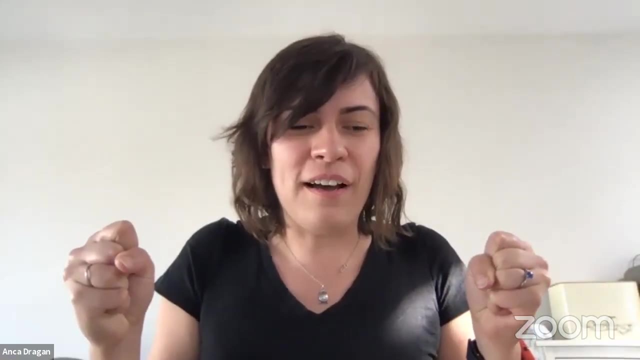 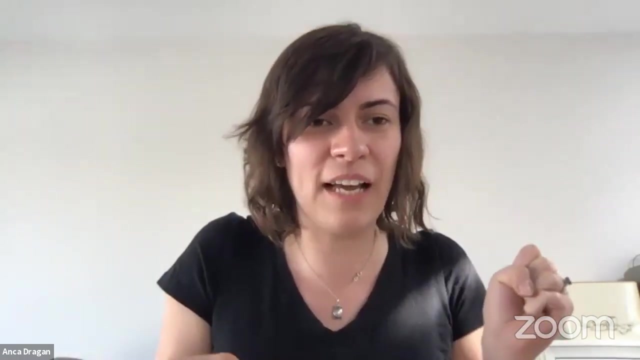 what I'm very familiar with, right San Francisco downtown, um, and now you know, just imagine that in your head and then take away the, the human driven vehicles, and take away the pedestrians, and take away the cyclists, and take away anyone on a motorcycle and what's left is: is you, that's it done, we're done. you know some people. 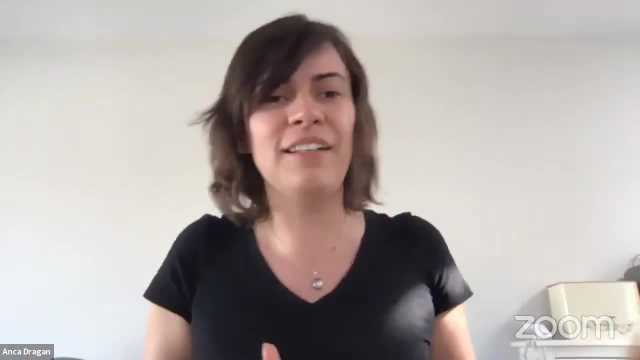 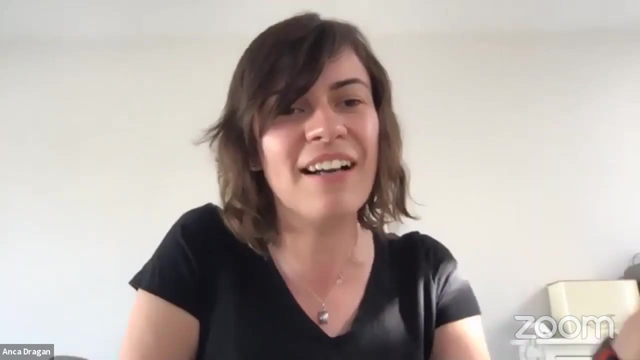 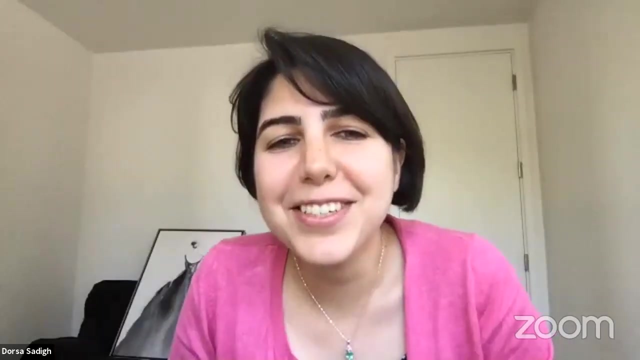 say, oh, but perception this and that, and of course, like maybe you know snow this and that, but like no, no, we're done, that would be done, everything would be fine right. so I think what's hard about the problem is is the coordination with people. but I'm biased because that's what I work on. 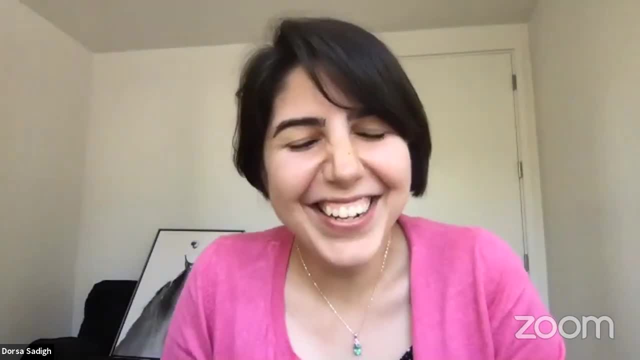 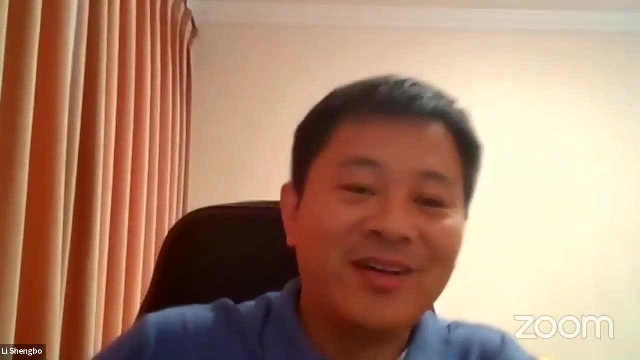 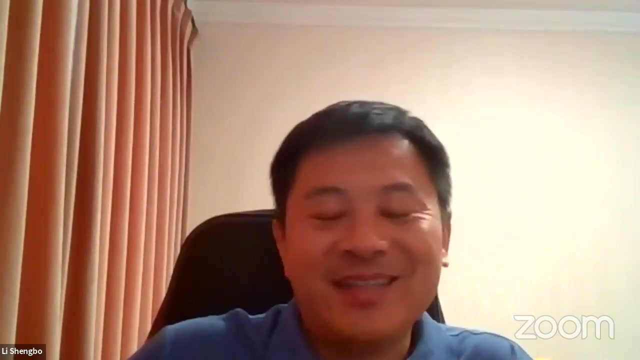 any other thoughts? can I, can I have some, some question for some, some answer for this question and uh. so first I want to say autonomous driving is amazing and it's the future of our road traffic and for me personally I really like it. but when we talk, I know autonomous. 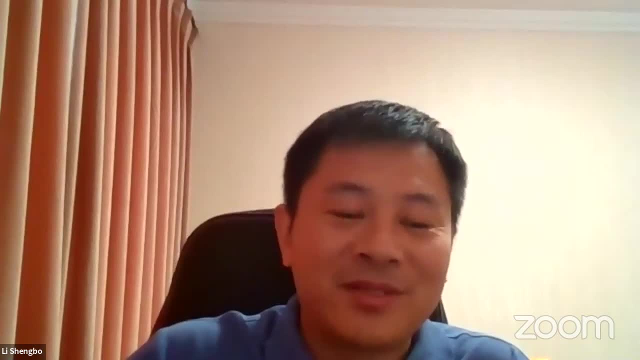 vehicles. we need to divide, divide it into several levels, like the SAE standard. so we have the level one, level two until level level five and for level one the level two. so basically we call it driver assistance system. it's it's already commercialized in our market. so if you look at, 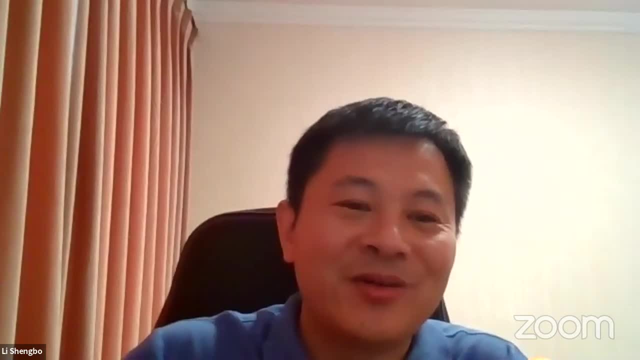 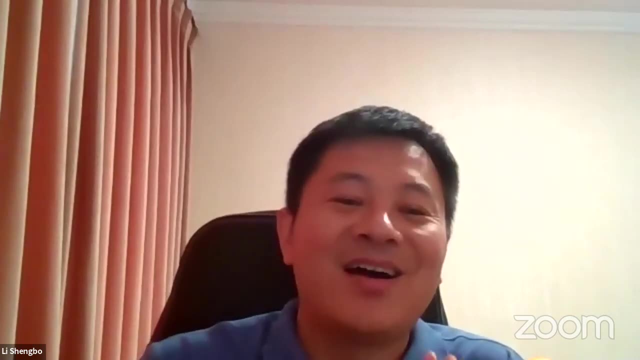 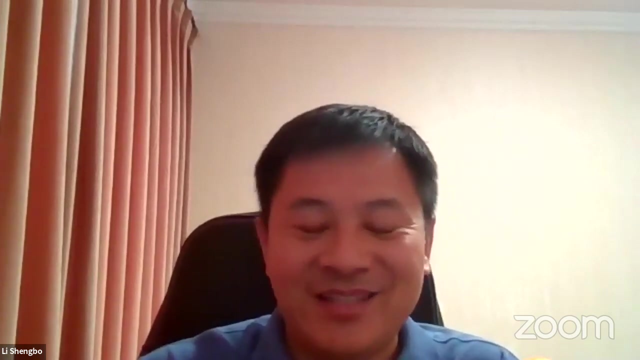 the autopilot of Tesla. you see, it's good. basically it's good, even though- and the manufacturer said, okay, it's addressing the system- you cannot use it as a fully autonomous vehicle. but you know, I think a lot of people want to try it and it's very. 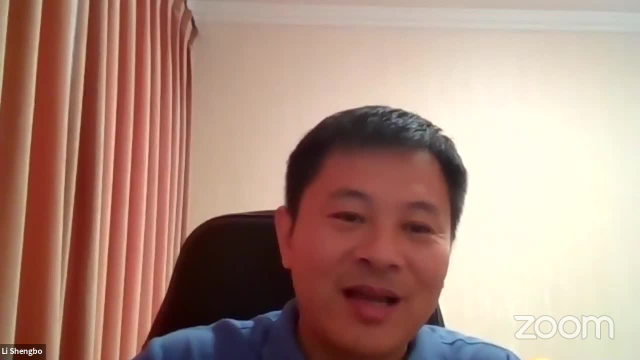 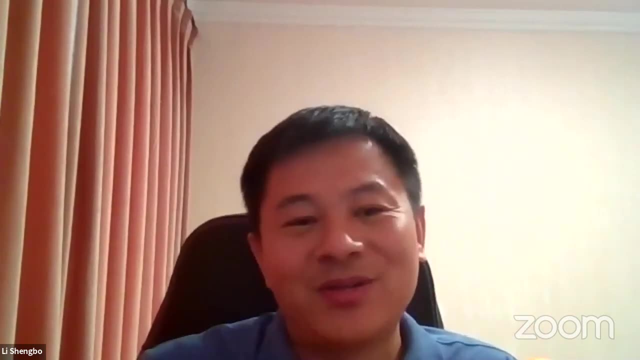 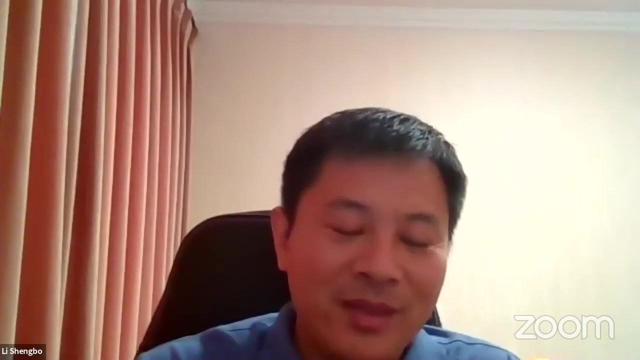 good, but when we talk about, you know, high level autonomous vehicle like the level four or even level five- the level five is our dream, so, which means if the people can drive the car to somewhere and the autonomous vehicle must go to that place, it's very challenging. so, basically, we think the 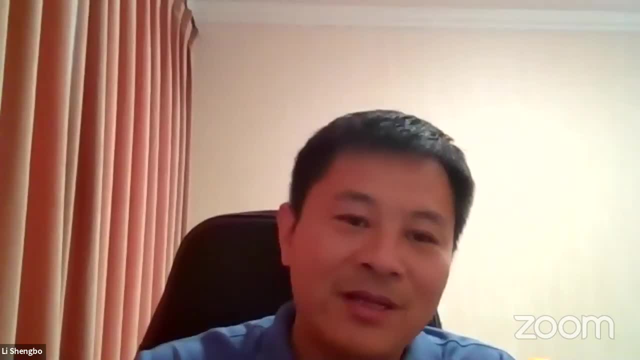 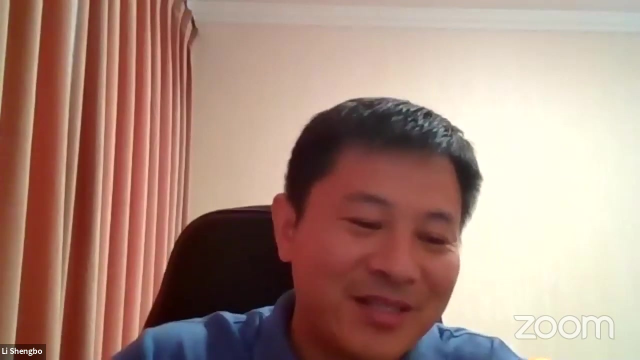 challenge happens in three layers. first is the environment perception. second is the decision making, that is, the motion control. so you want environment perception. still is not perfect. it's very good and but but still far from the perfectness. there are several reasons. why is? the road users are very complex and we have this. 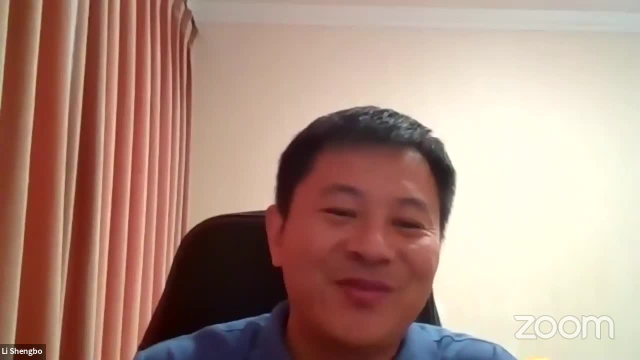 kind of losers. so if, if you come to China, if you drive a car in Beijing, you're saying, oh, that's horrible traffic. and and also the decision-making, decision-making, uh, is very challenging. and now for the low-level autonomy: conversion or decision is easy because we can design a role-based decision and it seems we 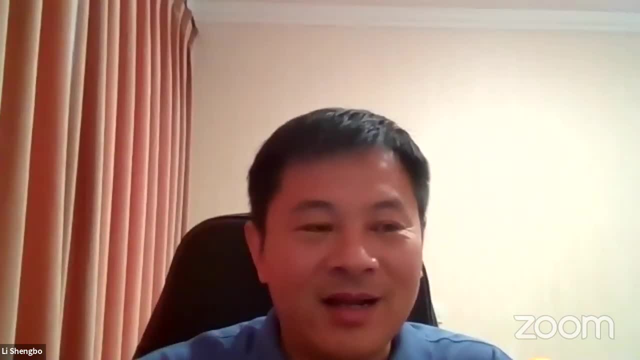 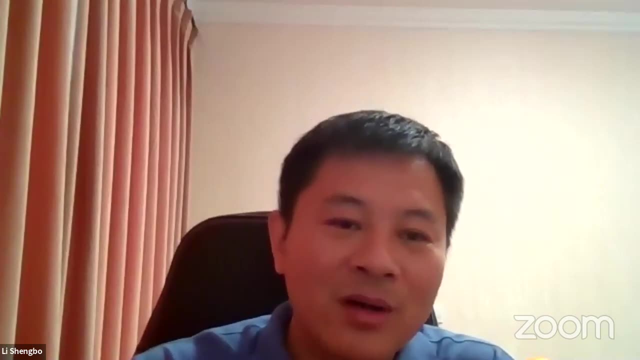 can apply it successfully. so we can let the car, for example, go straight or do lane change overtaking without any problem. but if you want to put the car into the city road conditions, to find more traffic, you have to put the car in the right lane and the lane change over time. you have toひao. 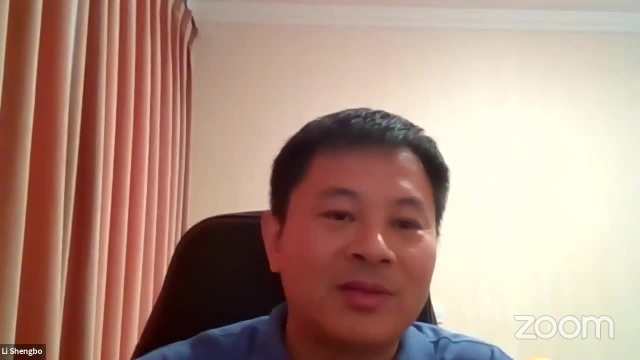 you have the mixed traffic flow and it should be very challenged. i think robot method does not work right. we need to apply other method, for example reinforcement line, even though we haven't seen any success applications of this method. but it's the future for the disservice algorithm design. 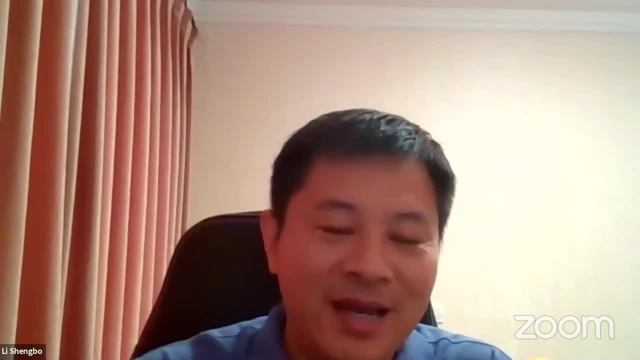 add motion control. i think for the normal condition it's okay and we can apply in the model predict control method as the motion controller. it works very well. but still we have a lot of, you know, other challenges, for example how to control a car in the handling limit. so because 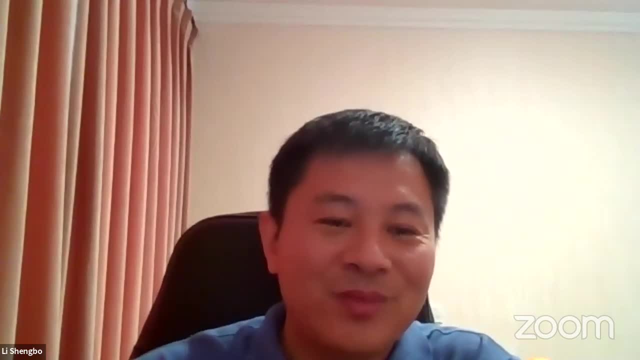 we know that in the low frequency road so the car may drift out and some good drivers can adjust car. but how can atoms controller can do that like human driver? it's still a challenge problem for us to do so. some comments about this question. yeah, i think we have a lot of work to do and 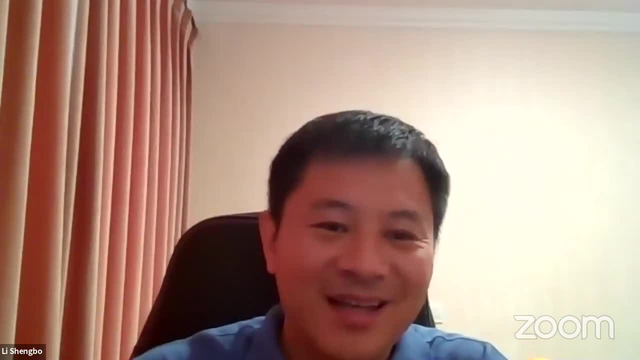 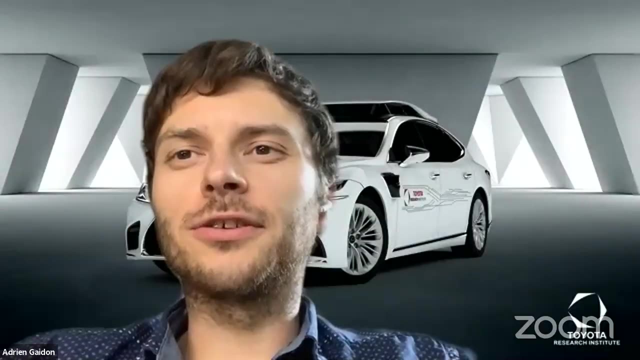 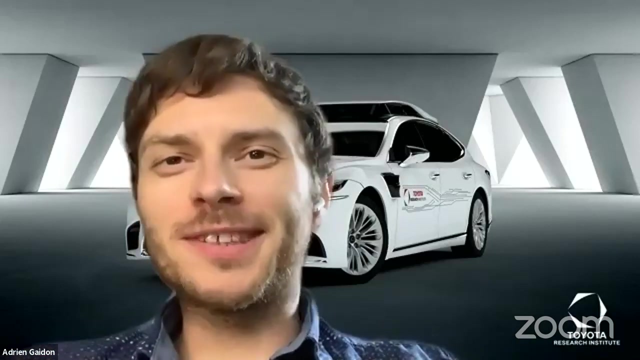 in almost all tasks of autonomous driving, and it's good for researchers and maybe a better idea for the market. i i agree. actually my talk was very much about that because i think, um, you know, toyota and tri in particular, we've been the most pessimistic about this. 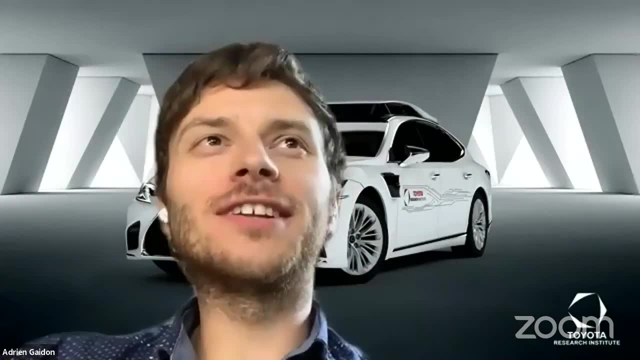 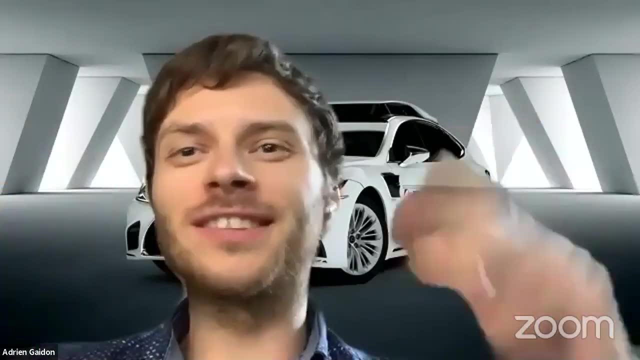 uh, we we started late on the autonomous driving, to be honest, because we thought it was very hard. then we we started the first thing. we said it's very hard and probably you know there's some dunning-kruger effect, like everybody thinks it's easier than than it really is. um, and and it's funny because 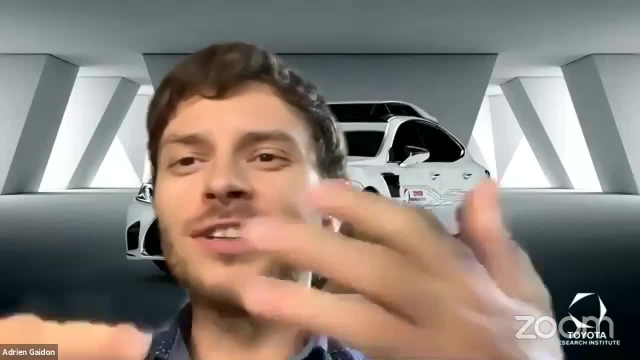 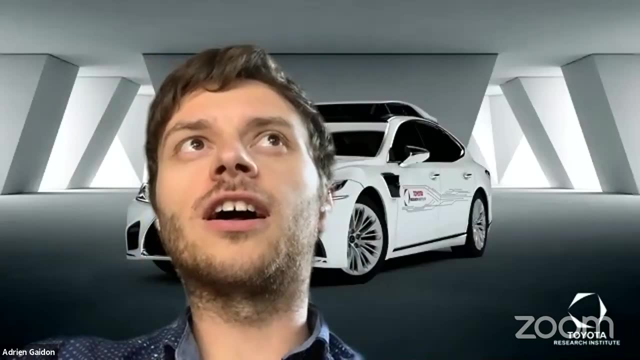 like now. people are saying: yeah, it's actually really harder than we thought, and there was recently an interview with gil pratt, our ceo, where people said: hey, this guy, he said it was hard, yeah, it's really hard, and actually i agree with wanka um i'll. i'll modulate this, though, by saying that: 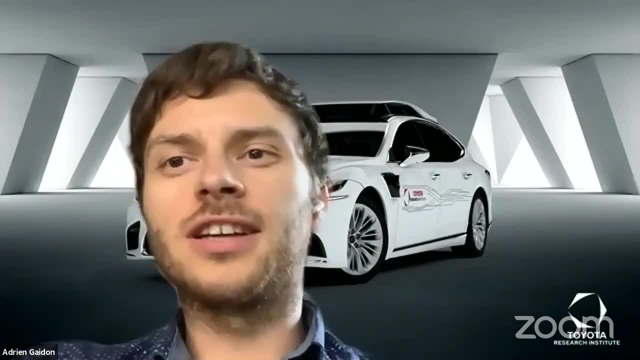 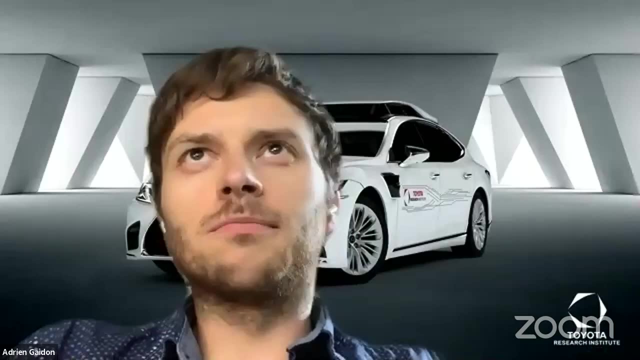 i think the whole stack has open research problems every part. um, so i talked about the three r's and p's, that was my title, and this is like that perception. perception sure is mostly solved, except in the long tail, and we know that it's kind of like eight, eighty percent, twenty percent of the. 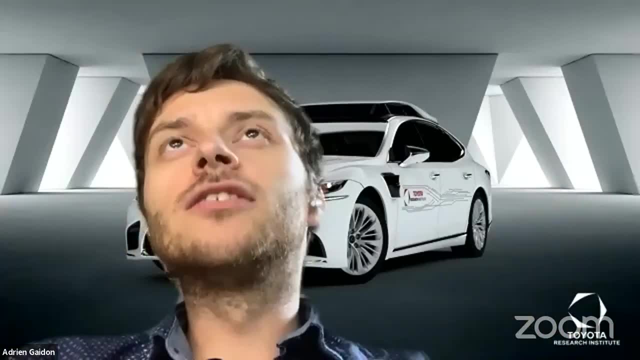 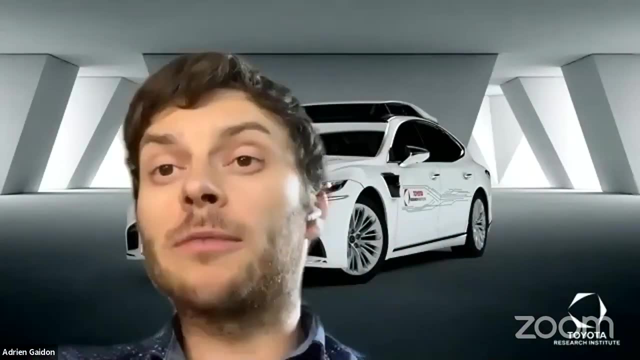 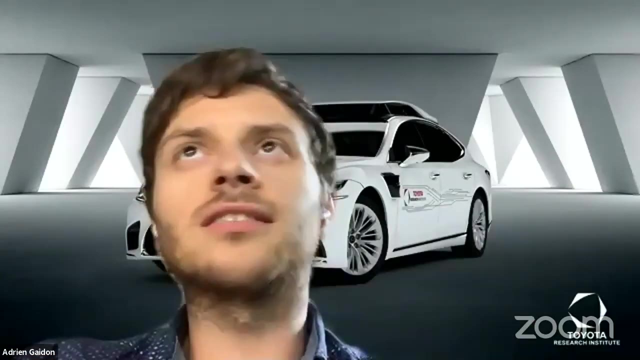 time to get to eighty percent right and the follow-up. so i think, like robust perception, like perception is solved, sure, robust perception, any condition, not so sure, um, random, like prediction, prediction probably the most open problem. right, and that's where i completely revonka the human element. right, it's randomness, contingency, intense multimodality, uncertainty. 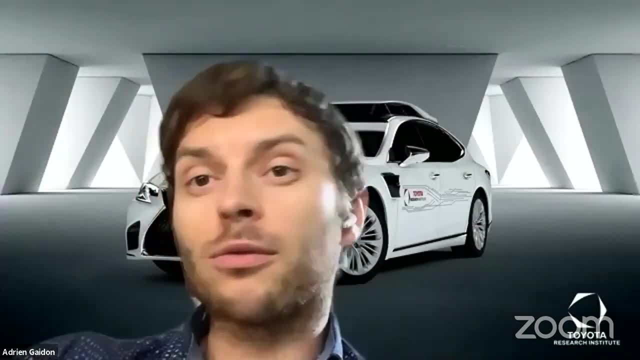 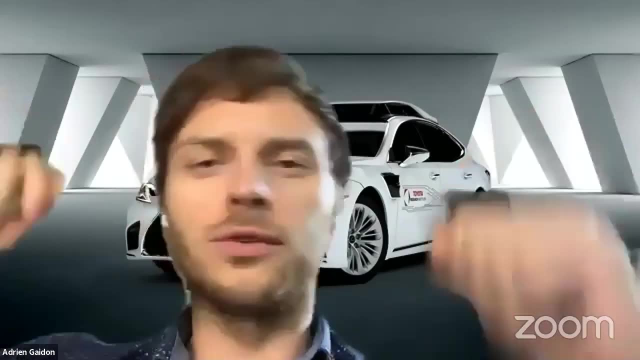 um, planning too. planning too, i mean for me, i don't know. i work with you, dorsa. i work with a lot of very cool folks at stanford on control and you know, coming from the computer vision field and thinking control is solved. you know, some russian guy in the 60s solved it and then learning how. 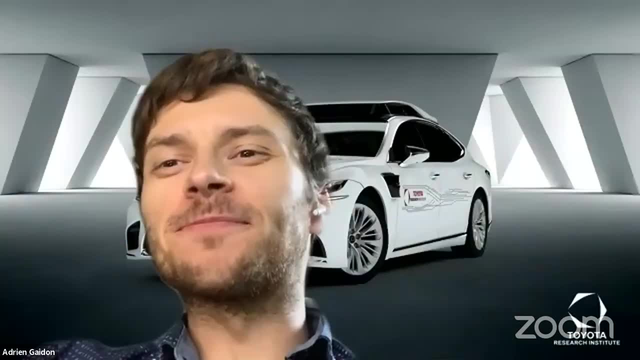 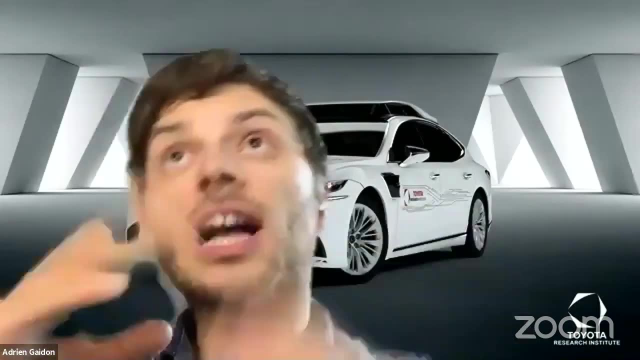 wrong. i was, uh, as always, benning fruger again. um, but in planning there's just so many open problems, so many many open problems, right and and then, if you look at everything, causality, i think, is one of the big ones. i mean, like you know, safety is obviously another big one, but in particular, 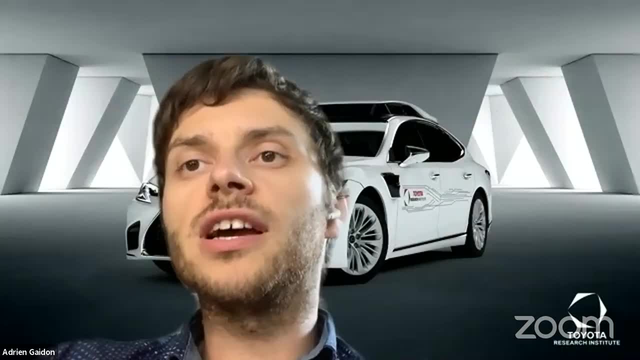 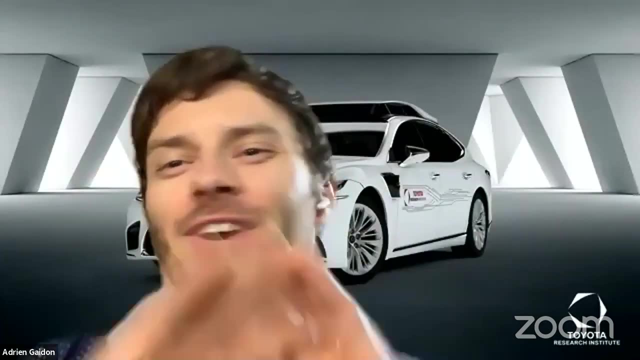 one of the conclusions i wanted to make in my talk about this of why we're not there yet, is because, because there are problems everywhere and every abstraction is leaky, the whole system is just so far from working together in coordination, uh, throughout. so we have like 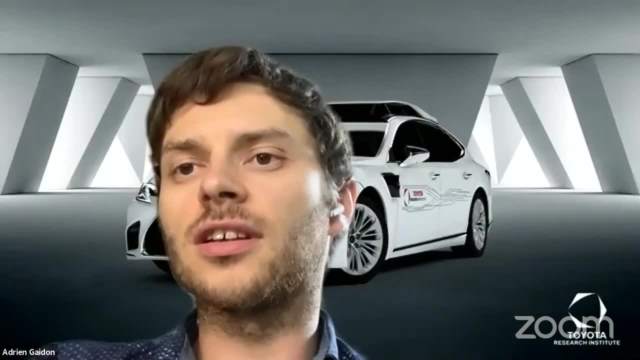 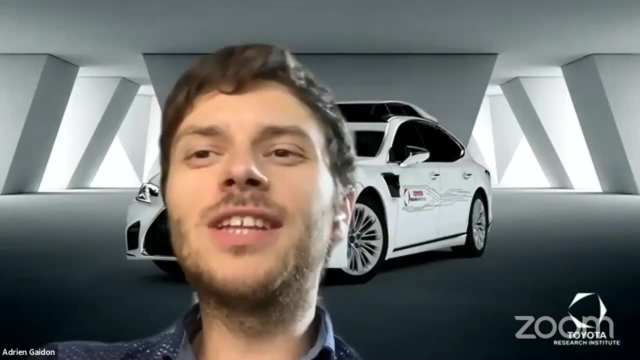 really good demos, like getting to a demo. people have been doing very successfully at this, like even back in 2009, you know, with google um. but making a product, uh, even in very restricted settings, it's difficult. so i think it's just much harder than everybody thought. 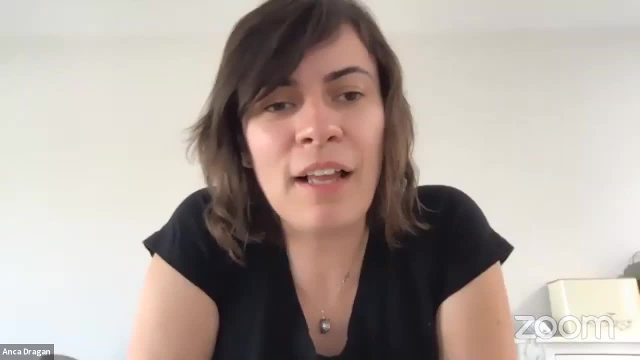 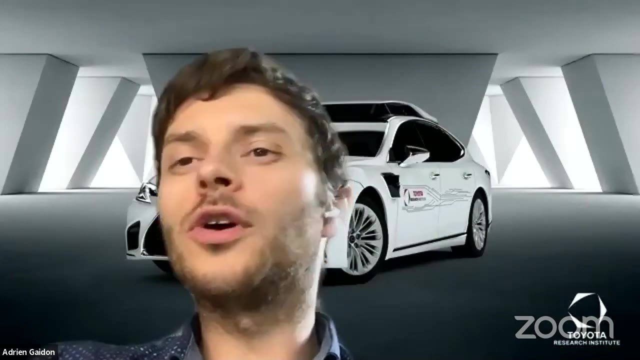 the world is open. so that's hard, oh, but no, elon tells us that it's going to be done by the end of this year, so we're, we're actually good. uh, i wait, are we in 2016.. oh, no, wait. oh, also on this. 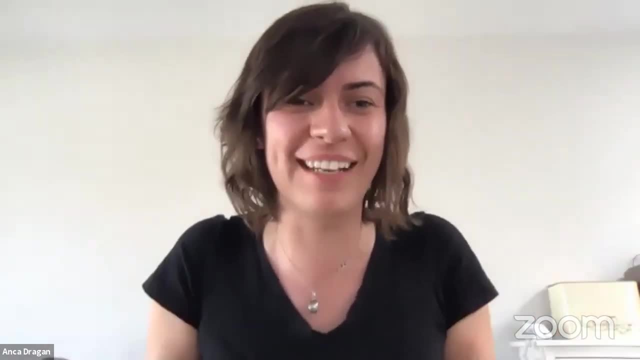 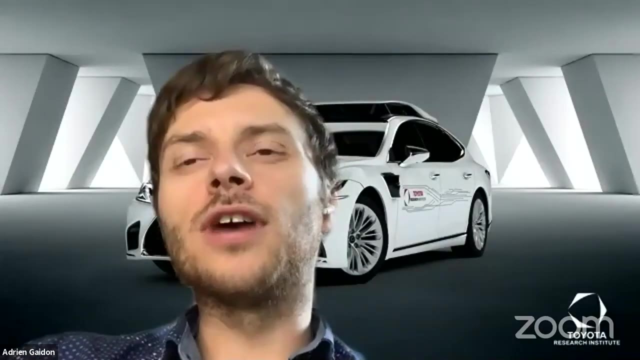 panel. i'm very much not a waymo person, i'm very much just my normal uc berkeley self. so don't take anything that i say as well. it's good. i think optimism is good. you have to be optimistic, right. it's like feynman, etc. like you have to believe you can solve the problem. right, if you don't believe. 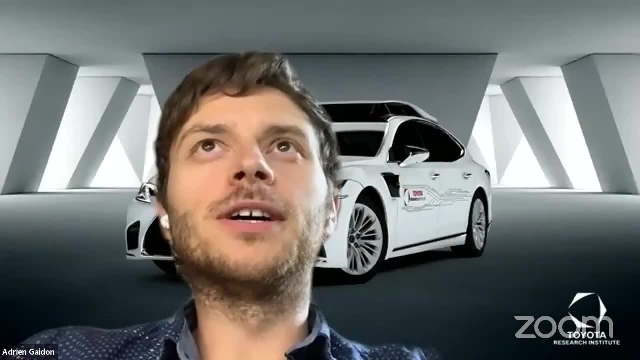 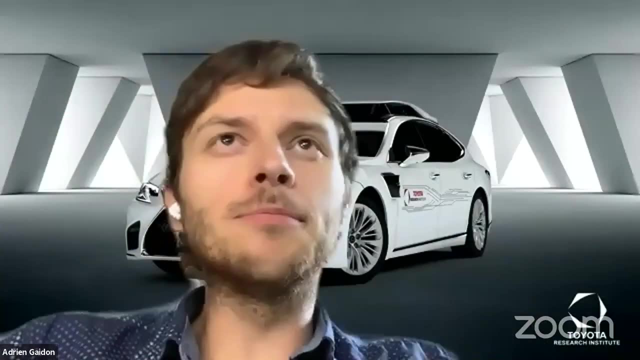 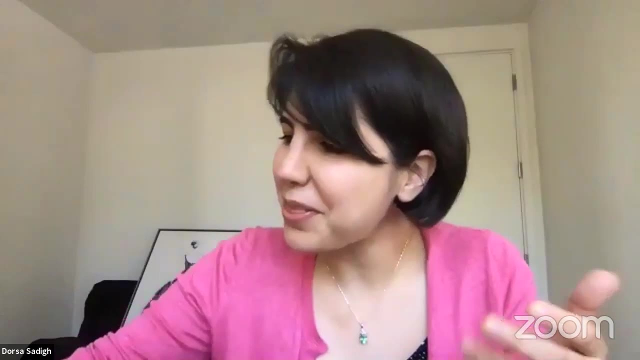 the problem? why are you even working on it? but but going from i believe i can solve the problem to the problem is solved. like i'm disclosed repeatedly, there's a bit of a bit of a gap that some people are not comfortable with jumping over. so i guess, building on that and and i want to think a little, 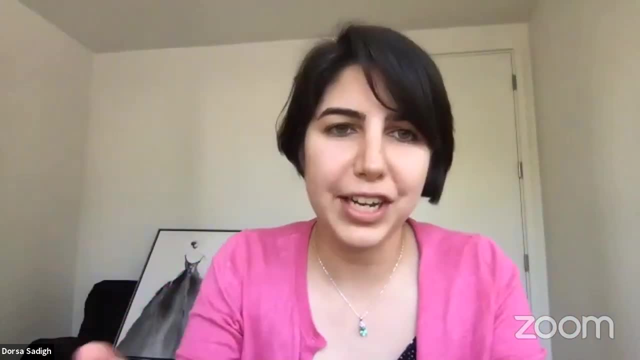 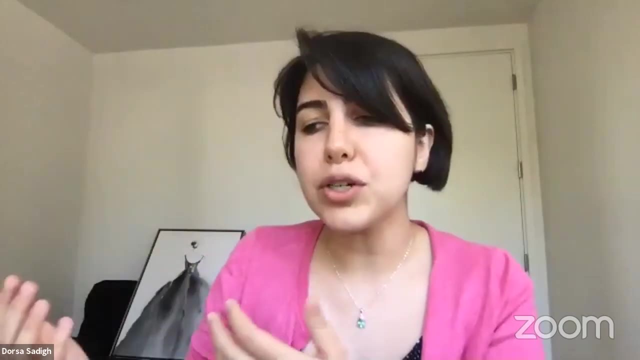 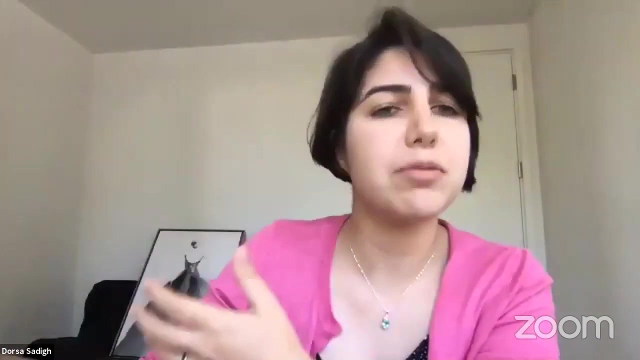 bit about some of some of the different approaches that we discussed today, right like we. we heard about, like game theory ways of looking at driving. we heard chang lu's talk. we heard anka's talk about like um driving and and twin types of ways of looking at uh driving, and and more like. 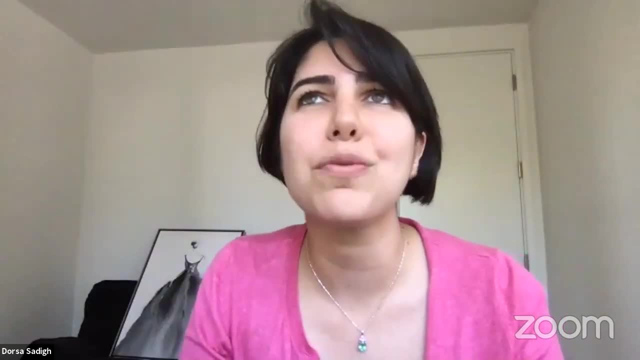 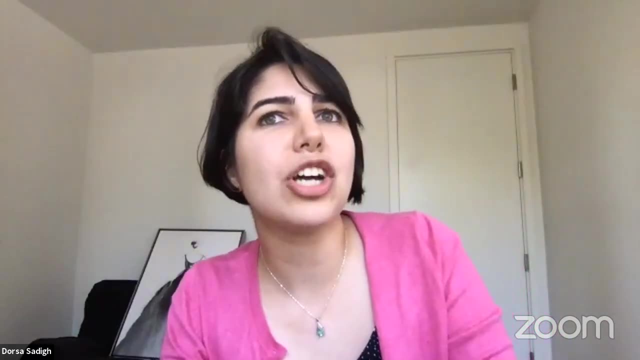 reinforcement learning and different types of learning paradigms that one can use, and- and i don't want to ask the question of should we go model based or data driven, because i don't think that's it- that's the right question to ask here, but i do want to ask this question that in general, 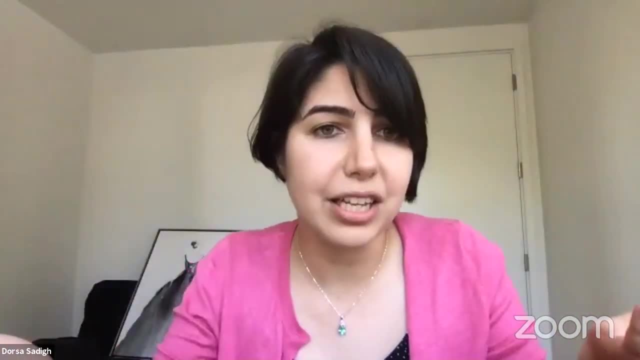 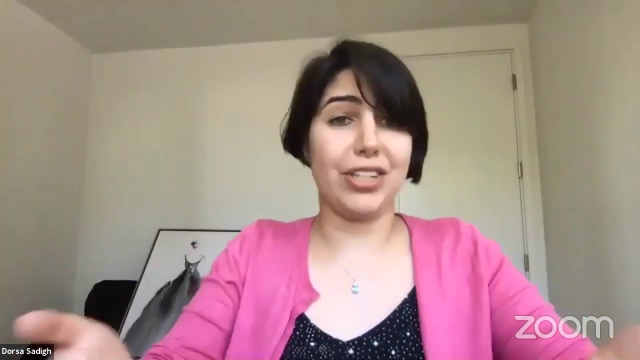 if you're designing your autonomous car, like today, how do you think about integrating these different techniques, like- not like you might want to use, like a learning based approach somewhere and a model based approach? but i think this is a bunch of problems, like, as adrian was saying right, like 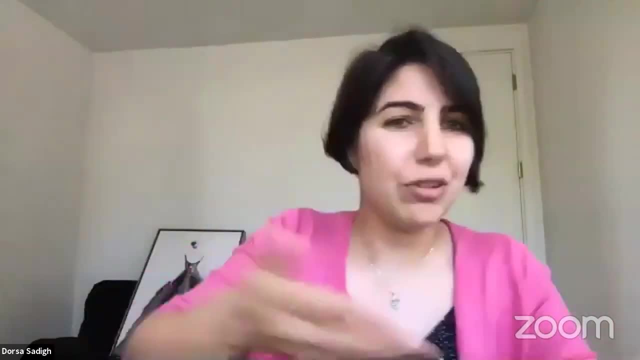 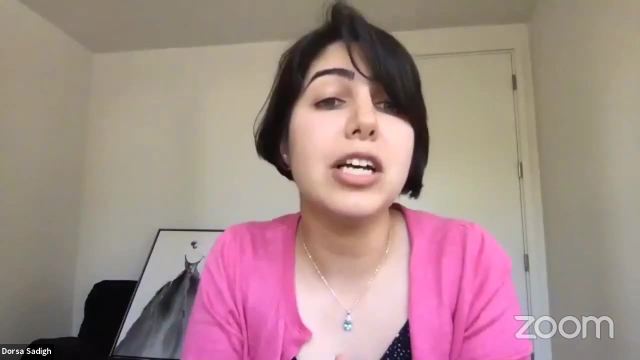 you have these different modules and each one of them have their own issues, and then they leak to each other. so how should we go about actually like integrating these different, different types of- uh, types of approaches, or or should we like- i will ask that too- should we like take an end-to-end? 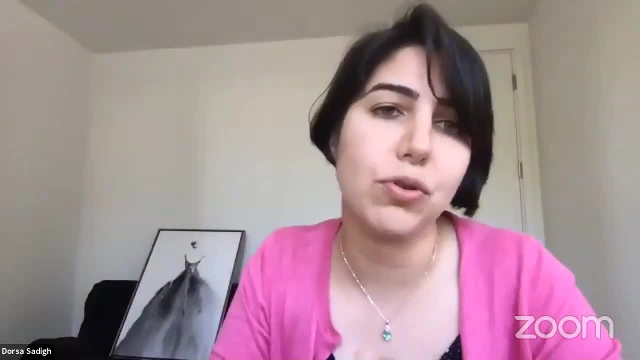 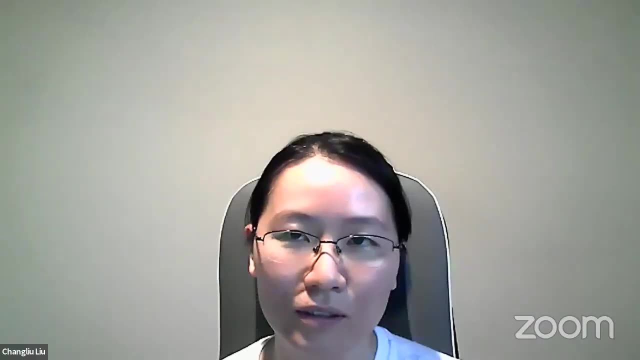 approach towards driving, or should we take a very specific type of type of model? this approach towards driving, um, i was wondering if uh chang li, do you have any thoughts on that? maybe you can start. yeah, yeah, also a question i've like, a lot i've been thinking about for a long time. so, in general, i would like 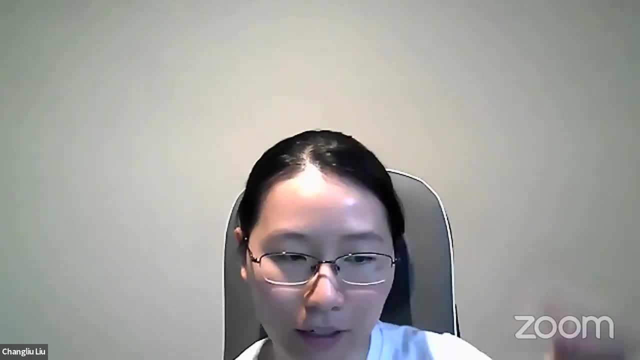 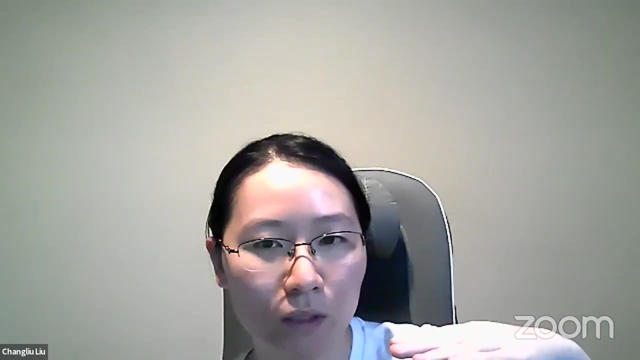 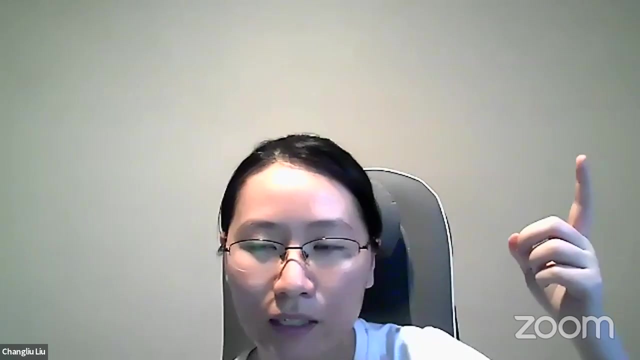 to say for the uh, like an autonomous system. an autonomous system or autonomous vehicle has full stacks, and if we're getting to the lower level or more physical level, we'll care more about the safety, and if we go upper level, we care more about the intelligence. and then this: 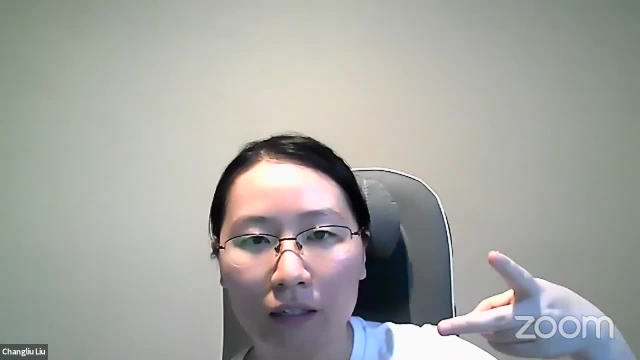 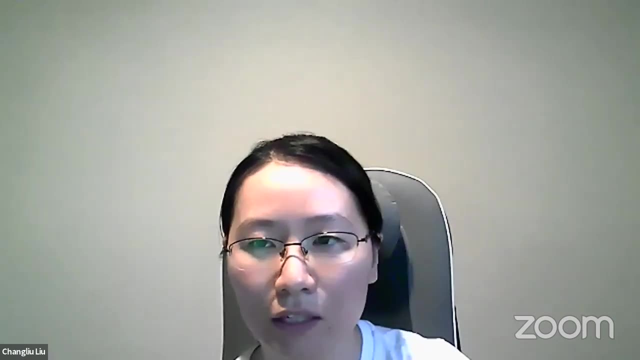 gave us a way to kind of leveraging that advantage of learning based method and the advantage of control-based method, because control-based method can usually provide us some sound guarantees against those uncertainties. so usually we tend to use more model-based approach in the low level to make sure that there's kind of a safeguard about the actions finally generated. 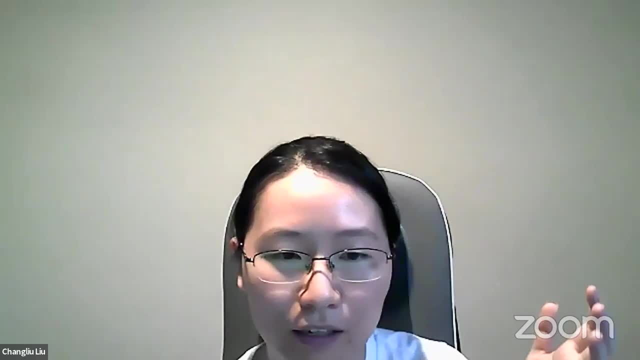 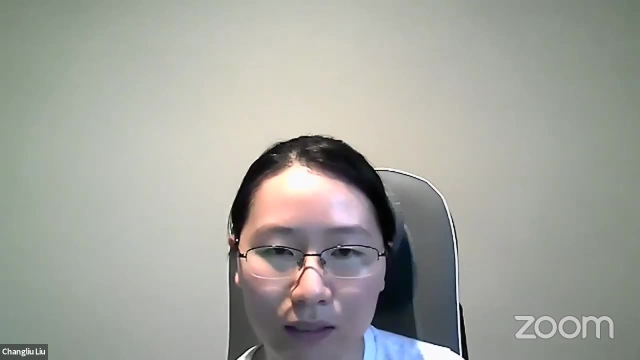 by the vehicle and if we get into high level, there are a lot of difficult interaction problems to reason about for the autonomous vehicles, and the learning-based approach can help us distinguish those complicated patterns from the other learning-based approach and then we can start to think about how we can make sure that our learning-based approach can be more human-like. 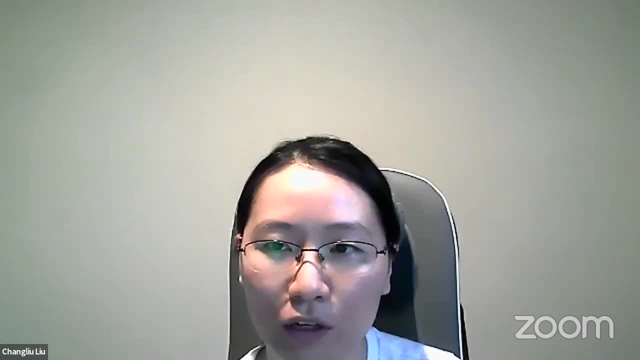 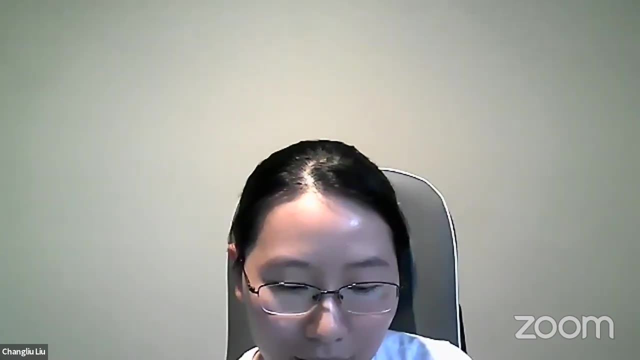 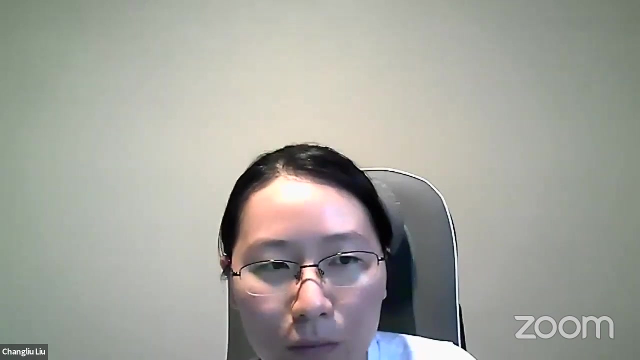 and more natural and more human-friendly. so this is one way, and also for end-to-end approach, i think i i although i'm not a big fan of end-to-end approach, but there's a lot of current work trying to make end-to-end approach more explainable. i think the the major problem of 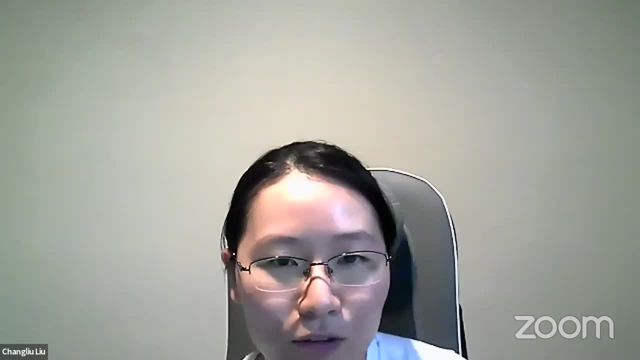 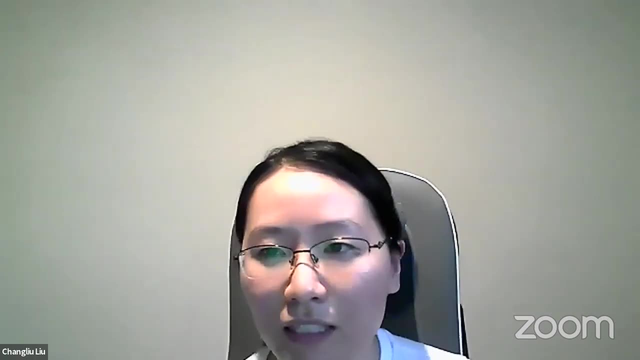 end-to-end approach is that it's not just about the data, but it's also about the- the other side of the spectrum. so it's also about the- the different ways of making your learning better, but also the different ways of making your learning better, and i think that's. 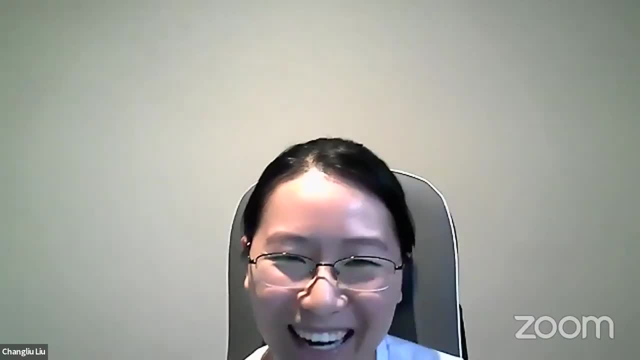 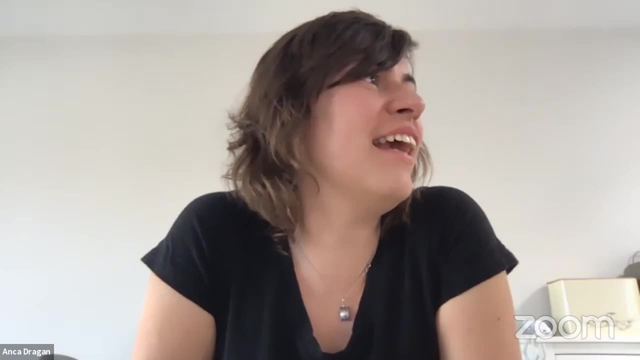 the one thing that's really interesting about the end-to-end approach is that you cannot explain if something goes wrong. but if we can make end-to-end approach explainable, i don't see any problem with that. yeah, so that's my thing. can i debate this okay? 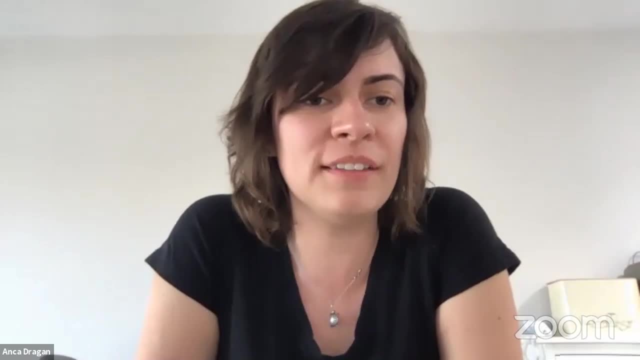 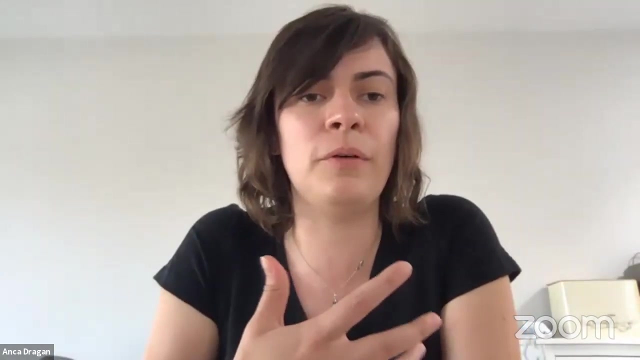 so. so let's see. i mean, i think I'd say maybe the thing that's related that can be a problem is, in a sense, debuggability. So you want a system that you can test out and improve, And when your main way of doing that is some form of messing with the data, right and 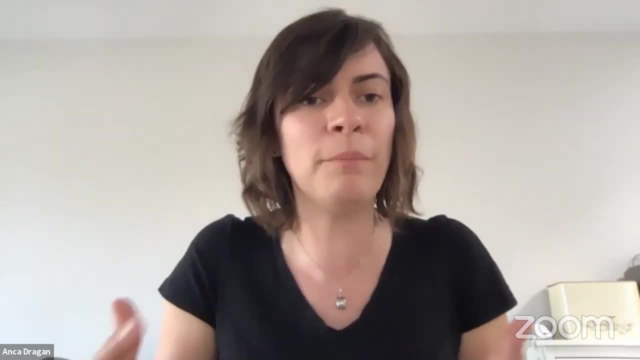 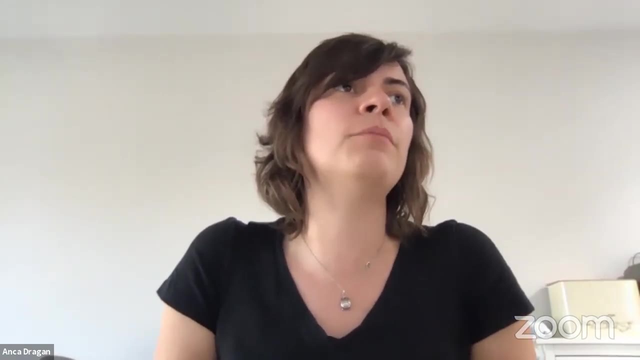 you can't necessarily intervene in other ways. that's a problem, But I think that there's also ways to address that, What I worry with. so I think so there's a few things that we should maybe have common ground on when it comes to terminology. 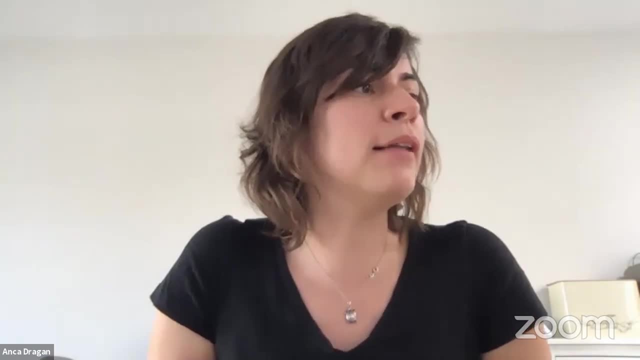 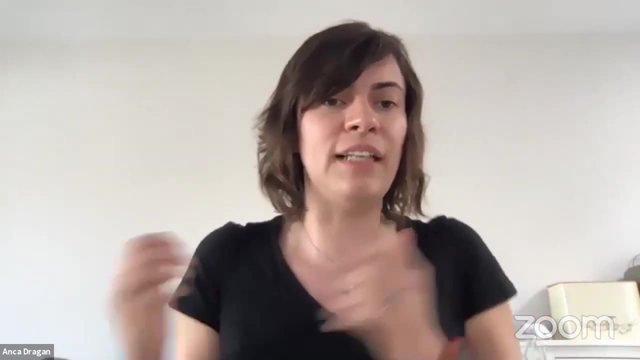 So you know, sometimes we make the distinction between end-to-end and sort of like non-data driven. So is it like planning-based or is it data-driven? And to me that's not really a distinction. It can be both data-driven and planning-based. 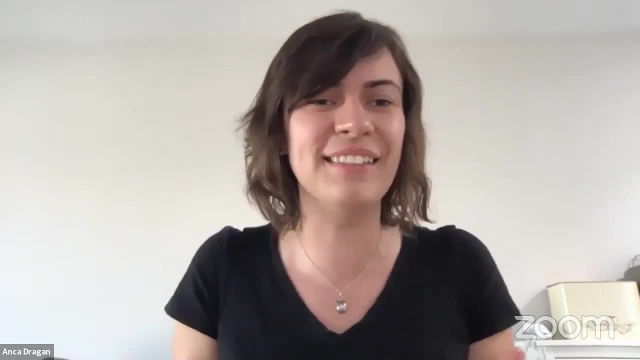 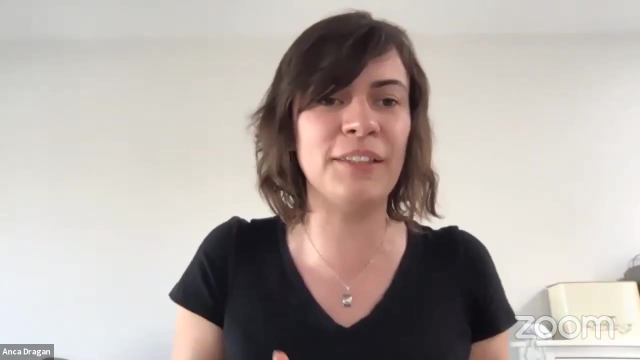 And I think it should be both data-driven and planning-based. And then there's you know sometimes. So I heard Lee talk about rule-based right- A control can be rule-based. Well, when you have a policy, merge out of doing optimal control, whether it's RL or 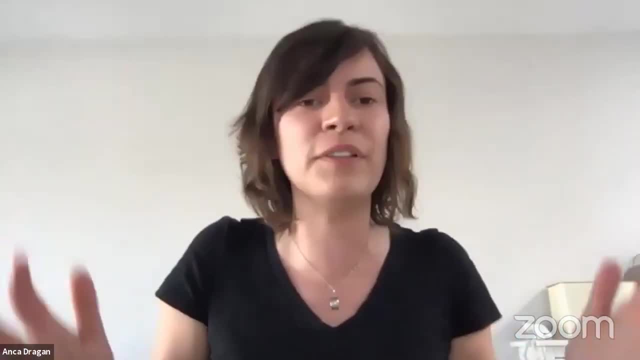 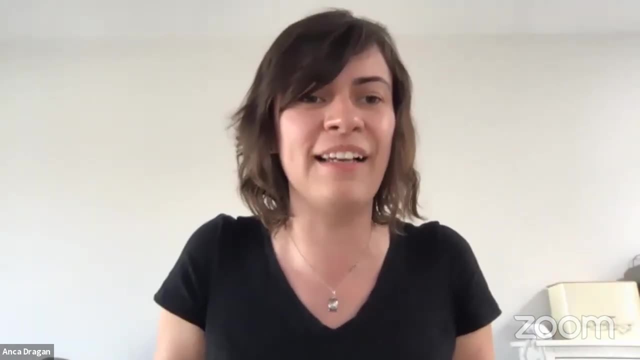 planning or you know whatever. however you set up, you know ILQR, it's the car figures out what to do. You're not really providing it rules. Rules would be saying at this intersection: stop in this way and here, do this and here. 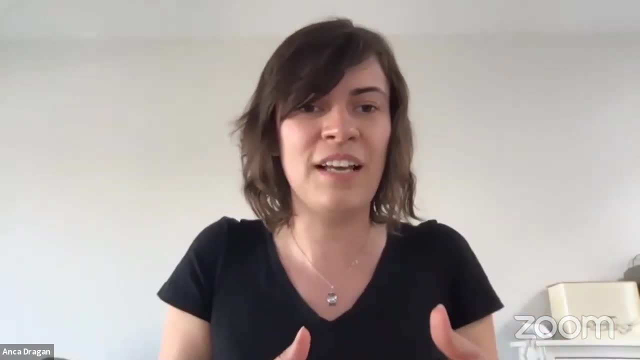 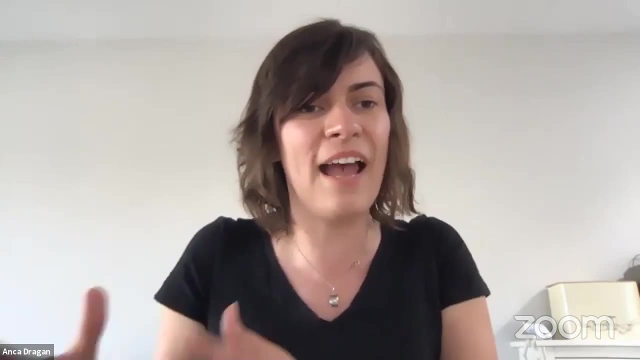 do that. So I want to very much differentiate between approaches that are based on either search or optimization And approaches that are based on rules, because we tried rules back in the day and it didn't go very well, because, of course, rules aren't very scalable, right. 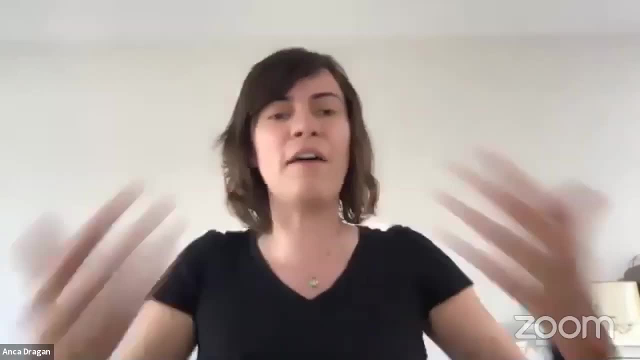 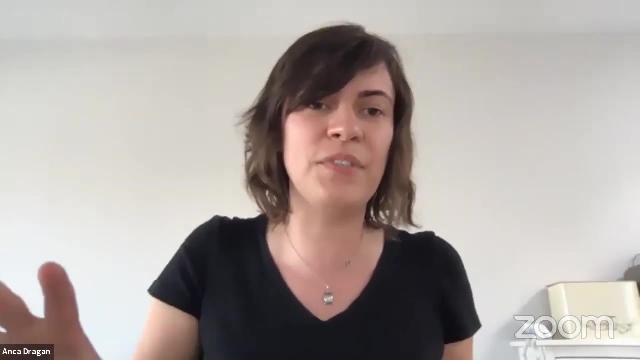 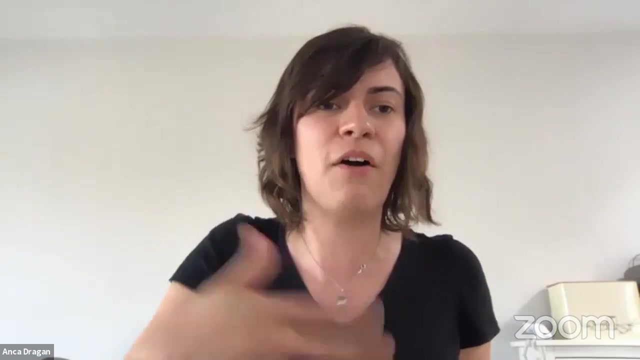 If you export. systems are all about rules. So I think we oftentimes say that you know traditional stack or rule-based approaches, But I wanted to say you know when you run MCTS right And when you run ILQR, all of those have one thing in common, which is the car is figuring. 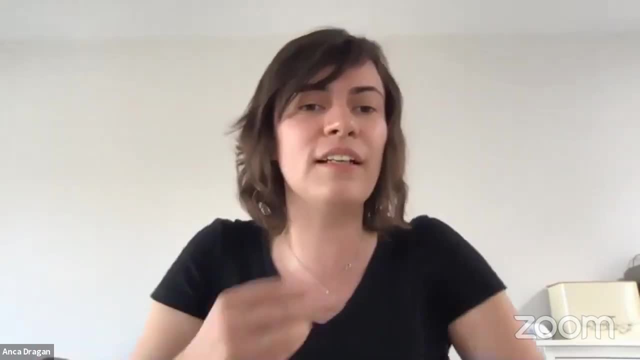 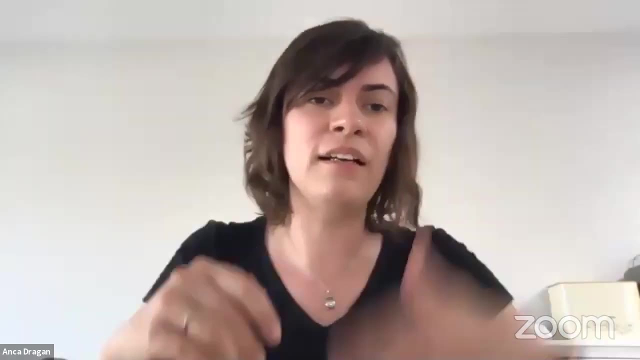 out what to do, And so I think So I wanted to draw that distinction too. So now, kind of going back to Doris's original question, I'm not sure that it's really like I wouldn't trust an end-to-end system to make high-level decision. 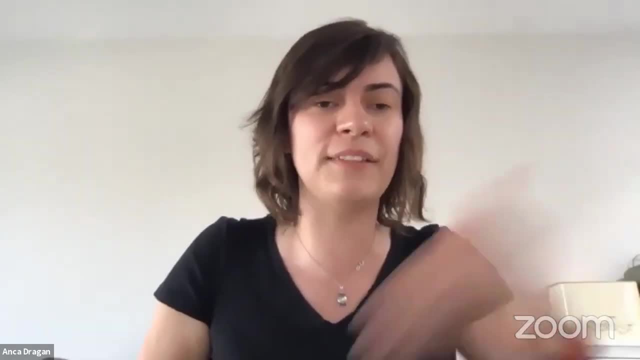 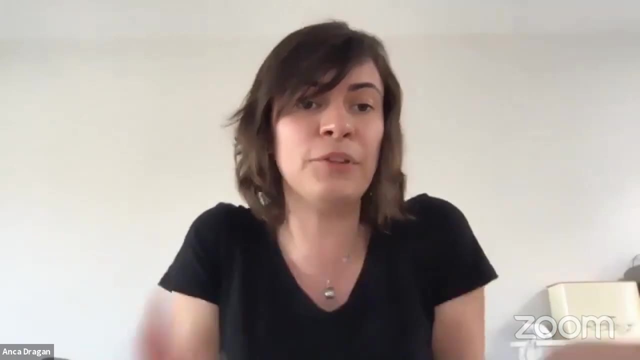 And I don't necessarily know what that means, because if it's end-to-end, then presumably it shouldn't. It shouldn't make the whole decision, But I wouldn't trust it to make high-level decisions about how to interact with people. I would. 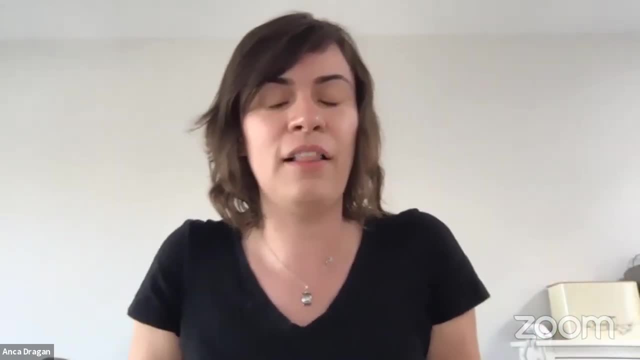 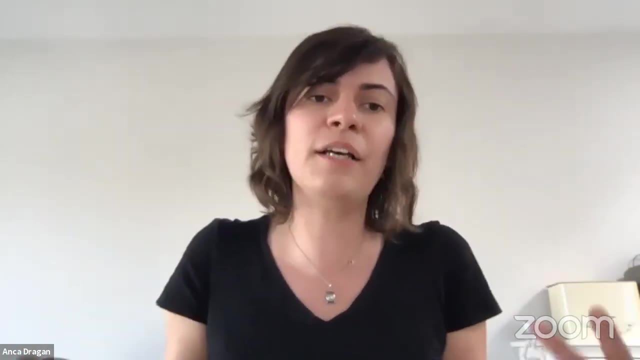 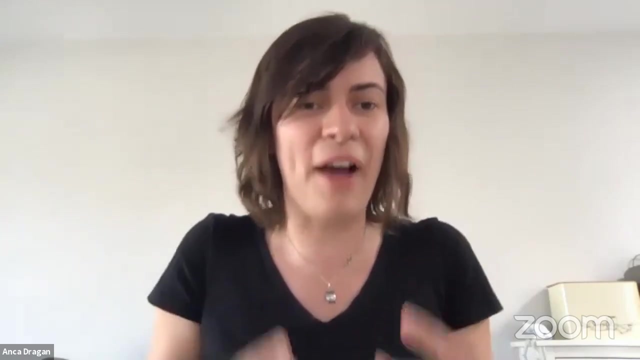 And similarly, I don't necessarily think that, Like a planning-based approach or a control-based approach, is the best one for the low level necessarily all the time. I mean, maybe the way I think about it is: how can you use the data in the best way, right? 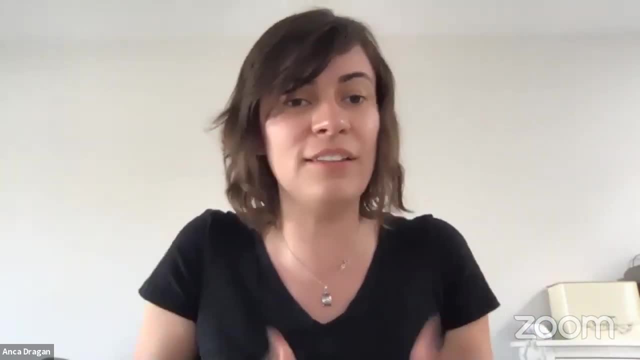 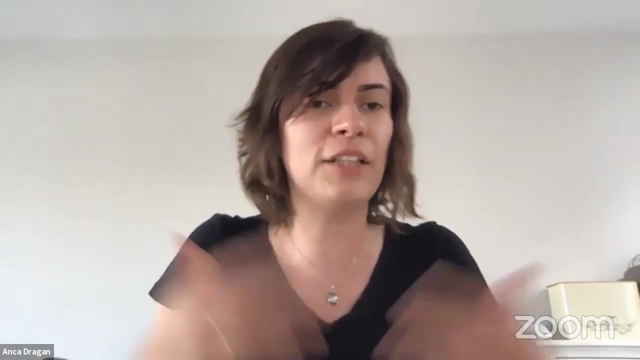 And one approach might be to trust these systems when they're in distribution and then rely on other methods when they're out of distribution. when you're worried about how this thing is going to generalize, That's one way to kind of slice and dice it. 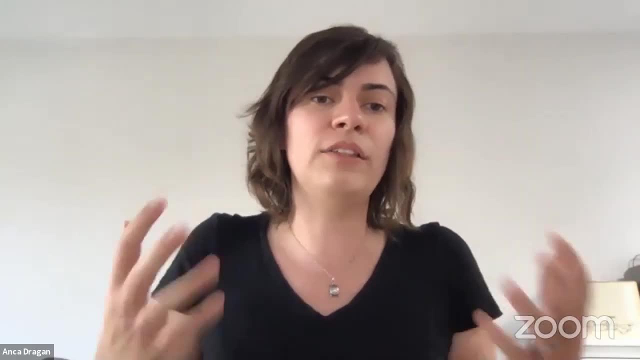 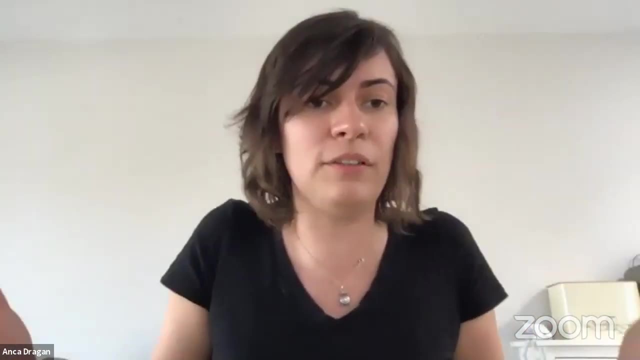 Maybe another way to slice and dice it Is to say: I'm going to learn a value function, right, And so that's going to be. so. I'm going to do whatever I'm going to do to learn a value function and that's maybe going to drive me, but I'm going to online do until some. 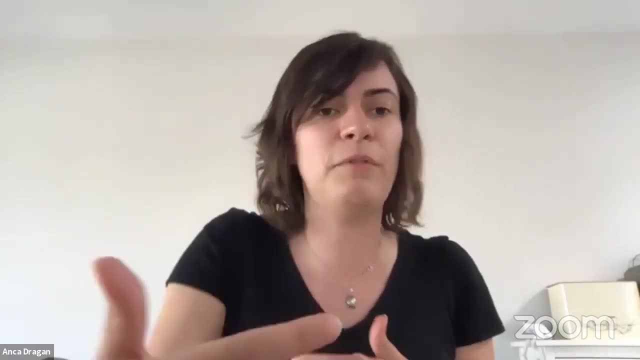 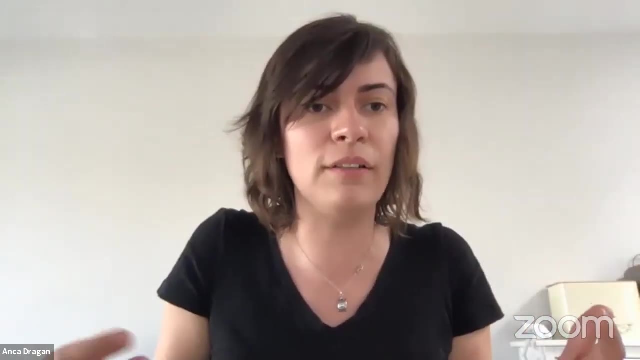 horizon, do some form of search, some form of planning, some form of optimization so that locally I can make safe decisions and so on, which is like the AlphaGo approach, right? So I think that there's a lot of space where you can marry. 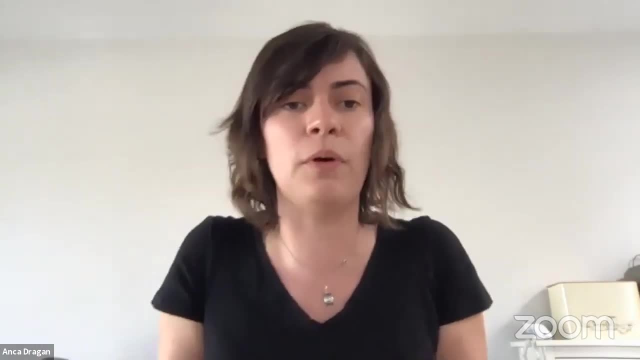 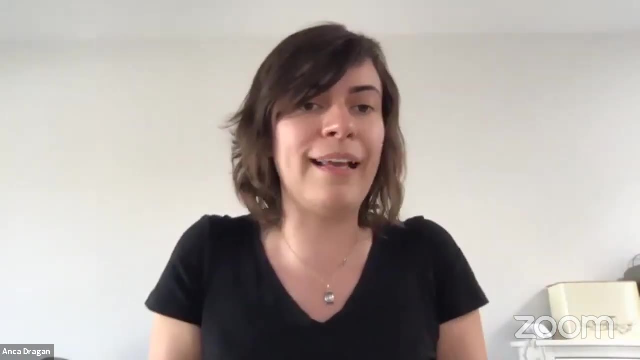 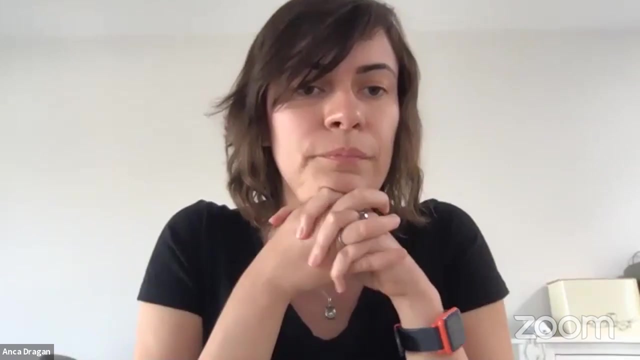 Data-driven approaches, where the data comes from practice or it comes from imitation, from seeing human, human data and marry them with approaches that are either search or or control or whatever. your method of choice is. Yeah, and I also want to clarify: the kind of end-to-end approach is not excluding all. 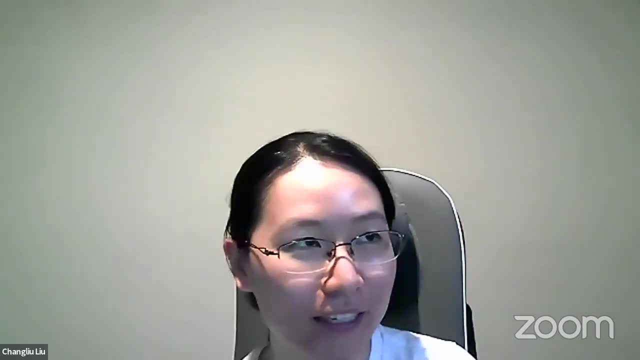 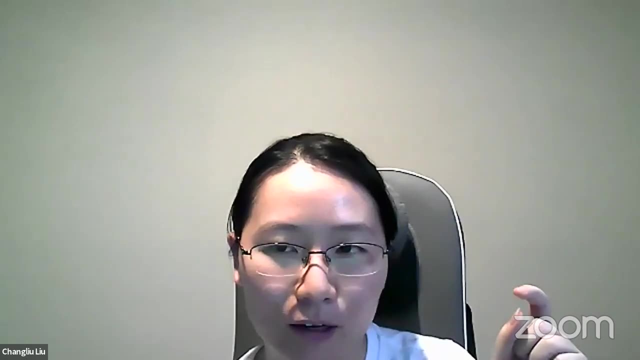 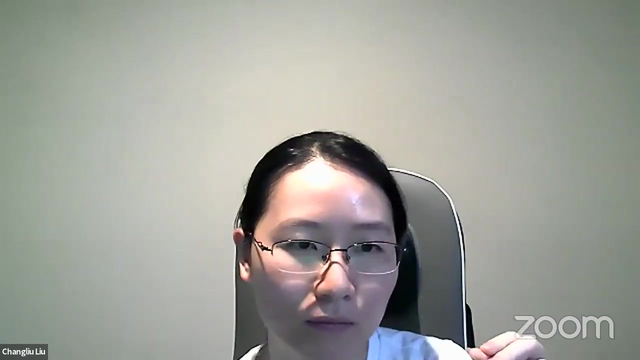 the kind of search and data or like kind of structure within it. The kind of End-to-end approach I was mentioning is that we cannot understand what is going on there and that we can- it's not easy to trickle the parts- or debug ability- trickle the parts. 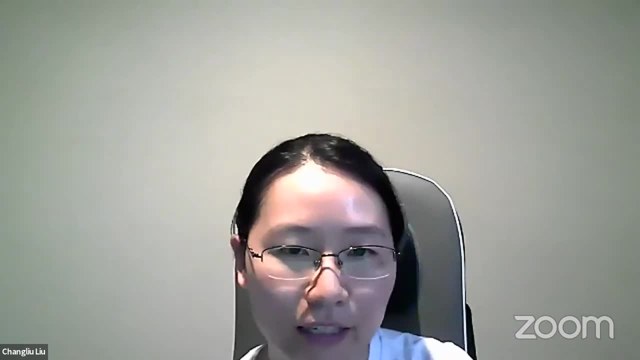 to better fit our data And in this way. that is not a desired approach, but if we can build more and more structures inside it, like combining with search and modeling based LQR, LQR stuff, that's definitely a good approach. 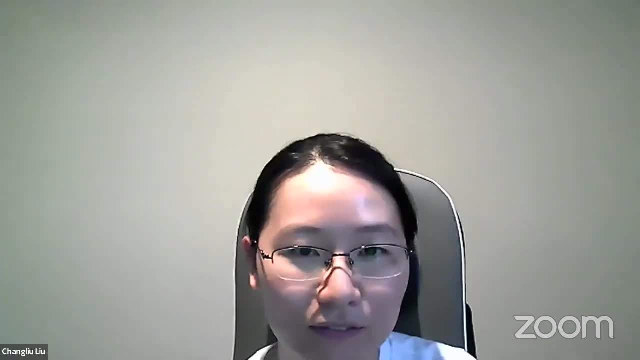 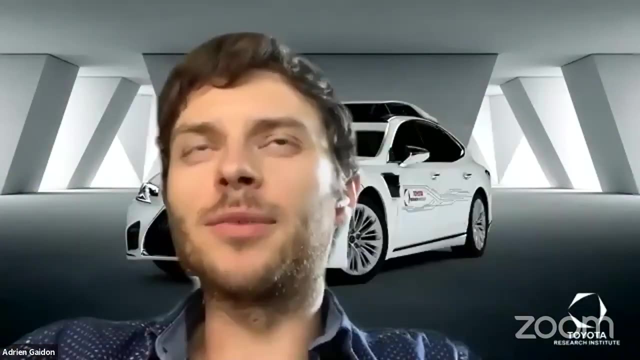 And I think that's why it's so exciting, because there's a lot of really cool work on. a lot of it is optimization right. When we do these kind of like two separate things and you can back, prop through, a lot of things actually turns out right. 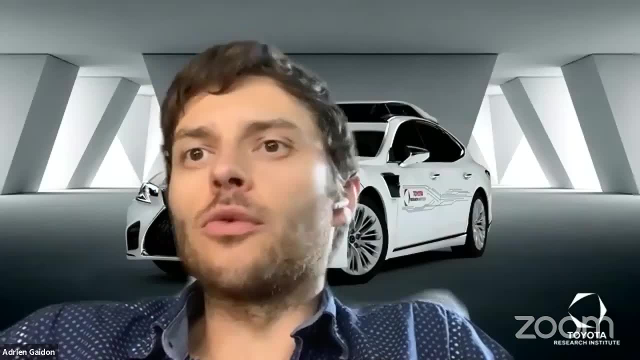 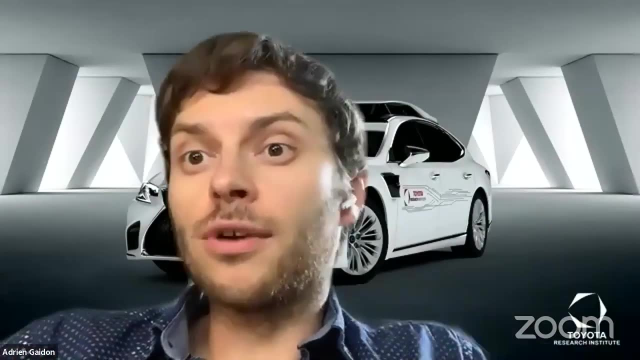 And so grading, grading based optimization is the is is the workhorse. So if you are doing an optimization, an algorithm, it's an optimization based algorithm. turns out like you can differentiate through MPC, right, And so you can. I really like this notion. 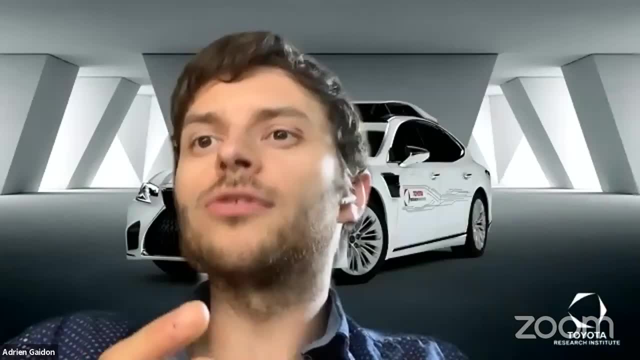 I really like this notion of structure. right, You can start to have an end to end, but modular approach where every you, you, you, you engineer, you engineer what you know right And you learn what you don't. 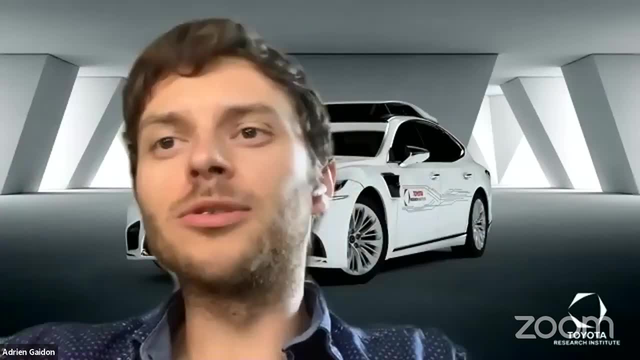 This is a quote stolen from Stefano Soato. I don't know he maybe stole it from someone else, but I really liked that, And so you basically put the structure and then you can back prop. you want the whole system to improve with demonstrations. 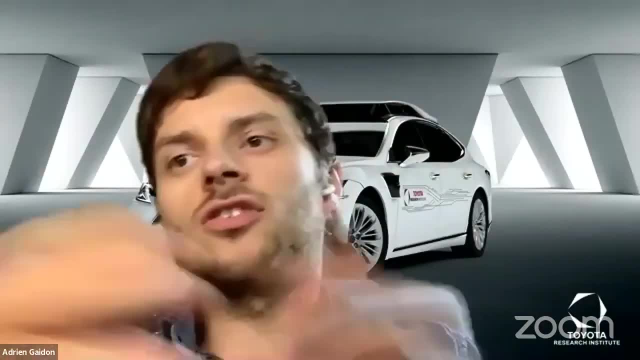 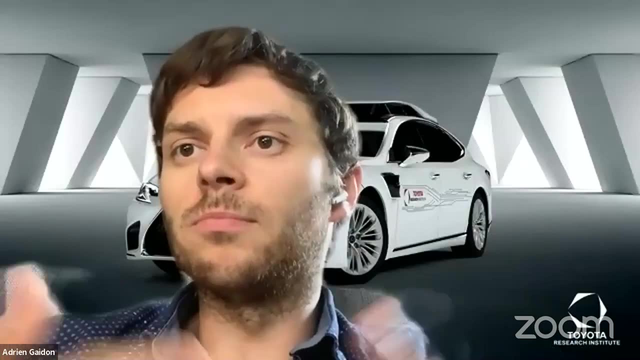 That's something that I think is really important. But but if it's just a big CNN, then you have these problems that Changvi was talking about. But it doesn't have to be now Because we have the mechanics. We basically like back, prop through crazy things, ODEs, whatever. 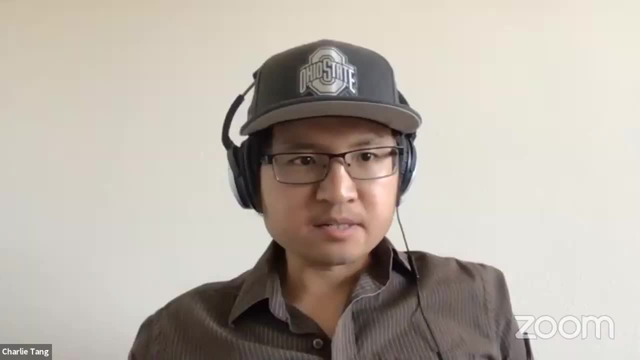 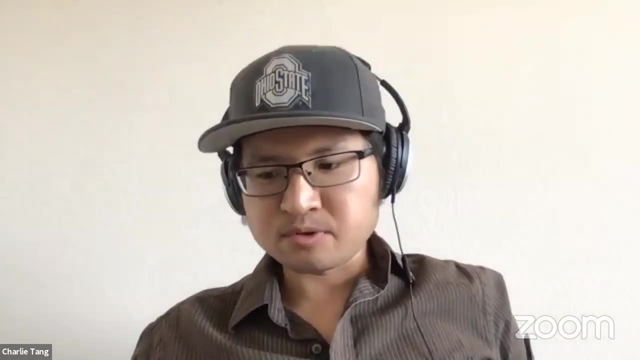 So So I'd just like to add something. I think I think everyone, most everyone in her field is. I feel like in recent years especially, we're sort of converging on this kind of the, the thing that Adrian just mentioned. 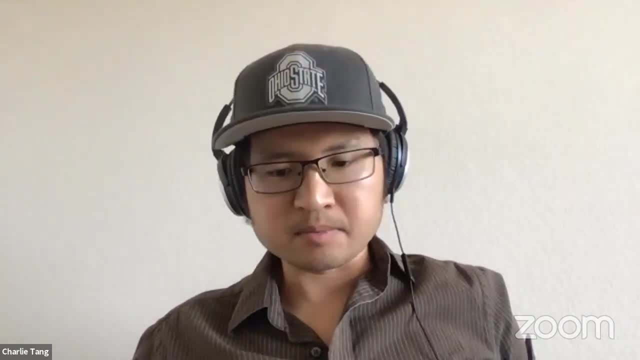 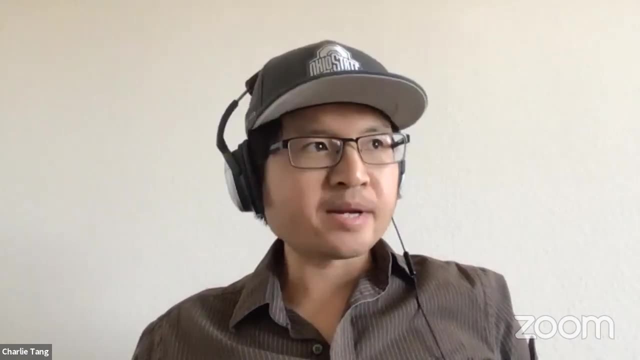 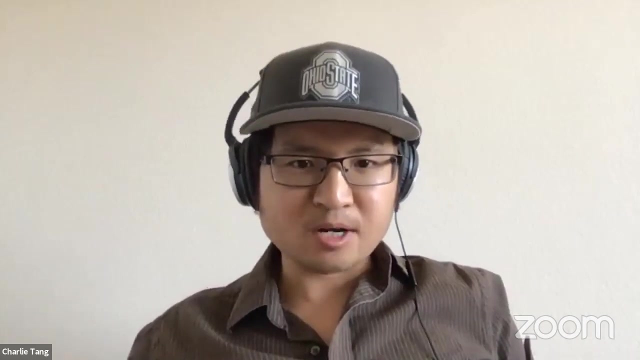 But one thing I think is missing that could be useful as a field in general as a whole is a really good metric, You know, like something like ImageNet. I feel like everyone has their own sort of way to evaluate, especially for different companies, different ways to evaluate, such as the miles per engagement or whatever. 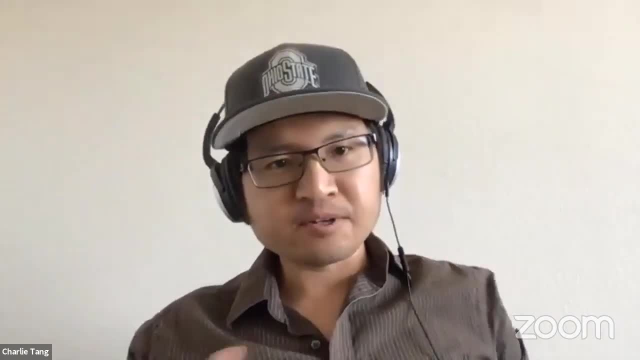 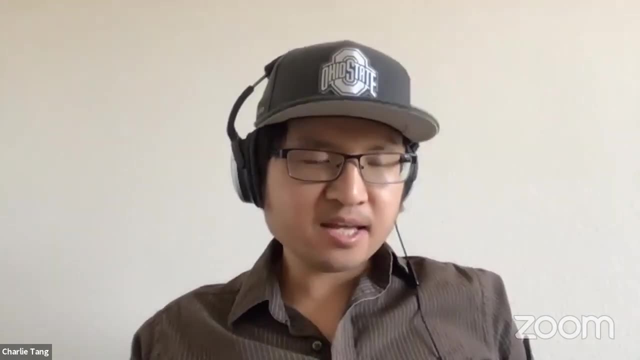 But it feels like you know, if the entire field, as a researcher, as a sort of industry, had a really good metric to really see how, while we're doing right, then you would clearly know where, where's the the gap. 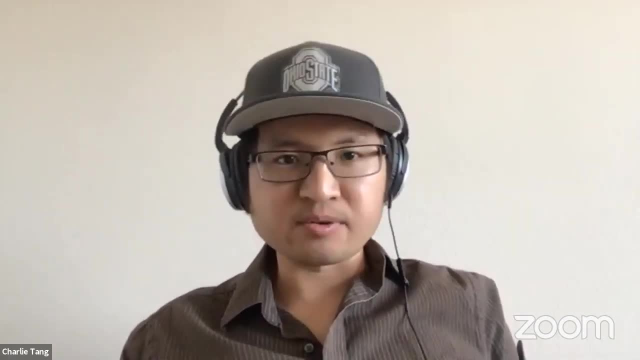 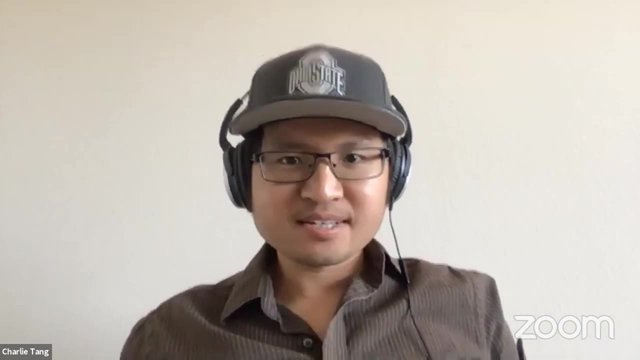 Right. So I think that could be something that's that's going to be very useful. now, Is it going to be Yeah, So I think I would say actually for for all of these types of data sets that are that are released. I think, you know, we're not necessarily, you know, that's really a 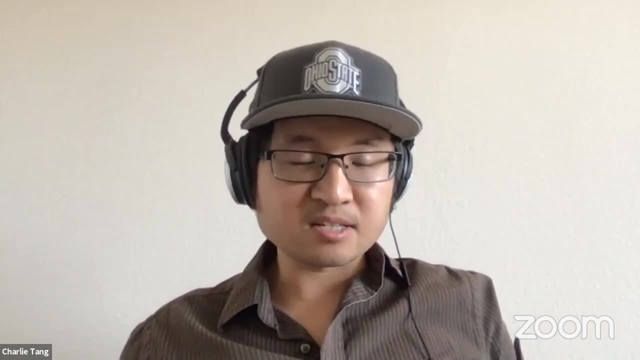 multiase community. So I think that's something that we're trying to. you know, I think a lot of us I would suggest is to you know the open source Engine and also to kind of make sure that you know you're not just sort of a local document that doesn't actually happen. 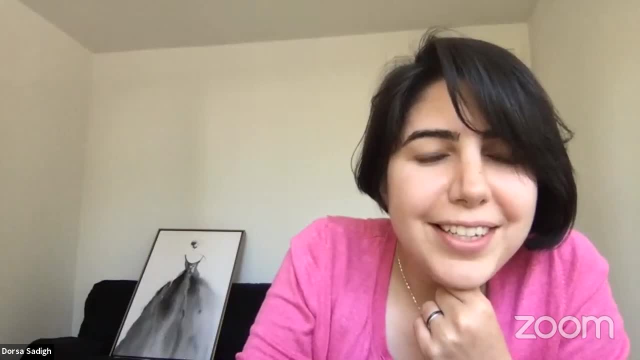 Right. I mean, a lot of these things are proprietary, But I think the latest push with the- you know the different open data sets that folks are releasing- I think that's a that that's a good trend in the right direction. 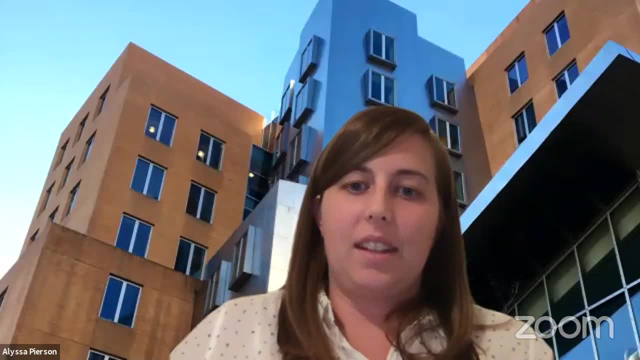 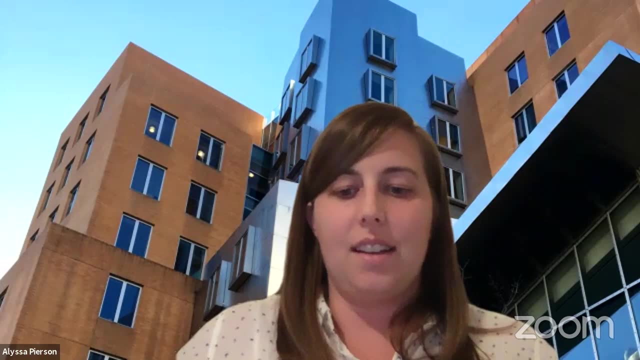 Any other thoughts? Alisa, do you have any thoughts on learning based versus? Yeah, think about with this design, or maybe something that hasn't yet been said is also: you know, we talk about the design challenges with a single robot, but for autonomous driving. 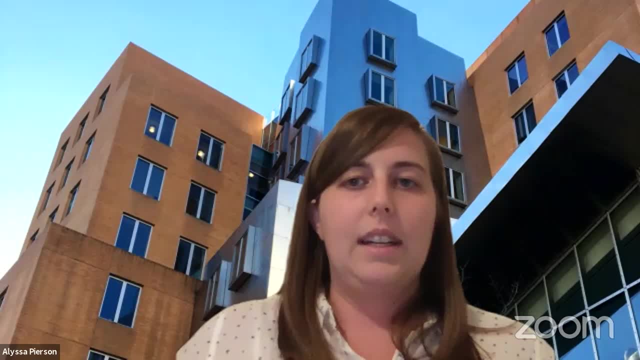 we eventually want to scale this to more than one car, And so you know, model-based planning versus data-driven. I think another important question with all of these approaches is how unique is your system to that specific vehicle or that specific environment, And so I think, whatever approach we take, we need to be cognizant of: does it transfer? 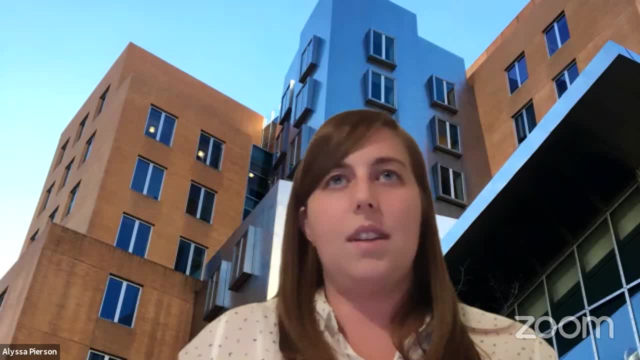 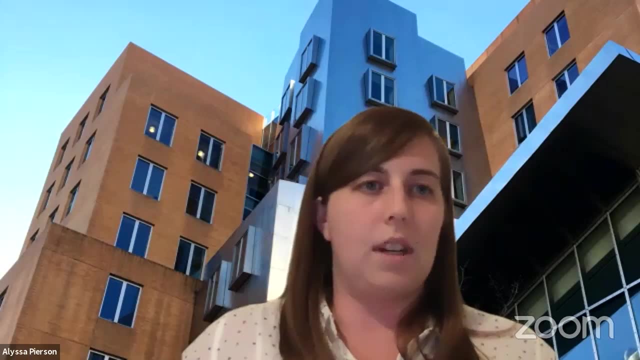 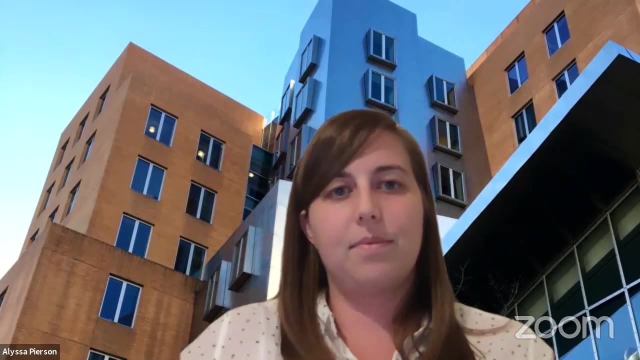 How can we transfer policies, How can we scale our learning approaches that, when we have different cars in different places, collect and combine and translate the knowledge that they have in a way that doesn't dilute or break the system, That makes a lot of sense. So, building upon that- you guys didn't mention this really. 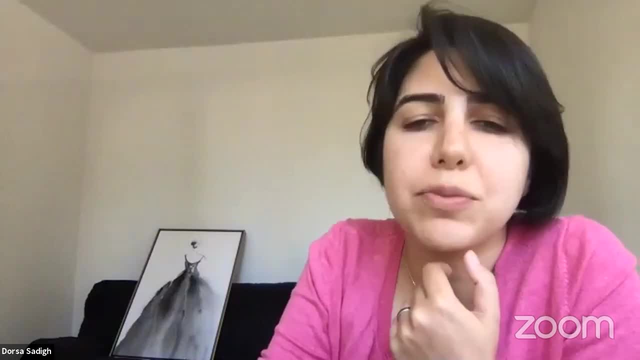 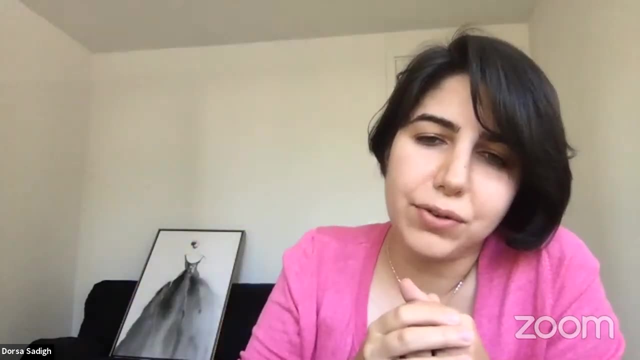 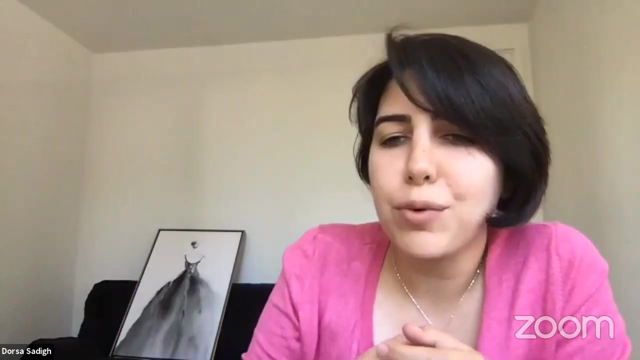 but it kind of hints at this issue of safety and explainability And there is a question from the audience and I kind of want to combine that with one of the questions that you already have. So the question from the audience is from David Connor And what he's asking is: could we get? 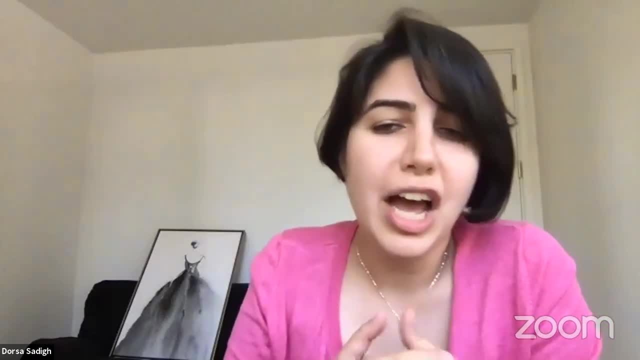 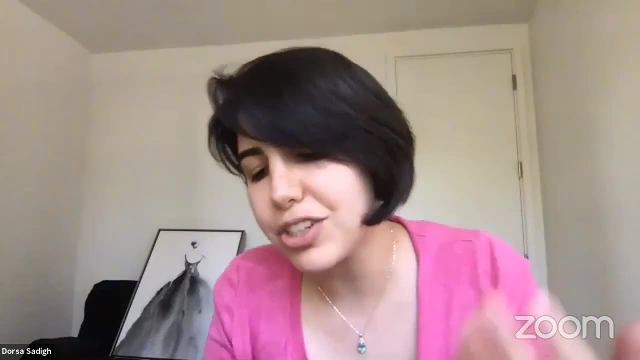 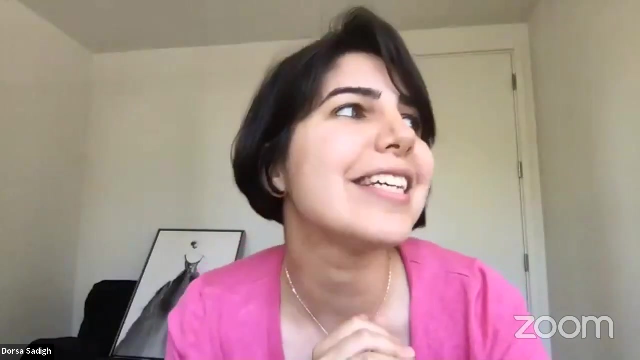 away with like not doing explanations, Like are regulators and lawyers at some point going to like basically make us come up with explanations? And I think the question that I want to add on top of it- sorry, I'm asking like too many questions- The question that I want to add on top of it is: 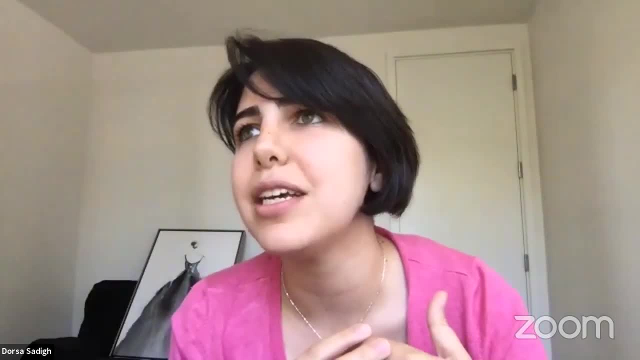 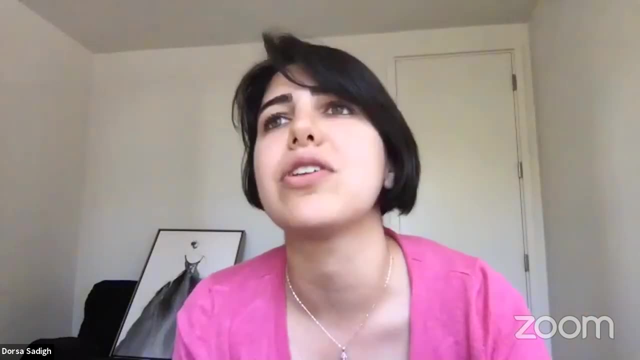 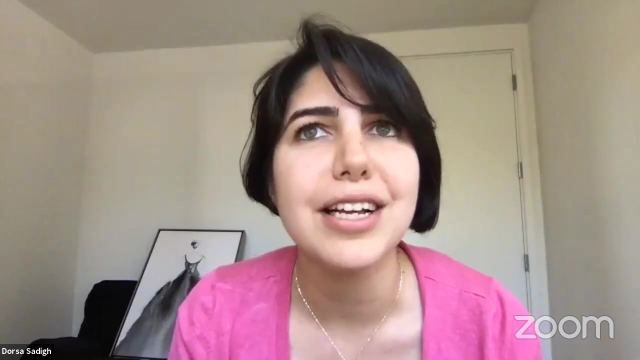 this issue of, in general, safety and explainability. I think in general there's this question of should we use learning-based systems when we are like making safety-critical decisions And kind of like? the bigger question for me is: how much should we care about safety? This is the. 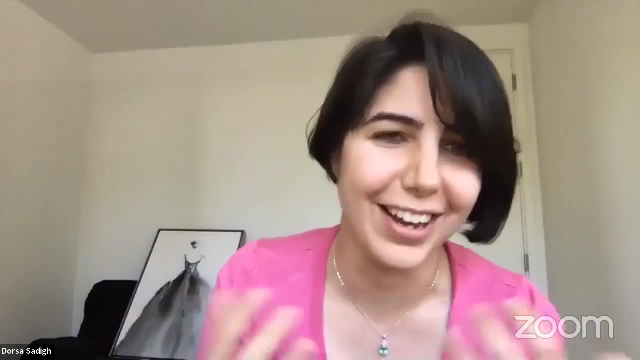 thing that I'm perhaps going to ask you. I think that's a really good question. I think that's a really good question. I'm personally wondering, like in general, when you think about autonomous driving, Like I personally started like thinking about safety very carefully and trying to like give probably correct. 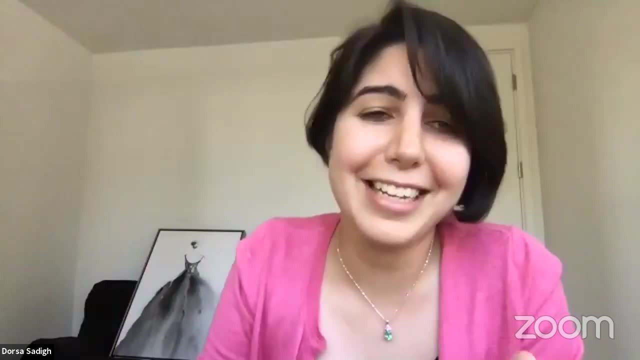 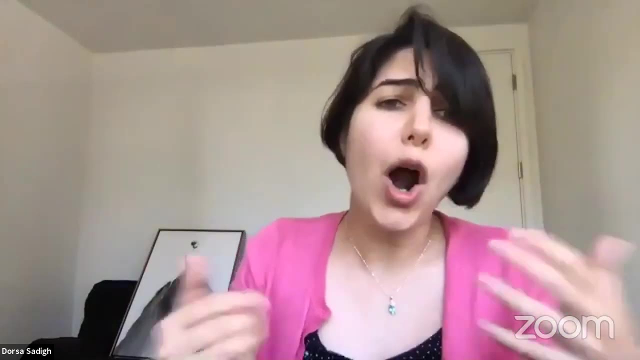 guarantees about things And over time, I'm personally thinking. I'm wondering, basically if that is the right way of going about it, Or how much should we care about safety? Or are people going to accept these systems that are that might not be explainable Or that might not be safe, Or 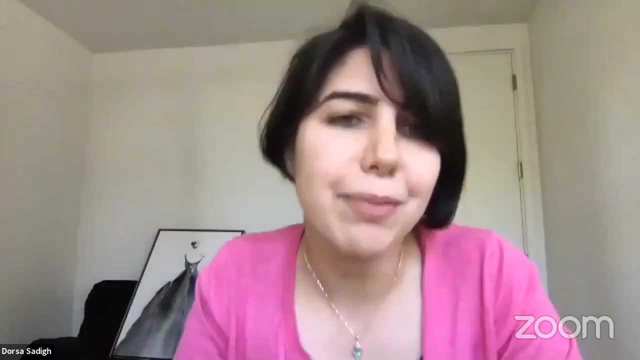 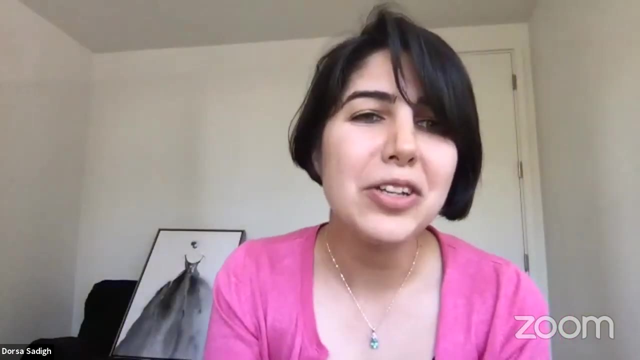 and how much? how much is that? how much does that matter? How much does that matter And how how much are regulators going to be happy with that? How much should we be happy with that as engineers? So yeah, general thoughts on safety and explainability. 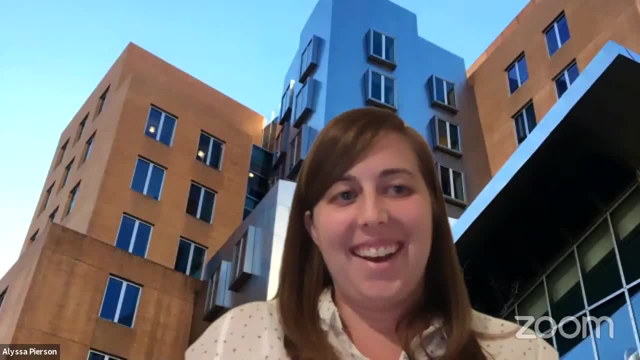 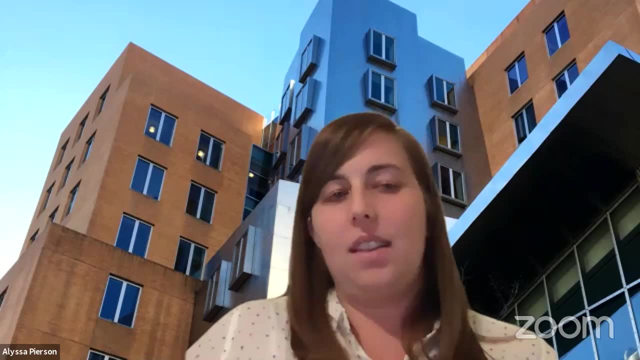 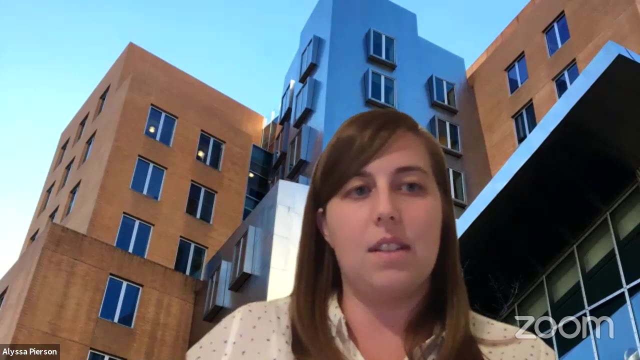 So if I can maybe jump in first. So I think this goes back to what Charlie mentioned before about metrics, where I don't think the systems necessarily need to be explainable but they need to have demonstrations that are convincing of their capabilities. 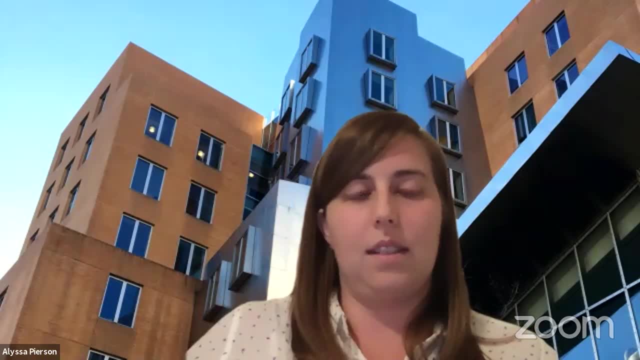 So- and I think that's analogous to right now- if you look at like airbag safety crash tests, Manufacturers don't have to explain how their airbags work, but they perform the crash tests and they get a score And if their systems pass the benchmarks that they have. 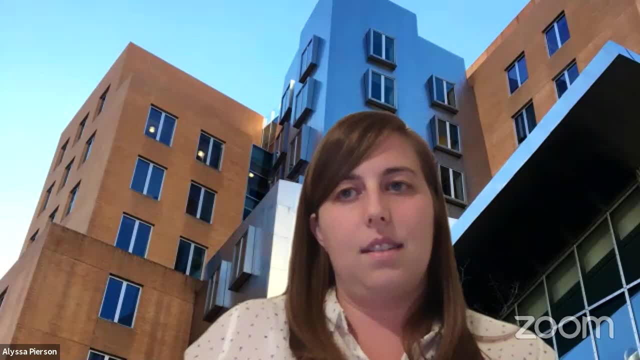 then they're considered safe. And I think that finding those scenarios and finding those benchmarks to demonstrate a safe autonomous system is a very challenging problem in and of itself, But I think that if we can define that, we won't necessarily need a full explanation. 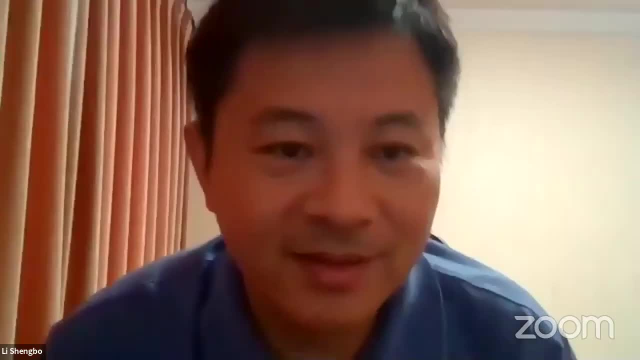 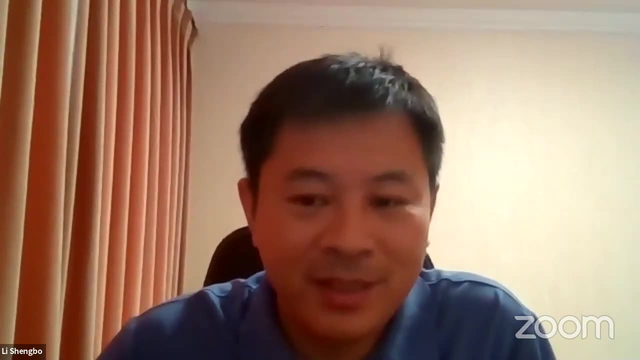 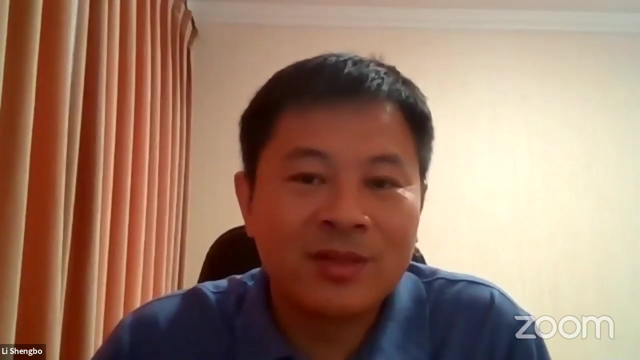 What's particularly challenging about? Can I add something? So I think you know people might have wrong understanding about you know explainability, So I guess more people want explainability. So they wanted, like we want to know, the LQ method. 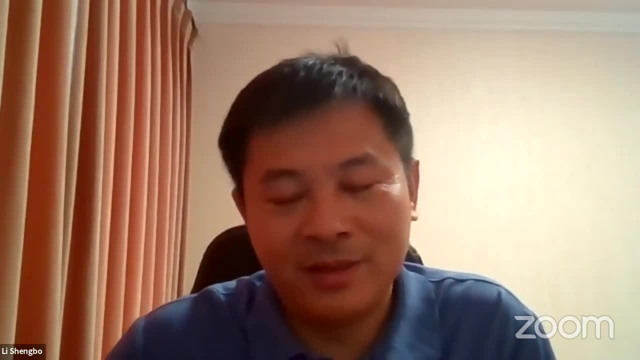 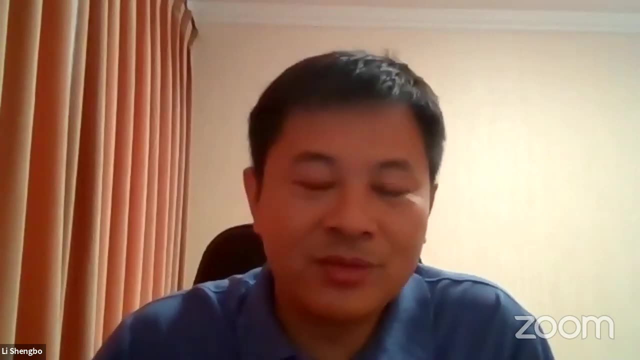 we want to explain how it works, how the So what is the mechanism behind? you know each method, But this is actually not, I think, reasonable or accessible for autonomous vehicles. So let's look at. you know the human brain, So do you think we can explain how a human 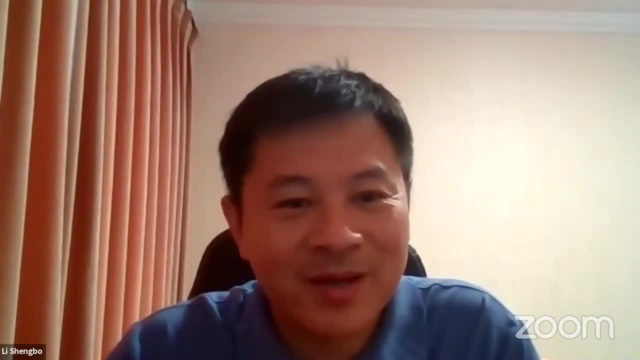 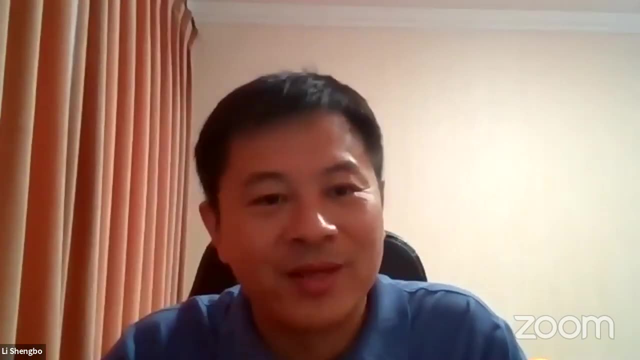 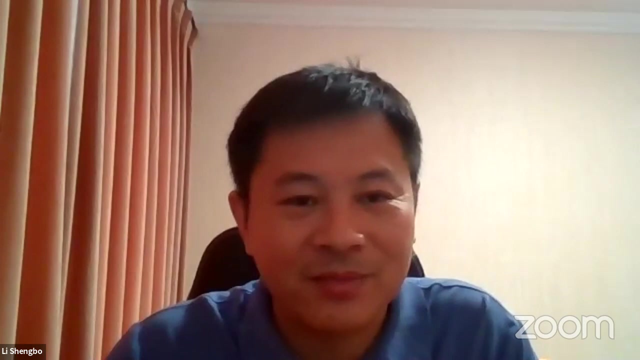 driver drive a car. So actually we cannot explain it right, Because, you know, our Neural network is too complex. We have almost 80 billion neurons in our brain, And how does it work And what is its driving behavior Or what is driving mechanism? We cannot explain it, But. 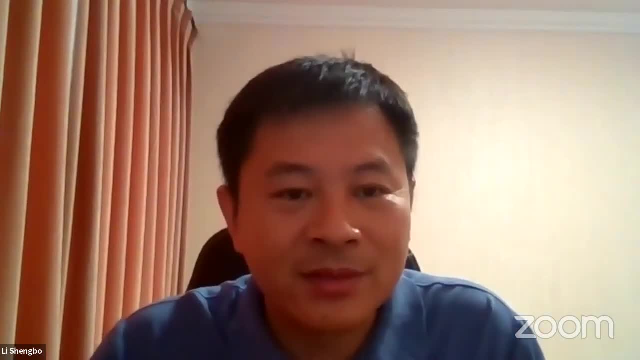 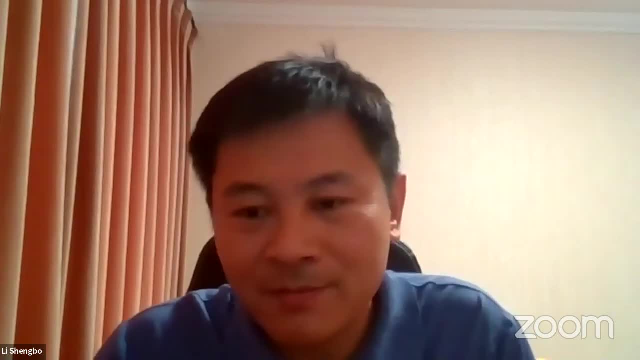 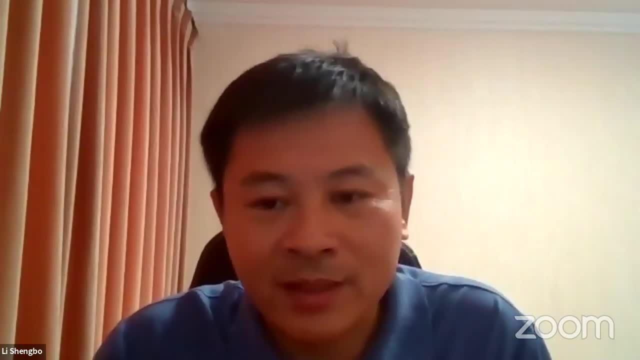 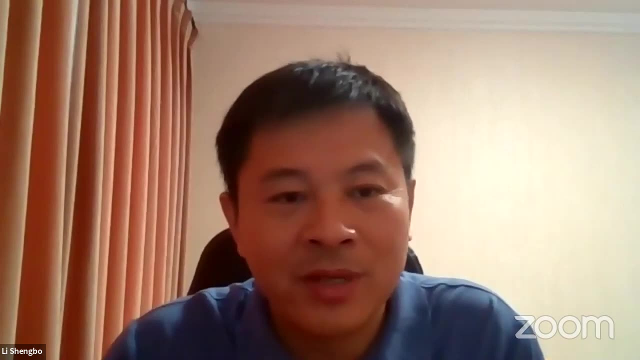 if you look at autonomous vehicle or autonomous driving technology, it's far from the human behavior you know: safety level. So, as a human, our average collision rate is about 1 billion driving miles around vehicle. I remember it's 20. 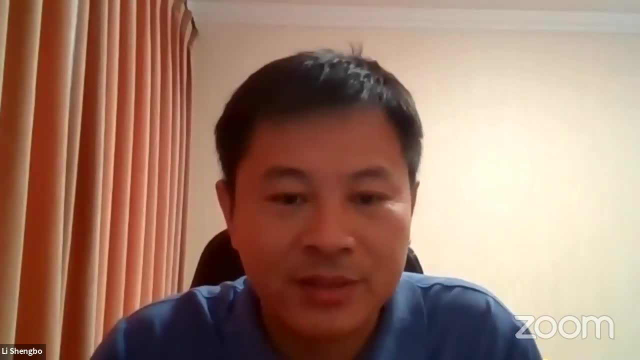 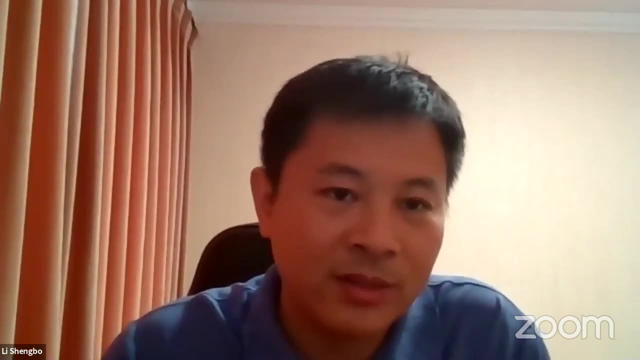 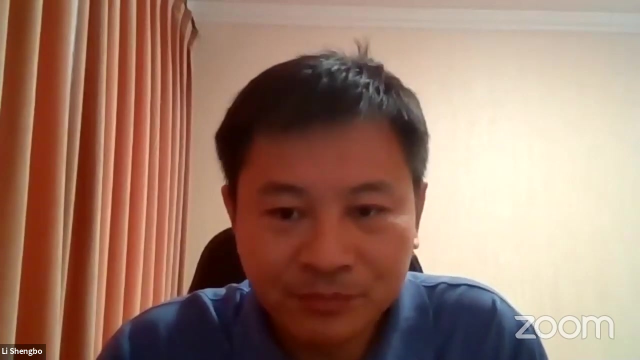 or it's 200 or 500 collisions. But if you look at you know the DMV data from California, where I see the best autonomous vehicle now in technology in today's market still has a far low safety level than human driver. So which means we need to increase the reliability of 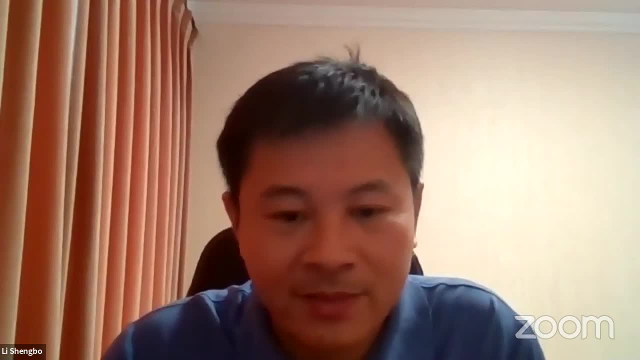 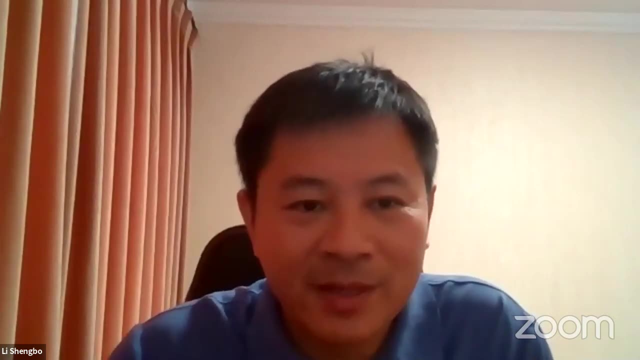 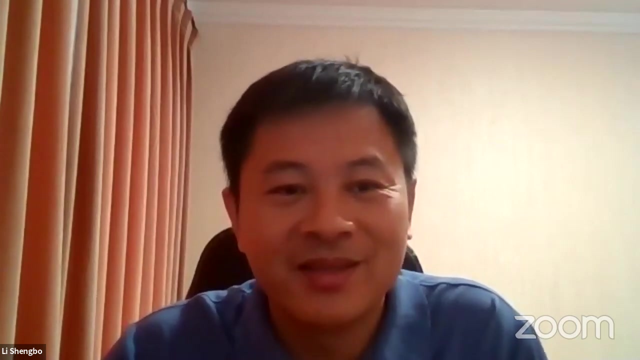 all different layers of technology, including environmental perception, decision making and also the motion control. So a short conclusion. So I believe explainability is a fake question. So if we can solve the issue of the safety, explainable becomes vanishing. So this is my comments about this question. 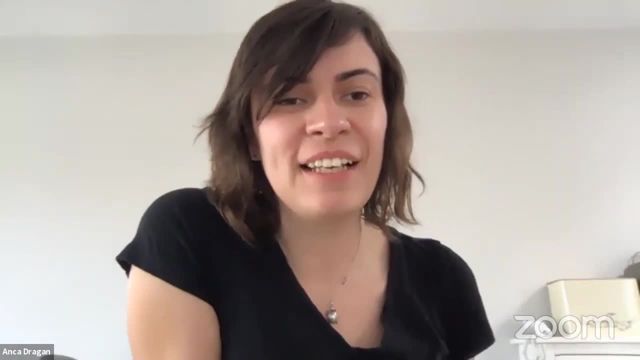 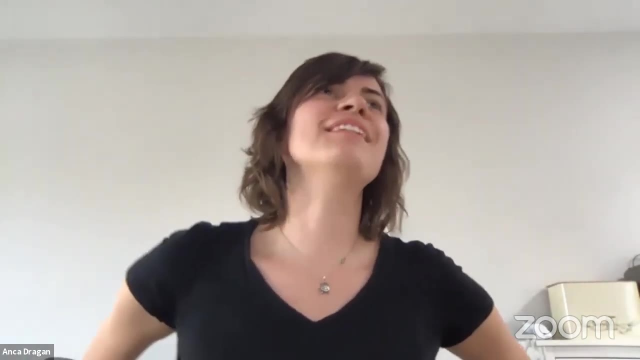 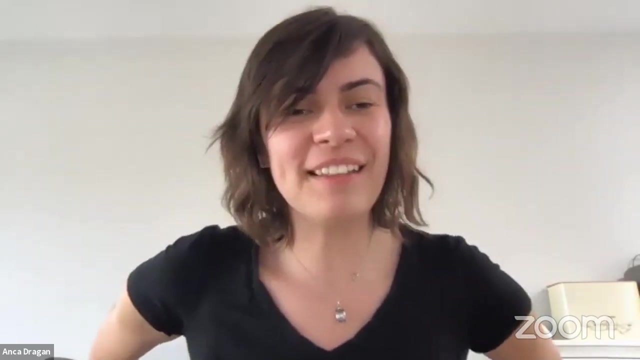 I think explainability is a kind of a red herring, because, especially as it relates to safety, right, Um, because you, you don't. so what? so there's a, there's a. it's not that we think that planners. 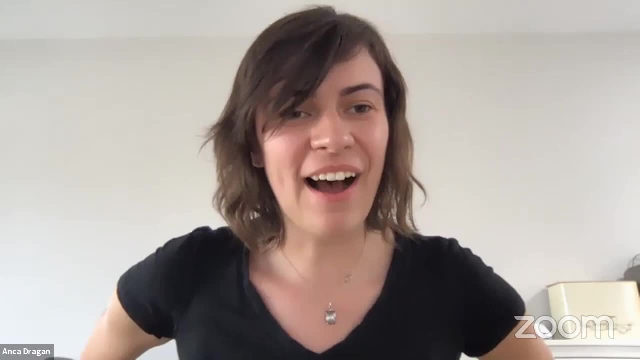 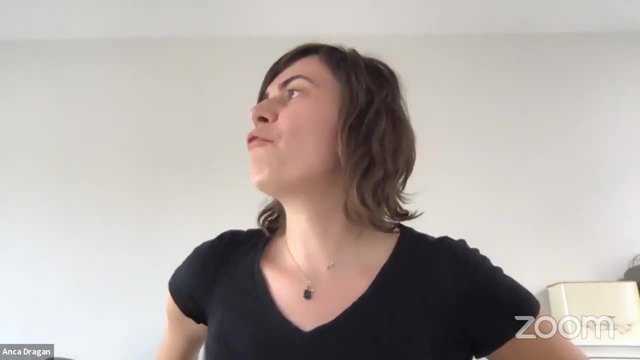 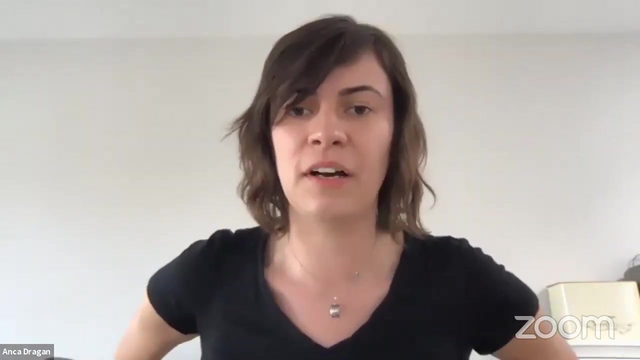 are safe because we can't explain them. Um, it's, it's. we think that planners are safe because if we test them in, you know a million scenarios and they work well, they pass those metrics that Charlie was talking about. Um, so it's not that we think that planners are safe. 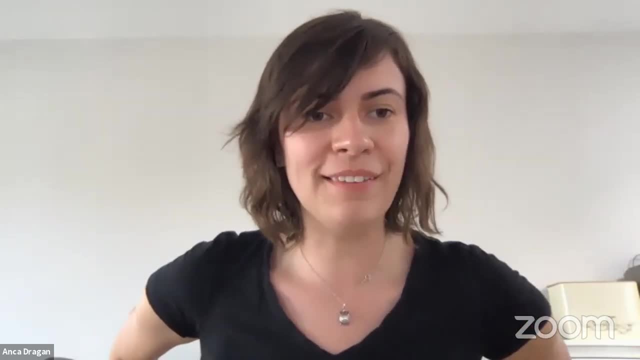 because we can't explain them. Um. so it's not that we think that planners are safe because we can't explain them. Um, so it's not. that we think that planners are safe, then that gives us confidence that they work in other settings And that I think. 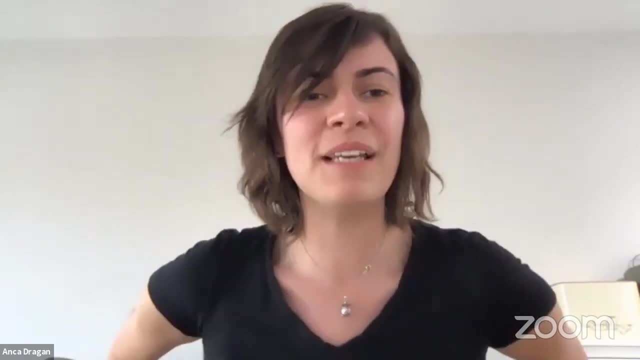 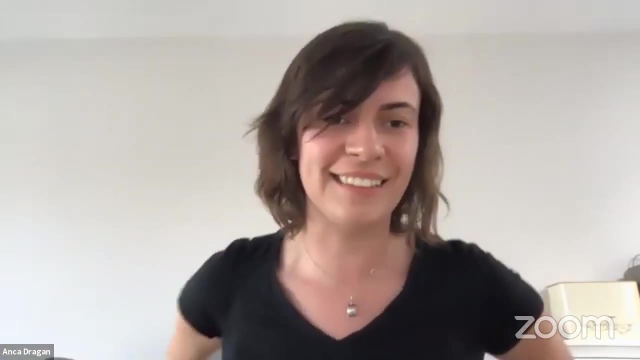 that's the challenge with establishing these metrics is that you know they're gonna be, they're gonna be tools that can do very well on those metrics, but you can't trust them to actually do well outside of that. Dersa, sorry, go ahead. 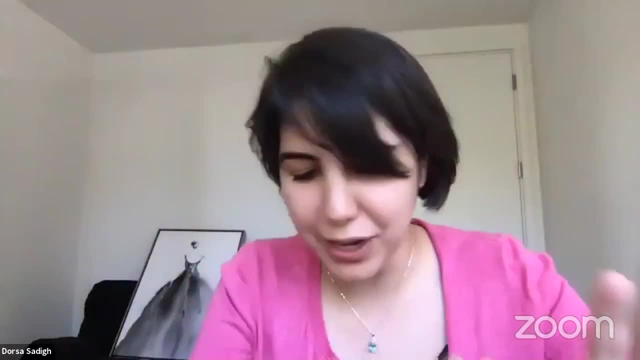 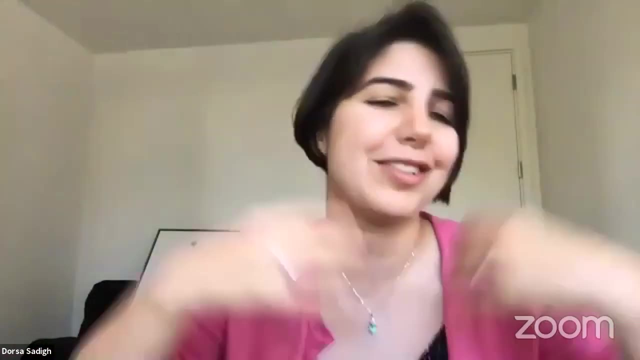 I was gonna clarify And so so I was basically: yeah, so I completely agree with that. But think of it as two questions, I think like putting and piggybacking on the on the audience questions. One is about explainability: can you get away with that? And 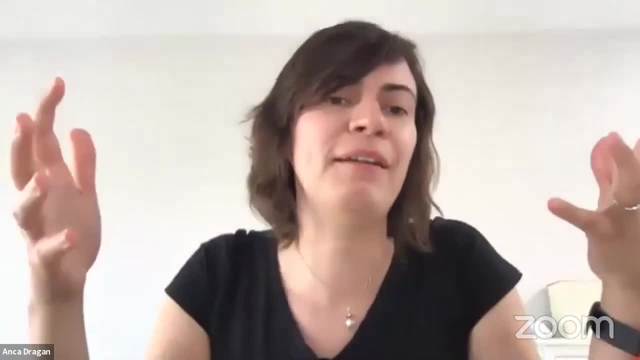 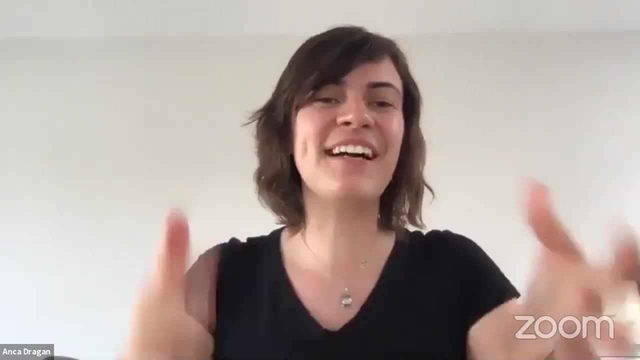 then the other question is: like just purely about safety, Like do we care about safety? Why? why? Yeah, why should we care about safety? And this is I mean. I feel like, whatever your car does, it will have to be using data, It will have to be based on at the very you know, if you want. 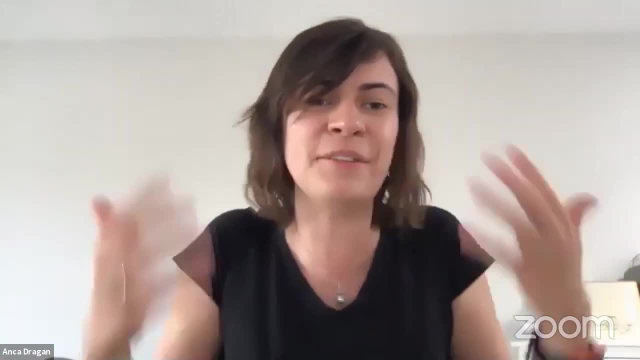 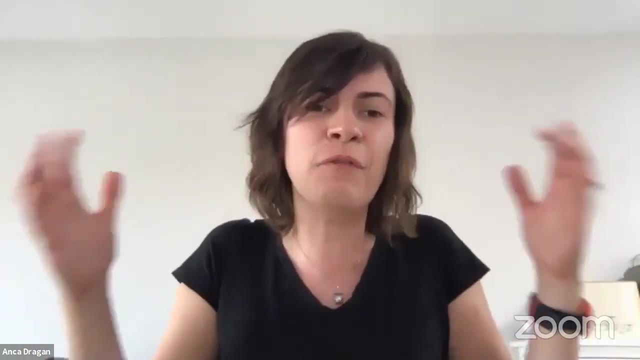 to use just pure planning. you're going to need a model of human behavior And let me tell you, you're not going to write down that model in equations from scratch and go to town right. You have to involve data for any, for for us to even imagine that the system will. 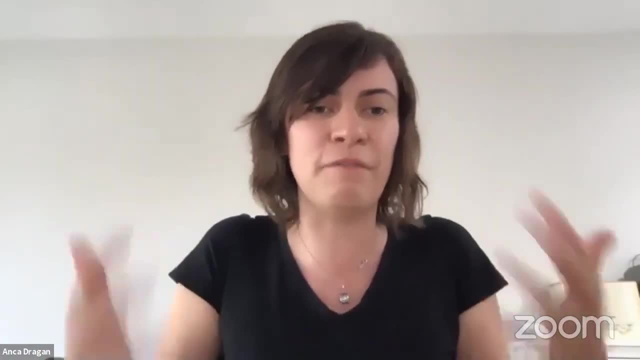 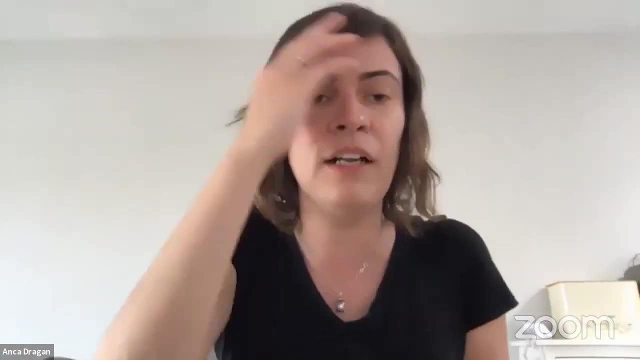 be anywhere close to successful? right, You're going to involve data to, at the very least, model the world and then maybe leverage that model through planning or through learning or to whatever. So when we talk about safety, whatever guarantees we think we have, they're under. 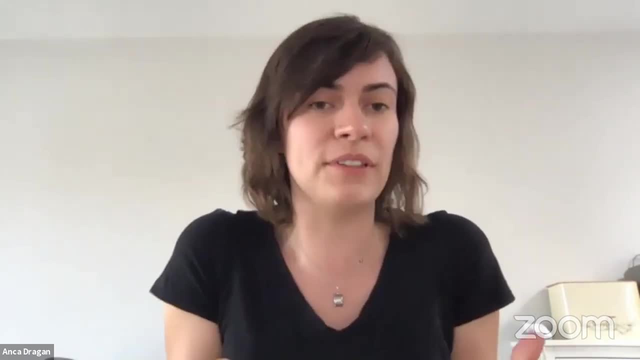 whatever assumptions our model is making, But those assumptions are wrong. And so you know, if you want real safety, then you'd protect against the adversarial environment, as control theorists do, but then cars never leave the car. So you know, if you want real safety, then you'd protect. 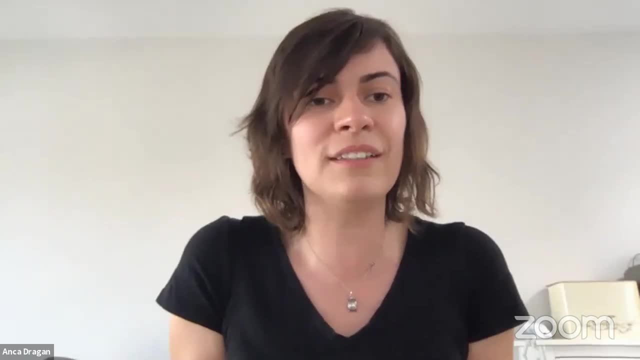 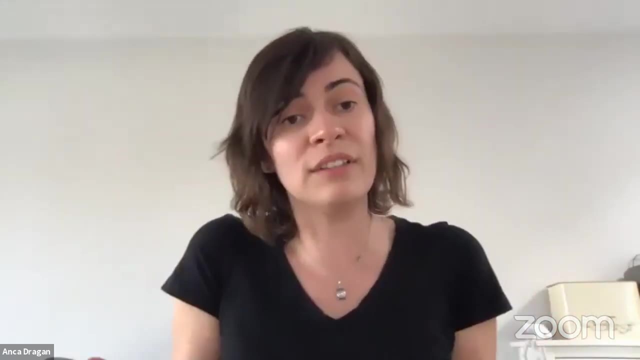 against the adversarial environment, as control theorists do, but then cars never leave the car. So the moment you step out into the real world, anything that you're saying about safety is under assumptions that you know which, and it's very useful, I think. 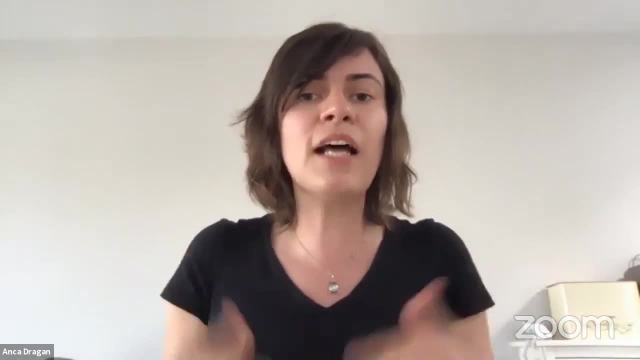 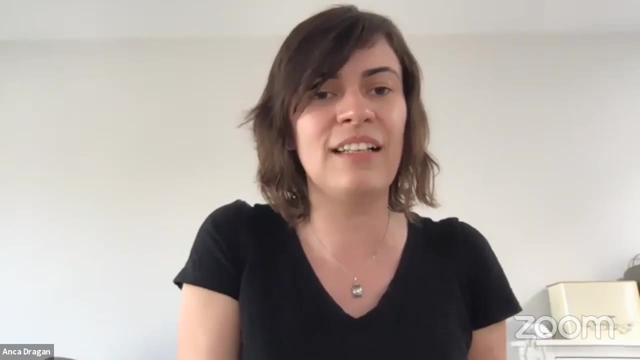 to be able to clarify these assumptions. But let's not mistake those assumptions for reality. Let's not mistake the fact that we have safety guarantees under these assumptions that you know our cars are going to, that we have those guarantees. for the real world, right, They're only going to. 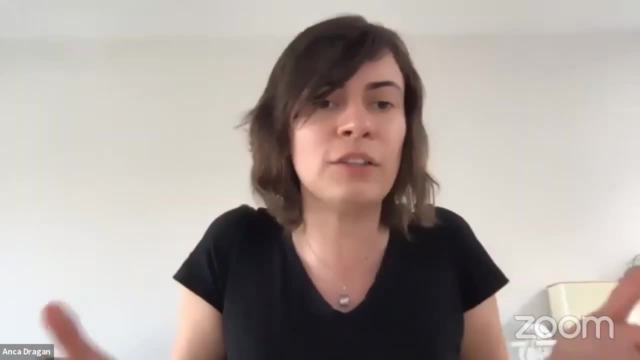 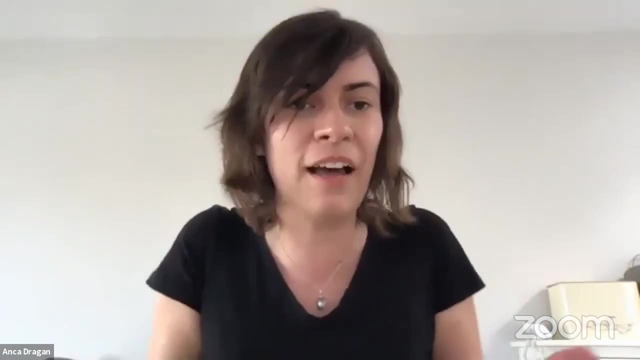 be as good as the assumptions are, And so I think, just because you know I was talking about people, I agree with Adrian that it's when I say people, I don't just mean prediction, I mean prediction and planning the whole enchilada all together. And I think that because they're 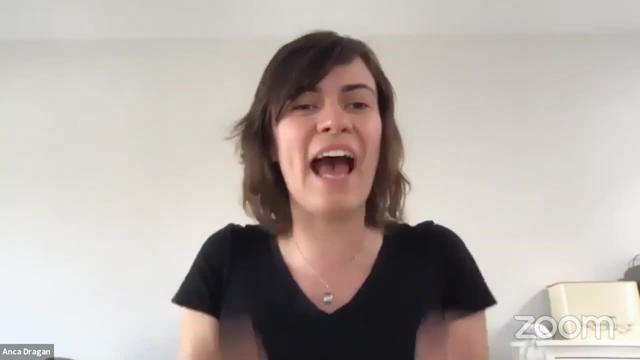 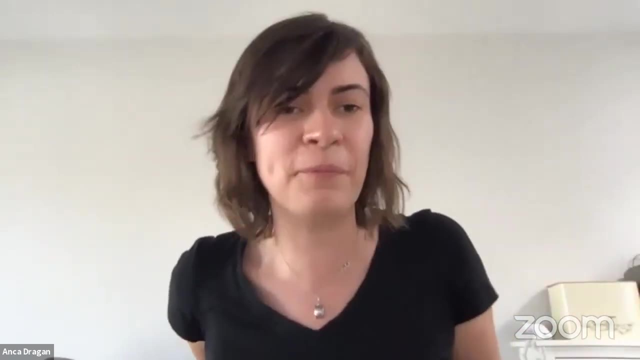 involved, and because we can't have a perfect model of them, right, that we're gonna have to. that's where the challenge comes, That's where what that's the hard part that we're dealing with, And when it comes to safety, that's that's that as well, And what worries me, just to come. 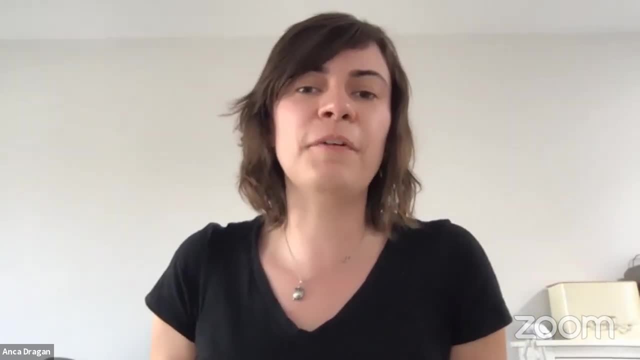 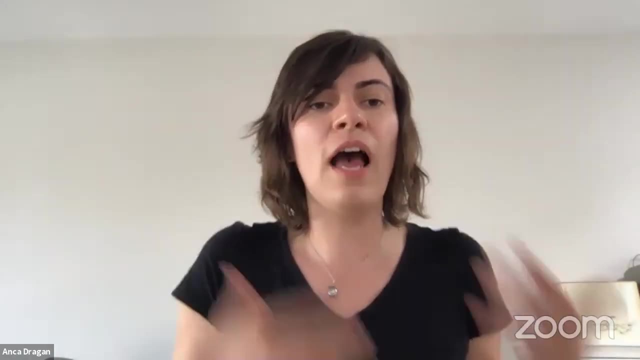 to kind of finish my previous thought, you know we heard from Melissa and from Charlie about, about developing metrics, And I think that I both think that that's useful and I also want to caution against that, Because I think that you can have, for instance, 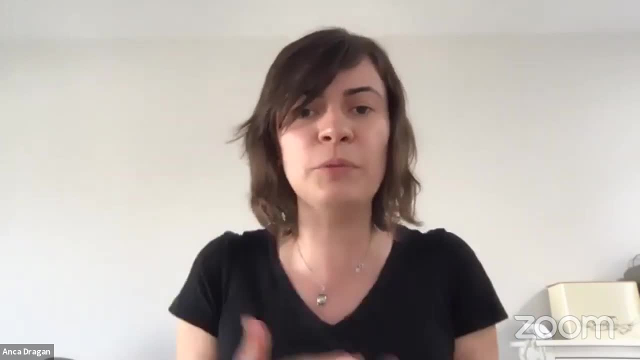 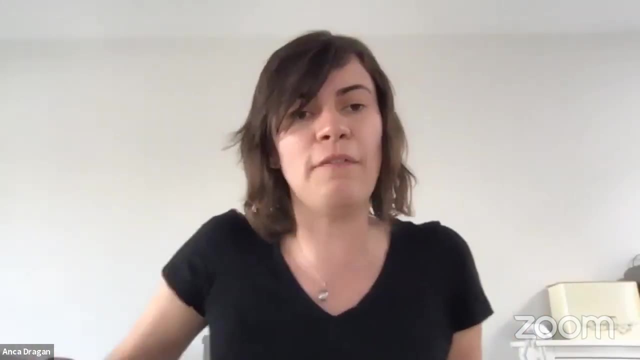 an end-to-end system can go to down to down on that and perform stupid crush that if you know about it ahead of time, right The? the worry that we have is what happens in this novel situation. that's not part of the data that you've trained on, whether it was you know. 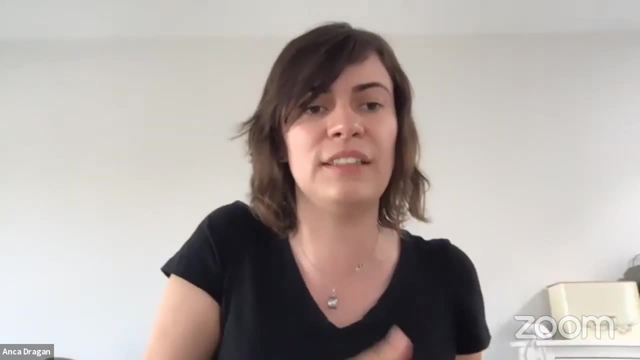 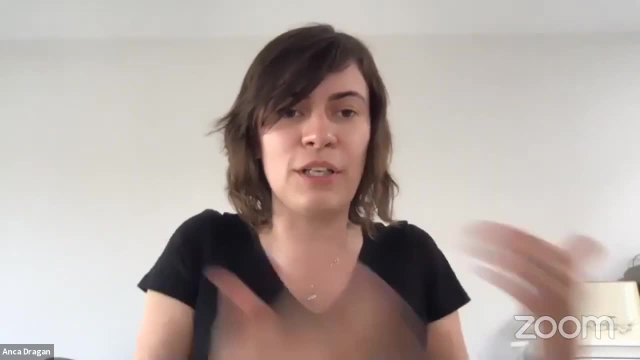 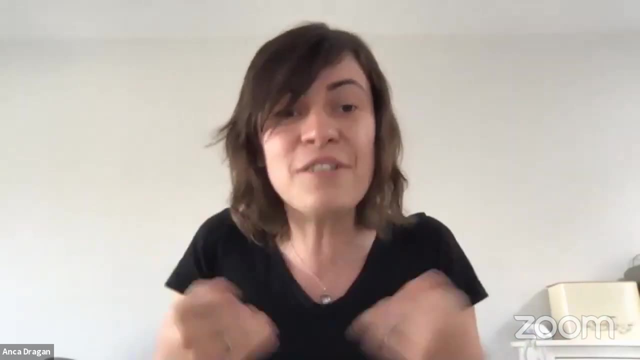 And the the challenge with that is, when I administer a driving test to a human, the fact that they detected this stop sign tells me that they'll detect stop signs in other situations. right? I cannot trust that of a learned policy that went from pixels to like steering. 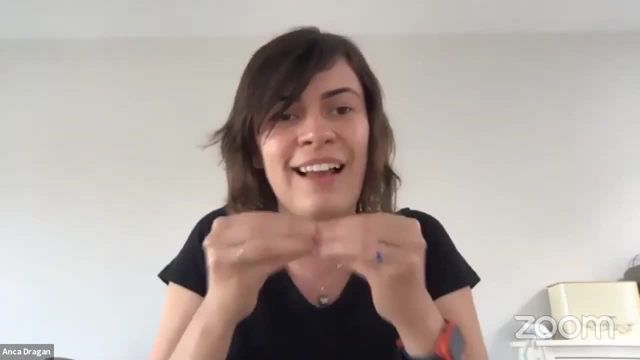 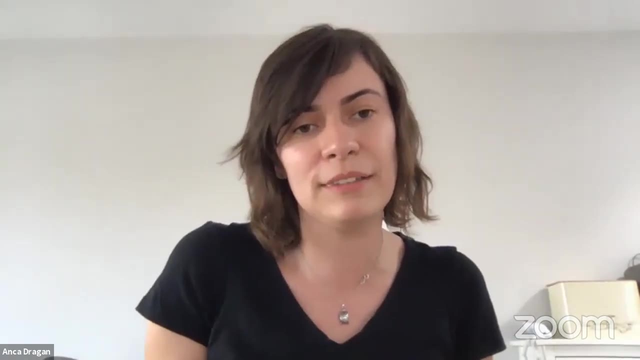 acceleration. I cannot say the same thing about that, And I think there lies the challenge of how to exactly develop these metrics in a way that we actually trust that they're representative of the actual performance of the system. Yeah, you were mentioning the question. 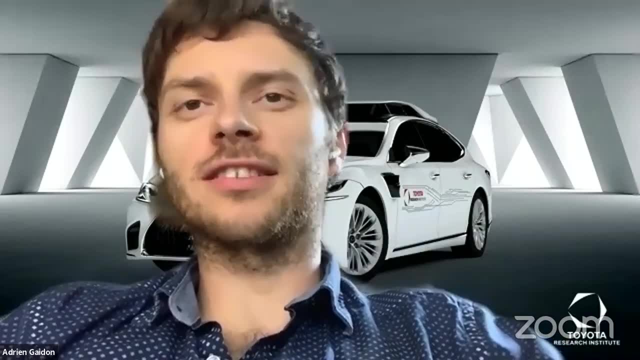 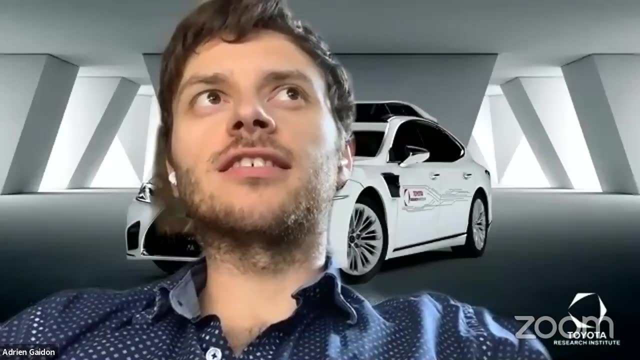 was mentioning lawyers. So beyond the technical questions there's- and I think this is kind of like the- there's kind of this dawning realization on us in machine learning these days that it's not just a technical angle to the questions, it's also the sociological questions. So I think 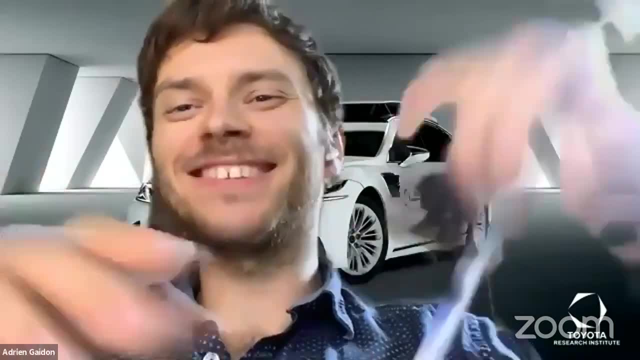 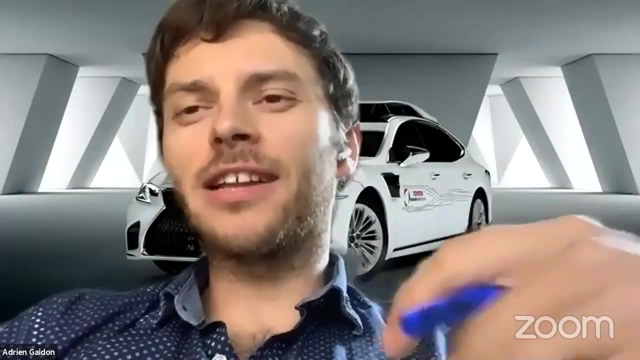 that question is another side of the human elements that Anka is talking about. It's really a social, it's really a sociological question, because what do people really want when they talk about explainability? right, It's something that people like feel, some people feel really strongly about. 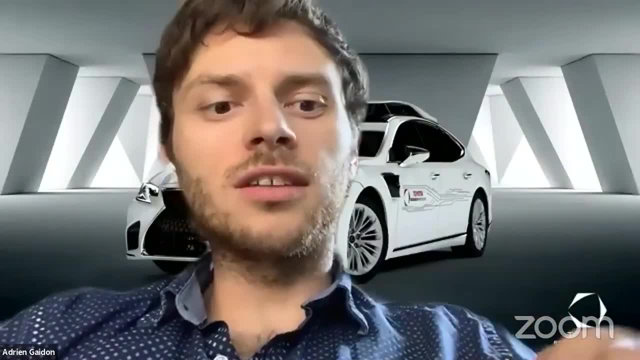 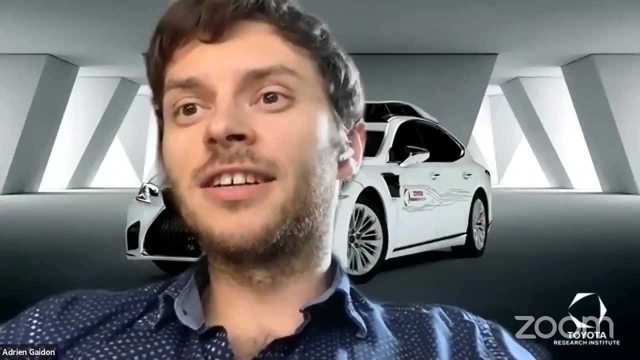 it and really want to do this. I think they just want understanding, right, And? and the reason why they want to understand the system is because they want to delegate some of the decision. I mean, this is the topic of this workshop, right? They want to delegate some decision-making. 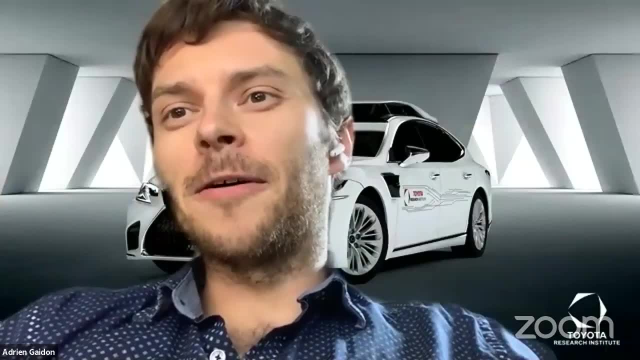 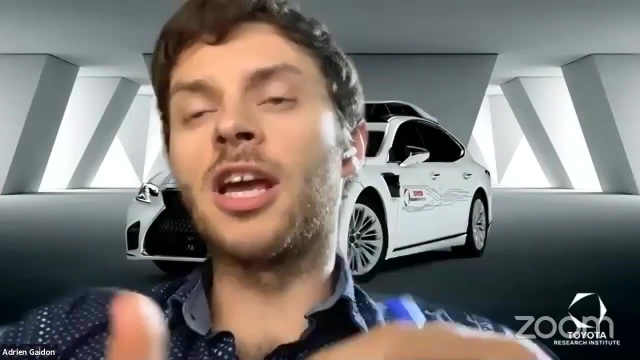 to a robot right And humans want to stay in the loop. I think, like one of the things that you're right, that we're working on is called this garden approach, where we're we're not talking about replacing the human, We're talking about augmenting the human. Eventually, we'll have autonomous cars. 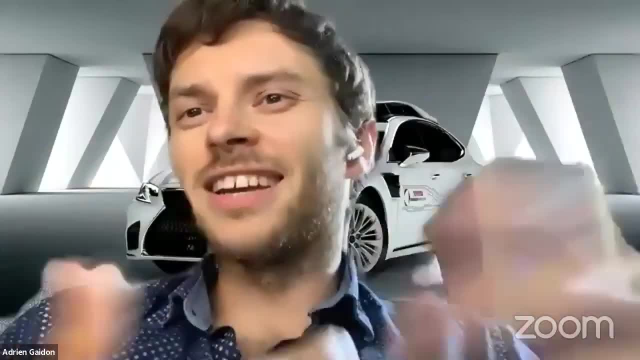 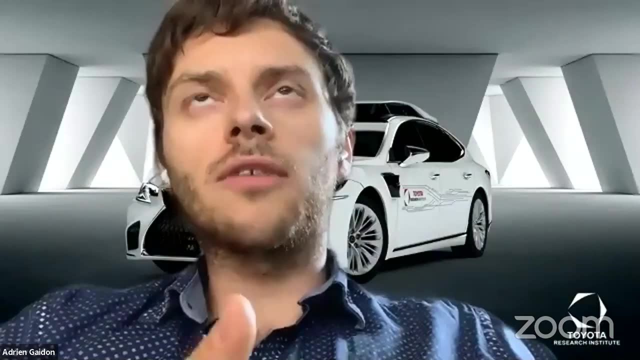 everything. But in the meantime there's 1.35 million people that die every day, every year on the road right, Thank God, not every day, So so. so how do you? kind of, it's a human interaction. 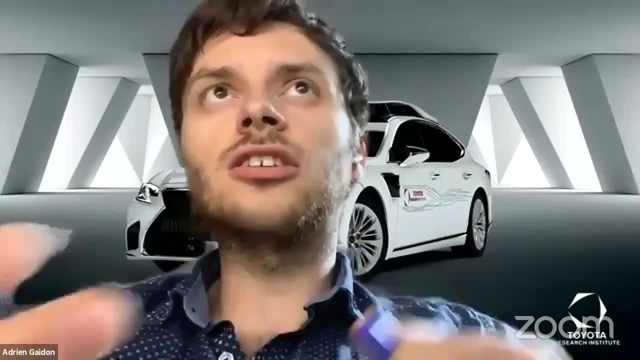 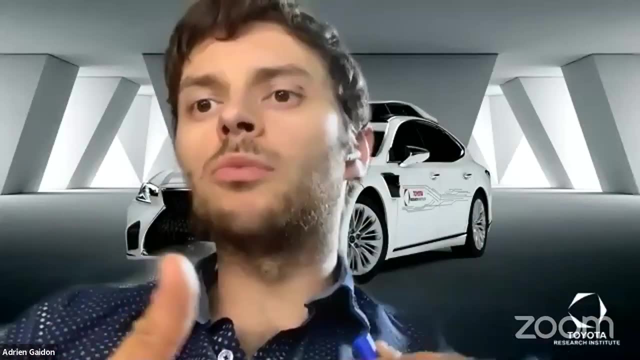 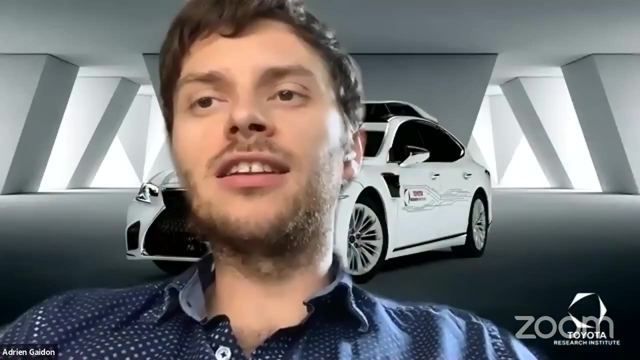 problem, right. How do you communicate decisions a machine would make to a human its approach to risk-taking and and make the human comfortable with letting the machine do that? Potentially over distant time horizons, but potentially in real time? right, And and there's the whole. 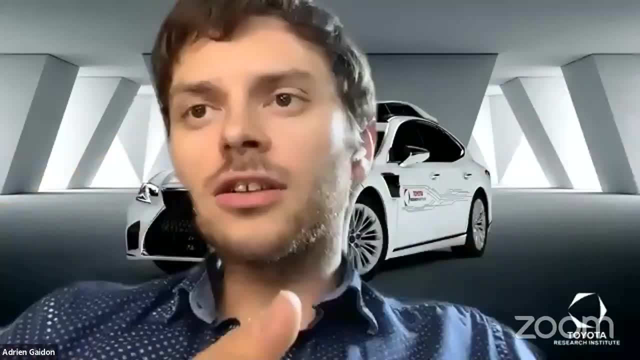 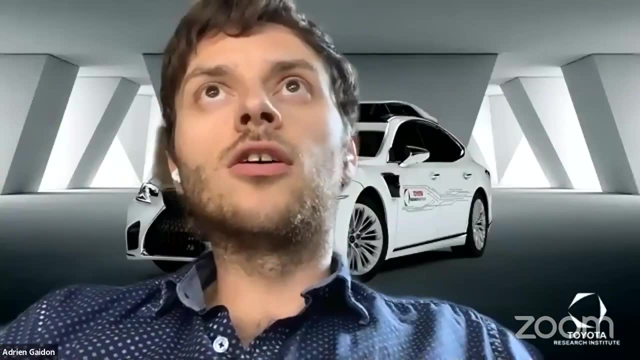 there, right, There's the UX element, there's the human factors, there's the and there's a technological side of it, And but there's also, like the sociological one and the legal one as the question from the, the audience member, And I think that, ultimately, like it's accountability. 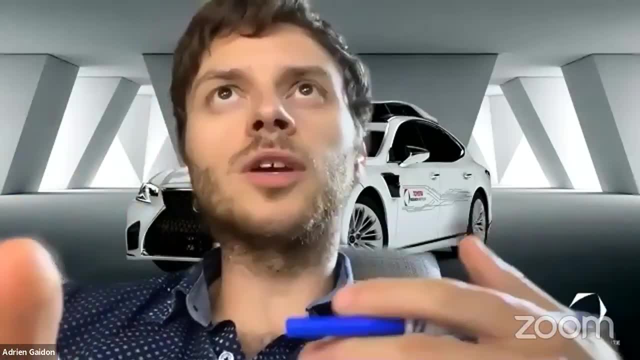 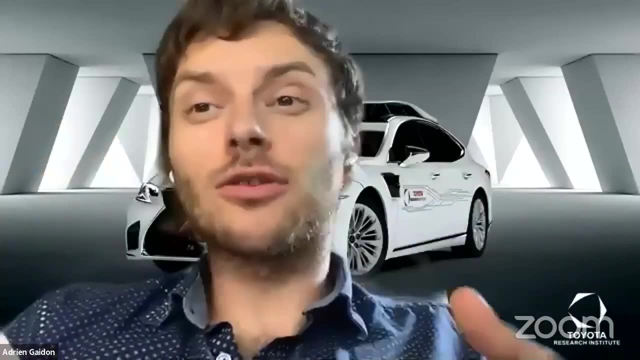 you care about right And and who takes responsibility, And when you think about human robot interaction. there is a decision that the human would like let the robot do it. And even if it lets the robots do it and it thinks the robots communicated clearly, the robot messes up. 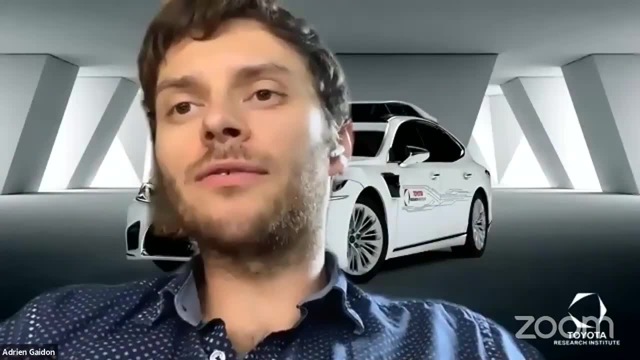 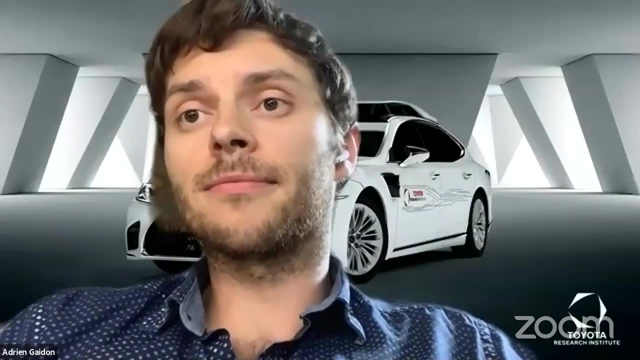 and the human might still say it's the robot's fault, And so ultimately it boils down, I think, to accountability is is is a really big, big question, And that permeates the sociological and the technological issues there. So so we are running out of time very quickly. 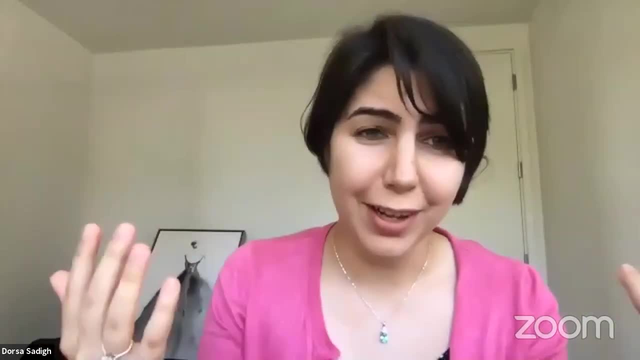 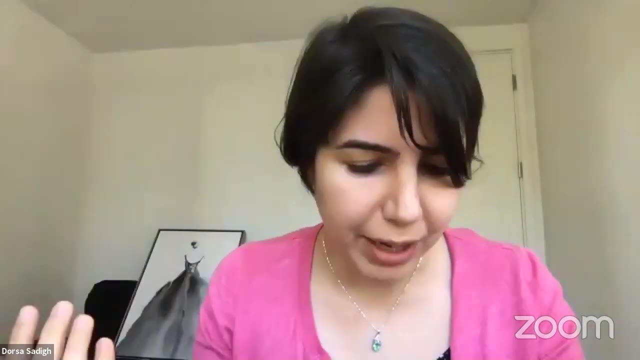 So I do want to just have a final, final question, a final thought, and I would like to hear from everyone about this, So I'll give you guys a little bit to think about it. So I think, in general, when we think about autonomous driving and how we approach autonomous driving, we do use a 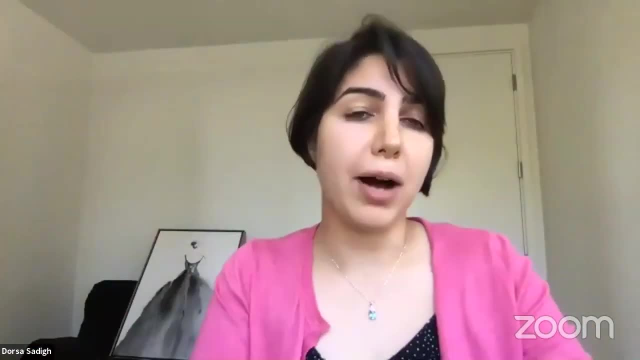 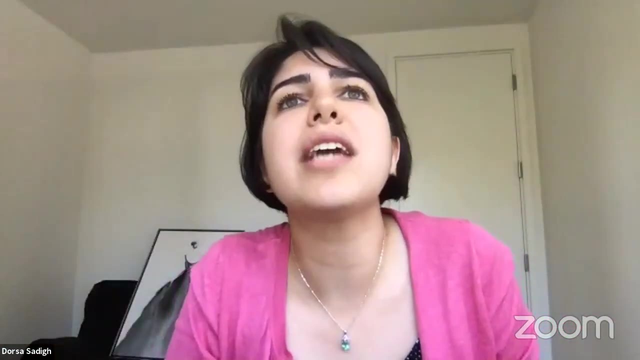 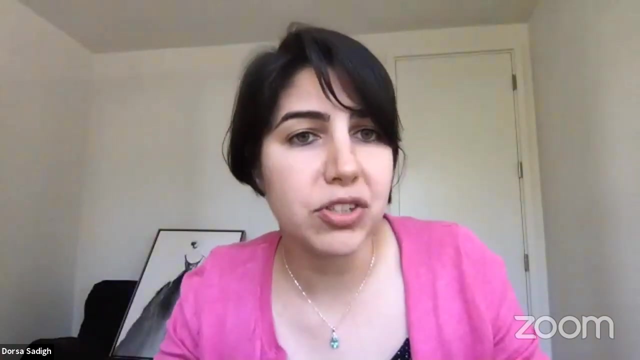 lot of things from robotics and reinforcement learning and machine learning to address problems that exist, and game theory and control to address problems that exist in autonomous driving. The question I have is: what can? what can the field of robotics or in a robotics conference now, what can the field of robotics learn from? from what we have done in autonomous driving over? 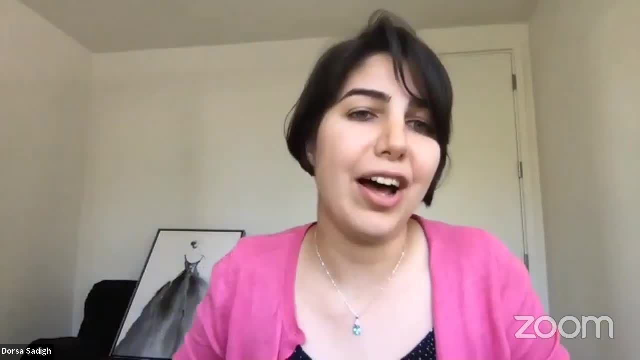 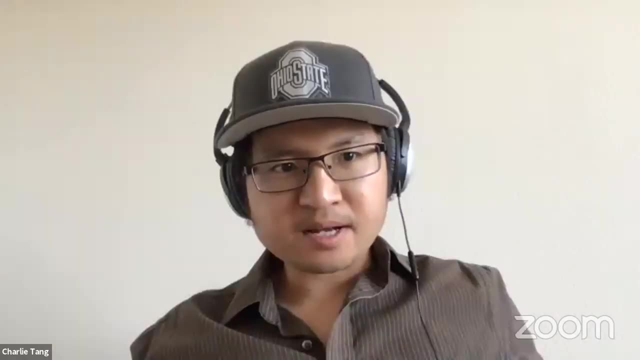 the past decade or so, So so what are the lessons to learn in general for for robotics, based on what we have seen in autonomous driving? I, I think to answer your question. I think the it's a simple sentence, but I would say 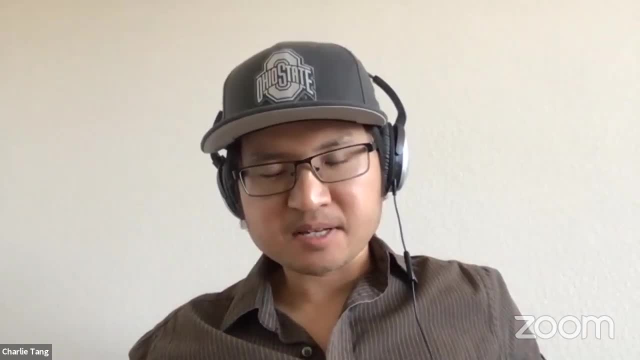 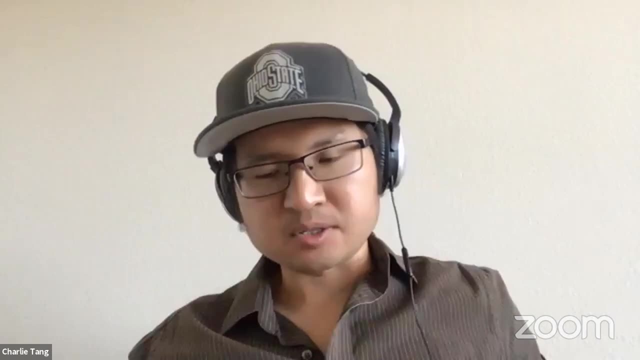 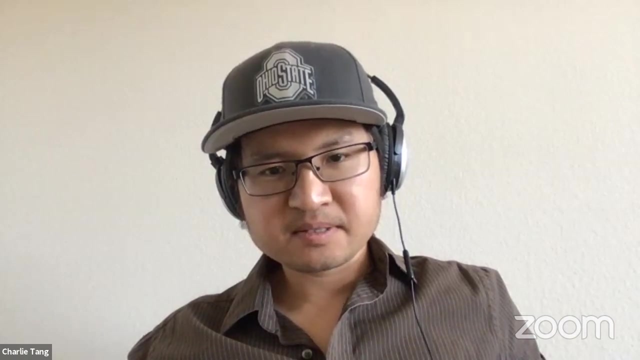 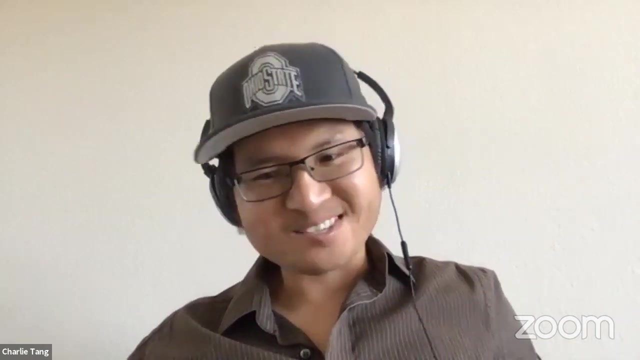 one lesson is the unreasonable effectiveness of data. I think it's not just for self-driving, but I think that would also equally apply to to sort of robotics applications as well. you know, decades ahead, That's it. I mean: just use more data, And I mean: 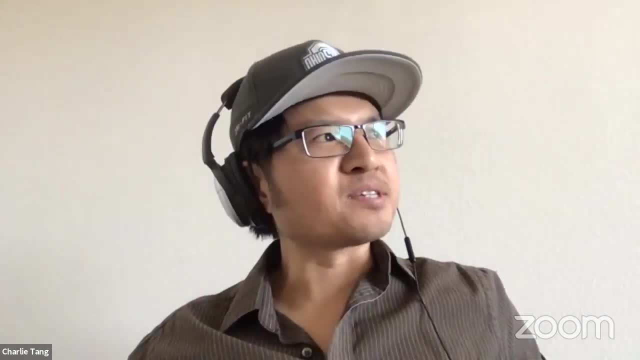 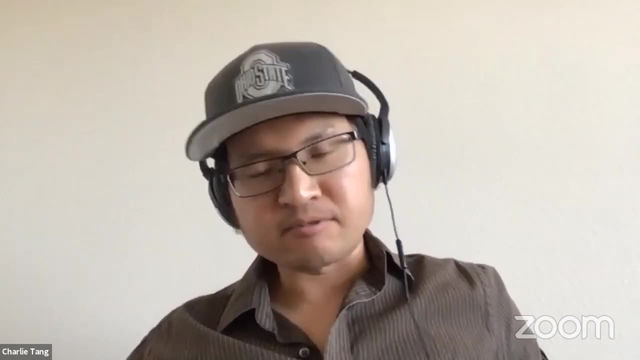 I think I think a lot of sort of you know in my experiences but as as others in the past in related fields, is that as humans- smart people, educated folks- we like to design our own sort of inductive priors, that devices and priors into these, these models. But 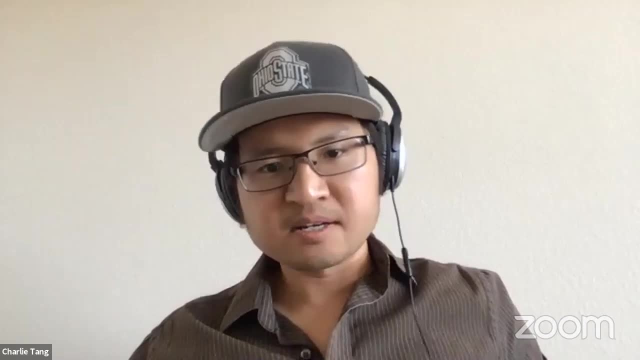 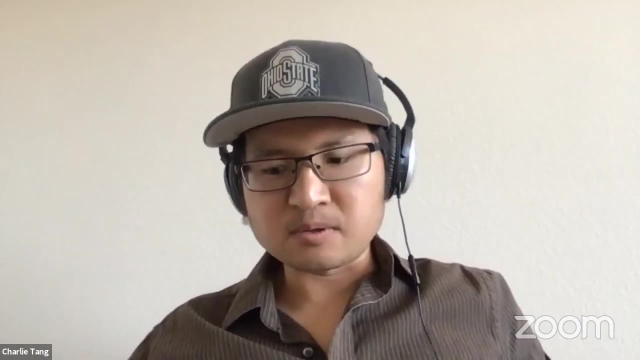 a lot of stuff that other people are doing, like, for example, opening AI with GPT-3. it's just lots of data- might also figure out something similar. So I think there's still lots of room to grow from that that aspect. but you know, safety criticalness, model-based planning, I think that's. 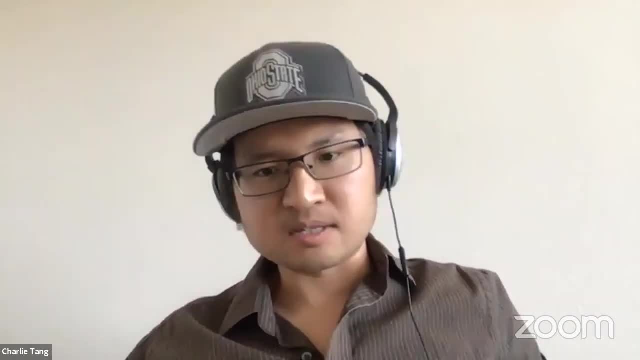 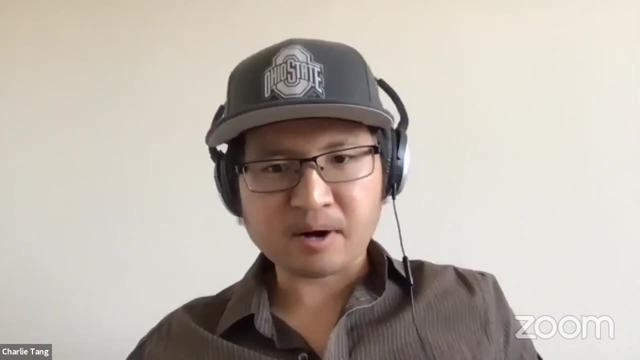 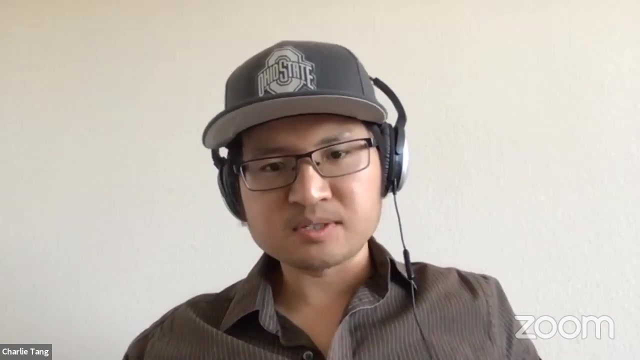 something that's particular to our application. Also, robotics is safety critical is a key key there. So I don't think it's just the same as generating awesome texts and paragraphs and chatbots and things like that, But, but I do think that that where where you can leverage the data- 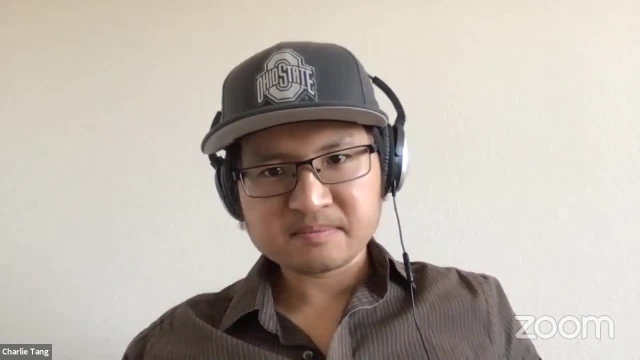 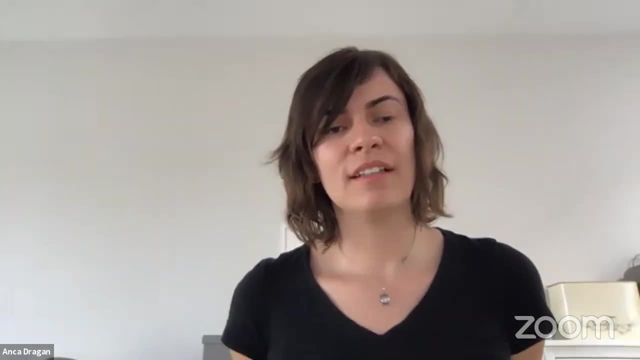 that's a big advantage that you can leverage the data to do it. Sarah Garskevich. General final thoughts are okay. Dr Maria Torgalski, I have a half answer, which is: which is, I mean, maybe kind of a personal thing for me. 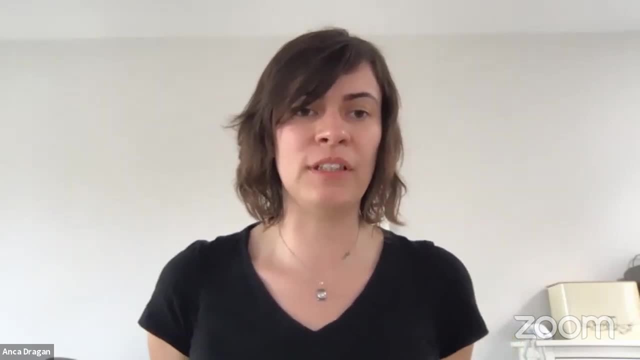 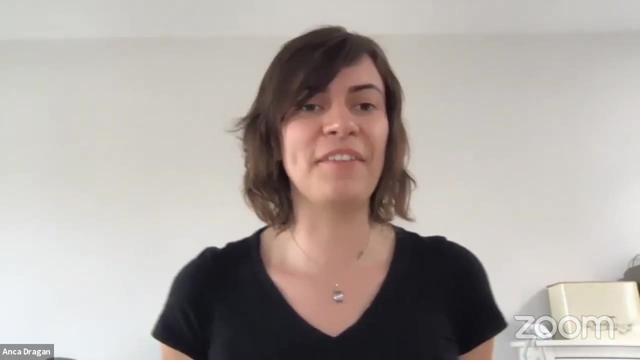 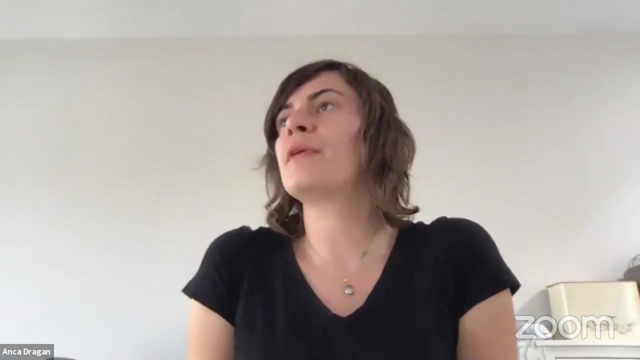 So I used to work in algorithms for interaction but in manipulation And and then Dorsak convinced me to get into autonomous driving when I joined Berkeley and we started working on the game theoretic stuff together And Um and I the. the reason I liked it so much is because all of the sudden I didn't have to. 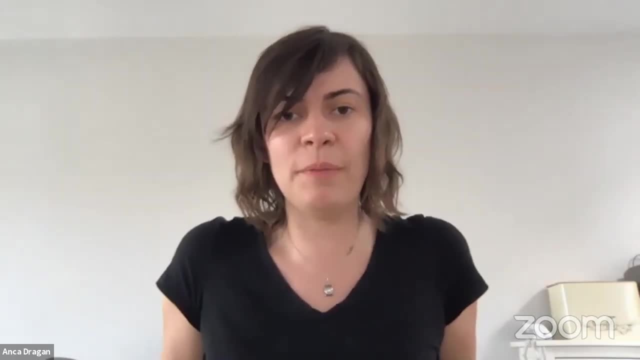 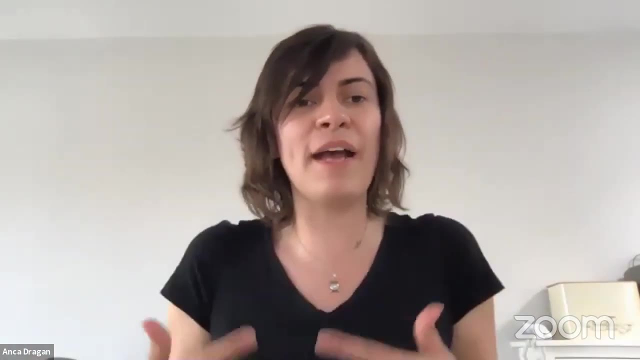 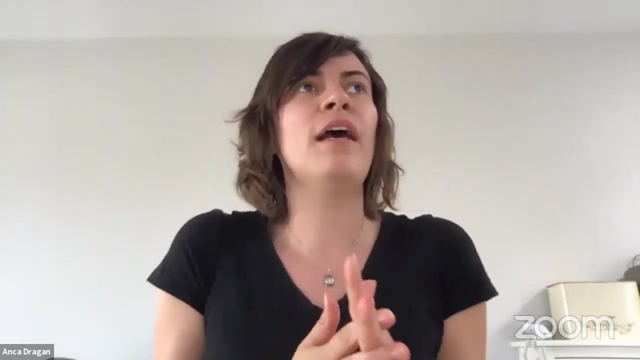 hypothesize capability, physical functional capability. It was there and it all broke when it came to people, And so you know, I guess the way I maybe say this is is that a lesson, at least from my very narrow way of looking at the problem, is that you can go very far without 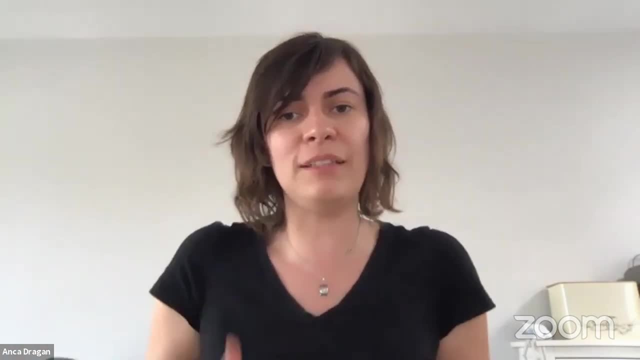 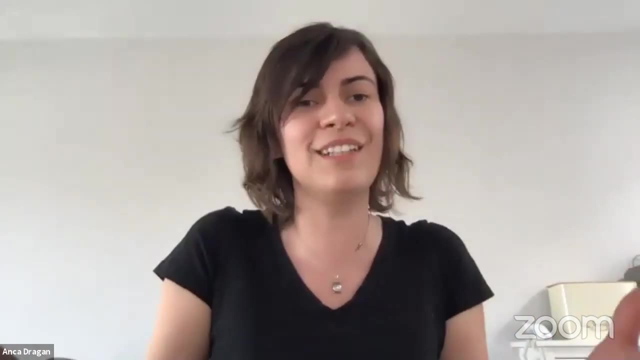 taking without putting the people into the equation, And it might seem to you like you're making great progress, And then you might develop these approaches that, when it comes to solving the real problem, which includes the darn people, um are, are just not, are not going to cut it. 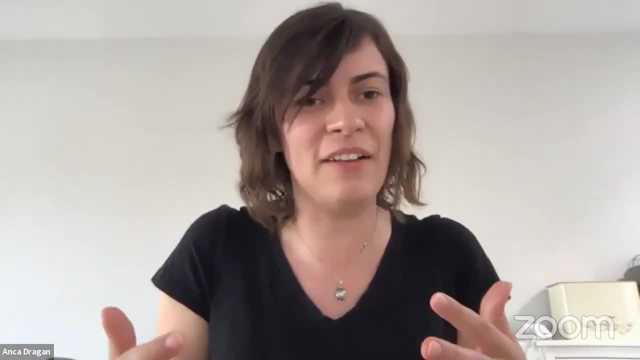 And so you kind of have to go, go back and then and then think about how you're going to solve the problem again, Um, so I think that's, that's a lesson, but I love what you said, Dorsa, too. 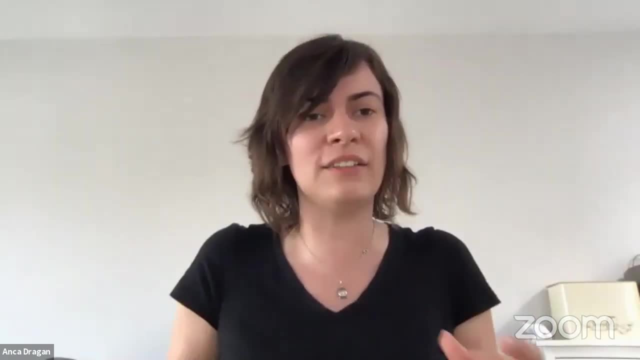 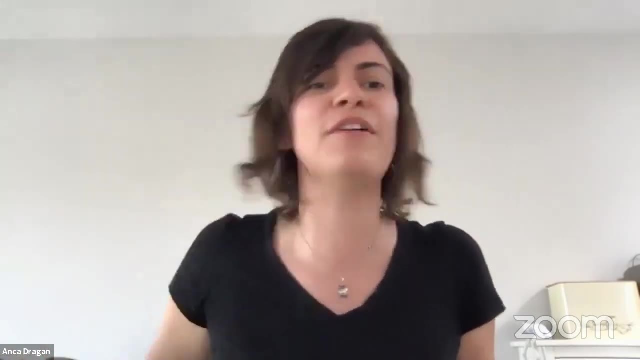 about just a very interdisciplinary like: do whatever it takes to solve the problem is something that the- the driving community, I think- has really well. first of all, put it in the real world, because you never know what's going to happen until you put it in the real world, And I think that's. 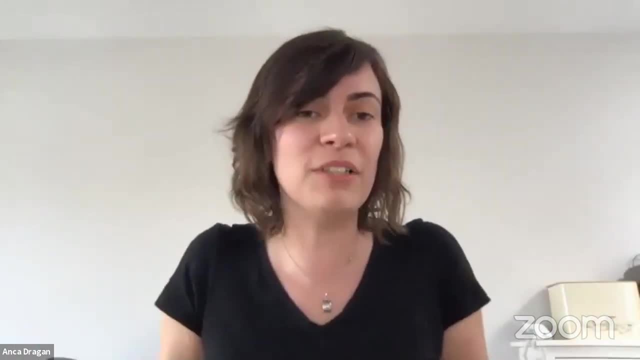 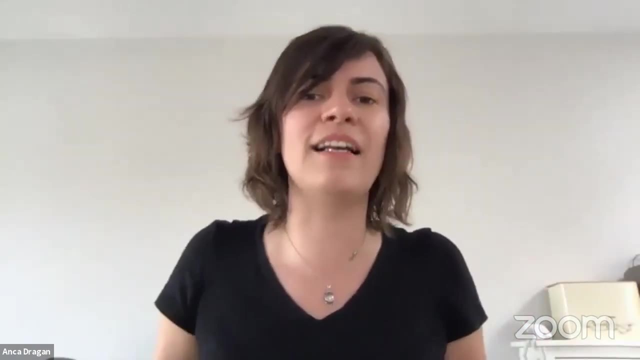 something that roboticists can embrace too, Right, Um, and a lot of them do, And then also just like whatever, whatever tool that you, you know, whatever combination of tools make sense. that's what's going to cut it. So it's not. you know, it's not. you know I do this. So 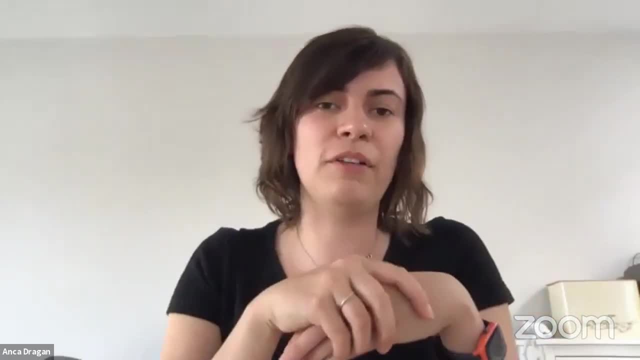 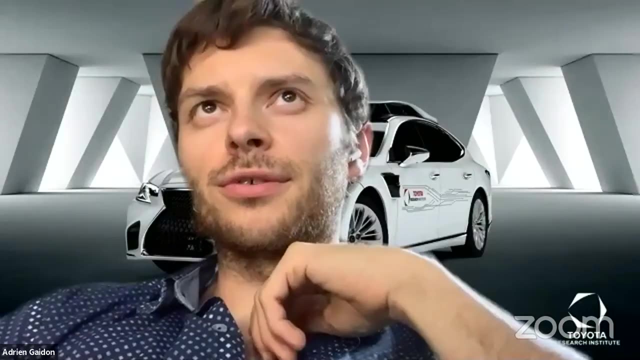 therefore, I'm going to try to approach the problem in this way, but really thinking about what the right combo or what the right tool is, without being too, um, religious about it. Yeah, I completely agree with that. I mean, for me it's just like I thought it was very. 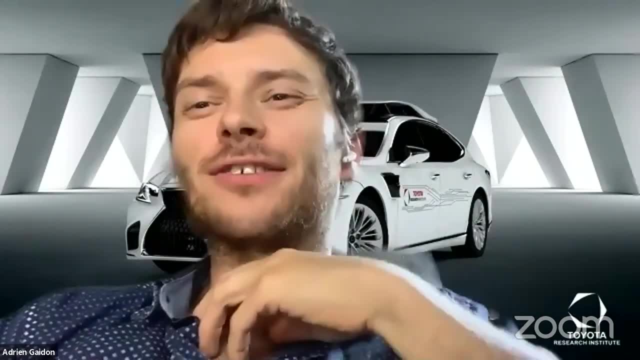 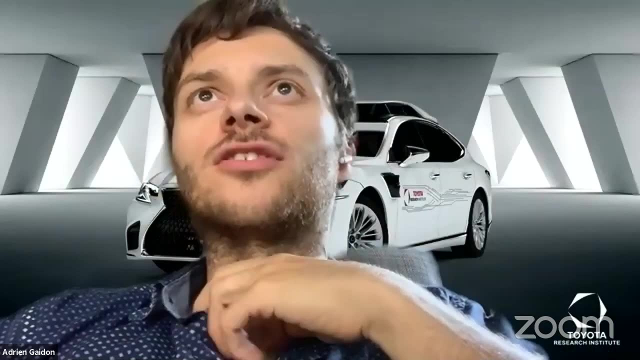 hard problem. I realize it's harder than I thought, And so I think that's kind of like. the conclusion over these past 10 years is that in 2009 or even 2012,. people thought they were there. Um, it's just hard, It's just really really hard. So, and it takes. 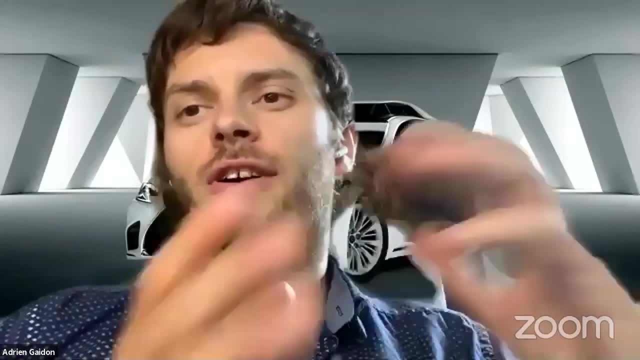 a village, right. So the reason it's hard is because it's the full stack. It's very complex. uh, from like. it's not just robotics, It's not just machine learning. You know, it's not a CNN that's going to solve it. I believe in data. 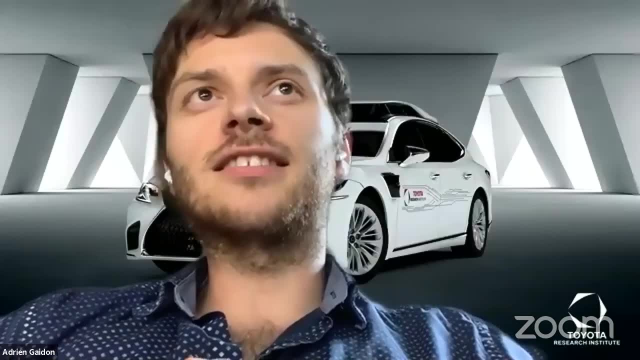 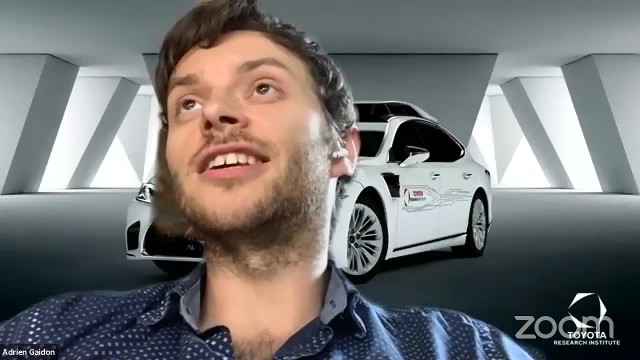 I'm a machine learning guy, but it's everything And that's that's the thing I learned the most in the last three years is that I- I just counted actually- I had 62 different collaborators in in in like three years, which is nuts, And I realized like, why, like? 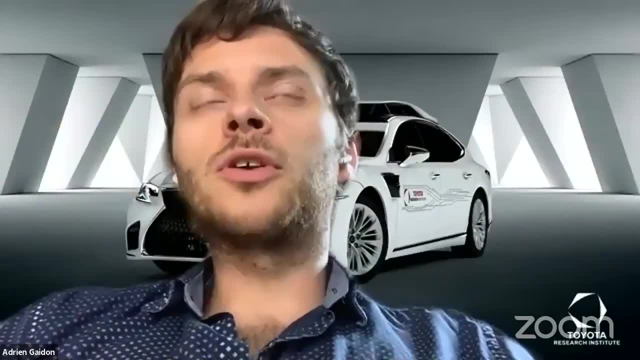 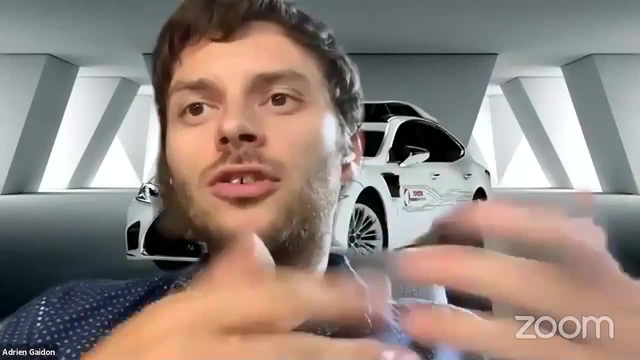 am I just such a social animal? And it's just no, because you know, when you collaborate in computer vision, you collaborate with like you have a group of people right That you collaborate with right And you you have your circle. Um, but when I joined and started, 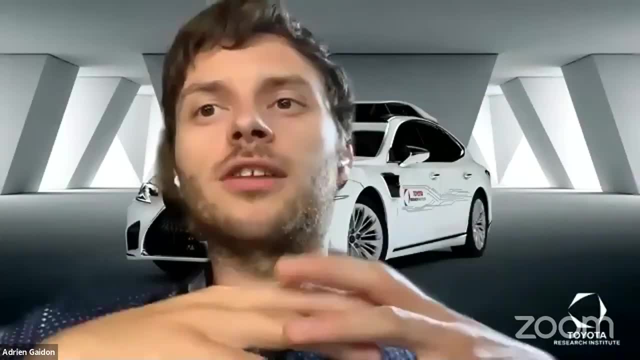 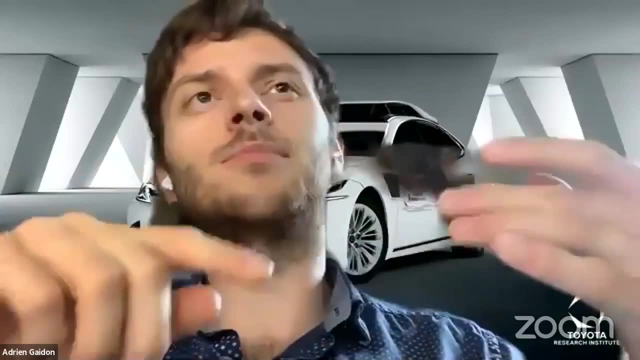 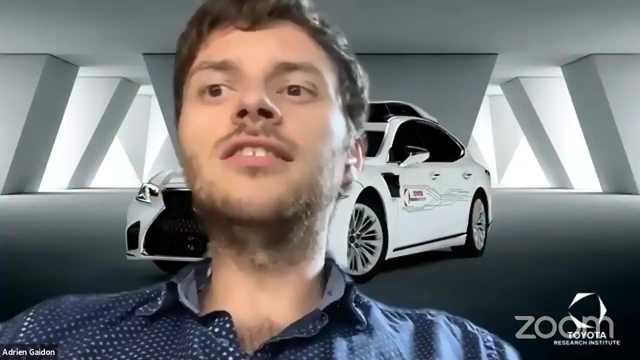 autonomous driving. suddenly my network exploded and I collaborated with people like like you, with like like robotics and people that had the human interaction experience, people that had like hardware experience, people that had control experience. It's just insane The breadth of technical knowledge that you need to just be you know at the current 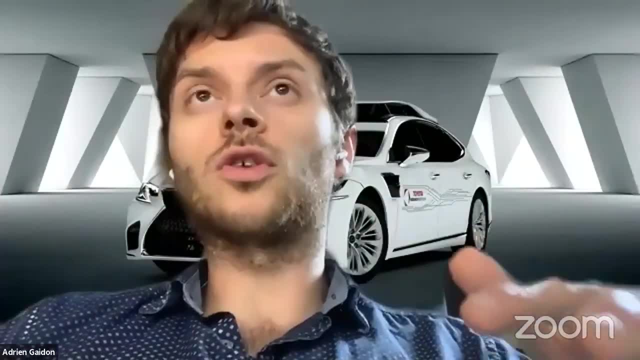 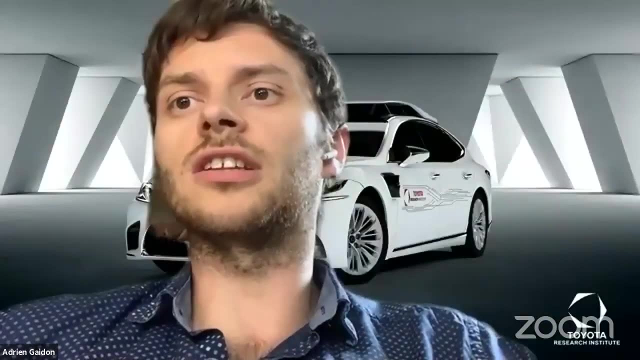 state of the art, which doesn't work, which which is by no means salt, So so. so the current envelope of knowledge you need for autonomous driving is huge, and you need to go even beyond that. So it really takes a village. It's, it's, it's going to be a massive. 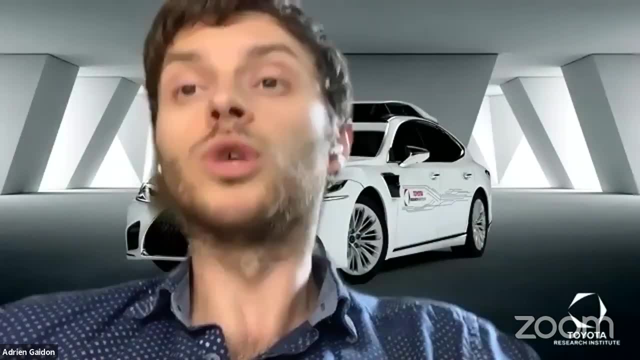 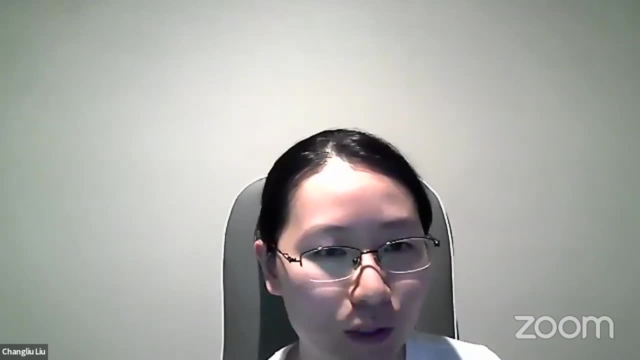 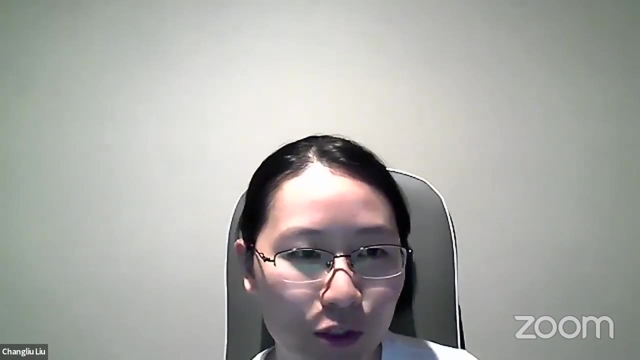 collaborative effort If we ever going to get to a real, real solution to this. Yeah, I totally agree with what has been said before And also I want to add to one point. I think the autonomous driving is a very rich problem which go beyond technology and which 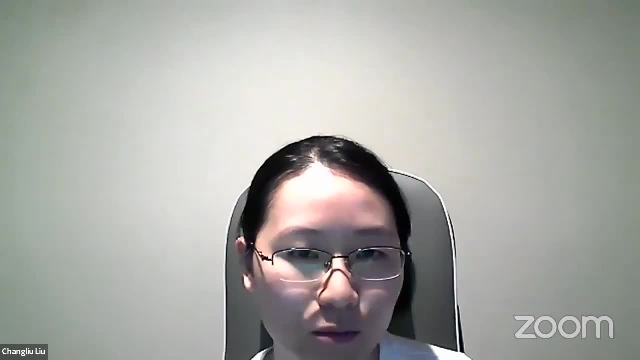 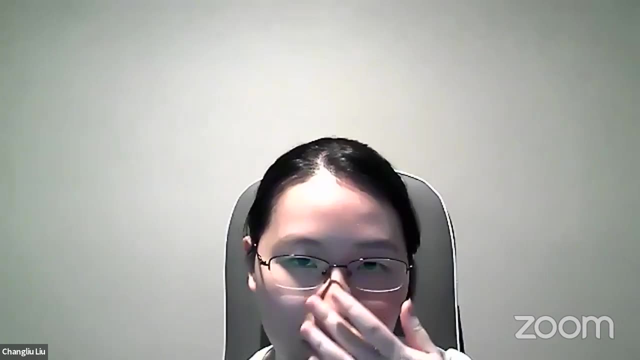 in order to make it come true, we need to think about more ethics problems, more like economic problems, more um politics and societal problems. And, uh, even you know I'm a big proponent of the idea of like, if we want to build a robot, we need to be able. 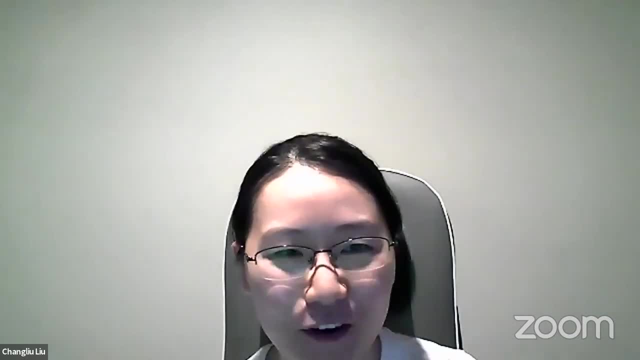 to build a robot that works on a humanoid robot. Yeah Yeah, None of those problems are easy to solve, as um we as researchers developing codes or writing equations, And I think similar stuff can also happen in the robotics field. For example, if we want to bring a humanoid robot into the real world, the same thing, 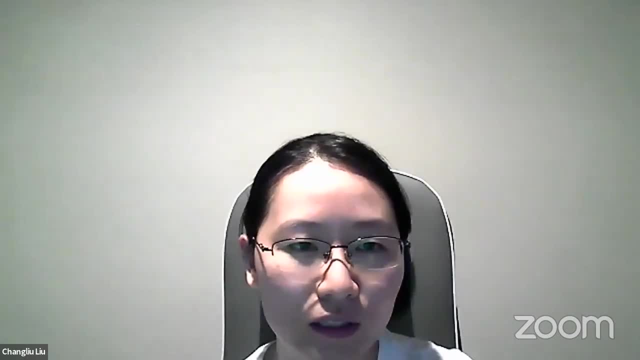 can happen. We need to account for a lot of things, but this also gave us an opportunity to, like um, carefully look at the pain point of the market- where is the true needs are, and then modify the problem and then develop technologies that can solve the pain points and maybe this way can it can allow us. 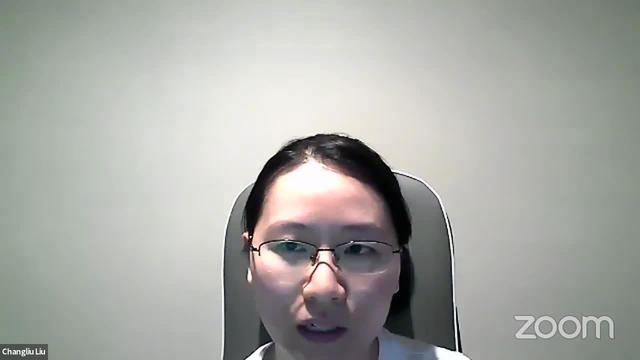 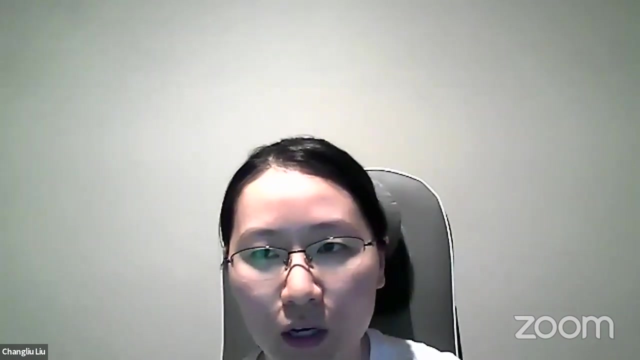 to avoid some unrealistic assumption or some truly relax some truly difficult problem using some constraints in the real world. for example, if we have communication, then a lot of prediction problems can be solved using communication in the autonomous driving. yeah, so this actually enriches the problem a lot and also we can bring this kind of idea into the robotic research. 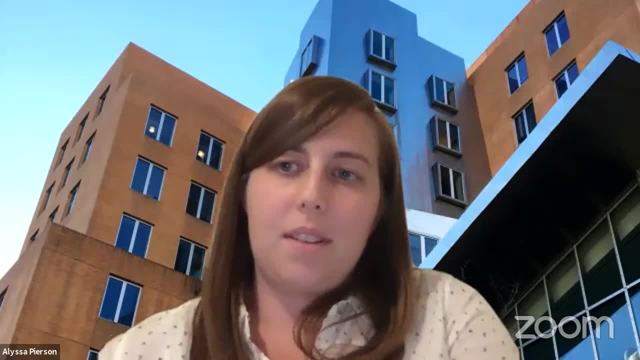 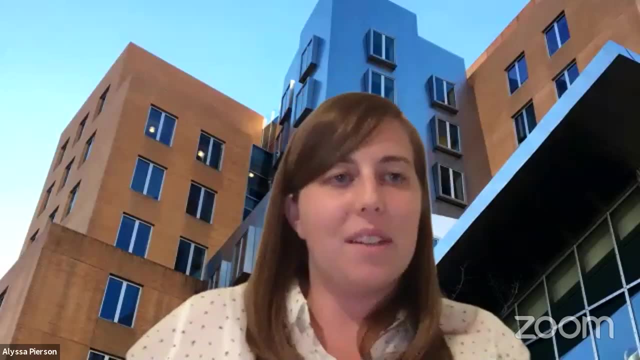 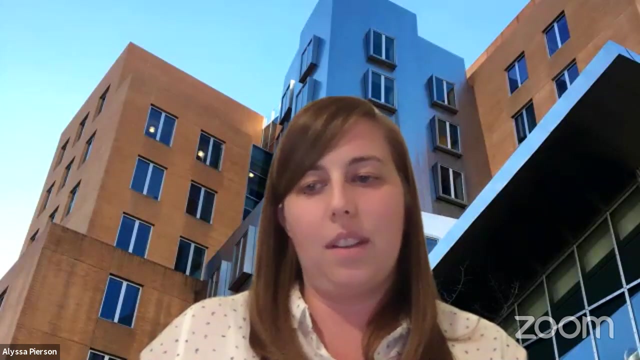 i think. uh, if i can add, so i was um. so i was a roboticist firmly in the multi-robot camp before jumping into autonomous driving over the past few years and my background was working with little you know, 100 three inch wide robots and trying to make a bunch of really stupid robots do smart things. 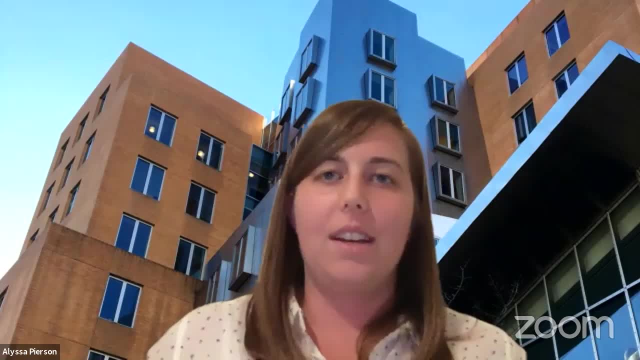 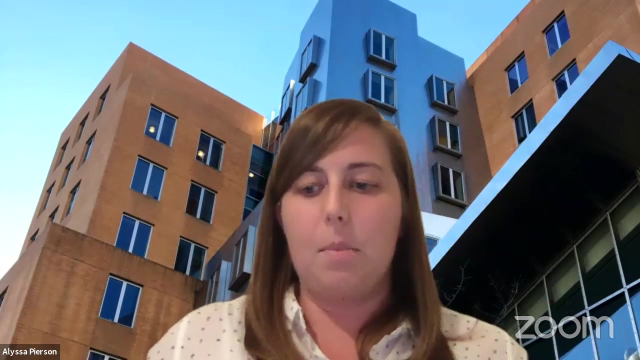 and autonomous driving is completely different, because you have very, very complex, very, very, uh, technically capable smart hardware and you just want to do it, make it do just what we think of as like a very stupid thing of just driving down the road, um, but i think of of what maybe? 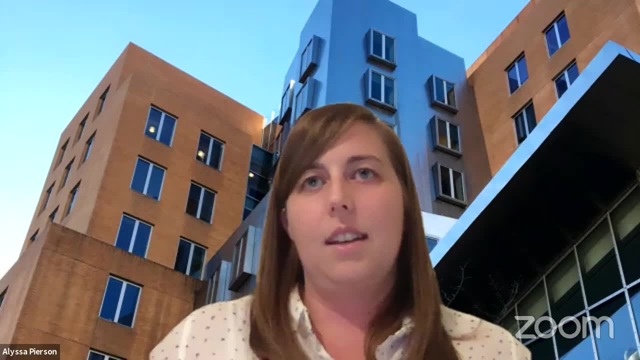 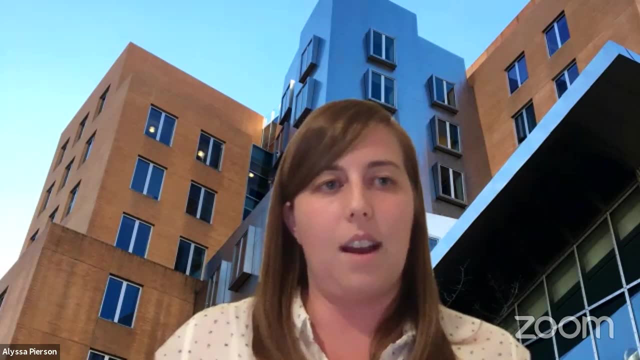 roboticists can take away from this. well, i think one thing that i've noticed- and it's been a really great opportunity to dive a little bit deeper in the digital world- is that i think that we can- and you know, like, when we have things really interesting, a lot of it's about like, like, can we use this to help solve problems? 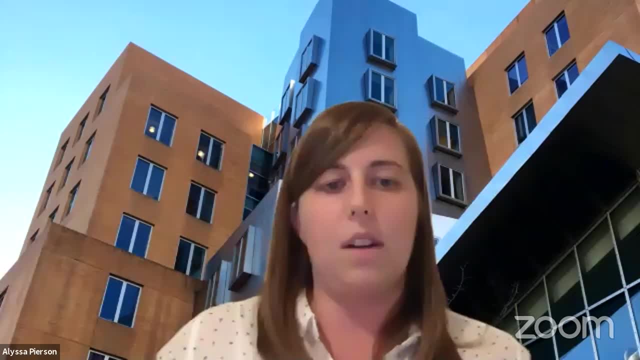 and how can we outsource this to the communities. but i think that being able to keep things to works, it's something i'm really proud of helping people to have. like you know, i'm absolutely looking forward to doing things like this, but also i think this product is a really great 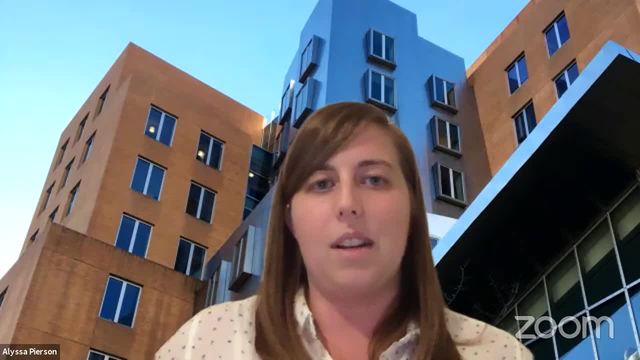 idea for the entire community is that to not be afraid to think of your problem as becoming much more complex than it is. to not be afraid, instead of just thinking of one tiny example of an environment with a limited number of interactions and you're a controls person, so we're just going to say perception is solved- but to really integrate all of that into the solution and also get your software organization in order. software management matters, especially as your problem scales. 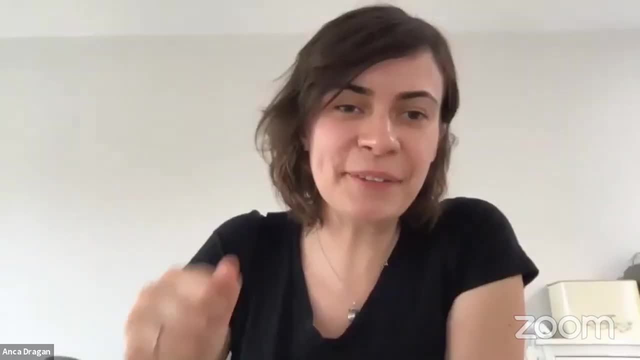 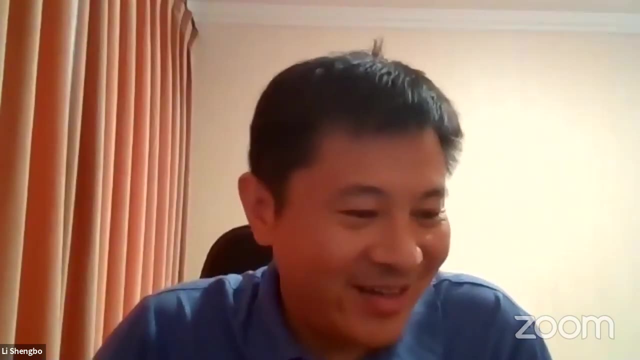 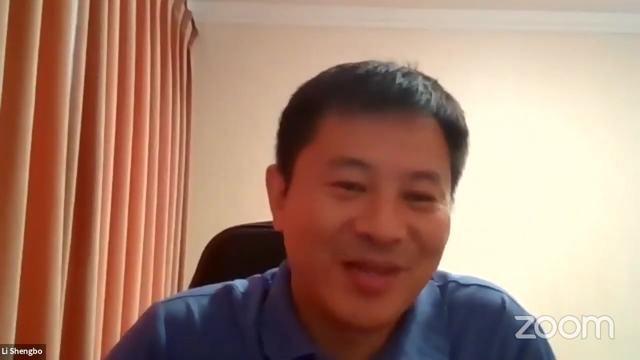 And the long tail is really long. It's a long road. I probably want to add some information First. I think we need to be optimistic about autonomous driving. So long as we can wait, finally, we can get a good autonomous driving system right. 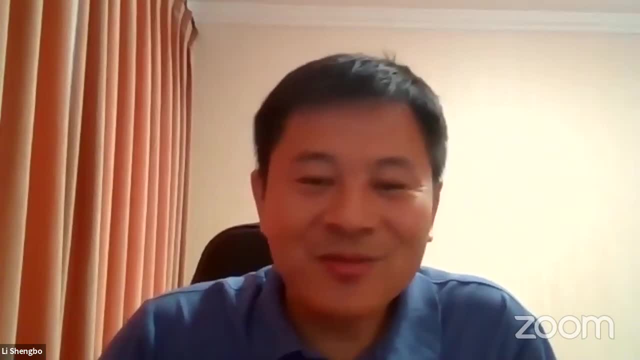 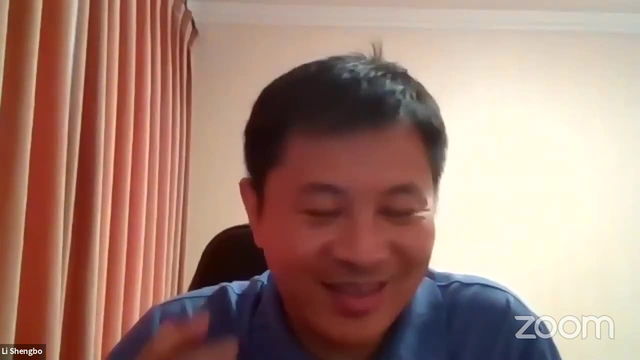 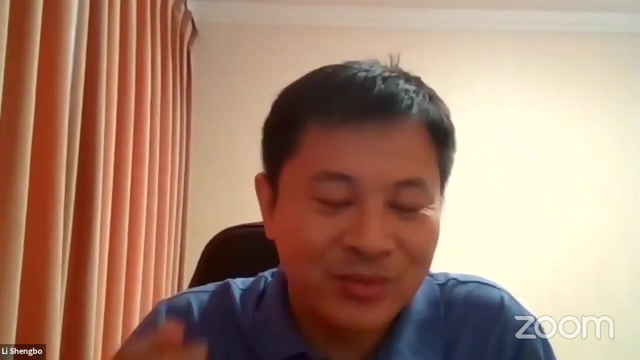 And second, I want to say so I agree with what people said, that technology is stupid And what's the clearest thing in this world is a weak human brain. right, We need to turn our idea, to turn our view to our human brain. 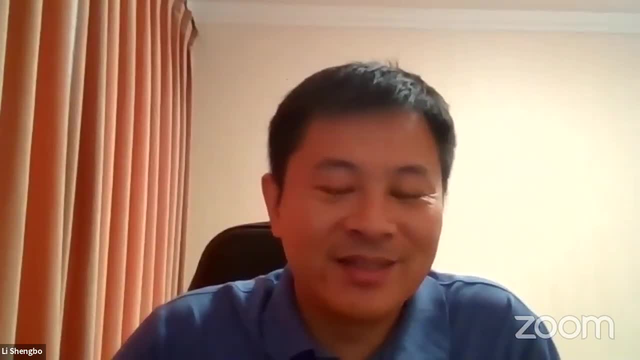 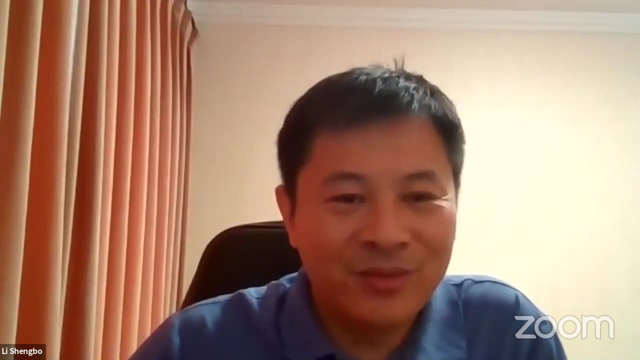 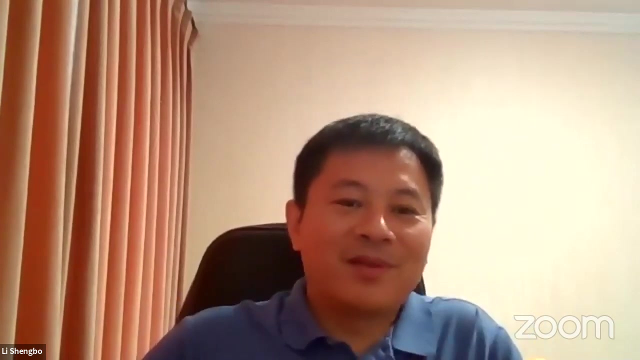 So how does this brain work and how can we get a new idea from the brain working mechanism? Maybe it's a good way to put new technology into autonomous vehicle R&D. This is my advice, Thank you, Thank you. Thank you very much for this topic. 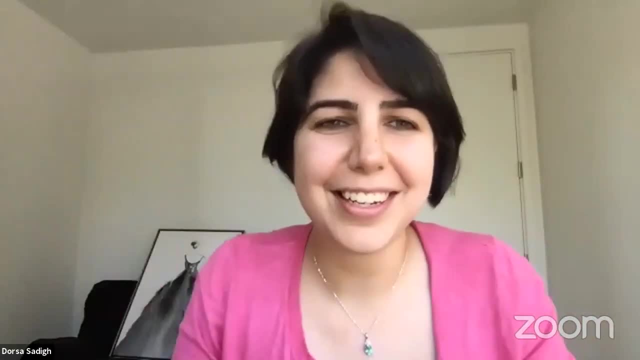 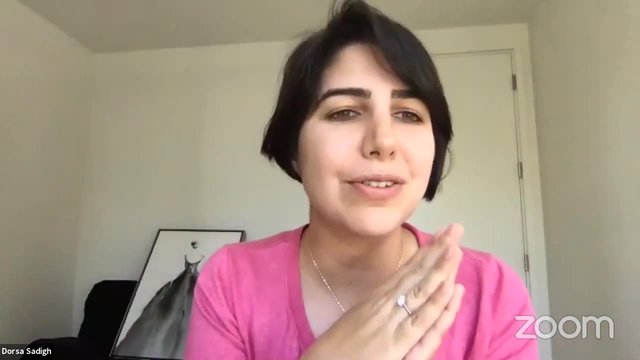 All right, Thank you so much. All great thoughts, Great, great ideas. It was really fun doing this panel with you guys, so I'm going to just now thank you all and switch to Rovon and Igor to take it away. 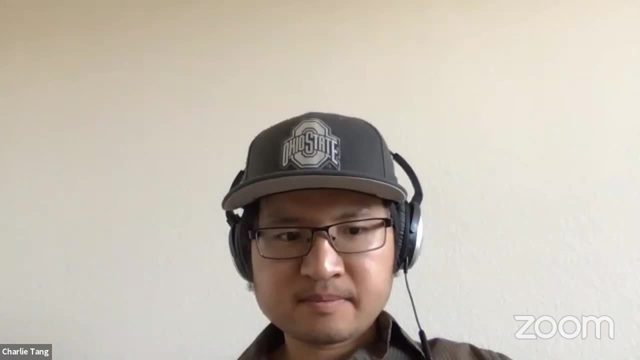 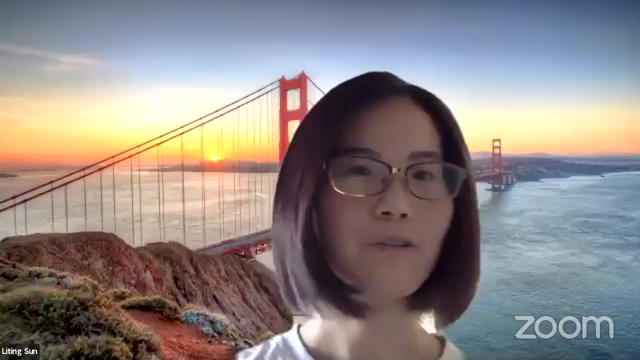 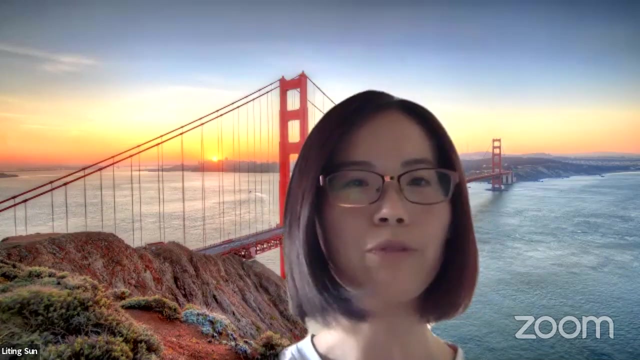 Thank you, Tuos, Thank you, Thank you, Thank you, Hi. Thank you for what a wonderful panel And I really enjoyed it a lot, And thank you very much for all the panelists for the wonderful discussion, And also thank you very much, Roza, for moderating the panel. 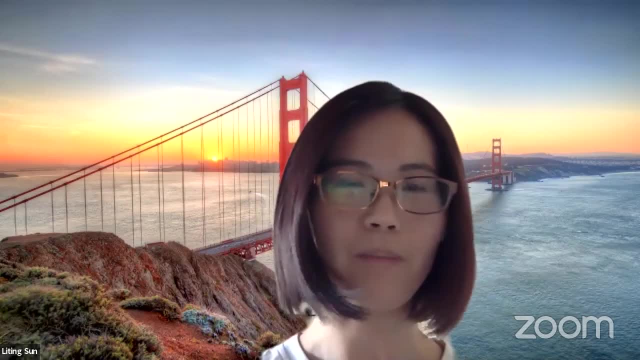 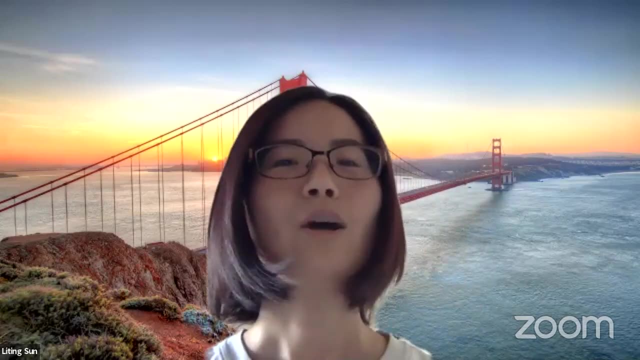 So that can actually be the perfect ending of this workshop. But just before we go, I would like to announce one last scheduled item, which is a little bit surprising schedule, which is the Best Paper Award. We have actually accepted many good contributions. 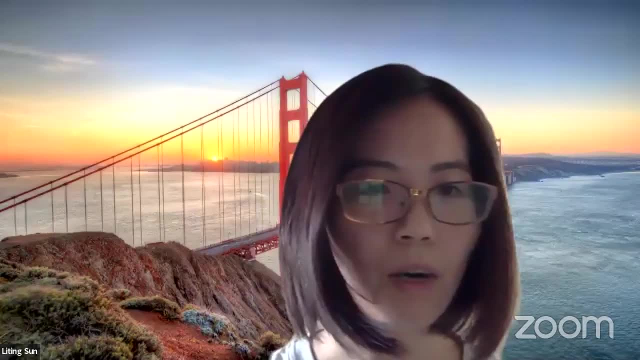 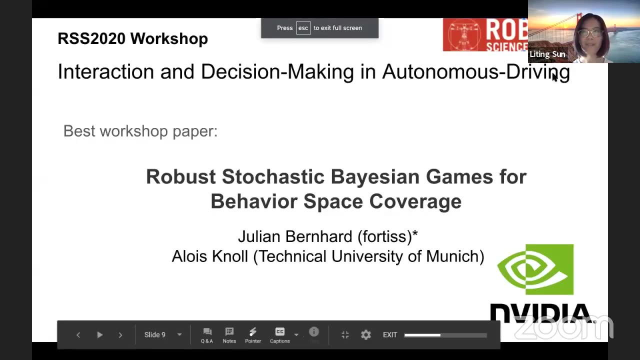 Among them, we selected one Best Paper, Which is the. Let me present it. I think I need to present it to show them. Yeah, Okay, The Best Paper is Robust, Stochastic Variation Gain for Behavior-Based Coverage. The authors are Julian Behard and Alois Knoll.